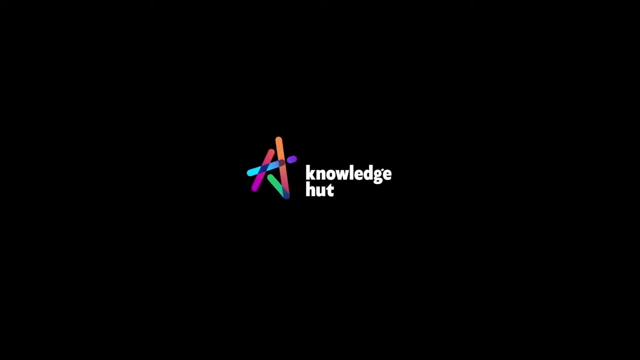 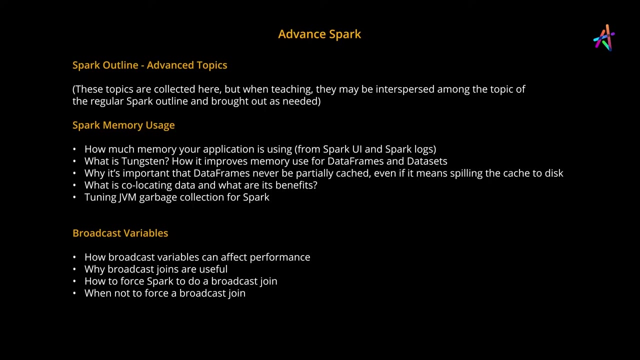 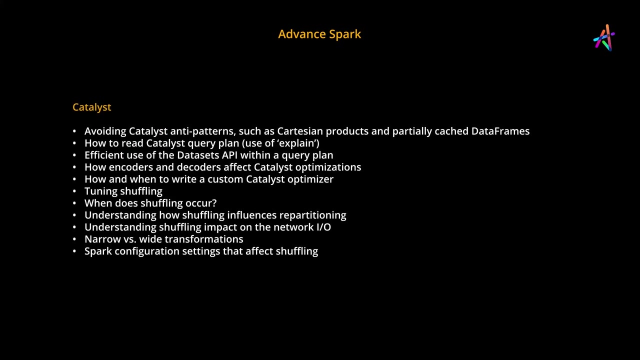 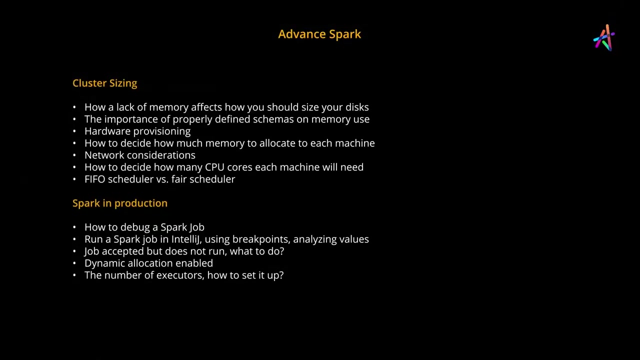 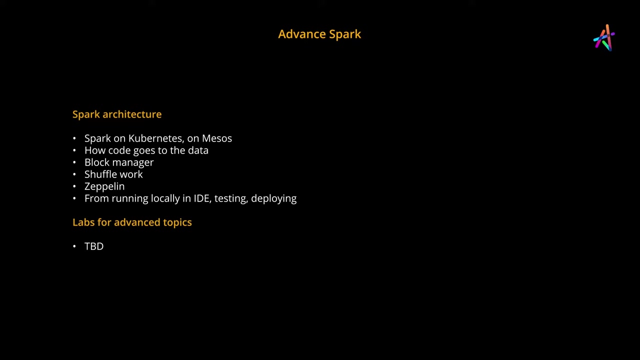 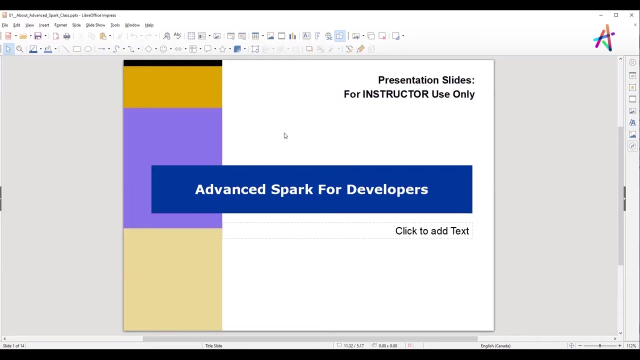 Thank you for watching. Thank you for watching Our course, Advanced Spark for developers, and what we're going to be doing is kind of kicking off with sort of a general introduction, a couple of housekeeping points. We're going for the next four hours, so we'll take about a 10-minute break, about two hours in 10-15 minutes, just so people can get up and get some activity in, and something like that. 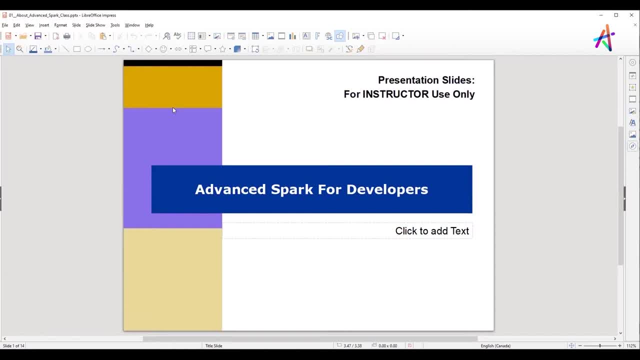 You know just, we need that cognitive break. We are going to be- I'll go through these slides just a moment, but just to kind of keep some other things in mind. We're going to be doing this for six days, four hours a day. 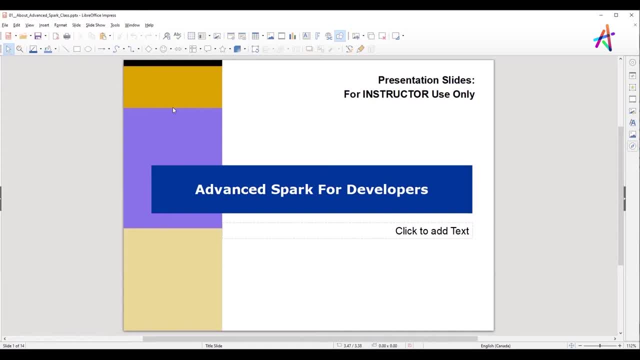 So it's a little bit different than just blasting our way through it. We're really- and we'll kind of tune this as we go along- but the general plan I'm getting is to sort of spend the first little while delving into the architecture and 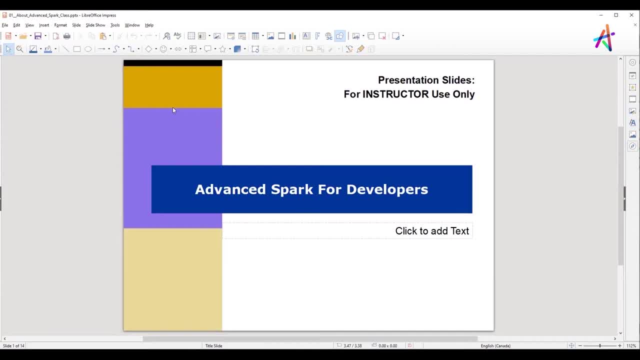 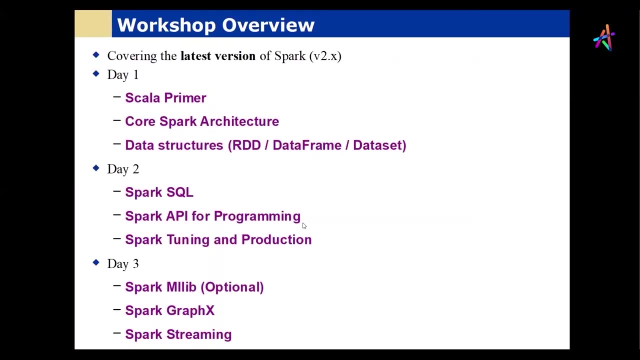 a lot of the conceptual ideas that form the foundation of Spark and related concepts, And then next week we'll really delve deeply into the tuning aspects of it And once we have a foundation on which to build. So this is kind of- or this is assuming- a kind of- a three-fold day approach. 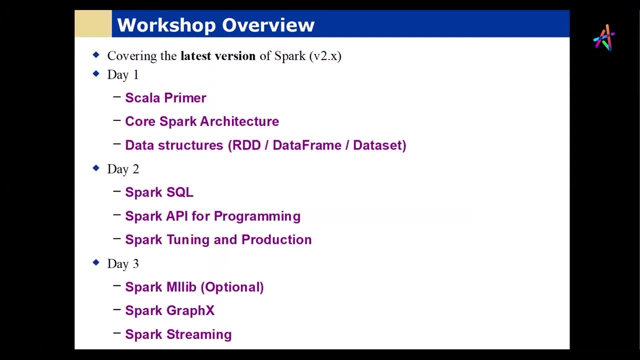 So we will focus on Scala in the beginning, And this is an important concept because, since Spark is written in Scala, many of the ideas of Scala are inherited into Spark. So sometimes understanding what Scala does from a conceptual point of view helps understand why Spark is doing the things that it's doing. 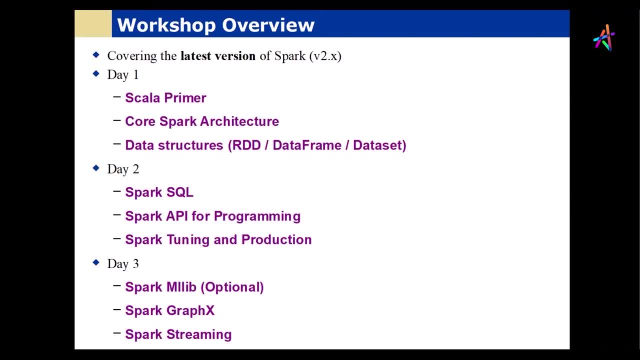 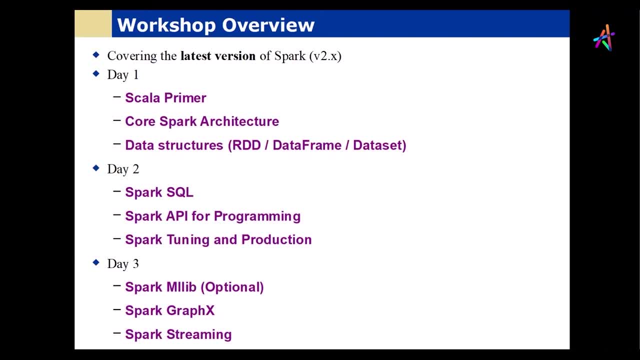 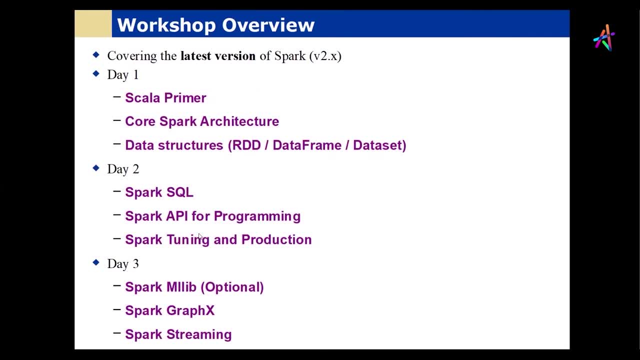 Since there are some topics we want to kind of add into there. That's the general plan. That's the general plan. Like I said, this plan is modifiable as we go along in tuning things up. There we go: Prerequisites and expectations. 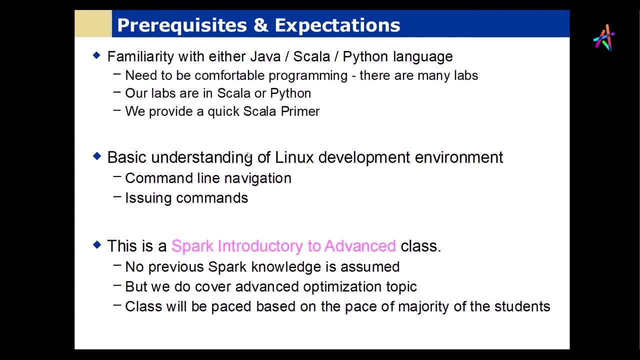 The request was made, specifically that we focus on Scala. This general programming model allows you to actually work in a number of languages, But we are going to focus conceptually on Scala and some of the other things as well. But we are going to focus conceptually on Scala and some of the other things as well. 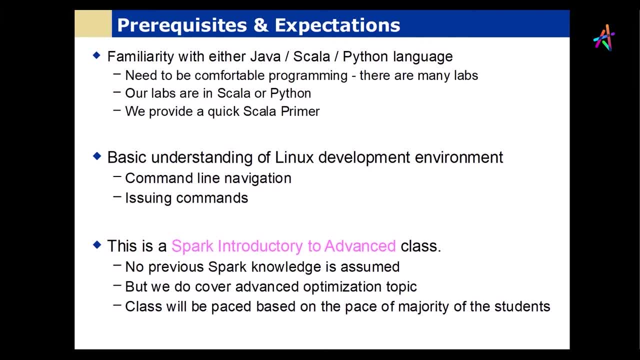 But we are going to focus conceptually on Scala and some of the other things as well. We will do a quick Scala primer. I am going to go a little bit beyond that because I want to get to the conceptual part of Scala And we're going to assume that you all have some basic familiarity with Java or equivalent object oriented programming, since those concepts will start to come up in various points in the course. 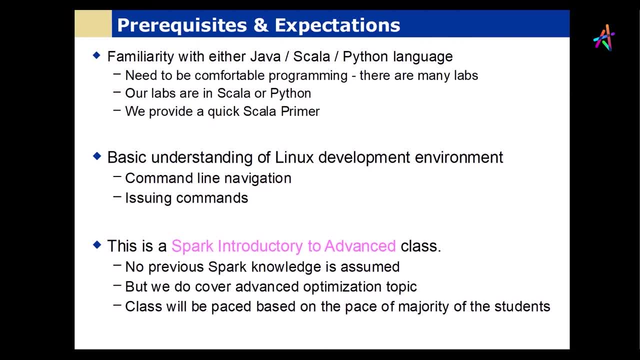 You should be able to work in a Linux environment And we will be using some virtual machines. I'll be assigning those out later today for you to experiment. And we will be using some virtual machines. I'll be assigning those out later today for you to experiment. 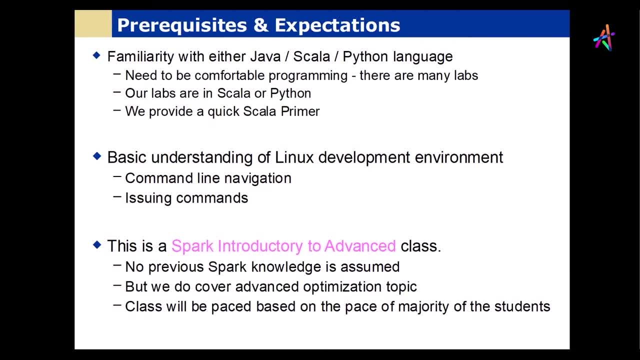 And we will be using some virtual machines. And we will be using some virtual machines And we'll have a full environment in there. So one of the things that I do want to caution you about is that if you're going to be experimental about things, you should experiment in the virtual machines that we give you, not in any of your own machines, because the virtual machines are no consequences environment. 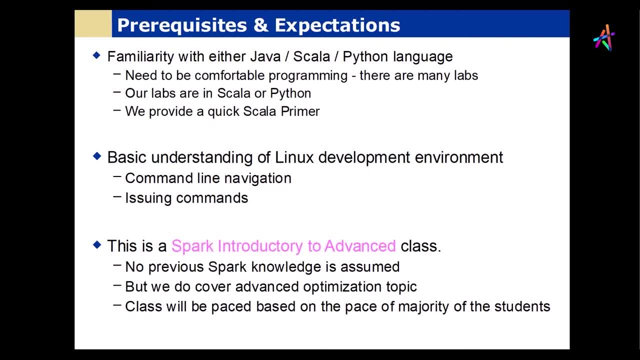 What that means. if something goes terribly wrong, we'll just restart the instance and get you back into a clean environment. We are not assuming Any knowledge of Spark, although you may have some, So I don't want to find out what everybody's skill levels in these areas are in just a moment. 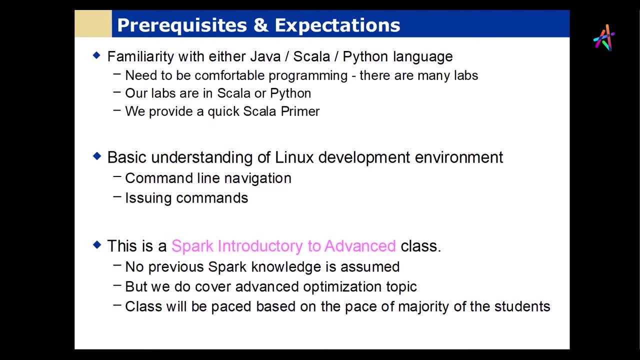 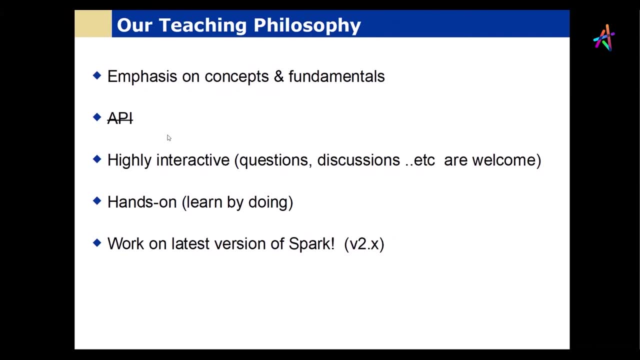 But we are going to focus- I said particularly Monday, Tuesday, Wednesday next week. we're going to be focusing really on advanced optimization and optimization techniques and the underlying optimization technology And we will adjust the class as we go along. A couple of things I'll just mention here. 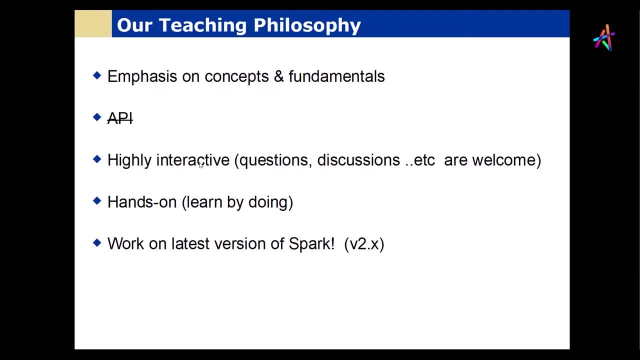 This is kind of standard stock slides, But first of all, this is the first time I'm teaching from this set of materials, So I sometimes might have to fumble around a little bit to figure out where things are. But do bear with me. 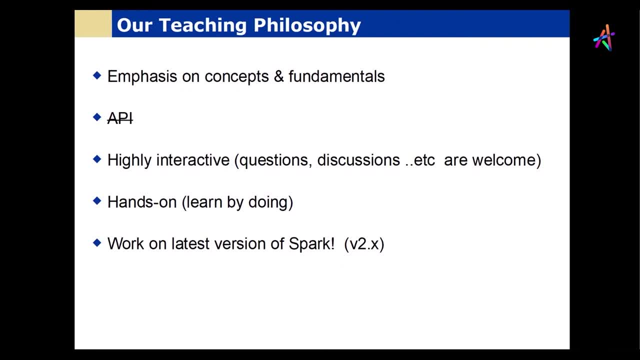 We'll get that sorted out. I've just gotten a hold of all the production materials a little while ago, So I was still sort of going through it then, matching up what I wanted to teach with what was in the various slides and various labs. 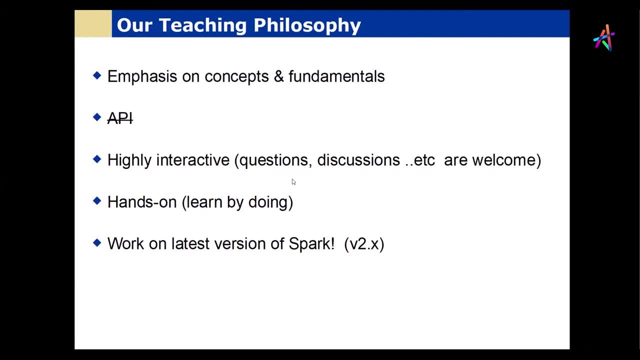 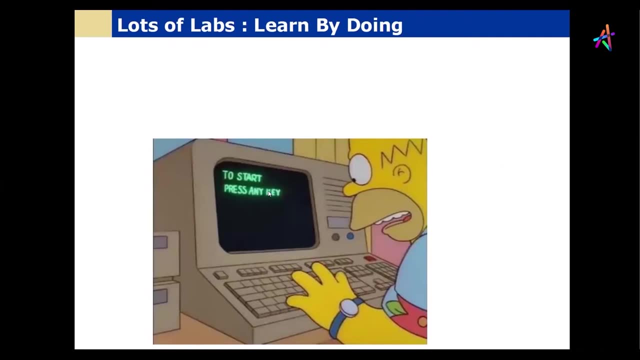 So I'm still making that matching here. So keep that in mind. The labs are by doing- we're going to be doing- lots of labs. Again, I'm going to encourage you: be experimental if you want. If you break something, it doesn't really matter. 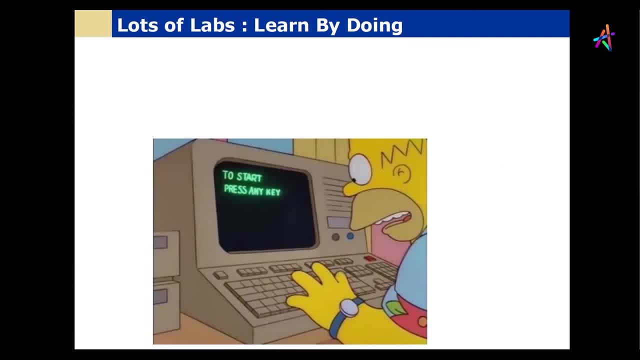 We'll just start it up again, But please don't be experimental in your own environment, because you don't want to screw up any of your own internal settings Or any of your environments. So we're going to assume that we know all of this idea, that we're going to learn the theory, which is what we're going to be talking about. 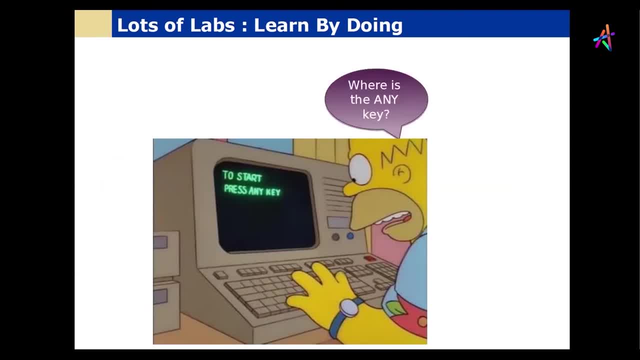 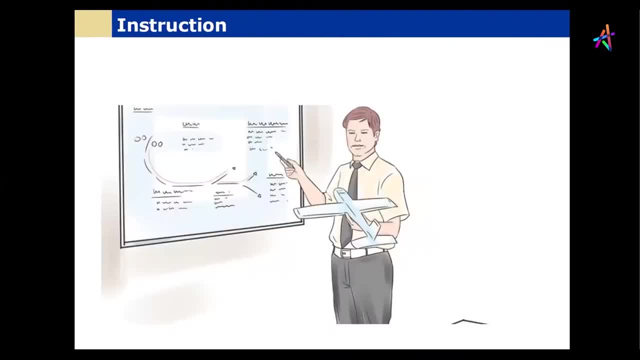 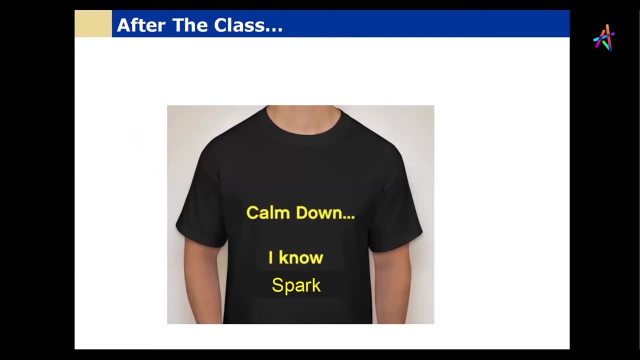 And then you're going to go and practice out a number of different exercises to reinforce the particular theory. That's the overall concept here. These are kind of cool images. There we go. Somebody's done some nice photoshopping there, So we're going to get to. 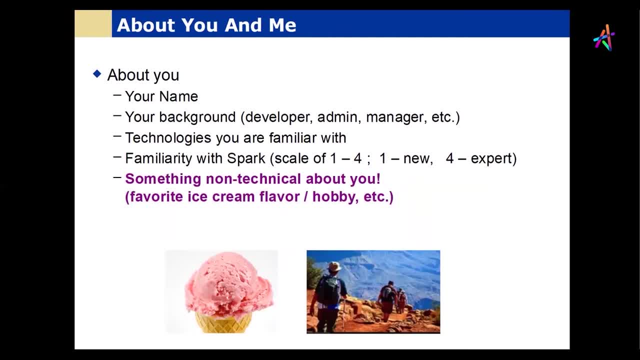 We're going to get to the actual start of the course now. It's kind of done that housekeeping. The other bit of housekeeping that I would like to do is with regards to the Zoom. I haven't used Zoom to teach a course. 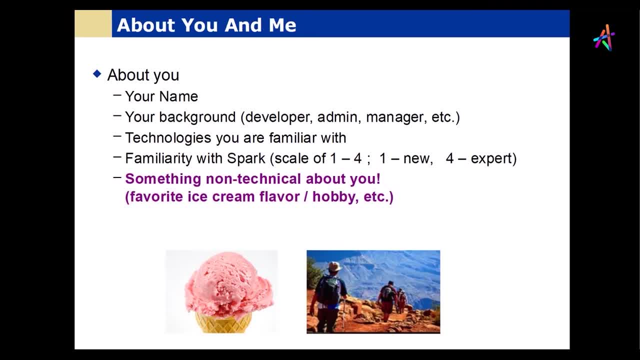 I've only used it for conferences. So I do believe there I'm trying to figure out- if there is a I've got to share and I'm there is a chat. So if you do feel you want to chat me, I will try and keep the chat window open while I'm lecturing so I can respond to those. 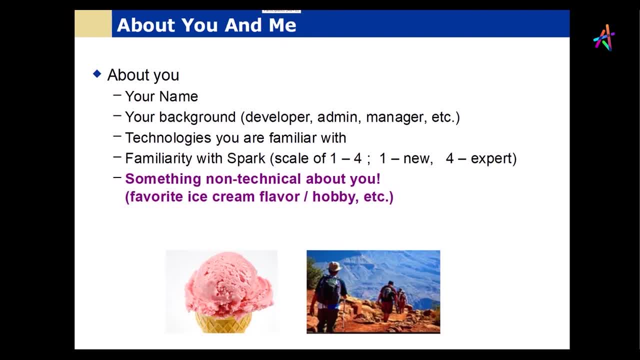 If you're chatting and I'm not responding, you may want to just give me a verbal heads up that you're chatting. Let me see. Is there anything else that we want to mention? I think that's probably the important thing. You can just speak up as we go along. 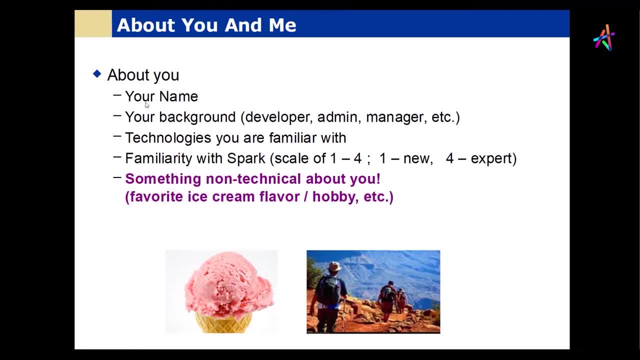 So I'm going to ask you all to give me a little bit of feedback on this, more or less aligned with this template. The purple or Violet thing down here- something non-technical about you- Not mandatory If I'm going to replace that actually with something else. 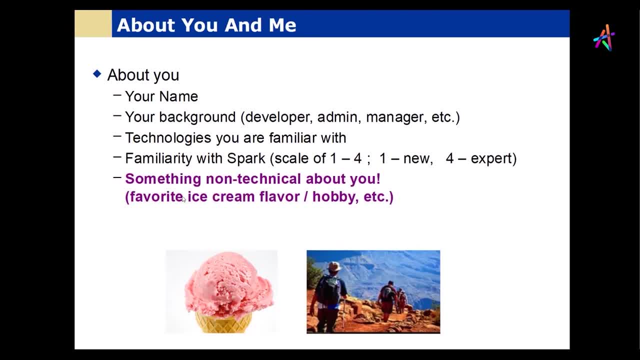 So we'll start with your name, your background And I'm also curious what your current role is, because sometimes that's not the same as your background. Very often technical people wind up as managers or team leads, Technologies that you are familiar with. 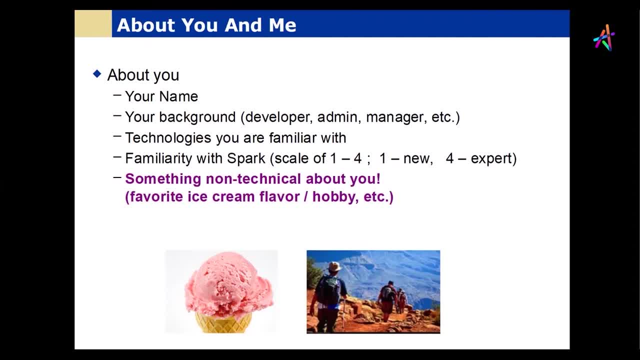 Again, technologies that are related To your work with Spark. So if you are very good at the piano, that's not something that's really quite relevant- Interesting but not relevant. And also I want to know about your familiarity with Spark. 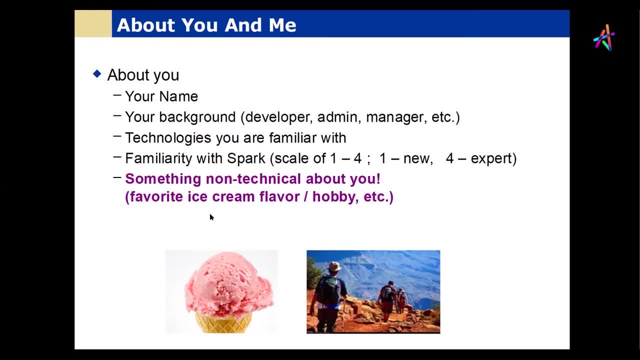 And also I'm going to add Scala in there as well. I'm particularly interested in the programming languages that you're familiar with. I'm also going to replace Number four. Oh, you can give me an answer to the last one if you want. 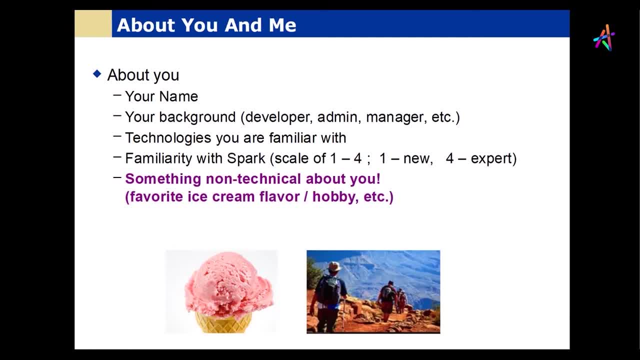 But the point that I would like to get from you is- And this is just kind of going to get me oriented- Is any specific things that are on your mind that you want to try and address during the course? So, particular issues, particular questions. 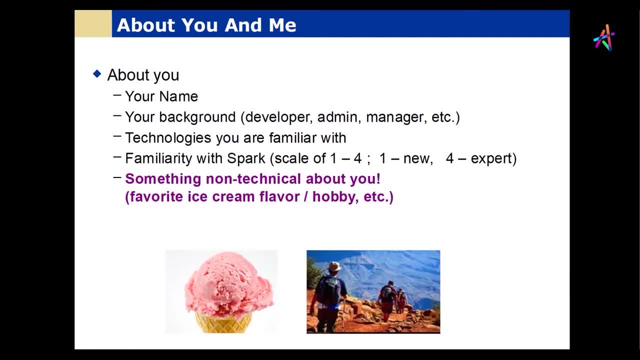 Things that annoy you, That you're saying, well, if I could figure something out, then I could get rid of this annoyance. So this is. I want you to think about that, And if you can't think of anything in that category right now, that's fine. 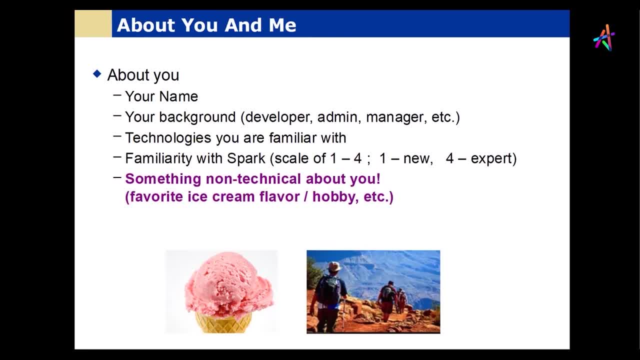 You're always welcome to add to that last item at any point during the course. It helps me too, because, as I'm presenting the material, if I know that that material is of interest to you or important to you, then it serves as a reminder to me to focus appropriately on the concepts that are relevant. 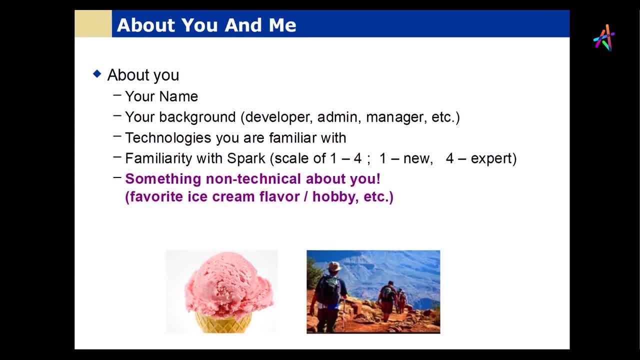 So I'll start To give you an idea of what's sort of expected here. My name is Rod And my background is quite eclectic. I started back in the 1970s as a theoretical mathematician, Which is one of the reasons I love Spark. 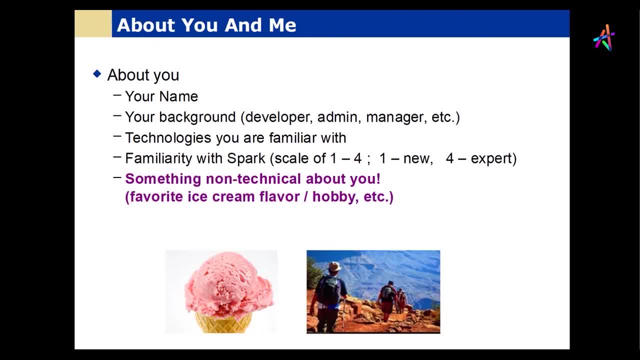 Not Spark but Scala. I also worked as a Studied as a cognitive psychologist and anthropologist, studying linguistics And looking at Cognitive structures, which got me into artificial intelligence in the early 1980s, in that first, or I should say the second- big boom of AI. 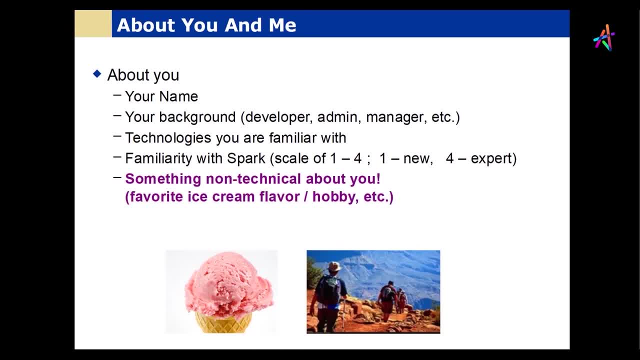 I wound up doing development work and scientific consultant and eventually became project managers for several AI startup companies funded by several of the computer companies. I'd spent most of my time up to that in the mainframe world working in developing things like language dictionaries, automated language dictionaries and so on. 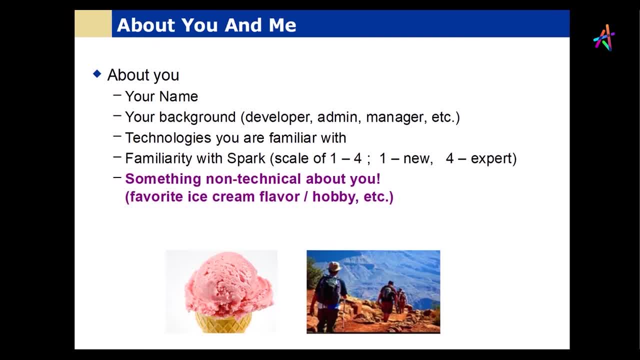 So I've been doing that for a long time. So I've been doing that for a long time. And that sort of environment, working with large corpuses of text. I wound up doing project management work for a number of research projects and development projects for a number of years. 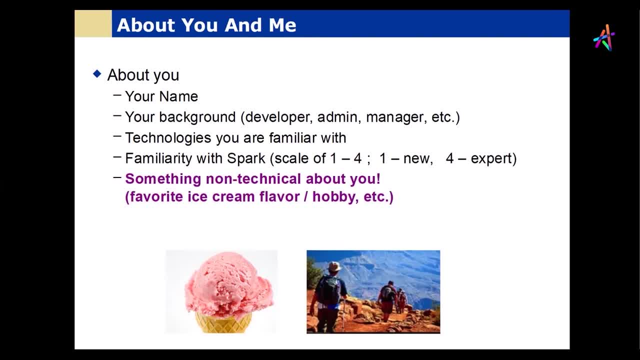 But I always continued to teach because I was an early adopter of a number of technologies, including object-oriented technology, in the early mid-80s, When everybody thought it was just going to be a passing fad, And I wound up doing a lot of teaching as I had to share these things that I was adopting with my colleagues and my coworkers. 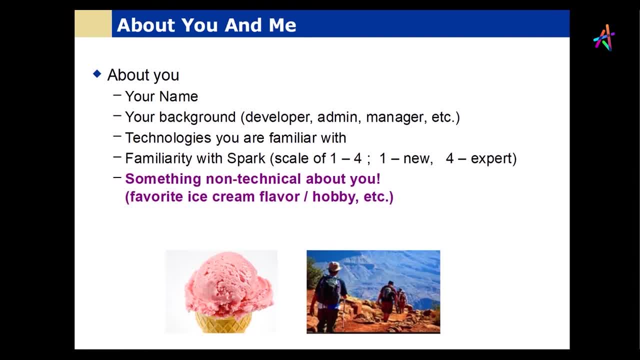 And my my teams. So in the late 1980s, early 1990s, I got out of project management. I decided that I wasn't a good bureaucrat and I was a really bad employee in that sense And I started doing consulting and teaching and had an opportunity to go around a number of different organizations in a variety of industries- Wall Street defense contractors. 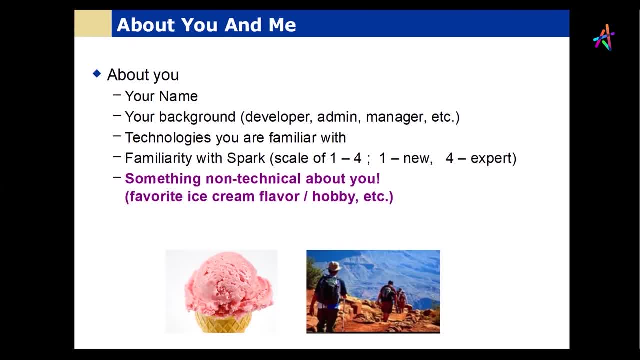 And I got to see what a lot of- and I've always tell people I was never really the smartest guy in the room, But I did get a chance to see what the smartest guys in the room were doing And that was of interest to me as an anthropology. 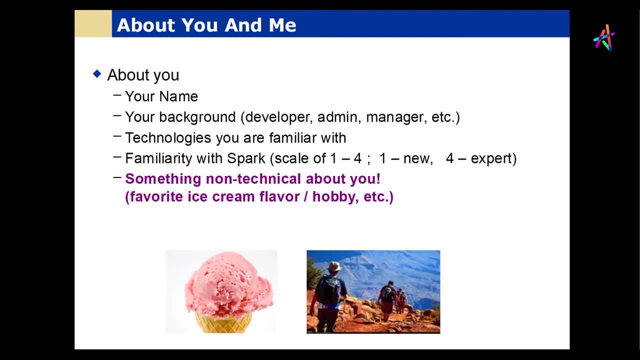 So I I tried to focus on: what are these people doing? that is really a best practice that I can take back and share with other people. I have been always interested in, of course, machine learning, working with data, data representation, how we manipulate data. 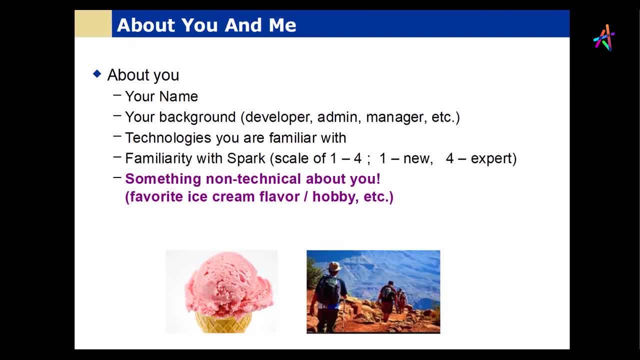 What's the reality of data in terms of what it tells us all? what are the effective tools for analyzing data and all of the These sorts of related issues that go around with data? So this is an area of interest to me. I got interested in the whole big data analytics world as it came out. 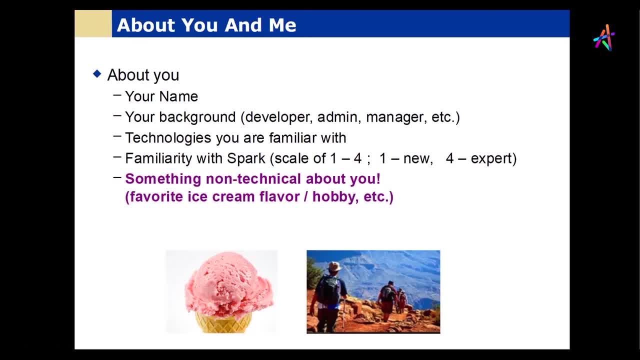 I've had my fingers in a number of pies. I'm particularly fascinated with Spark because Spark has employees, a number of what I think are brilliant and innovative approaches to the problem And I hope I can share some of the the kind of admiration. 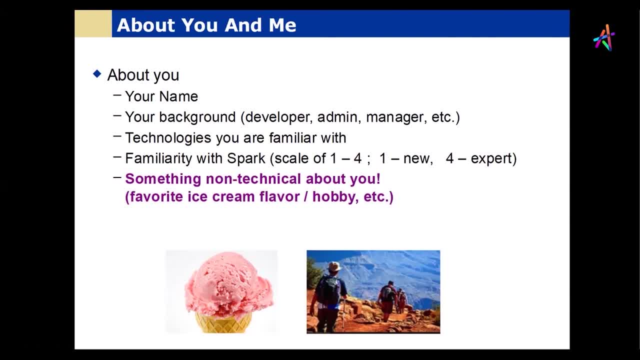 That I feel for the product with you as we go through the course. So that's basically I'm all over the map in terms of technologies as well, Programming in a number of languages, working from everything from developing executable requirements for business analysis to software testing, quality assurance, data modeling, domain modeling, all that kind of general technology. 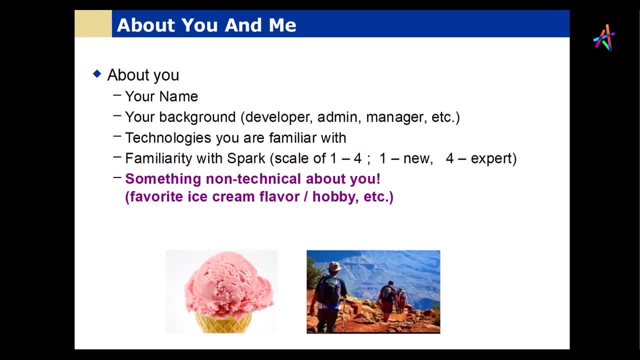 So hopefully, I'm bringing a somewhat unified approach to the, to the, to the class, And we'll be able to relate to all- All of you from different backgrounds. my particular goal for the course is to try to give you something that you can take back and use on a very practical sense. 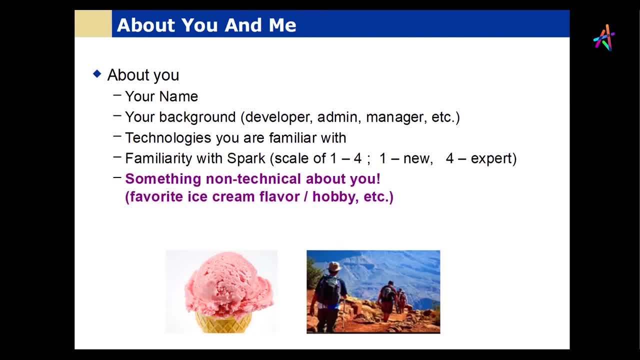 So that's generally me. So I'm going to kind of go through my list here and I've got a list of people on the chat window So I'm hoping that that's a complete list of not somebody is going to have to to to shout out. 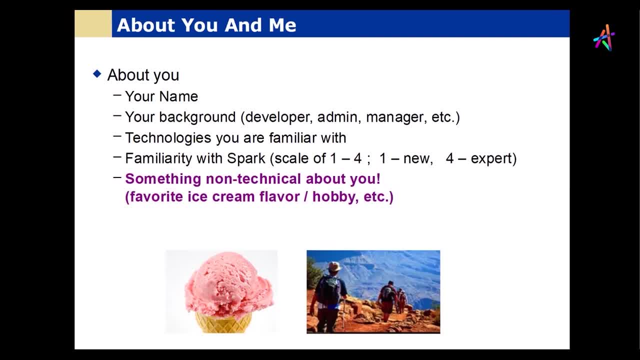 So we'll go alphabetically. Michael, how about you? Let's hear from you, Yeah, so I can start. So my current role, I would say, is officially engineering specialist. What that translates into is somebody who's been doing technology for, let's say, way too long and still wants to keep doing it. 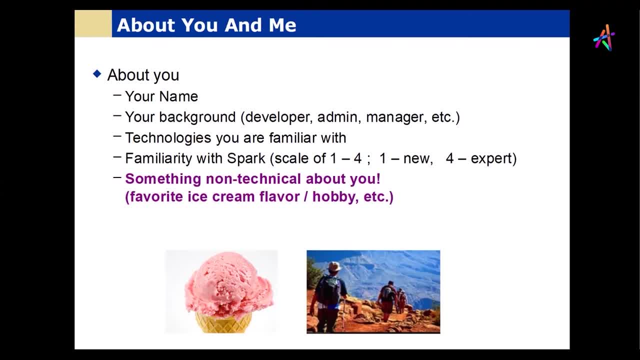 So we found a way for me, to find a way to make it interesting for me. So I've been with the company for a little over five years at this point. so we, which is way past the norm, so we have to find something. 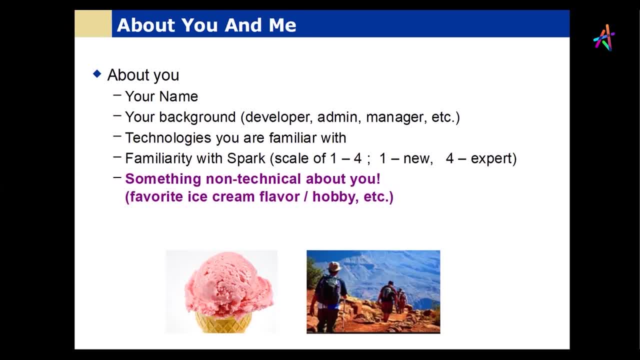 So I'm sort of looking at more at the, let's say, architectural implications of what the individual teams are doing. So the rest of what they're producing, I'm sort of looking at whether or not it fits within what we want to do, whether or not we can sort of challenge it to make it better. 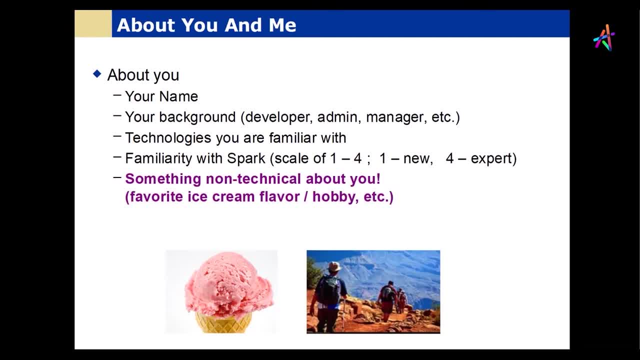 So more on a on a high level Now. that said, I'm still involved in in some projects, so I still want to keep- I like to keep- my hands dirty. As for, let's say, programming languages, I'm also, let's say, not sticking to only one. Way back when I used to do Java and C. then at some point I transitioned into Ruby, spent a bunch of time there, And most recently I was doing some projects in Golang, And right now I'm working on a new project. 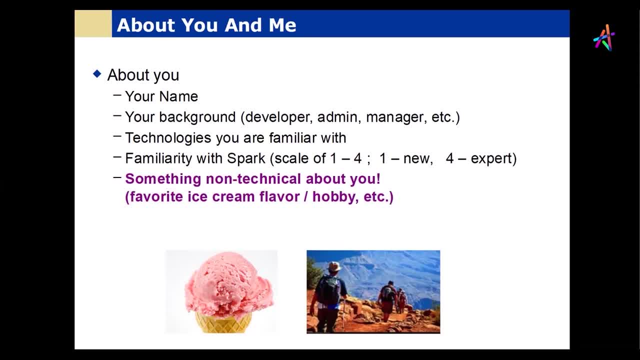 I'm starting to learn Scala so that I can be effective with Spark, let's say So, on that scale of one to four, I would say still maybe somewhere between one and two, Still trying to sort of figure out stuff that is you could consider basic, but that said, I can read code, so Scala is not really an issue. 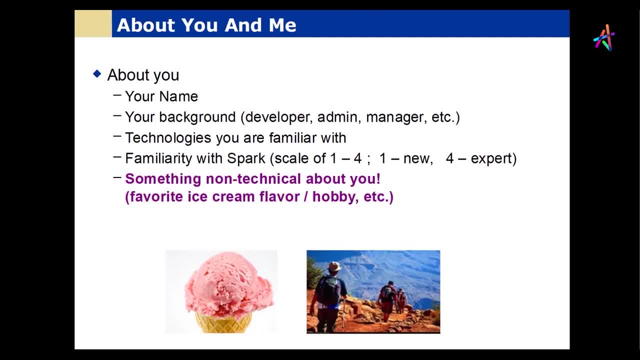 The most interesting thing for me is actually Spark Great. so yeah, you already say my name, it's Gregory, My title. what I'm doing here? I'm a senior data engineer, so basically in the data team, like we are responsible of ingesting, transforming, making the data available for the other team, services, stakeholders, so that can have like detailed reporting or insights, KPIs, metrics, hot water, cold water, whatever they want, basically. 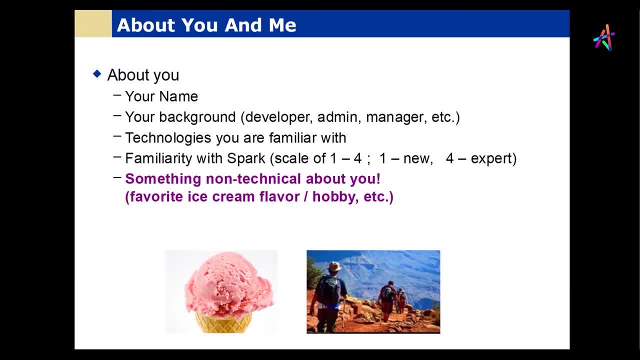 We try to kind of make it as simple as possible. We try to make it as real And about my background: I started as a C++ developer for a real-time bidding system. so it's basically advertising system that you connect, it's like a, it's like Wall Street, but for advertising. so you basically do bids in real time for an advertising spot and in a matter of seconds you fill this spot. you run an auction and the guy who is willing to pay the most basically fills the bid. Great, Yeah, so that's what I do. I'm the person who builds the spots with this advertising. Yeah, so I was basically working on the technology that allows to make the auction and also enrich the ability to make the bid for the people who are willing to make these bids. so give more information and context about the ad spots. 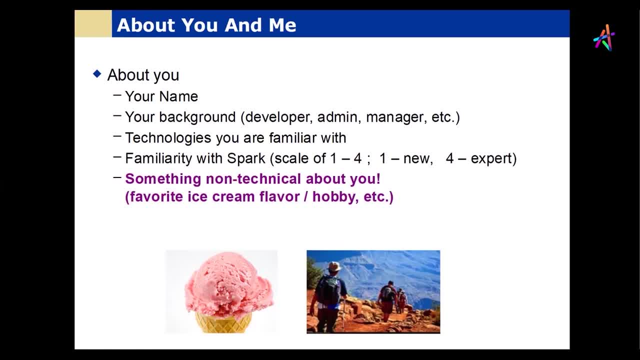 Yeah, I've done this for roughly five years. then I moved to data engineering, which is kind of closely related to the marketing part of the data. but yeah, that's it, Because to provide information, to be able to do a proper bit, you need to know what kind of information you have and run some analysis on top of it. 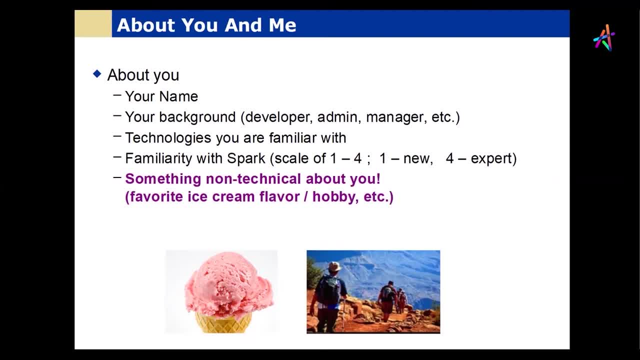 I switched from C++ to Scala and functional programming thingy and then naturally I kind of came to Spark. So yeah, in terms of familiarity with Spark- I don't know, it's really hard for me to scale, I would say. I would say two or three out of four maybe. And yeah, I'm familiar with Scala now since, I think, around four years. 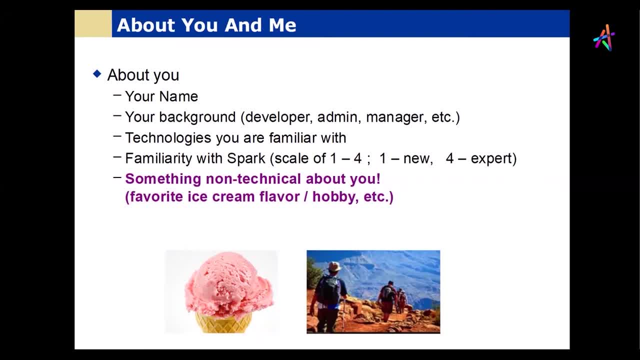 And yeah, so C++, Python, all the usual suspects. I do a bit of Ruby, although I hate it, so I wouldn't say I'm really familiar with it. It's like the mother-in-law: you know you have to see her, but you really like her. but it's okay, you have to do it. 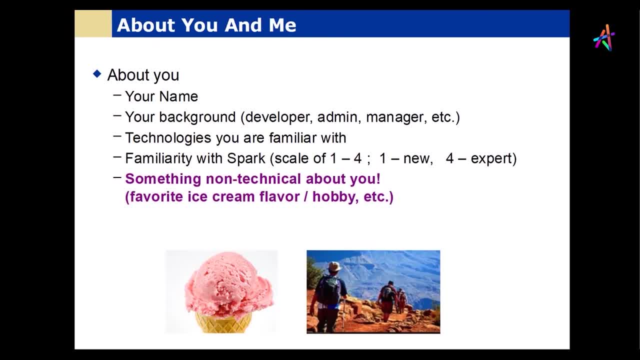 Something non-technical? That's a good question. I like climbing, rock climbing in general, Oh good. Interesting about Ruby is that Ruby has that effect. People either love Ruby or they hate Ruby. I've done a lot of Ruby and I'm not sure if I like it or not, but I do respect it. 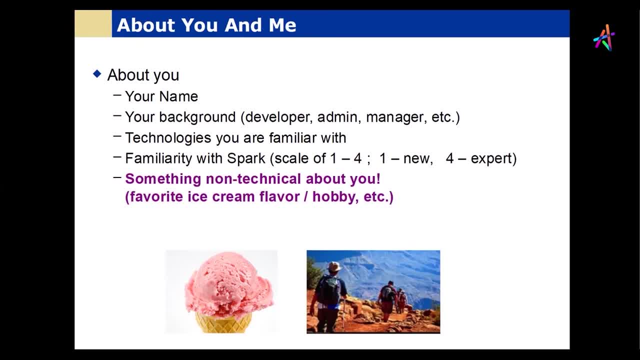 So we've got some good programming language here: C++, Scala, Ruby, Golang- one of my personal favorites right now- Yeah, So very good. Okay, thank you. So we've done, Gregory and Michael Robert, you're up next. 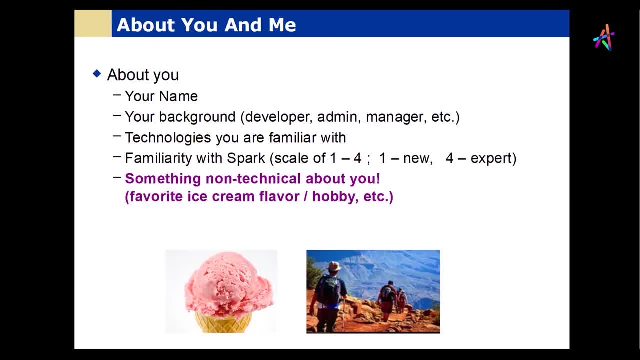 Yeah, my name is Robert, My background, so I left Hungary. I'm originally from Hungary and started studying in Germany as a computer scientist. I finished too soon and I got the offer to do a PhD, So I stayed for a PhD at the data management chair. 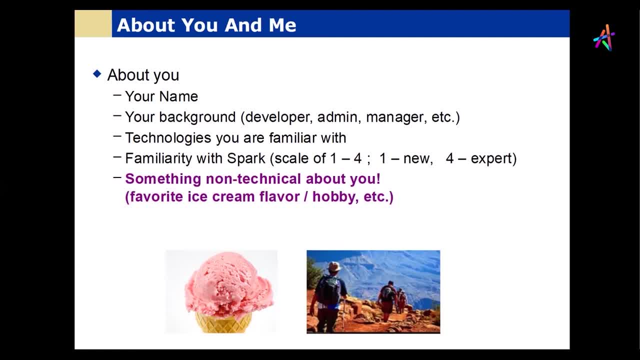 And after that I wanted to see the world, The word meaning Germany- So I joined consulting companies and there I was able to work with many different people and many different companies And, exactly as you mentioned, pick up the best practices and always try to get to the 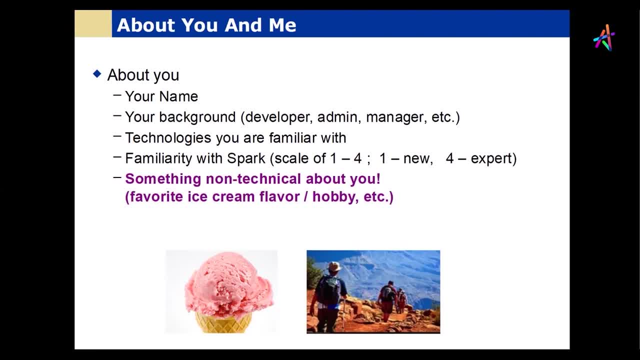 next place where I'm not the smartest in the room but there are other smarter people to learn from, Absolutely So I did that for roughly five years And worked in anything that's data related, So from back-end ETR processes up to front-end and even building a reporting tool that some 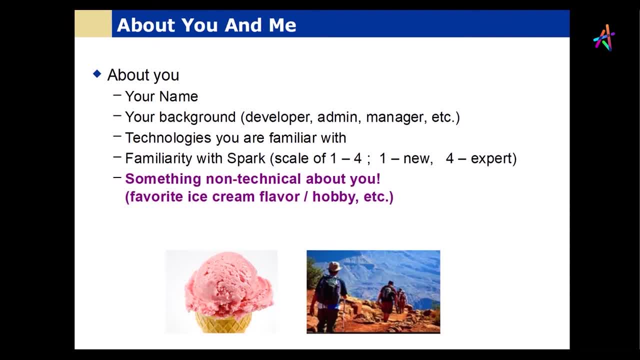 clients even use today. So, yeah, And after that I decided to not travel anymore, Also because of private reasons- And then I joined Creditics. And then I got a job. Yeah, I joined Creditics as a data engineer. Soon I became a senior and recently I became the team lead in the data team. 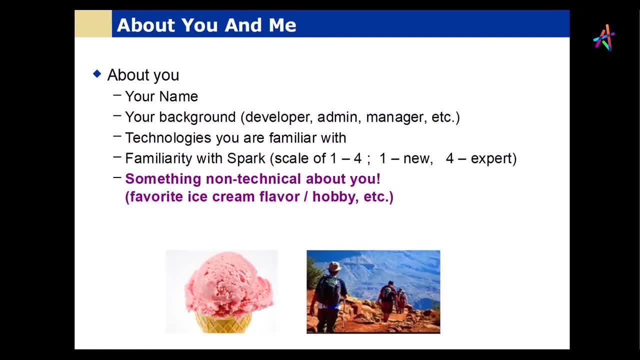 So our goal is to provide the data as soon as possible to all our users and make sure that we scale for more customers. Technologies I'm familiar with Well. during my phase as a consultant, I worked with basically any database system that's available in the market. 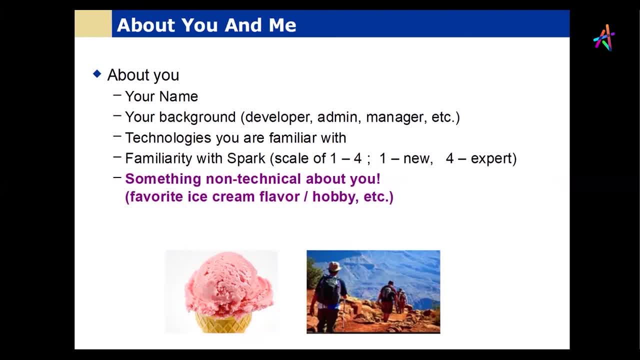 So just name it Most likely. I did some work with it And I really like to write SQL. That's one of my favorite. And from programming side I started with C++- Built actually a database management system in C++ back at university. 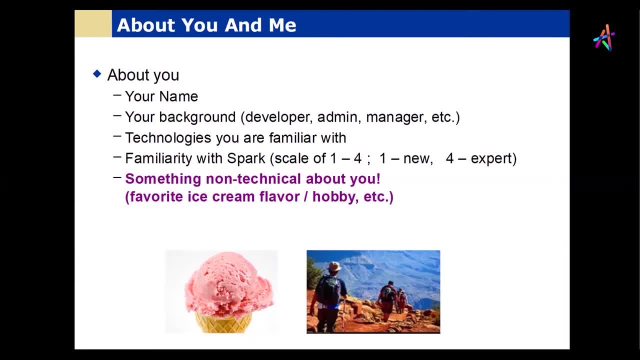 And then jumped into Java technologies. due to this consultancy work And at Creditics. I had to learn Ruby then, which actually I like, And there are also other languages that I had to pick up at Creditics, like Google and some Python, And recently we moved into Scala and Spark for revamping our data pipeline. 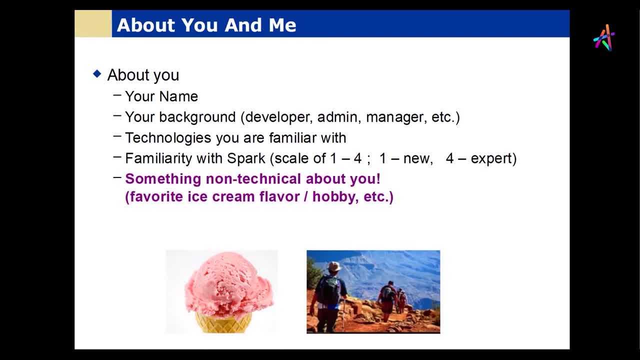 So familiarity with Spark and Scala is more in this two and three section. I would guess more in the two area, Since we had to develop our knowledge ourselves within the company. that's also why we are asking for a training, so we get a better overview. 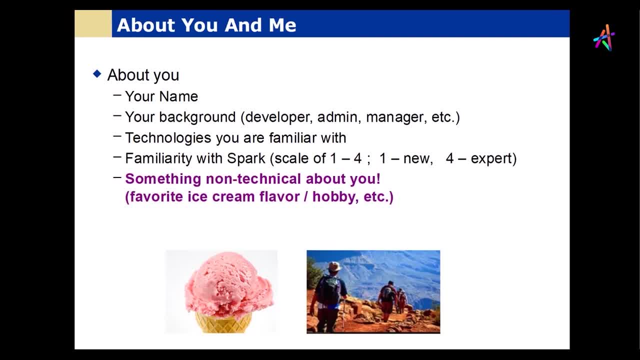 And some non-technical about me. Yeah, I mentioned it at the beginning. I really like to eat. That's the thing I did While I was a PhD student. I also learned to cook because the food was simply not good enough in the time. 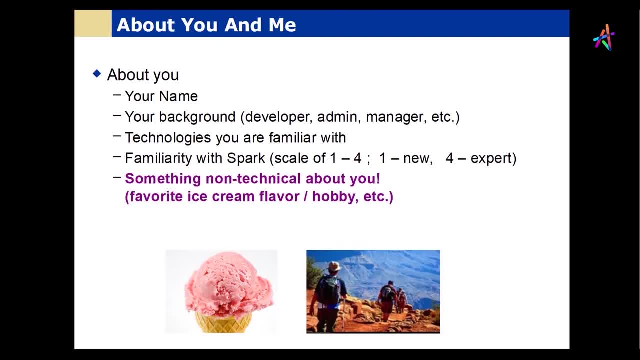 So I had to go back to my hometown. I was living, And I even brought it to the level that I worked in Michelin-starred restaurants, But then I decided to continue on the computer science path because it's more family-friendly. So that's also the reason why I moved into Berlin, where Creditics is operating its IT. 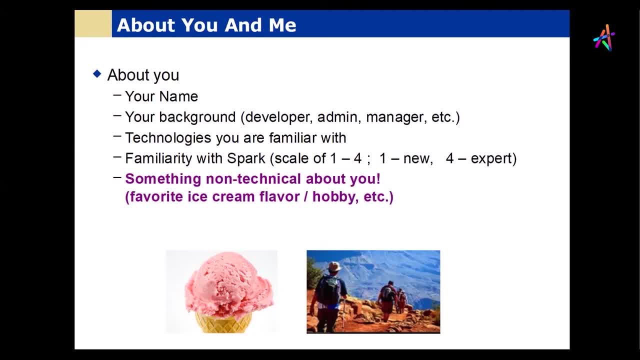 department because it has just the best variety of really good food in Germany. Oh really, I would remember that if I come to Germany. if I want food to go to Berlin, You have to go to Berlin. yes, But there are other cities as well with good food. 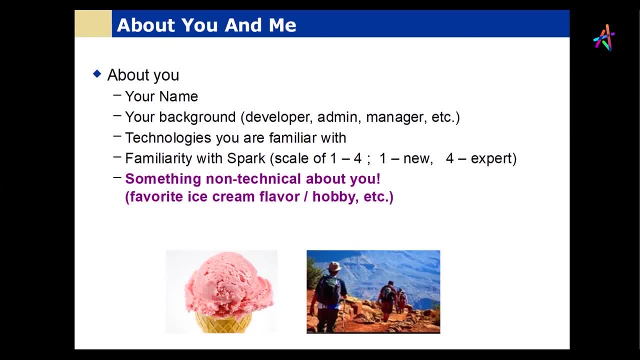 Yes, Well, I'll keep that in mind. Okay, Yeah, Okay, good, Thank you very much, And I think now I do not know how to pronounce the next name here properly: Evgeny, Or can you pronounce it? 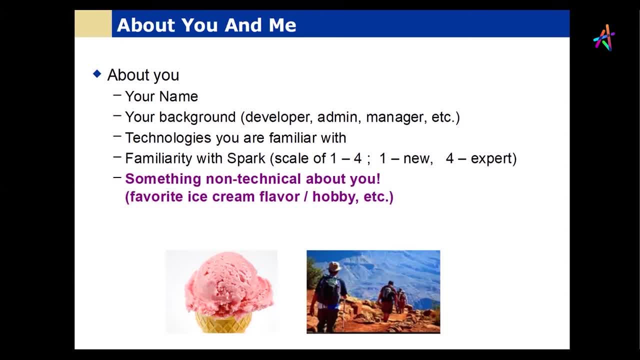 Hello, The closest you can pronounce is fine, But the proper would be Evgeny. It's not easy. Evgeny, Okay, Yeah, Yeah. I never know how the Gs come out and stuff, So Evgeny. Okay, Yeah, Yeah. So I started doing some basic web pages with PHP like 15 years ago, Found after some time. Ruby loved it. After that spend a lot of time with different technologies, trying new things, experimenting, some music. 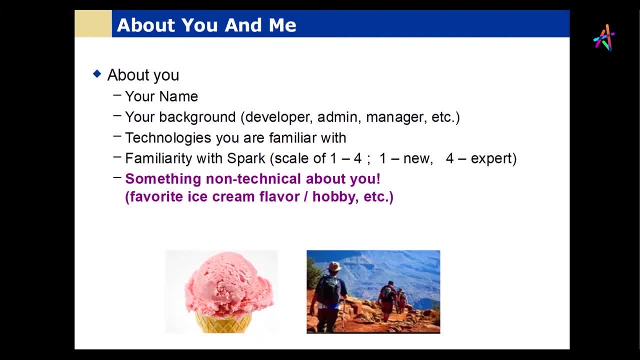 And then some years ago joined a company who was developing mobile video games And it was a lot of fun to be responsible for back ends of these games, especially we involved in some game mechanics like calculations and other stuff. Two years ago joined Creolitics, learned Scala somehow a bit. 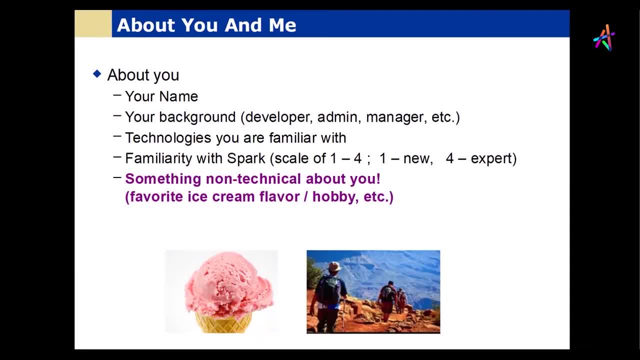 And yeah, currently I am in a situation where I am exploring the possibilities, so exploring new fields like data fields. Maybe it could be interesting for me. And yeah, in the past few months also completed Scala functional and Spark stuff on Coursera. 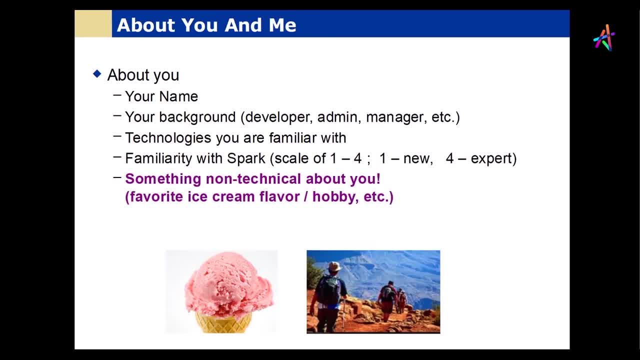 which I found very interesting for me. Oh good, Is that David Odetsky's course? Yeah, I think so. Yeah, yeah, It's from the creative Scala, at least first two parts. Yeah, It was amazing, especially his explanations of how language is designed and how it's supposed. 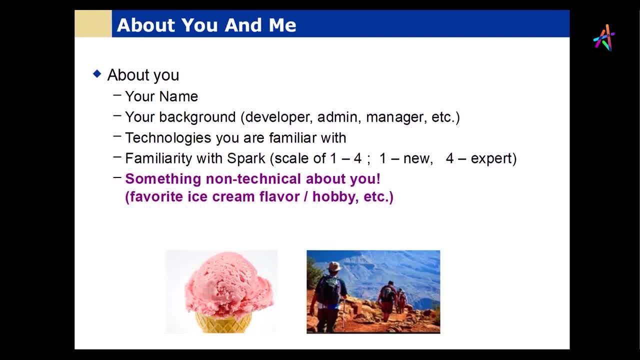 to work. Yes, And that's one of the things we're going to be getting into, So that should be familiar ground for you. Yeah, And so my familiarity with Spark would be around one, I'd say, And non-technical stuff. 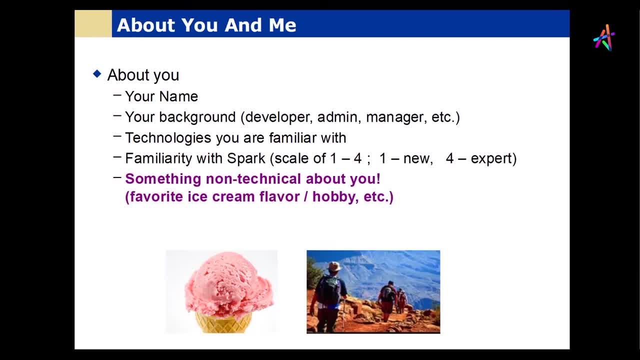 Yeah, So I'm really into Ping Pong these days. I never suspected that this is possible, but it's amazing. I'm sorry, what was that? Ping Pong Table tennis? Yeah, Really Okay. It sounds silly, but it is. 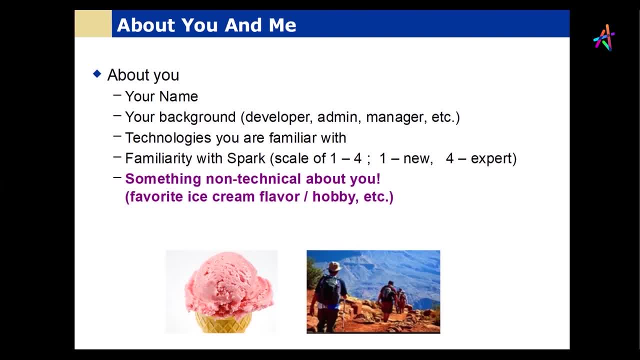 It is fun. Okay, I know that it has a wide fan base in Asia. I know Ping Pong stars over there are like rock stars. Yeah, I guess so. So if you ever want to go to Asia, you can go to Asia. 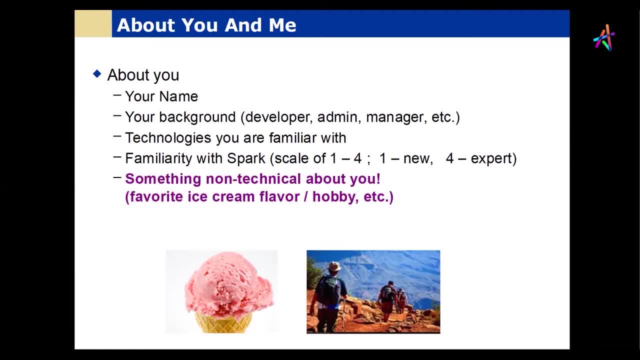 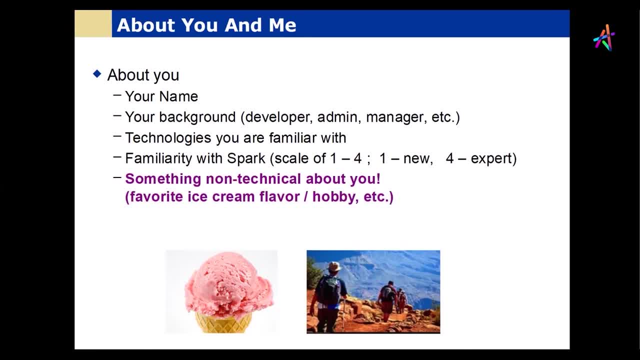 Gerald, how about you? Yeah, Hi, I'm Gerald. Yeah, How I started, I was going to university in Potsdam, so pretty close to Berlin, And this time probably a bit more data engineering or in kind of information handling kind of. 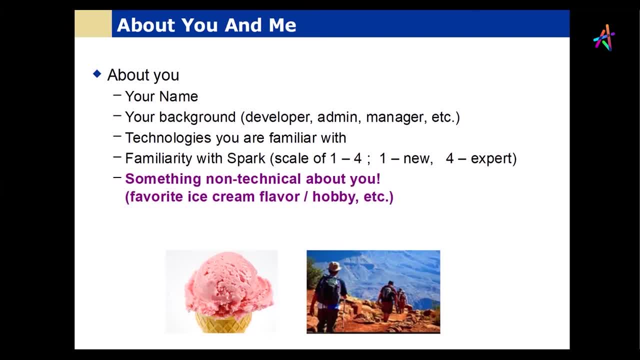 new stuff- Yeah, handling and so on- than in my whole professional time. I would even say so I got first contact with Hadoop and these kind of things, things that were kind of the basis for stuff like Spark and so on, and during that time, and also after university, I was mostly doing web-based 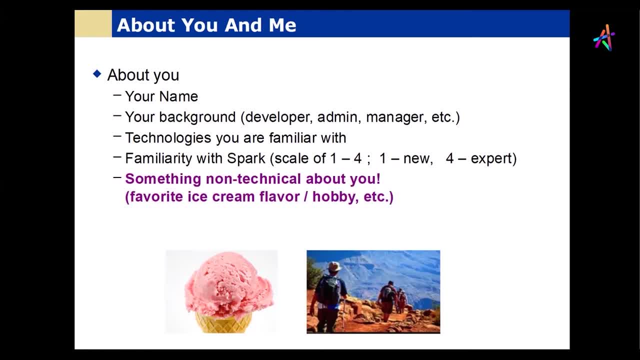 applications, not so much, let's say, rocket science, rather than the basic stuff, and I joined kind of Queryalytics six years ago. basically, I joined a company that was acquired by Queryalytics more than three years ago and I'm still working on the application that 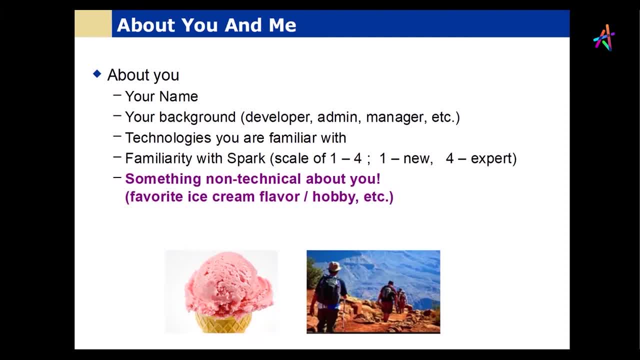 was brought into Queryalytics. Then we also have We have some Spark component written partially in Scala, partially Java. it's a little bit of a black box, so editing and changing things there is a little bit difficult and sometimes the results are surprising. so that workshop should help in this direction to understand. 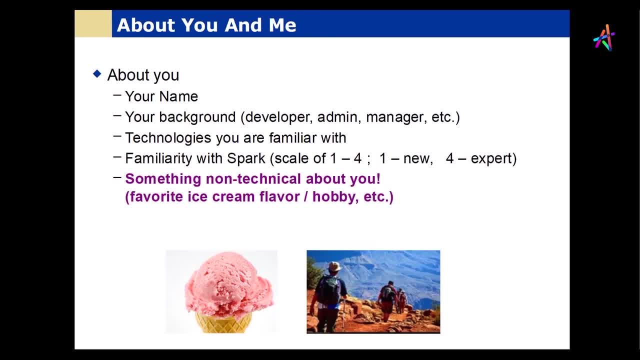 it in a better way. The general application is more- yeah, again, web-based application based on Java, Postgres, Elasticsearch, these kind of things and what else, yeah, in between, I also got into contact with Ruby Scala as well a bit, and I 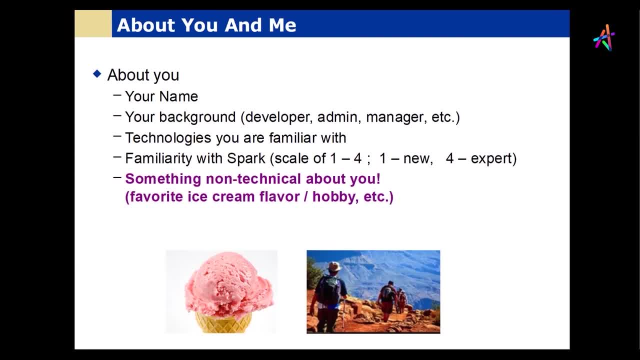 Yeah, Yeah, Yeah, I feel like the familiarization with Spark is probably at two, I would say, Not technical. I guess the reason why we started the workshop today is because we, because I just returned from a vacation, So you're the cause. 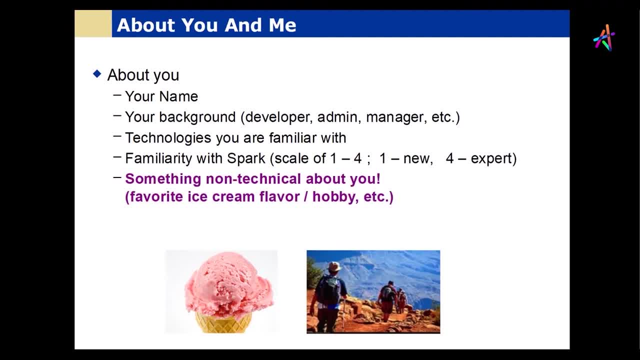 All right, Well, I'll have to. So you're the guy I have to make happy. All right, Good, I'm pretty sure that. Okay, Roman, how about you? You get the last one here. Okay, we have a couple more people. 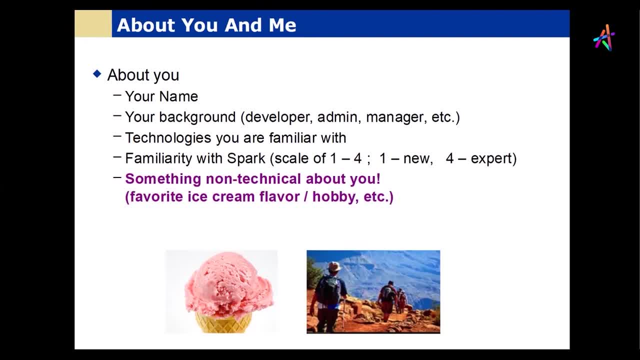 Oh, okay, They're not on my list, so you can introduce them as we go along too here, I'll have them introduce themselves. I think they're pretty capable of introducing themselves, so let us just start with me and then we proceed with this, Okay. 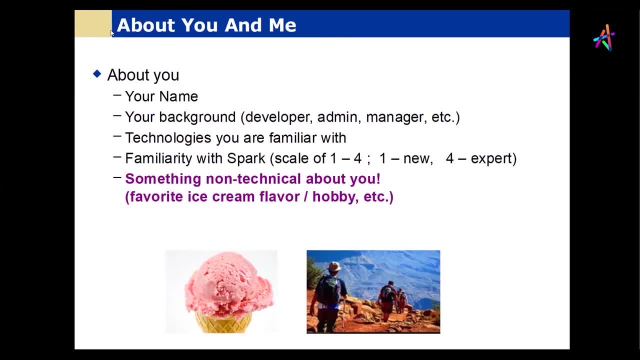 So my name's Roman and I started off as a developer, like more than 12 years ago. It has started off with supporting of a web-based application, mostly PHP, so this is the kind of experience I'm not proud of, And 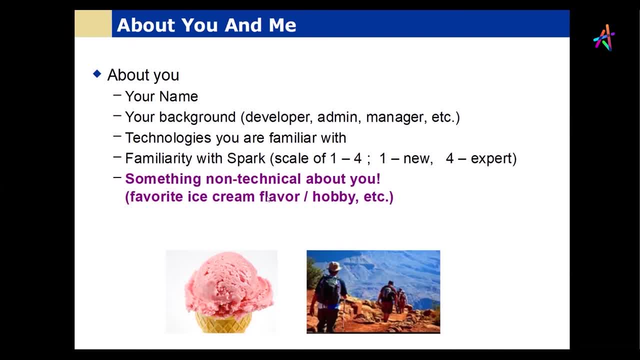 then at some point I decided to switch to Ruby because, yeah, I'm in the love-Ruby party here, so I kind of love this language. I'm impressed by its simplicity and, yeah, powerfulness, And I joined Cryolytics this year, actually beginning of this year. 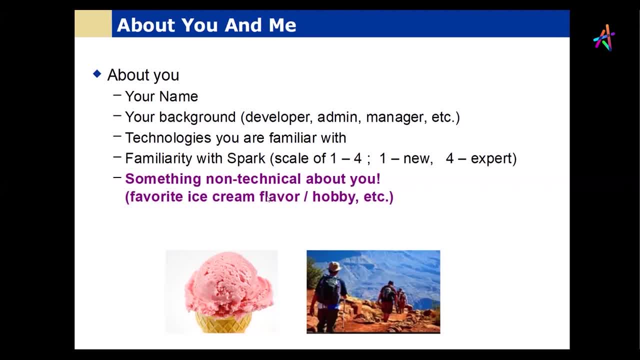 and my title sounds like: Well, it's complicated, It's Engineering Team Leads, Application Development something. Anyway, what my team is doing is we're developing one of the tools that is intended for our digital marketing, to automate some of the stuff they are doing, And 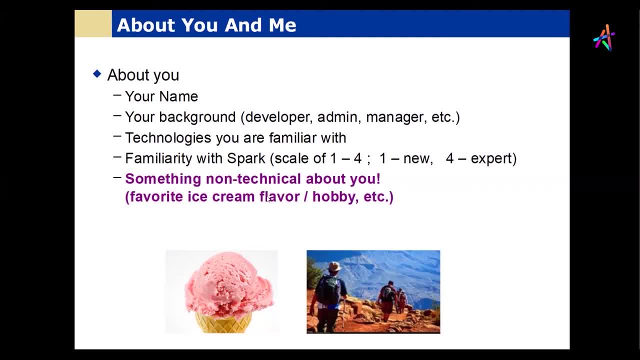 right now we Well, the focus of the company changes a little bit and we have to change our focus as well, And one of the opportunities that we're exploring is moving more towards from application development more towards the data processing. So, as far as I'm aware, all team members are 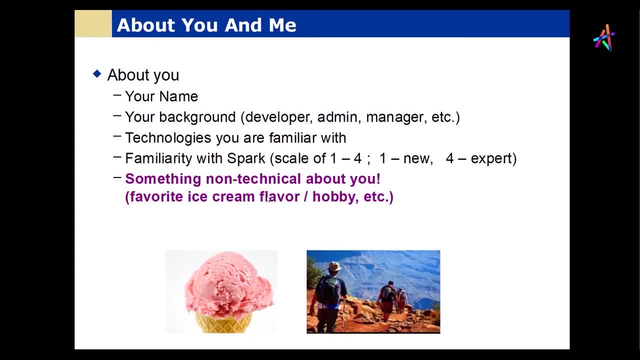 So yeah, Evgeny is actually one of my team members And actually all of my team members, as far as I'm aware, are particularly interested in the data processing topics, so we started to explore these opportunities. I have also started going over the 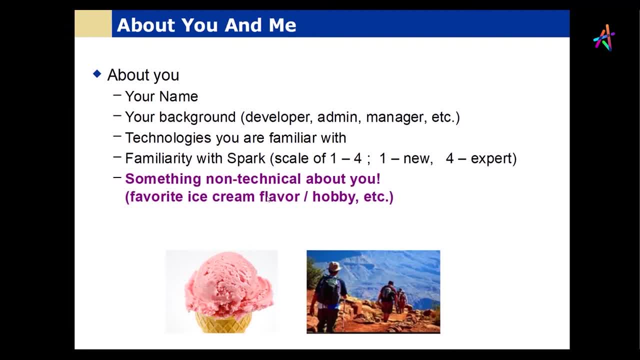 Coursera courses on Spark and Scala, and unfortunately I haven't finished, but I also share the same feedback as Evgeny had. So I really find them useful and pretty much clear to understand. So on the scale of one to four of my familiarity, 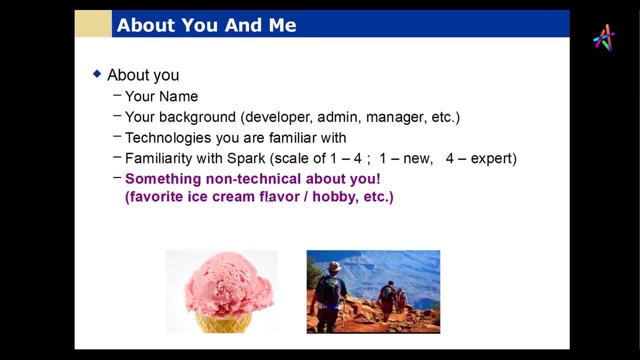 with Spark it's between zero and one. So I have just only started. I haven't completed it yet- And, yeah, it's actually a nice thing to me that we're going to touch upon some Spark basings on this course. So, yeah, this is really awesome, Fun fact. 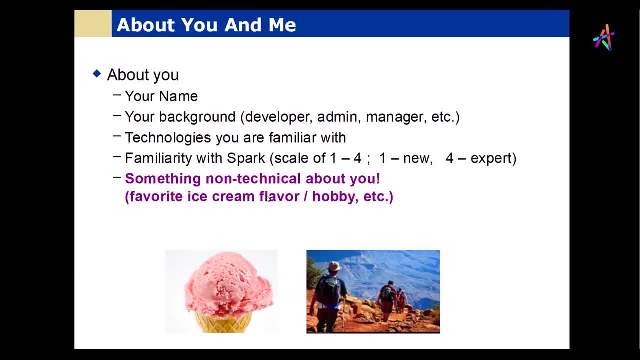 about me. well, my favorite ice cream flavor is Stracciatella, if anyone is interested. And I live in Germany for almost five years and haven't managed to learn German yet. Oh, that's an impressive feat. Well, you see, I live in Canada. 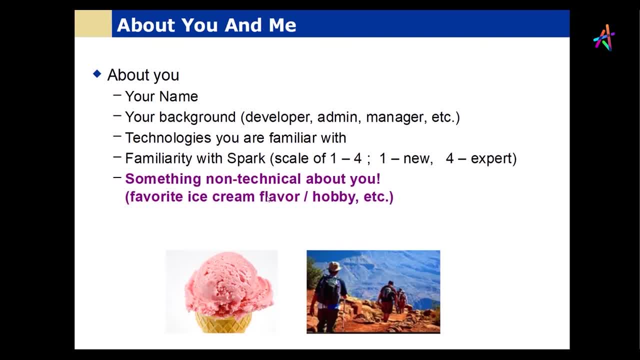 in a bilingual part of the country and I moved here from an English speaking part of the country And I have learned French to the point where I can sit quite comfortably in conversations and could contribute if I want. but I find it's more to my advantage to make the people think. 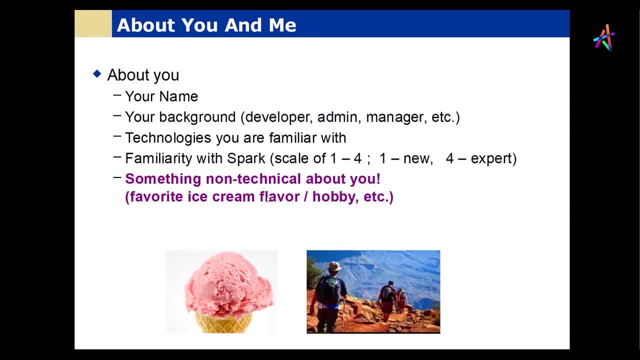 that I don't understand French, particularly when I'm in meetings. I learn a lot of information that way. when they talk in French, thinking I can't understand, So I understand that. Okay. so there's other people there who I haven't hit on, So maybe we could have somebody introduce. 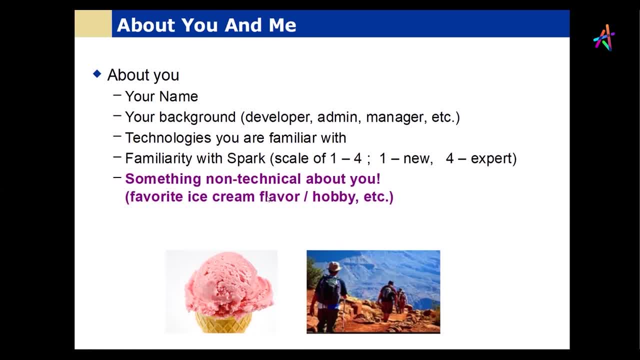 himself, who I haven't mentioned so far because I'm making notes. here There's two more of us, So I am a data engineer at Galytics. I've been in this role for the last three years. I'm sorry, what was your name? 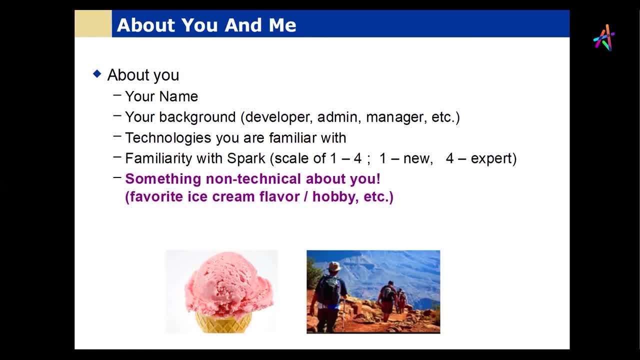 Manu, Manu, okay, Yeah, so I'm working with Gregory and Robert on the data team, So I recently joined the efforts of building this data pipeline and data warehouse in the cloud using Scala, Spark and so on. In that sense, my familiarity with both technologies. Spark and Scala is not super good yet I'm catching up. I would say 1.5 at best. And besides that, well, I have contact with C and Java in ancient times, More recently Python, Ruby, a little bit of Go, But yeah. 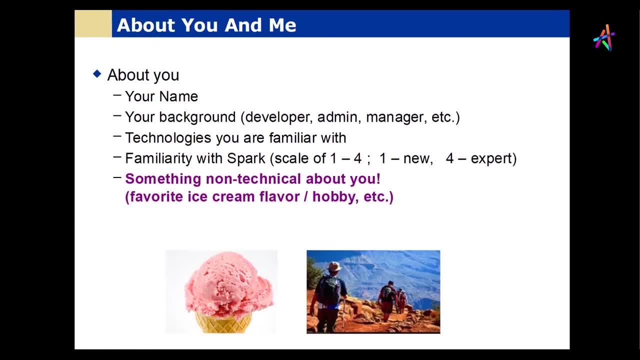 so I would say I'm mostly a Python developer And again trying to become a Scala developer as well. And ice cream, well, I would say pistachio. Fair enough, All right, thank you. Next person, The other person, I'm, the last one, I'm Yorgos. I'm coming from Greece. I've been in Galytics for the last two years. The project I'm working on is relatively new. We're doing Java mainly. I completed a course in Coursera regarding Scala back in 2013.. Yeah, my familiarity with Spark. 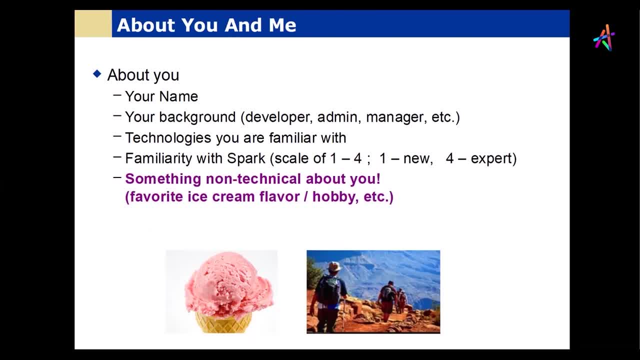 is zero. I just saw some YouTube videos and I started reading this online book, And some non-technical about me is that I also like biking, I like swimming And I'm gonna try to complete my first triathlon next year. Okay, excellent, Sounds good. 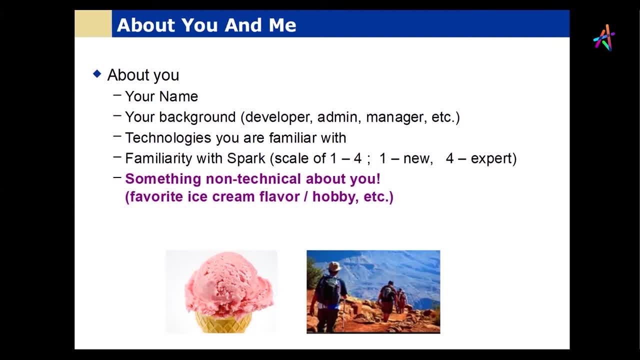 All right, thank you all. I appreciate that And we can get down to it. By the way, that marathon's interesting. My brother-in-law is a triathlete and his son, my nephew, actually just set the Canadian record for the. 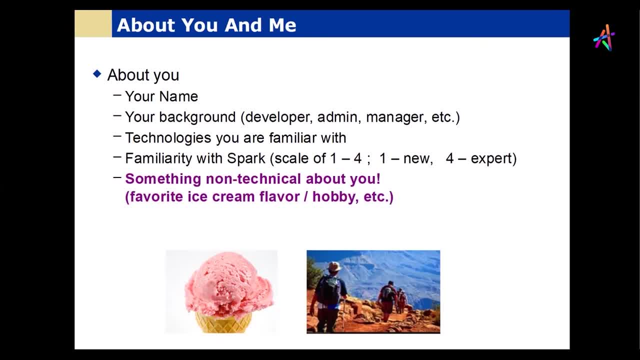 or actually set the Canadian record for the a number of years ago for the under 18 triathlon in Canada. So they're always off doing Ironman and all that kind of stuff. So I can really appreciate how hard that is for people to do. 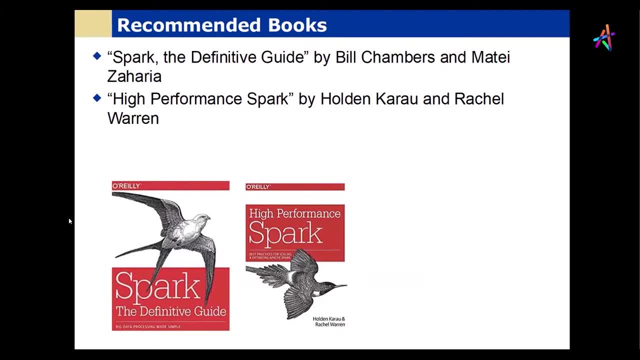 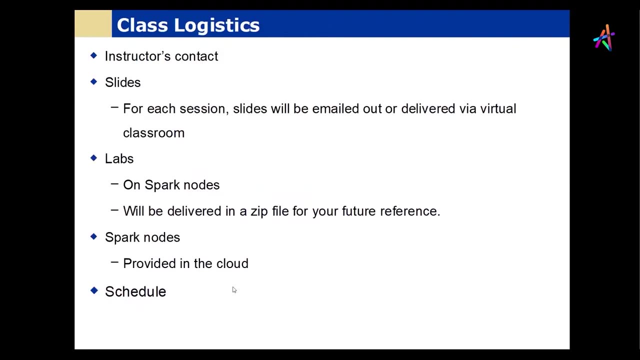 Okay, there's a couple of reference books here, And I will actually be referring to some of the high performance Spark material next week to give you a bit of a reference there as well, So you can follow up with the class with that And a couple of other. just final points. 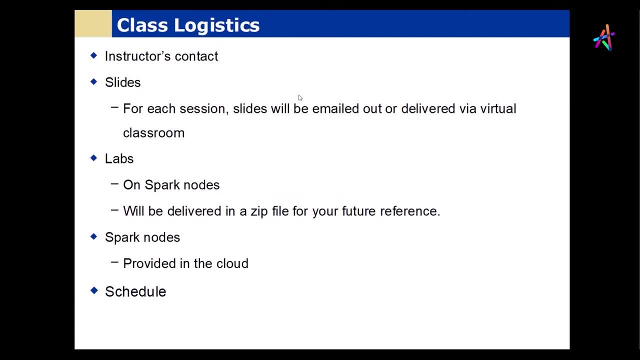 and then we'll get right into it. I'll give you my contact information. The best way to get a hold of me is by email. I'll type that into the chat window right now. That's generally the best way to get a hold of me if there's any kind of issues. 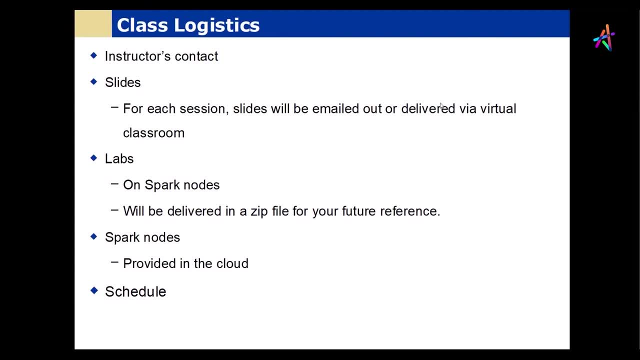 I generally tend to monitor my email fairly regularly. The slides will be emailed out or delivered. I will probably see about just putting them into a GitHub repository or something and letting you just pull them down. The labs and things will be on the nodes that you'll get. You'll also be able to. 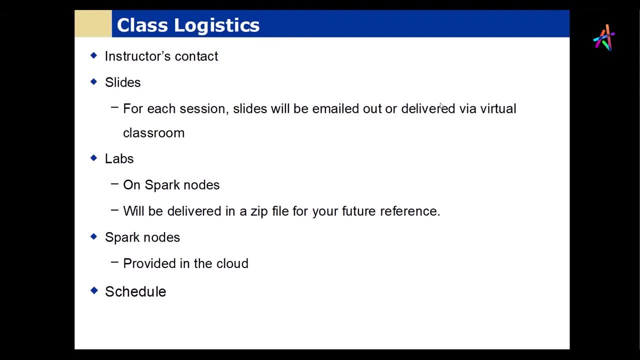 get all of the lab material as well, And a little bit later this morning we're going to set up your nodes that you'll be able to work on, And that'll be just a bit of an administrative overhead. I think we don't have enough, so I may have to spin up a couple more. 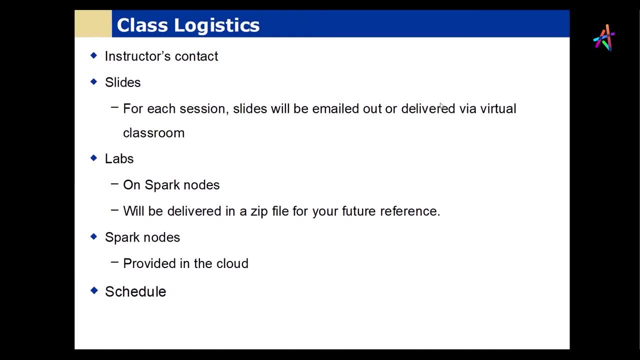 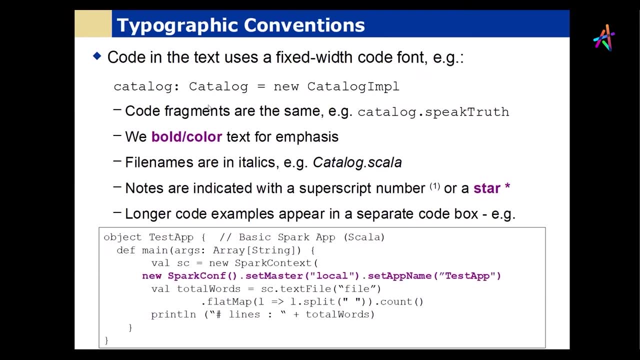 instances. But we'll sort that out as we get there and we'll do some walkthrough on how to actually use that material- And I think that's about it. for logistics, Typographic conventions, fairly standard boilerplate stuff. Basically, we're going to have examples of code as we go. 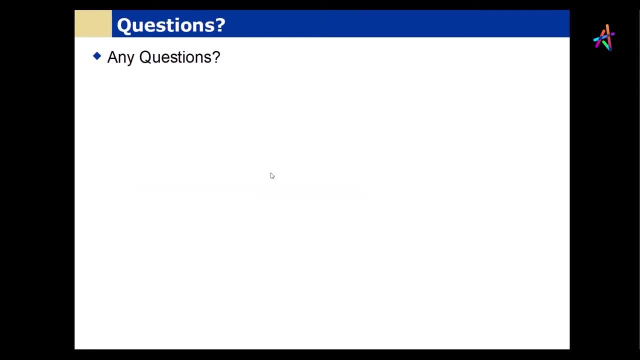 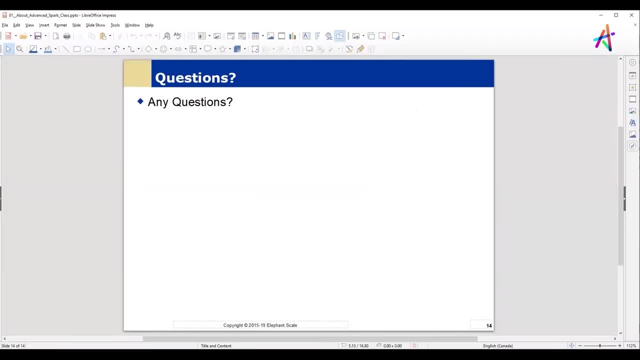 through. So there's different fonts that we use on there, And so we'll end up that session and we'll carry on and we'll do questions as we proceed. Now I'm going to start off actually with the Spark intro and then go back to Scala, simply because 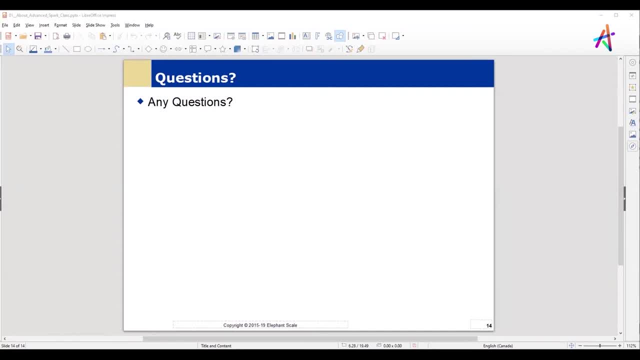 a number of people. we want to sort of understand where Spark fits into this ecosystem first. So we'll just take a moment here to load up. I have this Windows computer. I do this on for presentations. I don't normally use Windows, but Zoom and other things only run under Windows. So 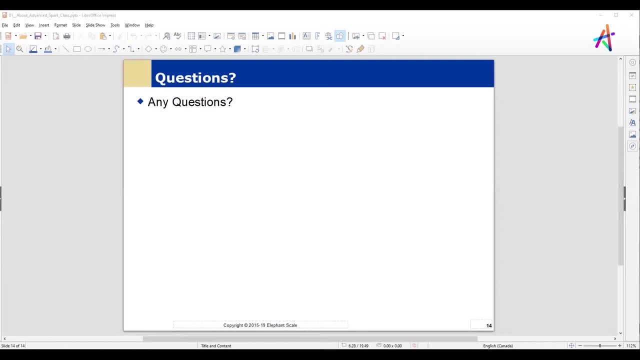 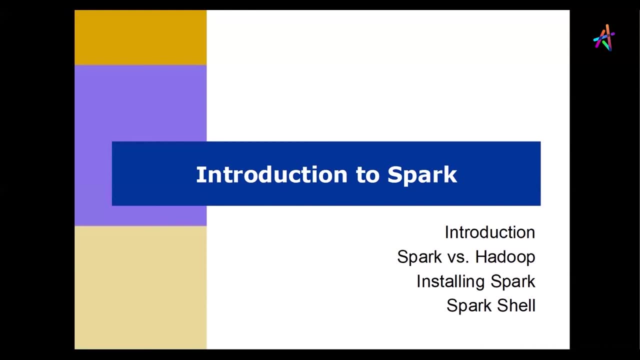 it's sometimes a little bit frustrating for me. I really hate Windows, So what we're really going to do? and we won't install Spark. I just want to go over the first part of this to give us a conceptual overview as to where Spark fits into the whole technology. 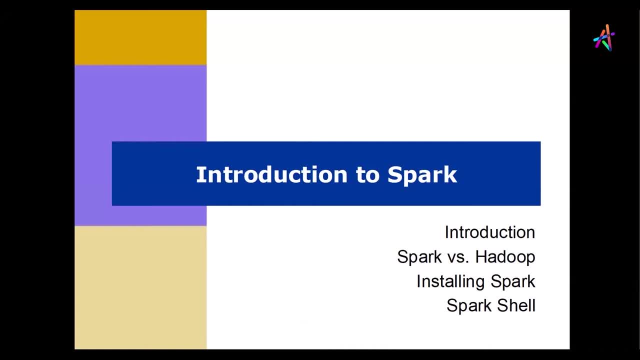 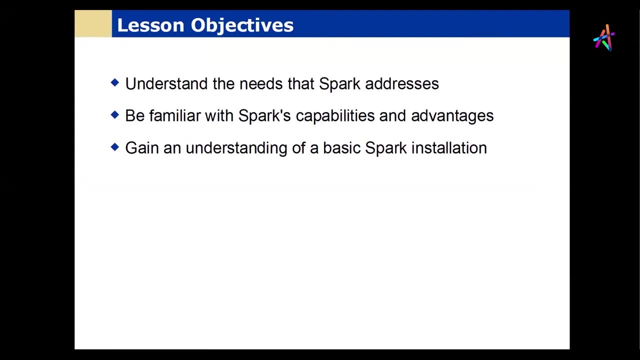 ecosystem. So let's jump into that. The particular thing we want to focus on is what Spark is actually intended to do and what its capabilities are, and then we're going to go back and look at Scala, because then we can see how Scala and Spark 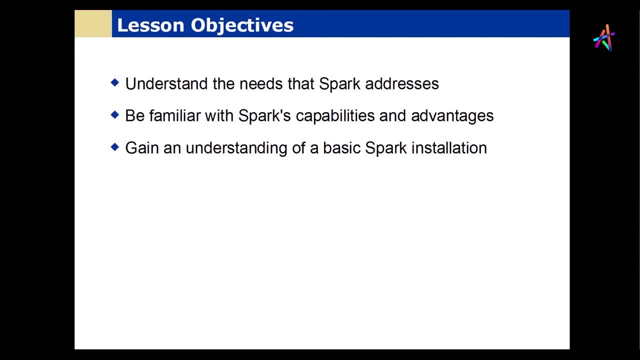 are related conceptually. I think if we just jump right into Scala it's a little bit. it's not as conducive to learning when you're not making those connections between Spark and Scala right off. So I think it's useful for us to take a little look at. 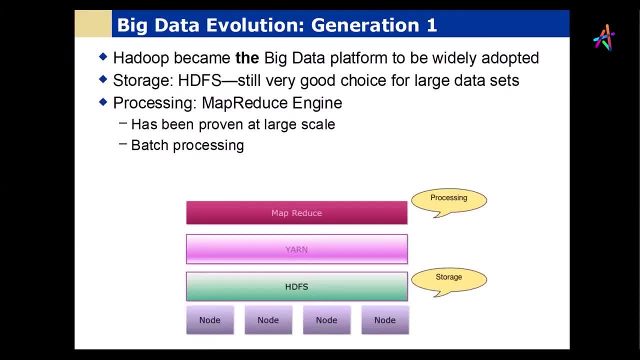 Spark as we go before we start. Spark comes out of the big data world and it is built on some gaps in the needs that existed in the big data world. Big data, of course- just to clarify for the purposes of this course- is data that's characterized by the four or five V's. 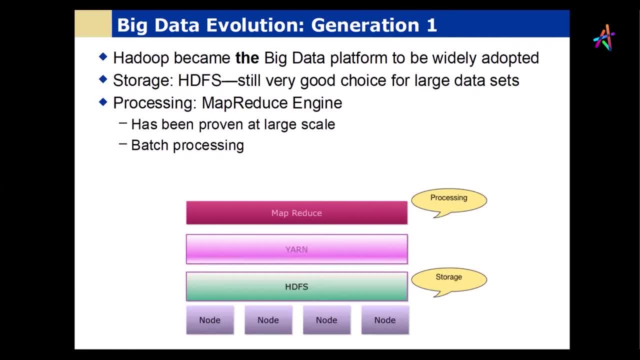 depending on who you're listening to. The most important ones from our point of view are large volumes of data from different sources and variety that we need to manipulate in some way. The whole notion of Hadoop comes out of a number of different projects that 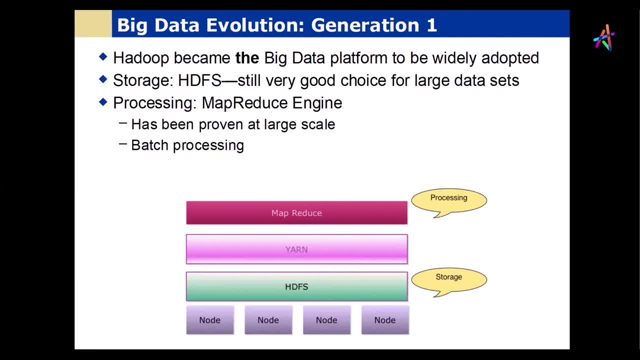 coalesced, merged with each other and borrowed from each other about how do you manage these large volumes of data in a close to real-time way. Hadoop was the standard HDFS. Hadoop file system evolved as a way to manage that data. The original 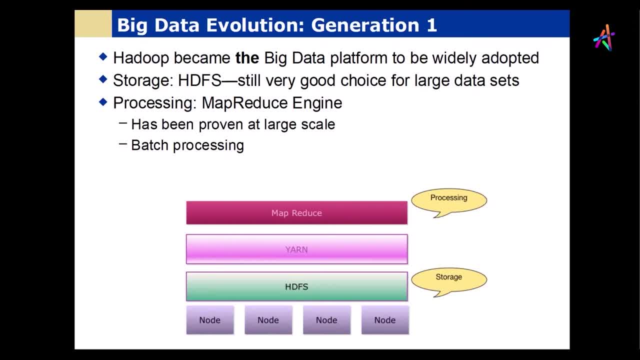 goal of these things was not to do a lot of real-time processing. It was to do analytics on large data sets. The initial approach was to focus on how do we store the data, first of all, and then how do we distribute out our 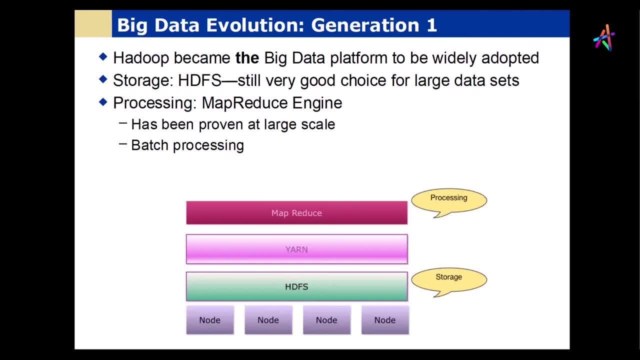 processing and do queries on this big data, get analytics out of this big data. The initial problem was very challenging. The problems that weren't addressed at the time were often problems of how fast can we do this? It was more. can we do this? MapReduce Engine. 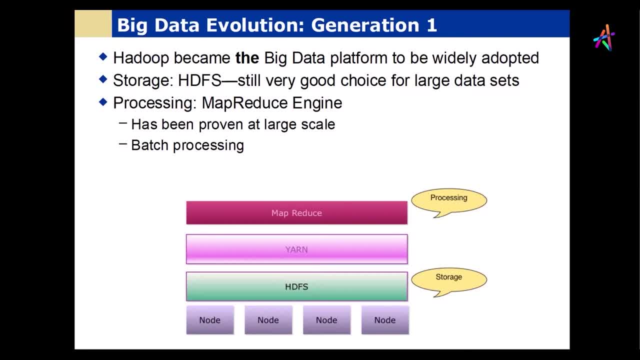 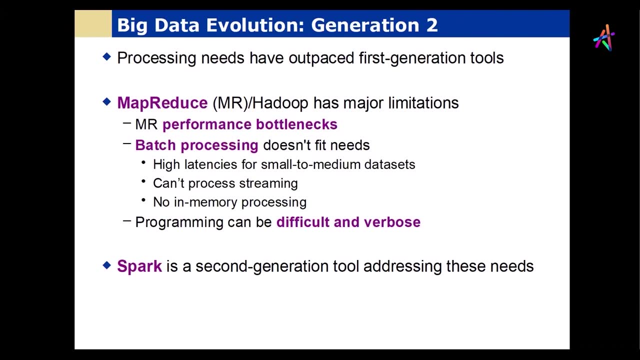 came up as the way of doing this distributed query analytics approach. It worked and everybody was very happy with that, but it was originally developed from a batch processing perspective. That had a couple of advantages and disadvantages. While we were now able to process large amounts of data, we had the MapReduce. 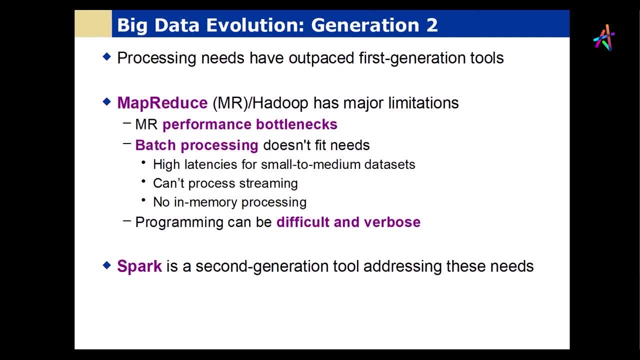 bottlenecks. A couple of problems that emerged with that were: the batch processing model that was used did not fit all of the needs that we wanted to apply this kind of approach to. In particular, we had high latencies for small to medium data sets. In other words, it didn't scale down. 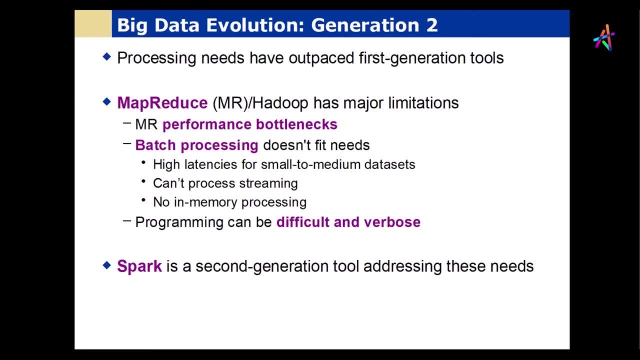 and give us a comparable improvement in performance that we would expect to see. There was a bit of a problem there. It was designed for high volume, large amounts of data. It didn't tune well when we wanted to look in other environments. It's not a solution that matched every volume. 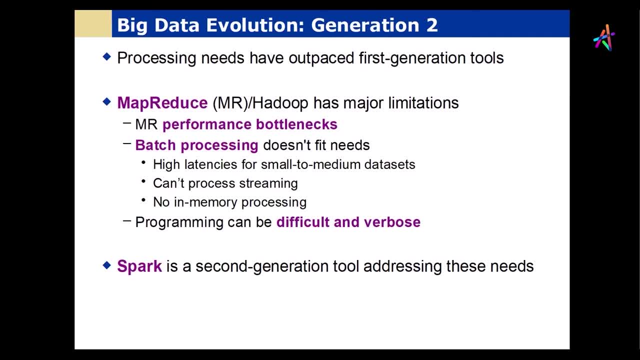 use case for data. The other problem was that it was processing data at rest using batch processing. It was not really applicable to some of the needs where we're wanting to process streaming data in real time, Because everything was done in terms of disk rights. the 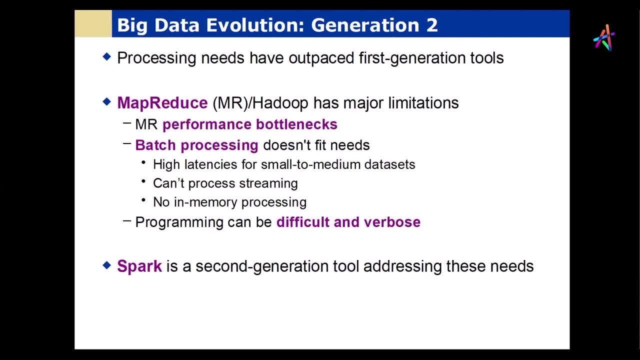 bottleneck in performance was often the disk access, disk speed, and there was a difficulty to optimize the performance because of this bottleneck that existed with this reliance on reading and writing to disk. It also had a programming model that was somewhat user unfriendly. It was very difficult and verbose, But again, 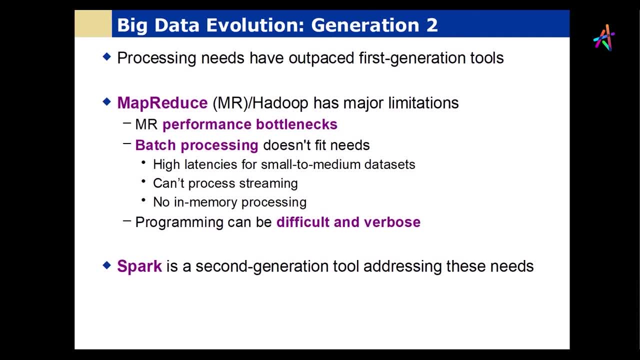 in all honesty, this was the first attempt to solve this problem, and it actually solved it in a fairly elegant way, given that there was nothing before that that did that, But it also showed there were certain deficiencies that needed to be addressed. Spark is a tool that was not intended to replace. 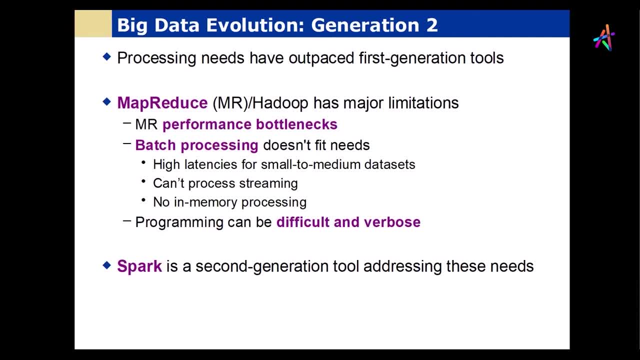 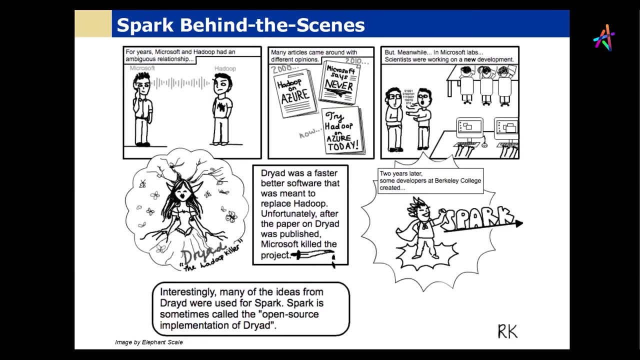 this approach, but was rather intended to sit on top of it and rectify a number of these deficiencies, More to fill in the gaps than to do any sort of replacement of what was there. So Spark is not saying this is the wrong tool or a new tool. Spark says this is a great tool. 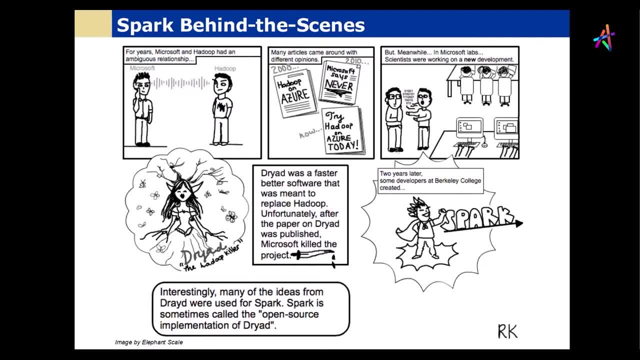 but you know what. it's not addressing certain issues and we're going to address those particular issues. I have no idea about this cartoon, where it came from or anything, but it's in the slides. But Spark comes out of a number of different approaches. 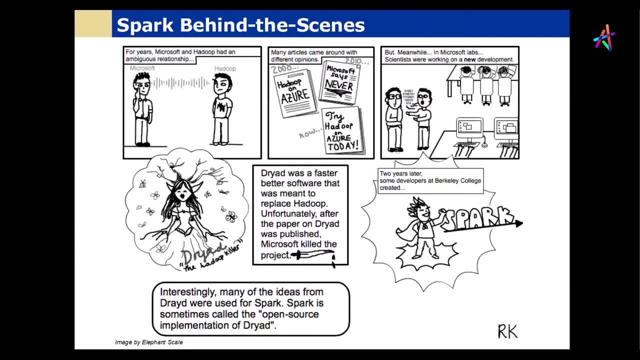 again in the industry. So Microsoft and Hadoop and Microsoft Labs and everybody's trying to solve this problem, And we do know that there was something called Dryad. Dryad was again, as you see there, the Hadoop killer, the original approach to say, well, let's get rid of Hadoop and put something else out. 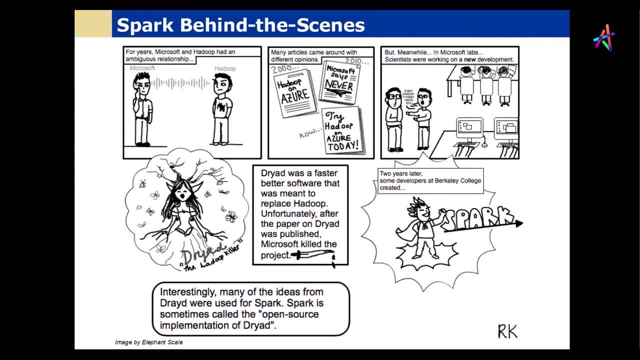 that works, And I believe this was at Microsoft, So it was better in software. but I think what happened was Microsoft, in their wisdom, realized that trying to replace something that was getting a large amount of attention and focus in the marketplace was probably not a good idea. There's probably other reasons. 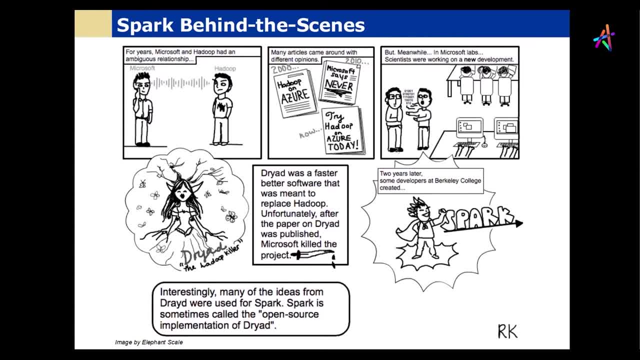 so they killed the project. But a lot of the ideas that were developed were recycled into Spark and that became an Apache project and took off And refocused itself from being a Hadoop killer to being a Hadoop colleague that worked along with Hadoop. So I think in the class we will be working with Spark in a 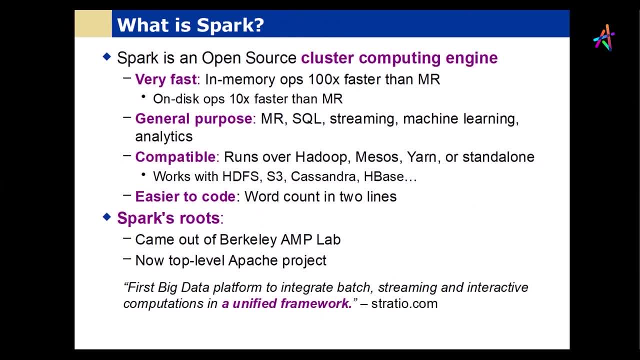 Hadoop and a non-Hadoop environment. Spark is intended to be a computing engine. It's not intended to be a big data storage system or anything like that. It focuses on the computing option, And the way it does that is with an architecture that focuses on using 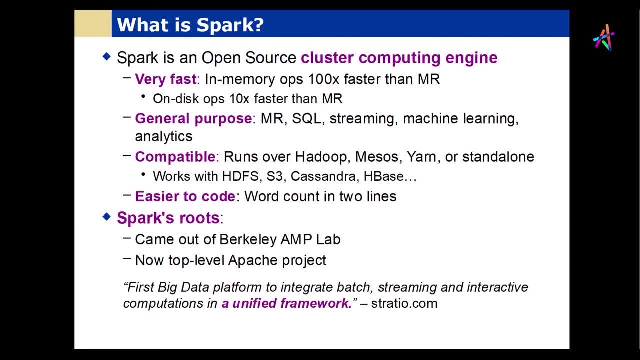 memory. Now, next week, we're going to be talking about things like Tungsten, which was where Spark has a number of subsidiary projects which are optimizing the in-memory operations of Spark in order to make it even better, in order to make it even more powerful. 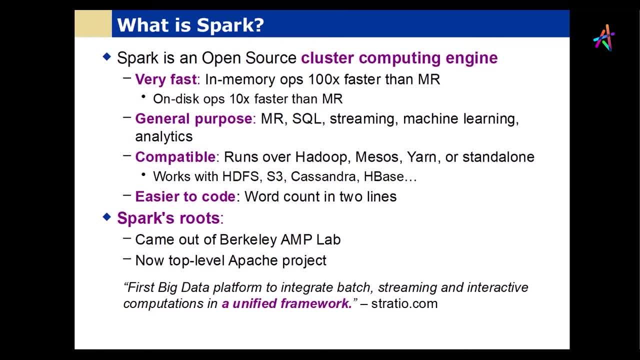 The disk operations are then optimized because there is a better relationship between what's going on in memory and what needs to go out to disk. So, whereas MapReduce is entirely- or not entirely, but primarily focused on reading and writing, the data Spark takes a different approach and talks about how do we maintain data in memory. 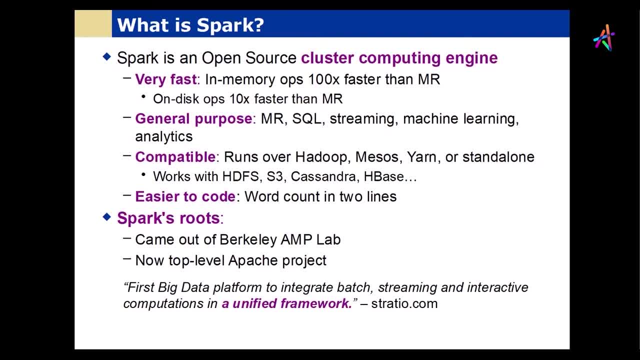 in a way that we can get much better performance. Also, Spark tried to address the issue of streaming data, and this is very important for real-time analytics, machine learning, particularly when you're responding in real-time environments, If you're doing security analysis, trend analysis, there's a number 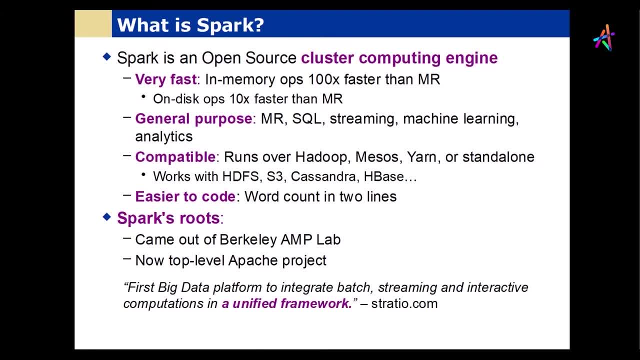 of things you want to do in real-time. You don't want to wait until tomorrow to get responses from that. The other approach that Spark took was to say: we don't want to create a new ecosystem, so what we're going to do is not replicate what's already there. So 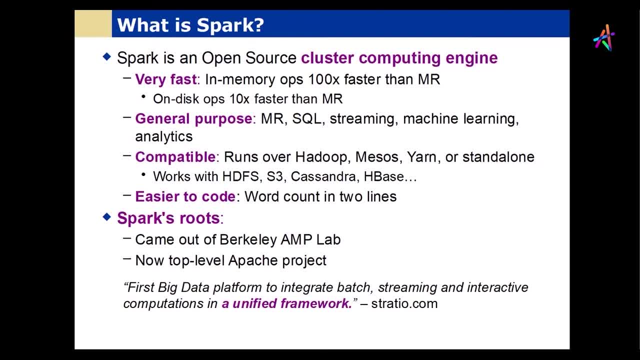 we're going to be compatible with Hadoop and the cluster managers, like Mesos and Yarn work in one of the standalone modes, So we're going to look with a number of other types of storage and data processing engines. So, rather than try to force people to choose between Spark and these other things, 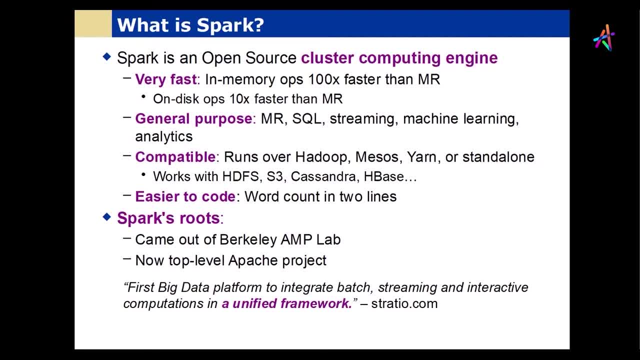 let's focus on what Spark is actually going to do and where it can contribute into this ecosystem. So the idea here is that Spark is intended to be a tool that enhances the use of all of these other products. It's also based on Scala, and when we come back and look at Scala, we'll see some of the ideas. 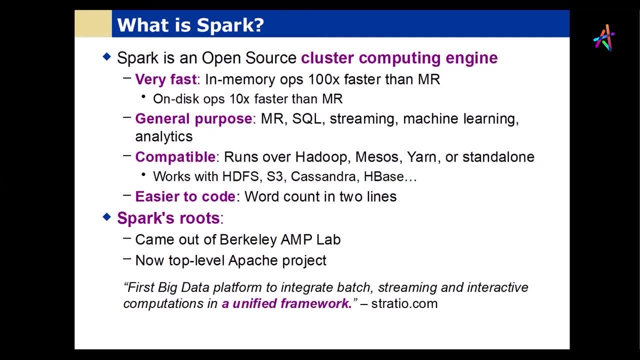 of Scala translate very nicely into a processing engine, which give us a very, very elegant way to think about how to process the data. So now Scala, of course, comes out of Spark. It's historically officially, after borrowing some of the concepts in Dryad, now a top-level Apache framework. 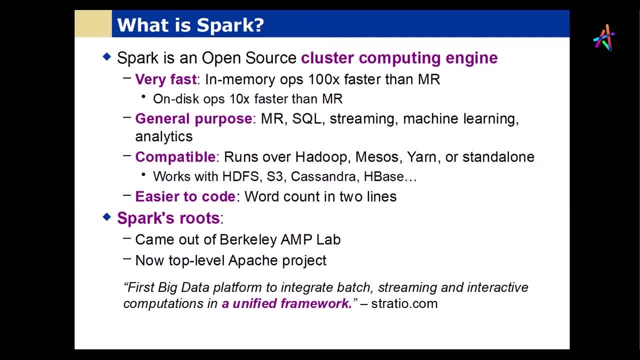 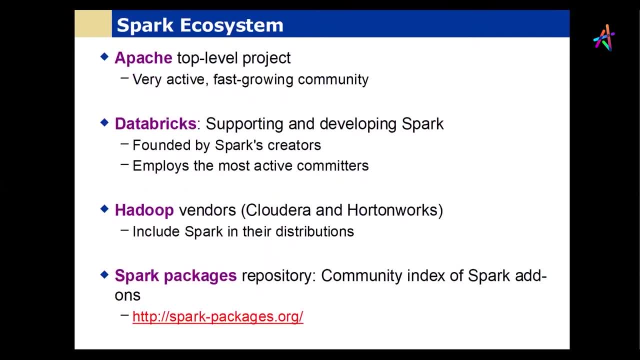 project and is now achieving a high degree of popularity because it fits those specific needs. A couple of people in the ecosystem is, of course, Apache, where it's got a lot of open source support. Databricks is a number of Spark creators, So there is actually a professional group or a corporate. 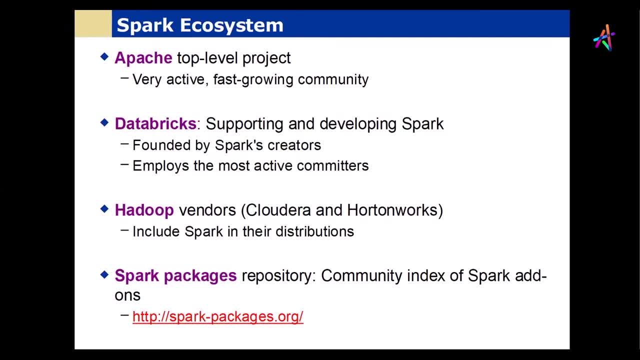 group committed also to supporting and developing Spark. So there's that interesting fusion between the open source community and a corporate community. The Hadoop vendors, like CloudAir, are also realizing that by bundling Spark it enhances the value of their product. so that Spark now 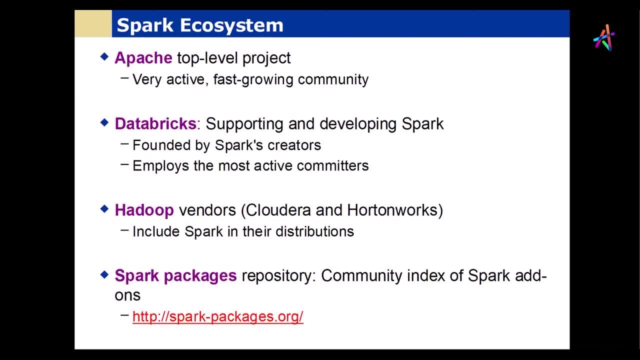 goes along with a number of those distributions And, like Ruby and its gems or Python and its packages or R and its packages, there is a large community index of Spark add-ons and I think that's. I think I had that link. We'll take a look at that a little bit later. So the idea too. 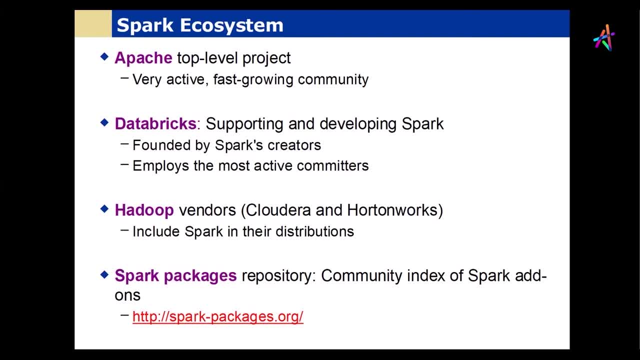 is that once you get a large community of contributors involved in bringing various kinds of packages that solve certain kinds of problems, you increase the overvalue of the platform. So this is that open architecture that means that adopting Spark allows you to have access to a number of packages that do things, so that 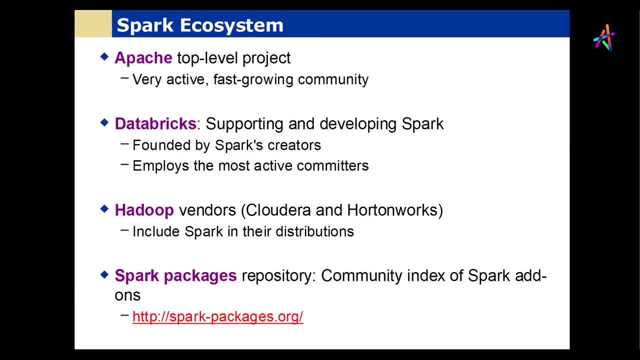 you don't have to build things from the ground up. As we know in Python, and especially if you've done any machine learning or data analysis in Python, you know that because there exist packages like Pandas and other very specialized packages, you don't have to invent things from the ground. 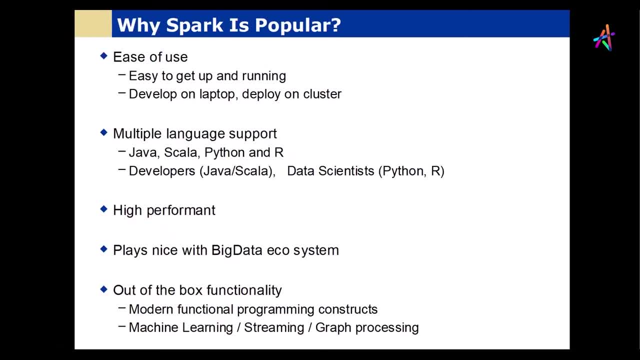 up. So this makes this whole thing very, very attractive. So why is Spark popular? Well, it's again. it's not an attempt to create an entire ecosystem, So it is a relatively compact package. It's elegant in the sense. 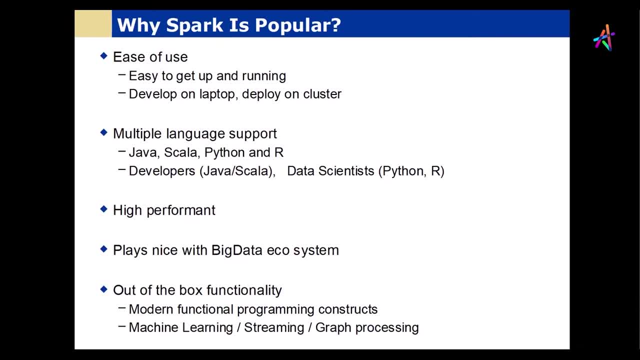 it's easy to get up and running. You can deploy it in a number of different environments. It doesn't depend on a particular technology. A couple of other nice things about it is that it has a number of programming interfaces so that it can interface with the. 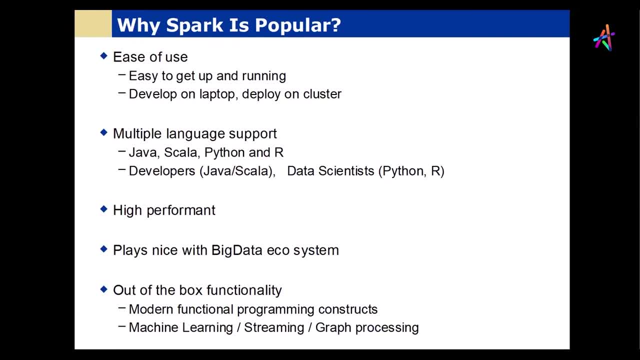 number of different development environments And they've divided it down into developers and data scientists here by language. But generally we're going to focus on Scala in the course And my personal opinion is that you really are able to get more performance out of. 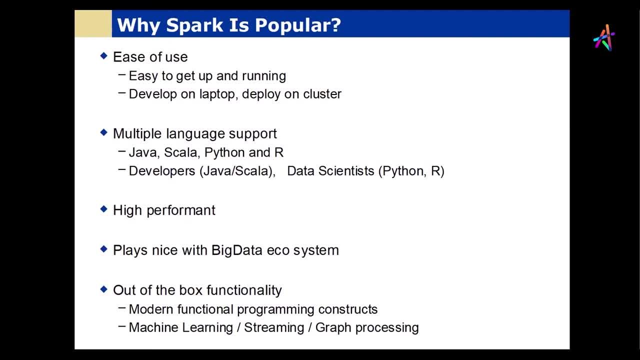 Spark. You're able to use it more effectively with Scala because you're thinking using the same paradigm that you're when you're programming in Scala. that was used to design and encode Spark, So there's a natural relationship there. High performance plays nice with big data ecosystems and 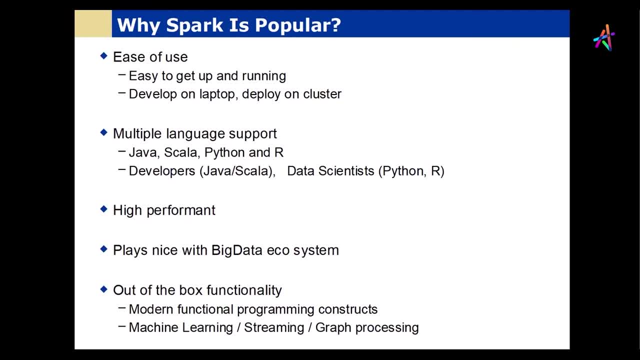 you can pretty much use it out of the box. And the thing we're going to focus on a little bit more this morning are these functional programming constructs and concepts. We're not going to be so much interested in the other kind of applications, The 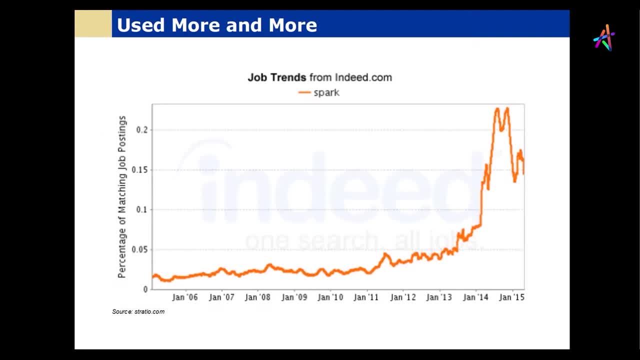 job transfer in Spark. just to give you an idea of its adoption rates so as of 2015,. you can see there was, by the way, that big spike I think is because there was that new release of Spark around that time. 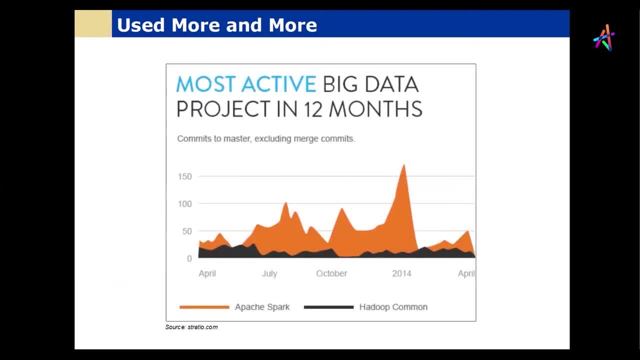 But there is obviously a trending up. good measures, One of the most active big data projects. again, this spike, I think, is around one of the major releases, of Spark, But you can see it's a pretty significant community. This is where things 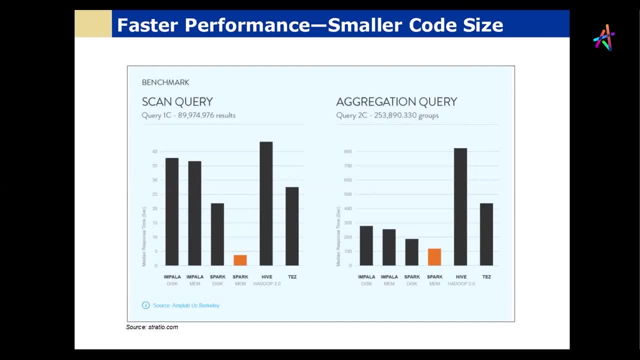 can really get interesting, And one of the reasons why Spark is working is when we're actually looking at benchmarking in terms of median response times, You'll notice that Spark, because of its architecture, is outperforming most of the other kinds of products that are doing this Now, other kinds of products. 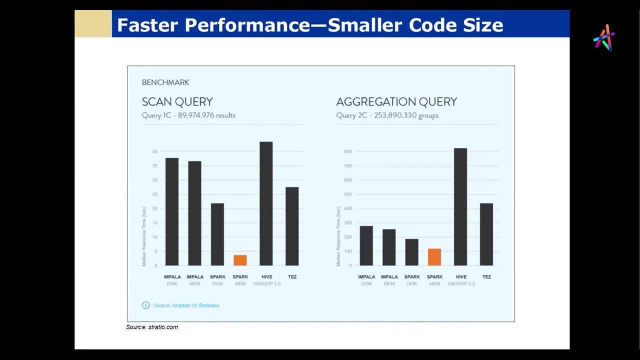 have advantages, but where Spark is really focused is on speed of performance in performing various kinds of queries and various kinds of data manipulations. So we are seeing this sort of high performance turnaround, which is what makes it really really interesting. You'll also notice the difference between Spark, where we're 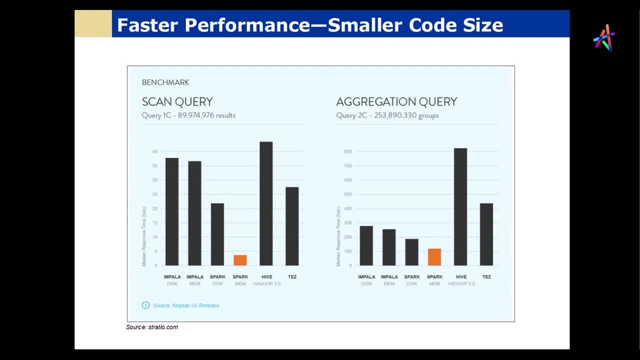 using a lot of disk access and Spark, where we're emphasizing memory. Even with the disk access, the architecture of Spark is producing significantly better performance than the other products, And once we move to more of an in-memory model and emphasize the in-memory model, then our performance improves even beyond that. So this is 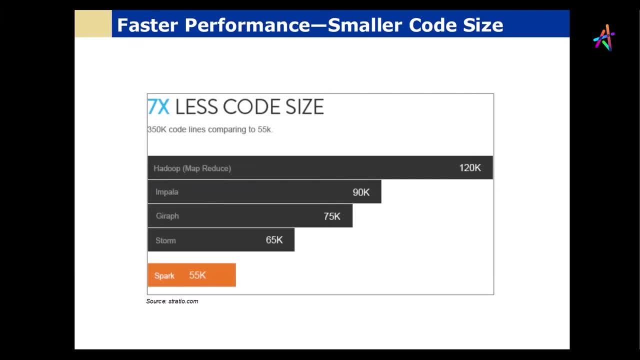 the kind of performance issue that makes Spark so popular. The other sort of thing we look at is the usability portion in terms of code size. So we have large amounts of code for other products but we again, partly because of the functional emphasis, have a small amount. 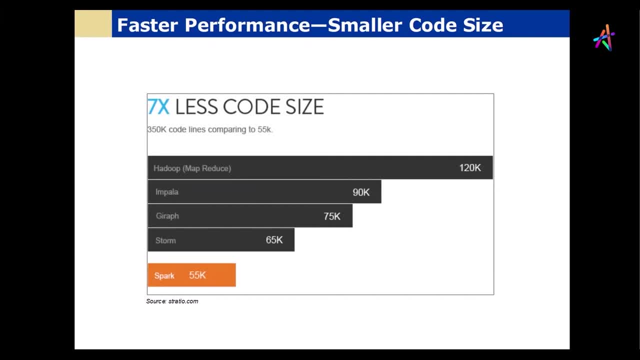 of code that performs the equivalent function in Spark. That again comes from the idea that most functional programming languages actually do more in fewer lines of code. The challenge we're going to look at today is: how do you think in a functional programming paradigm- And for those of you who have done Odetsky's course and other things, you 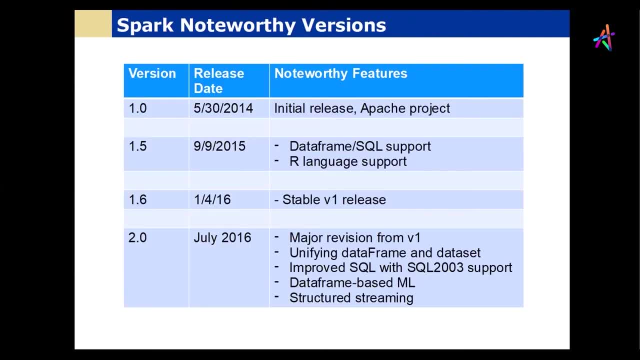 notice that it does require you to think differently about how programs work. All right, so there's some noteworthy features here. So the again we got that initial release in the Apache project. There's 2.14.. There's that big bump up And there have been a number. 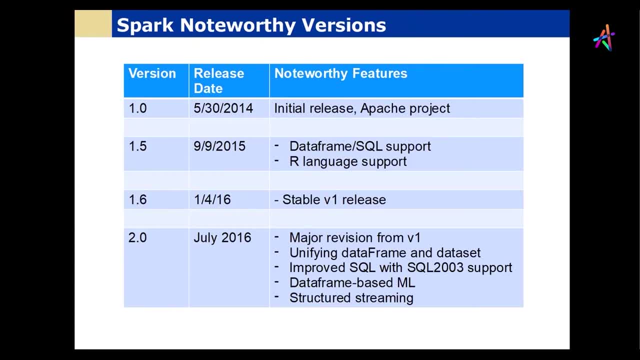 of incremental improvements in Spark. The original version of Spark uses something called resilient data set, And the was a really interesting innovation, but it still wasn't as good as Spark could be, So subsequent releases of Spark introduced something called data frames, which improved performance even more, And then 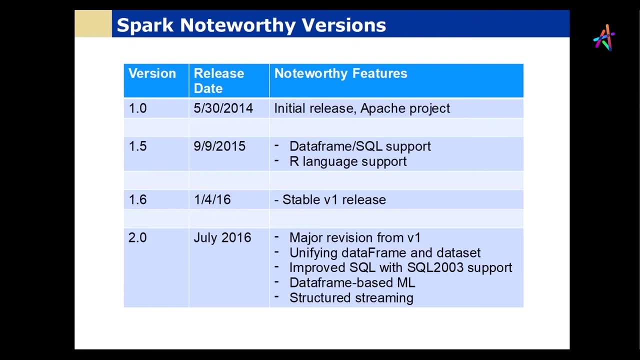 we finally moved into something called data sets in version 2,, which provided an even better model for working with data, And so the evolution of Spark has been along the lines of improving the ability to structure and manipulate data and get improvements on that basis. 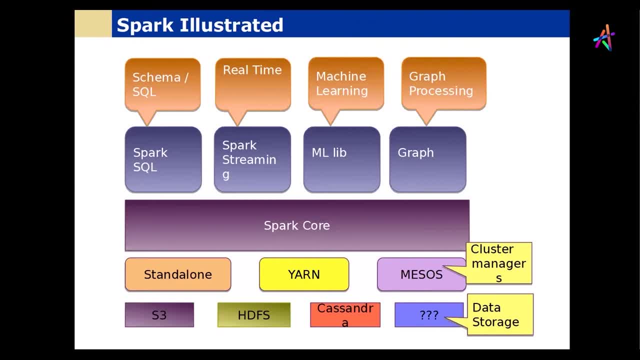 Here's the Spark architecture in terms of how it fits on with other environments. Down at the bottom is the data storage layer. And, again, one of the questions I hear people saying: well, should I do Hadoop or should I do Spark? And the answer is: well, that's. 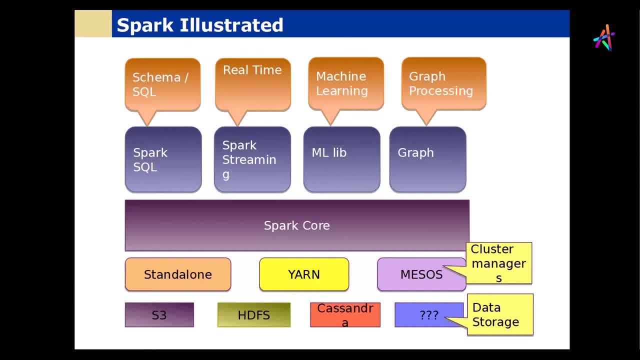 an irrelevant question, because they are designed to work together. The Spark itself is intended to cooperate with a cluster manager, which is the, of course, the type of application that manages the distribution of work and other tasks on the various clusters, And it also has 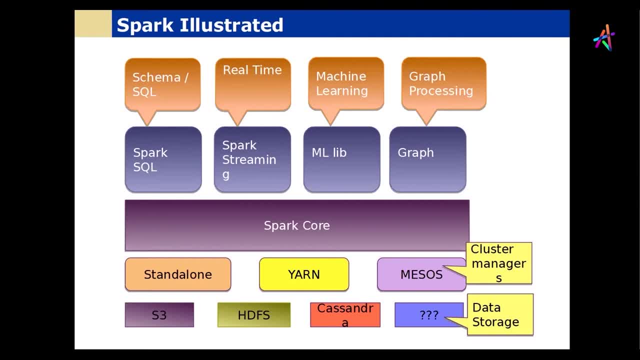 a standalone manager as well, So it can actually work directly with HDFS and other environments. The idea is that the Spark core delegates, or does not try to duplicate, any kind of the work that's already being done at this layer. It is intended instead more to sit on top of it Once we have the Spark. 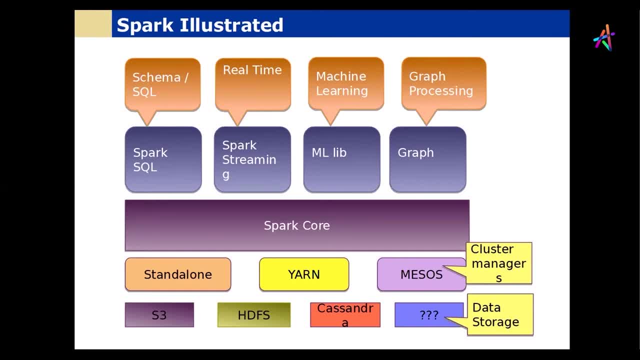 core. there's a number of packages that get plugged in on the top of Spark that now are able to do various kinds of tasks or adapt the Spark engine to tasks. So Spark SQL involves us being able to use SQL, and Spark streaming allows us to be able to work with streaming data Machine learning library. 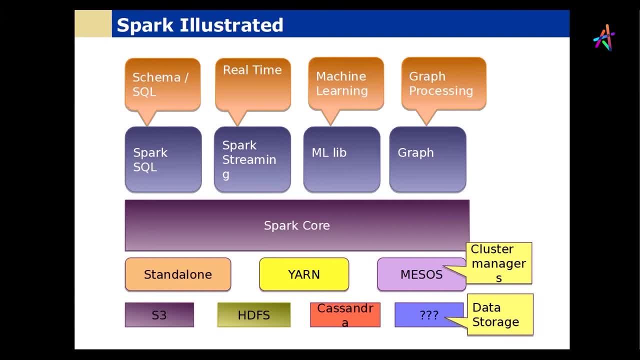 again gives us a machine learning component that sits on top of Spark. So rather than have Spark do all of those things at its core level, those are broken out into individual modules, similar the way that you can think of Python as having packages or Ruby as having gems that encapsulate various chunks of functionality. 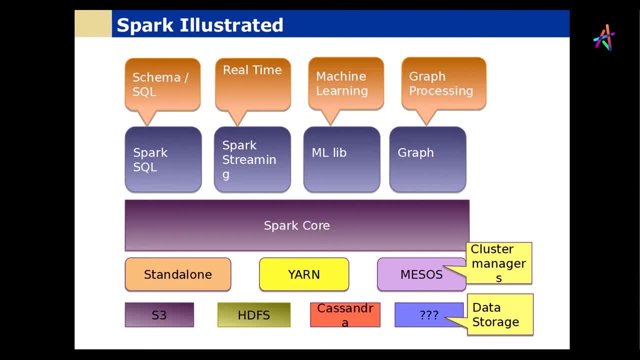 that have certain applications or are applicable in certain ways. So, in terms of its overall architecture, what we're really going to be focusing on this course is this Spark core piece, with maybe some reference later on in the week to a couple of these other modules, And we'll also be interacting with a number 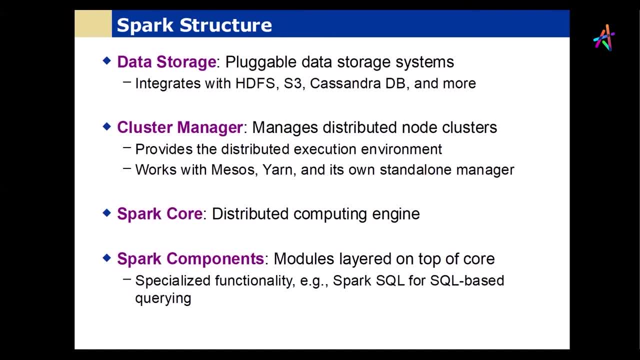 of these other components as well. So the idea behind the unplugable storage is that you want to have Spark freely able to use all these different kinds of storage mechanisms. You also want to be able to integrate with various cluster managers. In the absence of a cluster manager, it does have its own. 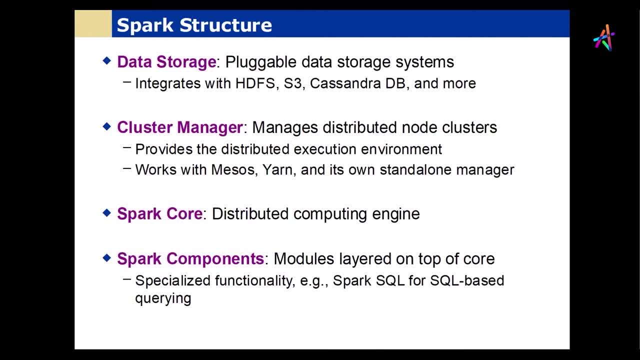 standalone manager, Cluster managers, meaning the thing that coordinates the various clusters in our data storage environment. And the thing that again we're really coming back to here is the distributed computing engine, which is the focus of this course, And then the Spark components, which are the modularization. So that's. 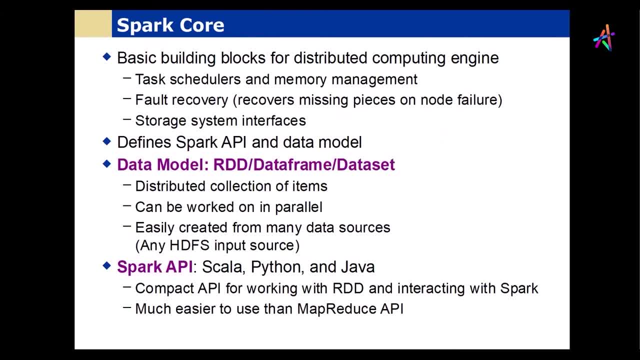 the idea of the Spark architecture. Spark has a couple of features that are important to emphasize. The one is that it has things called task schedulers and memory management, where tasks are units of work that can be done on a particular node without having to reference other nodes, And 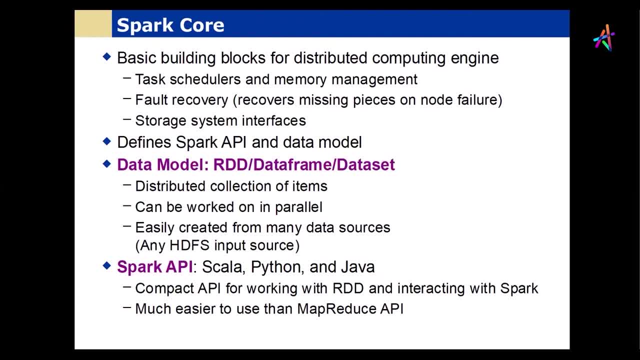 part of the optimization is going to be looking at how tasks schedulers work and how we do things called shuffles, which is where we have to reorganize data on the nodes in order to do an appropriate sort of computation. We also have this memory management model, which, again 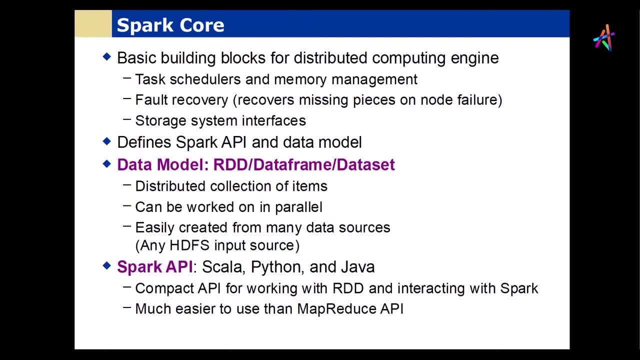 we'll get into with Tungsten to look at how memory management is being optimized through the use of some innovative ideas. Fault recovery: this is an important thing, So we want to have a complete failover, transparent failover ability so that if we do have a failure of a node, 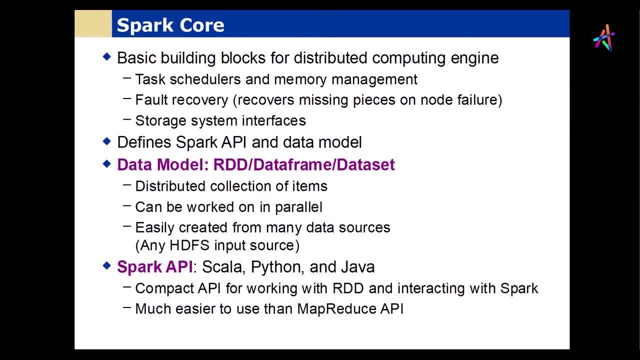 or we have a failure of a partition of data, we're able to fully recover that without any kind of downtime. So we're going to talk about fault recovery and the interfaces to the storage system. So we're going to get into each of those kinds of 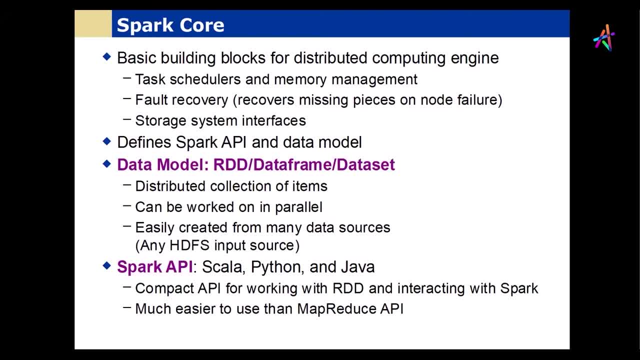 ideas as well. Spark uses a couple of representations of data and these have evolved over the years, So each one sort of builds on the other or complements the other. We'll look at each of these: RDD, distributed, resilient, distributed data sets- that's RDD. 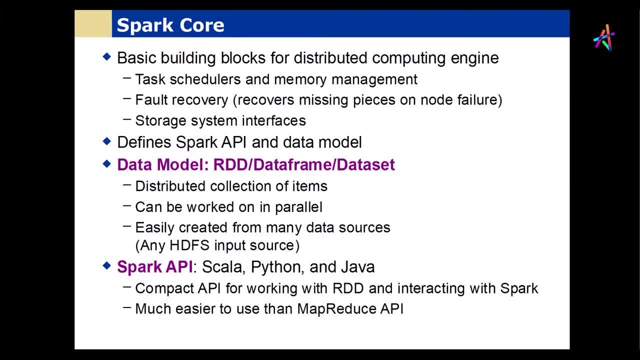 data frame and data set, and each one of them introduces innovations which allows Spark to process even faster. So the idea is that the data model and how it is being distributed on parallel is going to be opaque to you, more or less. That's going to be all delegated out to the how we take. 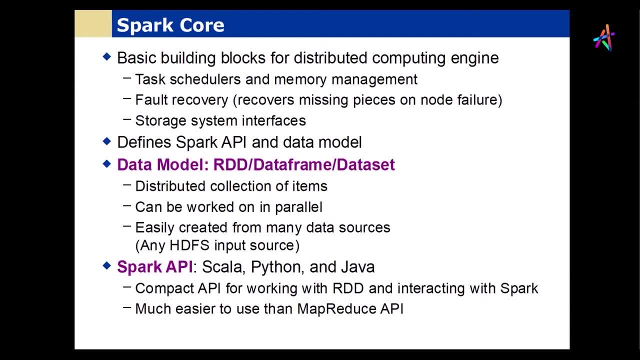 one of these resilient data sets. distributed data sets and how it is getting distributed out there should not be of a concern necessarily to you when you're focused on the processing of the data, although there will be considerations that you have to take into account. This gives us the parallelism and the 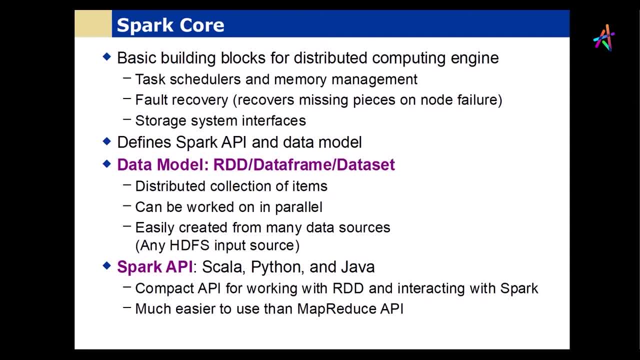 other ideas that we can create these RDDs, data frames and data sets from various kinds of data sources, just not an HDFS input source. but we can create it from text files, from in-memory data. We can do the ideas that Spark doesn't really care. 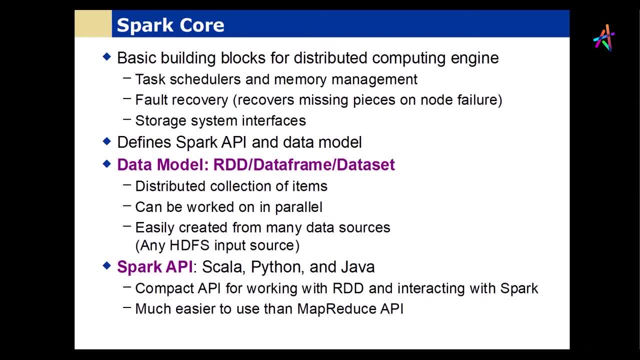 where the data comes from. What it's interested in is putting it into a form where we can get this high degree of performance, and we'll interact, of course, with the APIs on that. So the components that we're looking at are structured data where we can support SQL. 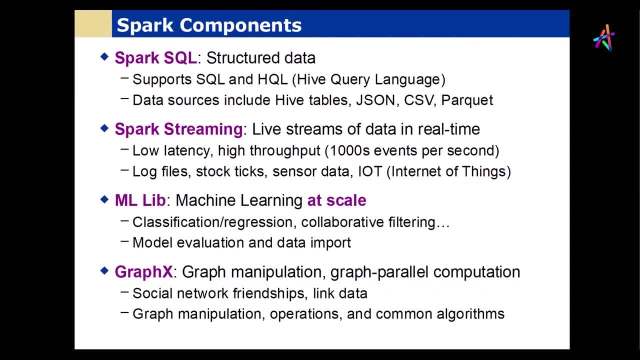 types of operations and for that we can take any kind of data that's structured in basically an underlying key value pair kind of model. So you can argue that tables and SQL tables are sort of the idea of a highly structured key value pair. So Hive tables, SQL tables. 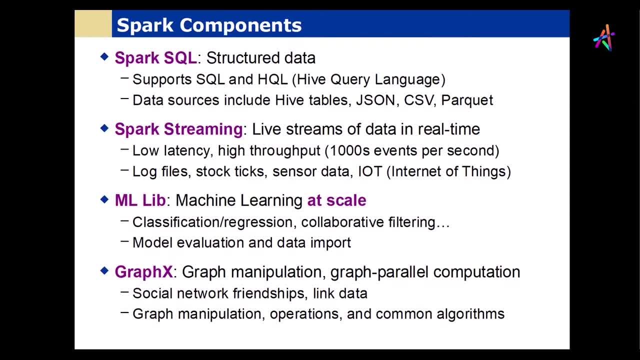 JSON data fits into the same category: CSV files, anything that would be representable in the spreadsheet Parquet, which is another data format. So the Spark SQL is a module that works with data which has a particular kind of structure to it. that's familiar to us in the QL. 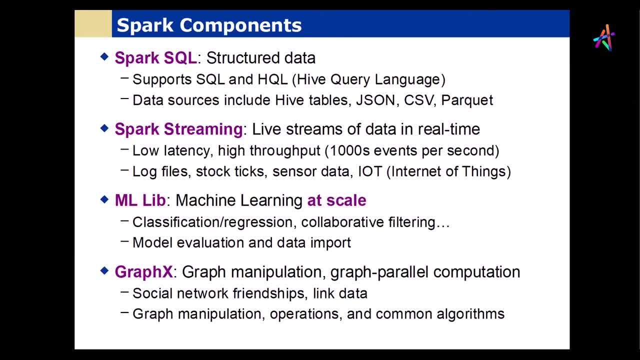 language worlds. Spark streaming manages a different kind of data, So you're looking at things like the example sensor data in particular internet of things. So there's another general application area. I do believe that's not something we're going to really touch on much in this class. Machine learning at scale. 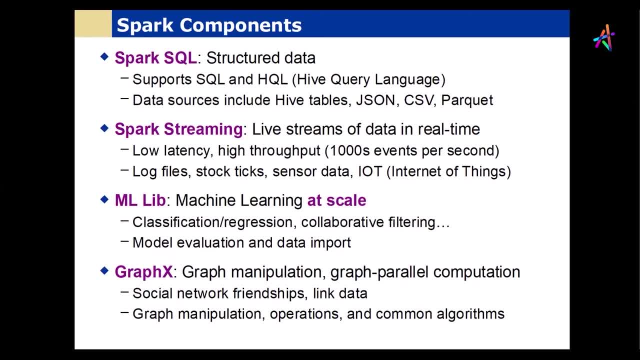 again requires massive amounts of data processing often and we might mention some of the applications, but we're not going to get into the machine learning at scale. But again, notice that these are very different application areas so we don't want to put them into the Spark core, We want to keep. 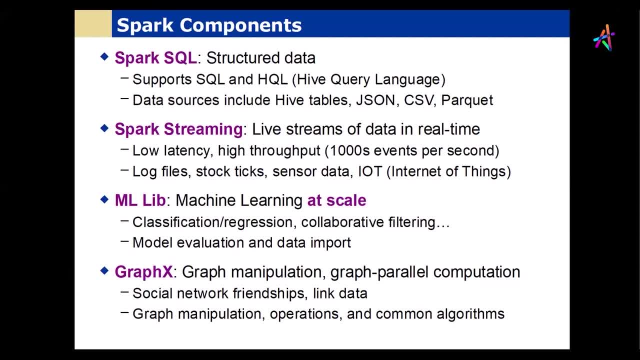 these as add-ons, And GraphX and graph manipulation is again another big area that's out there- using graph data sets and looking at associative relationships and other sorts of things. So there are a number of different components that get built on top of Spark. 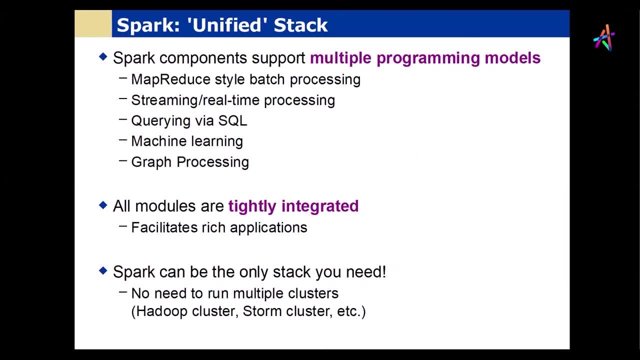 Okay, so you should get basically an idea here that what Spark is is this core which we're going to look at, which is this model of how you process data quickly, in real time, and manipulate data, And that is going to talk at the lower end to the various 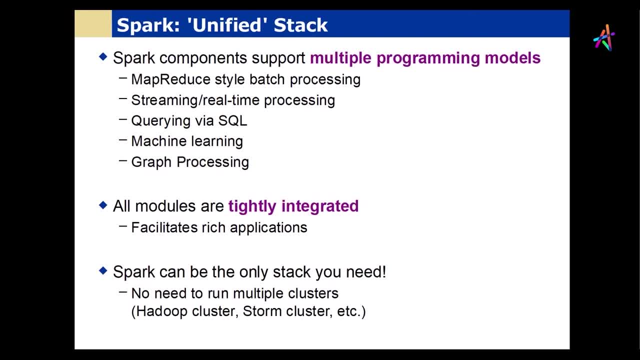 data storage systems, data availability systems, And then, on top of that, you've got these other modules which are going to add functionality for particular application domains or particular kinds of data processing that we're doing. Okay, so that's the first really big takeaway is just get a sense of this architecture. 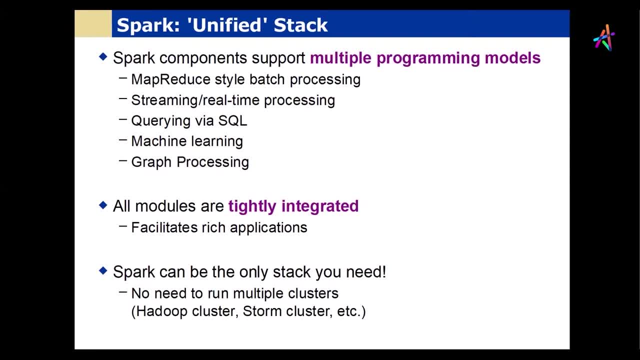 The modules are also what we call tightly integrated, so that they work in a very, very seamless fashion. Now, I'm not going to claim that Spark is the only stack you need, but because it runs a standalone, it could be the only stack that you have, but I will leave that as a 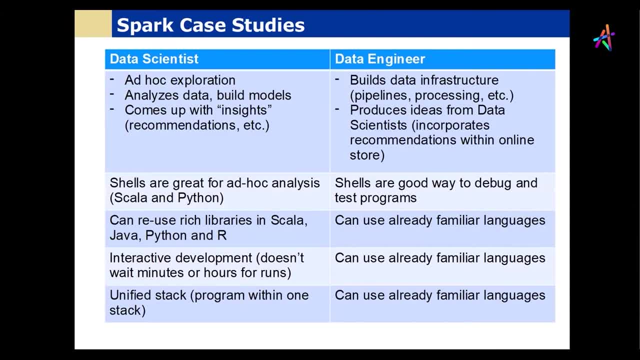 debate to purists as they want to go through that. This is a table I'm not going to spend a lot of time on, just basically, somebody's divided this down into the two kinds of approaches that people take: looking at data, The data scientist. 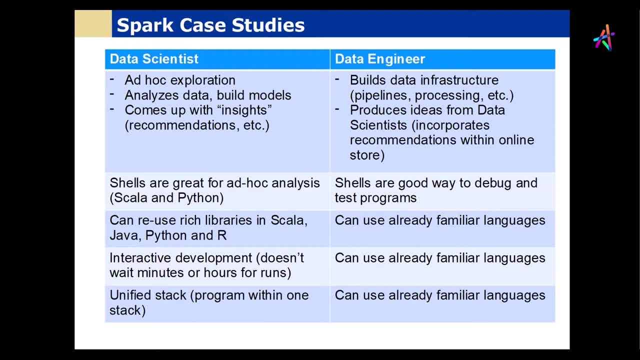 versus the data engineer. The data scientist is focused on. the data engineer is more focused on the infrastructure that surrounds the data. i think that's how they've kind of broken this down. um so again, building a data infrastructure versus ad hoc exploration. um so the a couple of the the ideas here is that there are probably some different kinds of shells. 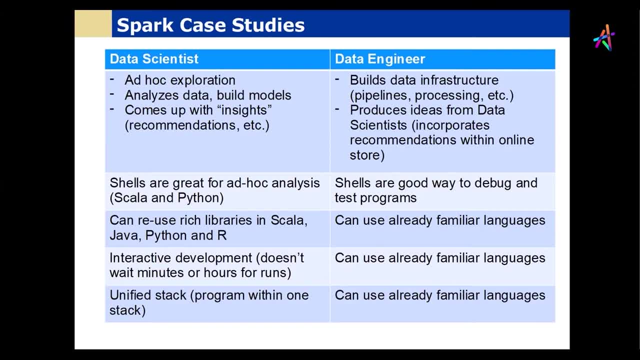 uh. data engineers often use things like are, uh, and the other thing we want to be able to do is to use uh, leverage existing libraries and work that are that are there. interactive development: again short turnarounds for data scientists when we're doing ad hoc exploration. 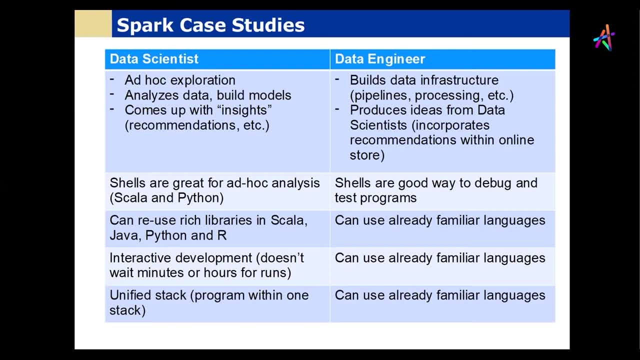 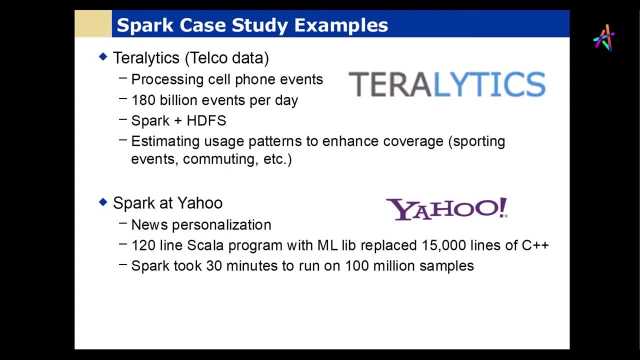 and uh the uh. again, the reuse of being able to use uh programming languages, a couple of these uh cases where it's actually being used. i'm not familiar with the details of some of these uh, although i do know of of uh. i have wonderful reports of what people are doing with spark. 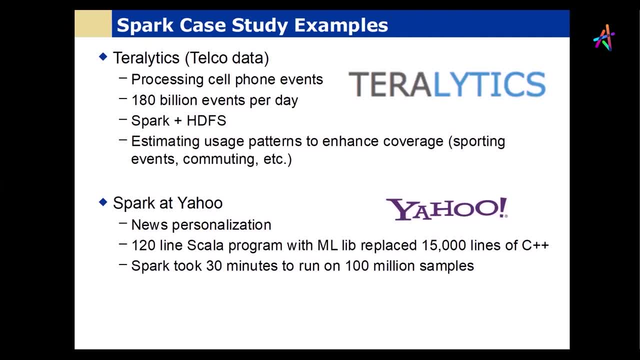 uh, so teralytics, uh, telco data- uh, this is an example of of using more large amounts of data. this is really important for phone companies because what they have to do is telco resources at a hardware level- actually very expensive- and being able to actually predict usage patterns. 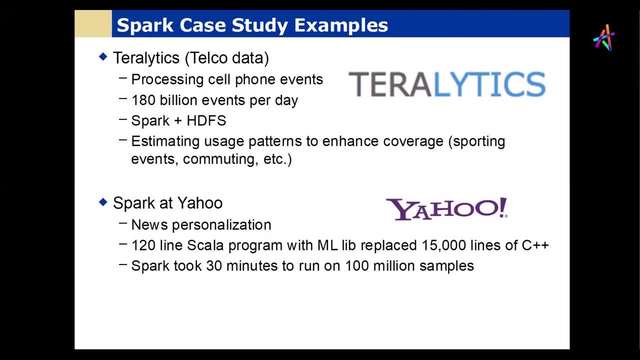 enables them to be able to do very, very effective cost planning. so, for example, estimating usage patterns to cut, to enhance coverage. one of the things that they know in north america, for example, is that all telcos know that the largest number of long distance phone calls are placed on mother's. 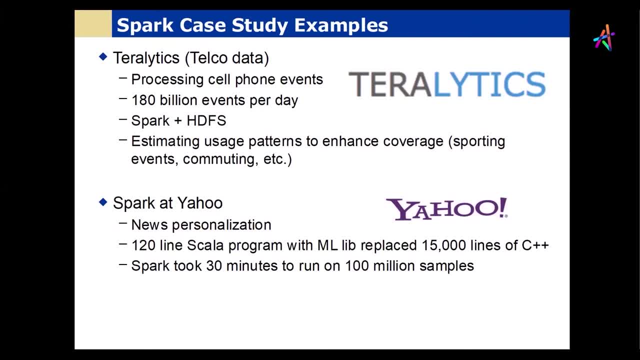 day. so on mother's day, you have to make sure that you can handle the stress of all those extra calls. and they also know that the largest number of collect long distance calls are placed on father's day. so having historical data to enable them to to know that uh enables them to be able to respond to. 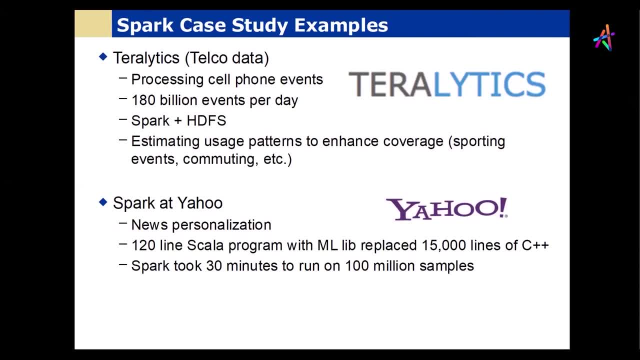 those effects and we get various kinds of peaks, uh. so, for example, we also know that that they, on an average day, the the two peak times for making phone calls are generally right after the start of business, when people return calls, and just before the start of business when people start. 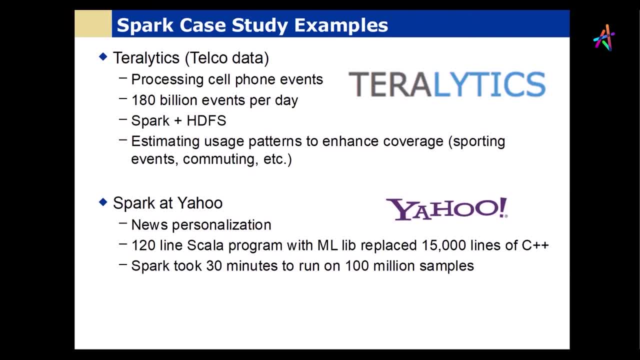 calling home. so, uh, we know that by analyzing data. so now, with spark, you can analyze these 180 billion events per day in a much more effective pattern and get your, get your uh patterns to become much more accurate. we get uh, which with um, better levels of tolerance. yahoo is another example. uh, and this is actually 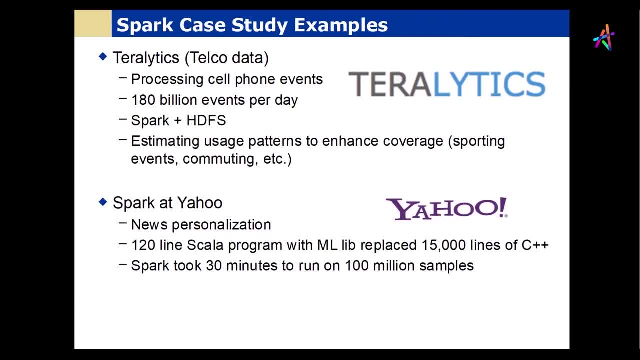 a fairly impressive number: 15 000 lines of c plus plus. now i i um somebody said they had had built originally a database in c plus plus. i actually did the same thing too with my team uh back in the 1980s um relational databases were incredibly expensive and we got some uh stuff from mit ai labs. 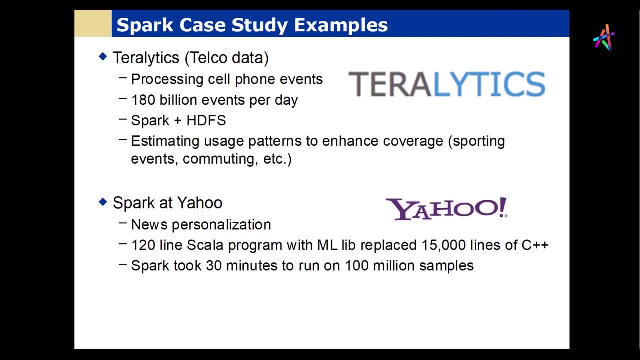 that enabled us to uh write, uh, uh, a really sort of primitive relational database in c plus plus, because we couldn't afford the fifteen thousand dollars a license everybody was charging at the time, uh, so i understand how difficult it is to write some of these things in c plus plus. i do. 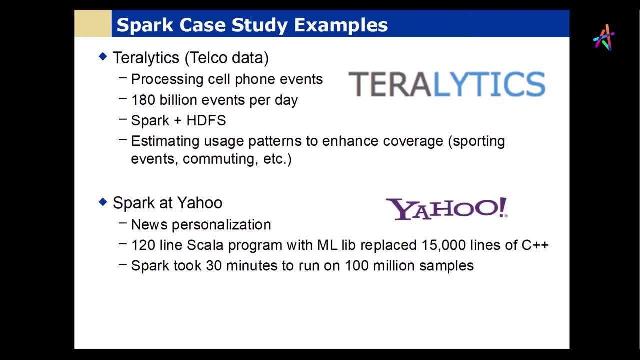 love the language. but yeah, 15 000 lines being reduced, 120 line scholar program- uh, that is a real performance booster. the spark took 30 minutes to run 100 million samples. that again, is pretty. uh, uh, uh, it's. it's a good thing. right in the last few months it's a very, you know, it's a good thing. 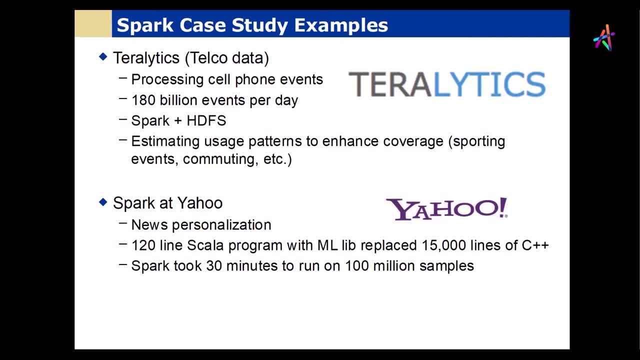 but i think it's a very good thing to do and i think it looks like um a completely different approach from what i've seen um in uh in the past, and the reason for that is that we understand that, just like every machine, that we can kind of change the way we write data. 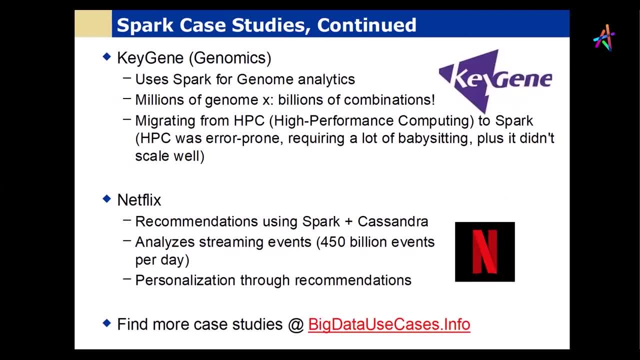 there's a lot of information out there that's not like, really it's not going to be there, like the fact that, uh, you know, we're not going to want to change how we write data for the sake of the size that we're working with and we need something that's really updated and that's 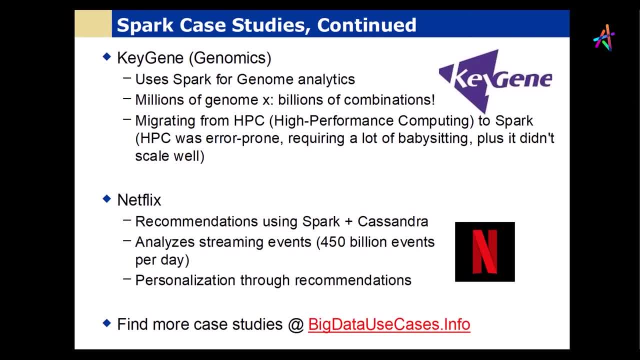 going to be really good for the machine, and i think that's something that you'll really need and not something that you'll need to make new changes for. it's not. it's not a really good new. enables us to actually do this kind of- I shouldn't say us, because I'm not doing it. 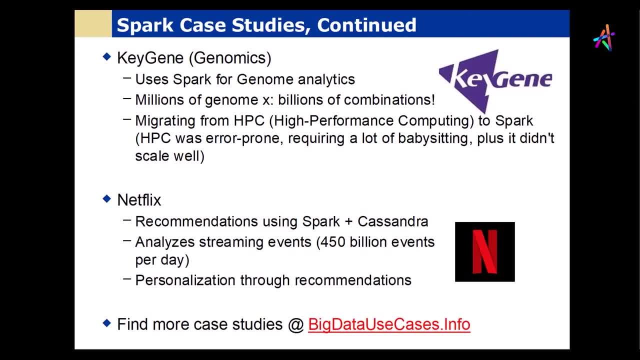 but enables people to do this kind of genomics. What people can do with genomics now is absolutely astounding, And that is really built on the ability to be able to process these large amounts of data. Netflix: this is where Spark is sitting on top of Cassandra analyzing streaming events. 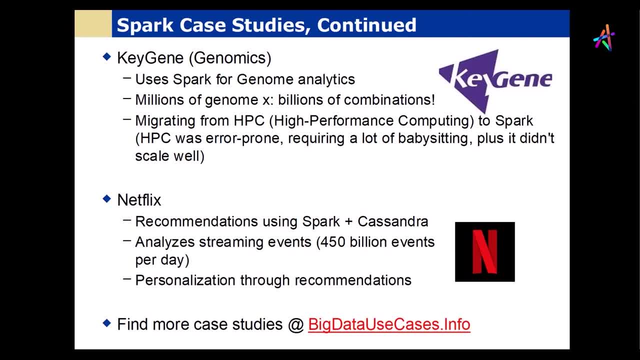 and doing recommendations. When I do have time to go on Netflix, the recommendations are always wrong, but that's because I'm probably not using Netflix right. But again, these recommendation systems in various cases are not just the ability to collect the data but also to analyze the data. 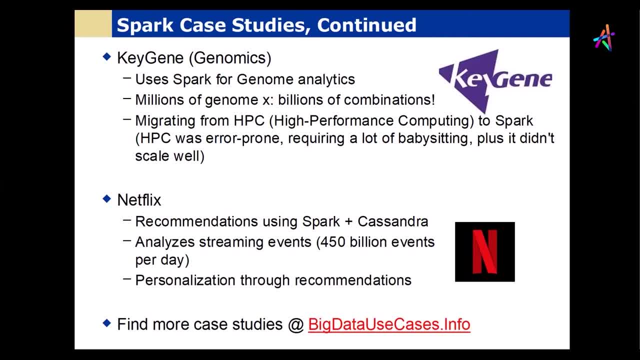 very, very quickly and not having to write massive amounts of code to do it. So the key leverage around here is not: oh, here's some really interesting cases. What we really want to take away from this is: a lot of these cases are possible to be able to deliver the results. 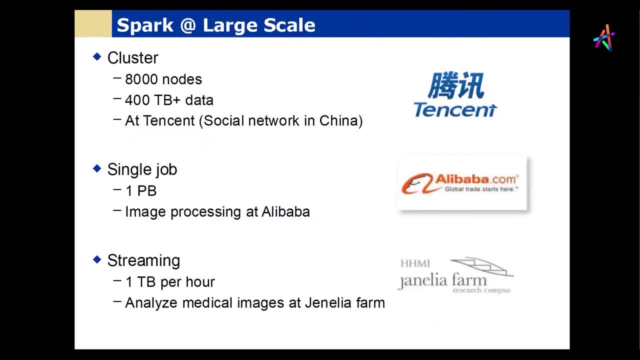 simply because we have something like Spark that allows us to be able to do this in a really effective and elegant manner. Example: the Chinese social network: 8,000 nodes, 400 terabytes of data. I think that's just mind blowing. Alibaba has a one petabyte job doing a single job one. 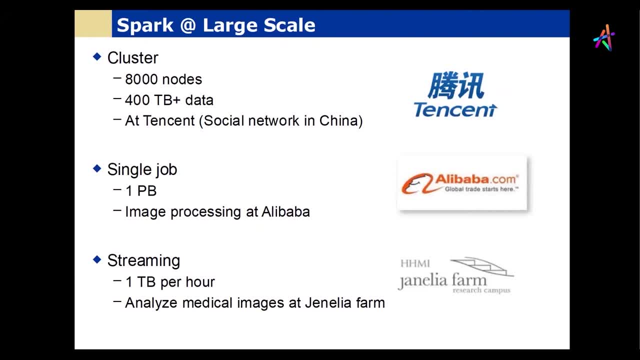 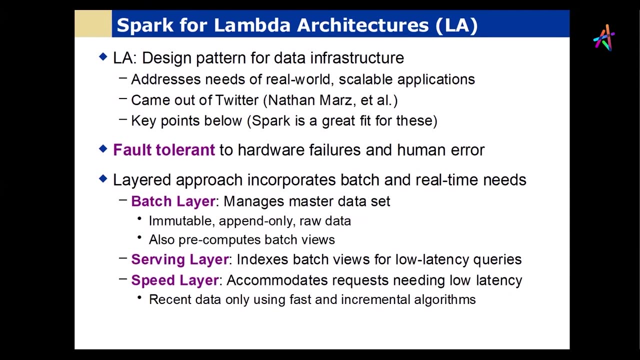 petabyte. This medical images at Janelia Farm. again, massive amounts of data, And while the storage systems that scale can manage this data, it's the idea of the Spark model gives us the power to do that. There's one other architectural thing we'll. 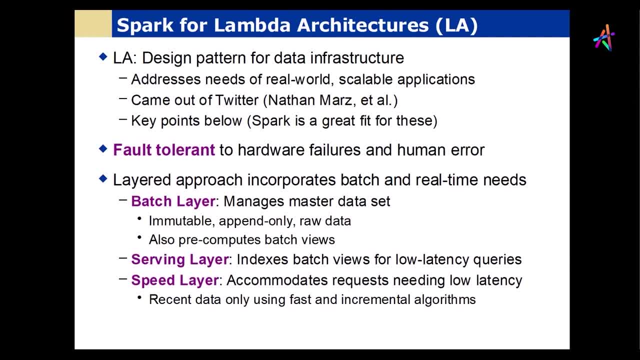 look at here just before we get into a little bit and do a little bit more, and then we'll switch back over to Scala, And this is called the Lambda architecture pattern, which is an interesting approach which tries to leverage the strengths of these systems in multiple 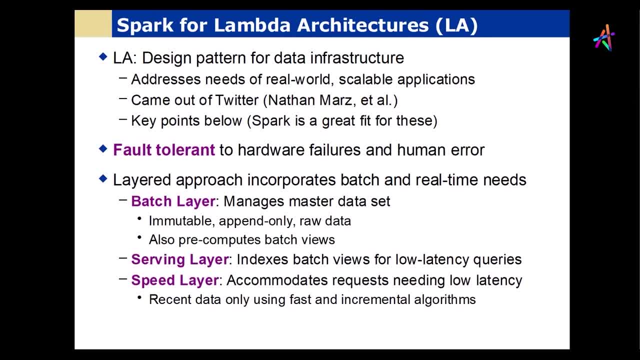 environments. It is a pattern that Spark works really well with, and it's a pattern that's becoming increasingly important, And this is where we're trying to work with a, and this is a problem we found in sort of- not sort of- but in data warehouses as well historically, where you would 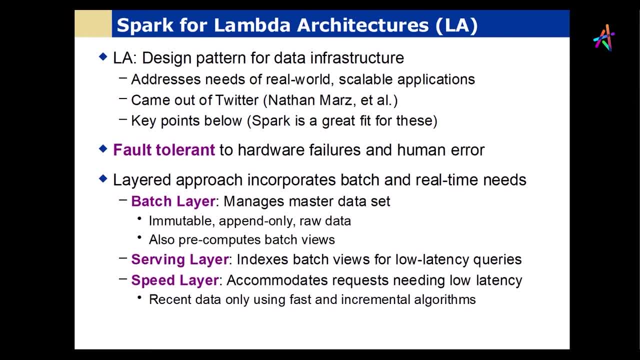 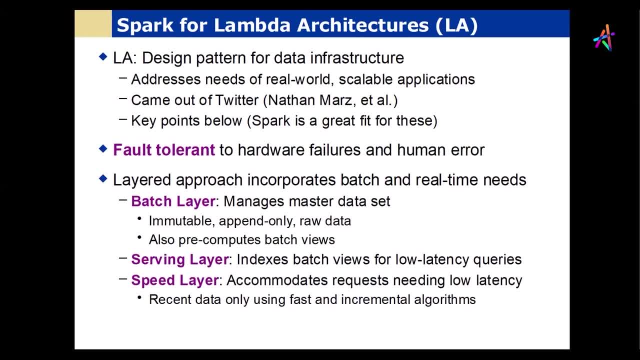 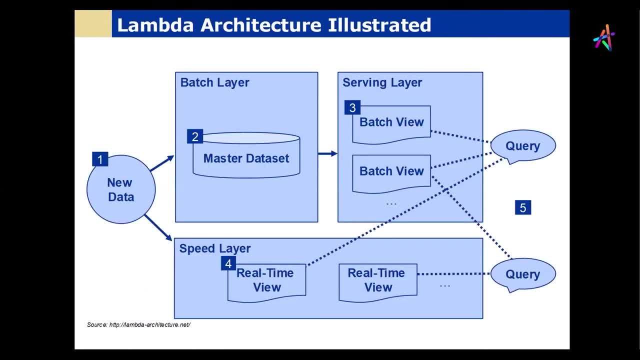 real time components, this accumulated margin of data that you had to want to get access to. So the Lambda architecture works, where we have split down our data into two kinds of storage streams. One goes into a batch layer, which is our master dataset, which can 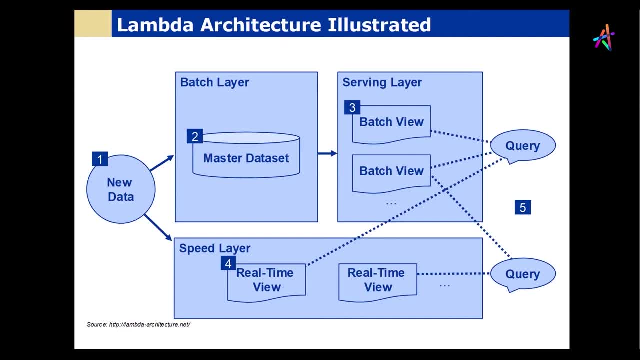 be considered to be the accumulated repository of the data And that can go through various product components, specific parts of the data. One can be the assets, physical properties, processing models, to produce a serving layer with different batch views that can be queried. 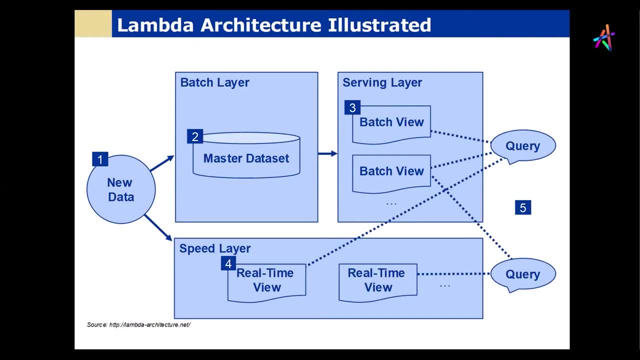 And that would be a typical historical kind of data warehouse approach or a more ETL type of approach. And then on parallel with that, you've got the speed layer, where a new data is also in addition to going to the master data set, is also being put into a very fast real-time view. 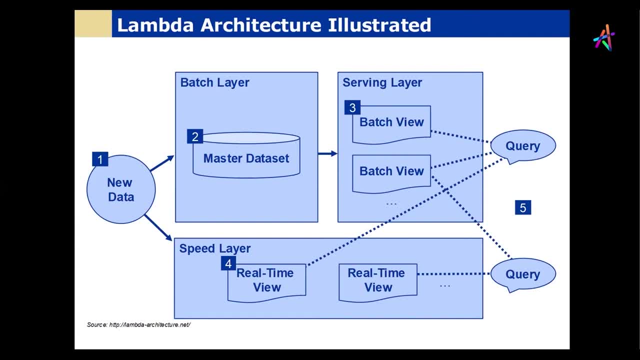 of the data which you can also query. So your queries can now incorporate both real-time views of the data and batch views of the data to give an integrated, up-to-date model. So the idea is to split the data into two- so we call them holding areas- and then being able to run an integrated 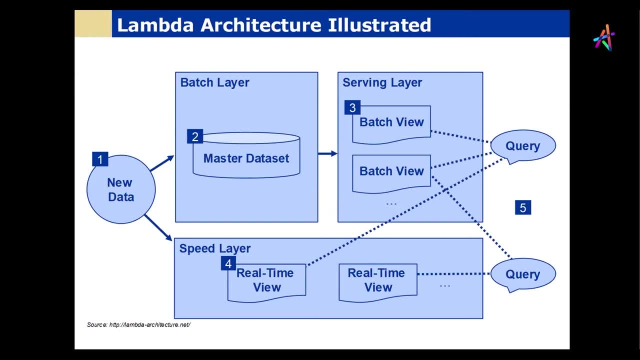 query on the two holding areas. This is called the Lambda architecture, although I've got to tell you I'm not exactly sure why it's called the Lambda architecture. That's just the name somebody came up with, But I'm sure there's a good reason for it that I just haven't found it. 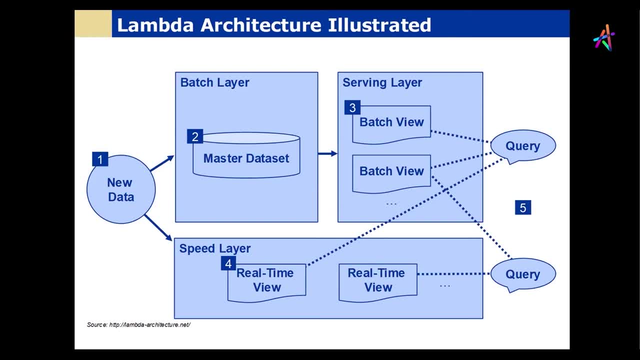 I can give you an explanation, because you basically have two branches and the Lambda letter is. That is a good explanation, if any. So I will go with that. That's a good, I'll go with that one, But, as you can see, this is an architecture that solves a number of sort of problems we have. 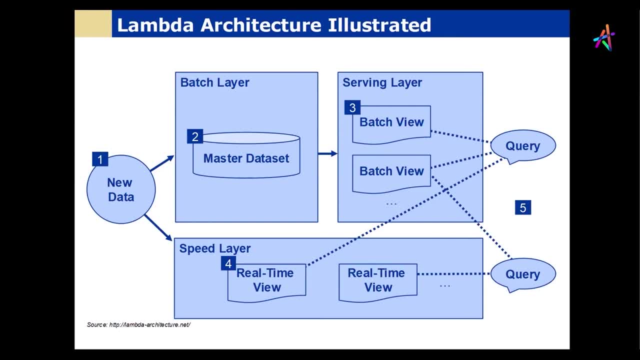 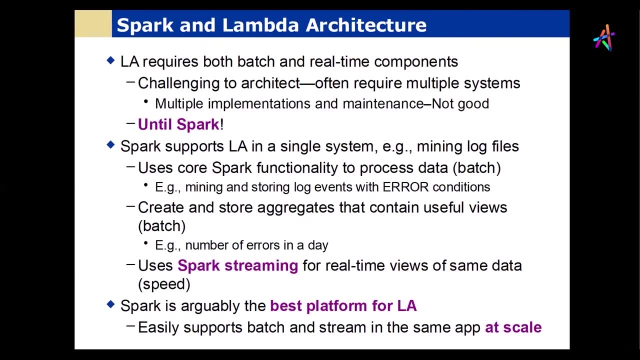 in trying to deal with both historical and real-time data at the same time. Thank you for that. I appreciate that insight. Okay, So this is the challenge that we've got here In that kind of architecture is again: how do you integrate these two disparate kinds of data? 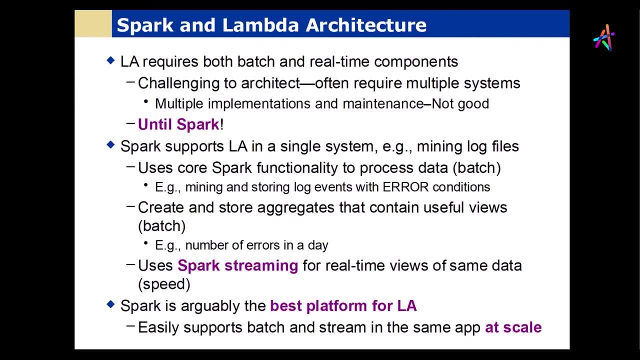 holding areas And what Spark does is because Spark basically has this kind of unique data representation model, It is able to actually process the data by integrating both the streaming view and the The batch view And, if we get a chance, I'd like to maybe see if we can come back and touch on a 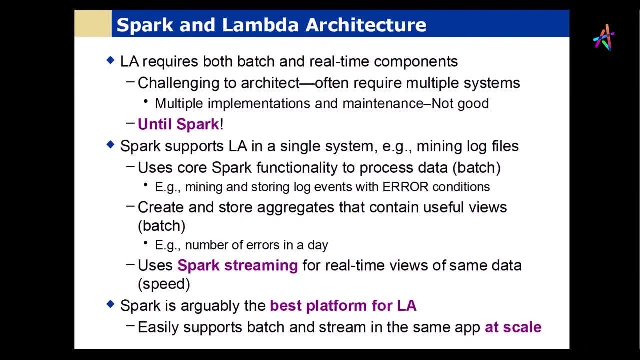 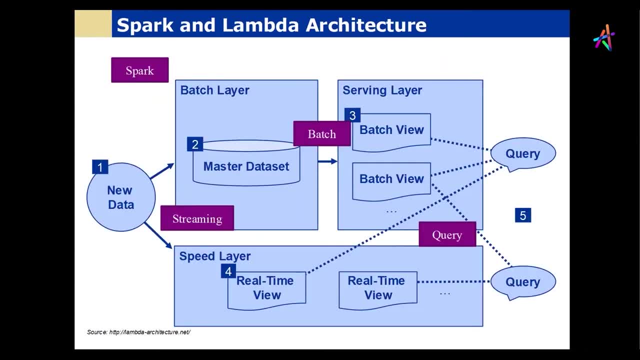 little bit more about the Lambda architecture and next week Because I think there's some interesting ideas here about how data actually can work in terms of designing data applications. And so here's where Spark actually is able to fit in all of the different bits and pieces where it's creating views. of the data that can work, And so that's kind of the challenge that we've got here. So that's kind of the challenge that we've got here, And so that's kind of the challenge that we've got here, And so that's. 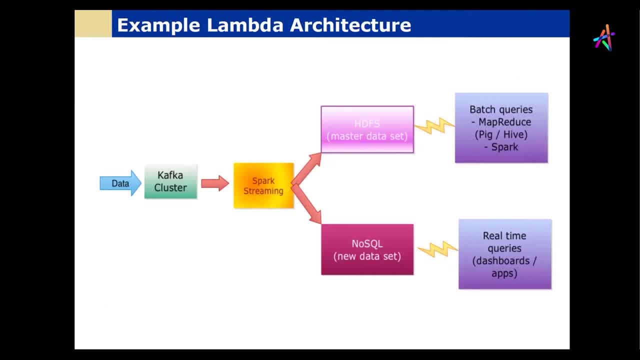 kind of the challenge that we've got here. And so that's kind of the challenge that we've got here, So we'll come back and revisit this at a particular point. So here's again where we wind up looking at a real-time architecture. So we've got Kafka, which is pulling a lot of real-time events in. 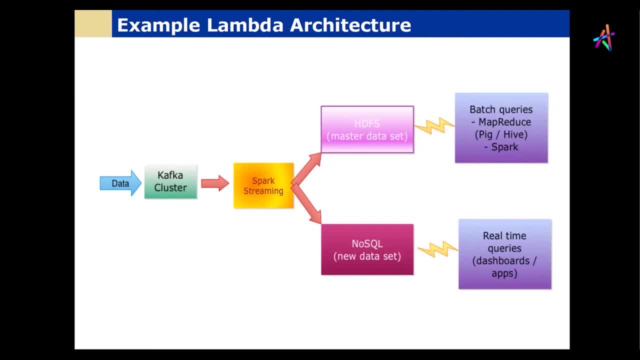 It's going through the Spark streaming module, which is able to then work with the data in a couple of different representations in both the persistent world and the real-time world, Or I should say the batch world- Again, typical HDFS type of application- And also create this. 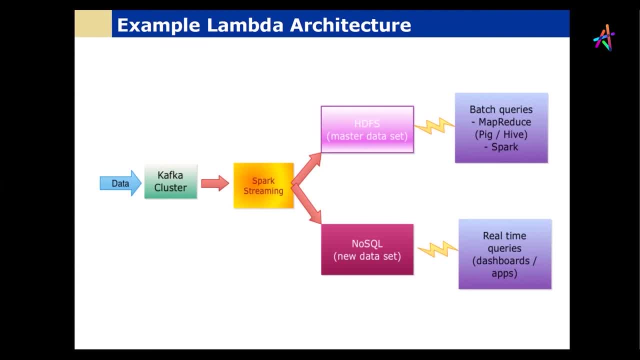 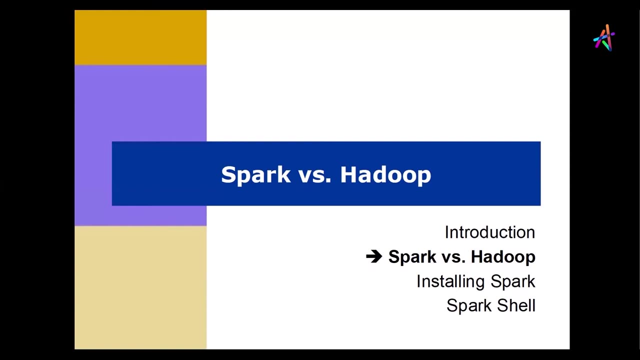 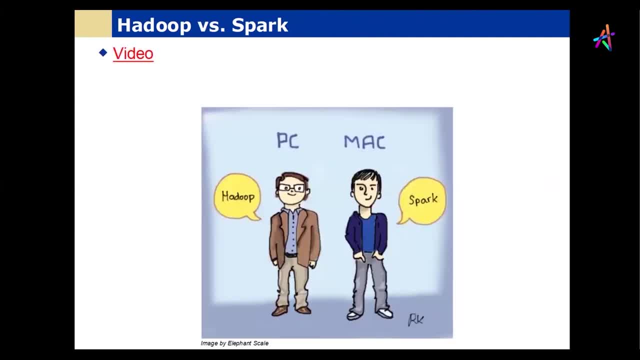 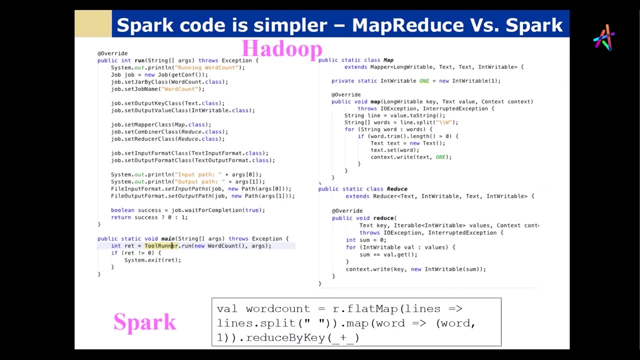 Spark timeline again. I couldn't figure out what this thing was until somebody pointed me back to those old commercials where they had those two actors going: hi, I'm a PCI, Hi, I'm a Mac, And I'm not particularly thrilled with this representation. But this is the part that's. 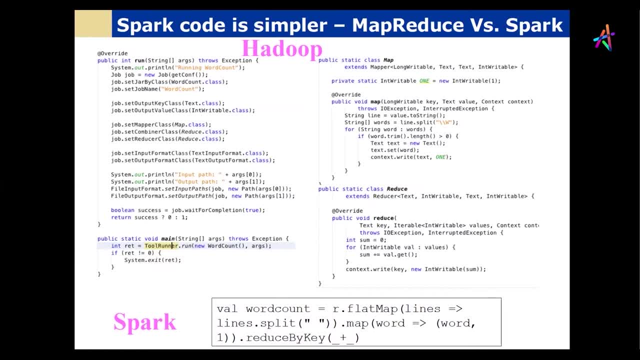 really interesting here- And I think it's important- is that if we look at the amount of coding required to actually do various kinds of processing in a Hadoop system- And again I have to go back to say this was Hadoop- We can't underestimate the innovation. 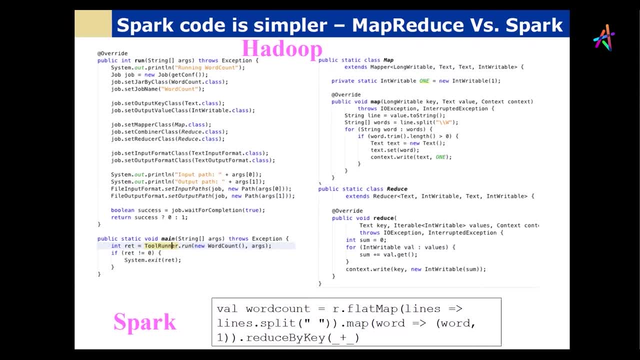 of the innovation that Hadoop made, So it was the first one really that made this available. So it obviously had some areas that needed a little bit of work, And this is one of those example of areas. So we've got this. I believe, yeah, this is a Java implementation of Hadoop performance. 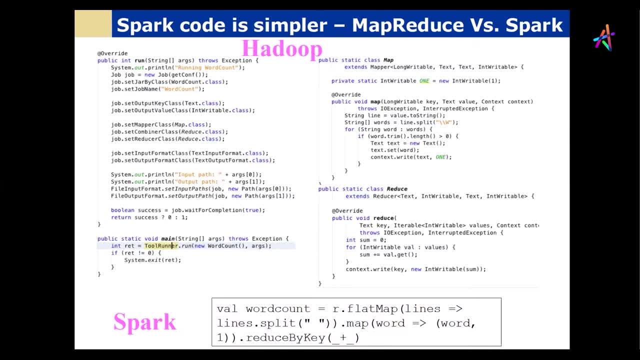 And down there in Spark we've got the same equivalent code being represented as a couple of lines of code. Actually, if you put it out, it's actually one long line of code. So we're not saying here that Spark is a better programming model than. 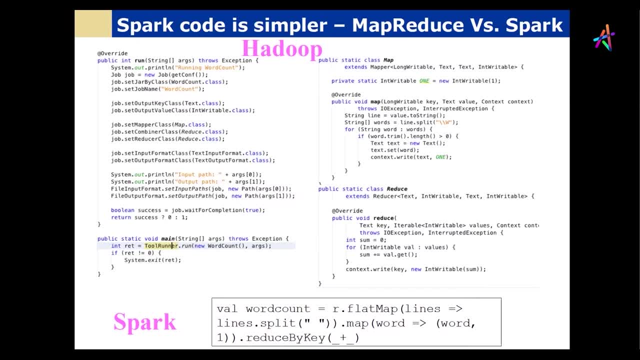 Hadoop. What we're saying is that, because of the tools available in Spark and because of the way Spark is structuring the data, we can take advantage of more elegant programming models. And I don't know about you, but I kind of like the Spark implementation here a little bit better. 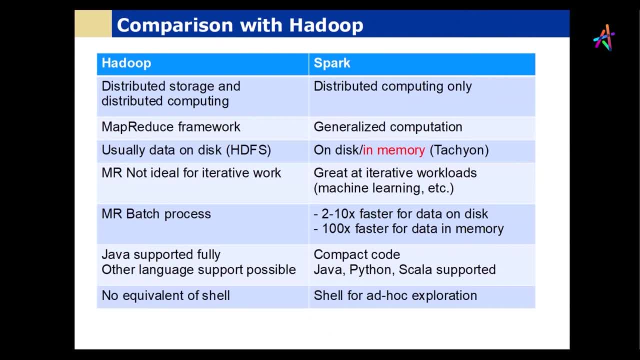 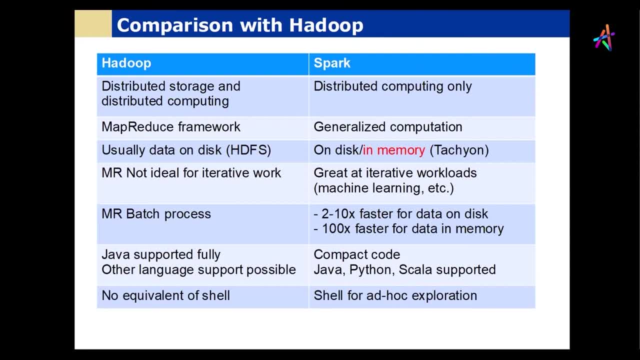 made it this way, And I think we made it this way, And I think we made it this way And I think that they do two different jobs. even though Hadoop does some of the stuff Spark does, It was never intended to be a Spark kind of engine. It was really focused on how do I actually distribute? 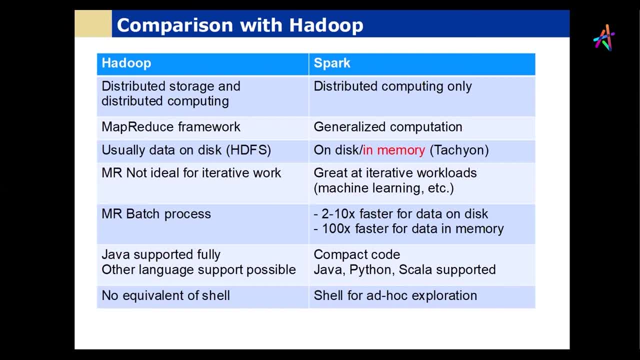 and work with data in a large-scale environment. So it's really focused on distributed storage and then adding computing on top of that, whereas Spark doesn't care about the computing, So it doesn't have storage. It doesn't have to worry about that whole layer, It delegates that off. 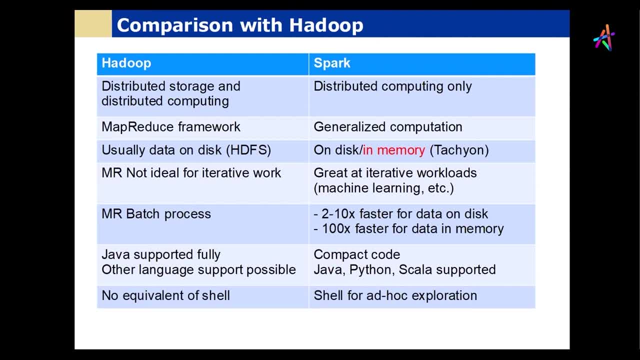 to Hadoop, So it's riding on top of Hadoop And I think that's really important And I think other storage engines. It uses a MapReduce framework. That's the model that came up with it, So you're locked into that model. And again, that's not intended as a criticism, That's just. 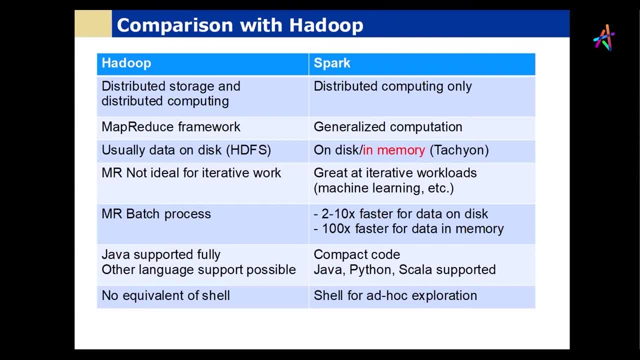 the reality of the situation. Spark is looking at more of a generalized computation, So it's not locked into that model. Hadoop, again, is focused on the disk, So it's HDFS- again a very significant innovation, But Spark because they're not having to worry about building that. 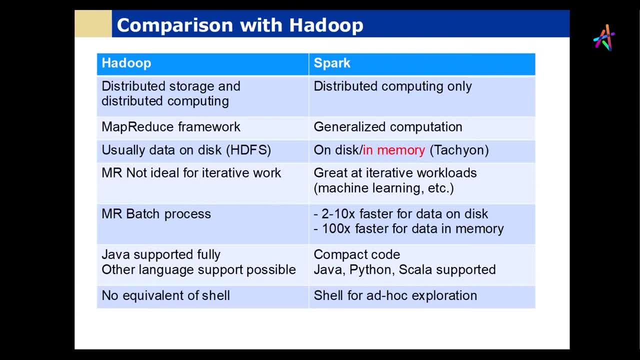 model can actually use a different kind of model that focuses on in-memory and its relationship to on-disk, And we'll mention Tachyon is one of the projects that is associated with that. Later on we get into optimization. Hadoop doesn't work for iterative work because it's primarily a 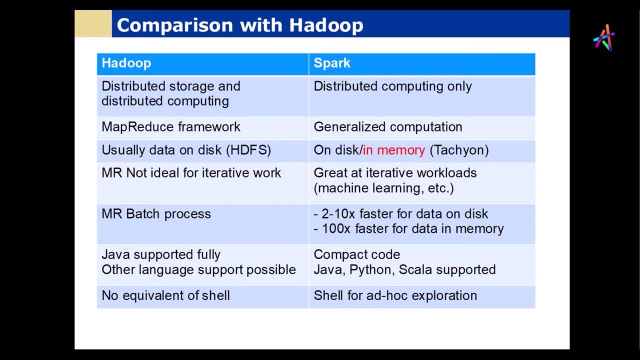 batch processing, which was how it was originally intended to work. So it works great for that particular objective. But Spark is designed for the general purpose. So it looks at the iterative workloads and, again, because of its memory model and how it's structuring data, 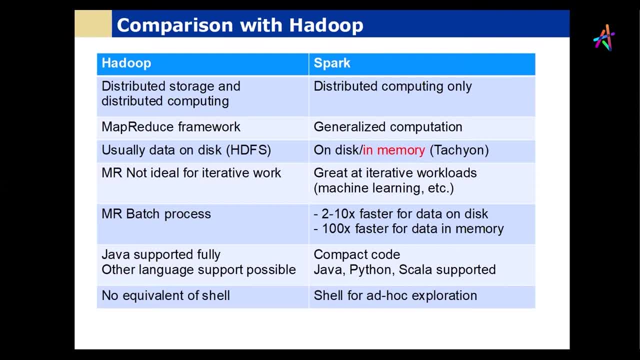 it just works faster. The Java is the core programming on Hadoop And Java is a great programming language for what it does. But again, as you can see, it can be very verbose. But what Hadoop does is because it employs a lot of the functional programming concepts and model. 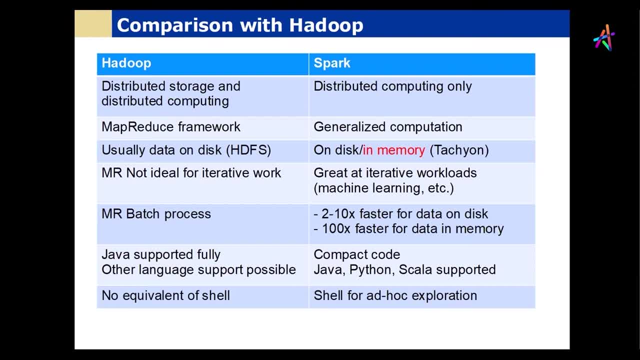 it winds up being a lot more elegant to program in, And Hadoop doesn't really have a shell, So we have to have things that build on top of Hadoop. Whereas I keep wanting to say Scala instead of Spark, I have to keep watching myself Where Spark has various kinds of shells. 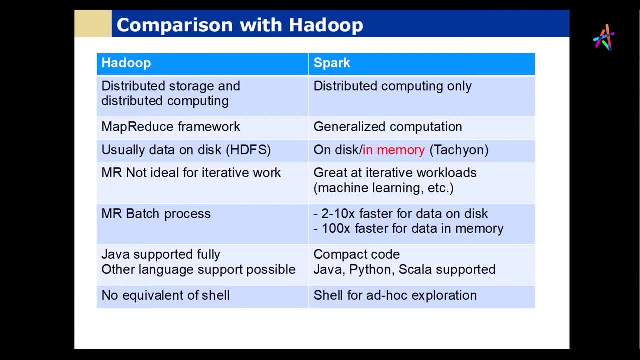 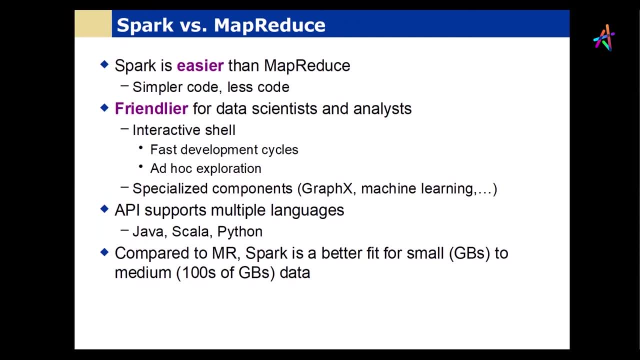 And we're going to work in the Spark shell as we go along, And I think there's just the arguments we've been made. I don't think we need to beat that to death. Compared to MapReduce, though, Spark is a better fit for small gigabytes to medium gigabytes of data. 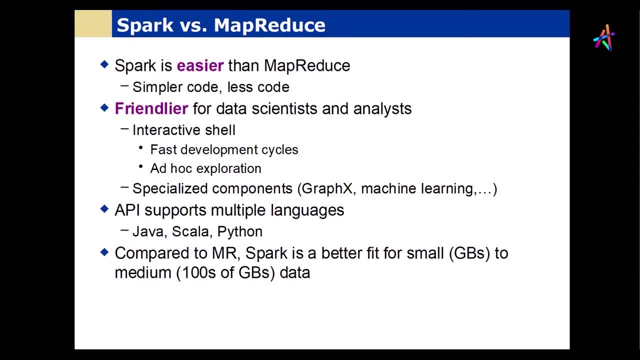 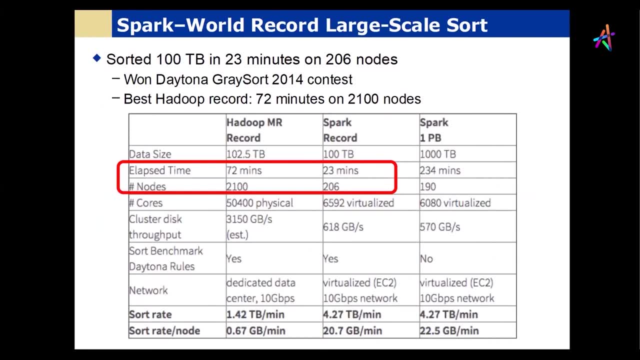 Simply because it manages the data in a more effective manner than MapReduce. Here's a couple of benchmarks. So Spark wins when the what is it world record large scale sort So versus Hadoop and Spark. And we've got elapsed time: 72 minutes versus 23 minutes. 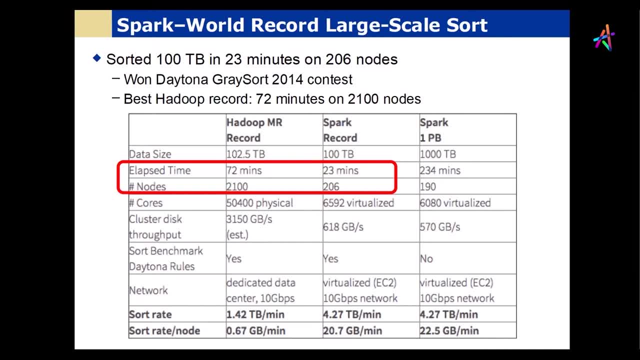 And we've got a sort rate here of 0.67 gigabytes per minute And here's 20 gigabytes. overall It's terabytes per minute. So you can see, we get performance enhancements. So it's not just theoretical. We actually see this model And where that 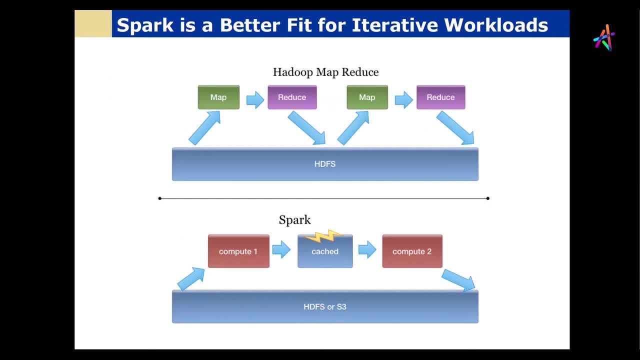 performance is coming in, is this gap here where we're actually, instead of doing a chunk writing to disk, doing a chunk writing to disk, we're doing a computation And then we're caching the computation in memory, if possible, sometimes spilling it to disk and then doing a computation. 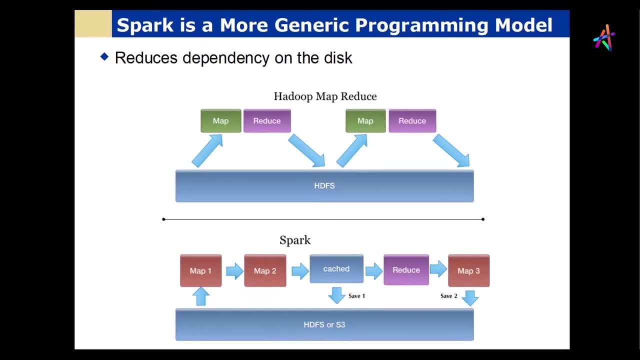 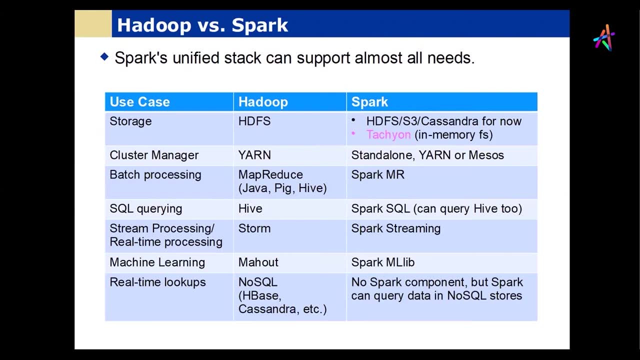 again, So that we're not just doing a chunk writing to disk but we're doing a computation, And then we're we wind up being able to streamline the approach with options to be able to save to disk at various points, And we also have the stack support, So we can work with a variety of these particular. 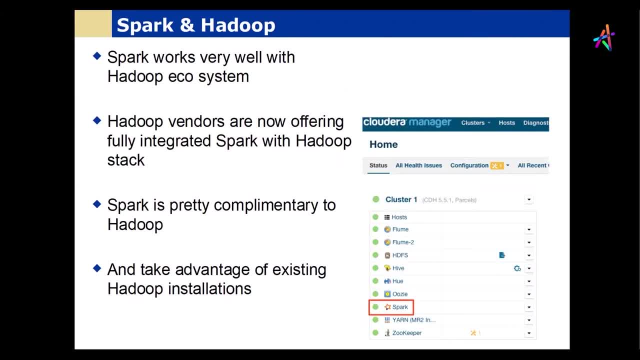 technologies And again, we're not going to get too much into it at this point. These slides are basically kind of driving the same point home over and over again. This is the big thing that you want to take away from this is: Spark is complementary to Hadoop. 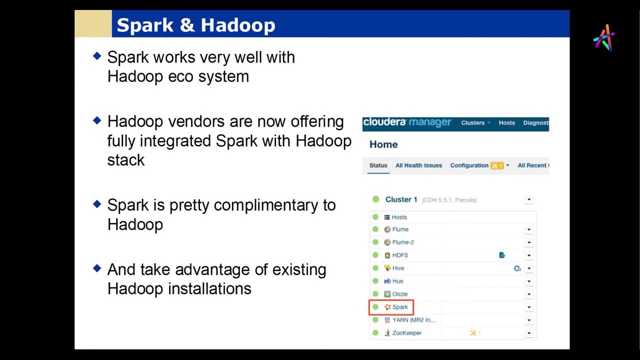 It doesn't replace Hadoop. It does replace some of the things that Hadoop tried to do that were kind of add-ons- not add-ons, but kind of ancillary to the storage model, which, in terms of that, is particularly the programming stack that is on top of it. 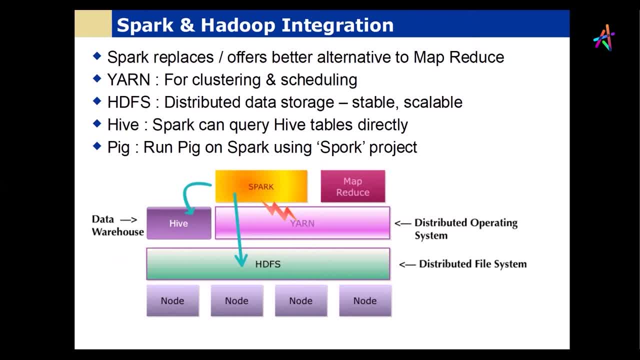 So Spark sits on top of the HDFS, manages it and can operate through a number of the distributed operating system cluster managers that are out there. So the idea is Spark only does what it has to do. There's a number of different ways we can actually run in different. 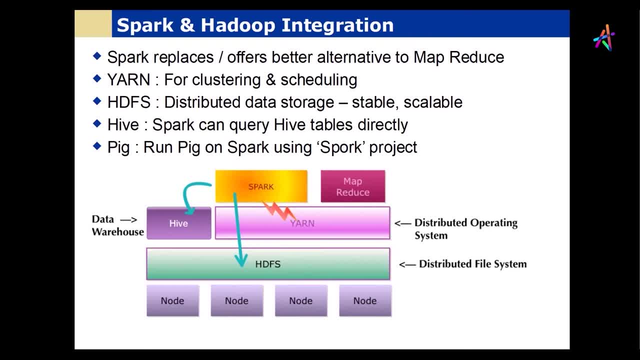 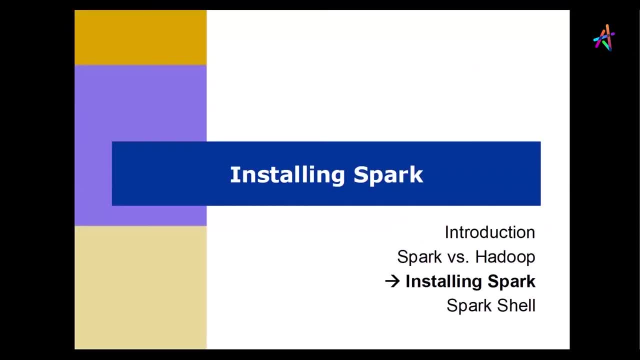 environments. Spark can query Hive tables directly. for example, It can run Pig using the Spark project. It can work on Yarn, So it does a number of things. So that's basically kind of an idea of the kind of overall idea of Spark. We're going to come back and install Spark. 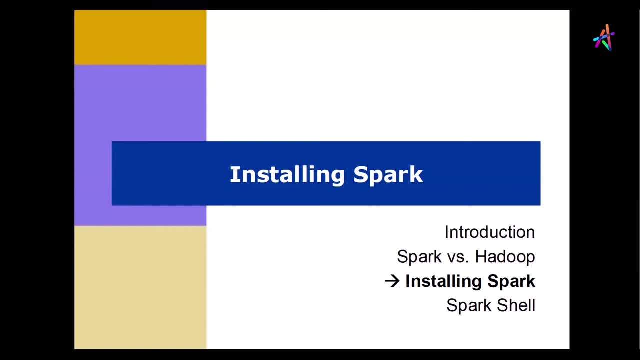 a little bit later, But we're going to come back and install Spark a little bit later today. Let me see, I'm going to check on my times and things, So at this point I'll ask any questions, Everybody doing okay on this. Do people still use Hadoop, and why? 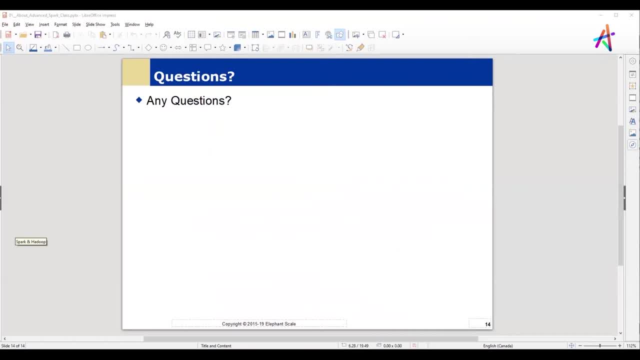 Yeah, people still use Hadoop because it got a wide distribution there And I'm not sure how much of the market share Hadoop has got. But basically the Hadoop model is extensively used And again, sometimes I find it I'm in so 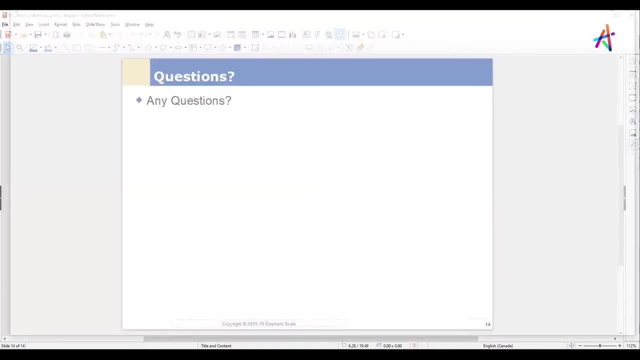 many areas. I find it difficult to keep up with what the current market leaders are in some of these things. But generally, yeah, when I'm talking to a lot of clients I do see a lot of Hadoop installations, because it kind of went with it And now they're just kind of sticking. 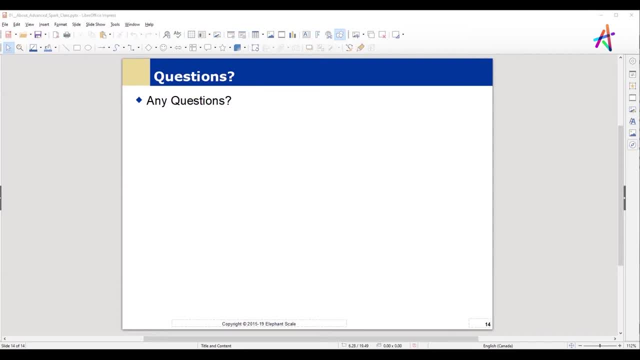 with it at this point And there's talk about doing other things. But yeah, I am seeing a lot of Hadoop out there. What's your take on that? Well, Spark is like 10s or 100s times faster, better, cheaper, whatever. So Hadoop should die. 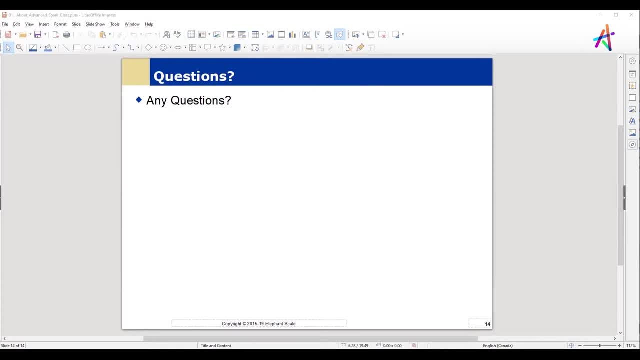 Well, basically- I think again, this is the point- is where Hadoop is primarily being used as a way to store data in a distributed environment, And so Hadoop is. I think what we're actually seeing in the marketplace is where Hadoop used to be sort of the complete solution when it was the 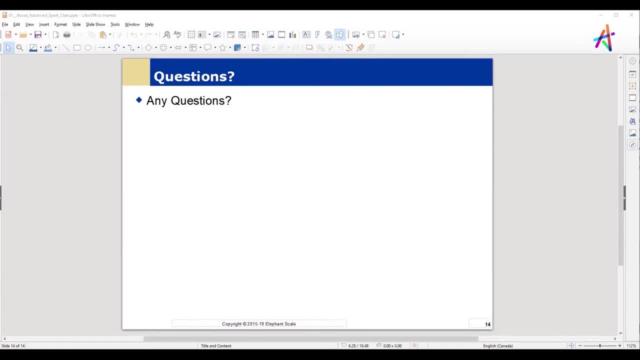 only one in the marketplace. It is now more of a- you know it's more of a. you know it's more of a- storage solution, While there are competitive other competitors out there for other large-scale data storage solutions. But I think what we're really seeing, the transition is people instead. 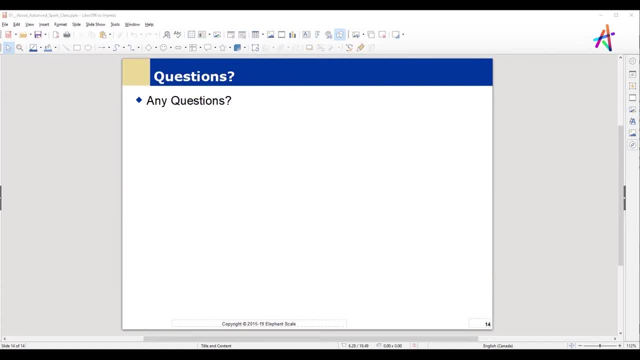 of doing the actual analytics using Hadoop and the tools in that are tightly coupled to Hadoop. they're starting to use Spark on top of Hadoop to get, as you said, the speed of processing. So I would say that Hadoop is out there. a lot People are committed to it for a couple of reasons. Number: 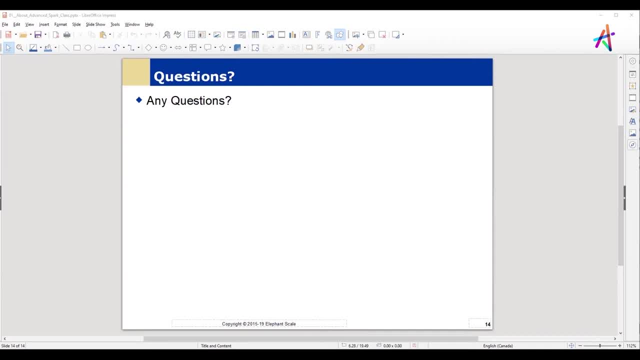 one. it's their storage solution, But in those cases they're often bringing Spark in as a processing engine on top of Hadoop in order to replace the Hadoop MapReduce component and get better processing. in that sense- And I do know that other people there are other large storage- 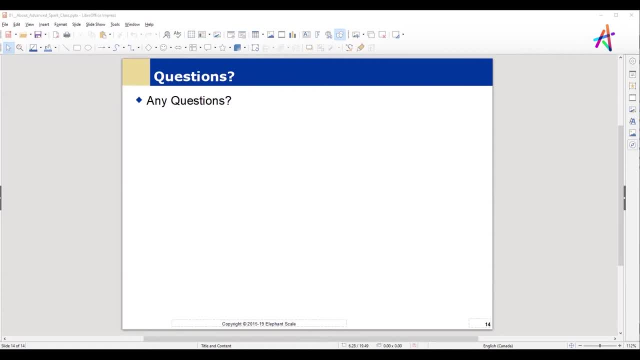 solutions that are sort of out there that people are switching to. But yeah, I would say that Hadoop is probably going to be around for a while as a storage solution as opposed to a processing solution. Does that help answer your question? Yeah, And remember, Spark isn't really focused. 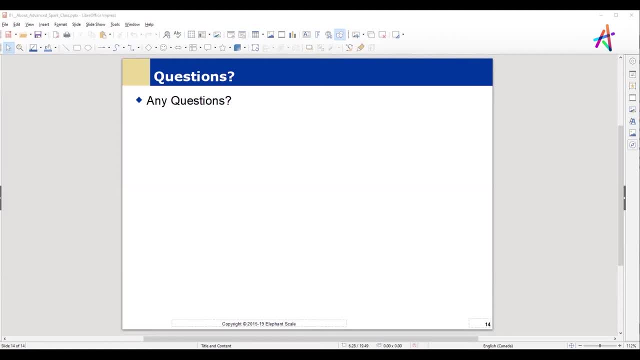 on trying to build a storage solution. It's focused on building a processing solution, All right, Okay, So we're going to talk a little bit about Scala and functional programming, And I think I have, I'm going to. I'm going to actually use a little bit different material here. 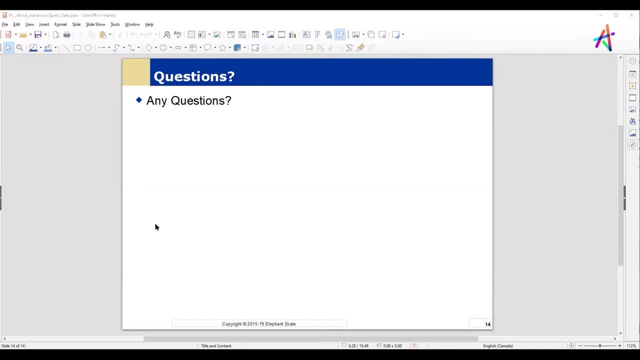 Web Services, Azure And I'll. this is. I'll give you the URL for this. I'll put it in here if anybody wants to just grab a copy of it. This should be. this is the Scala by example. Martin Odersky is the guy who's going to be. 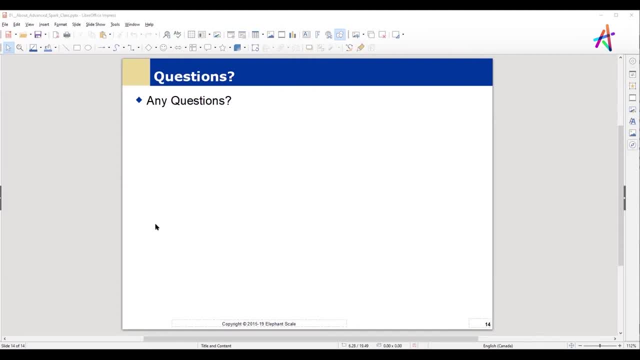 talking about Scala, I think somebody, a couple of people here are taking a look at this course on Coursera. Excellent course. He always looks a bit mad to me, but angry, but I really love his approach. He always looks like he's a bit annoyed with whoever's making filming him. But but the big 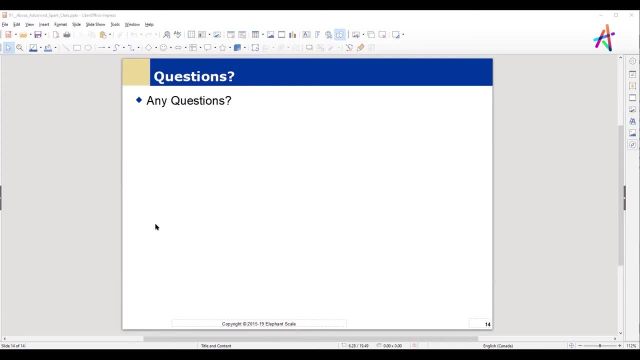 important thing we want to. Screen sharing is paused. That's not good. There we go. The Zoom share, Can you guys? Oh, I think I- I'm sorry, This is my Problem here- Let me. I want to share my whole screen here. There we go. 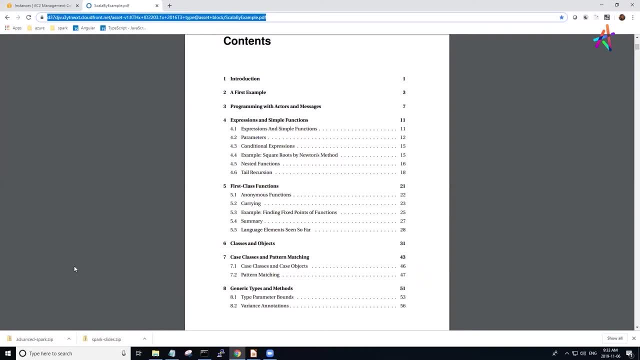 I think that'll probably be a bit better. Okay, Can you see my screen? Yep, Yep, Okay, good, I am fumbling around a little bit with the, with the tools here. Okay, So the big important thing about, about Scala, if and then now we've got people with a variety of programming. 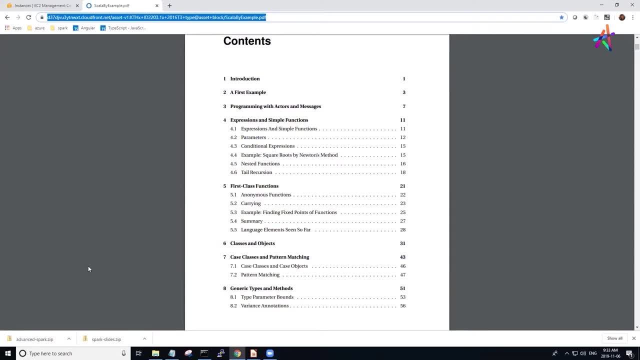 languages. We've got people coming from Java, people coming from C++, Ruby, Golang. there's a lovely range of programming languages there. Scala is intended to implement a functional programming paradigm which involves a a change, a substantial change, in the way that. 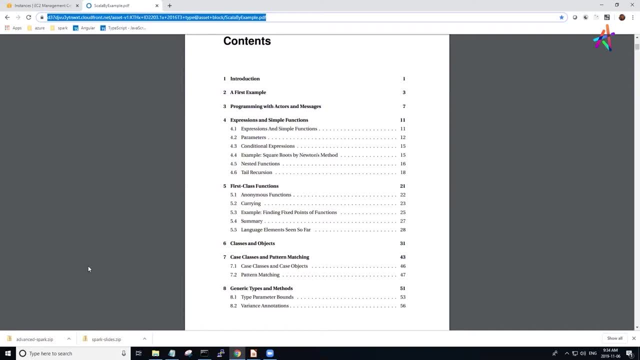 we think about, about doing code, And this comes from the idea that in mathematics, we have these functions and we are able to describe an entire programming paradigm. And so you know, we're able to describe an entire programming paradigm, And so we're able to describe an entire programming. 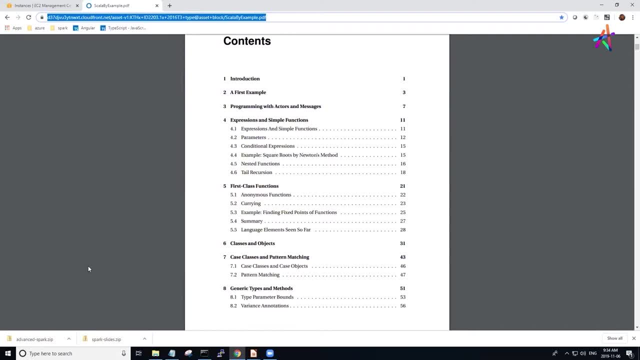 paradigm, And so we're able to describe an entire programming paradigm, And so we're able to describe a computational environment, and computational environment uses something called a Lambda calculus, which is a a way of being able to implement programming languages, provided that the functions have no side effects. In other words, they they are, are basically: 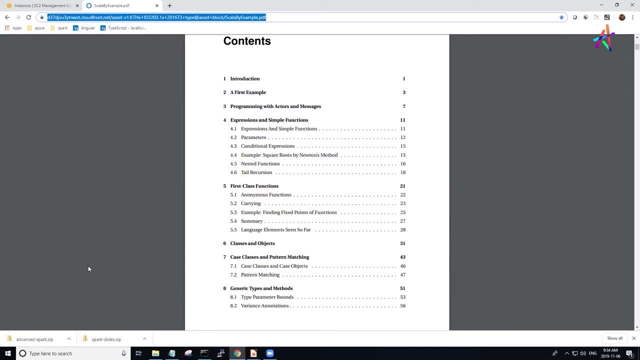 stateless. The fundamental idea in a Scala environment and a functional programming environment is that you want to keep things as immutable as possible And in a certain system, certain sense, you don't change data so much as you create a new copy of the data that has. 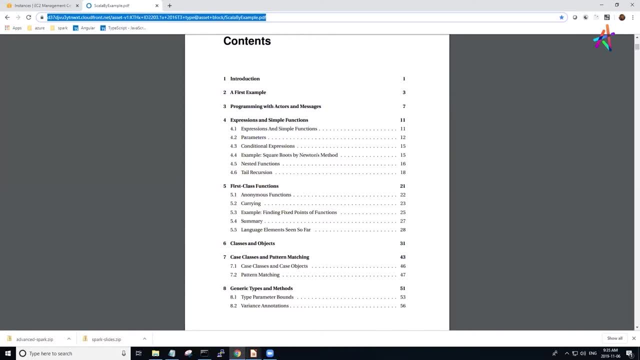 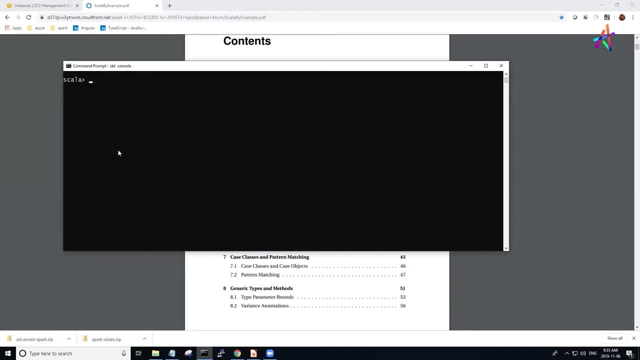 changes from the original version. So I put up a little Scala here in my environment, simply because I think it's easier to see on the screen. So one of the things that functional programming does and Scala does is it really blurs the distinction, and I'm going to mention this up. 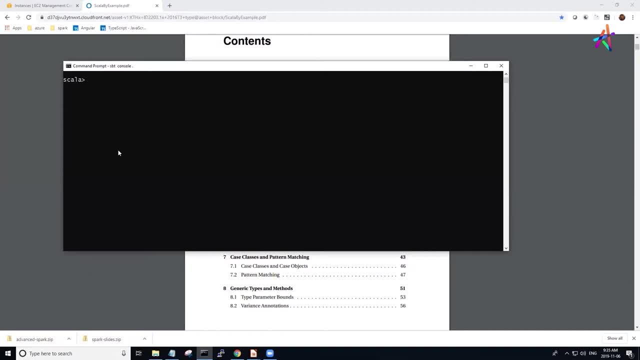 first, because I think this is an important point- between function and data. It basically thinks of them all as objects, and this is what we often call first-class object, And it really becomes clear when we look at the difference between a simple function that we might have. So we have. 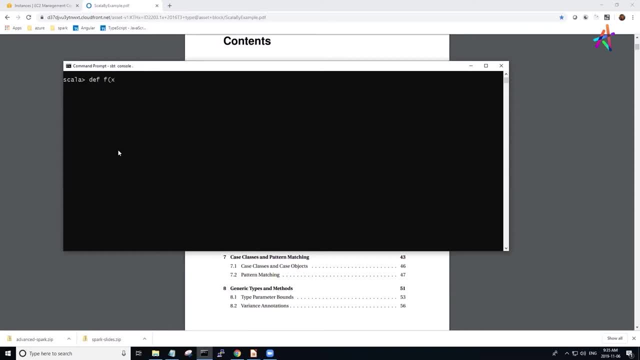 def, we'll say: and that's going to be equal to hold on here x plus one. okay, and we'll do that. and now we've got a function and of course we can apply the function to two and we get three and we can actually do this. 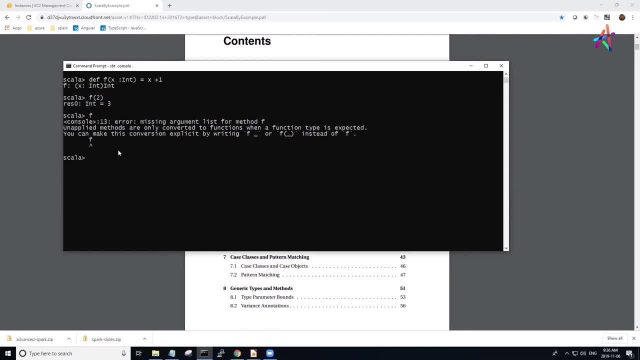 as aне and we get an error. So it looks fairly standard, but there's a lot of things that are going on under the hood And we can see this when we actually use that same keyword to define what appears to be a variable. okay, And this is, and if I do x, we get three again. But 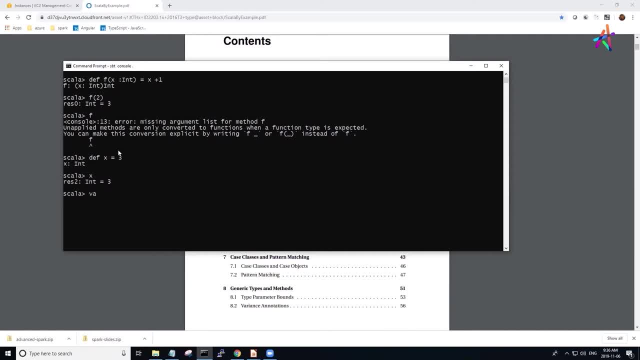 I also can describe a variable by using this notation as well, So it seems like I have the ability to do things in my shell, to do something like that. So this is just a simple example to illustrate that things are not exactly what they appear. if you're thinking, 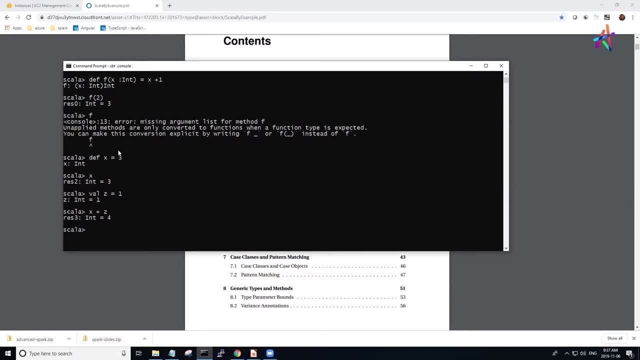 about this from a more traditional perspective. So let's figure out what actually is going on here, And this is, I think, Martin, in his course, actually does. a lovely, elegant explanation of this is that these are basically called rewriting rules And we have to, instead of thinking in terms of computation, we think. 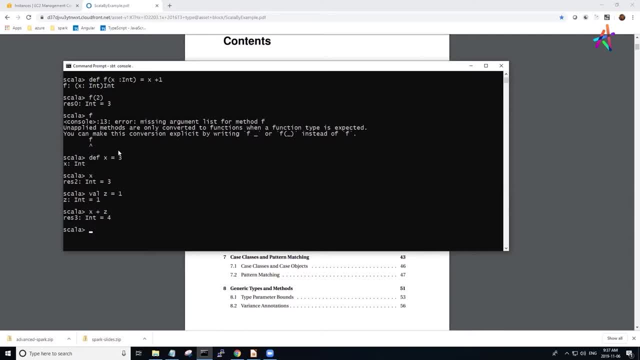 in terms of evaluating things as you go along in kinds of rewriting rules. So in functional programming we think of things as things as you go along in kinds of rewriting rules. So we tend to blur the distinction between functions and data. They're all just things. 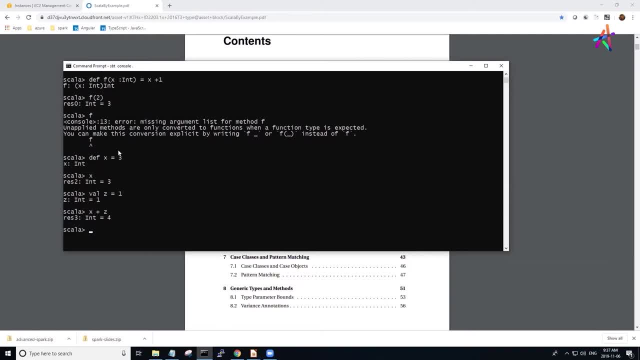 that we can manipulate in some way. In particular, functions are basically things that can be assigned to variables, And we'll notice up here that you start to see this in the notation here, And what we're really doing is saying there's an equal sign here, just like we've 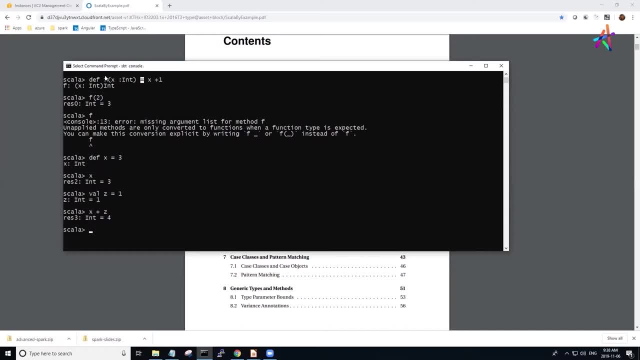 got down here And this is really saying: I'm defining this function f or this symbol f, and I'm going to rewrite it. And whenever you see f, this function, so for example, when you see f, where do we have it here? f2,. I want you to rewrite this statement as: 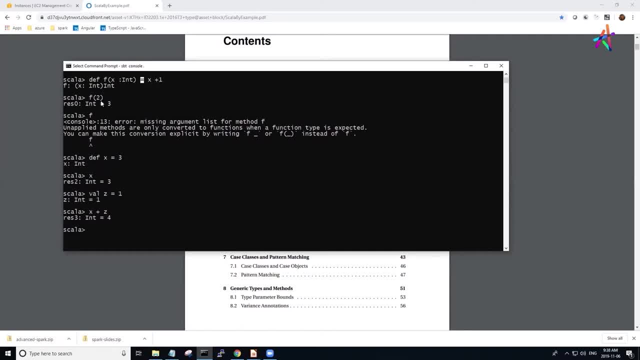 x plus 1 and then evaluate it, And that's what we're getting here. So there's a rewrite rule. So instead of thinking of this as creating some kind of object code somewhere off in memory and then we're doing a call. 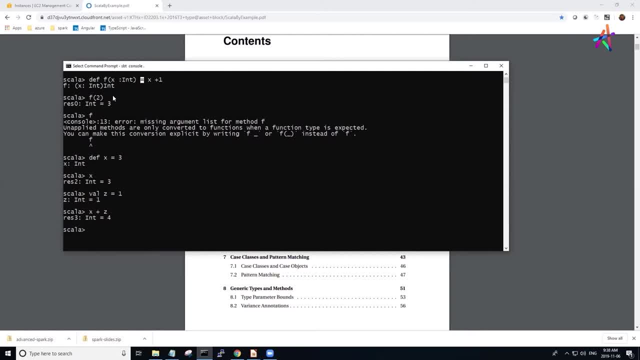 To that object code and pulling it and then executing it. what we're really doing here is, we think in terms of this, it's almost like a macro expansion, to think of it. Now, obviously, there's a lot more going on under the hood, But the idea here is that this equal 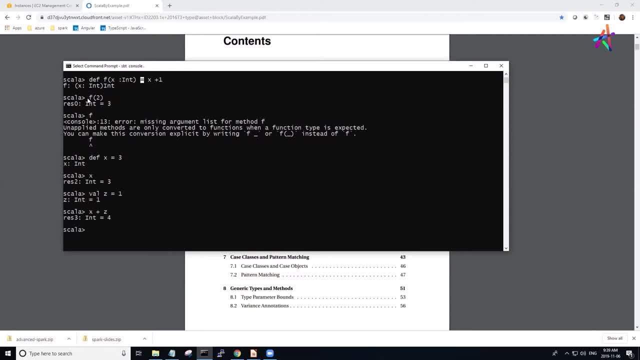 sign kind of gives you a clue that what we're doing here is: we're working with this rewrite rule. And similarly, here we're saying: whenever you see x, for example- and I use the use it here- rewrite it as 3.. And in this particular case, I get 3.. So this def is basically. 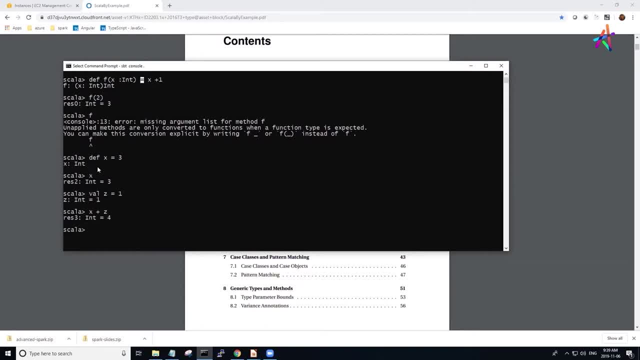 defining the stuff on the left-hand side of the equal sign as the stuff on the right-hand side. And it's saying: whenever you see the stuff on the left-hand side, rewrite it as the stuff on the right-hand side. Now the vowel is a little bit different because it's: 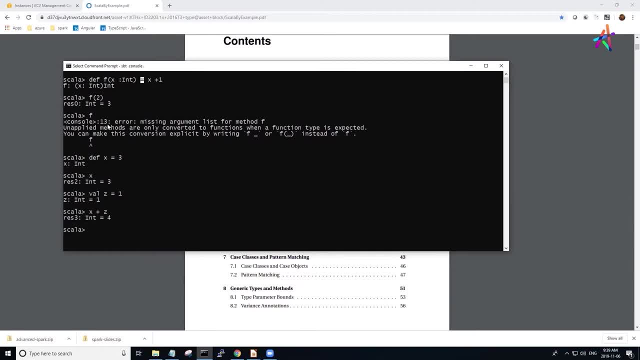 not getting a rewrite rule- And this, by the way, is something we often term call by name- in which we're doing this rewriting And then, when we get to a point, once we do the rewriting, then we do the evaluation In this form. here we're saying: 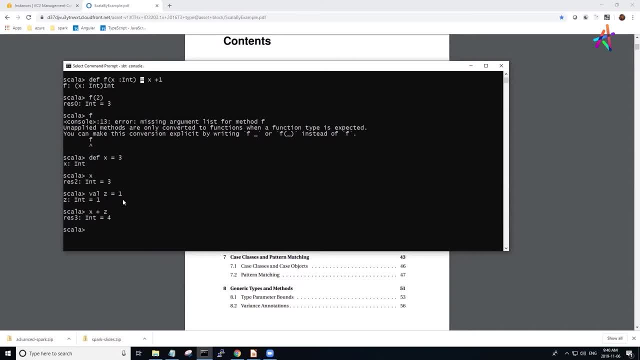 evaluate what's on the right and then take the results of that evaluation and assign it to the variable x. So there's two different processes going on here, although initially they kind of look like the same thing, And we're going to see this as we go through in. 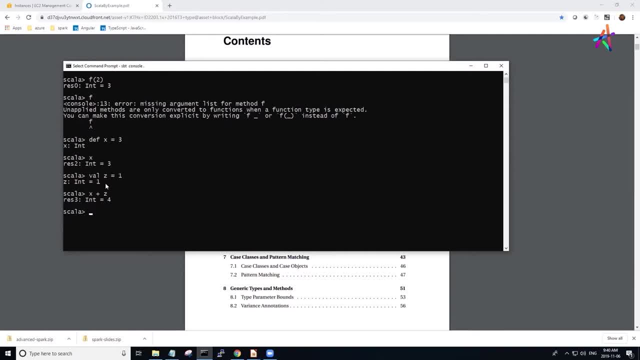 the code. So, for example, let's take a look at: let's: okay, let's define x to be 3. And so if we do f of x, we get the result 4.. And if we now say, I think I can do it this way, F equals to five. Okay, Whoops, That's a. 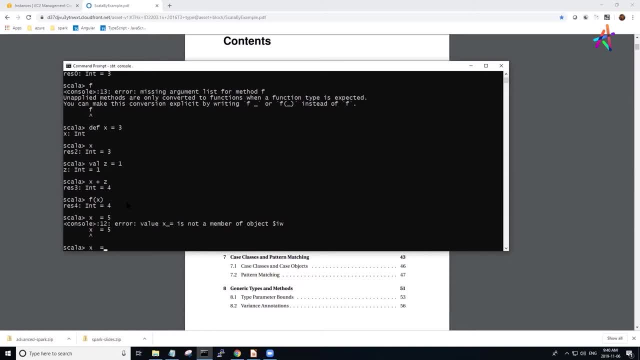 sorry, there The way I've defined it. So let's do a var X equal to one, Let's do F of X, Okay, And X is equal to two. And the point here is that if I, if I were to go and change that, that value of X, 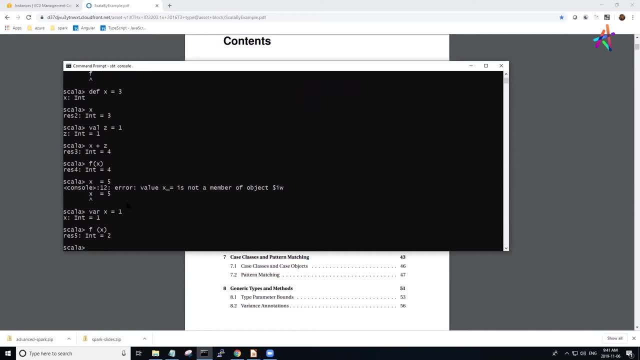 it's going to affect the rewriting. We'll get more into that a little bit later. I'm sorry I'm just going to skip over that example, but I what I wanted to do it illustrate here initially is that when we have a 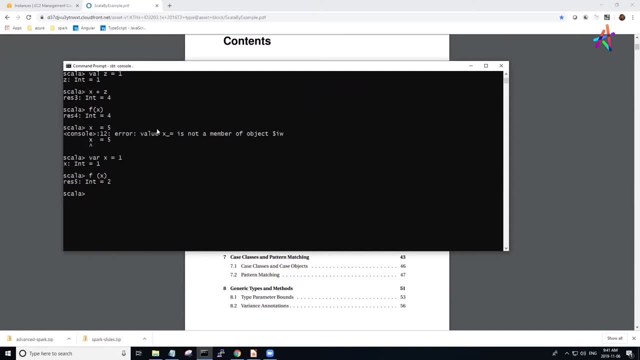 a value. it's what? when we think in terms of traditional programming, distinction between functions and data, it's not quite the same. So we're going to come towards the Scala primer. Let's do one more little thing here, a def, and we'll do function G. 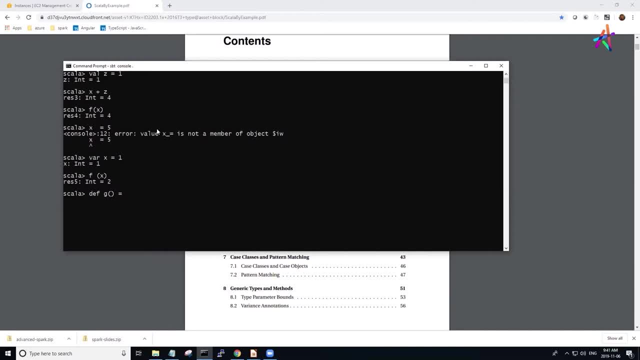 which takes no parameters, And we'll set this equal to X. We'll set this equal to. we'll just do a computation here: Seven plus one. Let's see if that'll actually work. Now, if I do G notice, it doesn't even look like a function call. 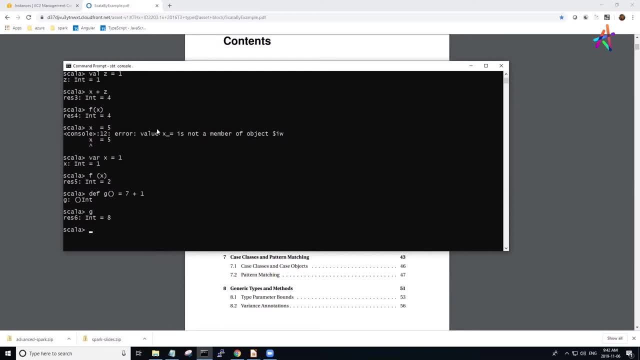 It looks like a variable call, because now I've rewritten G as seven plus one And because of the of the def and I wind up with eight. Okay, Why couldn't I have done that with F up here when I did? when I just put F, I got an error. 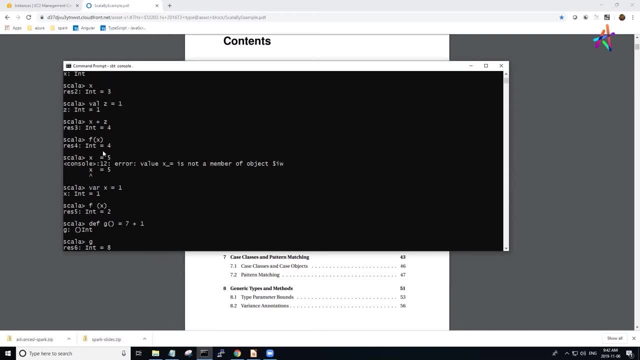 And the reason why is because F basically has a rewriting rule. If I look at the definition of, of, of F, here we go. It has a rewriting rule that says substitute. whenever you see F substitute, do this rewriting rule, but rewrite X as whatever value was passed into X. 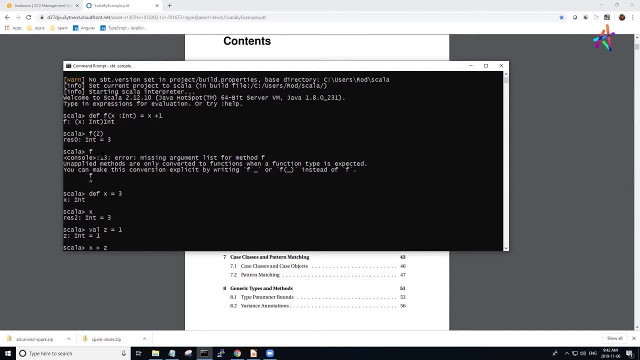 So we're getting a fake. So this works as a rewriting rule, but this one doesn't, because I left something out. So when there's an unapplied, methods are only converted to functions when a function type is expected. So in other words, we're saying: 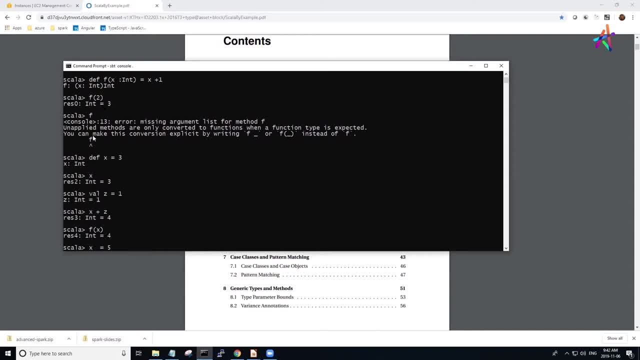 Oh, there's something fundamentally wrong here. I can't. I can't implement my, my rewriting rule. On the other hand, when we look at G, what G is saying is: just rewrite. Whenever you see G, rewrite it as seven plus one and evaluate it. 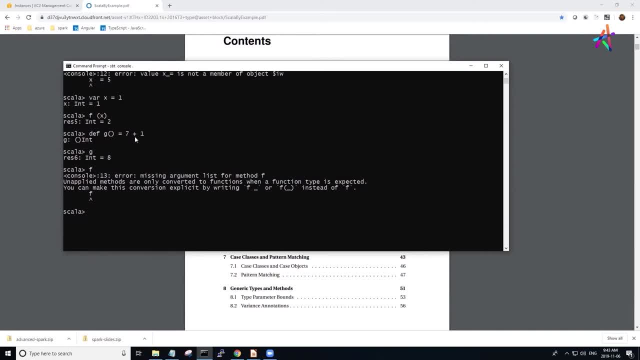 There is no need to rewrite any of the any of the placeholders or parameters in here, So I can freely call G without or an argument list and the rewriting rule works. Now, I'm making this point because the problem that people have when they're learning Scala is that that 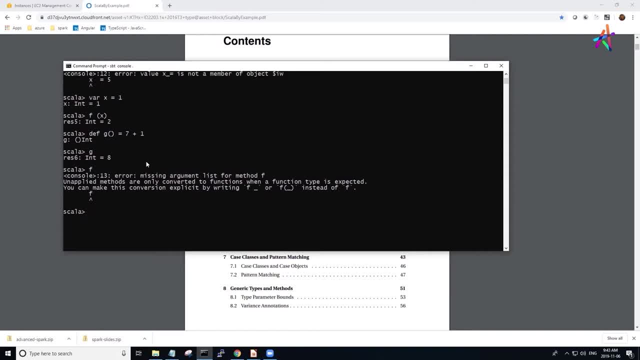 last line G without the argument list looks really confusing because it doesn't the compiler expect to see the parentheses to know that this is a function. And again, that is a result of programming languages where we make a distinction between functions and between variables. All a function actually is is a. 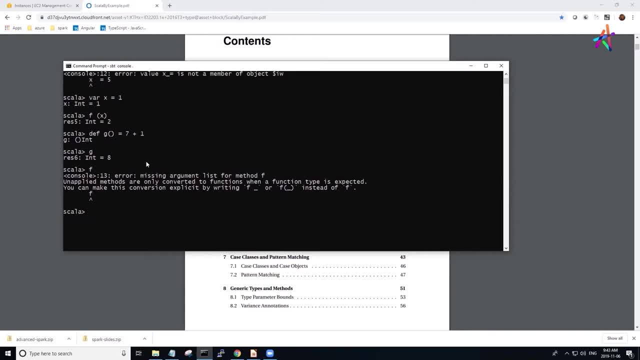 is a string that can be evaluated, where we rewrite some of the values before we evaluate it. And once we get that idea- and we'll see that idea occurring in how Spark actually manages some of the data- Okay, Is that? is that idea fairly clear to everybody? 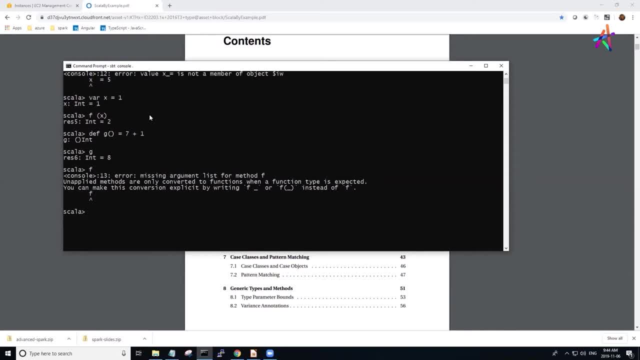 Is that we have to think about this in a completely different sort of way from what we might be used to Makes sense. Yes, Yeah, Good, Okay, It's a simple idea, but it has great. it has a lot, of, a lot of of implication for it. 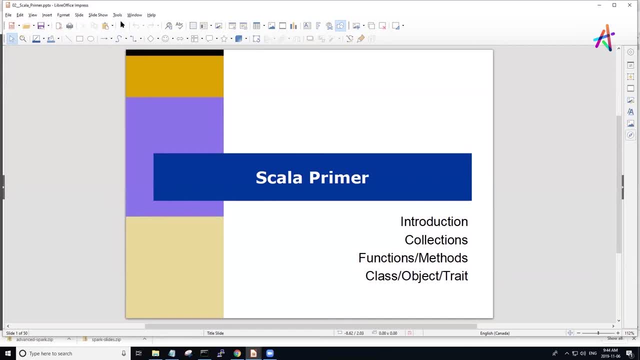 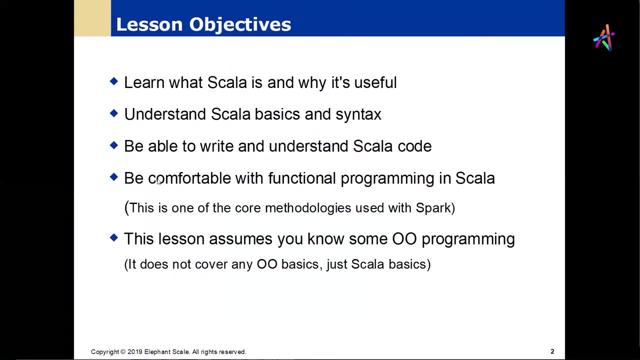 So let's take a look at our Scala primer here, and I will come back and look at some of these ideas as we go along. Okay, So first of all, a couple of things about Scala is that Scala is built to compile down to the 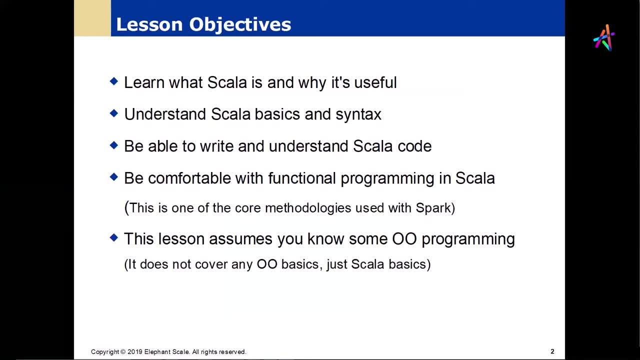 Java virtual machine or a JVM. What that means is that is that we can run our code in a JVM. Now that is important because the heart of all the processing that's being done in Spark is being done through JVMs, And when we get into looking at the memory models and sort of things, 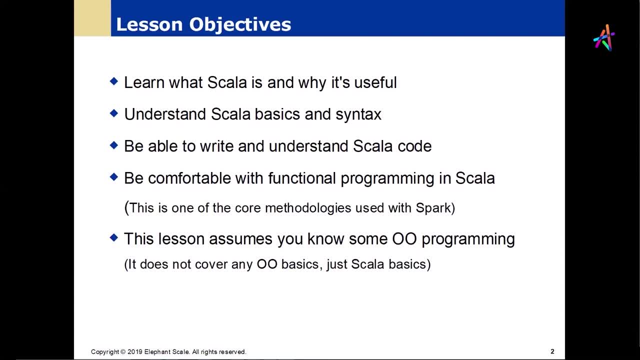 we'll see that that tungsten works with the JVM memory directly in order to uh improve efficiency and performance. So what we can do is is basically um, embed Java within Scala. uh, because it compiles down to the same thing. 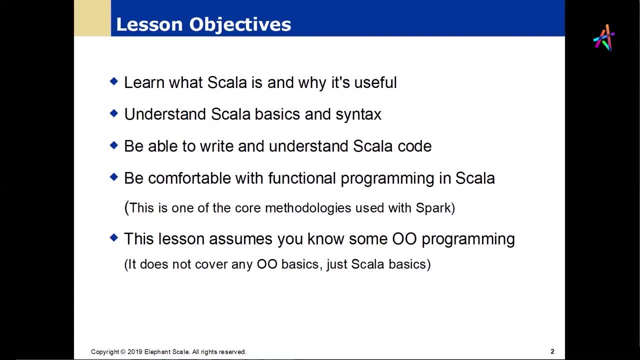 So Scala itself is not just a functional programming language, but because it basically has object oriented definitions, it also has an object oriented component, And I believe Martin was kind of looked a bit grumpy when he said: well, you know, we have to do some processing because Java is. 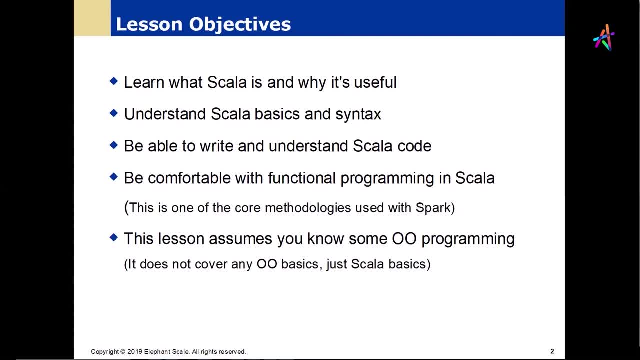 uh, a procedural language, So Scala does it as well. Uh, that's where Scala breaks from being a purely functional programming language and incorporate some of these ideas. So there's two different programming paradigms that are going on inside Scala, but the functional concepts are the important ones in understanding what's. 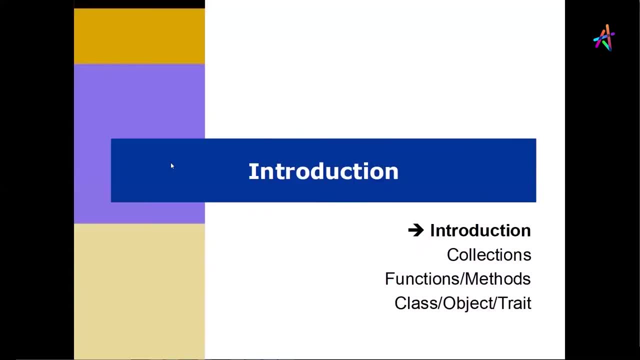 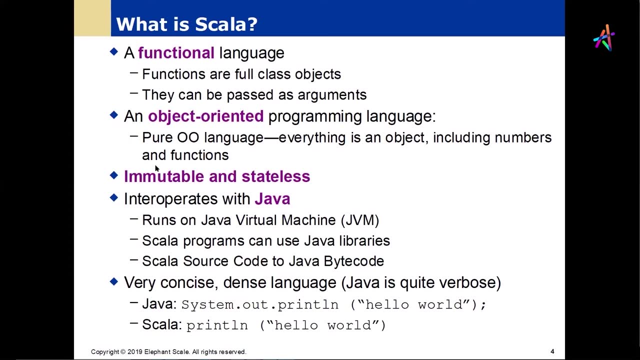 going on in Spark. So let's take a look at a couple of these ideas here and then we'll we'll uh get a chance to to look at the uh, uh functional languages. So Scala programs use Java libraries. 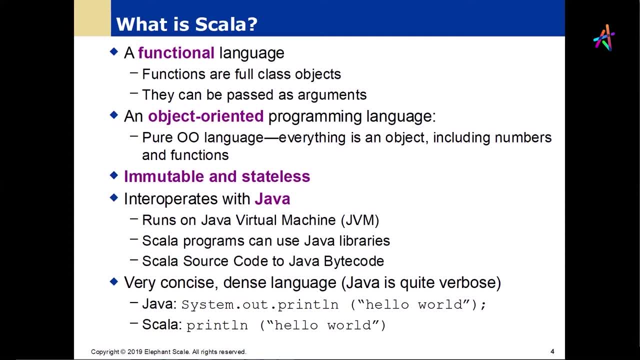 Uh, it's, it can be object oriented, um, uh, which is useful because if you're porting code in from Java, you don't have to completely rewrite the code. You can do staged kinds of of whoops, sorry. 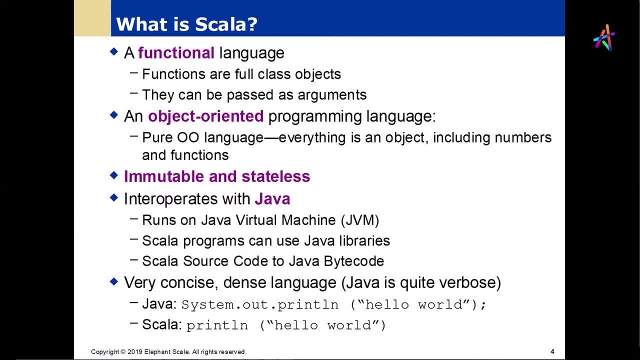 my microphone slipped. here. You can do staged kinds of of trend transitions. Um, hold on here. There we go. Sorry, I have these cables running everywhere and I move my chair and it gets wrapped up in the wheels. Uh, so we'll get into more about. 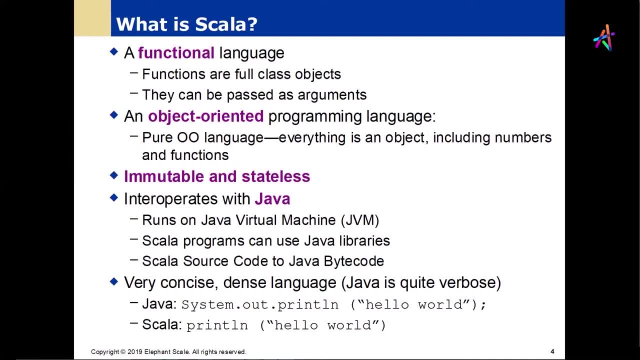 what the functional things are. the functional aspects of the language are as it relates to spark, Um, but at this point we would call Scala a mixed paradigm language. It does support the object oriented approach with Java. So anything you know about Java, knowledge about C plus plus object. 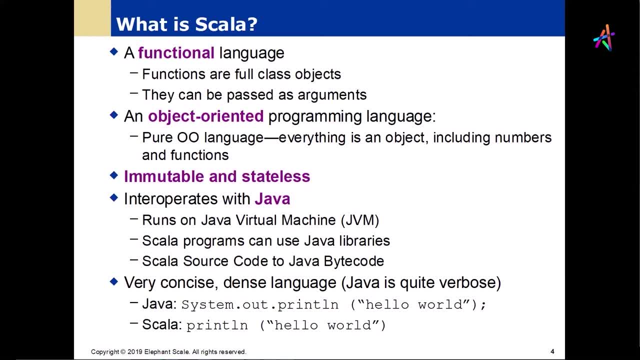 or your programming generally applies into into Scala as well. Uh, but Scala also has uh aspects of other programming languages, like it's list structure, comes right out of of list. So if anybody, if anybody's ever worked on Lisp and it's elegant list structure. 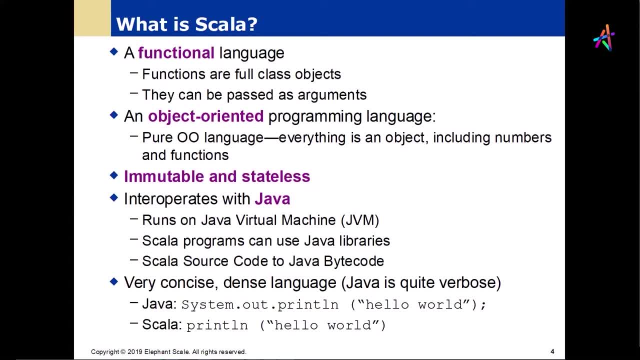 that's really great. It's got pattern matching. That is is really fantastic. Um, it's uh, also got a lot of the really functional components that we want to use. The idea behind functional programming is that things should be immutable and 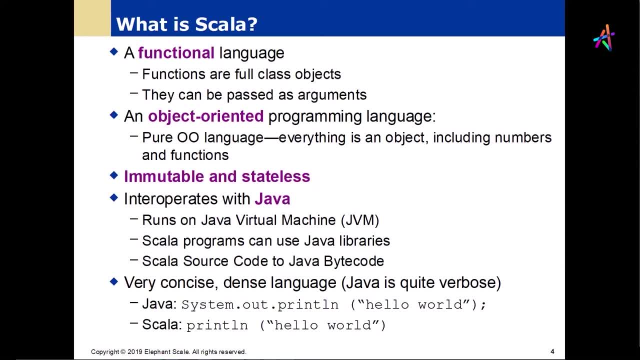 stateless, And the more we introduce state into objects as side effects, the more likely things are going to break on us. The RDD model is built around around this concept of immutable and stateless. When we create one of these resilient distributed data sets in Spark, 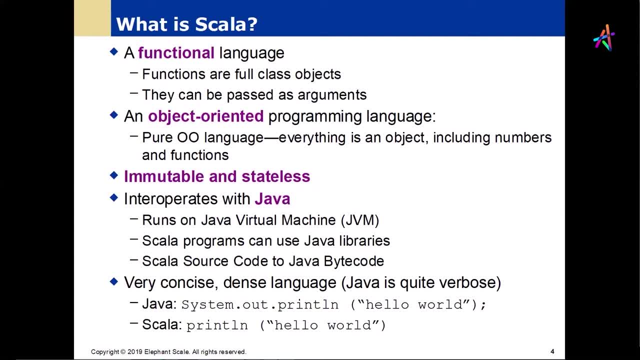 they are immutable. They don't change. That's one of the reasons why it's able to do fail over. Instead, what we do is, if I have a piece of data, um, in the example that was once given to me, as suppose, 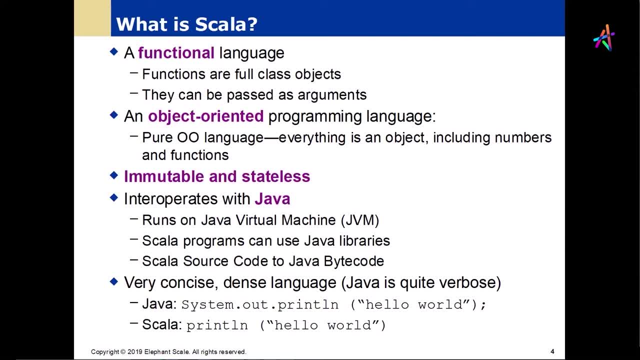 I have a form that has to go to three people and each person has to sign off on this form, So it goes to person number one. Now, in a typical procedural uh approach, person number one would get the form- sign it. 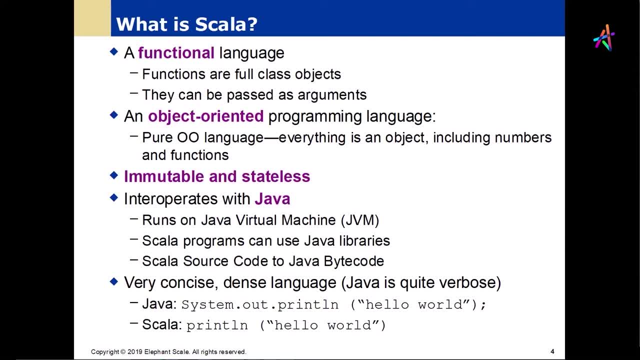 give the form to person number two and sign it. And the form is changing as it goes through each step of the process And we can never go back and see what the form was like when the first person got it after it's gone through the process. 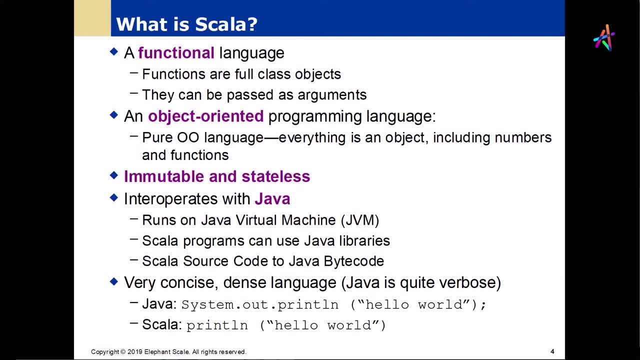 because it's changed. We can't go backwards. but what if we did it in a, in a functional approach? Now we have a form. It goes to the first person Say it's Martin, Martin doesn't sign the form Instead. 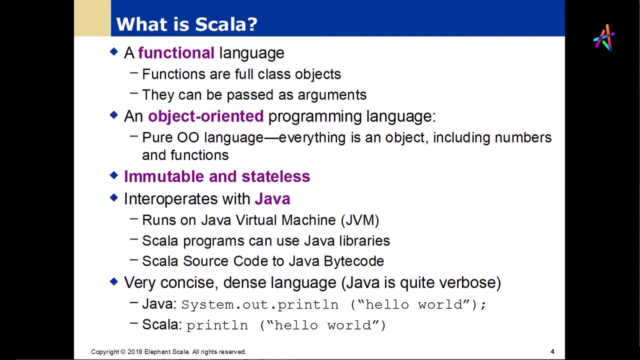 what he does is he photocopies it and then signs the photocopy and hands the photocopy onto Robert and Robert now photocopies that And then he signs the photocopy and with the two signatures now and passes that on to a Vigny or whoever else is. 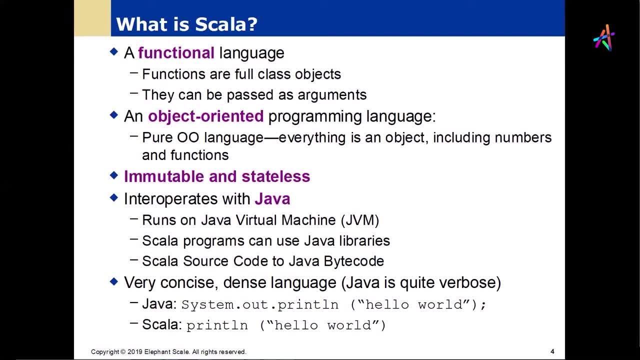 there, Uh, and what happens is that every time somebody does something, they're really creating a new object that they pass on, And the and uh once, once they've they've photocopied and passed on, they can either keep the original form. 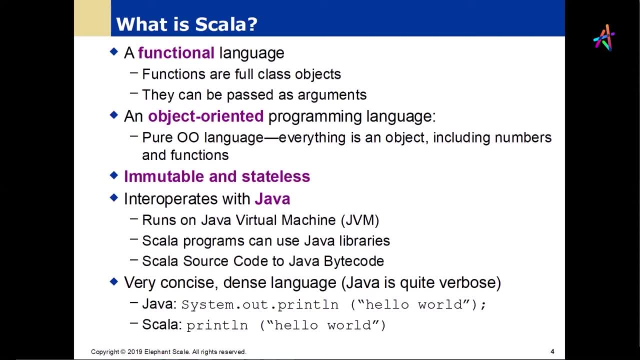 So when it gets to the end, it could say, uh, we can actually go back and say, well, what did the object look like when we first started? Well, we just go back and look at the original form. We can roll backwards on the other. 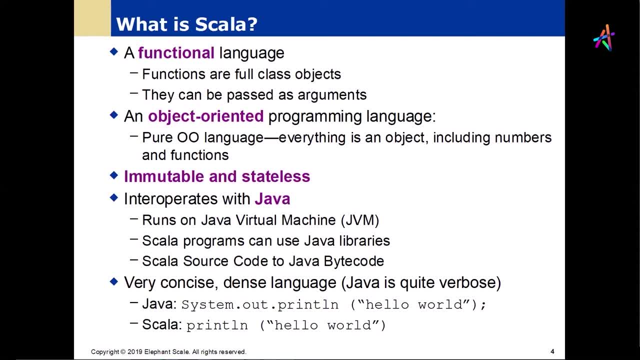 And uh, and, on the other hand, if we finally get to the end and we see, yup, that's good enough, and everybody can destroy their intermediate copies and throw them away. So this is the idea behind what we talk about: immutable and. 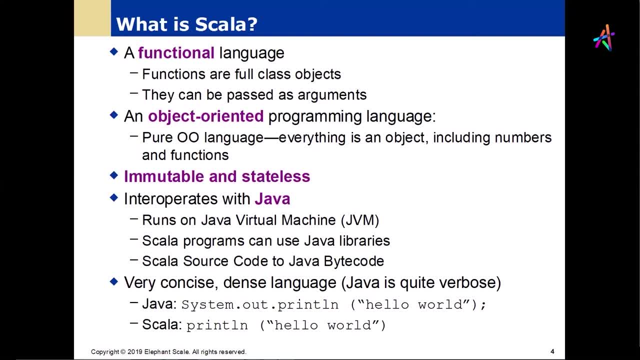 stateless. It's not that anything doesn't change, uh things. instead of of changing an object, we create a new copy of the object that incorporates the changes. Now that new copy is immutable, And that is the principle behind these resilient data sets. 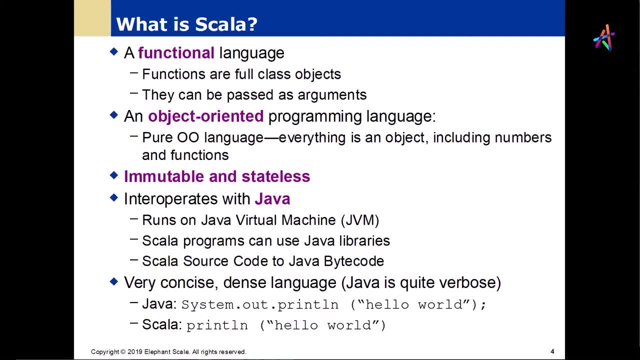 The distributed data sets is they follow exactly the same idea, so that we can always roll back to various points and be the with the ability to do that, we're able to optimize the operations that are in Scala. So this is the functional programming concept. 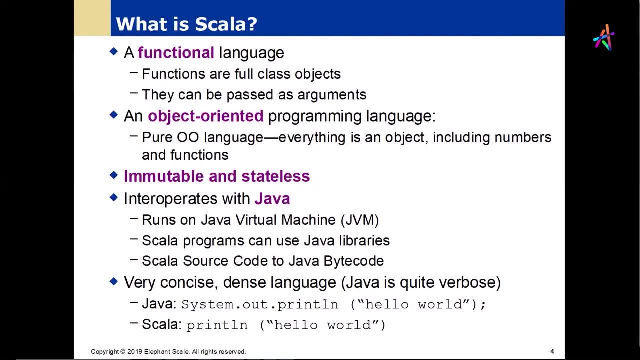 That's really important in- uh, I'm sorry, in spark. That's really important as it applies to spark is this notion of immutability and statelessness. So every object only has one state. it's created in a particular way And it's got that particular state in our 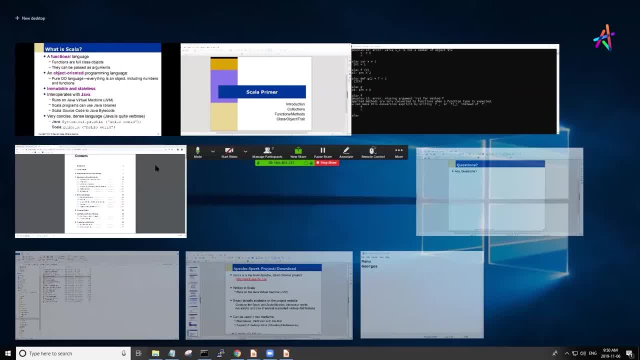 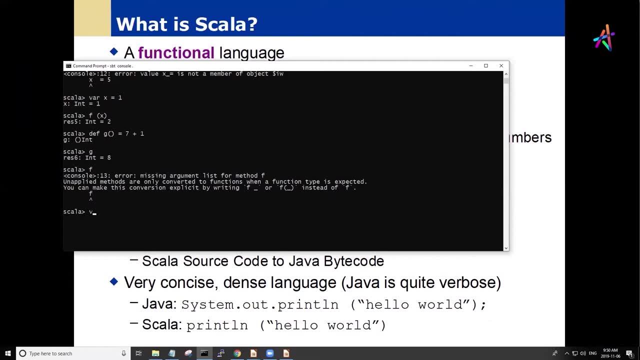 in our Scala programming environment we have a, a condescension to that, And this is the difference between uh, a vowel, which is really the the um, um, which is really the idea of a functional programming object. 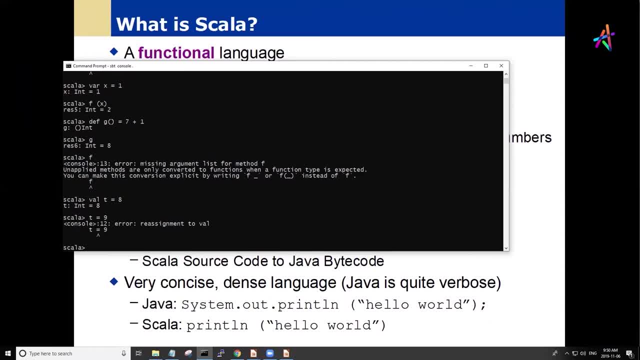 because once that's created, uh, I cannot. I cannot change it. It is now immutable. The VAR keyword is the incorporation of the Java type of programming paradigm, where now, if I put VAR equal to eight, okay, now, at this particular point, 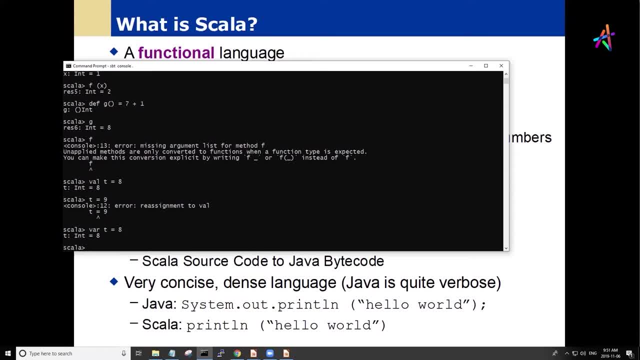 I should also point out a point about the syntax is that I now have two different variables T. I have the original one, which is the VAL, and I have the new one I've just created, which is the VAR. Uh, I'm not getting an. 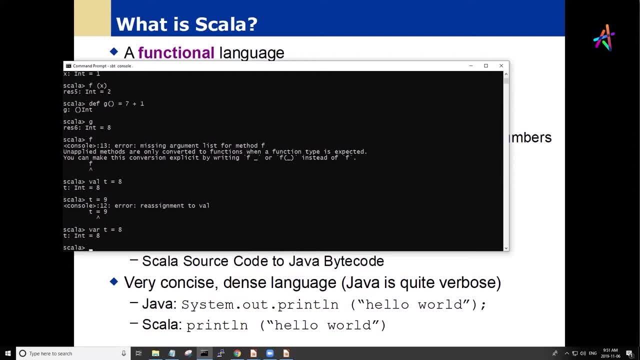 uh, an error here, because in functional programming, uh, if I drew that with doing this in a procedural environment, it would look like I'm trying to redefine a symbol to have a different meaning. Uh, the functional programming paradigm doesn't work that way. 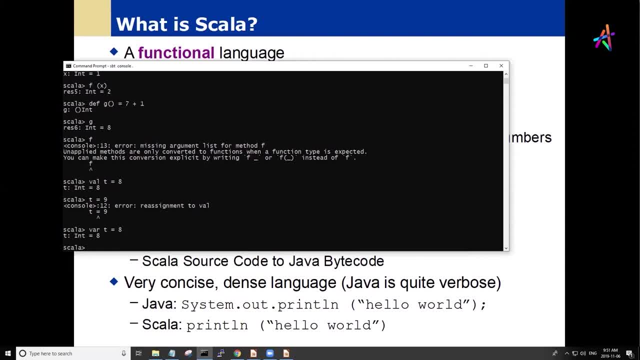 It says: okay, you created this object T. it's sitting out there. Now you're creating a new object T and it's going to shadow that old object T there, So that old object T is no longer accessible. that you created with VAL. 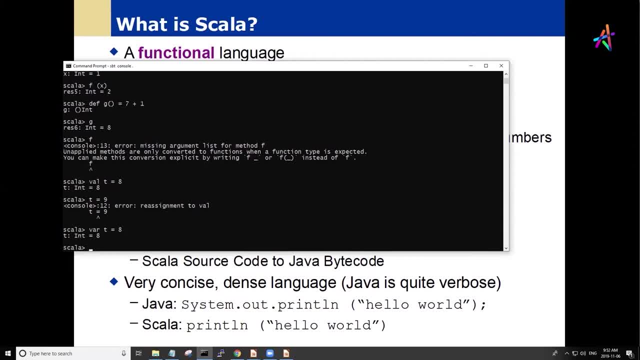 You've now got a new object called T, which is VAR, And that that that kind of shadowing effect is very typical of what we find in in functional programming. However, because this is a VAR, I am now able. 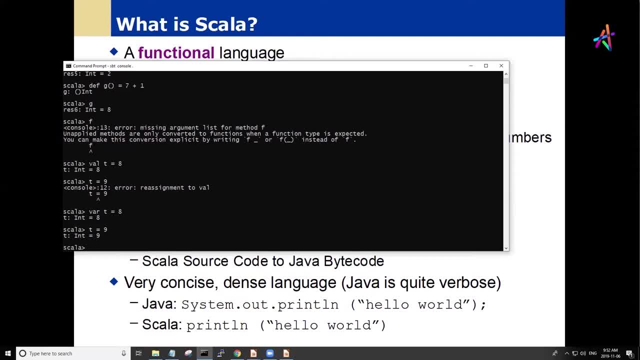 to to make that assignment, because now I've created a mutable object, So my VAR is a mutable object, My VAL is an unmutable object. VAL is very much like a resilient distributed data set in um in Spark. It follows that model. 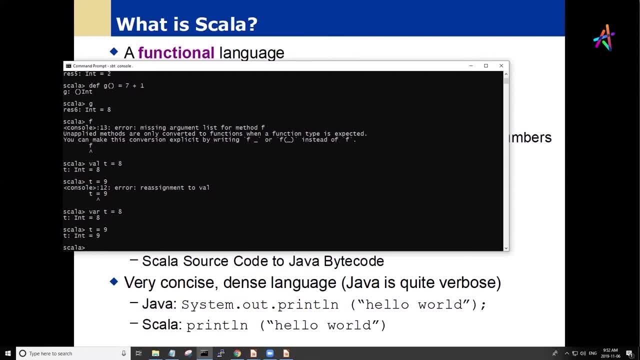 It doesn't follow the model of the VAR, which is immutable variable. So we have beautiful variables in Scala, not because Scala wants mutable variables, but because we want to be. we want to be compatible with the Java code that's in there. 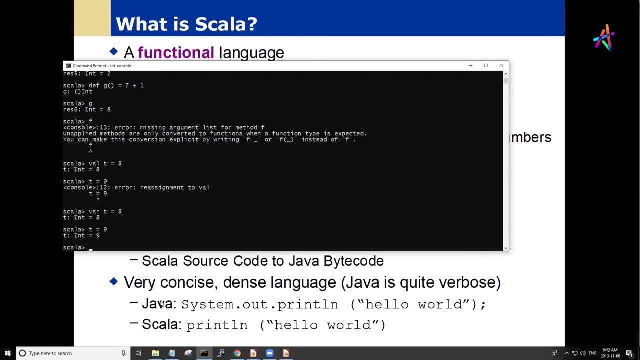 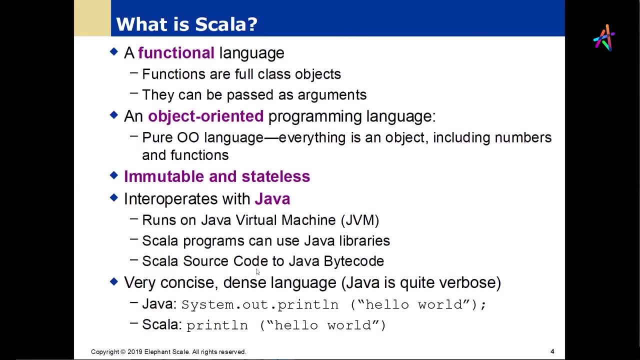 So there's the distinction between the VAR and the and the VAL. Okay, The Scala and Spark. There we go. Um so, uh, that's. that's one of the, the kind of things that we're going to see when we talk about immutable. 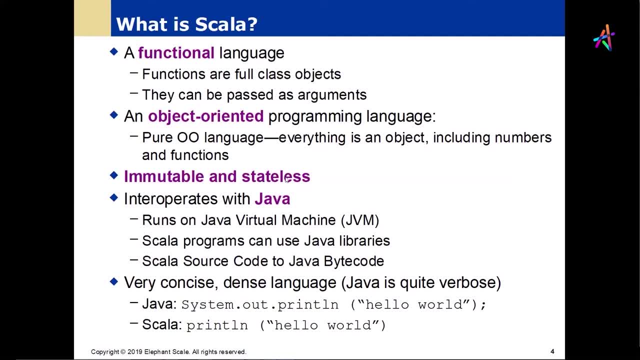 And again I'm stressing that because that's a point that's important for Spark. Uh it uh mentioned, interoperates with Java, operates on a Java baby M, so it can operate on all use, all of the Java libraries And 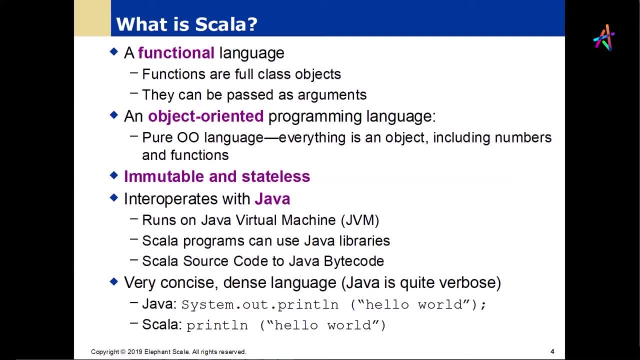 uh, it does create bytecode, And one of the keys is that it has this wonderful compatibility with Java that is leveraged by Spark. Uh, it also tends to, uh uh, be a little bit more compact in its notation. We'll get a chance to play around with it. 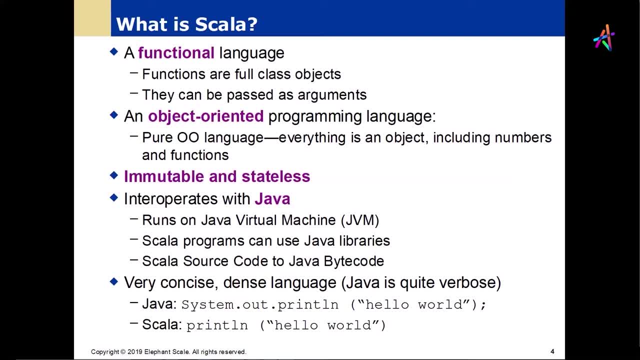 I'll go to Martin's thing. We'll take a look at some specific examples. Um, the, the uh, that, that that uh illustrate some of the things we're going to need to know for Spark uh. 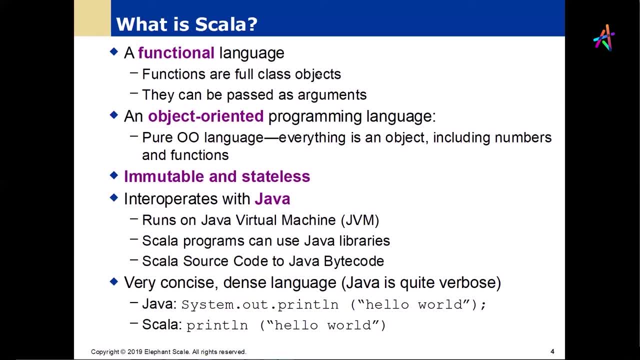 functions are full class objects: uh in, um, in, uh in, uh in uh. mathematics: We talk about uh, uh, um, uh, uh, uh, um, uh uh. first-class. 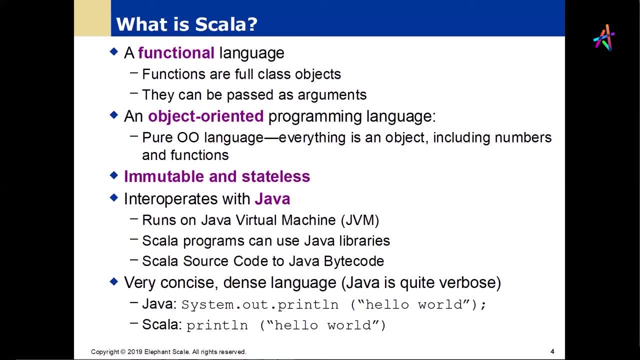 uh, object. We talk about functional objects. If you've done any done any functional analysis? we tend to manipulate functions in mathematics all the time. We can sum up a number of of functions Any time. we do a like a. 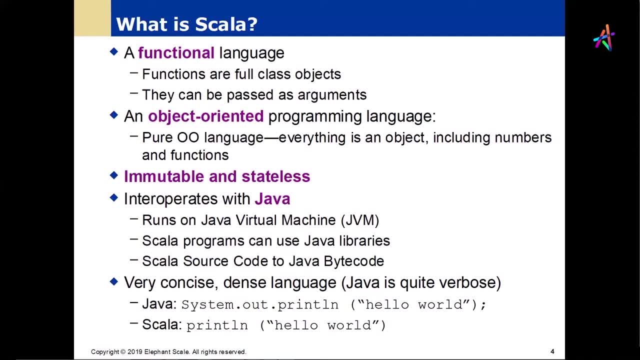 an infant series or something like that, where uh or or we're summing up, uh, some or any kind of analytical analysis. we're very used to using functions as as basically data objects And uh, what the? 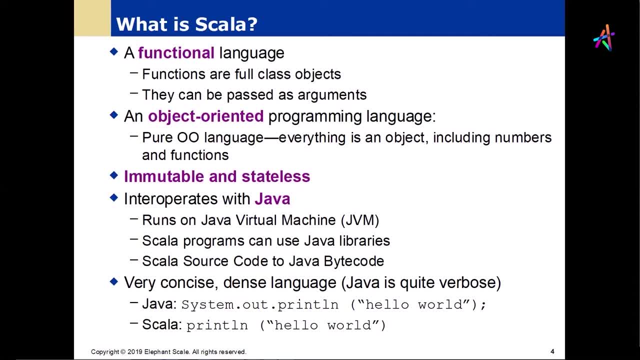 a functional language is is where we have the same ability to do that in code that we can do in mathematics. So it's a natural expression of mathematics. So we're going to see a lot of that And that, of course, is one of the 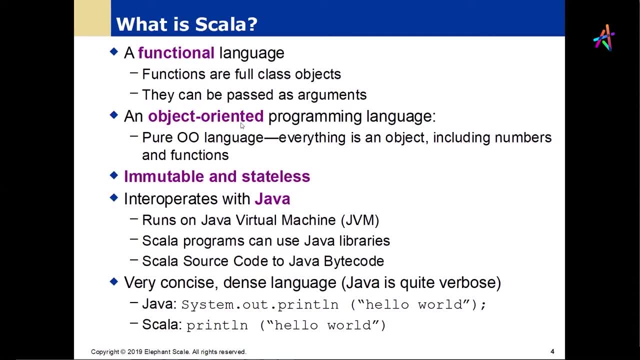 the strengths of it And you notice that that idea of passing functions as arguments is heavily adopted now by many programming languages. So, for example, Go was built, you know, with its Go routines is that's built right into the design of the language. 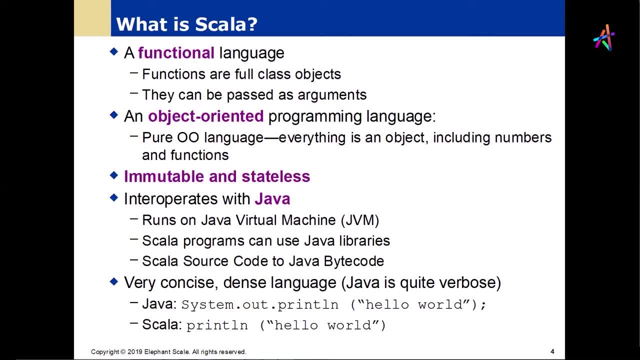 Um uh, and if you're working with uh uh, Python has uh aspects of a lot of functional programming unit as well. Those languages are not actually functional programming languages, but they do incorporate some of these ideas about what functions can do. 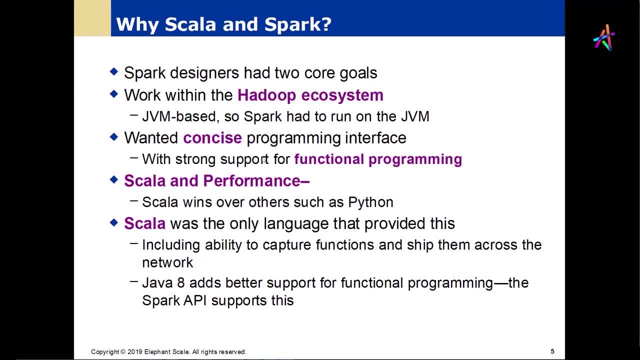 Okay, So, um, so we go back to the spark for a moment. two core goals work within the Hadoop ecosystem, where we're basically using all this, all this data that's sitting out there on these Hadoop clusters, And we also want to have a very 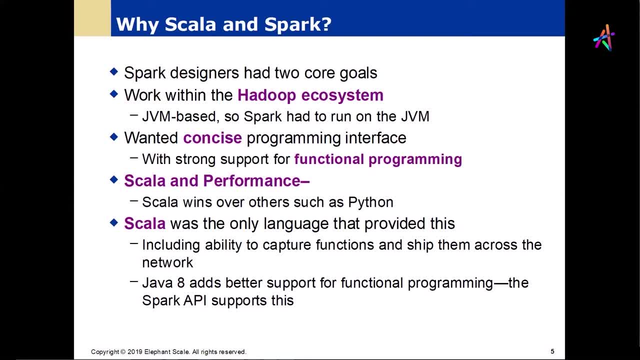 very elegant programming interface. Um, and we also wanted to employ- I keep saying we- I'm not going to actually do it, I'm using the Royal- we here, we as a community, uh, uh, or, I'm speaking on behalf of the developers- wanted also to get a elegant programming model. 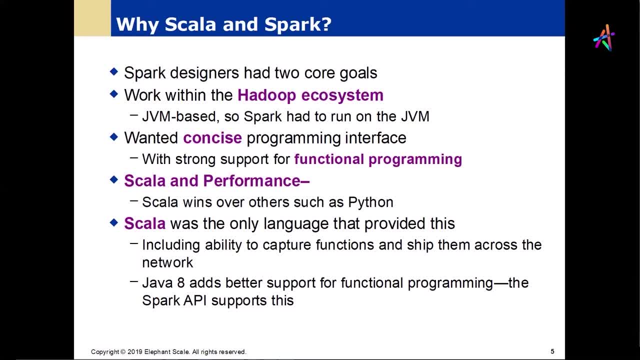 recognizing the fact that we don't want to spend a lot of our time writing and maintaining large, large chunks of of code, So the uh Python is a possible candidate. The problem with Python is that it does not do strict typing. 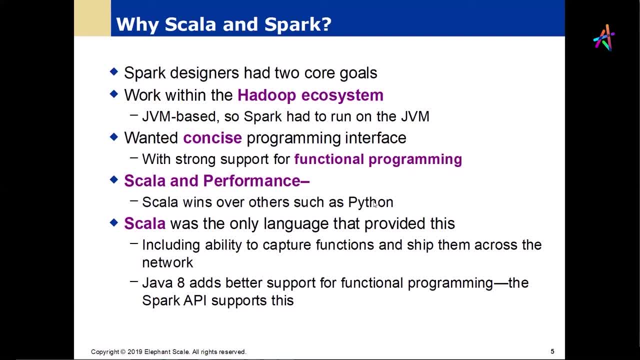 Uh, it's not a uh to checking, which means that some of the efficiencies that spark needs can't really be done in Python effectively. So Python is not really the optimal language for working with spark because of its untyped nature. Uh. 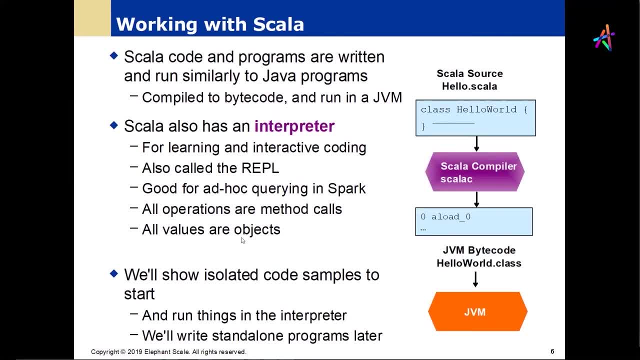 and and, and we've got some Java, um functional programming, that we can kind of leverage here as well. Uh, so Scala code and programs run, uh follow the same process of being compiled down to byte code. Uh, Scala C is the compiler. 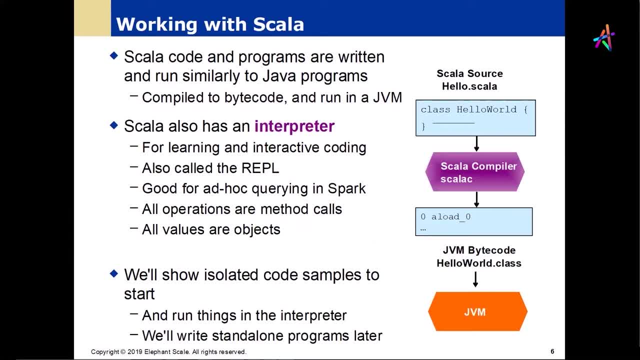 uh, where we can, uh, basically, uh, uh, run it the same. We run a Java code, but we also have an interpreter, which is what I'm using with that rebel to give some examples, And that interpreter also then allows us to work in a 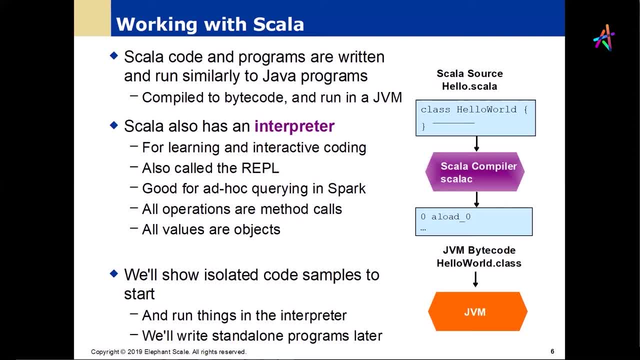 in a Spark environment and a Spark shell to do similar kinds of queries. Uh, all operations are method calls, uh, and that's going to be something that I'll demonstrate before we'll take a quick break Again. this is another point that you have to get used to in Scala. 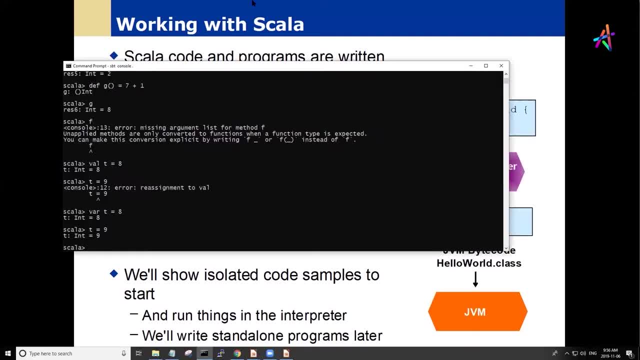 So let's go back into my Scala language here and let's take a look at a couple of things that look really odd to start with. Okay, So first of all, this doesn't look odd at all. That doesn't look odd because that looks like an operator defined in a standard programming language. 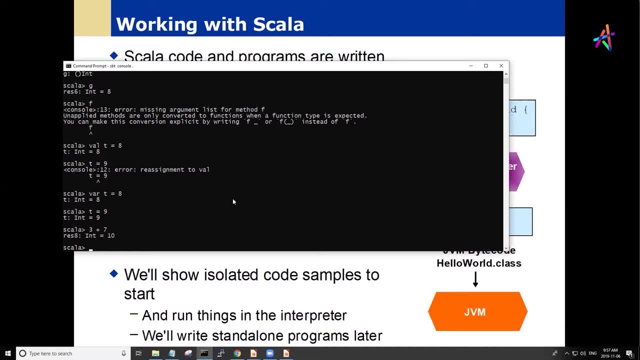 The problem is that that's not an operator, That's a function, And I can rewrite that as in which being able to do that and get the same result shows me something that's actually going on in the language That's not immediately apparent. 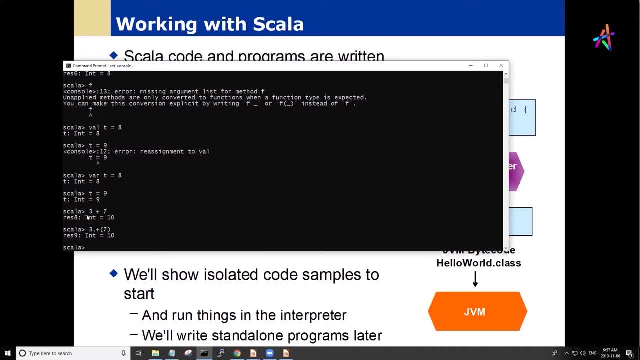 This infix operator notation in Scala is syntactic sugar, Whereas this is actually defined in the- you know the grammar of most programming languages- as an operator And there's an argument on both sides. in Scala It is really, uh, just. 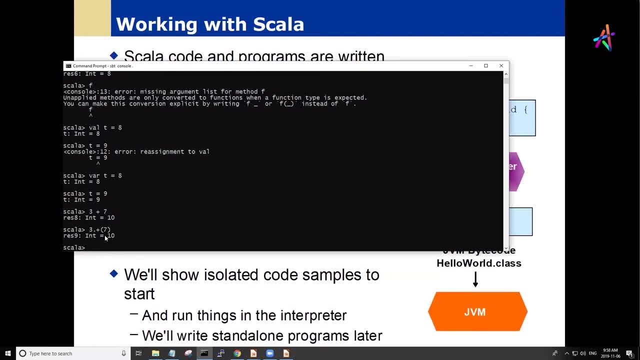 uh, another way of writing this piece which says: I have this expression here which just happens to be a literal, and the um, and I can call a function or a method on that literal which is called a plus sign, and give that the argument. seven: 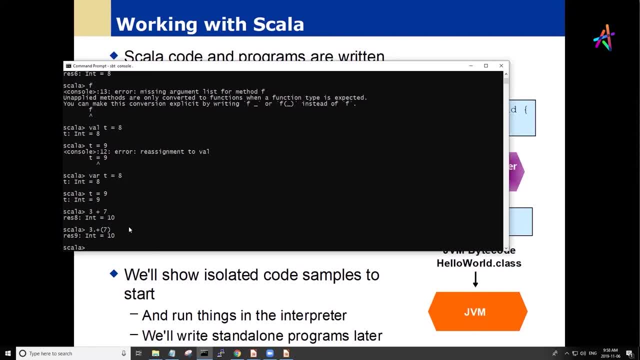 And this would be the same as if I had written a function called add and uh for an integer class and assigned this to an object in an integer class and called the add method on it. It's exactly the same idea, So there's a couple of deep concepts here that are important to understand is, first of all: 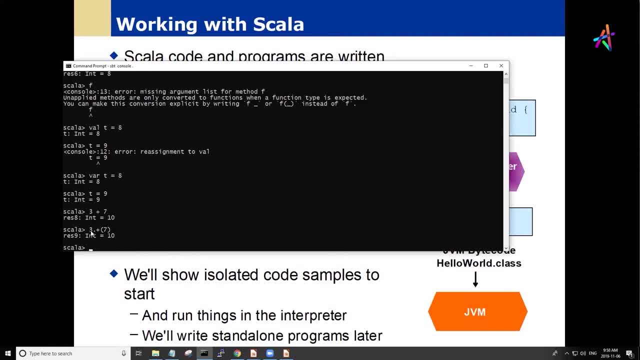 these literals are no different than anything else. So in word Java a literal is very different. Like in Java, you couldn't call a method on the literal. You have to put the literal inside of some kind of construct and then call that on the construct. 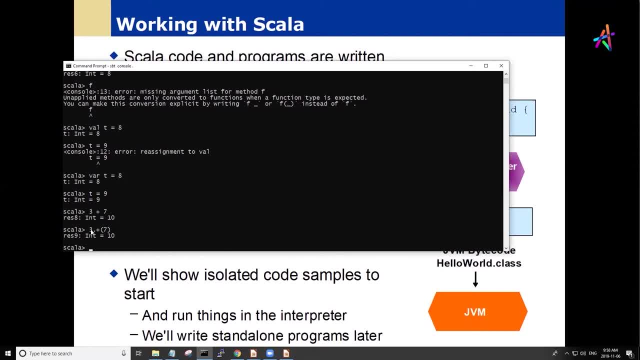 Or even if you wanted to do, uh, you'd have to call some static method and pass the literal as an argument, And we've got things like the int classes to give us that kind of programming construct. Scala takes a very different approach on this. 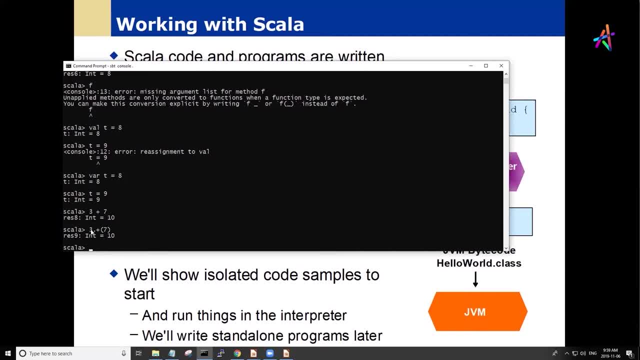 What Scala says is that everything is an expression, So everything evaluates to something. Uh, the only difference is is that a literal evaluates to itself And what Scala realizes that when I evaluate the literal and I get the same result back, I'm done my evaluation. 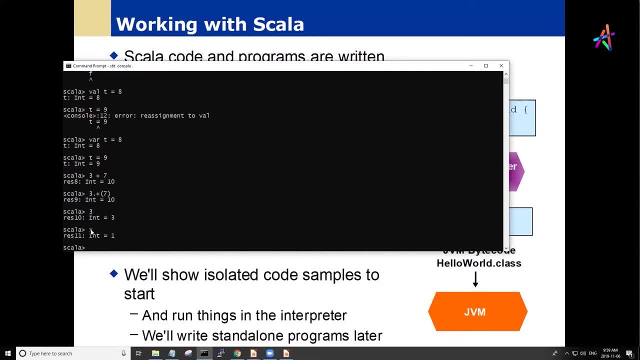 So when I put X in here, what Scala is really doing is saying, Ooh, I've got an expression. I'll evaluate the expression and I get a one back. Now, we'll evaluate the one, I get another one Back. 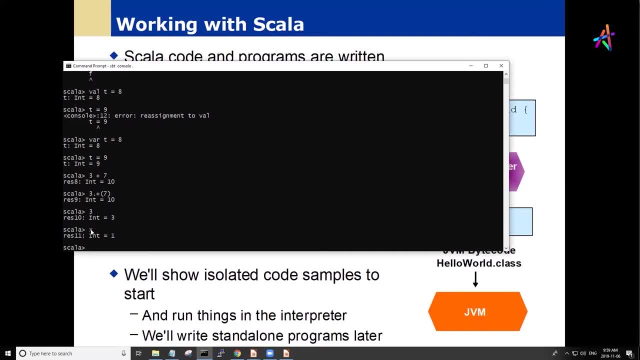 Okay, My evaluation sequence is terminated, So the final result I'm returning is going to be the one. So we again have lost the distinction between literals and variables here. They're all just expressions. Everything returns a value in Scala. Well, that's actually pure Scala. 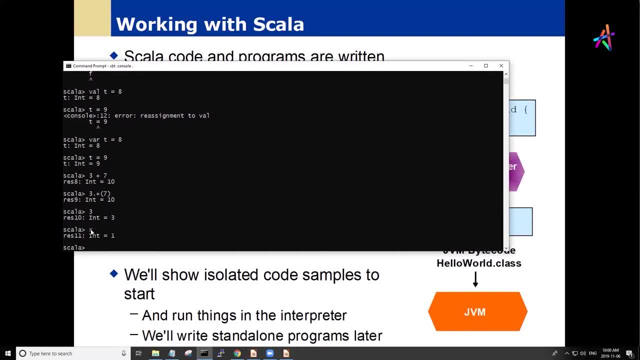 So our if statement looks a little bit different. So I can say: there we go. So I can. I can say this: uh, except this string. but the literal is found: Uh, ah, thank you, I knew it was some. 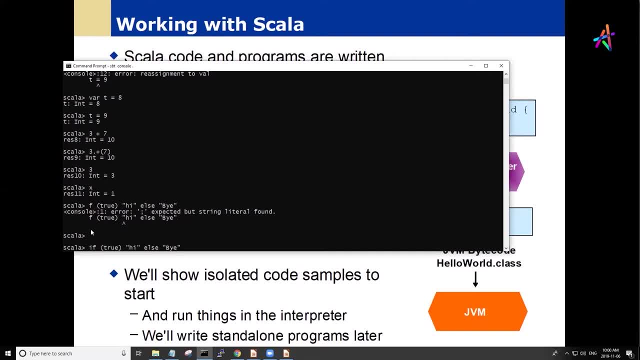 some ridiculous error like that. There we go, Because I'd already defined F, Okay. So what's happening here is that um in, in, uh, if I've. I've looked at this from a procedural point of view. 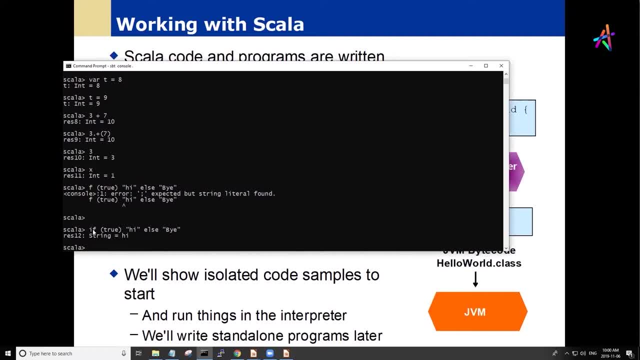 what I might think is happening is that I'm encountering a control structure in the language and I'm encountering a Boolean condition which I evaluate, And then I would execute a whatever code is here, or I would. if it's false, I'd execute whatever code is here. 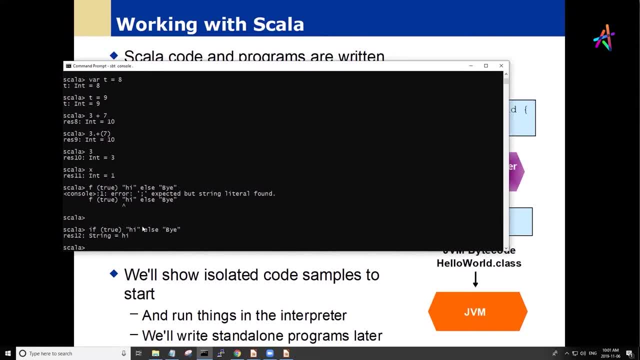 And I would think of this as being like a framework, a framework that holds these two alternative ways of executing code. in functional programming, We think about this really really differently. in functional programming, We're we're, we're basically saying: rewrite this. 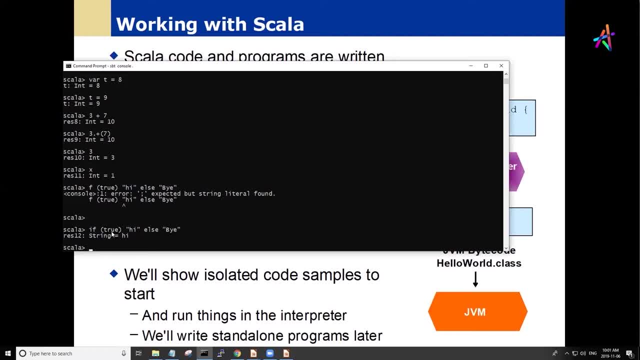 And if we have, if, uh, and if this, this first part, is true, our rewrite rule says: then then then basically rewrite it as this: if this is false, then rewrite this whole expression as this, And in this: 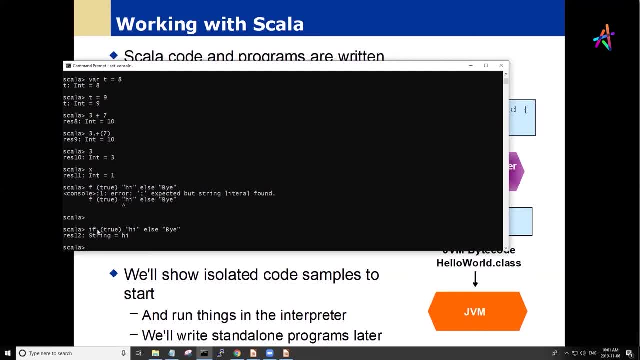 this particular case, what Scala did was that okay this expression, if true, high, else by okay. When I apply my rewrite rule, I get the string high. Then I evaluate, rewrite my high, I get high back again. So I'm finished my evaluation. 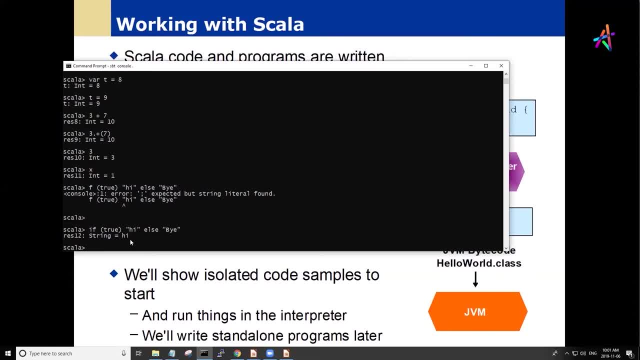 So it's a different way of thinking about how these things work And, of course, what I can do is I can go and assign that result of that Computation into into a variable. Okay, All right. So what I wanted to point out in this initial kind of discussion is just a. 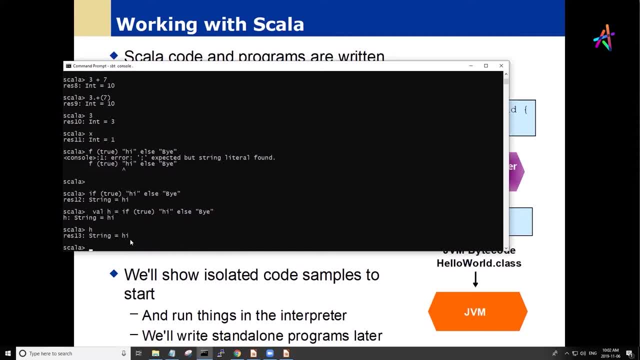 couple of little examples to show that, as we go through the rest of the Scala, is that what's going on under the hood? while it might look syntactically very similar to what you're used to in other programming languages, there's actually underlying ideas that are quite different in terms of how. 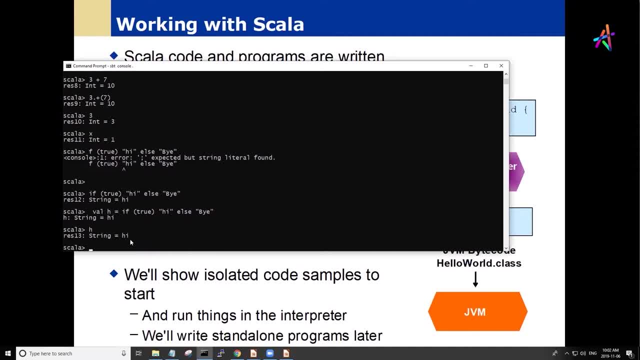 you read the code that's in Scala versus how you read the code that's in Scala The code that's in another programming language. The reason I'm making this distinction is that these concepts are the same concepts that show up in how spark works with its data as well. 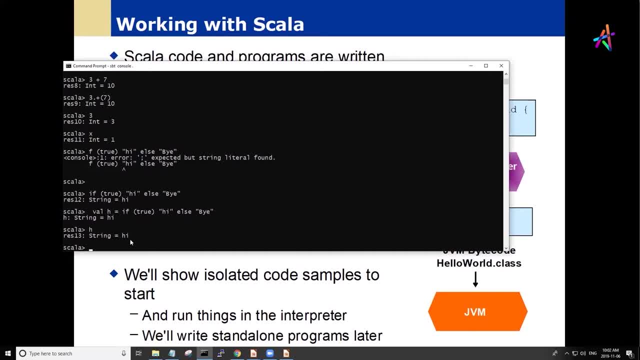 Okay, So let me just take a quick moment here and say: how are we doing? everybody, Everybody- is this working for everybody? so far, Is this a let's get some feedback on how we're we're coming along here, guys. 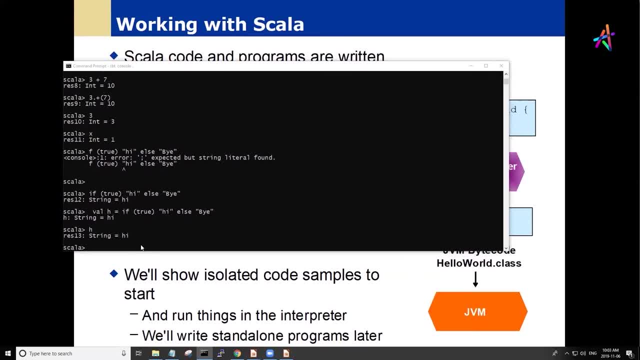 How are we doing? I'm sitting here, Pardon, You're still here. You're still present, Okay, Is it finding this useful? Yeah, I was already introduced to Scala a bit, So maybe people who are new to Scala for. 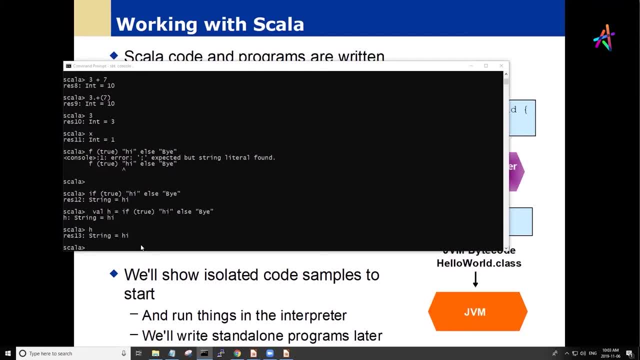 I think for them it's useful. Yeah, Okay, How about some of you guys who are new to Scala Is this? is this being useful for you so far? Well, these are the kind of concepts that we have already learned, because. 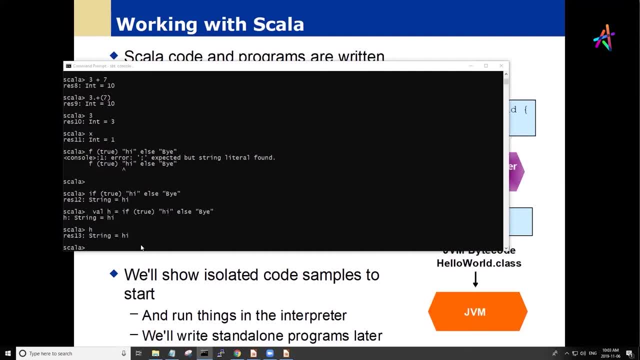 because we haven't to work with Scala in production, But it's always good to touch upon the basics, Okay. So yeah, that's. we still constantly keep in mind that things are built in a certain way in Scala than in the language that we used to. 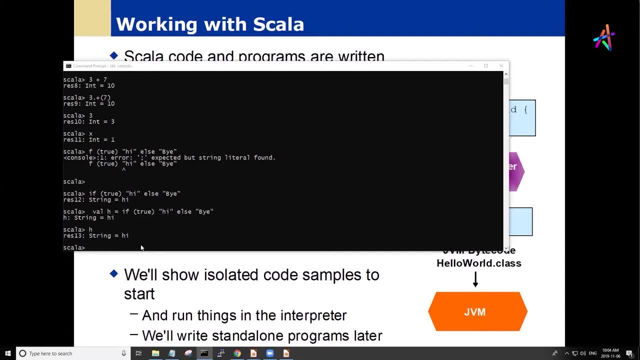 Okay, All right. Anybody else want to? to chime in? I'm always trying to to adapt to what we're doing here. Anybody else have anything that they want to add to it? You guys want like a bit of faster pace, or do you want to? 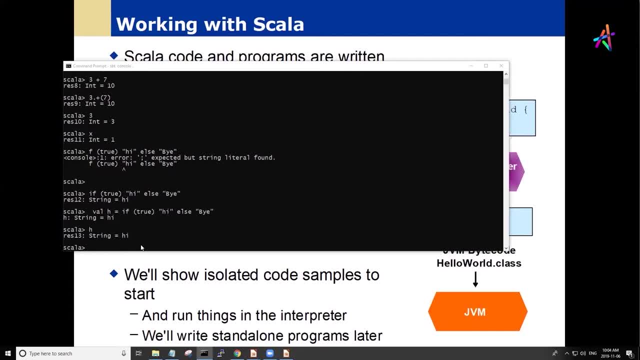 Nothing new so far. It's good, I'm sorry. Could you just repeat that There was an echo? Sorry, Could you repeat that I got an echo. I just said that. nothing new so far. Nothing new so far. So this is all familiar stuff to you guys. 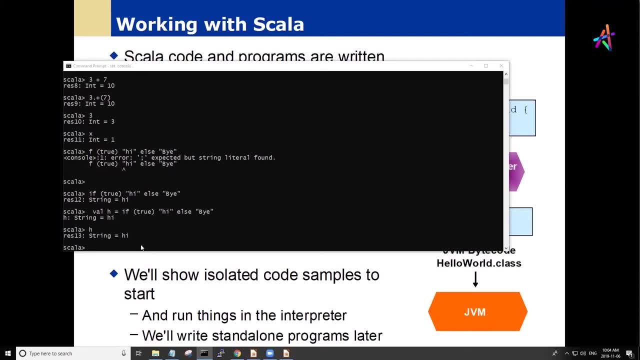 Yeah, Yeah, I would say. even so, I would say that even people that don't aren't really native Scala, people sort of know this by being exposed to other functional languages. So me, for example: yeah, I haven't really done any real Scala work. 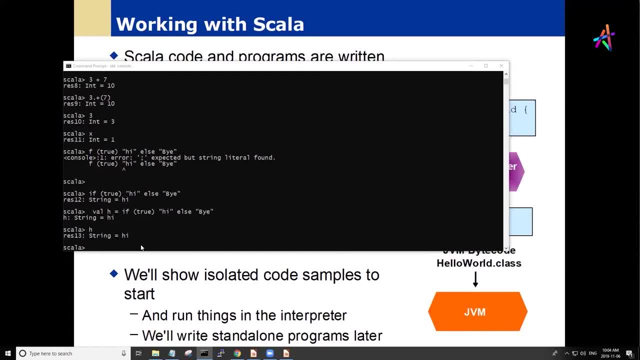 I did touch a little bit of a lot of the projects that we have, but I was exposed to other functional languages that sort of already covered these types of topics. Okay, All right. Well, what we'll do is we will take a break for about a fifth. 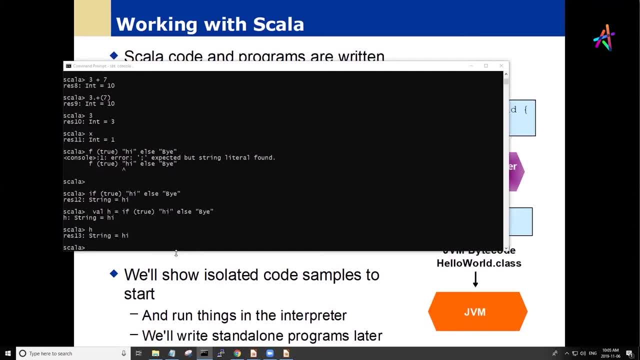 say 15 minutes, Everybody chance to go and get some stuff, and then we'll come back and we'll we'll finish up with this slides and we'll then start into getting up some virtual machines and signing them out to you. All right. 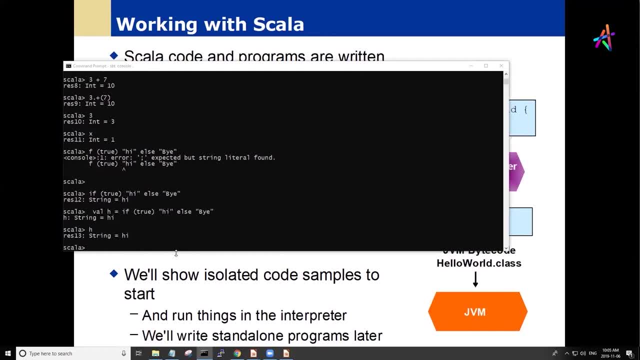 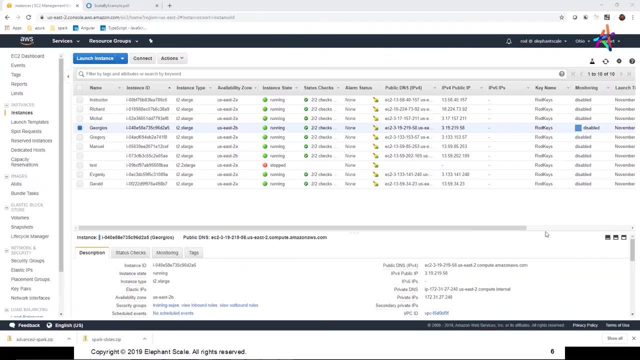 Super perfect, Thank you, Thank you, Okay. Okay, guys, How are we doing? Are we back? I'm back, Almost All right, I'll give everybody a chance to settle in. I've just been setting up the virtual machines here and we'll 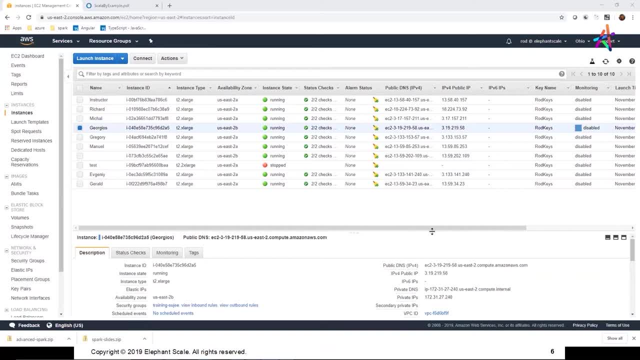 we'll spend some time just getting you guys logged in so you can play around with them. before I go back into the presentation, It's just something we need to get done. on my screen, I think you should be able to see the instances I've set up. 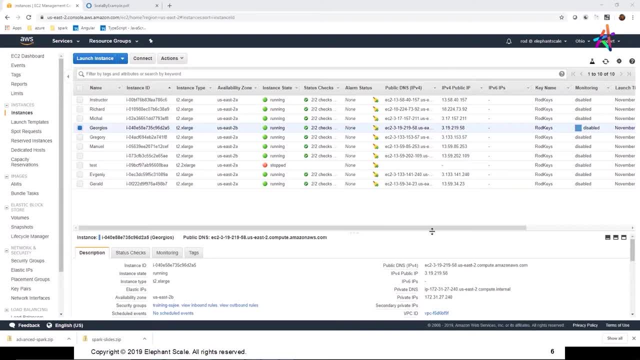 in AWS And I think I've got everybody accounted for. My account might be off. Is there anybody whose name is not on that? I think Roman and me We are missing, but we don't have a Richard. I don't have a Richard. 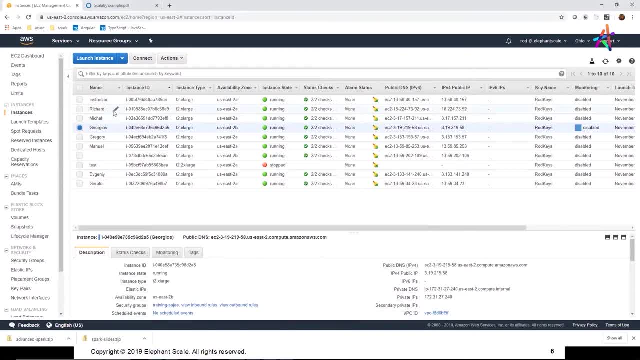 Okay, Well, who is speaking there? Robert, Robert, Okay, That probably should have been you then, Unless you want to become Richard and Roman, Okay, All right, So now. is there anybody that's not accounted for at this particular point? 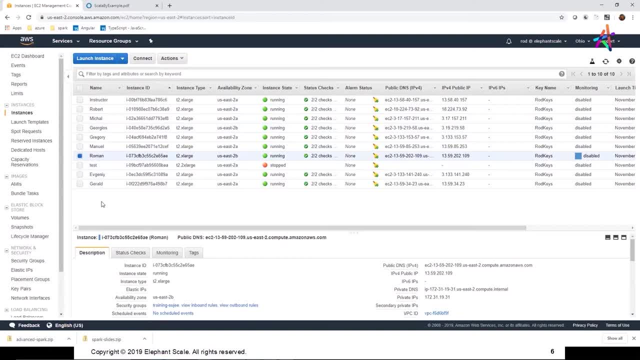 I think we're good. Should be everyone. Yeah, I'm sorry. I think everyone is on the list, All right. So this particular I'll I'll assign everybody a machine here with an IP address And I'd rather than you try to copy them off the screen. 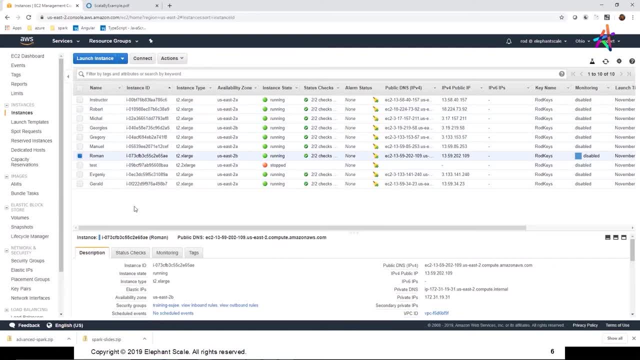 I'll just go through and chat them individually out to you, So you can just do a cut and paste. There's two pieces of information you need on each machine. One, of course, is the public IP address. So I'm going to start with with Robert and I'll even. 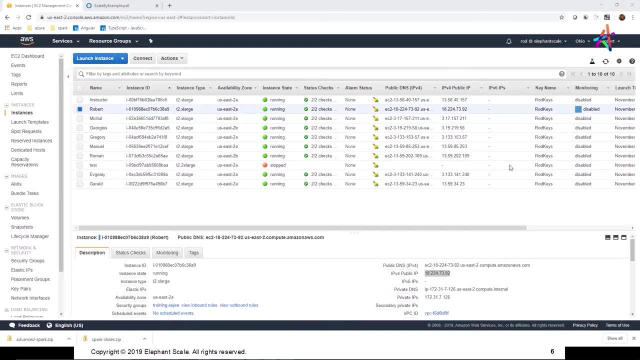 I might not get dollars. So, Robert, there's your IP address And the other thing that you're going to need is a password, And generally, the password is going to be this instance ID And if you, if you are, are, if you do want to grab it yourself, 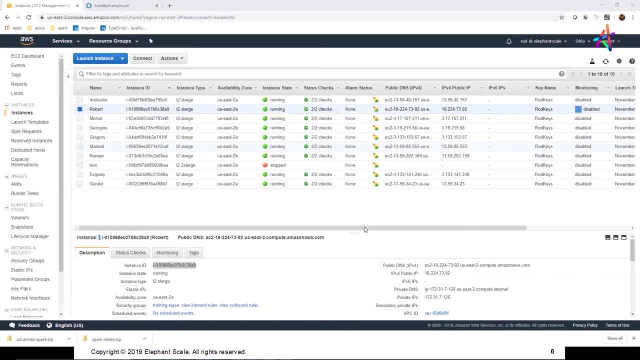 So so there's. there's Robert, And I was trying to figure out a fast way to do this, So that's Robert's Thanks, Okay, And so then we'll go to Michael. Here's your IP And Michael's instance ID is that I ran up a few of these the other day and tested them. 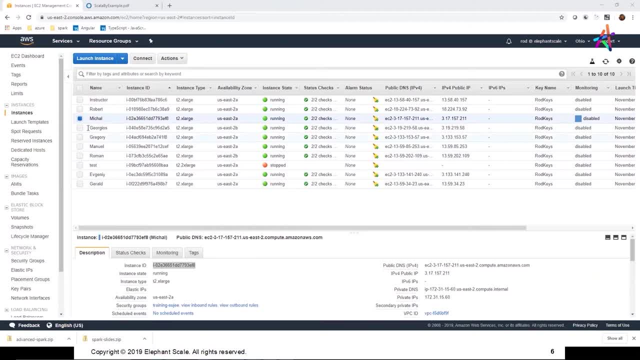 I should see be fine. Okay, Glorious, Here is your IP. I open the file And your instance ID Probably be the best way to do this, Gregory, helps avoid people trying to make copying errors, copying off the screen, particularly with this. 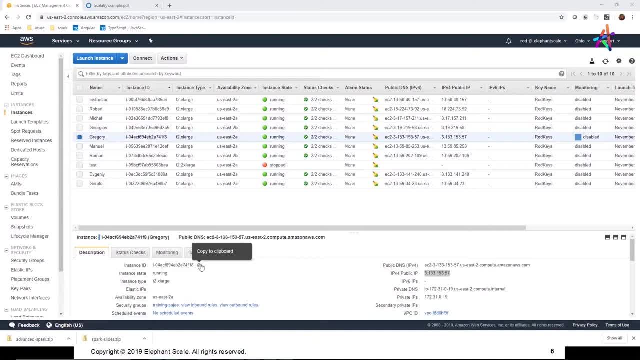 these instance IDs And you can kind of match up on the screen, If you're with your IP address, to make sure you've got the right one here. Okay, Manuel, Yeah, the instance ID is going to be your password And I'll basically show you how to get onto the machine. 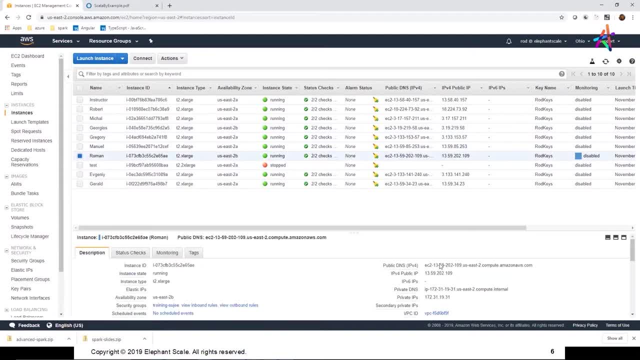 Uh, this is actually a new environment for me too, So I had to play around with a little bit. Um, oops. I was dreading this part. I knew this was going to be tedious somehow And Vigny Everything. 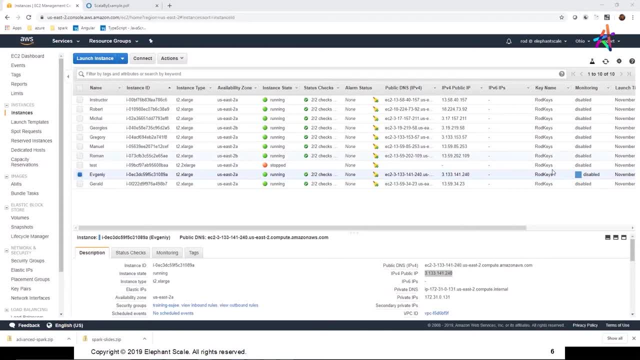 Good job, Good job And finally, Gerald. Okay, All right, So if you want to paste those away somewhere in a little text file, you're going to be able to use that information If you just want to paste that away. 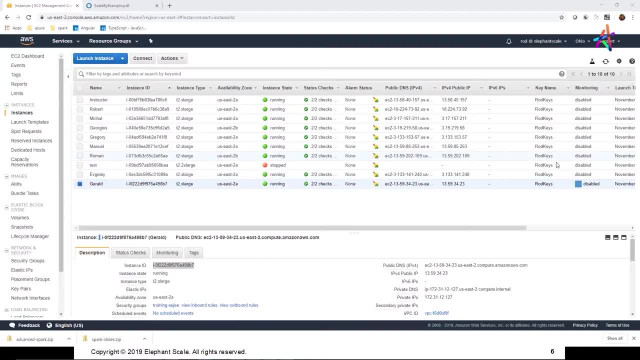 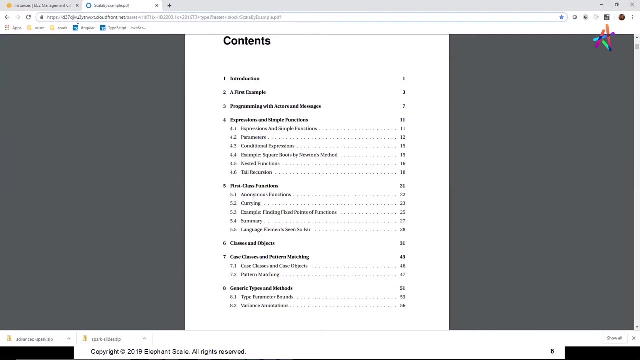 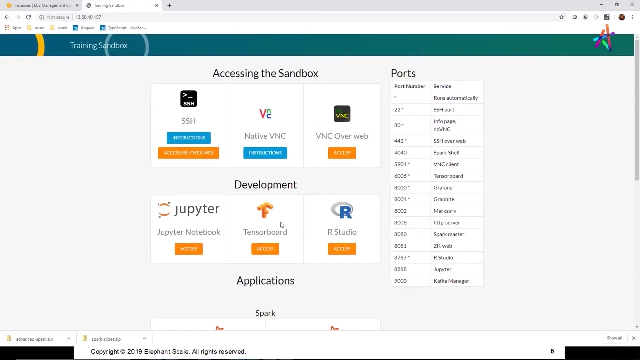 And what I'll do is I'll introduce you to the to how we're we're getting onto this. It's fairly straightforward. So what you want to do is go to your your IP address and what you should see is this training sandbox environment, and there's a couple of things that 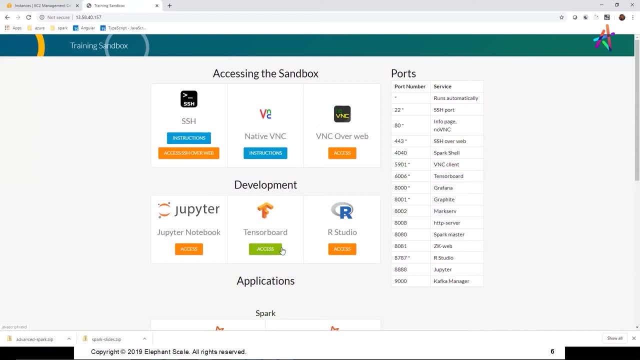 we're doing. nothing is actually set up in terms of spark. you're going to do that- set up as one of the labs. so there's a couple of places you're going to actually, um, we're going to do that a little bit later on this morning. we're actually going to set things up. uh, there's a couple of 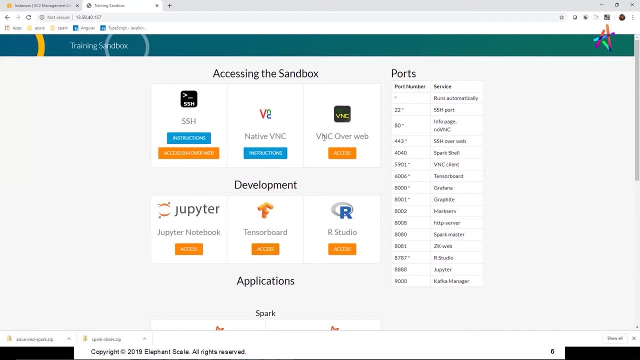 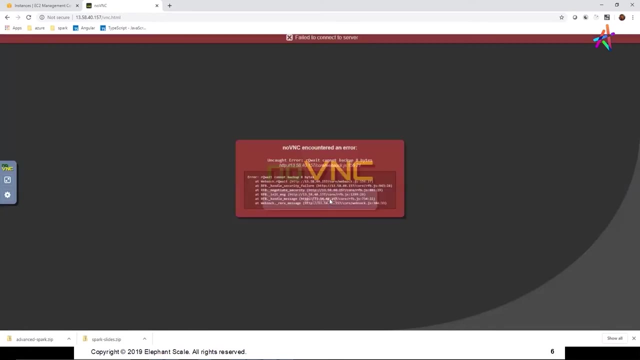 things that are useful for you. uh, this vnc is is a remote x desktop and you're going to be able to access that uh by if we do access over the web. uh, we're going to get this, uh, this no vnc and okay, okay you. 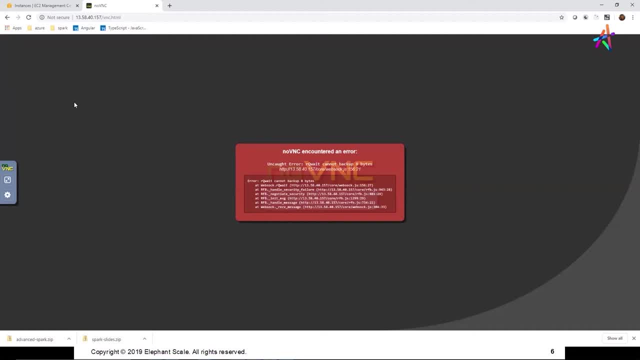 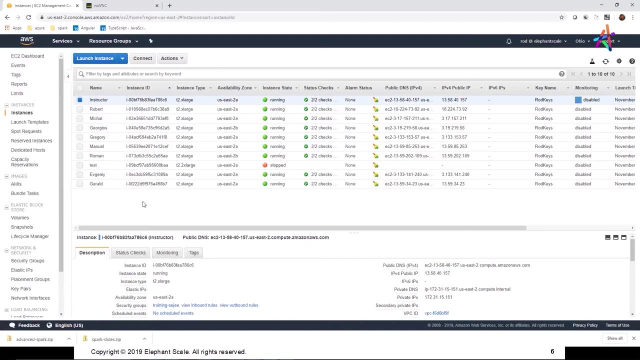 okay, i just did this. is anybody else getting that problem? yes, ran this test last night and it worked fine. i think i tested on your machine, robert. worked fine. i got too many authentication failures. really same thing for me. new connection has been rejected with reason: too many authentication failures. 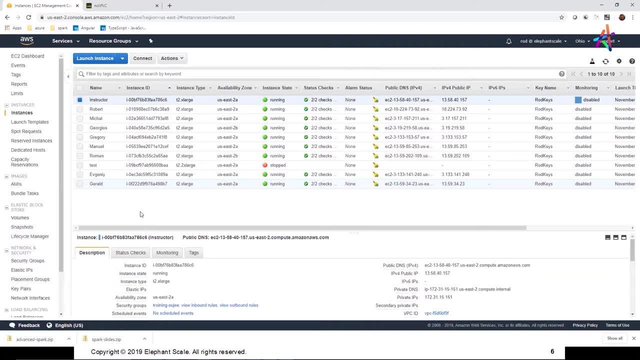 thank you. yes, all right, because i was in there last night working with it on on one of the machines and it seemed to work fine. um, so i'm getting an error on my machine too here. okay, so what i might do is: uh, we'll have to. 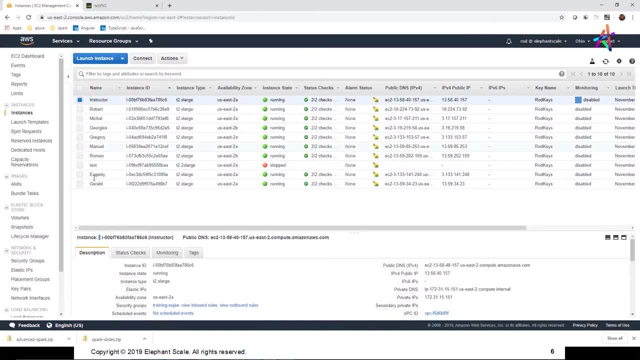 maybe hold on to that. i'll try and resolve that issue. tests work perfectly. pardon, but my, my machine is fine. who's that? i just, uh, it's evgeny. okay, and uh, i just logged in into this stage. yeah, so you got in, okay. okay, so let's have a little poll. uh, who was able to get in successfully? 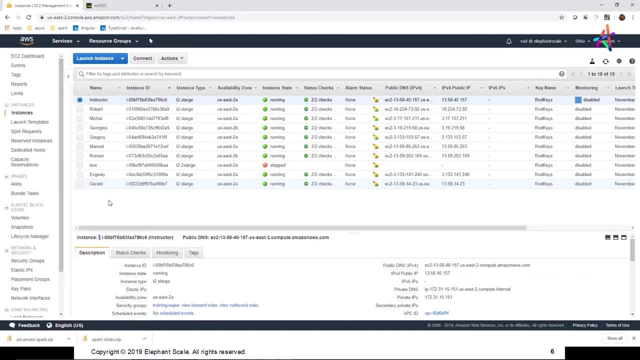 evigny one. i'm still trying. okay, how can you enter the password? just just this. uh, yeah, the password is that instance id that i gave you. so i gave you an ip address in an instance id immediately following, so our own here. speaking, i'm trying to do ssh and 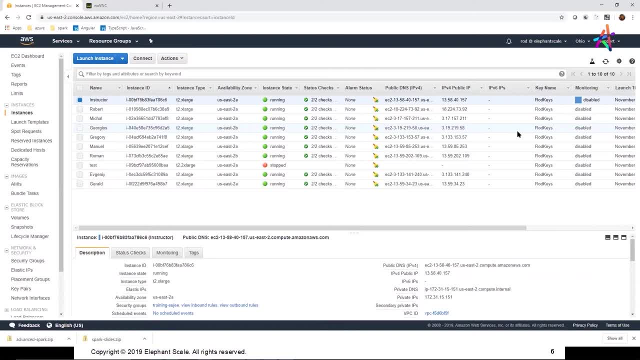 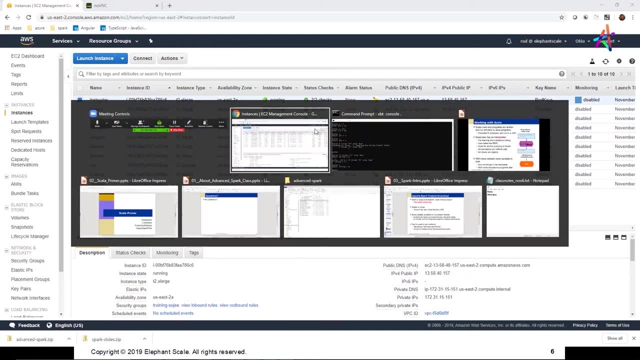 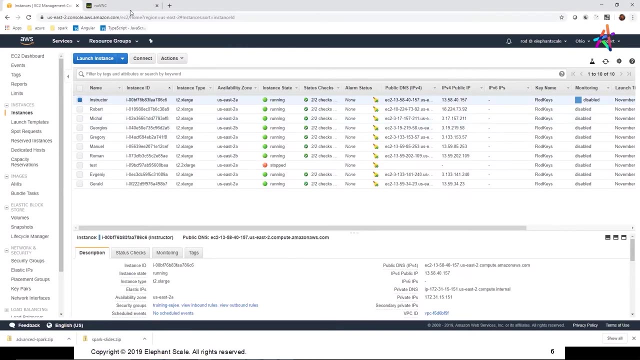 when i enter the password, it asks for password again. yeah, same for me. okay, you don't use your ubuntu user. that's what the instructions say. yeah, here, what i'll do is is: i'll at least try that part. um, so ssh works for me. this is mike. 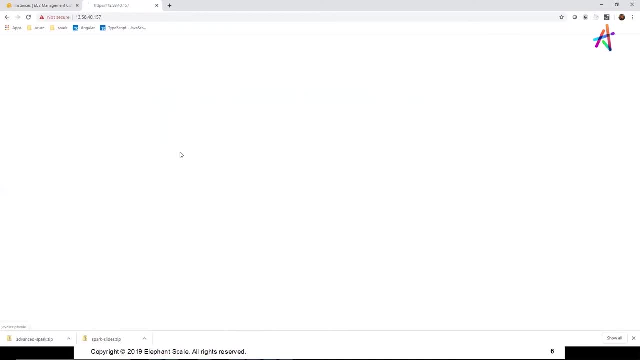 yeah, i think the ssh is not a possible SSH over the web- Maybe a problem, but I just SSH using a terminal and that was fine. Yeah, Yeah, so this should be fine. The password should be that instance ID. oops, that's the IP address. 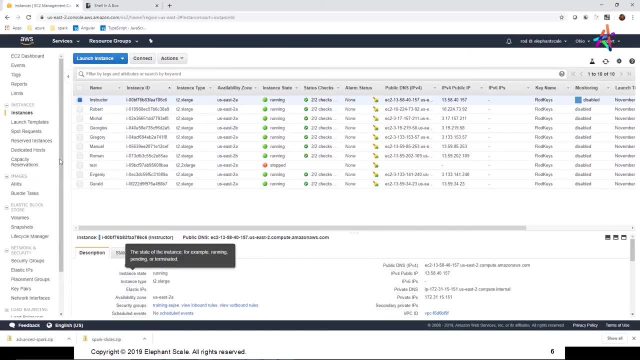 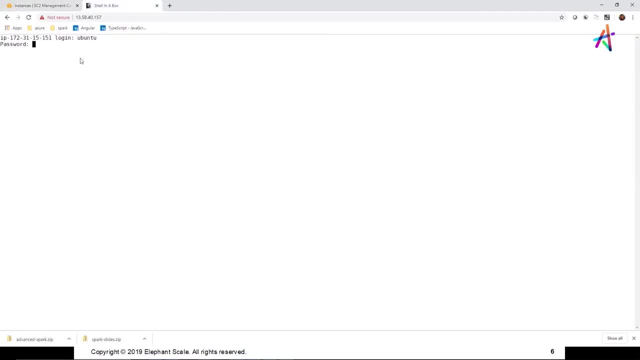 not the instance ID. So I'm getting the wrong password both in a web SSH and normal SSH. Oh, really, okay, Looks like I got in. That's one more, the address and the All right, so I got in fine with my SSH. 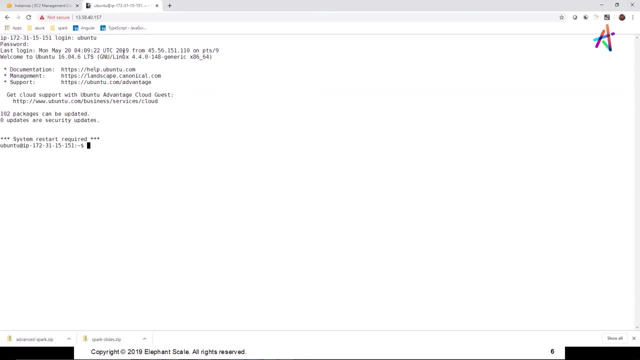 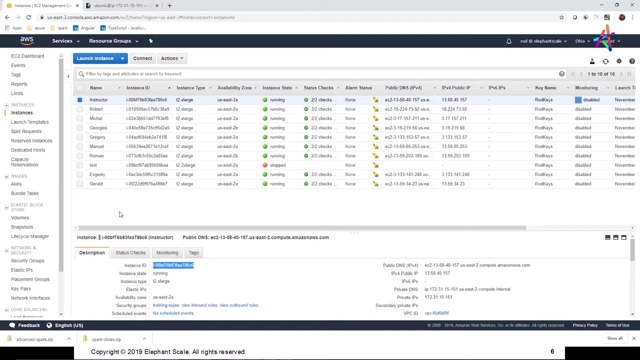 but I'm running into problems with the NC. okay, All right. so if you are having no problems with your machine, send me a message, send me your name and I will keep your machine up. If you are having problems, then what I'll do is I'll try to spin up. 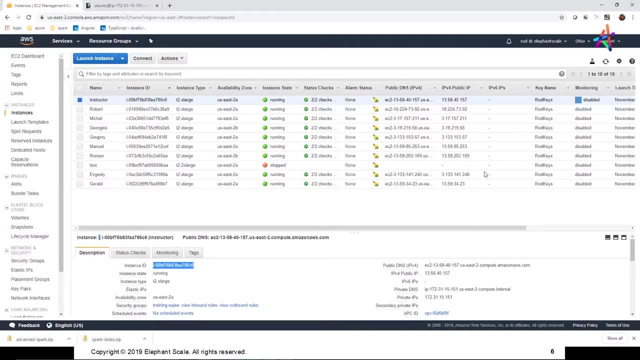 another instance for you and see if that doesn't solve the problem. okay, Maybe also people could double check passwords. So yeah, Roman speaking here, I confused the first line and the second line because they're all coming all together without any blank line. 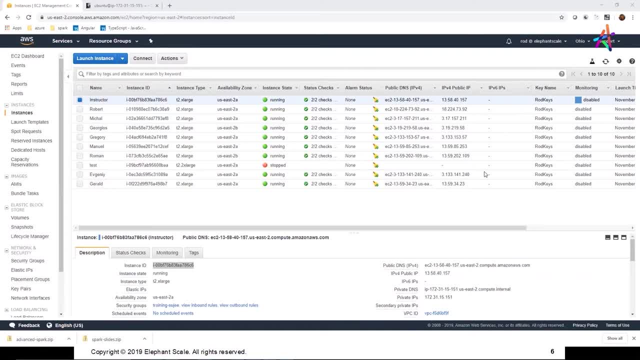 Yeah, okay, So I grabbed the wrong password. That's the wrong password actually. Okay, So you're. So if any other people run into the same issue, then the password is the one that goes after the URP and not before. 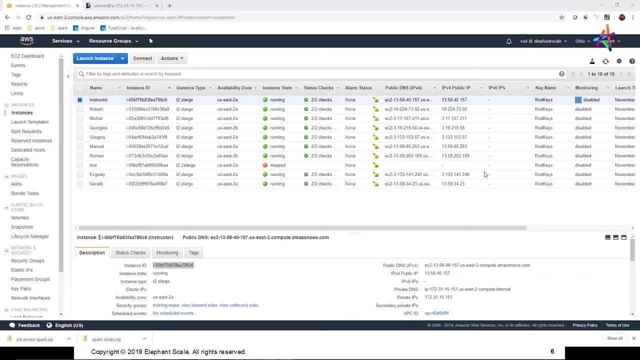 Right, Yeah, I should have probably done that a little bit differently. So SSH, the machine works for me as well. So, Robert, can you get onto the BNC BNC right? BNC via browser doesn't work, but SSH into the machine works for me. 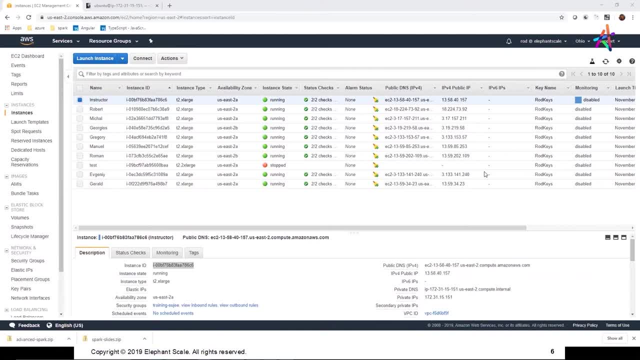 Okay, None of them works for me. Gerard, speaking same as Robert, Okay, well, I'm gonna have to ask Robert. Okay, Robert, Michael, how about you? I just want to get a little count here. So SSH works for me, but BNC also fails. 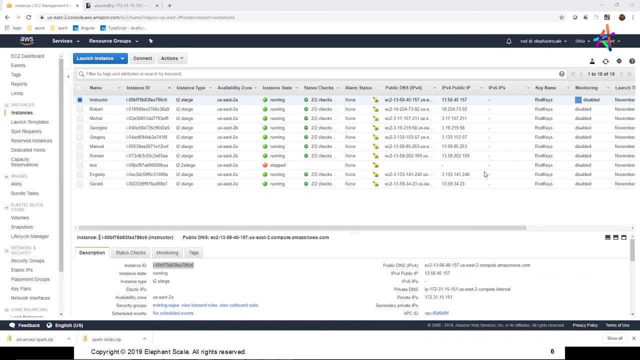 Okay, Gregorios, how about you? BNC works for me. It works for me. It works for me. Okay, how about BNC? The BNC, I haven't tried. Okay, Alright, Gregory, are you okay with SSH in? 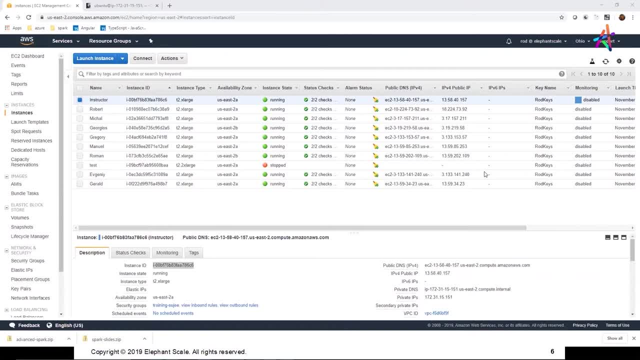 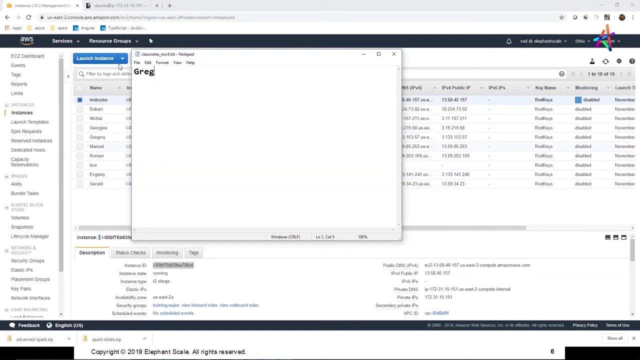 None of the works like terminal or web. Pardon, None of them works like either from the web or the terminal. Okay, Okay, so Gregory is to to restart. okay, okay, manuel, how about you? hi, corinne, just fine. unnecessary to know vnc though. so ssh is okay, vnc is no. is that what you? 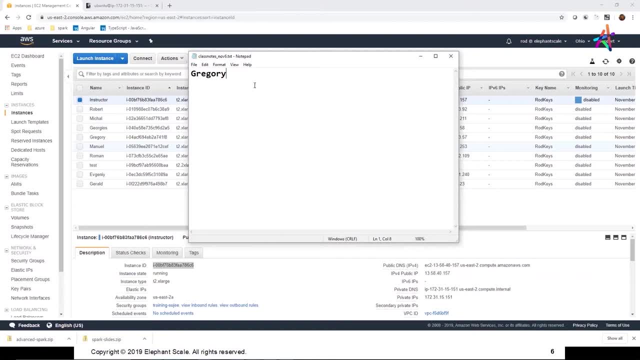 said: yes, okay, roman. uh, i think you already told me so, just remind me. so i connected through the normal ssh, so through the console and uh web. i didn't try. okay, all right, evicny, i've got yours already. sh client and gerald: uh, did you send me a message, gerald? what's your status? 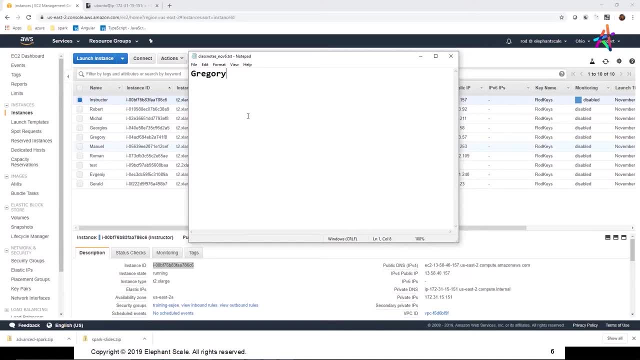 uh, vnc is also not working. okay, see, i was into, i went into a couple, i went into uh uh, mine, the instructor machine and robert machines last night and did vnc and it worked fine. so i'm not. i'm gonna have to figure out what's happened. 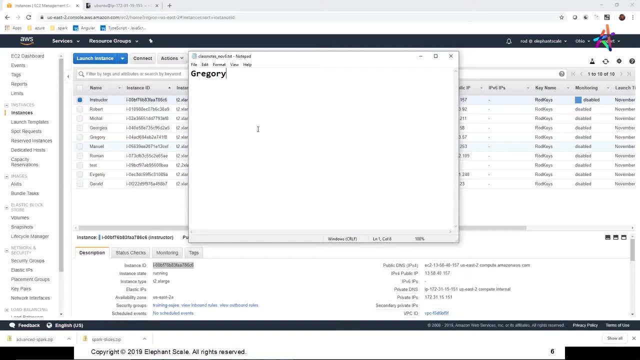 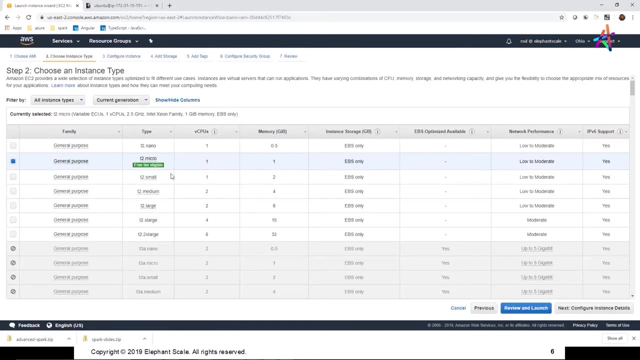 between now and then. so, uh, so, as it stands right now, gregory, you're unable to get into your machine at all. no, okay, so i will. so i'm going to spin up a new instance for you, gregory, okay, and we'll give you a shot on that. 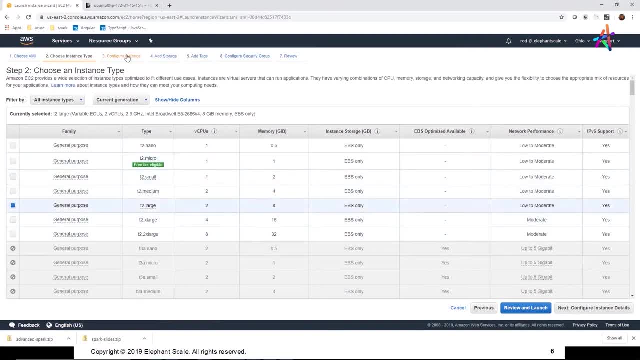 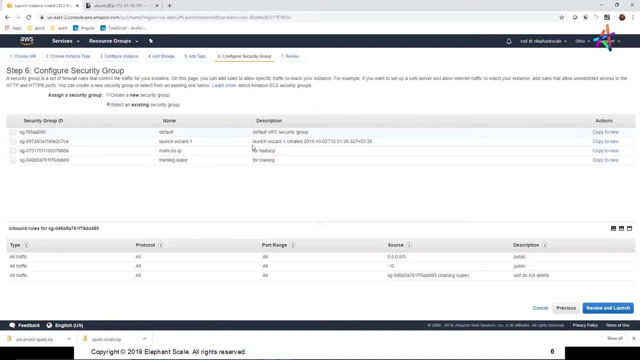 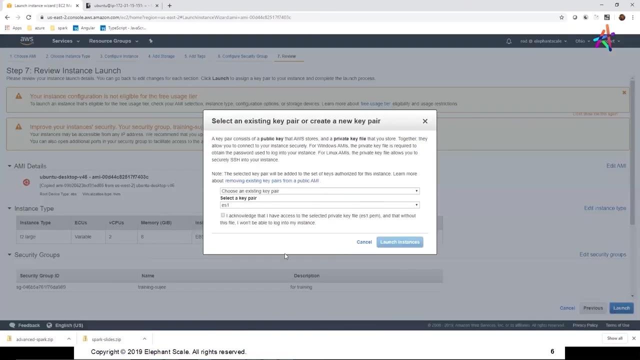 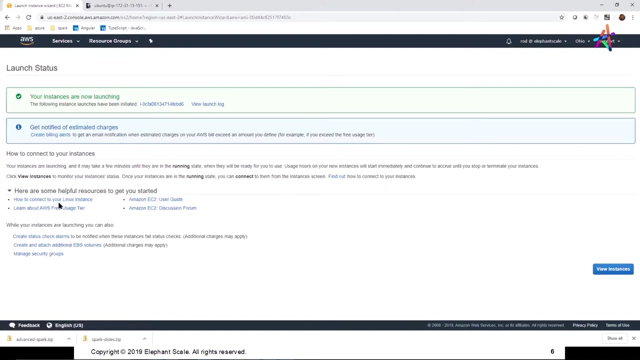 i'm not sure how to access vnc, because whenever i i type the ip address, i go to this web: login, ssh, ssh. so there's no option for me. i've logged into ssh, but i'm not able to click on the vnc anymore. i don't see this thing. okay, all right, um. 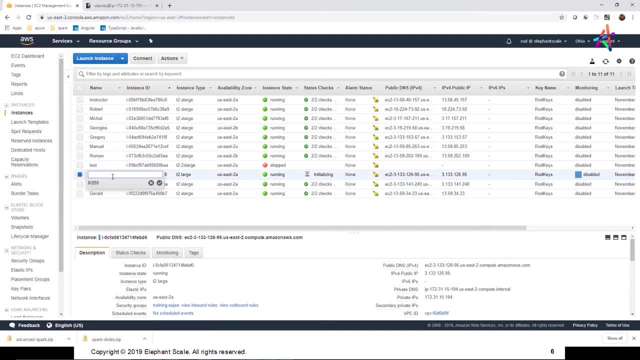 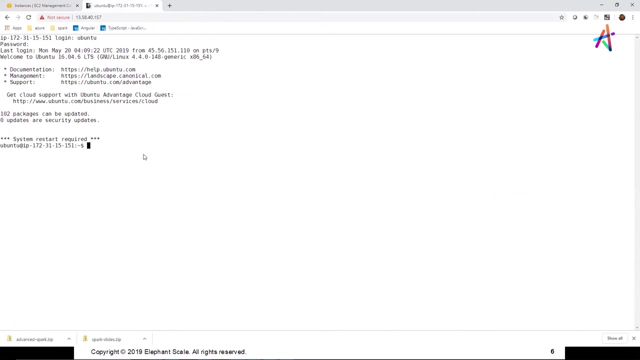 and i've tried also both two browsers and also the other browser is the same, all right, no, i cannot know from the from the web. i succeeded from the web, but not from. oh, i got it now from. it's okay. yeah, okay, but uh, i have access now from both web and uh terminal. you're talking about ssh? yeah, both. 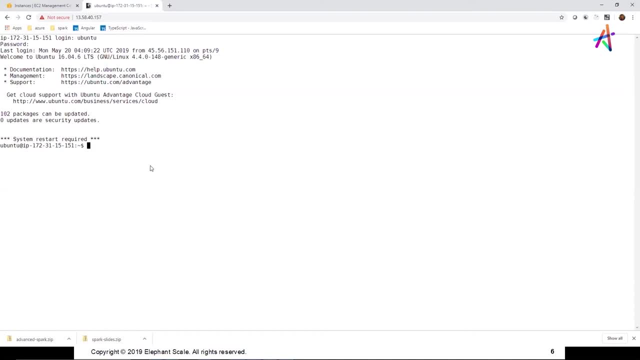 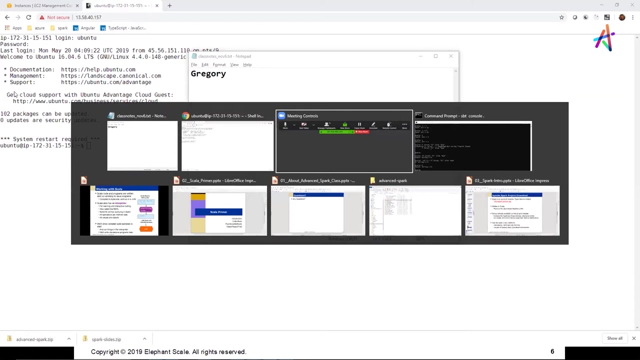 here, both from two. okay, i have a suspicion maybe, um, killing that process and starting it again might be the process. i'll i'll try and work on that after class, okay? well, at least we go, okay. so, gregory, i have spun up as another machine for you, but you can maybe kill it because the first one works. 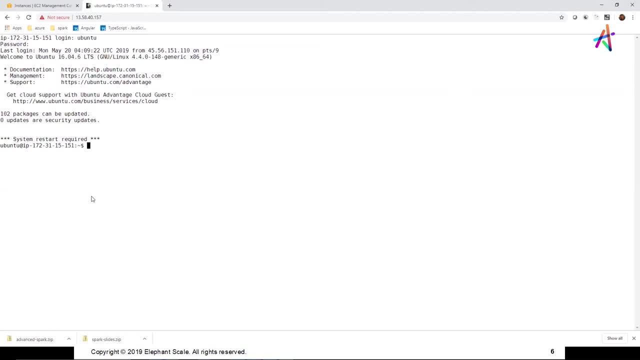 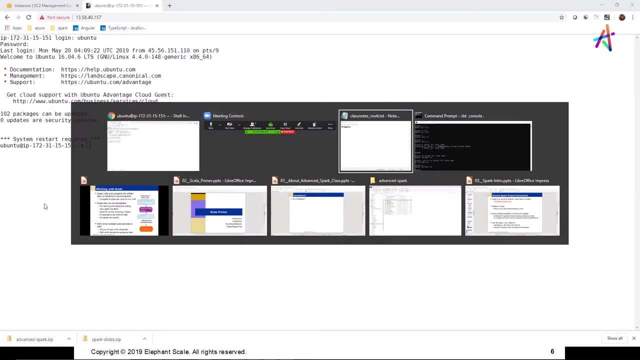 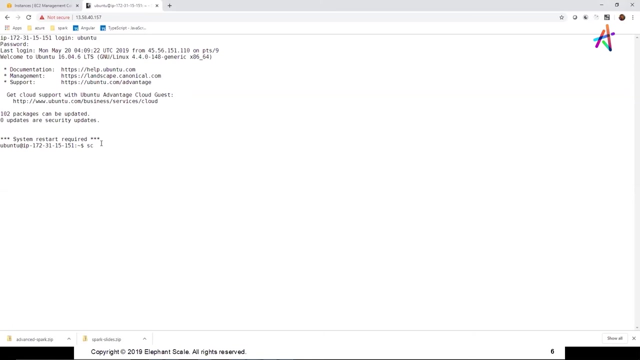 oh okay, all right. okay, well, all right. this is, this is the nightmare. you test everything the night before and then, when you actually get into class, it doesn't work. you know, okay, well, uh, at least, if you're in the terminal, uh, you are going to have access to uh, to uh, uh. 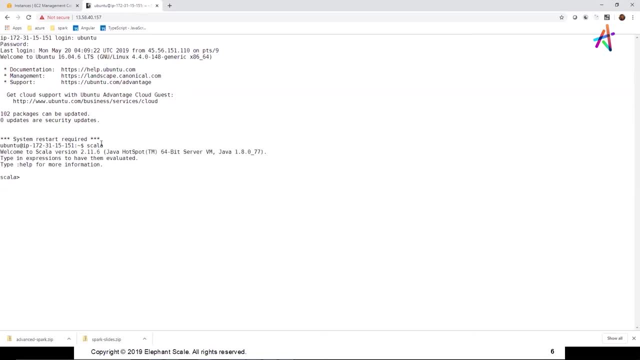 you should have access to a scala shell so that you can work um in the scala shell there for the for the various exercises. i do believe that there is also vi on the machine, so uh in, without the virtual desktop, we can at least uh do vi on there. 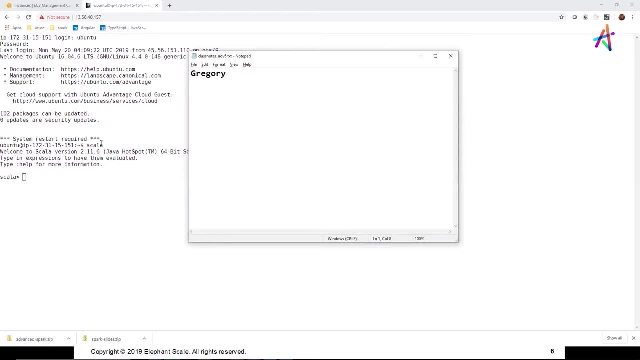 all right, and we'll try and resolve that issue after class and, if i have it, and when i come up with a fix- not if i will come up with a fix, and then we'll- we'll implement that tomorrow so that you guys can can work on the desktop the way you're supposed to. 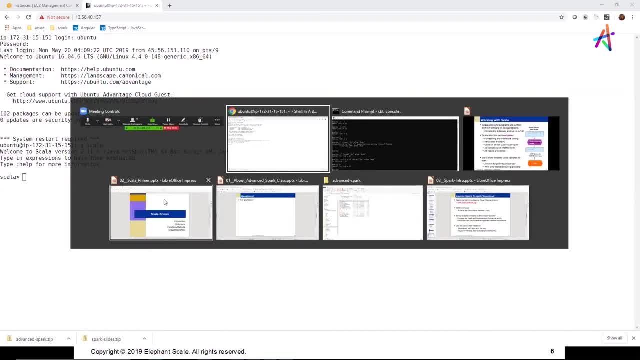 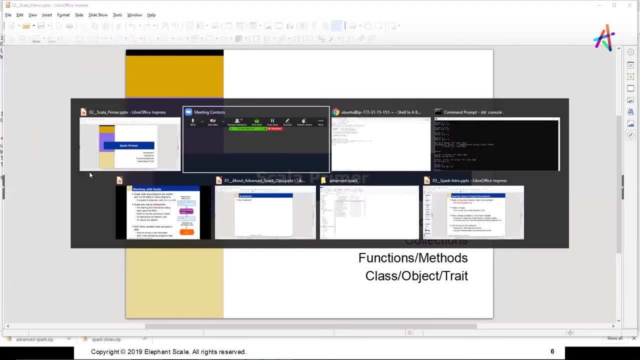 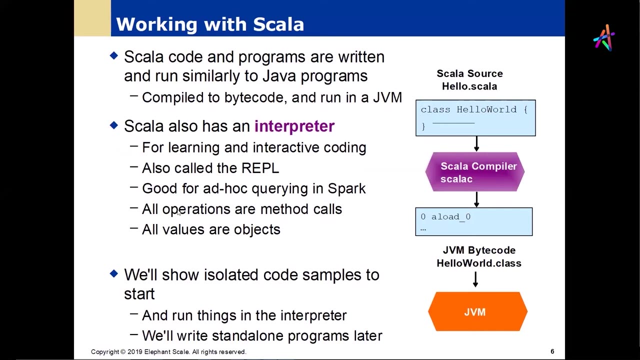 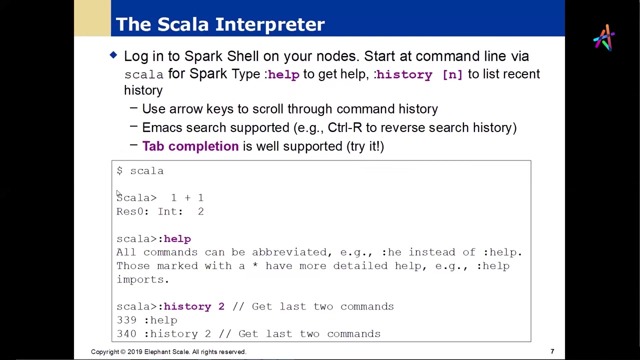 all right, um, so let's go back into scala, uh, and uh, pick this up again here and we'll work on this. here we go, okay. so, uh, let me see where we are here in time wise. we are 10, 30, okay, um, okay. so, uh, a couple of things about scala that are suggested here is: we're going to work on our 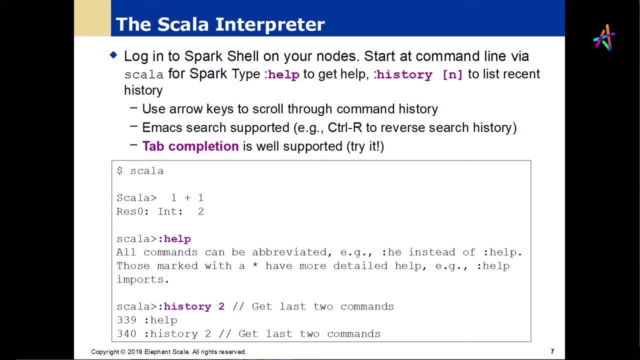 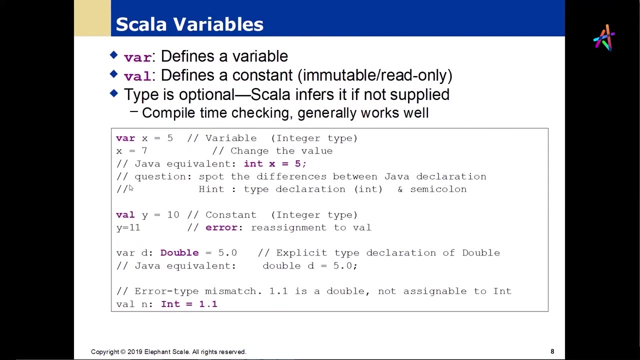 environment. uh, we can do a simple uh, a simple uh repl loop. have you already seen that uh colon help gives you commands? that uh, that uh help on the various commands. and you can also do a history using the, the history command, uh colon history. so there's some good stuff. uh, well, this is what we've mentioned before: um uh, var and val define. 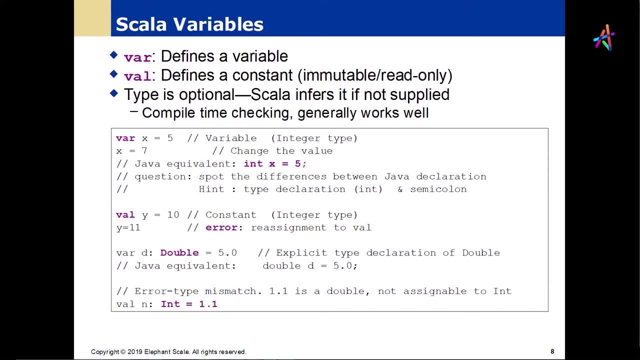 variables: uh, where var is a mutable variable and val is an immutable variable, uh scala uses type inferencing so that uh, the type of the variable is inferenced from the literal that's used to initialize it, uh and generally um, as with uh, with job uh. if you try to assign a value to a variable that's not typed uh correctly, then you're going. 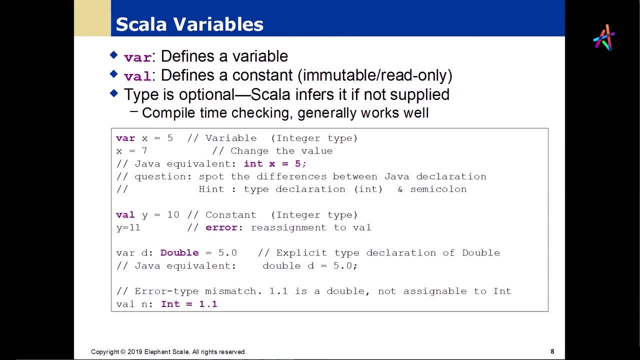 to wind up getting a mismatch. so the first couple of lines of code there, uh, are demonstrating a var and that in the val y equals x. and we have demonstrated that. the uh syntax on var d colon double uh gives an example of typing explicit type declarations. uh, if you are from the java, 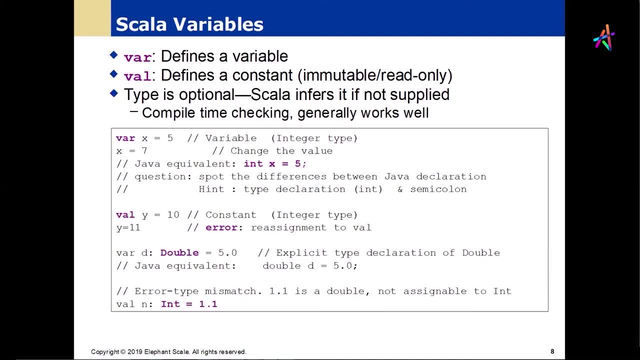 world. the thing to notice is that the scala types are capitalized, whereas the java types are not. the attempting to assign variables to the wrong types produces an error. this is important because typing is one of the the key things that spark uses in some of its commands i had mentioned. 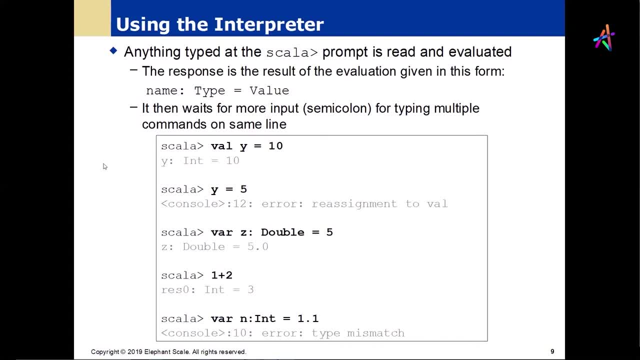 before that, everything that takes place in the scala environment is evaluated as an expression. everything is an expression, with the provisio that we're not doing something like from the java world or something that's not an expression. uh. so again, everything is a rewrite rule. so basically, we're assigning a? uh, a rewrite rule here for y and when we actually uh reference. 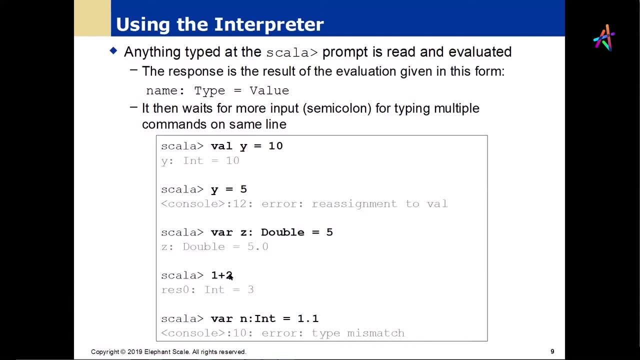 it, we get a rewrite rule, just like this is a rewrite rule. so this is rewriting: one plus one one, and then the plus two evaluates to a function call and that gives us three uh. so we uh again have uh, both uh, this immutability and the the use of of um, of strong typing. 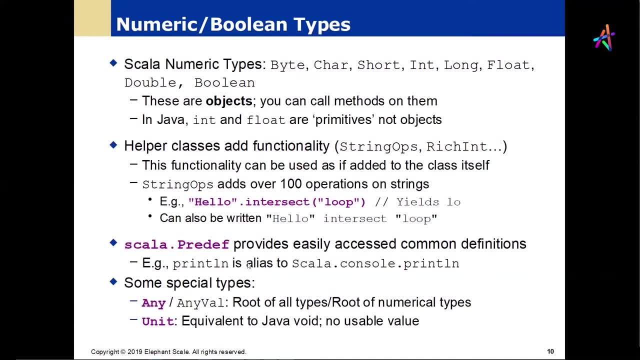 uh, the scala numeric types are byte, char, short, int, long. you know what you would generally expect. uh, they are um objects you can, you can call methods on. we see it'll be a little bit more illustrative that with that functional call on a three uh. so this gets back to the idea that 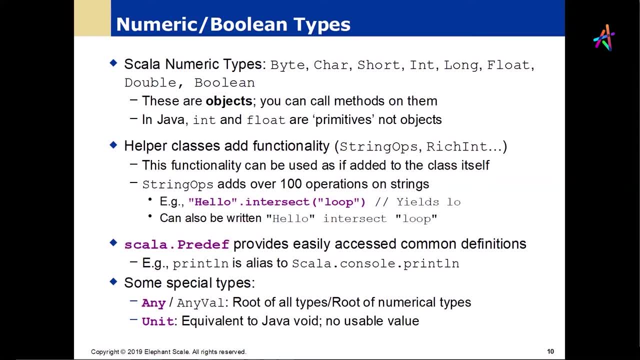 everything is an object, which is a little bit more of an object oriented. now, if you're in ruby, that is also a concept that's shared in ruby, uh, where everything is an object. so that's a very ruby type of way of approaching this. uh, so the notion of distinction between ints, between ints. 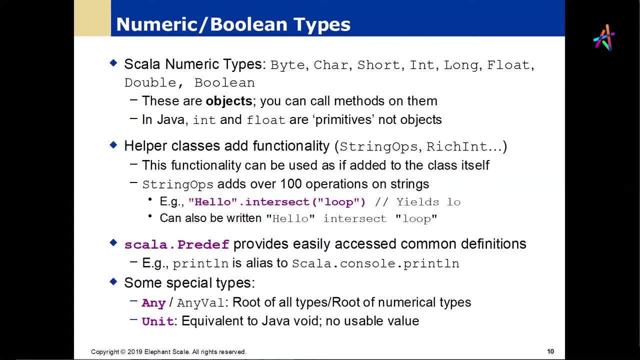 between primitive types and user defined types is really blurred in in uh scala, just like it's blurred in ruby. there are uh helper classes which give us a wide variety of operations that we could perform. so string ops, for example, gives all kinds of great operations like intersect. 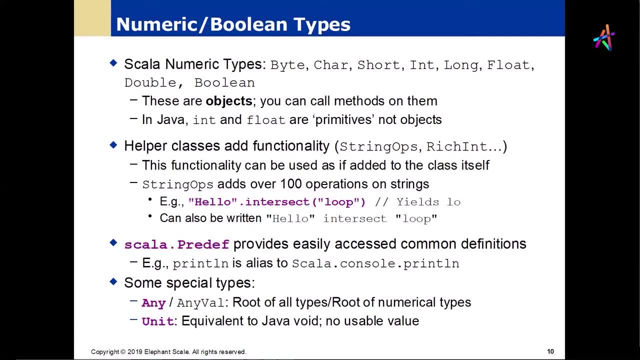 and a number of other operations. and again, you notice in the example, is that the string is an object, we can call the method right on it with the appropriate uh, with the appropriate arguments, uh, and if the second point, there is also again that syntactic sugar anytime the 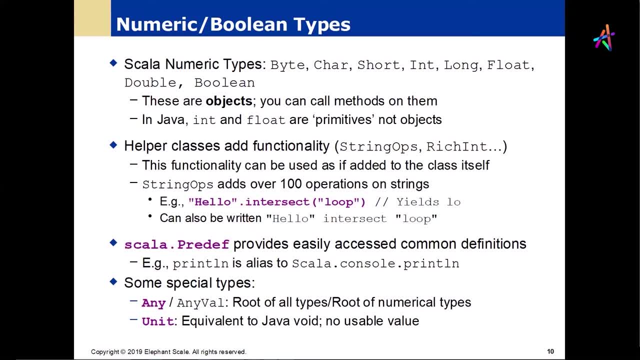 you have that kind of structure where you're calling an argument on or you're calling a method on an object with a with a parameter. you can rewrite that as an infix notation to get hello, intersect loop. uh, exactly the same way with an arithmetic operator. the distinction between 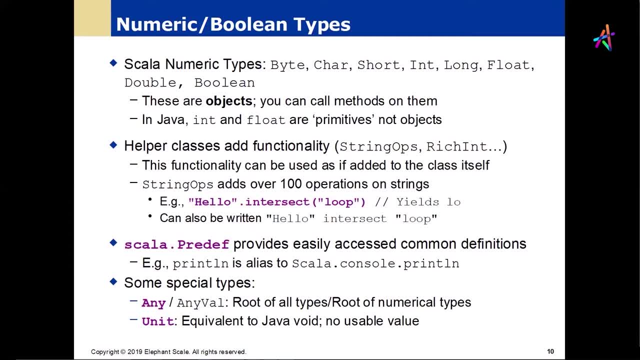 these kinds of of monadic operators and uh um on, or actually actually they're technically dyadic operators, i guess. but operators that take one argument can be easily rewritten as an infix type of notation on two arguments. that often produces some readable code, but it also can be a little bit confusing for. 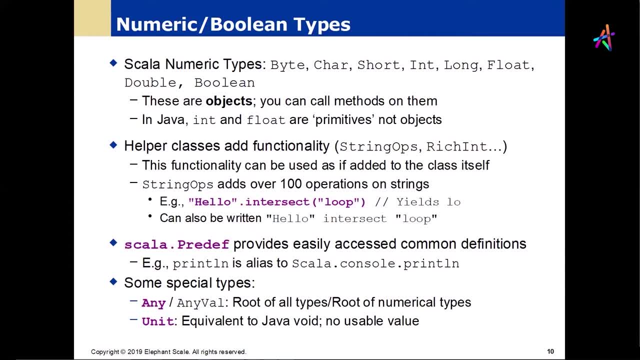 people who are not used to the fact that this notation takes place, that there's actually a method call going on in there, but again, that's consistent with the use of the operators in the language. uh, let me see there is a, um, a couple of of special types. uh, 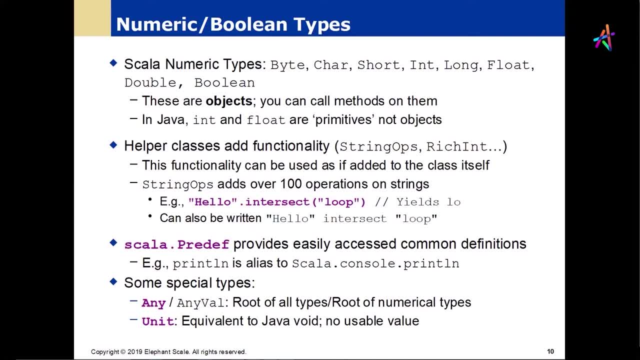 over the scale up. uh predef, uh gives a bunch of easily defined uh convenience functions and we have two very special types. one is the any, which is the root type of all numerical types. which is any val, uh, which is the numeric type- sorry, any is the root of all. 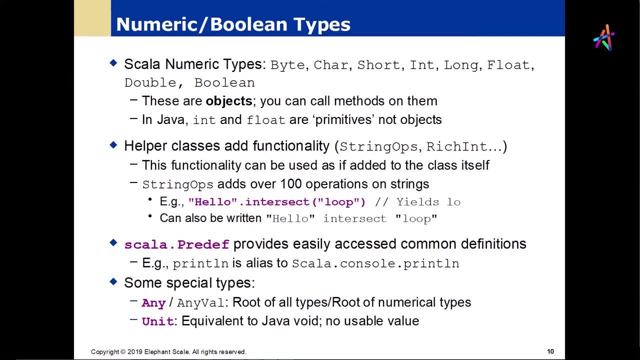 types. we'll have a little tree here at some point. uh, and what what scala does is always tries to go to the lowest point in a tree and doing inferencing, and if it can't, it goes up one level in the tree. to figure things out: unit is equivalent to void. it's more of a. 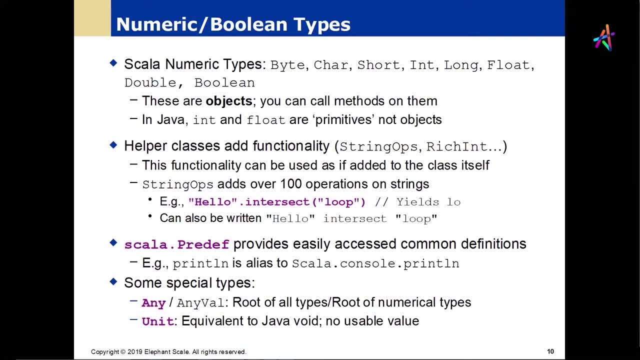 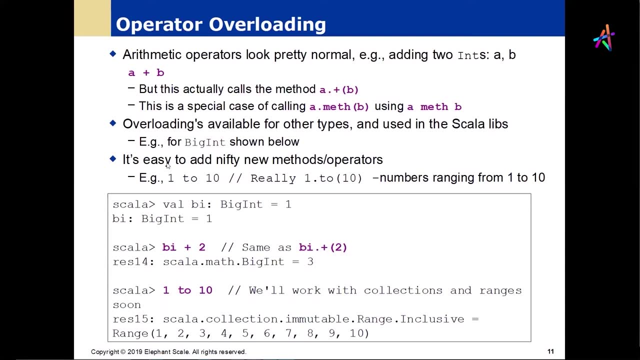 place marker in notation to let us see what's going on there, rather than any sort of actual computation or usable value. so there's that little thing um arithmetic operators. oh okay, actually it's in here too as well, and so this gets the uh, the uh, basically the idea of how we think. 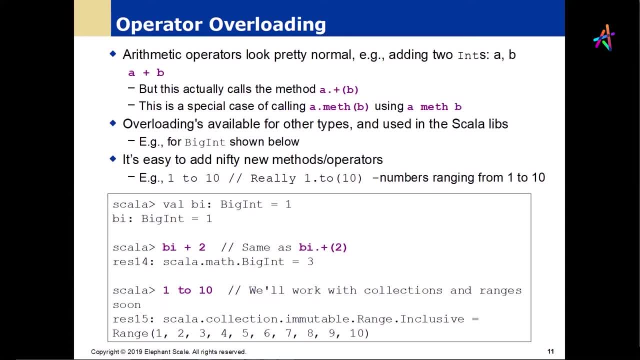 about the operators and what's actually going on under the hood, so we can actually add different kinds of operators. um and uh, we can. we can work with those a little bit later on. hold on here. i'm just making an adjustment, all right with you? just getting a little bit of feedback here. there we go, the uh, a couple of. 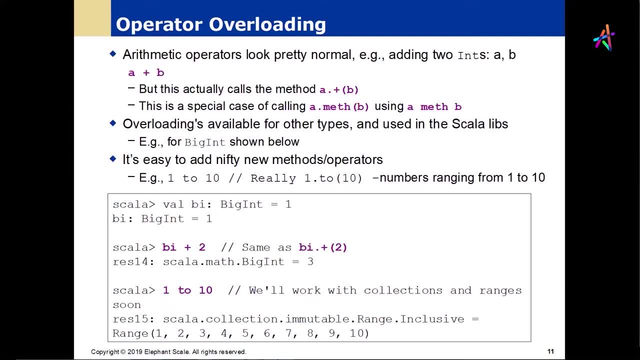 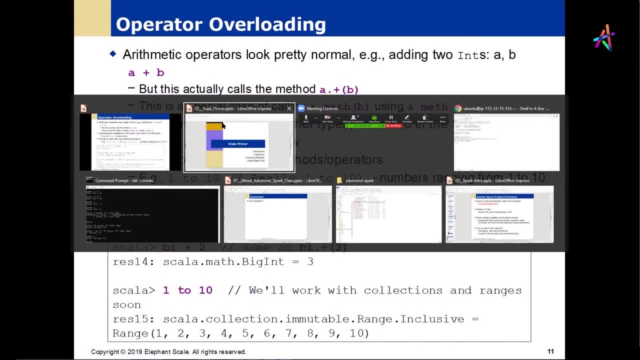 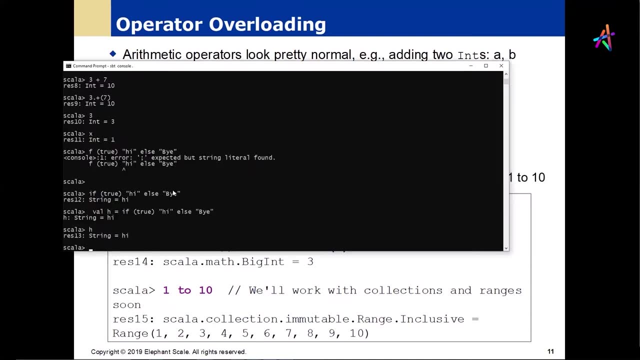 interesting things that can take place here. um so, for example, uh, we'll go back into my thing here and again- the notation, if you're not used to- or functioning- uh, hold on here. functional programming. this can be a bit odd at the beginning. uh. so, for example, a one to ten? uh, whoops. 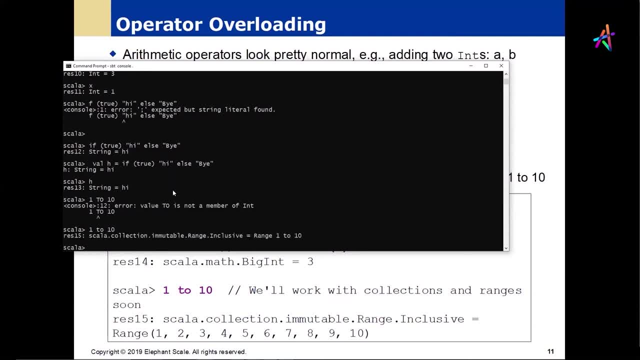 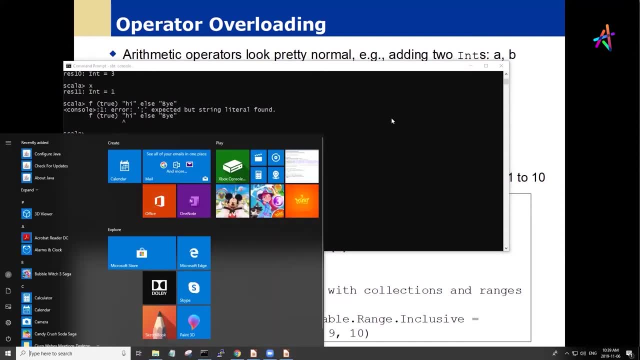 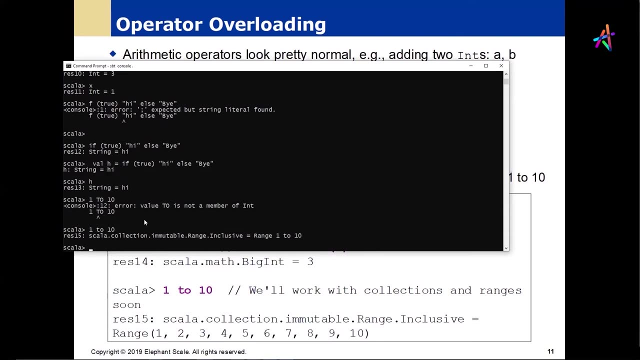 got a caps lock on there. uh, immutable range, um, okay. so what i'm actually doing here is i'm actually, um, uh, i'm actually uh, uh, creating an object. so i could actually say bar x equal to uh, one to ten, and i'm actually creating a range object. so now, if i actually list x, i can see that it's a range. 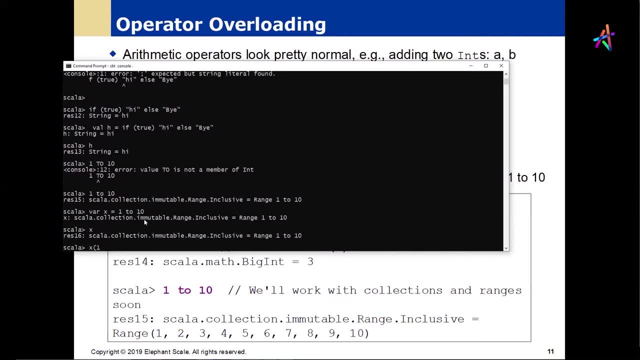 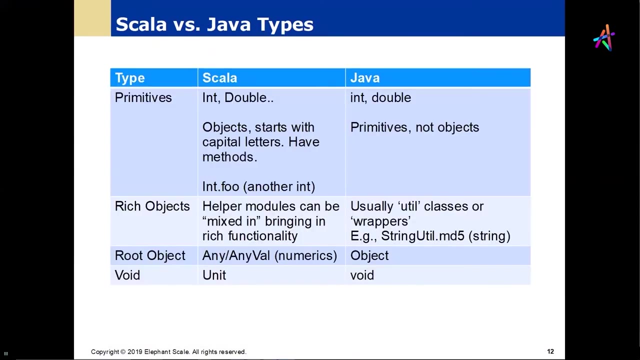 object and i can do things like think, actually get the, the second element out of x again. it's a rewrite rule um, in which we're actually uh, uh calling a method too, but we're using it in a particular infix notation. so, uh, in Scala that is an expression that can be evaluated, which we're actually seeing here. 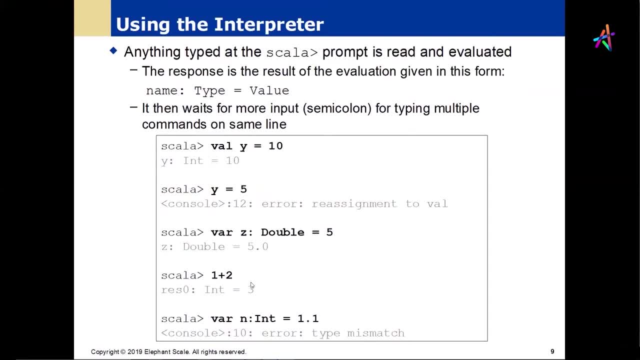 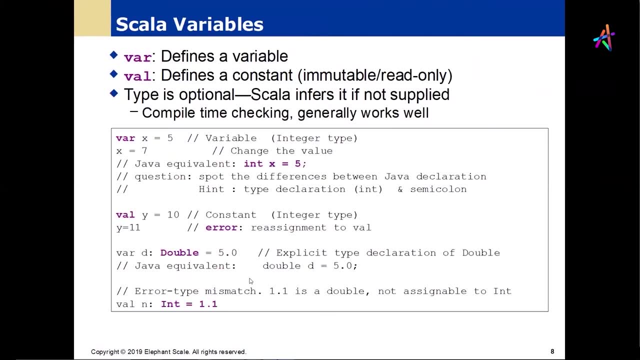 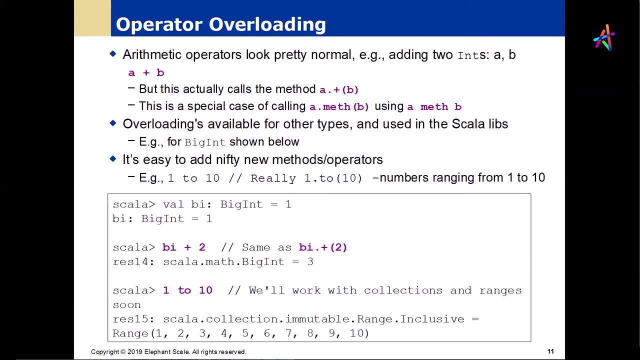 okay. so we'll see this kind of notation now and then, uh, let me see where are we here. we did, just did that one. there we go. yeah, we did there. okay, that's where we are. so the generally, the collections or ranges are going to be immutable and we're going to see that we often 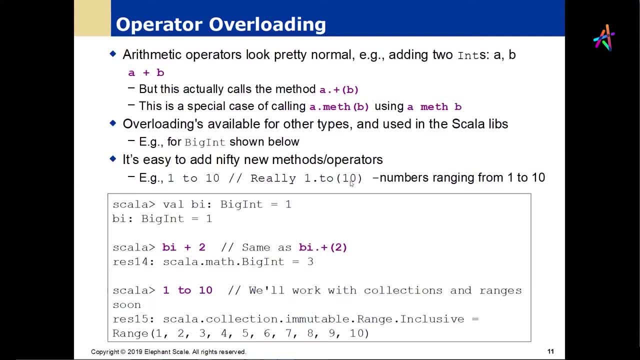 want to to change that. so here is our again. the expression that this really is is one dot on the operator two, which produces a, a collection, an immutable, an immutable collection. normally things are immutable by default in Scala, whereas if we want them to be mutable, we can. we can declare: 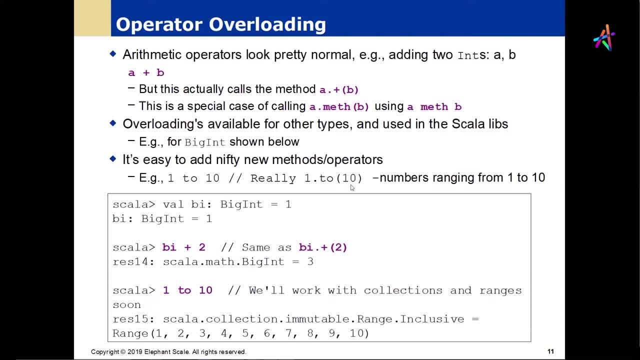 them to be mutable. so there's a couple of different things that are mutable, immutable. one is the rewrite rules for variables, which is the val var distinction, and the other one is whether or not the actual object itself can be mutated, in terms of, for example, a collection is going to 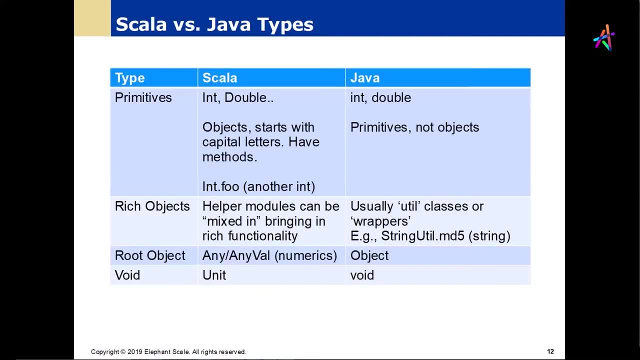 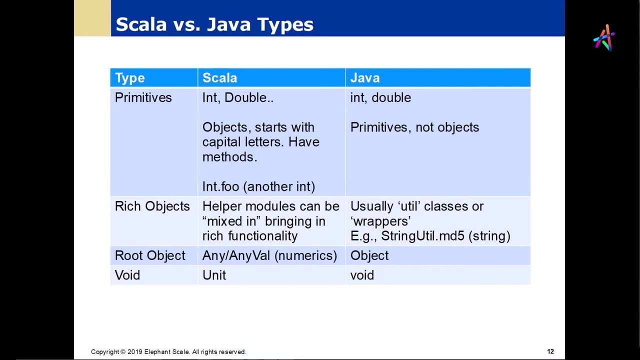 there. the difference here in Scala is that again we notice that the the literals are not, are not primitives, that distinction doesn't exist. they are objects. again, very ruby kind of way of looking at it. there is are a couple of implementations in the object-oriented oriented side of Scala which is a little bit different than the Java model. it actually goes. 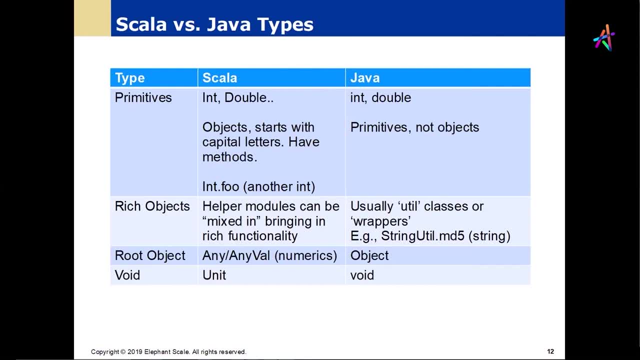 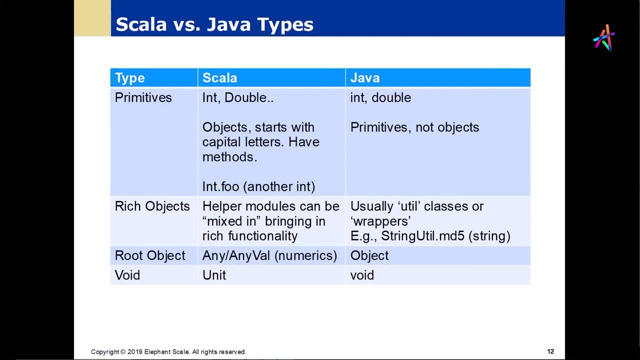 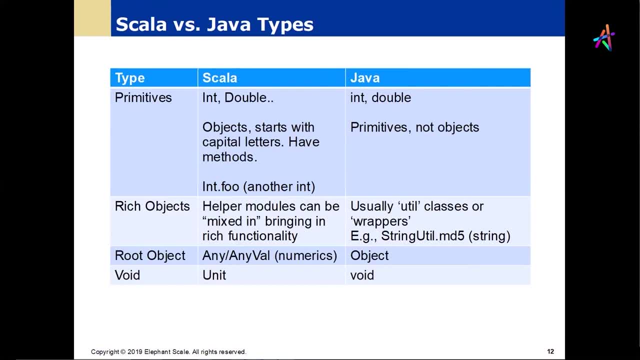 which are not necessarily representable by something as lean as a Java interface. so we want to use some kind of other mechanism to to do that, and this goes back to an old, old technique. there are again: the. any is equivalent to the object root class in in and in Java. 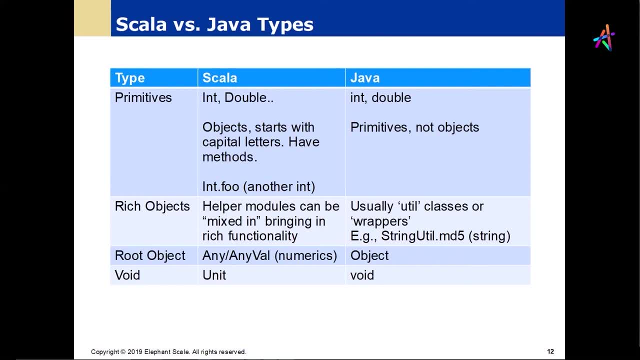 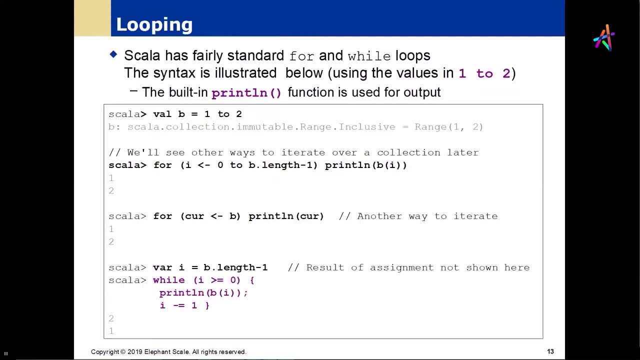 interesting little historical work. note back in one of the first object-oriented languages called zeta lisp. they didn't have classes, they had flavors, and the root object was a vanilla flavor, which was kind of interesting. that was the original work that came out of MIT AI labs, the 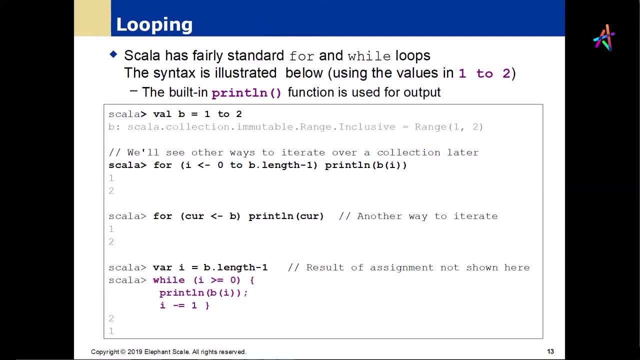 there's a standard syntax for for a while. the primary difference you have to keep in mind with these control structures is that they are expressions, they evaluate and they produce a result which can make things work very nicely. so if we take a look at the examples we get, B is 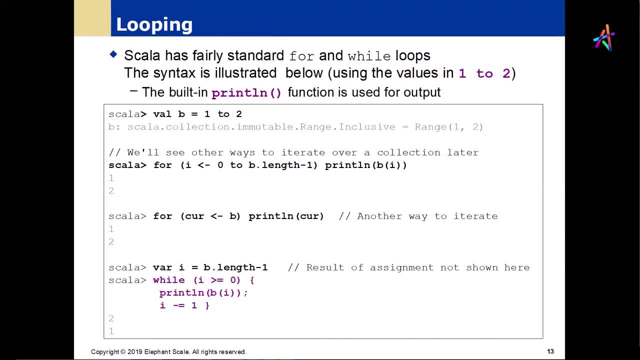 an immutable collection from one to two, which is essentially an ordered pair, and we can also now you iterate over a collection. so the syntax is in that second line, so we all an iterate over that. collection B: we use something that looks very similar using that reverse arrow, so we're basically 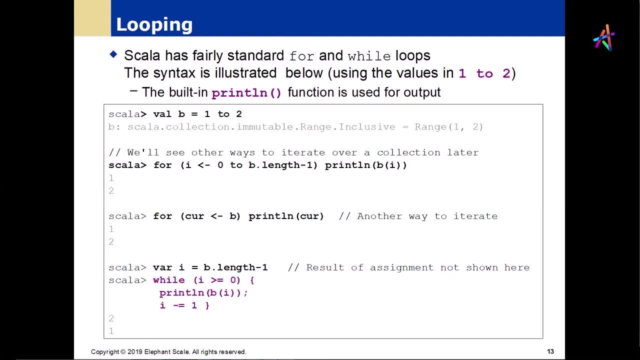 declaring a locally scoped variable, I, which is running from zero to the length of B minus one, and for every point, for every iteration on that loop, we're just printing a line out. the line so it is is similar to the normal kind of for loops, just a little bit of. 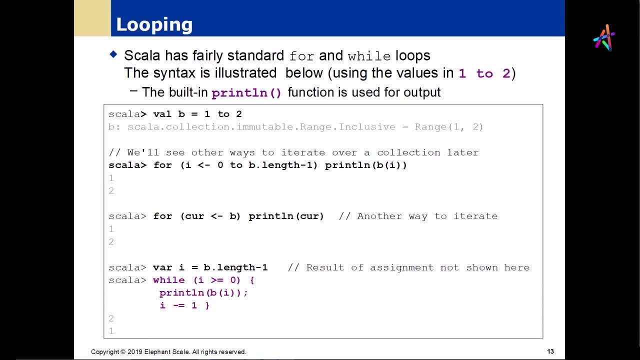 syntactic issues that we have to look at. and we can even do it shorter by implying the iteration loop. so in the second line, saying for current and then left assignment, arrow B, since we've got a for loop and since we've got an iterable object in B, the implication here is that we're going to 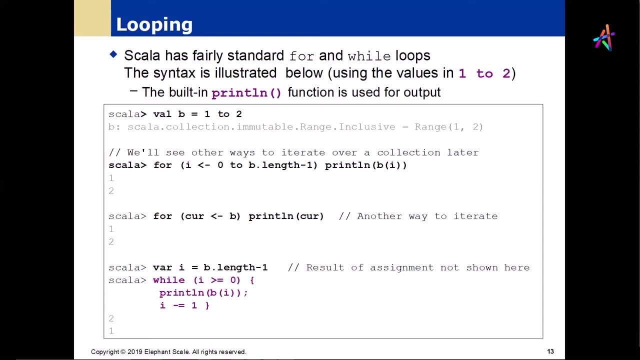 have an iterable object and in each iteration, the, the element, that's the, the current element, is going to be in, in, in, in cur, which makes the makes it a lot easier to work with. and then what we can do is is also assign the results of that for loop into an object we can. so we can assign the results of. 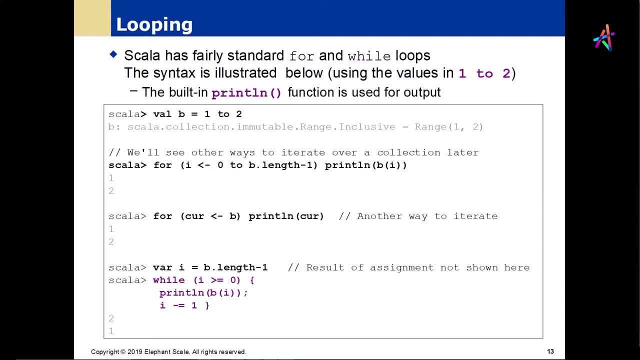 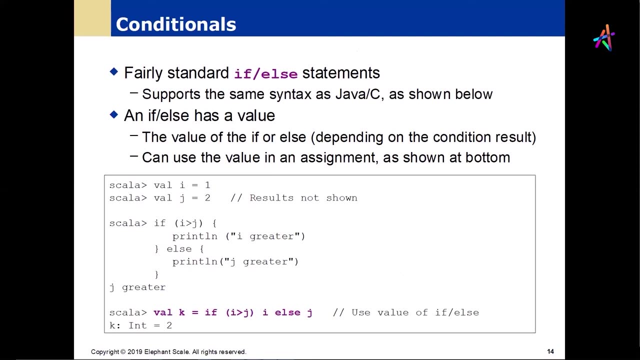 the various structures here. so we have the those kinds of of operations that we can, we can re-perform in looping and we'll. we'll take a look at Martin's book just to get they get a little bit richer sense of the syntax a little bit later. 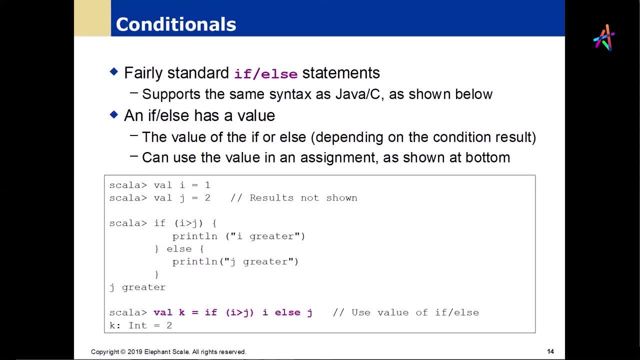 standard if-else L statements. we kind of looked at that earlier. I mentioned that a point is that this is again an expression that evaluates, so you can see it in a variety of different formats and we we tend to use very compact notations here, so that last line gives you the idea that again we have an expression is: 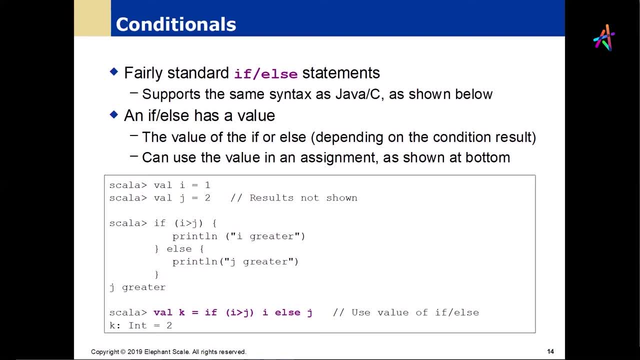 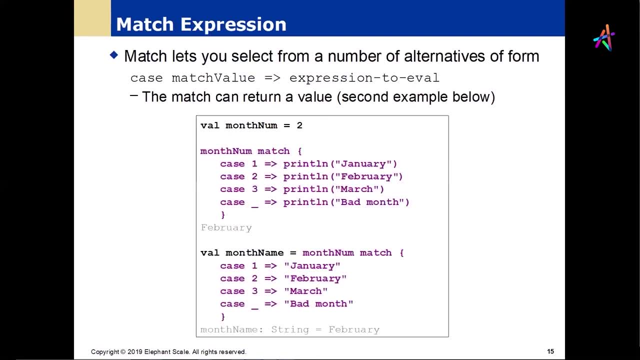 a rewrite rule instead of a, instead of just an thorough a flow of control like we have in Java. the thing that sometimes confusing for people is that the rules themselves are the rules themselves for how these things work in control. structures are a little bit different than Java, although the the control 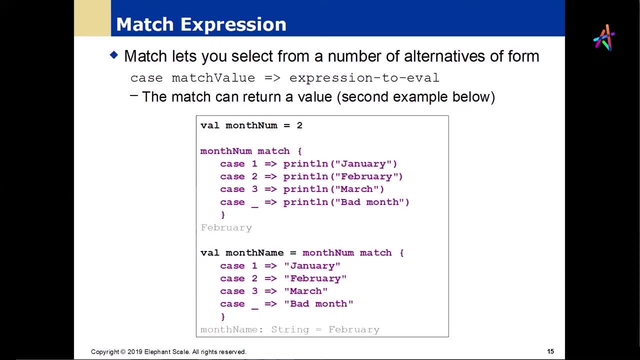 structures themselves look very much like Java. so you have to be careful, if you're new to Scala, to not think in terms of Java when you're looking at some of these similar foamy kinds of structures. The other structure which resembles, in sort of a generic sense, a switch case statement. 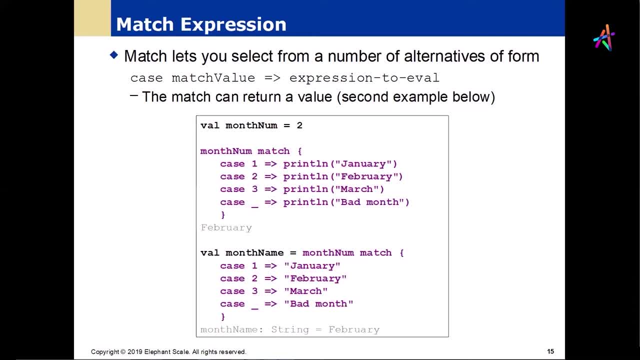 that we would find in a procedural language is a match, and we'll see the use of match a lot, which basically has a something to be matched and then a series of patterns that you can match from. So if we, for example, take a look at the first one we've got, the monthNum is a match. 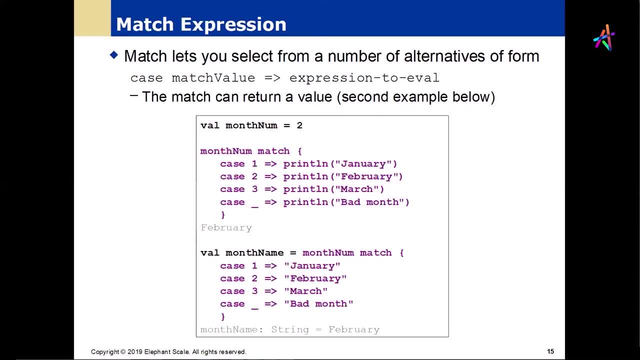 and we're going to match on the values there. So we're going to set cases1, case2, case equal to 2. three and we get the appropriate match. The underscore is sort of the else case on this one and we can now also assign the, the result, back to the as a variable. 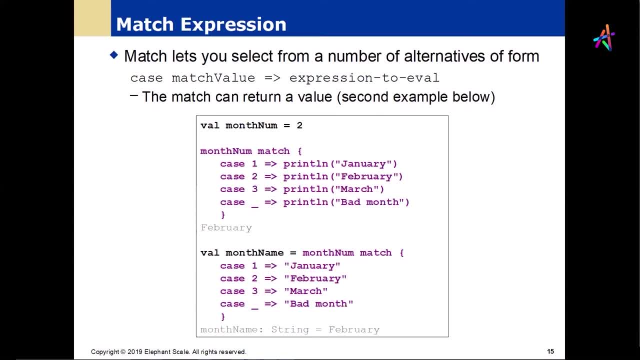 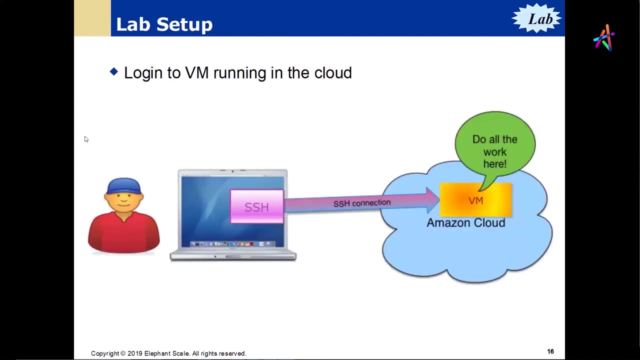 We'll take a look at that a little bit later on in more detail. I'm just going to mute one of these because I'm getting some strange feedback. No, I can't mute it, Okay, all right. All right, okay. so now we've basically got our. you guys have already done this part. 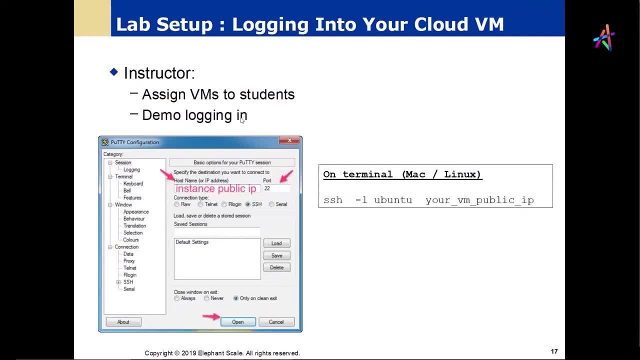 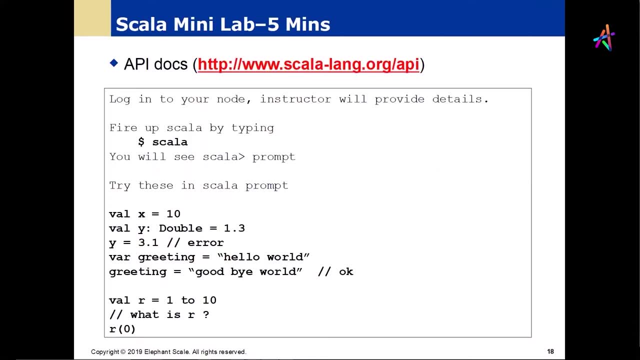 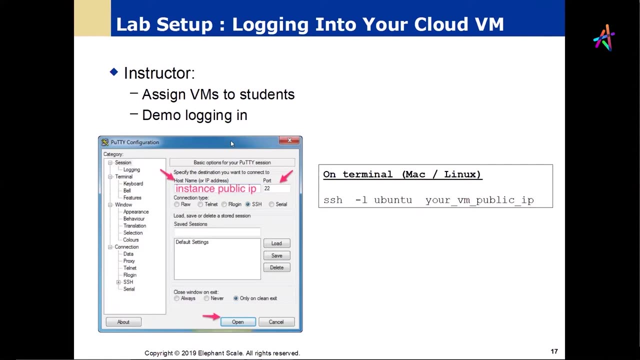 So we've got you logged into the cloud. here Everybody's logged in, At least on the terminal, And you can log into your node, And actually there's something different than what I was told to do. Sorry, this is Roman speaking. My SSH connection, for some reason, is now broken. 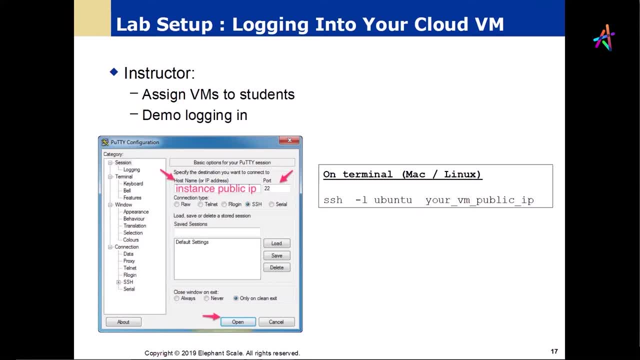 Can you please restart the machine or something? Which machine was that? Who was that that just made that request For to restart the machine? I think it was Roman, but it seems like Berlin is not responding anymore. Maybe they don't have internet. 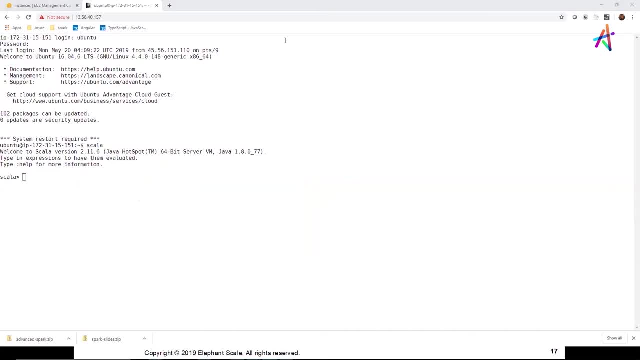 Yeah, so Mike and me are not in Berlin, and that's sometimes the case that Berlin loses internet, Really Okay, Yeah, that's the downside of Berlin. So good food but no internet. Okay, so Berlin, it might be dead. 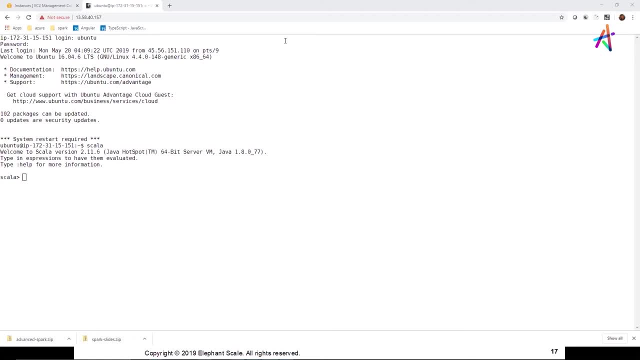 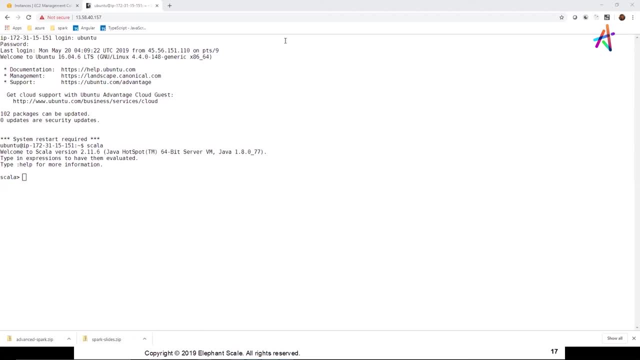 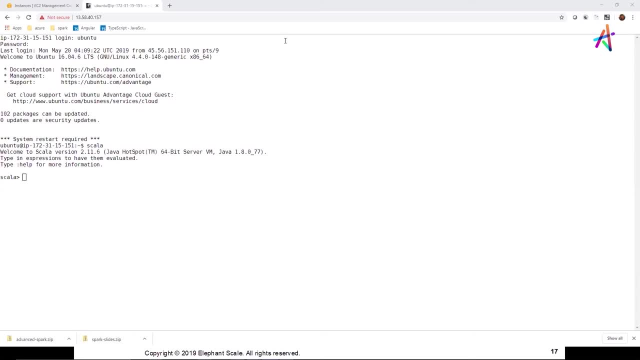 So I just got the information that on the floor there sitting the virus lawn just went very, very slow, So I guess that's causing the issues. Okay, Okay, Okay, Okay, We'll give them a little bit of time to get straightened out there and I'll wait until. 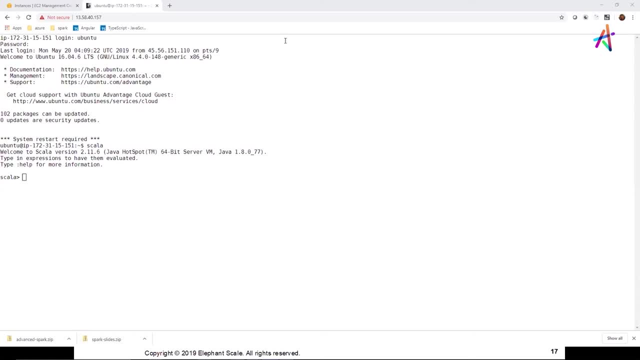 I get a go ahead from them that they're actually up and running. Is that just with you guys, your Berlin office, or is that an issue that happens a lot in Berlin itself, as the city with wonky internet connections? The joke was that Berlin doesn't really do internet well as a city. 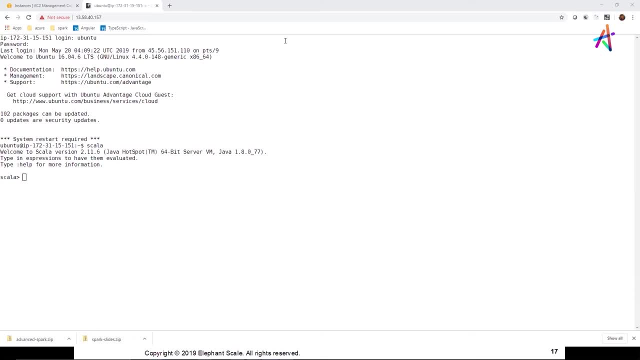 Okay, Okay, Okay. We moved from the previous office location to the new office location. We supposedly have a different cable there, obviously, but also in the previous location we had internet issues. Yeah, And that was fiber, mind you. 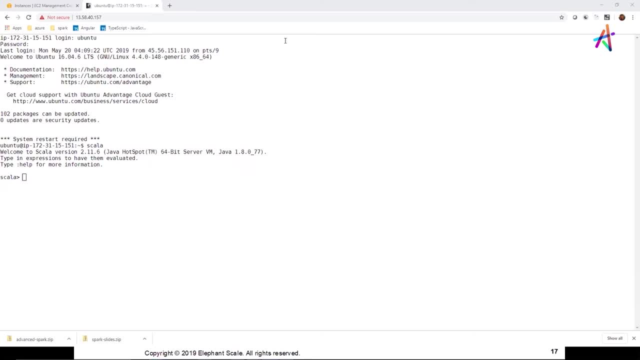 Okay, Oh, people are coming back now and going away. Yeah, I'm not sure how they were solved. Yeah, Yeah, I'm not sure how they were solved, because in the room they are they don't have capers. Well, well, you know I'm not going anywhere, so I mean, I don't want to, you know, like, 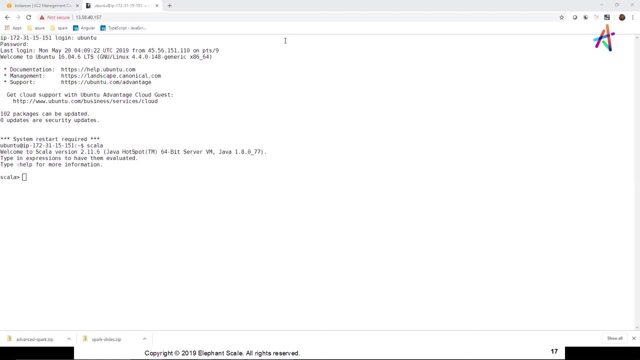 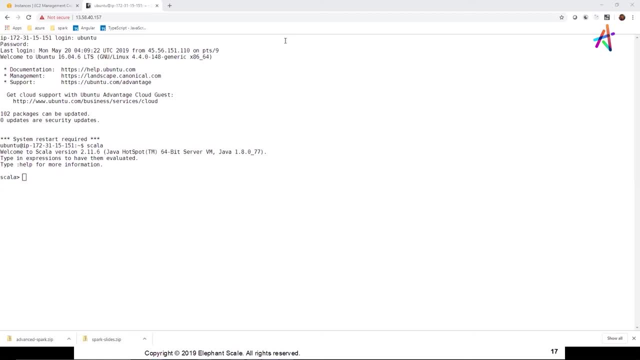 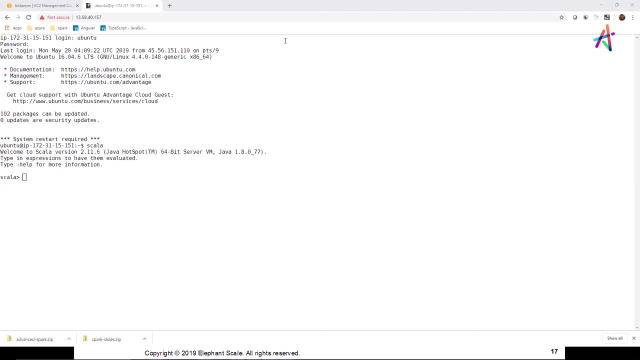 Um, so until now it's quite basic and yeah, I think, except for Roman, everybody should already know these few introduction. okay steps, at least for Scala, for Spark, I'm not sure. for Spark maybe it's good to start from scratch, but for Scala I think we move on quicker. yeah, if we get. 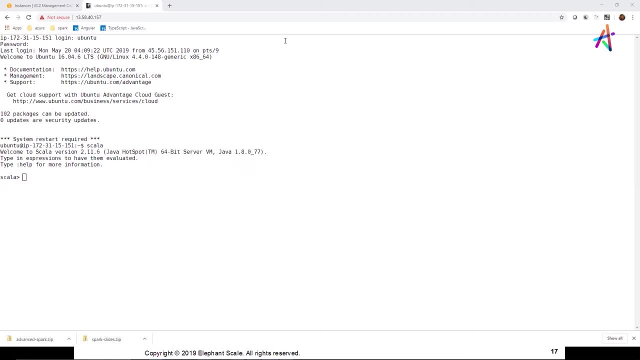 internet. if we get internet, sure all right. well, that's good to know, because it's hard, it's hard to judge coming into a class like this, because often people say, oh yeah, we're, we're comfortable, Scala, we're comfortable with this. when you get in there, it's kind of like no, you're not. 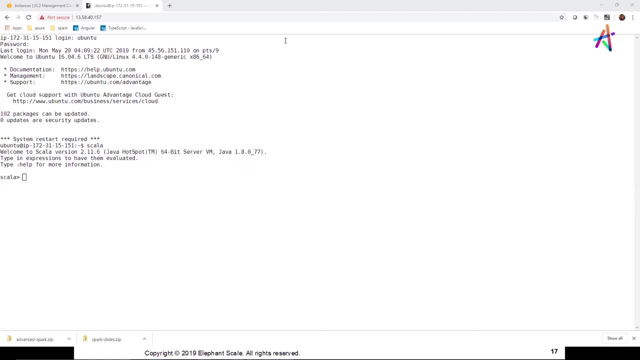 um, so we have to kind of: yeah, so that's true. of course, whenever you have um training with multiple people, you don't really know what to expect. so, yeah, I'm training another class in the evenings. it's supposed to be for programmers, and I have three people who never programmed in. 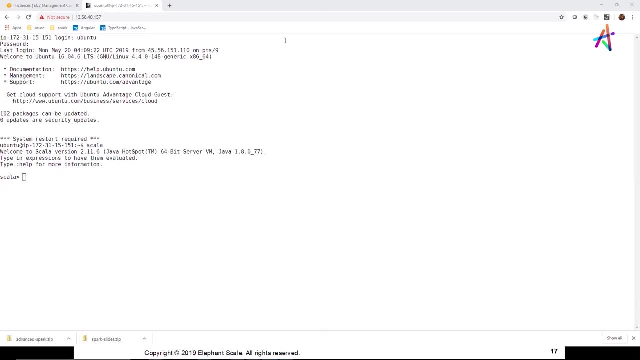 a class. so I'm kind of like, oh gosh, we are terribly sorry, but we're back. what are you sorry that you're back you? yeah, well, I. I hear the internet went out all over southern Europe, so you know you guys did something wrong there. all right, looks like people are are slowly repopulating the environment. 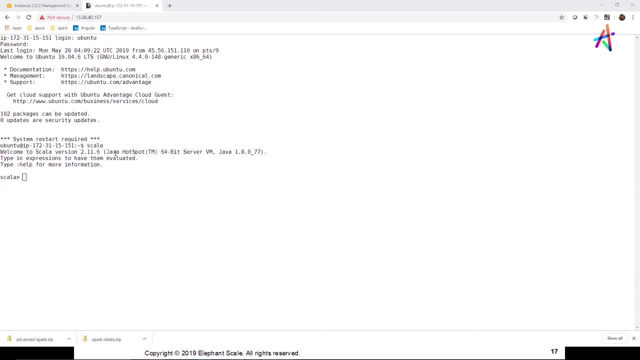 I think I was. I'm going to you, let's do this again. no, cool, all right, are we? are we missing anybody? uh, no, I just uh. I don't mean, I don't the password, I don't think it's one. I managed to just like share again. 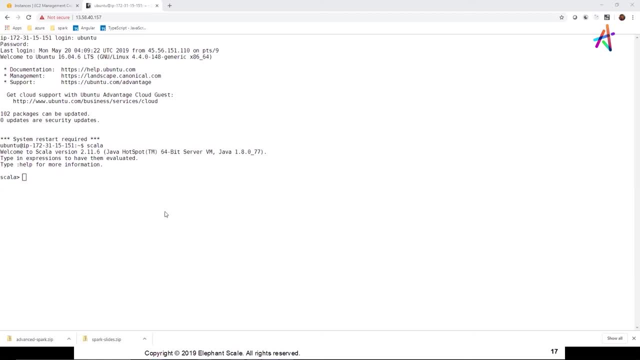 all of them, I think copy paste. sorry, because the chat, of course the chat history, is gone, all right, well, we'll do this information to our private chat everybody, okay? well, we'll redo that part right now. okay, but this time we'll we'll try and I'll try and chat it out to you individually. 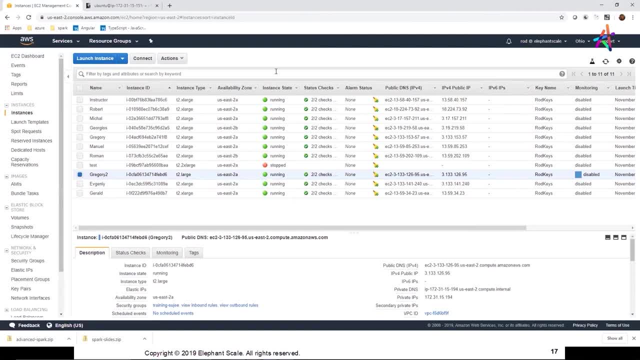 and then you guys can cut and paste it. um, let me see. uh, Robert, do you still have your information? yes, I already copy pasted all the IPs and passwords into our private chat we have in the company, so everybody should have access to that. all right, if anybody does needed their information. 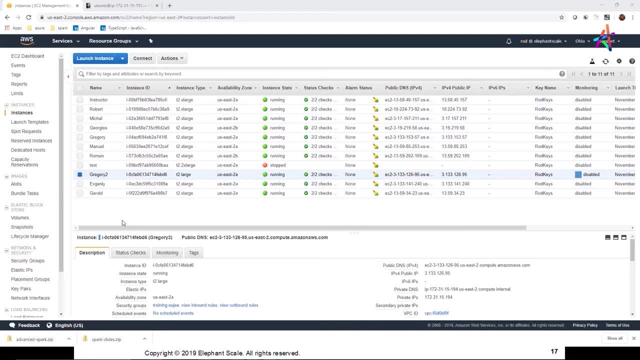 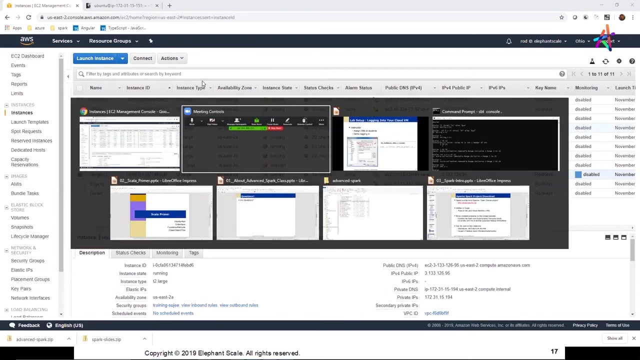 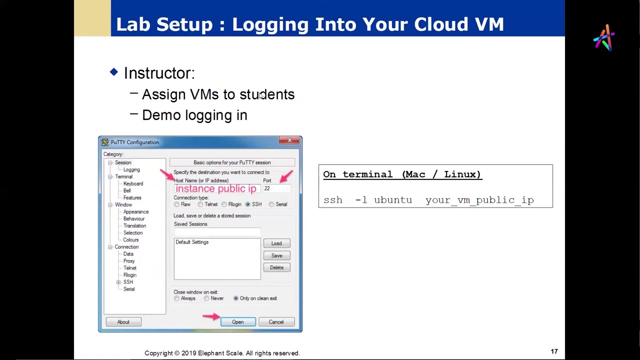 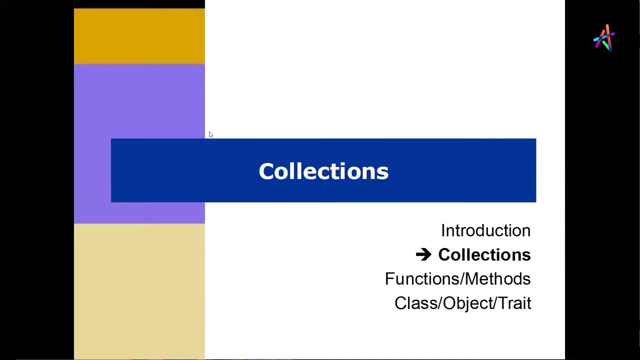 so these are anonymized. okay, just pick any. just don't kill my jobs, all right, okay, yeah, well then, are you fine? now can we continue? yes, I think so, okay, good, all right, okay, so we've got that done, and what we'll do is just quickly, uh. 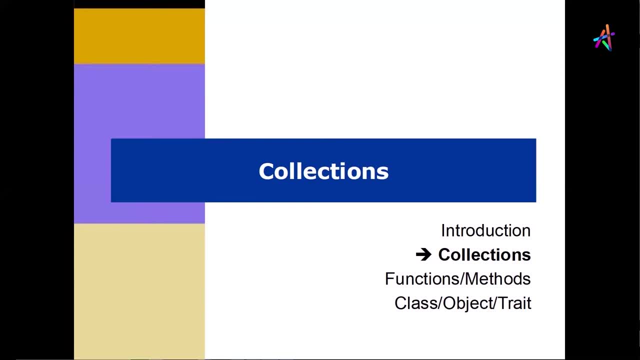 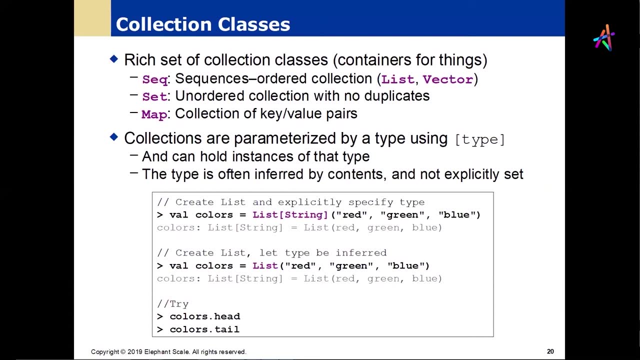 do a quick review of functions and other things. collections: Again, this might be a little bit basic, but just on the off chance we'll just so. we'll just go through this very quickly If anybody has any particular points they want to explore. 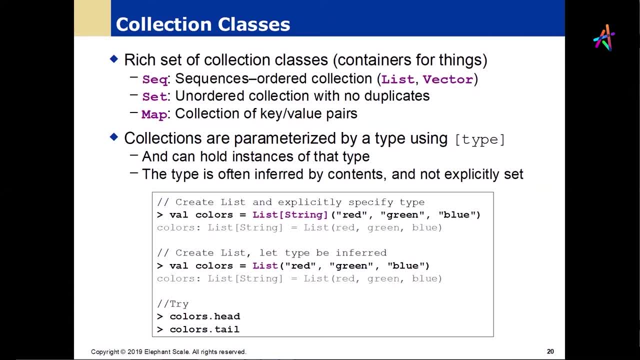 then please raise the issue, But I will assume that this is more of a review now for you guys than anything else. So, collection, classes, sequences, basically the three standard types that we find- sequences, sets and maps- We parameterize them with a type. if we are parameterizing them. 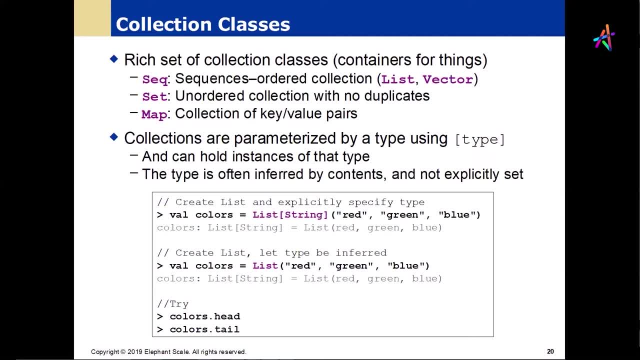 And we have a variety of different operations on this. The one thing I will mention as an addition is that these lists are structurally quite different than arrays, in that they represent more of the kinds of lists- lists- that you see in very highly recursive languages. 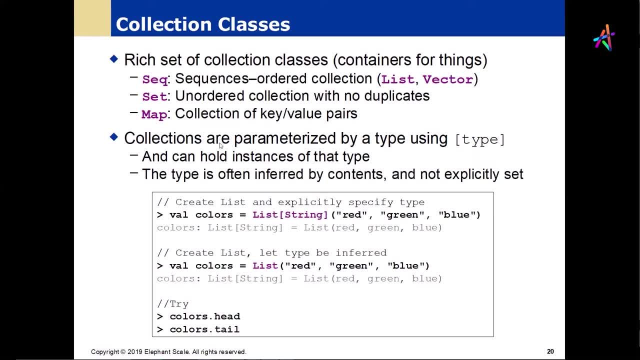 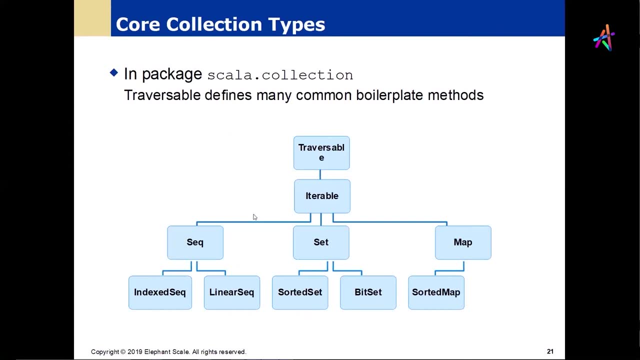 So these are actually more like a linked list as opposed to something else. So the various kinds of head tail operations are very much like the cons and catter operations that we see in other programming languages. They operate under the hood the same way. The collections are basically traversable and they 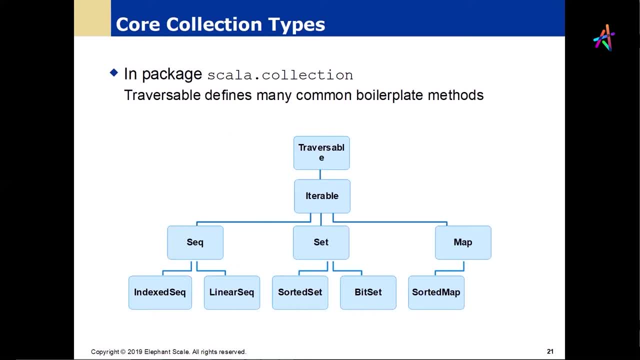 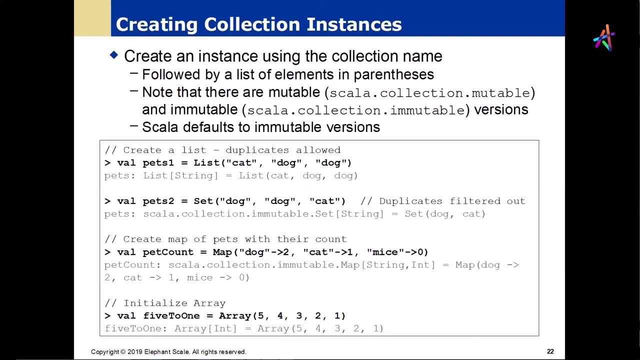 have the various categories. Again, you'll be able to explore this on your own if it's not completely familiar to you. but, again, similar standard boilerplate methodologies. We can create collections, instances, using a collection name with a, so there's an example there of creating the various kinds of instances. 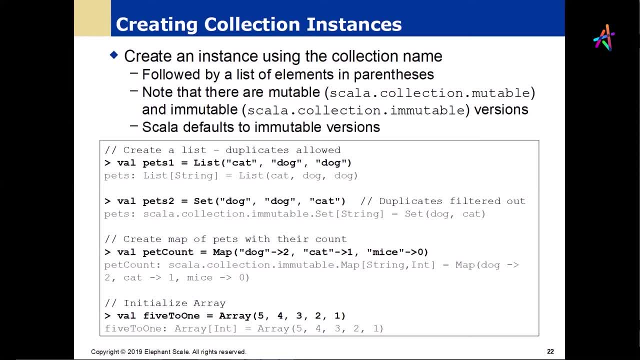 Arrays are different in the sense that they store the data somewhat differently And there's an underlying a difference in how they're they're structured. We won't get into the details of that in this class, but just to notice that there are some underlying structural differences. 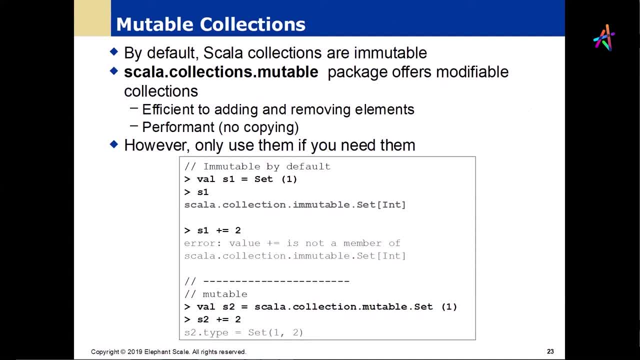 Collections are immutable by by definition, but we can use, so the. we have to have mutable collections which allow us to add and remove elements. And but again, if we want to keep in the, in the principle, in the, in the, in the spirit of functional, 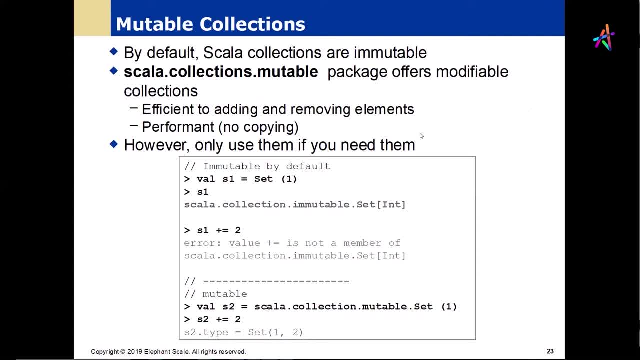 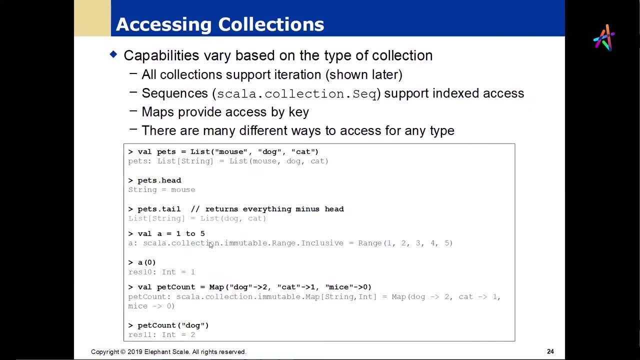 programming. we don't generally tend to use those unless we absolutely have to. So there's the. there's the example of mutable, immutable by mutable and immutable, different kinds of capabilities, naturally on the different kinds of collections. So the examples given there just show this: standard kinds of lists with a head. 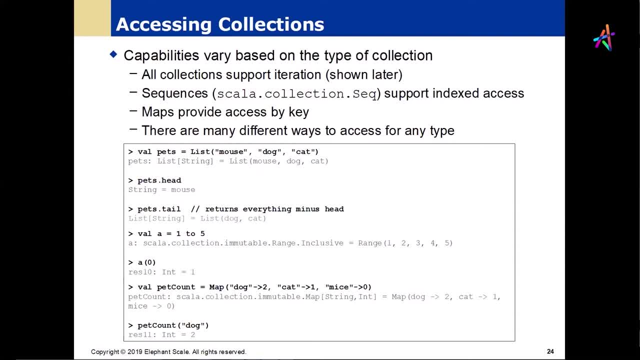 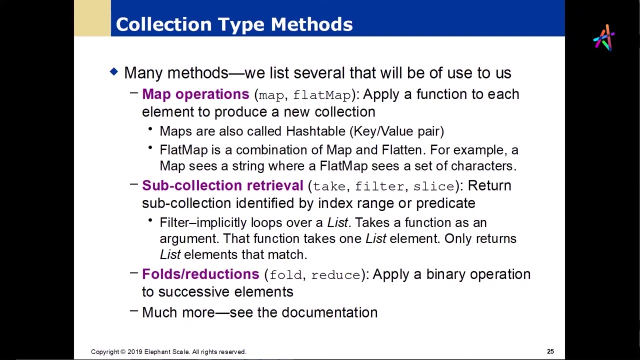 and tail operation, a range operation, which I demonstrated earlier, a map operation which allows you to go and access by key as well. So very standard operations, nothing that you'd expect that would particularly difference. The functional operations that we have are similar to what we find in other. 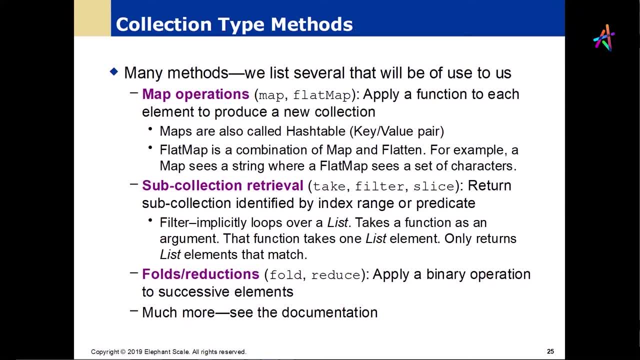 functional programming languages. map operations which basically take a collection map, a function to it, produce a a another map or another. collection map generally tends to do a one-to-one operation and flat map does a many to many operations in some sense. 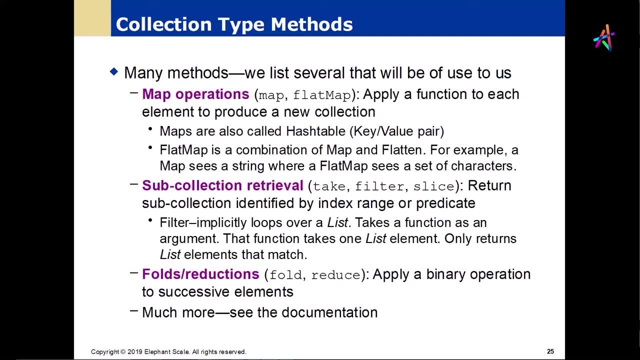 So we can. we can do a variety of different operations with those, And we'll see those particular as we get more into, as more as we get into the, the, the spark portion of the course, Sub retrieval collections are exactly what they sound like. Take filter slice. 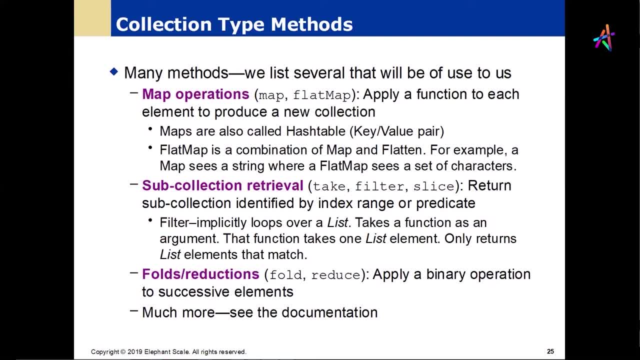 we get some kind of a predicate for doing a extraction of some subset. So the comment here is kind of good. filter implicitly loops over a list and takes a function as an argument. So it it gets that, it it creates an interesting cognitive view of it. folds and reduce, apply operations. 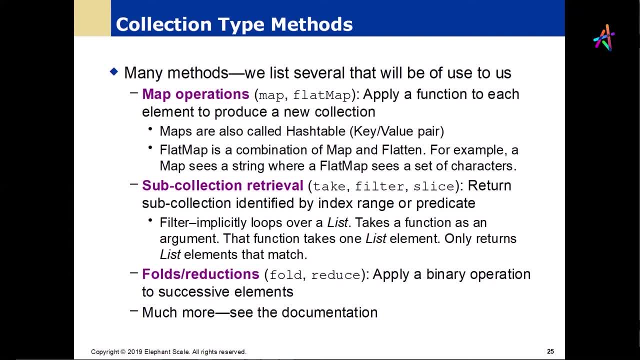 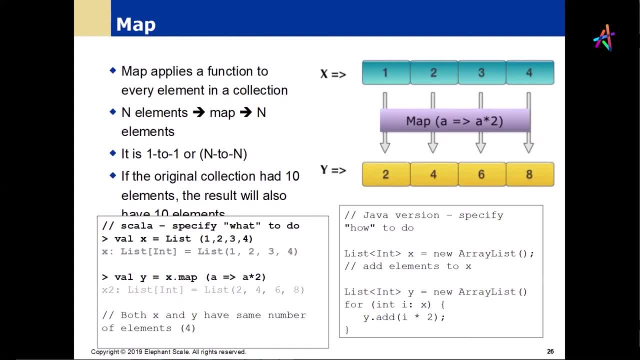 to success. successive elements. These are all fairly standard, So they're supported in Scala. There's the idea of a map function, where we're using a syntax, And again the point of this thing is that the point of this slide is that 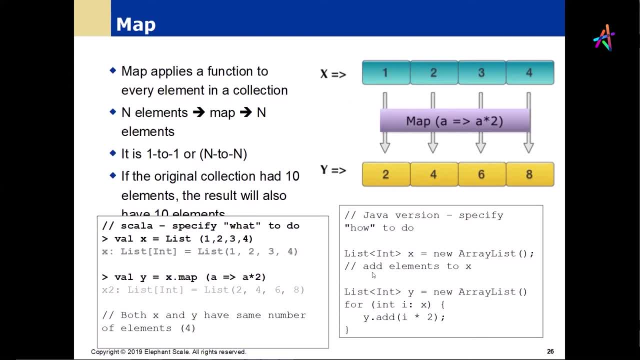 we're applying this as a single functional operation, whereas in we're using a procedural language. we're coding through the how to do it, whereas Scala is telling us. we're telling Java how to do it. we're telling Scala what to do. 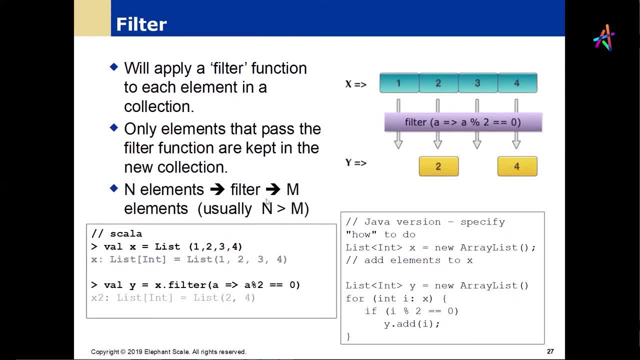 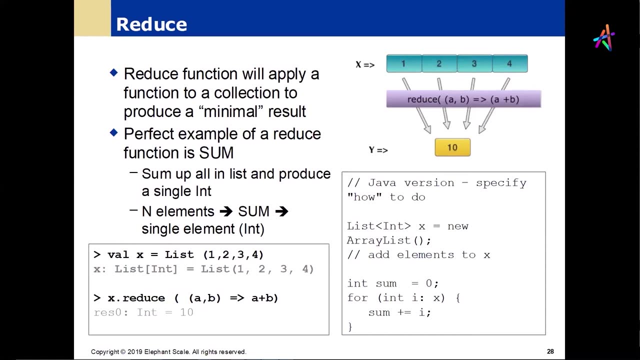 Okay, so filter function again as an extraction function. these are gonna be fairly important later on when we start to thinking about how these functions interact with each other in processing set of data. So everybody should be clear on this. Reduce function basically is a collector function. 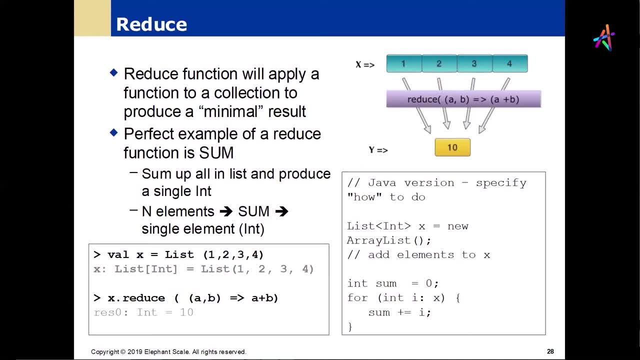 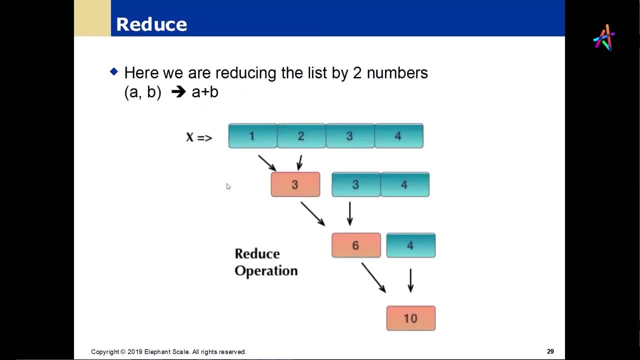 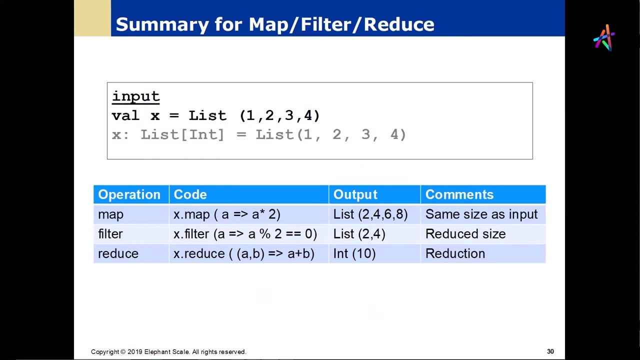 or an aggregation function of some kind, some kind of aggregation operator, And the example being presented here is some. and then we have reduction, typical example of using a reduction operations through addition to do a reduction of a list, And so this is primarily the essence of the operations. 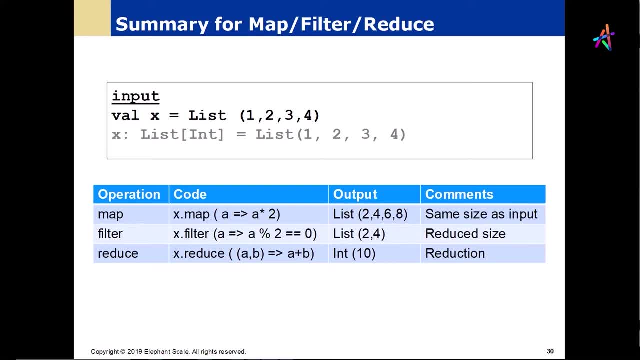 that we need to be concerned with. You should be familiar with all of these and the underlying conceptual concepts behind them: the mapping, the filtering, the reducing And, of course, at this point I'm assuming everybody's familiar with the concepts of. 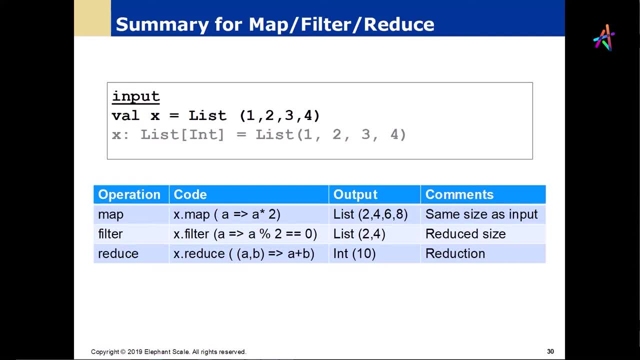 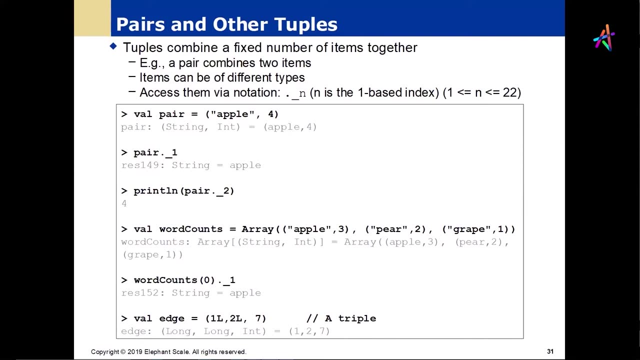 of anonymous functions. Anybody not familiar with that? I think everybody should, given the programming languages you've been in, So we'll we'll take that and move this along. We can define tuples, which are ways of structuring data. So just by using the tuple notation, which is the parentheses. this is similar to other. 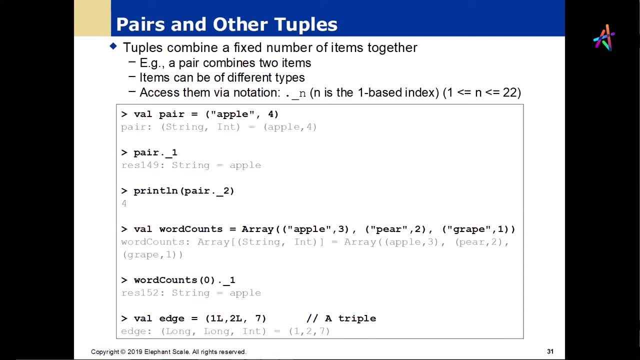 other programming languages, like we'll see in, like you will see in something like Python as well. The only thing that that might you might want to note is the, the use of the underscore notation to reference the various members of the of the tuple and, of course, if we had three triple. 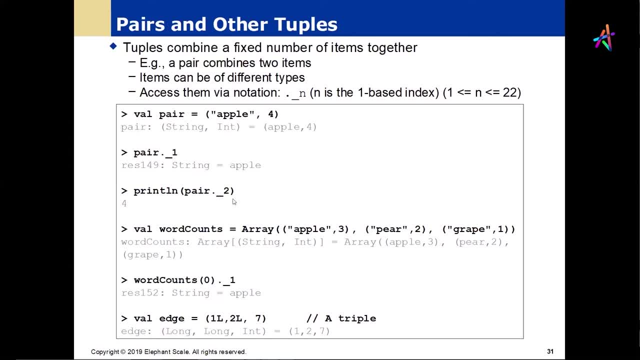 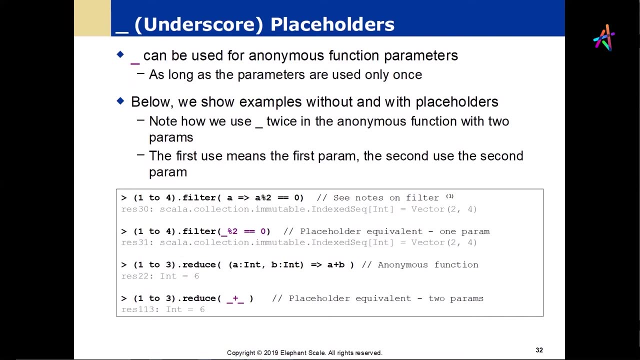 we could underscore with three as well. So this is the notation for for generating tuples. notice that this tuple is a different data structure than the The list. We can use this underscore placeholder For anonymous function parameters, which a lot as long as the parameters are used, or 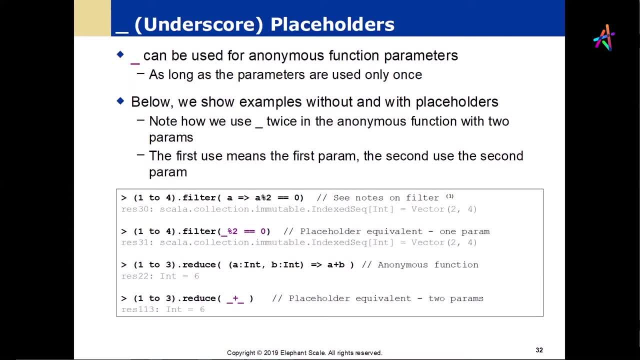 used once. So the Basically it's more of a positional assignment rather than named assignment. So when we have To parameter positions, The, the thelandIcenectare n Cristo, the order in which the underscores appear are the order in which the assignment takes place. 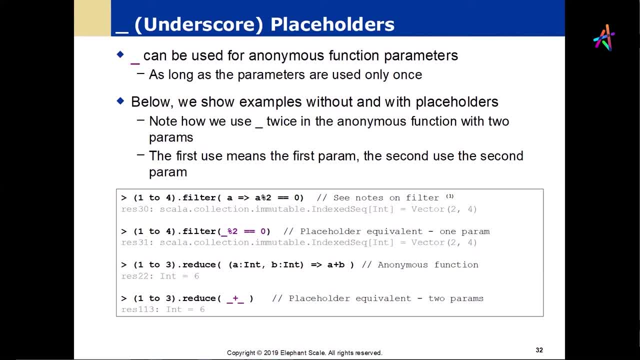 So the first example shows replacing a named parameter with an unnamed parameter so that we, since there is no name parameter, we don't really have to worry about it. Personally, I don't really like this notation, just as a personal preference, because I find that 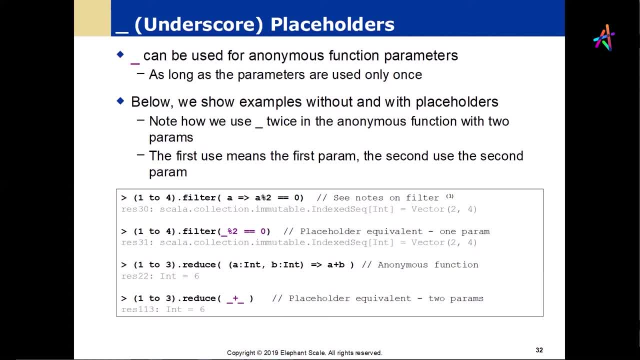 I prefer the readability of the other form, just for other people reading my code. but you know that's just a matter of personal preference. I mean, I think from the point of view of elegance I like it, but in the point of view of code maintenance I don't like it. 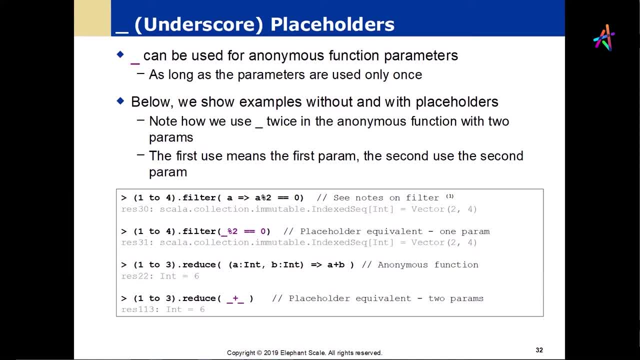 just simply because I got to think about other people reading my code, so I tend not to do that. On what you can see for reduce function, again, we have the two placeholders and they're assigned positionally, which means that the first underscore is A, the second underscore 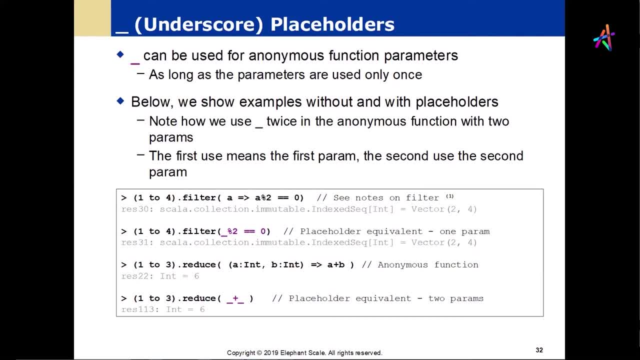 is B And it's positional. Again, very effective, very, very quick. Once you're used to it, it's a lovely notation, but the problem is that I always find is other people reading your code, And also I'm also the kind of person, though I should indicate, that when I have a complex 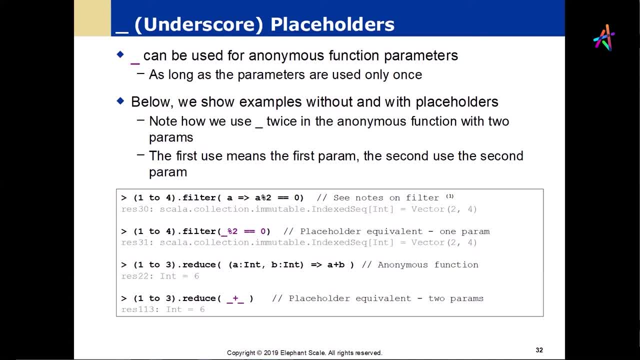 computation. I put the parentheses in to explicitly do the sequencing, more for my benefit than for the compiler's benefit. I often find that it's important for me to have a very clear idea of exactly what the order of the underscores are, And so, again, it's very, very, very quick. 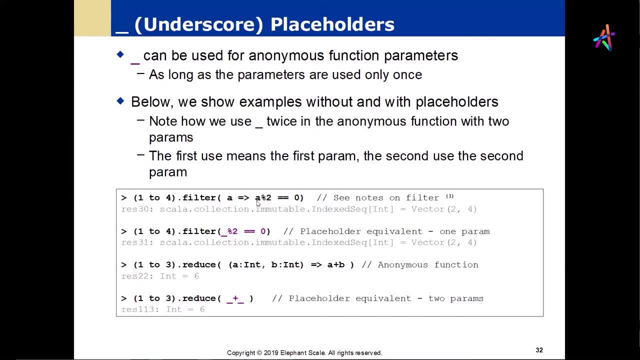 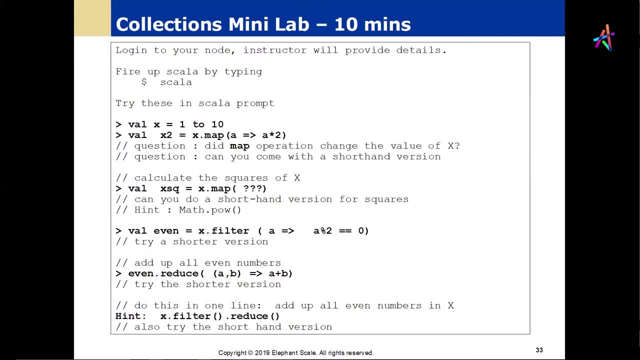 I'm not going to go into too much detail about what the order of operations are in an expression. So I tend to do that a lot, So we just did that. There we go, So we can go and you guys can experiment with a couple of these. One of the things I should point out is that I'm 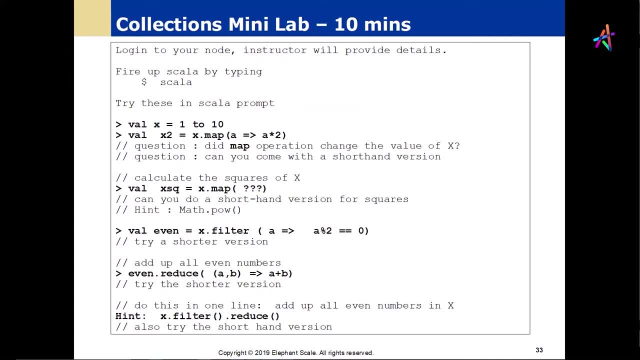 sort of committed to at least going through the material. So we'll give you guys a couple of minutes to play. I'm not going to do this now. I'll get you guys. give you guys a little bit of time. I'll give you guys an opportunity to experiment a little in the environment towards the end of 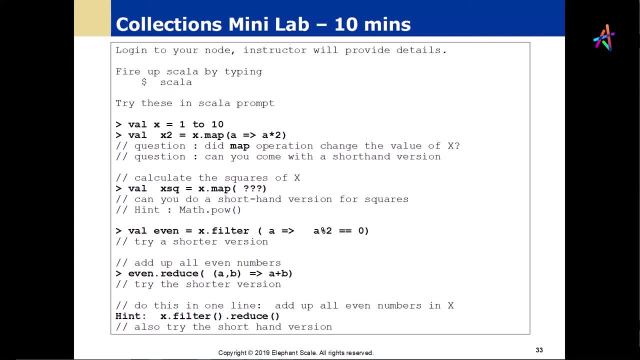 this morning's session, But I'm not going to stop and have you type in val equal 1 to 10.. You can go back and experiment with some of these things if you want, And if anybody wants me to go back to any of the slides, you can do that. If anybody is unfamiliar with Scala in working with the 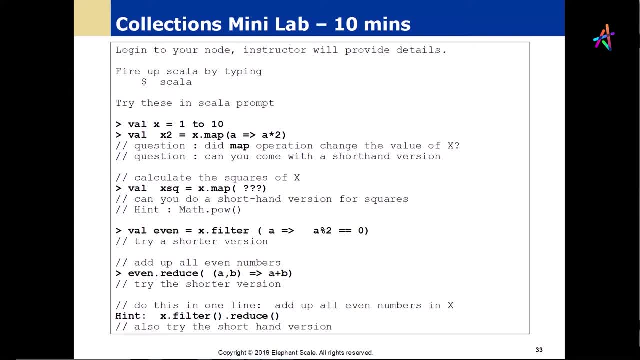 language syntactically. do take advantage of the opportunity. So does anybody want an opportunity just to kind of play around with Scala for a little bit before I move on? It doesn't sound like it. Can you go to the slides later? 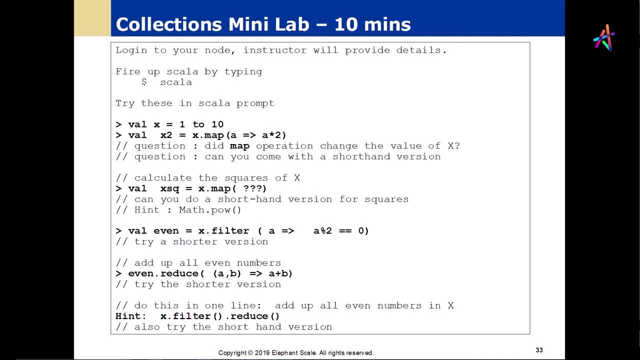 Yeah, I can give you the slides later. I'll make them available to you, All right, Yeah, that's good. Okay, So we can do that later. Okay, You might want to play around with a couple of these things. 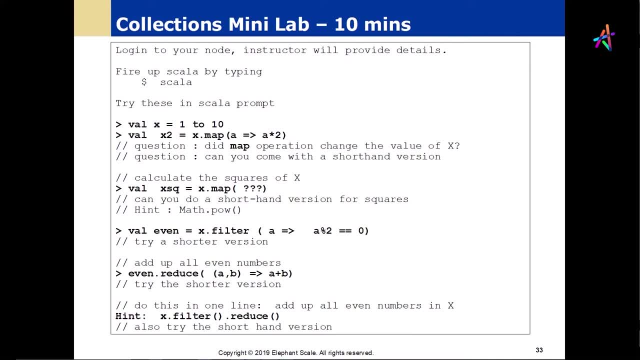 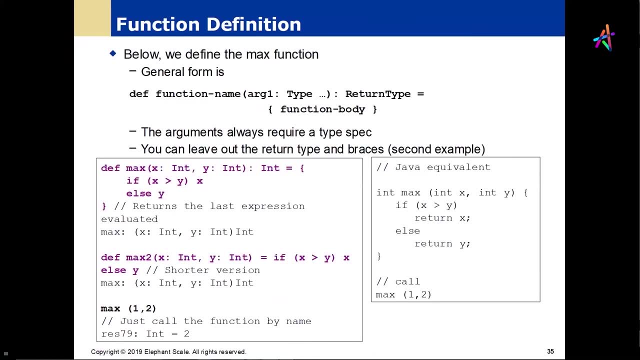 just and really the only reason I want you to play around with it is just to make sure that if you're new to Scala, you've kind of understood the concepts. Okay, So very quickly functions. Again, we won't spend a lot of time on this because this is fairly 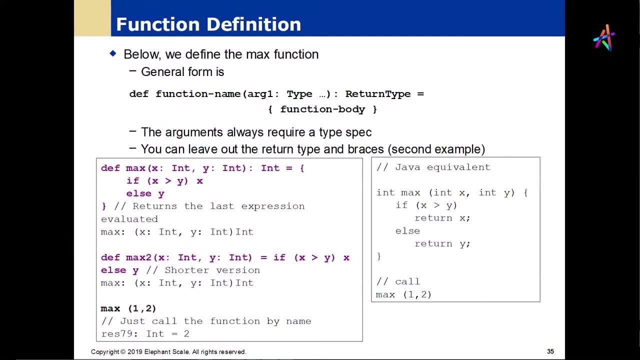 standard, But again we have to think in terms of the rewrite rules as opposed to more of a traditional approach. And again there's no specific return values, again, because we're always thinking in terms of evaluating expressions And we also notice again that the equal sign 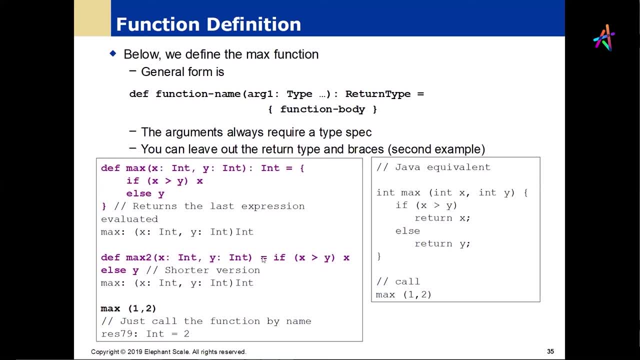 reminds us again. This is a rewrite rule And if we do have a block, then the block here, which is the parentheses, always returns the value of the last expression in the block. An empty block returns unit, which means that it's returning the equivalent of a void. 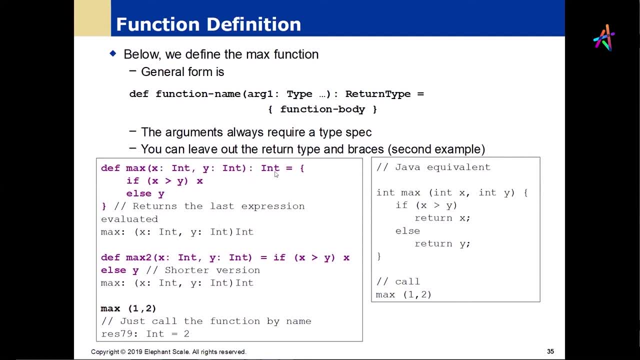 You normally do not have to indicate the return value of the function if it can be inferred from the expression. However, the one exception to this is if you're doing a recursive function. you do have to put the return value type there, Otherwise the compiler can get confused. 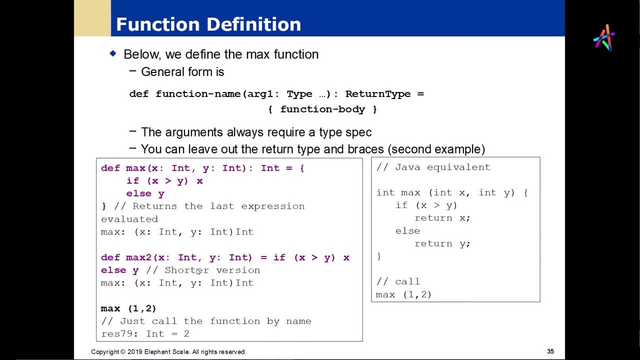 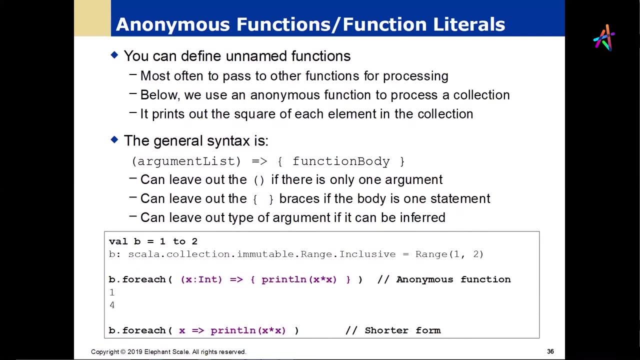 So let me see Anything else I want to do. Call the function by name. I think that's pretty much basic Unnamed functions. of course you all should be familiar with this And the standard arrow notation which we're going to see. of course quite a bit. So I don't think anybody 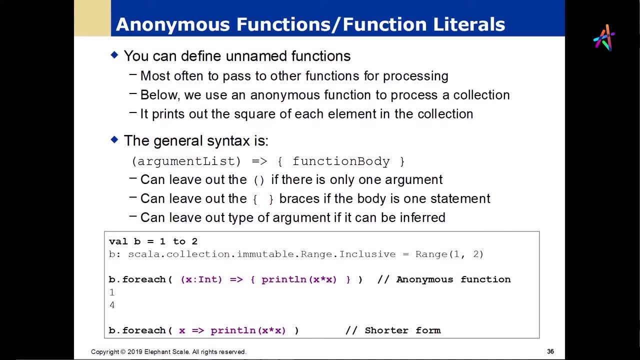 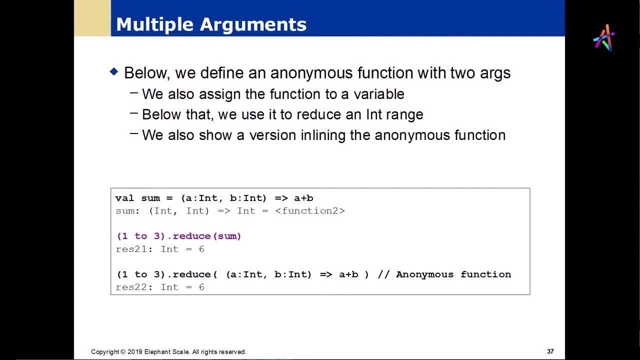 should have any problem with that, So we'll. we'll leave that as it is. Again, standard with multiple arguments. You can use a variety of different approaches here, including that using the underscore notation. So the important thing to also remember is that we need a function signature, So 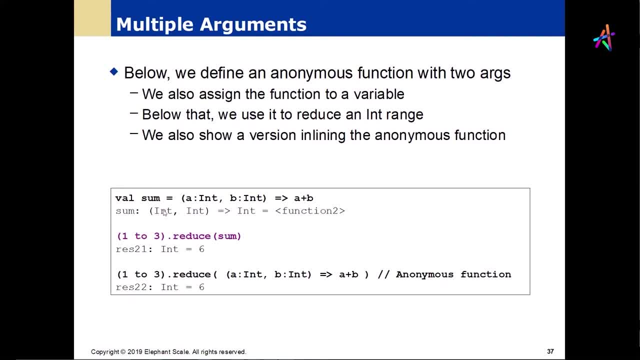 what we're actually looking at here is the type of a function, So we're assigning again. the distinction between defs and valves is somewhat different. What we're doing here is is assigning a function to a variable, as opposed to using a def. so when we actually do a def, 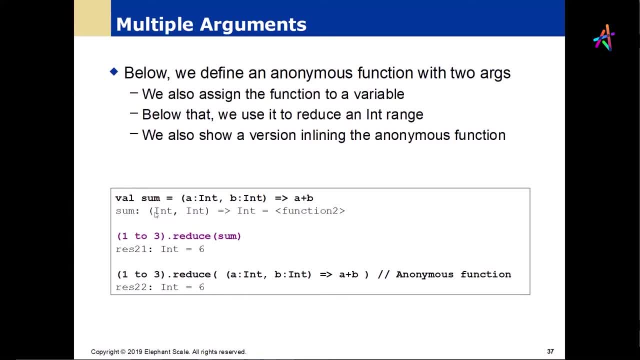 we're actually doing sort of a call by name. This is a call by value, and what this is actually returning is a function that takes two integers and returns an integer return type being inferred, the, from the what is returned by the body of the expression. So we can do the. 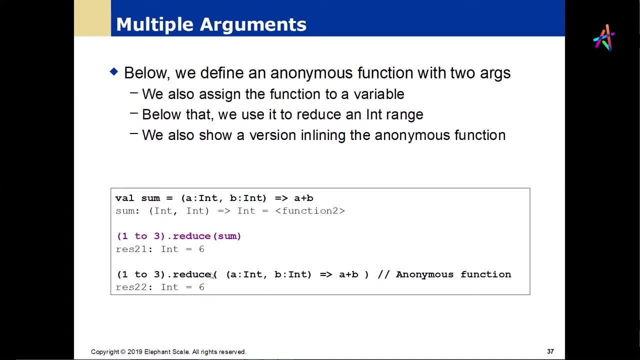 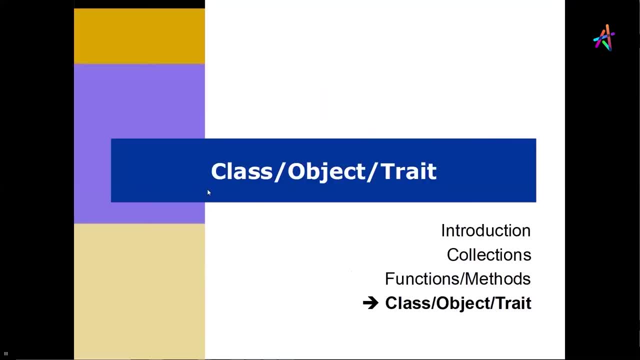 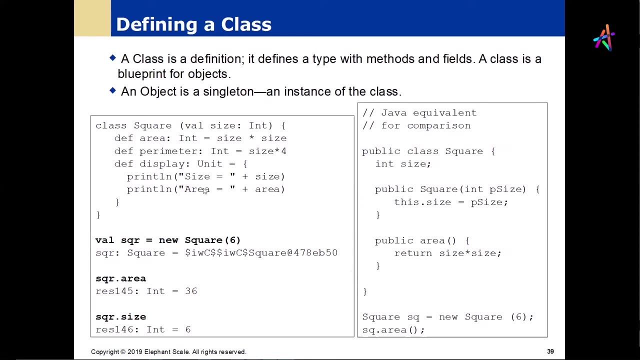 similar kind of thing here, Again inlining functions. so we use our anonymous functions wherever it's convenient. Again, nothing that's particularly out of the out of the ordinary Class objects and traits. well, again, this is where we're getting a little bit more away from the functional. 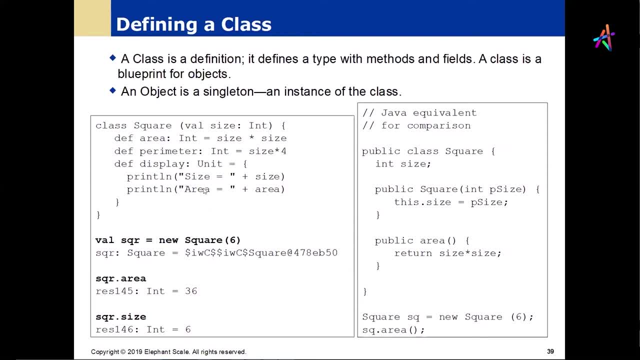 programming side of things and we're getting into the class definitions which are similar to the, which are similar to the Java definitions, And I'm going to ask one question. if somebody might want to think about an answer is: why am I? 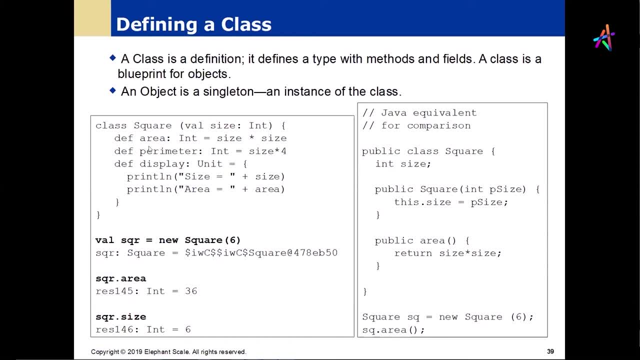 using def to define the. why am I using def to define the instance variables in my class definition? Anybody got a thought about that? Yes, Why don't I put var in there? I mean I could, but So in the end they have to be evaluated when you're calling it otherwise. if 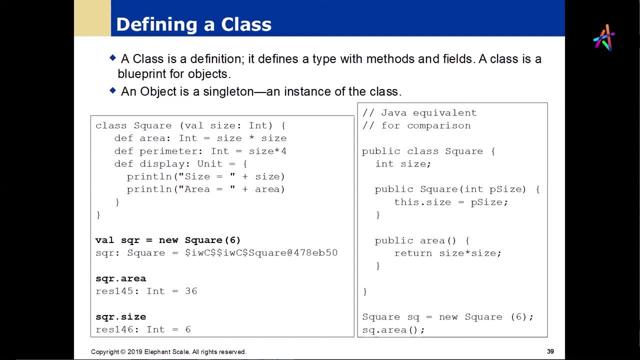 it would be a while, it would be evaluated too soon and it would be fixed. Yeah, actually, this is just reminding me that I want to evaluate these things actually when they climb, when they- not when I'm defining in the cloud, but when. 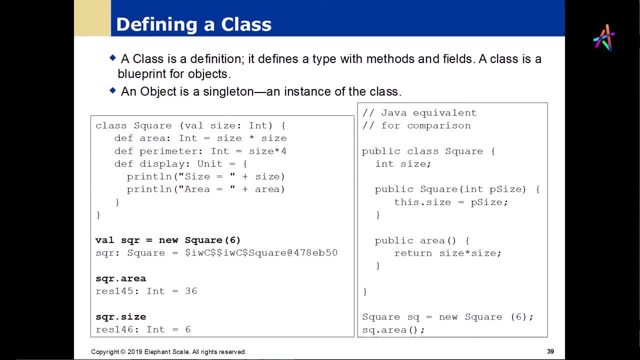 it, won't it? the instantiation time Exactly. So it's controlling when those things are evaluated. Thank you very much, Perfect, Okay, So I can create a new square object And that's the point of when things are evaluated. There's some rewrite rules for that class definition when you get to evaluate it. 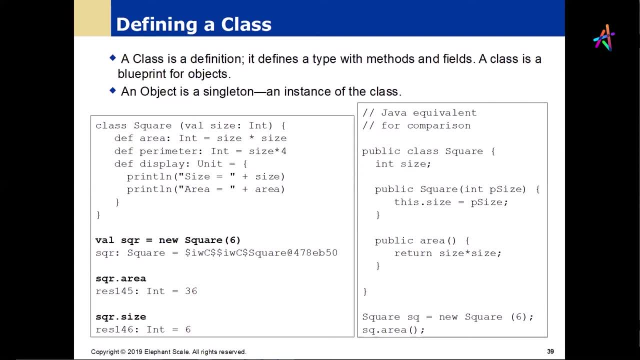 Other than that, it looks very similar to the kinds of definitions that we see. Everything, I believe, is public by default. I think that's how it works. Again, so many different rules and languages. I'll have to check on that myself, scoping rules of what the default is In this. 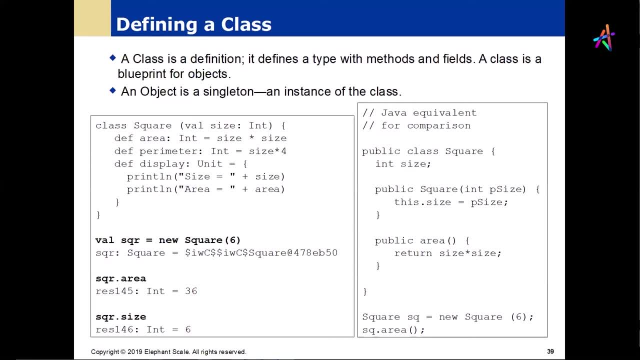 particular case as well. we also have a special singleton class which is object. So object is a class definition, but it instantiates a single instance of itself. So you can only have a singleton Singleton for that particular object. So you'll see that in a variety of places where for 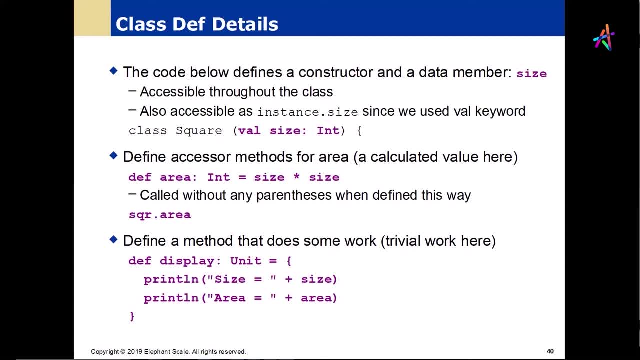 example, at the root of an application or something, you'll have an object as opposed to a class. Constructors. we also have this interesting notation here which is a bit different for accessors. So the data members scoping rules are the same, Access rules are. 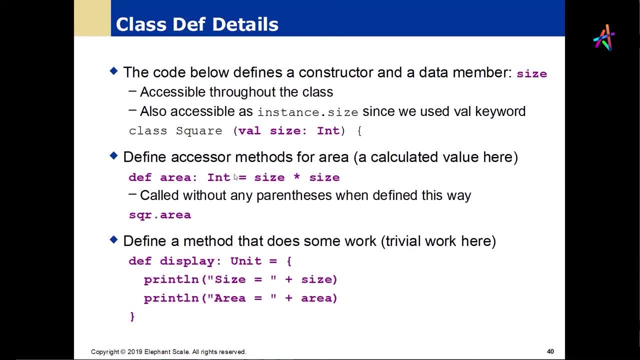 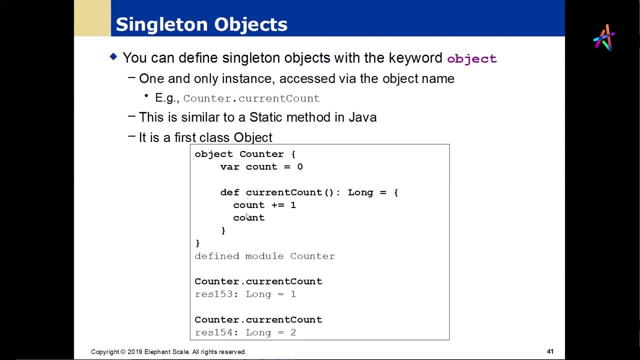 generally the same for Java, And we can also define methods. So all that's the same as Java. Singleton objects: again it's a class that instantiates a single object of itself And again this is a really much cleaner implementation of the. 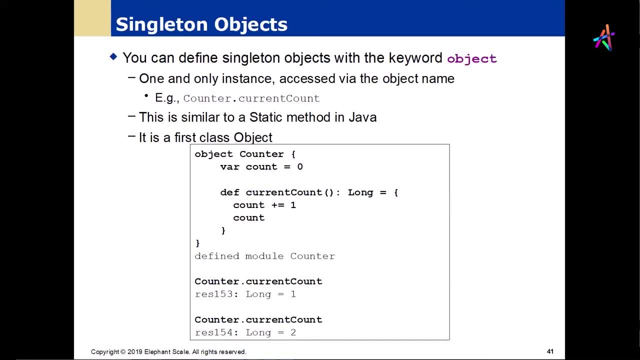 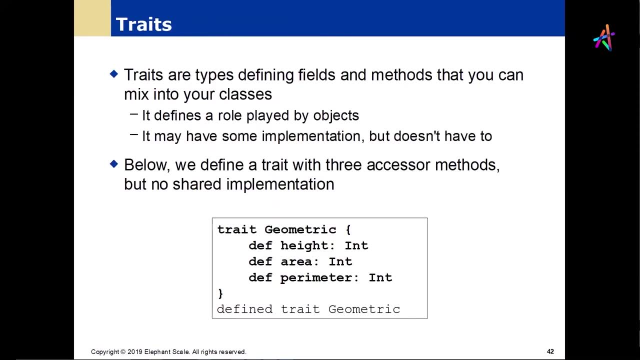 notion of a global object or encapsulating some kind of top-level global context. The notion of a trait is that it looks very much like a class, but it basically is used to provide what we call mix-in functionality And it can represent a role played by an object. 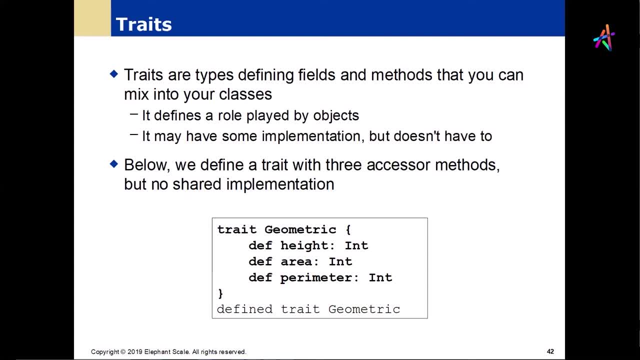 It does have to have an implementation, but it doesn't have to. If it doesn't have an implementation, then it's much like an interface on Java, But sometimes you want to include some functionality, So this would be a trait geometric which basically defines an informational. 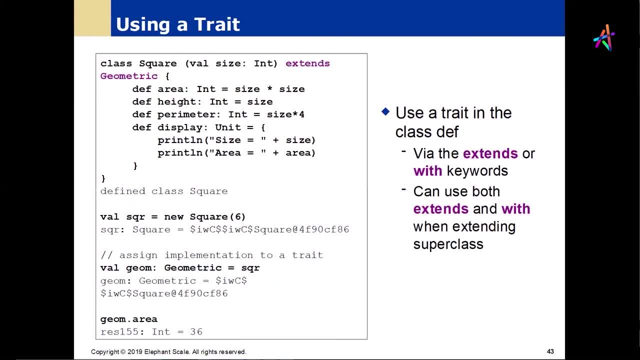 structure that is going to be shared, And then we can use class And the- everything is the trait here- in the same way that we use a Java interface And we're extending the class here, And we also use abstract classes in a similar way. 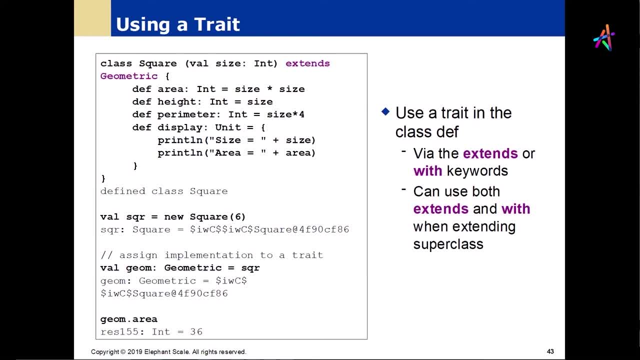 So we can create an abstract class in Scala, which also is a class definition that we don't want to use as the basis for inheritance, So we can have a new square. New square implements all of the appropriate methodology. This is very much exactly the same as Java. 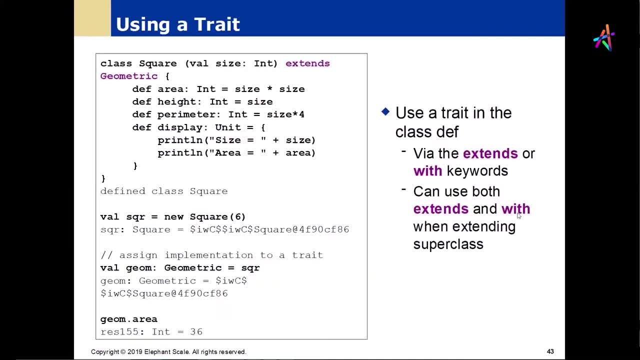 We can also use with to get the equivalent of multiple inheritance. We generally have a rooted single inheritance model and the mixins represent additional components that are added in to avoid the crossing inheritance hierarchy problem where we have multiple inheritance languages. So generally if we had other mixins we could have extends geometric with, and then we 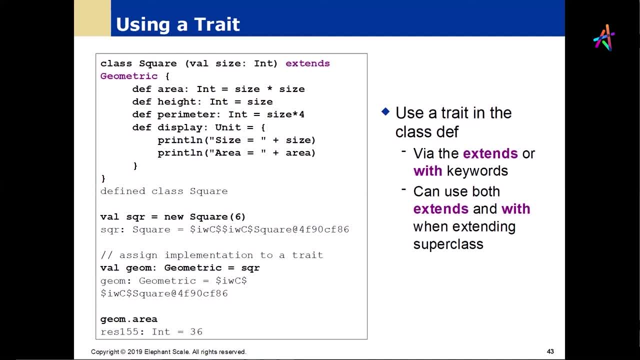 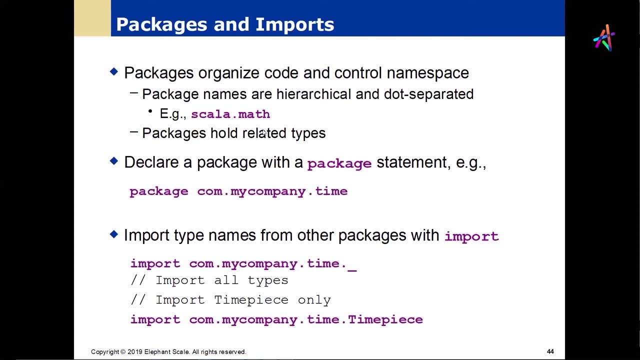 could add other mixins in there And there'd be examples in the Odetsky book if you want to take a look at it. Other things to notice: so traits are mixin classes a little bit more like interfaces in the sense of how they're used, but a little bit richer than interfaces. 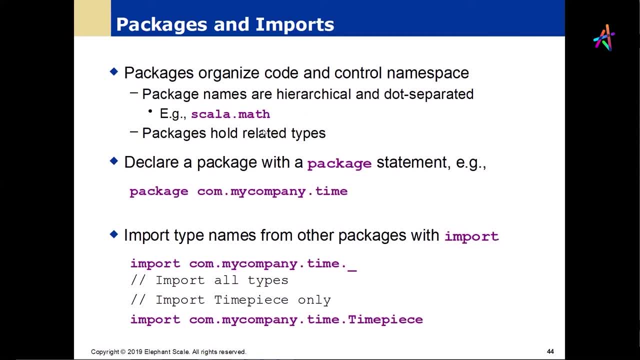 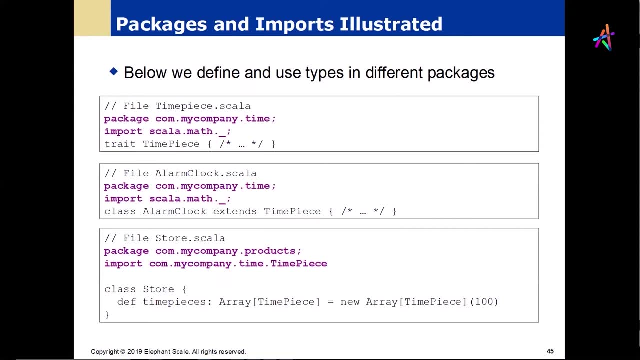 The packaging works basically the same as in Java, With the difference that we use the underscore character as the global wildcard to import everything from the package that we're being imported from. We use types in different packages, And I think let's see what this one's about here. 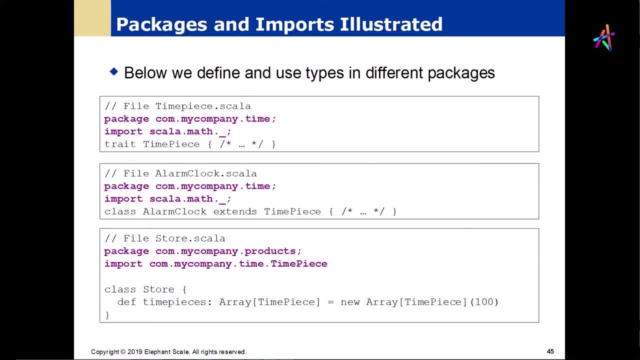 Yeah, so we're using time here. So, again, fairly, it's the standard packaging and import system that we see in Java because, again, it's built on data, It's built on the Java platform. So if you understand how the Java packaging works, you pretty much got this thing down. 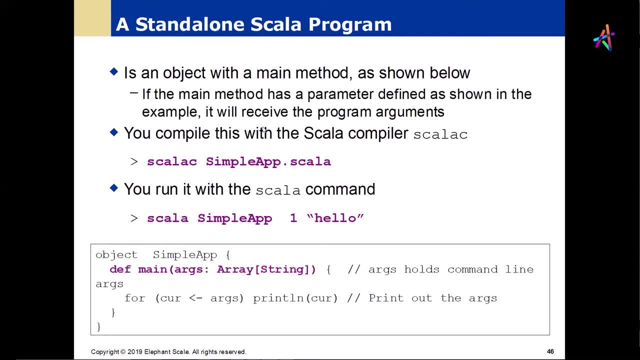 nailed. Okay, The compilation process is similar for Scala as it is for Java. We use the Scala compiler, just like Java C, and then we run it with the Scala command, just like we run with the Java command. And when we do this, we have a main method. 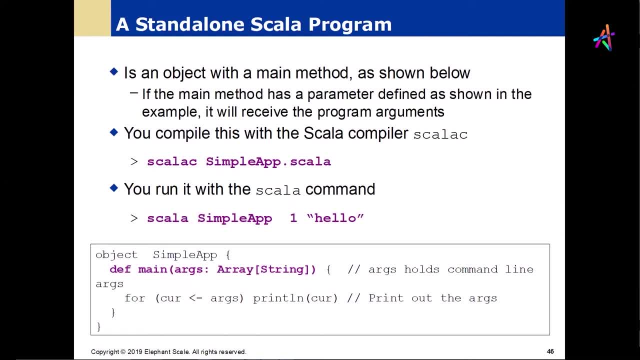 Which gets the program arguments. So it is generally an example of where we use the object. So here we've got an object simple app. It's got a main method, which is the entry point, And it's got the execute that's executed. 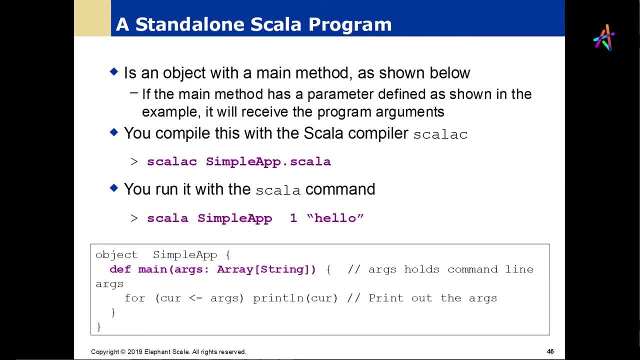 So we can execute the application, simple app, with a command line argument which is picked up, Command line arguments which are picked up and used, All right. So the idea here is again: we're Okay, We're not nevying too far from Java, but we're kind of got some interesting variations on. 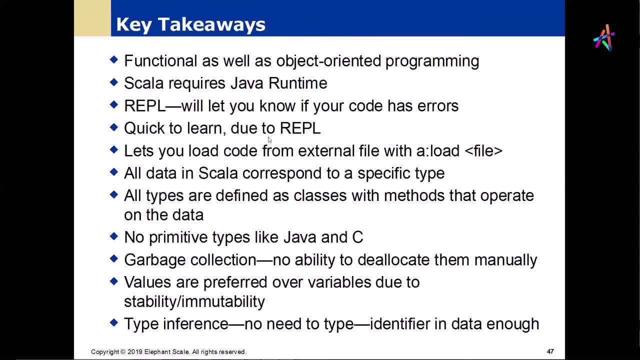 the methodology. Okay. So now we finally reached the end of this particular section. So key points: functional as well as object oriented programming Running in a JVM. there's a REPL which is something you can use to play around with. We do have the option of loading code. 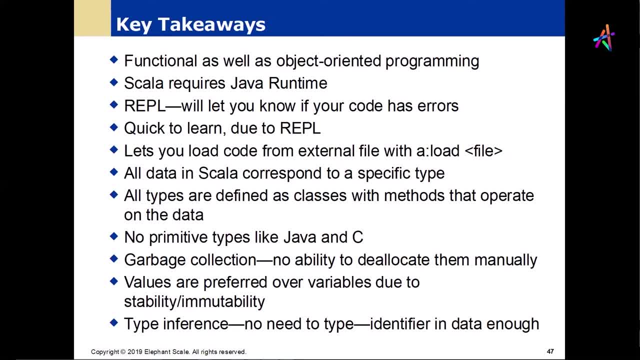 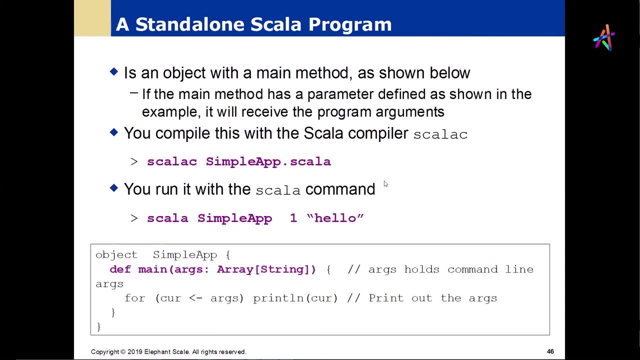 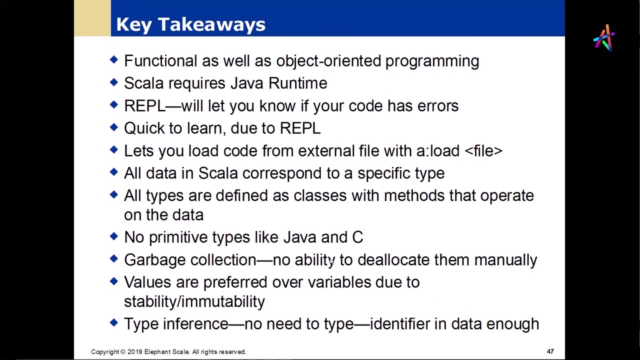 Scala is strongly typed. Everything is a class, defined as a class. Even literals are all objects. There's no primitive types. There is- Hold on here, Oops, My mouse is. My mouse is rebelling. No primitive types. Again, it's using the garbage collection. 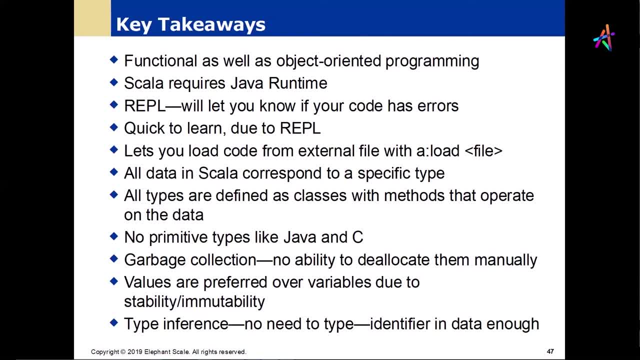 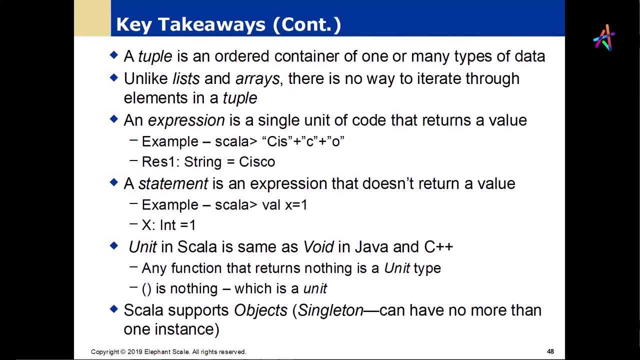 Something like Tungsten overrides that garbage collection. We prefer the immutability. And then we have type inferencing- All of those things we've demonstrated or seen. Tuple container of one or more data types, lists and arrays. No way to iterate through elements in a tuple because there's no internal iterative structure. 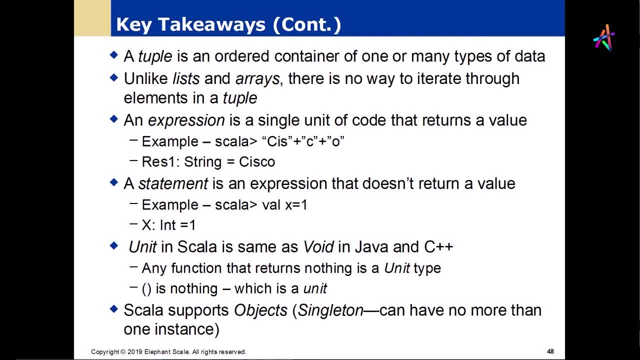 associated with it. They're just collections of things, Expressions. We've seen that Evaluations of expressions are basically applying rewrite rules. There are. There are some things that are statements that don't return a value in. That's just syntactically difficult to do. 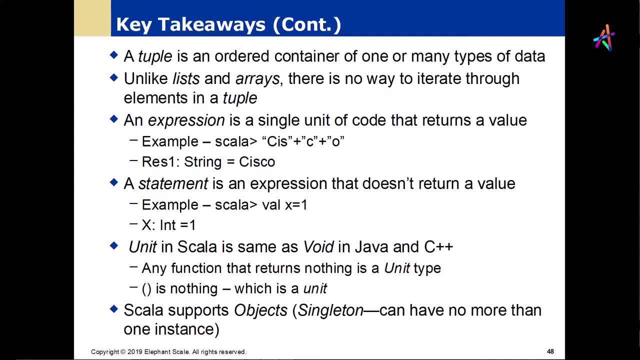 So mostly they're things that define things like val x. It doesn't, You can't assign that to something, but it does return an evaluation. in a certain sense It tells you it created something. Units the same as void And And. 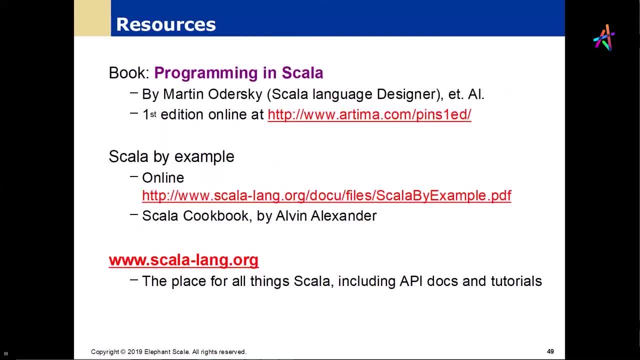 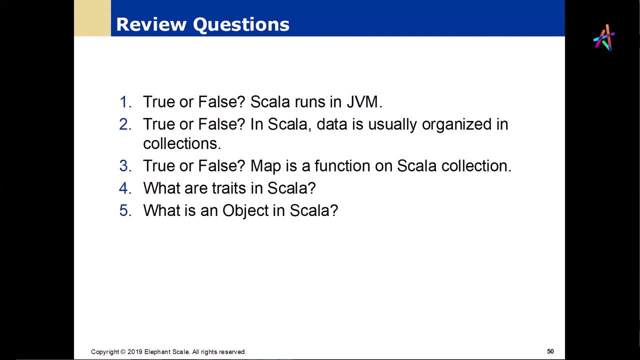 And objects, and that's, I think, what we really want to cover off. Okay, So I think you should have any problems with those, And if you don't know the answers to those, then you probably need to take a look at a. 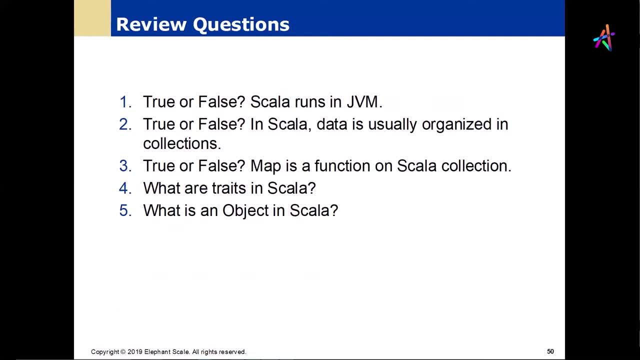 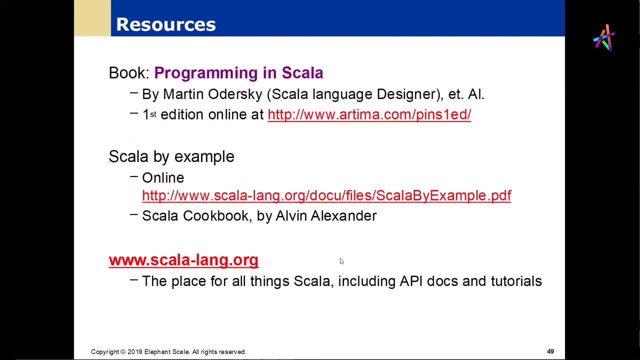 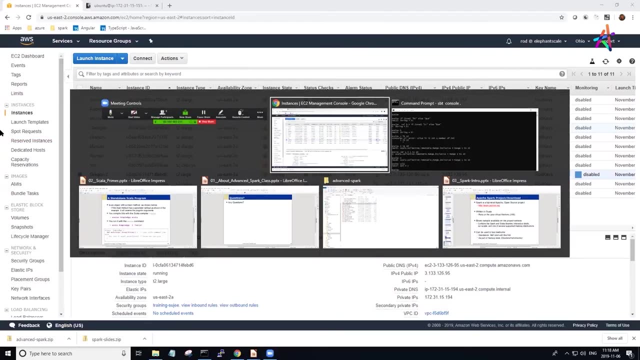 couple of things, But I'm judging by the feedback. Everybody shouldn't have any problem with those particular problems, Those particular questions. Okay, So Again, If anybody wants to do a little bit more reading of Scala on their own, that. 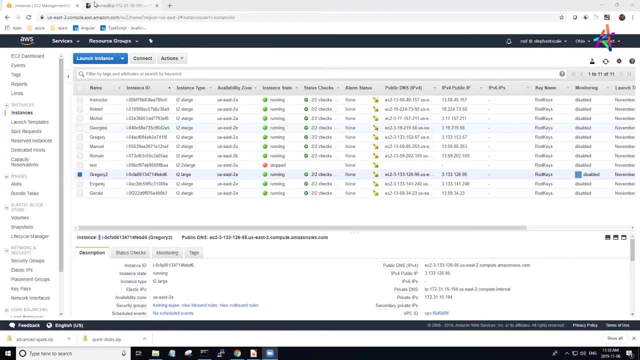 What we want to do is: I had it set up here, Here we go. I put the link in the chat for the Scala by example, So you can. You can take a look there for some of the more More interesting elements about the Scala on their own. 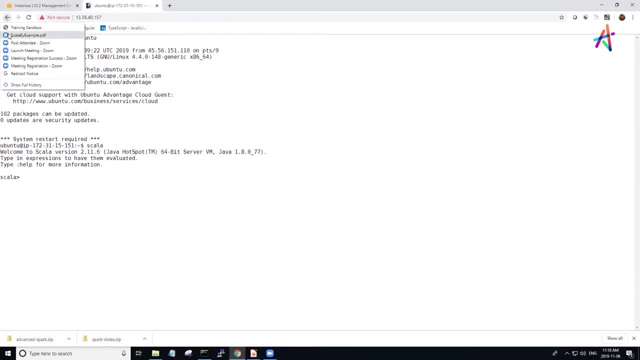 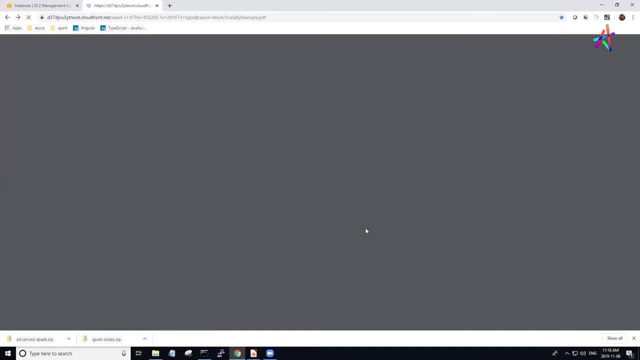 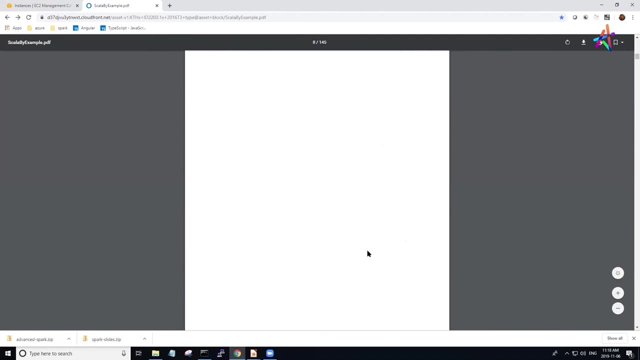 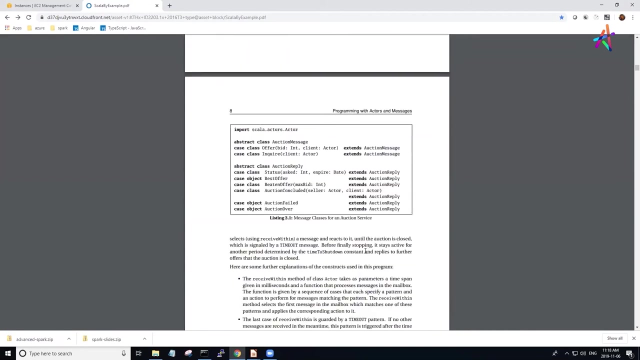 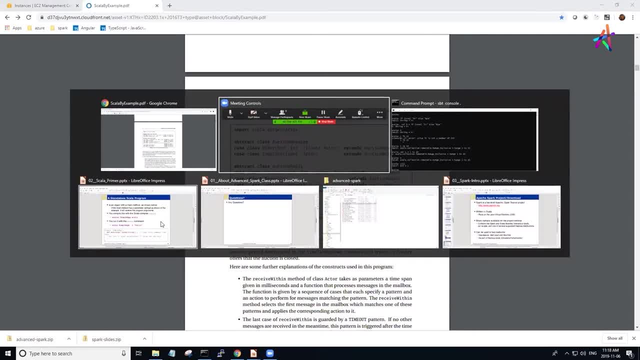 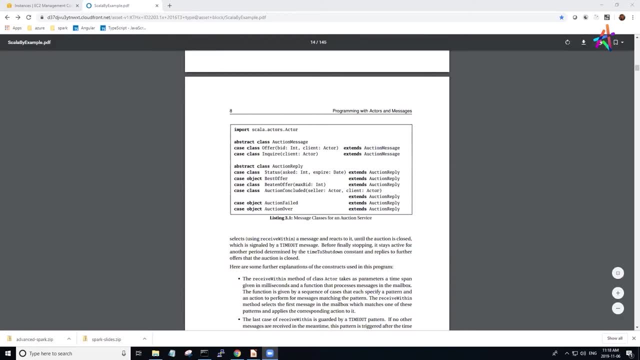 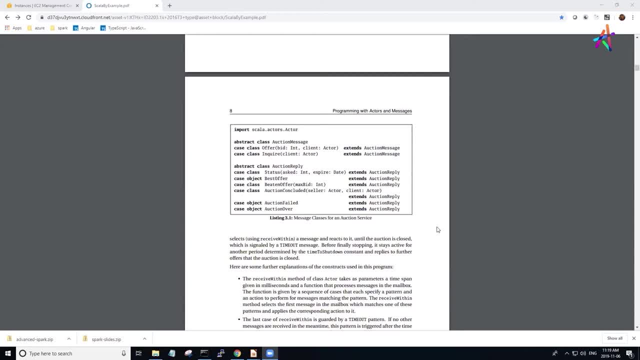 virtual machines. I'm going to see about fixing that VNC problem today, but I'll leave them up until I find the solution for it. anyway, I'm getting an echo. I'm having a hard time understanding that. I have a suspicion. I know how to fix that problem, but I want to test it before I take. 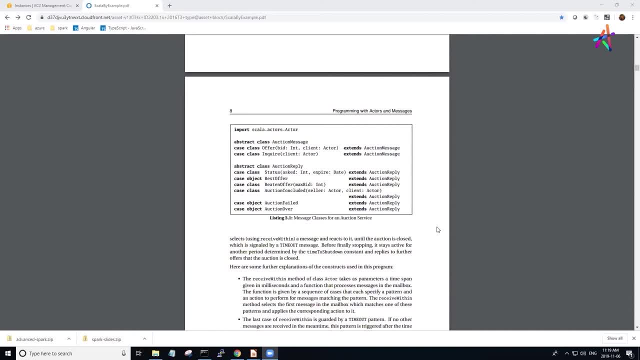 up any class time doing it and then you can do some of the other stuff on it as well. But I'll leave them up for now with those operations and I'll work on one of the machines to see if I can resolve that particular issue. 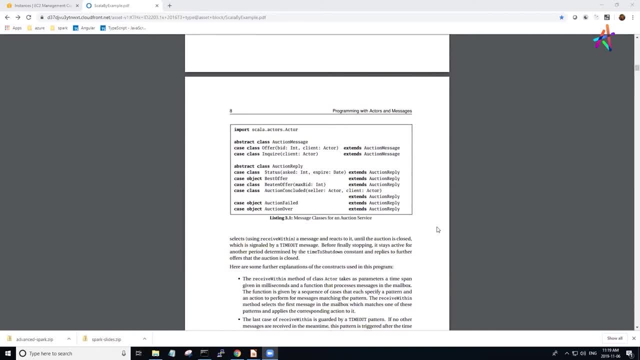 So the issue with the VNC? are you talking about the VNC? What are you talking about? I'm sorry, Could you repeat? So are you talking about the issue with this VNC server? Yeah, Yeah. So I think restarting the machines already works, or just killing the VNC server and 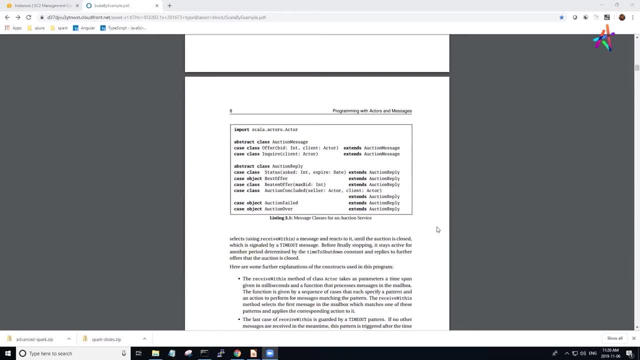 starting up again. So the problem was the machines were up for one day and I guess someone on the internet tried to log in a thousand times and we were locked out. Oh, excellent, Yeah, but my client is not connecting because it says: 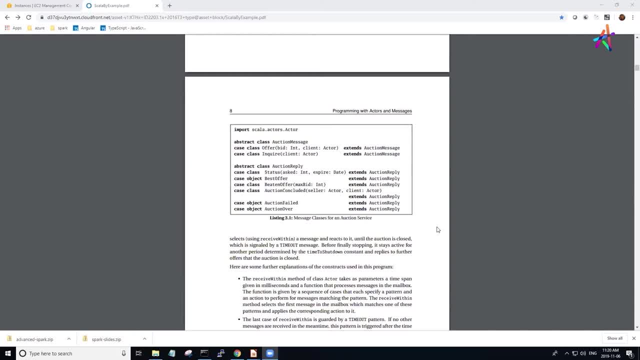 I think the settings are uncomfortable or somehow wrong. I Googled and there are some host encryption settings which are set to true and the mock bind is just unable to. Okay, I'll tell you what I'll do, guys, is that I will actually restart the machines. 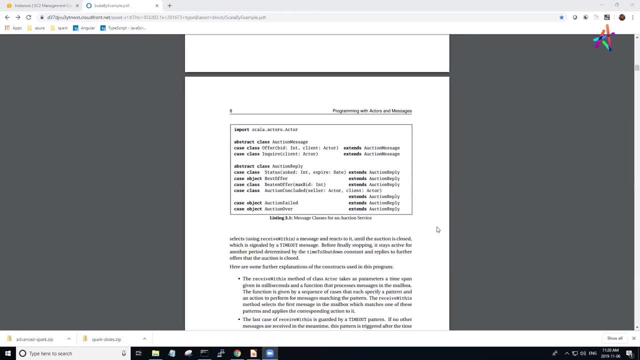 We'll wind up with new IP addresses and things, but I'll restart them just before class and we'll see if that doesn't solve the problem. Because, now that you think of it, I started up the machines and I did my VNC test, right. 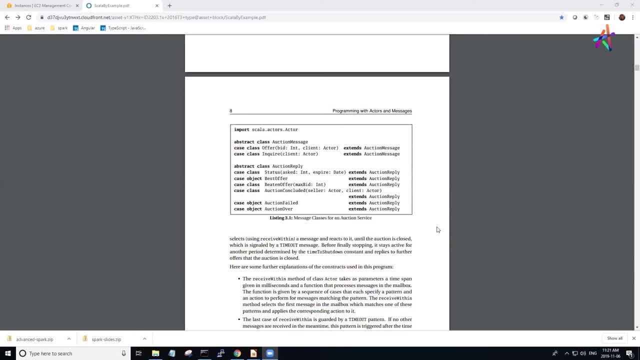 when it started, after it started up and I had no problems. So I think whoever did that analysis about attempted logins across the internet, I think you're probably quite right. It never even occurred to me. That was actually brilliant thinking. 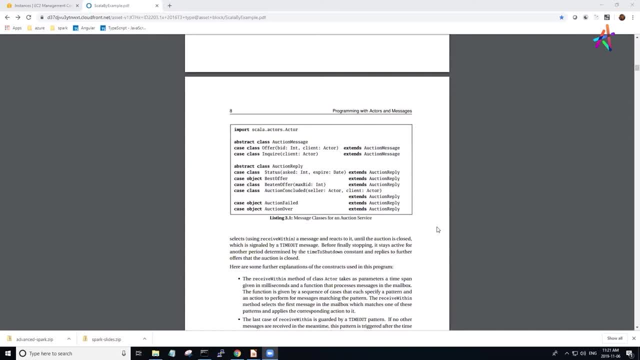 If you're looking for a job, talk to me. I'm fine with it. thanks, Okay, Oh, brilliant, Brilliant, Okay, Yeah, That authentication failure, I think, is probably directly due to that. so thank you, Good point. 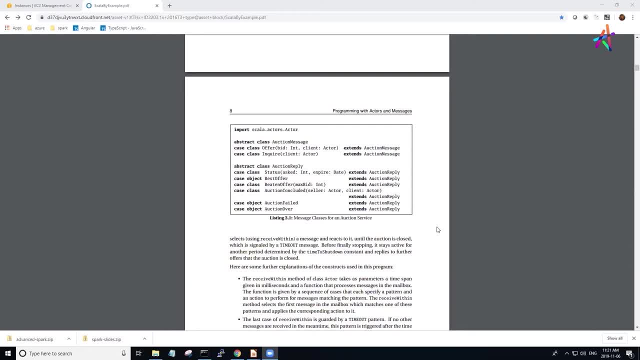 And I will try and resolve that issue later And once we get logged into it, Hopefully you can just stay logged in and if we have problems we can restart or something to that effect. Okay, Okay, Thank you all very much. 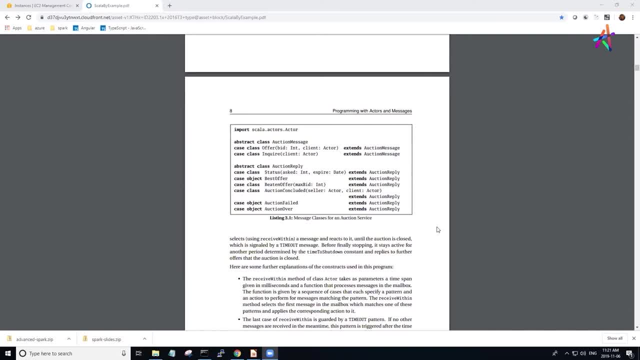 Okay, So we're good with Scala, and if you guys want to just play around with that environment, or a Scala environment, I will leave the machines up for the rest of the day so you can use the SSH and play around in there at some point if you want. 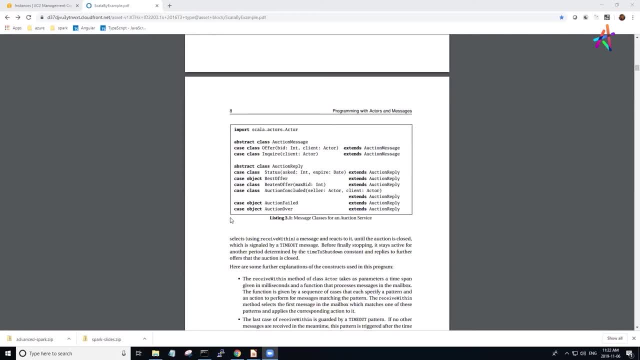 And if I do, If that is the correct solution, I will just reconstitute the machines just before class and let you guys log in right away at the beginning of class, so that we can basically get that authentication in place. All right, 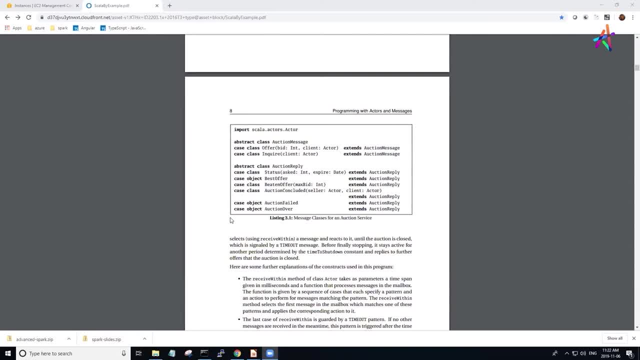 Thank you very much. Okay, So now, if there's no questions, we'll get into the real content of the course, which is our Spark. We've already talked a little bit about Spark. I'm not going to do the Spark installation today. 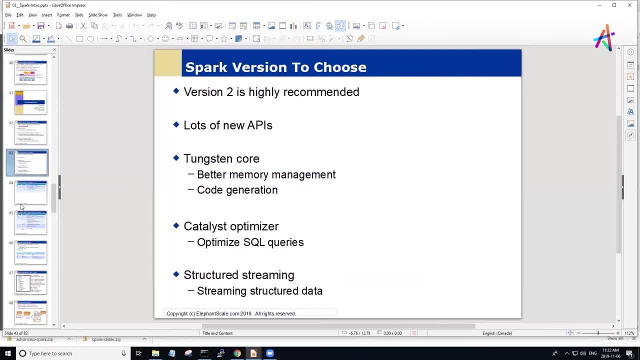 I'm going to wait until we get into the machine tomorrow so that you can actually Not going to lose it if I have to reconstitute the machine. plus, we'll just pick up with that first thing in the morning tomorrow or the first thing in the afternoon for you guys. 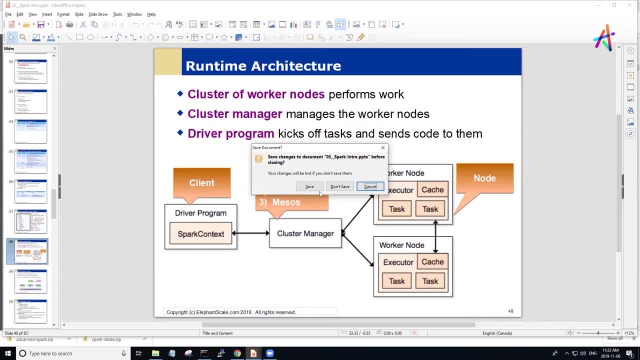 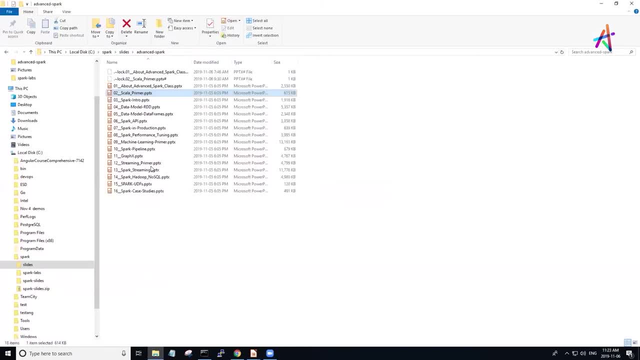 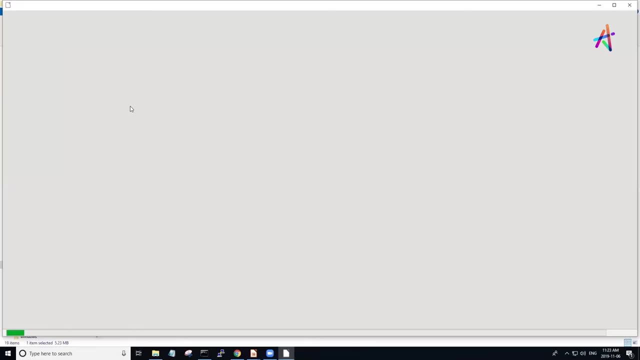 So let's get rid of that one. We've done that one and we want to spend today and tomorrow working on this notion of the, The data model. So we've talked about the intro to Spark. I think we've covered out most of that. 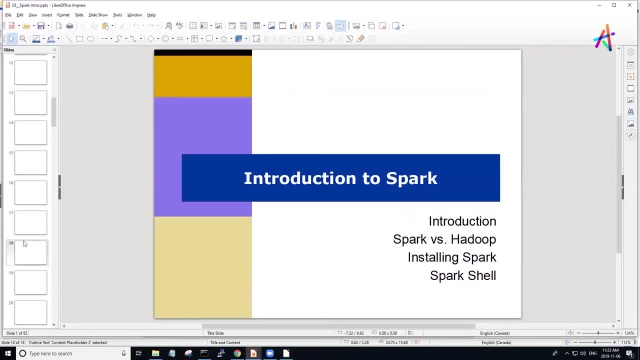 Let me also double check to make sure we've done that point All right, And I think we've covered off what we want to do at this particular point. Yeah, Okay, We'll come back and look at that one later, after we. 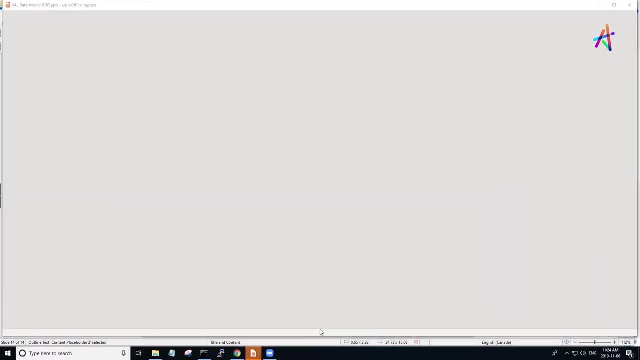 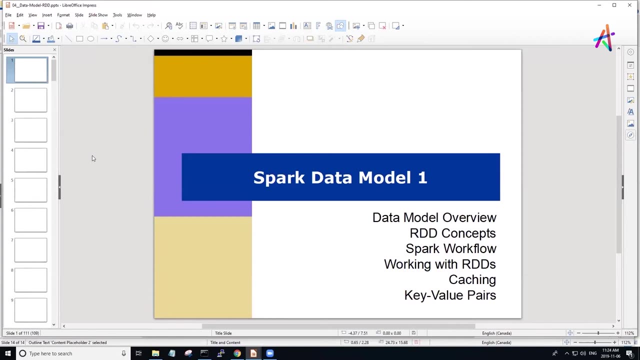 Come on here, Let me get this data model. we're going here, Okay, So now we're into the heart of Spark. So those of you with zero Spark and one light on their Spark, this is where, hopefully, things will start to get fun. 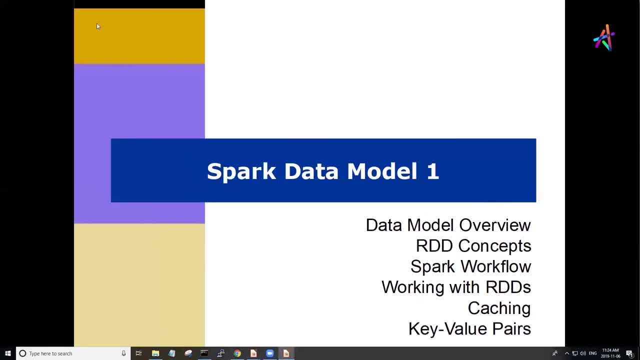 Okay. So one of the things that we also want to emphasize is that I'll refer back to some of the ideas in Scala that are showing up in Spark. We've seen Spark from an architectural point of view. We've seen where it kind of fits into the ecosystem, what its goals are, what it's intended. 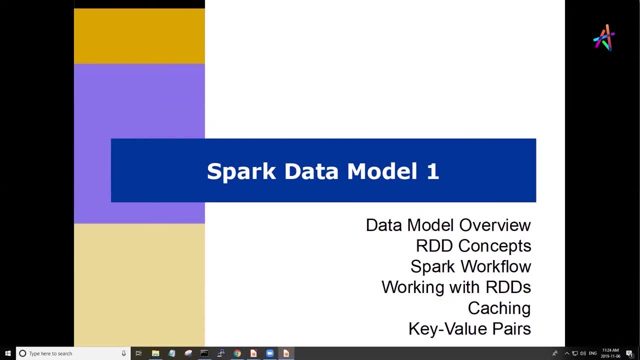 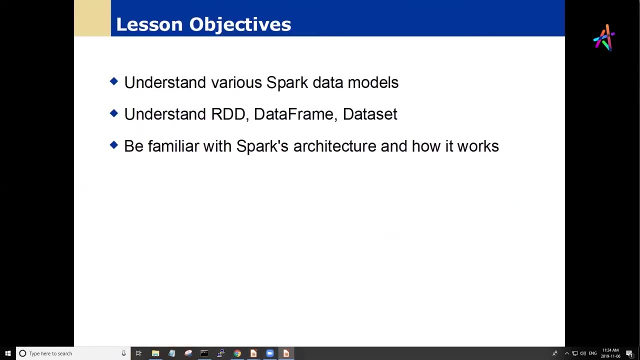 to do what it's not intended to do, Which is to replace the data storage mechanisms or to be a node manager, although it can be if it has to be. So we'll start with the notion of the Spark data model, since Spark is all about data. 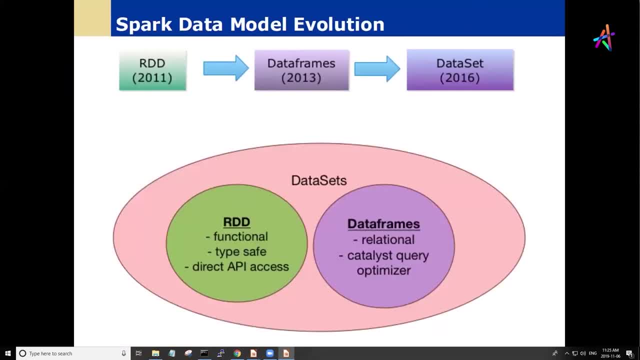 And we're going to start with the idea that there are multiple data models in Spark And these correspond to multiple versions of Spark. The original one was the resilient distributed data set. This was changed or not exchanged, but this was complemented by the introduction of data. 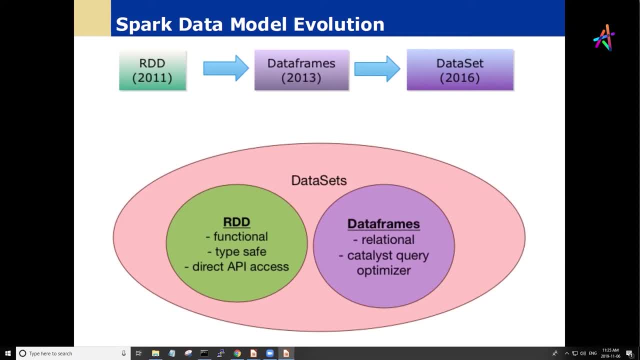 frames. Now, the big difference between RDDs and data frames is that RDD sees data as basically opaque. So if you've got a bunch of data, you can see the rows and the records and the data, but it has no concept of the internal data. 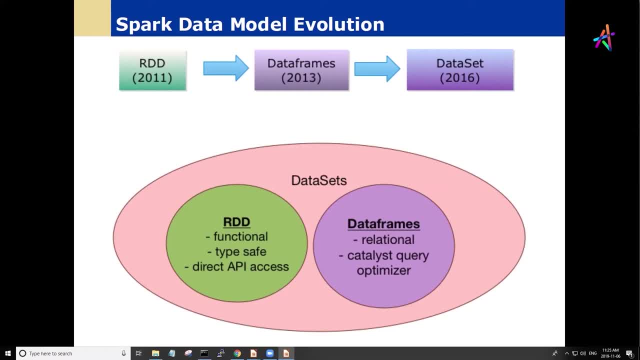 Okay, Okay. So it's a very complex structure, And what that means is that certain optimizations that it could do based on data structure are unavailable to it. What data frames do is they introduce a schema into the data and allow data to be schematized. 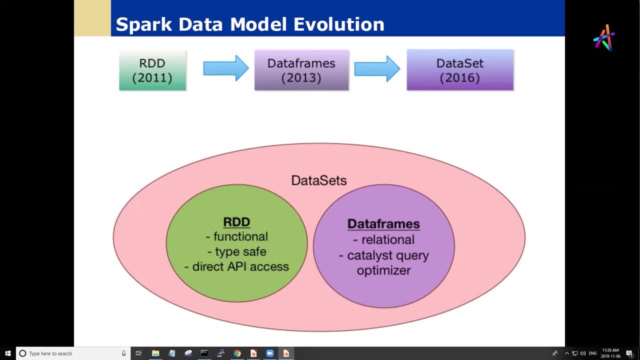 so that now we can perform optimizations based on the actual structure of the data in the records. And this is where we also introduce the catalyst query optimizer, Which is the tool that, once we have this catalog structure, can make optimizations based on the internal structure of the data, which is something that RDD could not do. 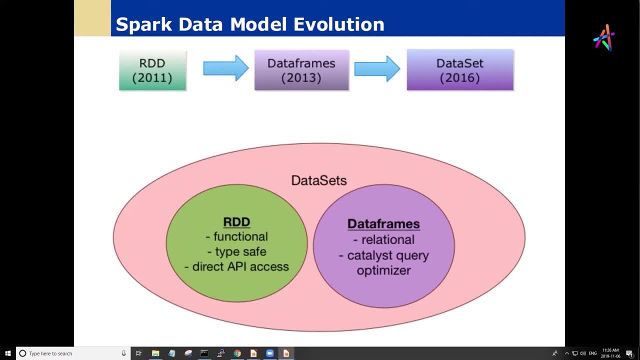 In 2016,. we have data sets, which provides a unified interface to those so that we can have a more integrated environment, And we'll generally think mostly in terms of data sets And in fact, we generally do talk about data sets now. 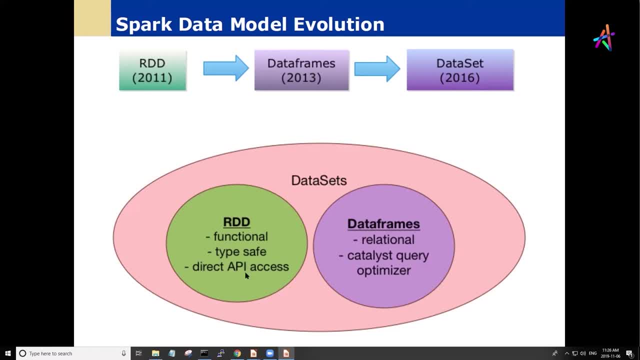 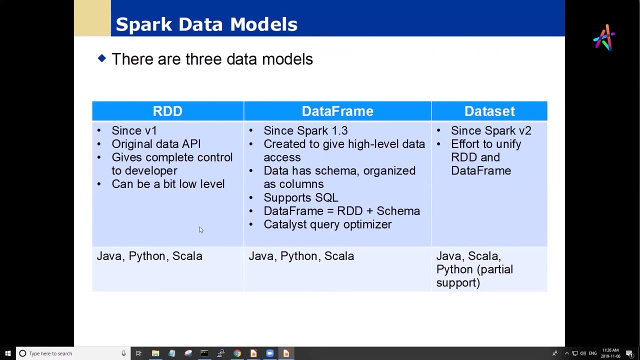 But we'll talk about that later. Okay, All right, Thank you. Take care instead of these two discrete categories, And we're going to find that most of the time, we can pretty much treat data as either one of these things. Okay, so the three data models, again summarized here: 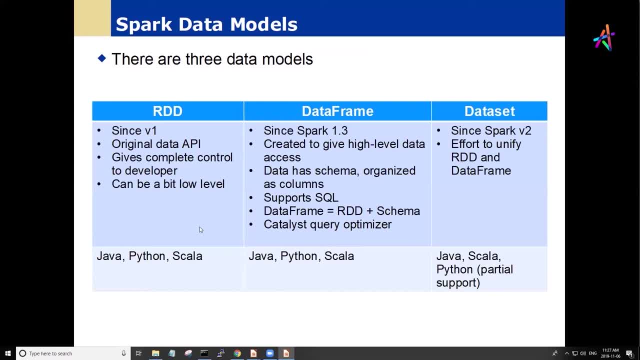 the RDD gives complete control to the developer and again a little bit low level. But we're going to look at the concepts behind it to see how Scala actually operates with the data. So we've got a data frame, again schematitized. 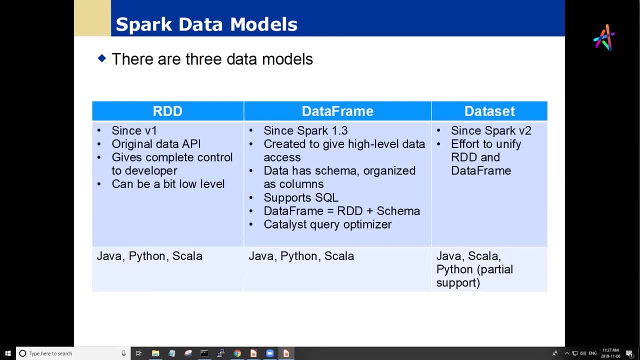 organizes columns, supports SQL, And so it is a RDD, but with an associated metadata about the structure of what's going on in the roads. This is an important innovation, because a lot of the data that we work with is structured data. It is schematitized. 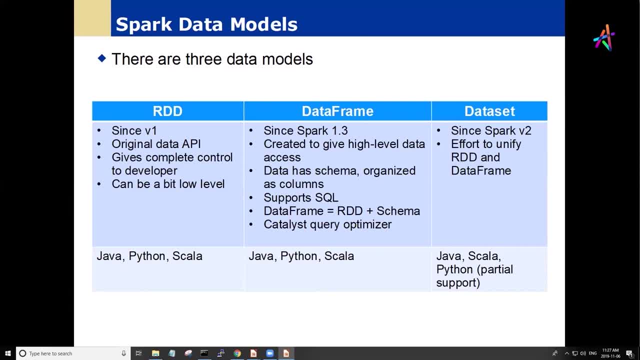 So we want to be able to extract those schemas. So everything from CSV files to JSON files in a certain sense is schematized. So it's not schematizable because it has some kind of structure, Whereas raw text is generally something that's not schematizable. 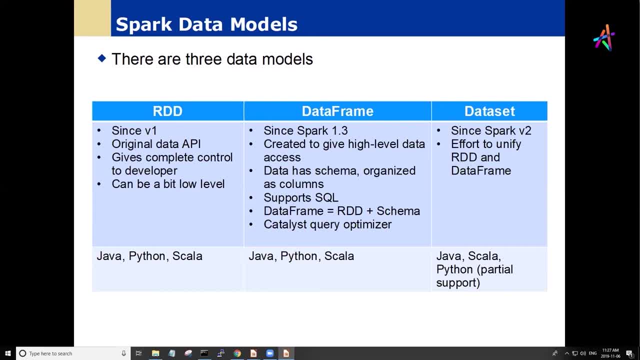 It's just text in lines. There's not a lot you can do about that, And a data set is really an attempt to provide a unified interface to the data, whether it's represented as an RDD or as a data frame. Not all data can become data frames. 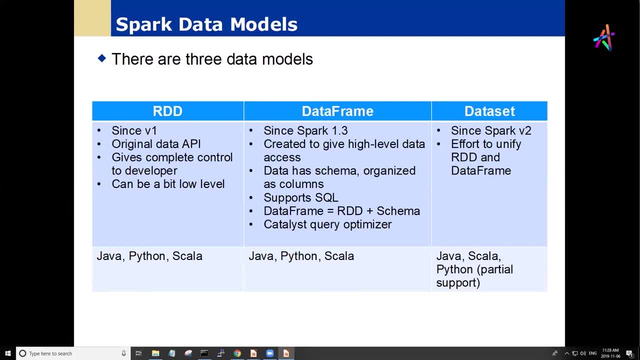 So the and again, if you've worked in Python with data analysis and Notion, so Pandas. or if you've worked in R with data frames, the idea of a data frame is not unique to Spark. It is a common way of representing data. 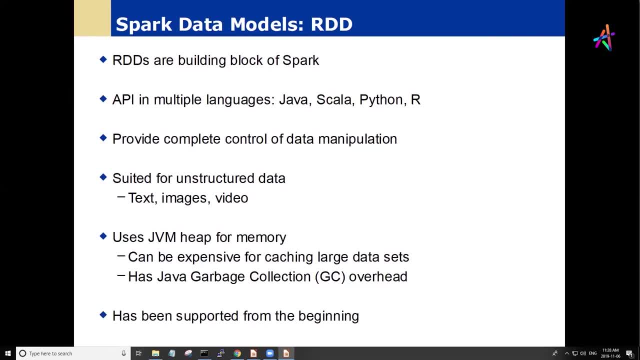 So the RDDs are still the building block. We access it through multiple languages And it's really, really the tool of choice for the unstructured data I just mentioned: text, but again, images, videos, anything that does not have a schematizable structure. 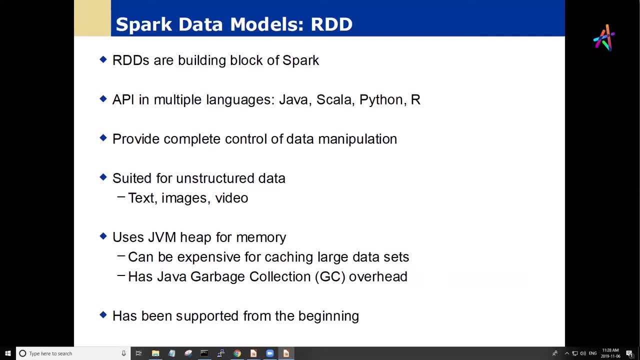 generally you're going to use as RDDs It is. it uses the heat memory. Even with the tungsten optimizing, there is still going to be some problems with memory And we'll take a look at some of those memory management issues next week. 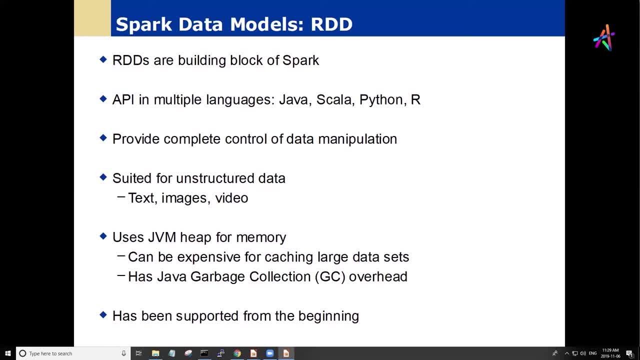 Today we're going to, and tomorrow we're really going to, focus in on the data models and get a good understanding of that. It's because the RDD these are more or less opaque, We can't really optimize a lot of things. 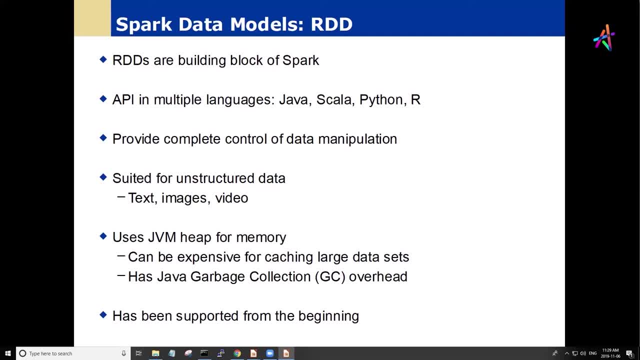 including caching. So we wind up caching perhaps large chunks of data that we could have cached more optimally if we knew something about its structure. But again, for some data we can't do that. So this becomes the. this becomes what we wind up living with. 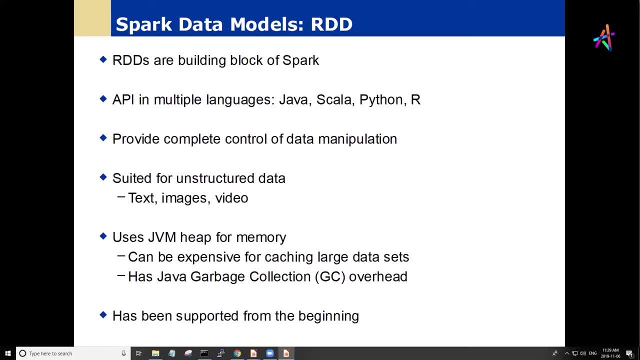 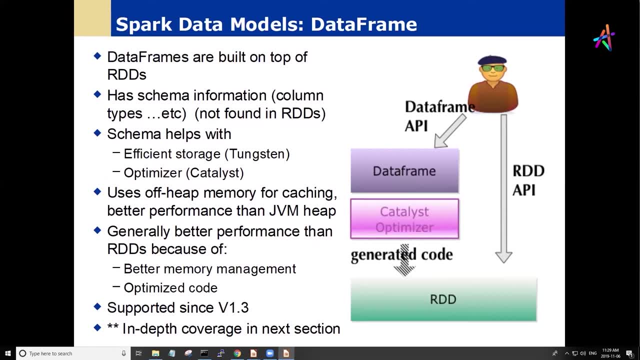 but we can optimize some of these things in other ways. So this is the core. So this is the core of the of the model. Now, data frames are again, like I said, an RDD with an associated schema. All right, guys. 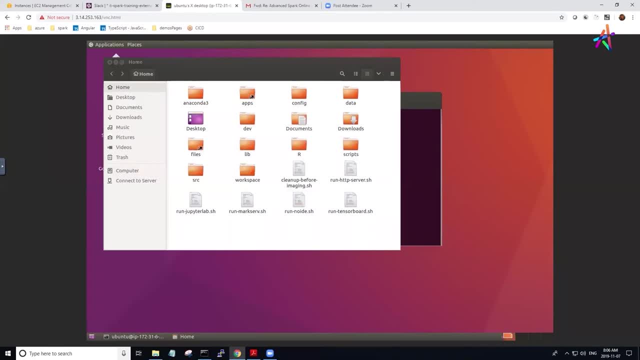 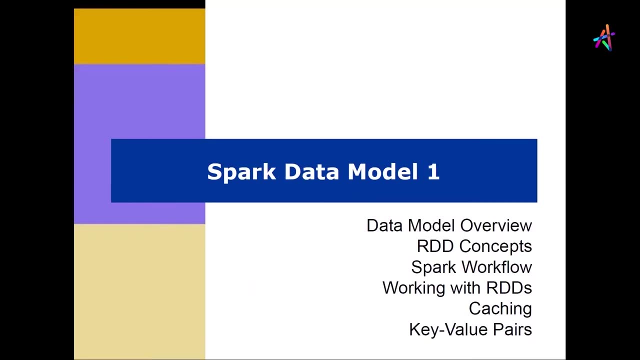 welcome back to the second half of the first day. basically, Let me switch over to my, and we were working yesterday with the with the data model Proceed along, By the way, with regards to that labs repository. I didn't, that's. 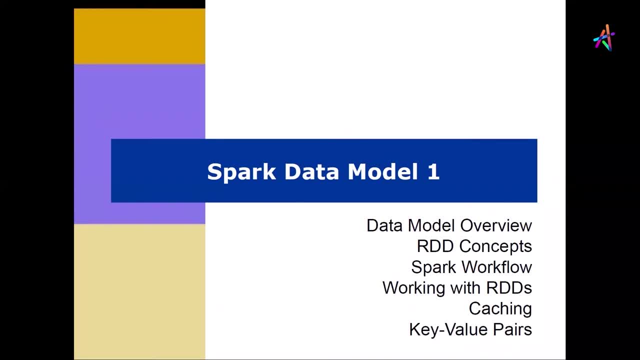 that is a repository that we can access over the machine, But I think what I'll do today, when I have a moment, is I'll make a clonable repository so that you can actually work with them on your desktop as well, because there are some documents in there that you might need. 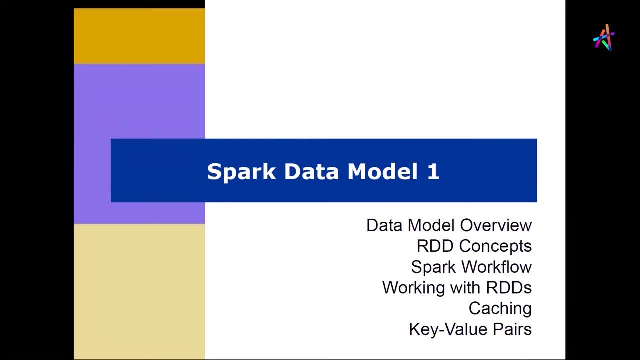 So I will. I will attend to that. I just didn't have a lot of time and I'm converting the slides to PDFs, So I'll finish up some of those slides again as well and pop them in the repository and then give you an update. 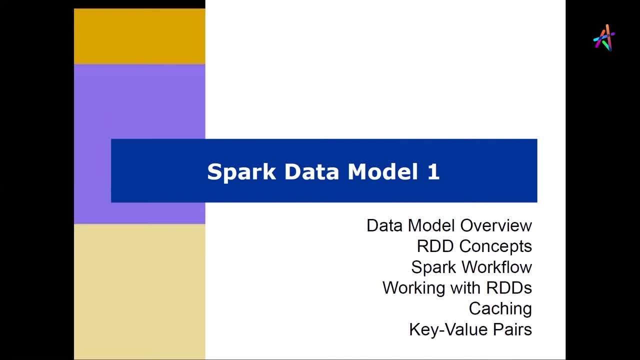 so that you can do a poll and get the slides And if there's any other, if there's any other administrative matters you'd like me to take care of, just shoot me a message in Slack and I'll. I'll take a look at it. 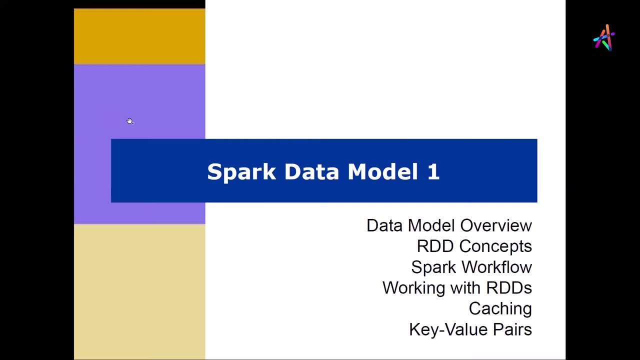 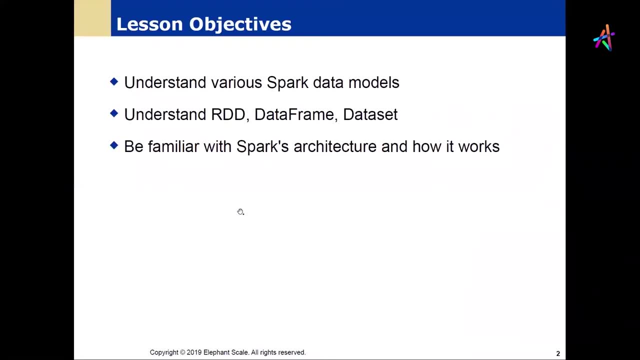 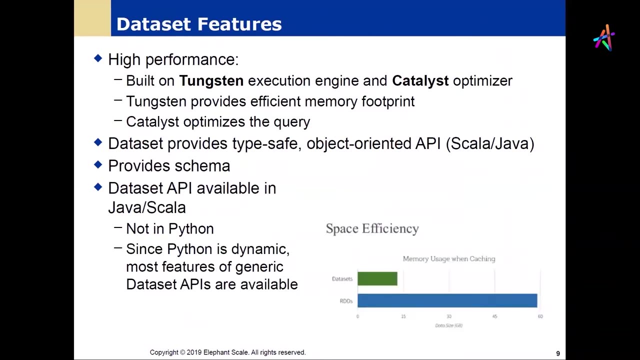 All right, Good. So we started talking about the, the data model, yesterday. I want to close this off And this is: I think we got through these concepts here of this, these interfaces, And I believe we got certainly to there. 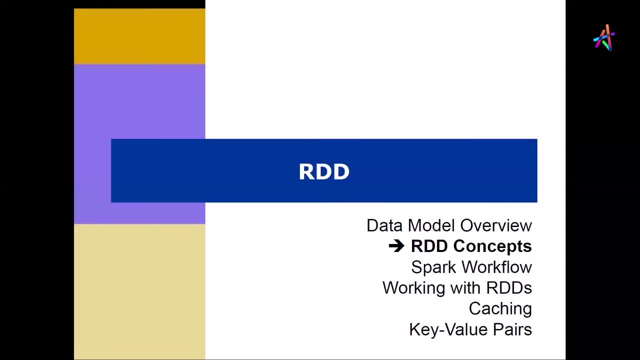 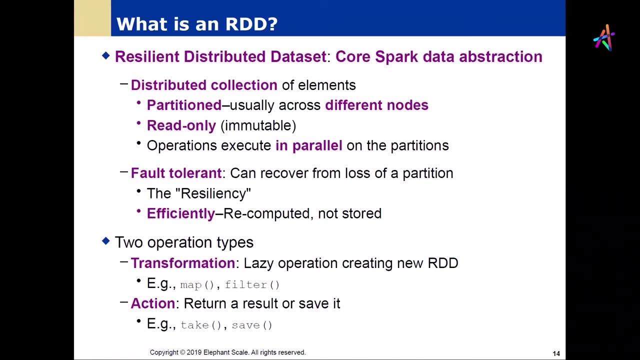 Okay, All right. So we did that first section, the data model overview, and I believe this is where we got into the. this is where we sort of left off. So first of all we will ask: are there any questions from that? 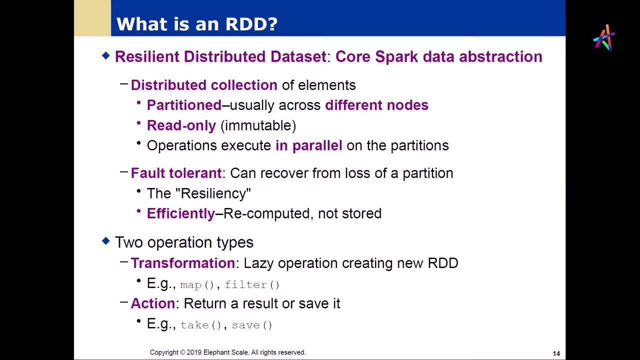 from yesterday. All right. Now this resilient data set- distributed data set is- is an abstraction that formed the core of the original Spark release, And the idea here was the that you are not directly interacting with the distribution model, So it is distributed. 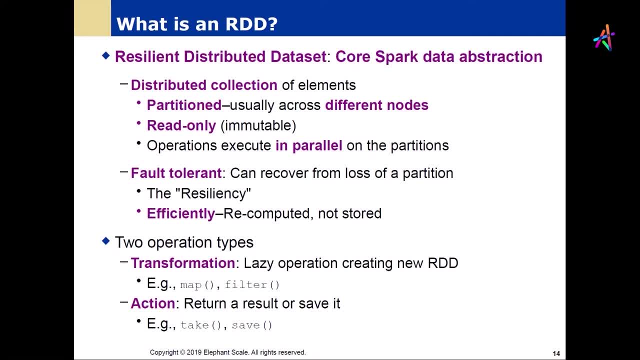 and across multiple nodes. but because Spark is not doing the management, it's delegating off the. it's delegating off the management of the data and the various partitions to whatever manager is there, So it doesn't have to have a multiple nodes to work. 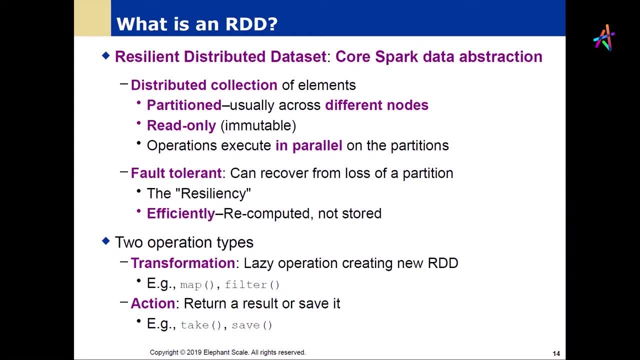 It's going to look transparent to you, because what you're really doing here is saying what you want to have done on the data, not how it's going to be managed across the nodes. We get into tuning, then we can alter the parameters. that will, in fact. 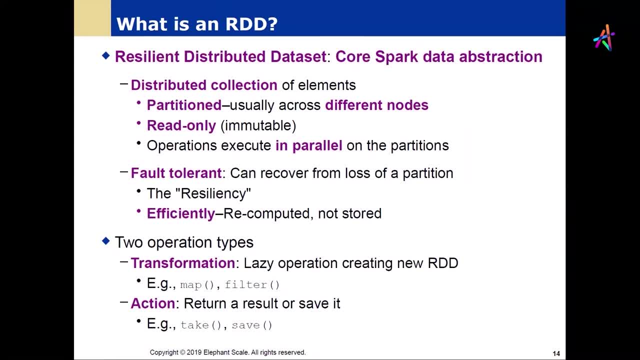 work with that and enable us to tweak how that actually is working by by supplying various tuning parameters And we'll take. we'll be taking a look. I think most of next week I was going to be looking at the the 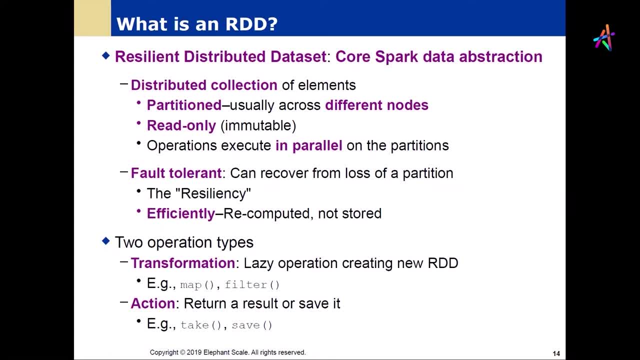 the specific ways that we tune Today really we're going to get trying to get the big picture, especially for those guys who are new to to what's going on with with Spark. So the distributed collection, the distributed part, means it's partitioned. 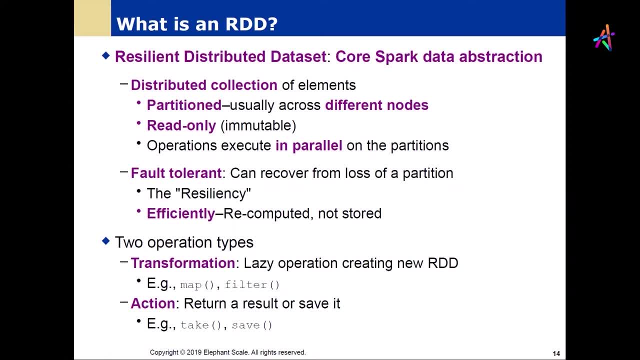 usually across different nodes depending on the manager. That's transparent to you. It's also read only, And there is a reason why it's read only. It's a. the influence of that is, of course, the notion of immutable in. 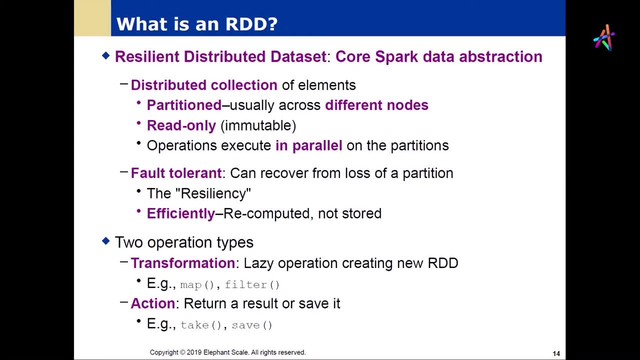 in the underlying Scala, which is is written in, but it gives us an opportunity to do optimizations. In fact, it's the fact that it is read only is one of the reasons why this in fact works as well as it does. The operations are executed in parallel on the partitions. 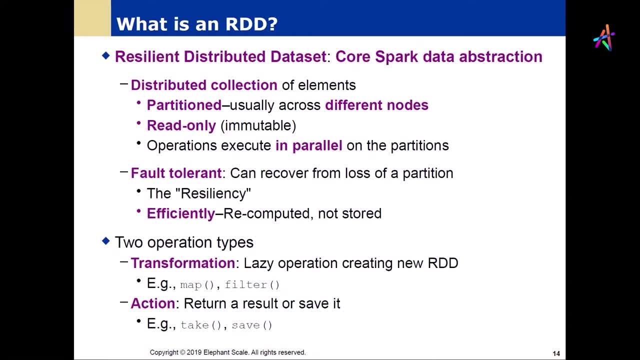 same as you would expect for the standard kind of big data partition, MapReduce. That's all managed at the infrastructure level. It's fault tolerant And that is where the that is where we get the, the read only property being highly supported, because if you are having a read, 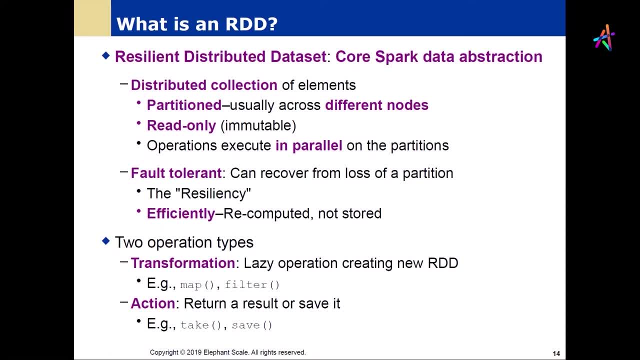 only set and you lose part of it. you can reread part of that set. If you have a set that is mutable and you get a loss at some point in the mutation, then it's very difficult sometimes to go back. Maybe you can. 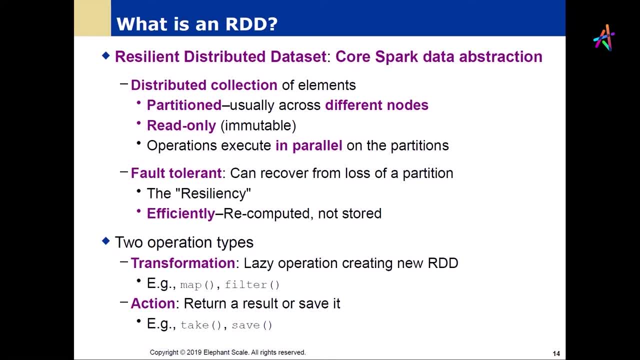 but it's very difficult to go back and reconstruct the set before that mutation took place And that's, and so that's more of a theoretical level. but the idea is that this, this ability to have an immutable data frame or data set- 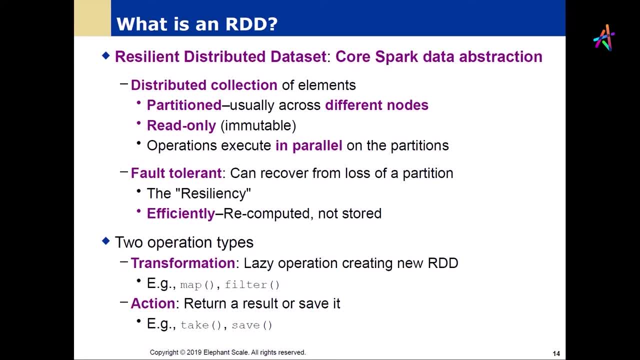 I'm going to not use those or an art, I'll call them RDD, So I'm not going to confuse them with the spark data sets. to have these RDDs being read only gives us a lot of capabilities to do this failover, Because we can recompute. 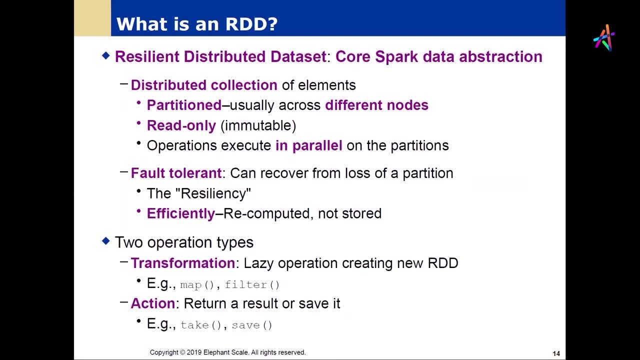 not stored. We can get to that, to back to that state that we were in before we had a, a, a failure, and we can do it fairly effectively. So this is done efficiently, So we're not going out and fetching stuff. 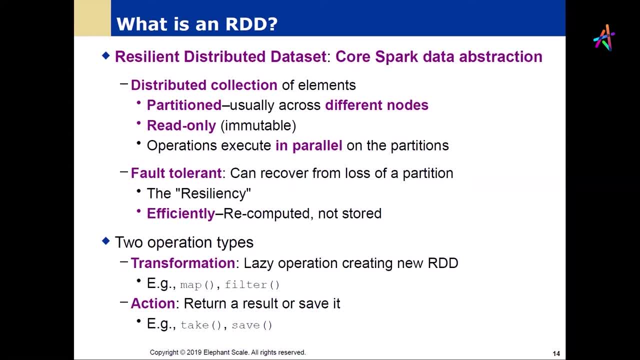 We're? we're basically just recomputing what we've got to to replace the- the missing data, When the key to the, to the optimization at the RDD level is that we've got to replace the- the missing data. So what we're going to do in this example is that we break. 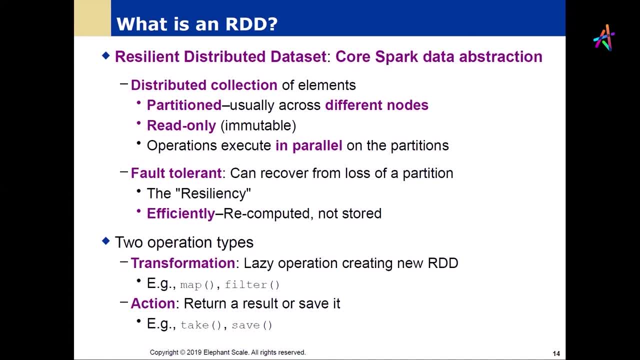 down the the things that we can do with an RDD into two kinds of operations: transformations which are not actually executed when we invoke them- In fact, they stack up- and what's called an acyclic directed graph And we don't do any mapping or filtering or things that transform. 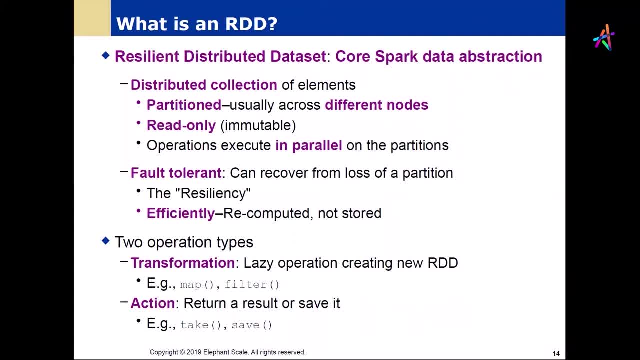 data into some other form, We actually have to return a result and that's called an action. So when we finally have to get the delivery, say: now we're going to, now we're going to, to, to, to take the results. 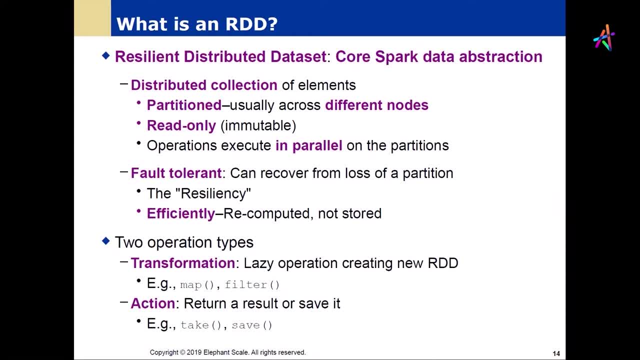 we're going to save the result, Then we go and we execute all of the transformations, And the reason for that will become apparent in just a moment Now, the. the analogy that I heard from when I was kind of delving into Spark is to: 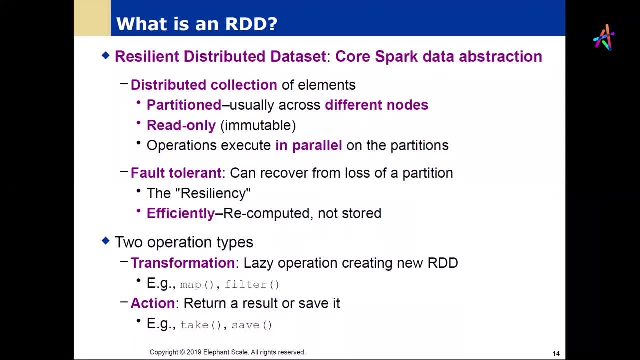 to kind of uh uh, crystallize this. this, the concept behind this algorithm is: if you are running a kitchen- uh, in a, in a, in a fancy restaurant and you have an order comes in for a particular 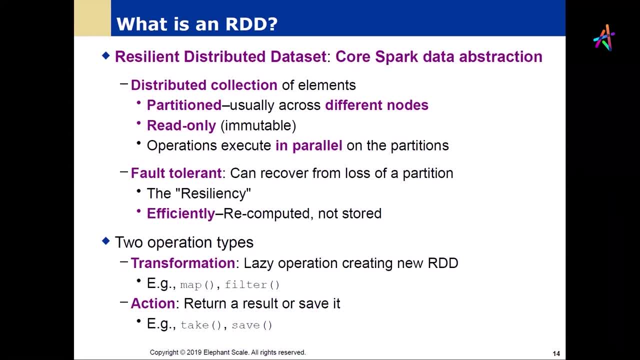 uh, uh. for a particular um meal, you're going to have a group of people coming in and they're going to have a banquet and they have a menu. So what you do is you don't cook the meal at that particular. 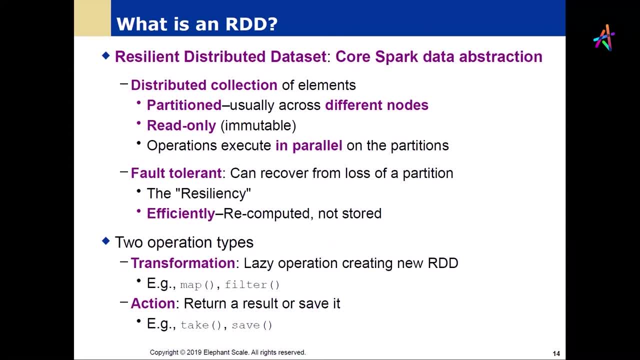 point. You basically sit down with your staff and you figure: okay, if I'm going to cook, you're going to do this, you're going to do this, then you're going to do this, And you, you run out a whole action plan of what's going to happen. 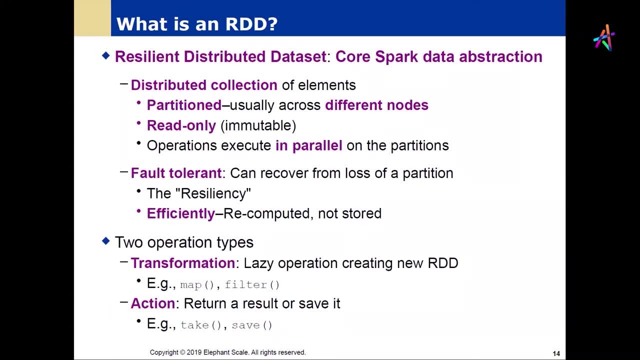 And each person will have their step written out. They'll know exactly what to do. but there's no point in doing it because nobody's ordered the meal yet. Then the people come in, they order the meal, then you put your plan into effect. 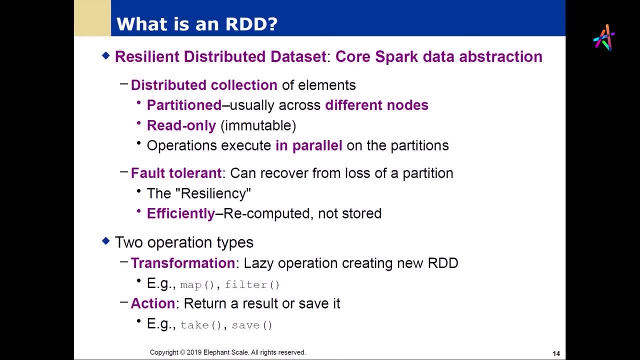 And the thing about the plan is that you may, as you're developing, and say: oh, wait a minute, there's a more efficient, efficient way to do this. So this is kind of an analogous idea. is that when we're we're doing these transformations, 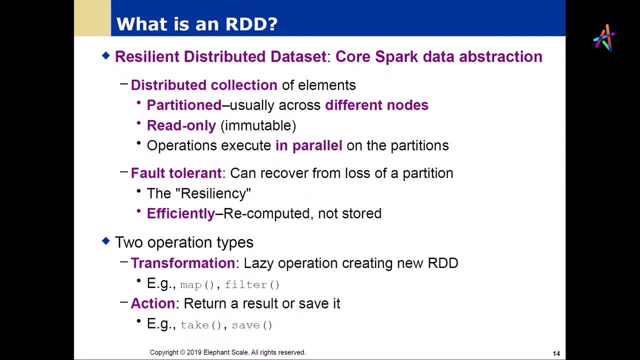 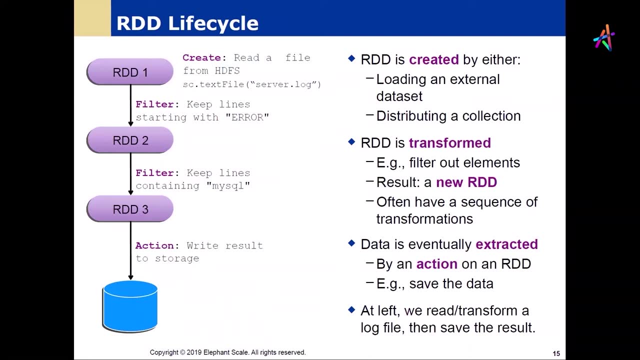 we're just documenting what we're doing And then we're going to actually go and execute them only when we actually need to produce a result, And that gap gives us the the opportunity to do some, to do some optimization. So here is the example of the 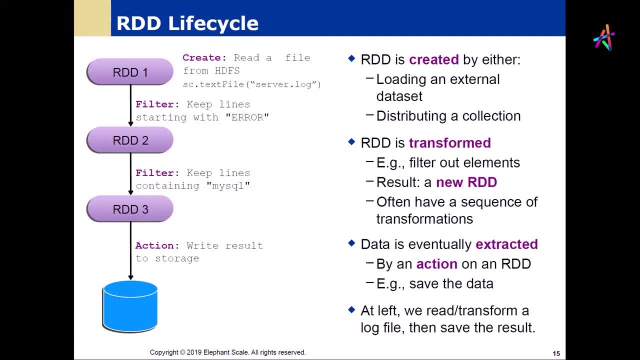 of the of what we might call the life cycle of a resilient data distributed data set. So so we will usually create it in one of two ways: We'll either load it from an external data set or we'll do something called distributing a collection. 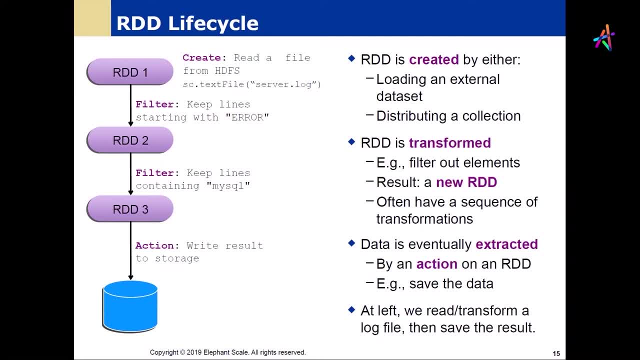 And that is where we take a collection of data And we we basically allocate it out to the, to the distribution manager, to say, okay, distribute this parallel, parallelize this distributed out for me, And we wind up with a collection that's being distributed. 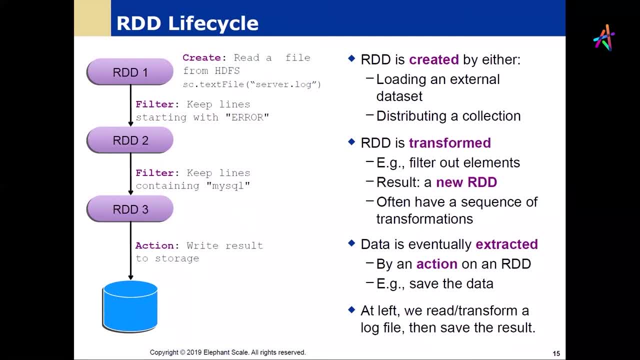 So the data is created. Now we go through a series of steps which describe what we're going to do with the data. So the first step in the in the process- and you can see this already- sort of looks like a directed graph. 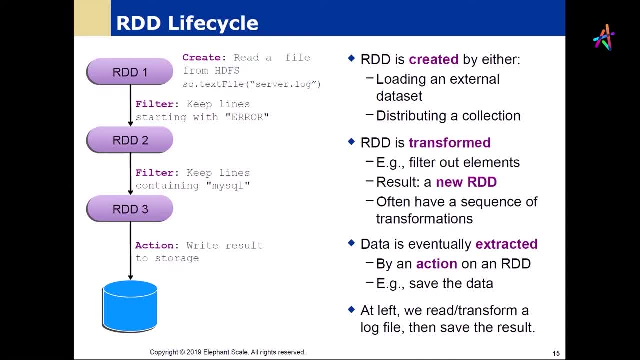 is. the first step is is: we've got a log file and we only want to look at the errors. So we're filtering out all the lines starting with error and we're reducing the data set. Then we're only interested in my SQL errors. 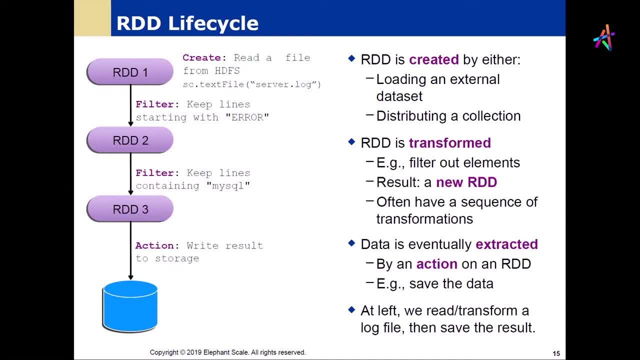 We filter again and then we get the data set, And then we filter again and then we get the data set, And then we filter again and then we get the data set, And then we get the right result to storage. It's. 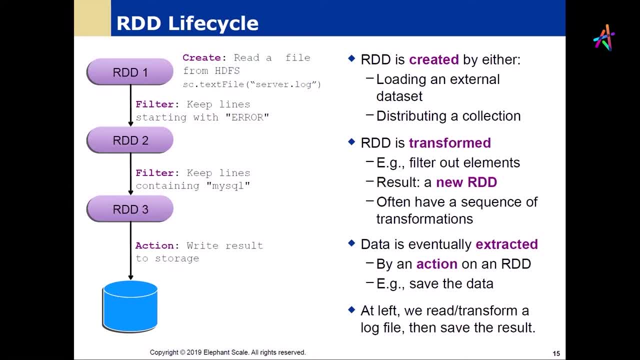 so the transformation in this case is doing a couple of filters to filter out only the data that we want, based on a couple of criteria. Nothing is actually done until we say write the result to storage. Then Spark goes and executes the three RDDs that are: 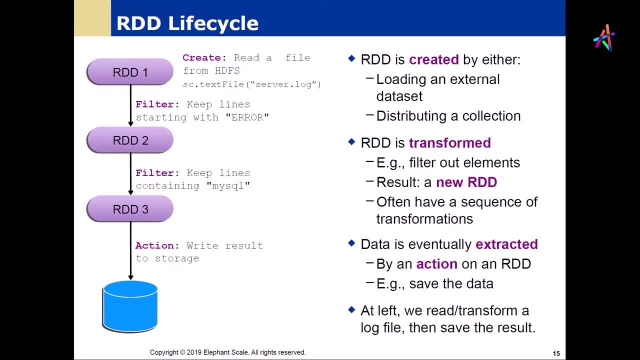 are the three steps in in working with the RDD. Conceptually we think we think of three RDDs being created. So we think that RDD one we filter and we actually create RDD two And then we filter it, We create RDD three. 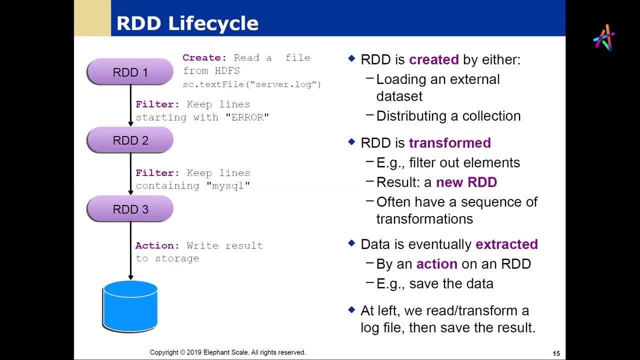 That's not actually happening. That is done at a conceptual level as we think through the stages and the transformation. So there's not actually three data sets necessarily being created. The what's happening behind the scenes is that we're we're executing a sequence of actions on a particular resilient data. 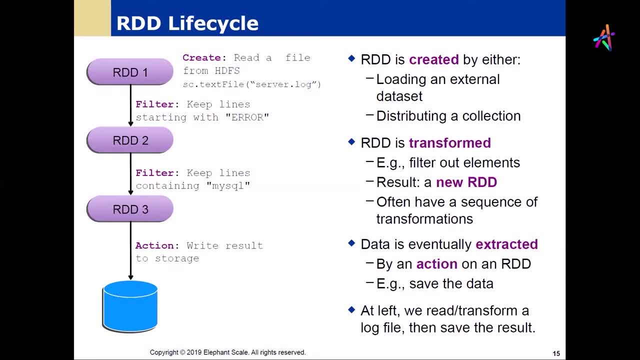 set And we're not. we're not creating multiple, multiple data sets. So there, and that's what's one of the optimizations is going on. So it looks initially like we're creating all these copies of the data set. We're not really creating copies of the data set. 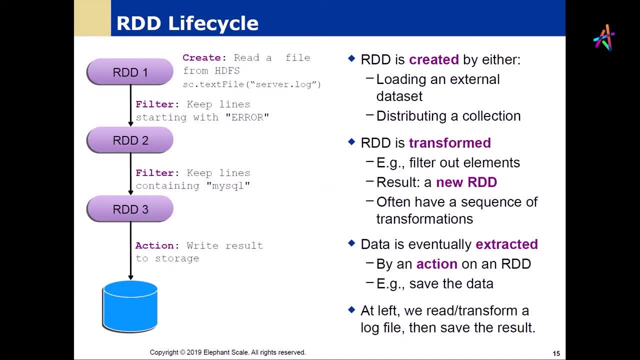 What we're really doing is specifying what we want to do on the output. We're visualizing the output of one of the transformations as an RDD at the, at the, at the logical level, And then we're going to think: well, 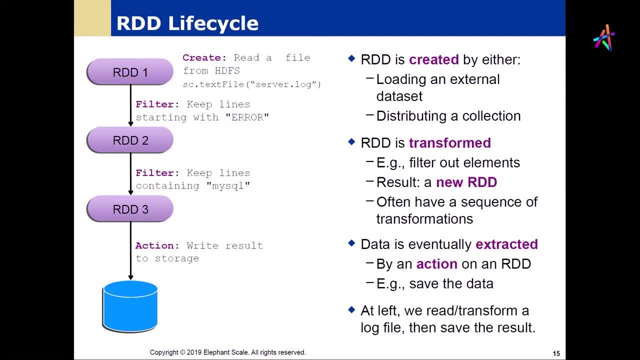 what can we do with this? So each RDD represents the output of the previous transformation. Okay, So this, this, this is this- can be kind of confusing for people as we, as we, as we start off, So this engine does not immediately compute the results. 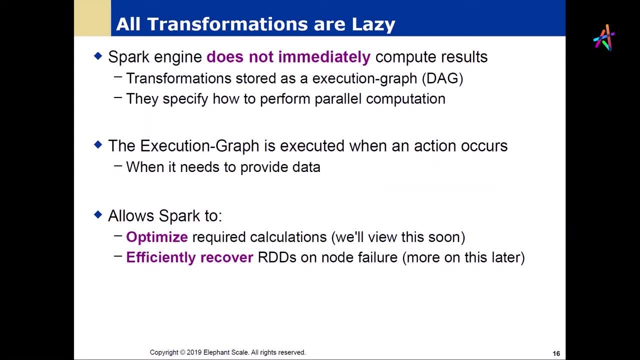 They're stored as an execution graph, which is our directed acyclic graph, And then they specify how to perform them. This specifies how to perform things in parallel. So the this, the graph, is executed as an execution plan when the action occurs. 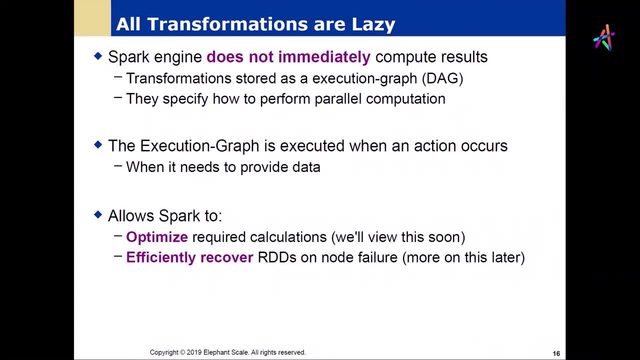 That's, and this only happens when something needs to be done and returned as a result. So this allows Spark to do a couple of things, And one of the things that we're really interested here is is: can we? how does this help us do an optimization? 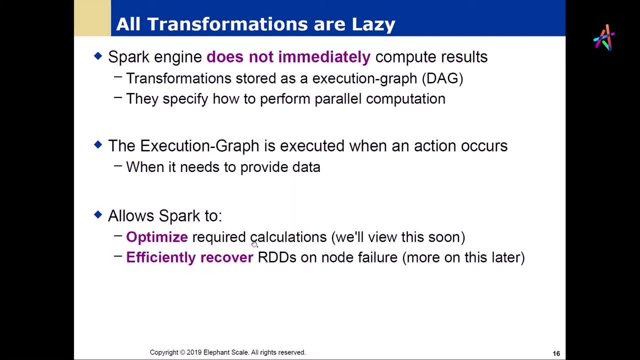 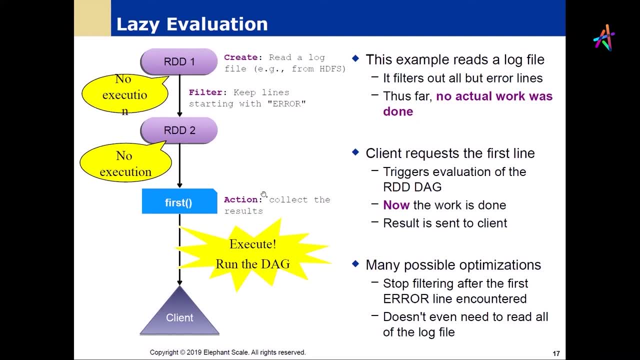 And we can also do an effective recovery. So we'll take a look at those things in turn. So here's the example again. excuse me for a second. I apologize for that. I'm just getting over a cold. I don't want to cough into the microphone. 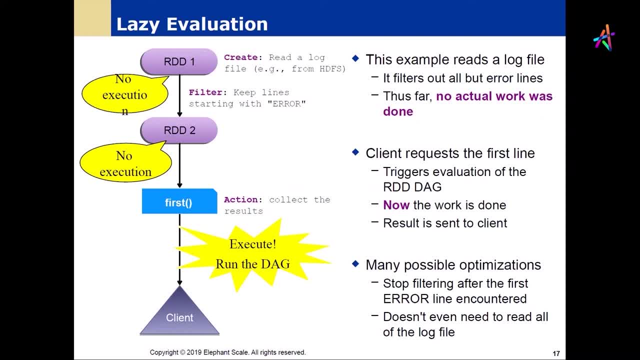 It's just rude. So this is what I mentioned here Again, it reads, reads a log file, filters out all but the error lines. It doesn't even read the file at this particular point. It's just specifying something it's going to do. 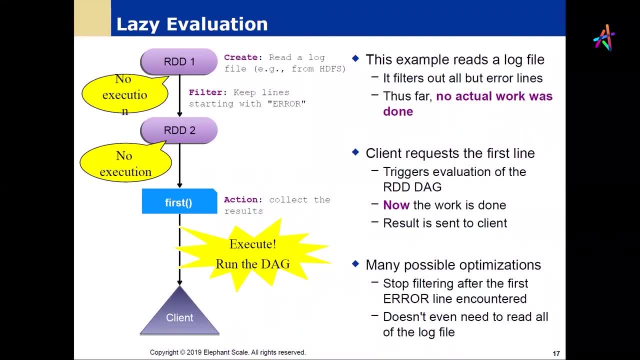 And if you actually go and read a non-existent file, you won't get an error If you're doing this. let's say, for example, in the in the REPL loop. So if you in the REPL loop you say: 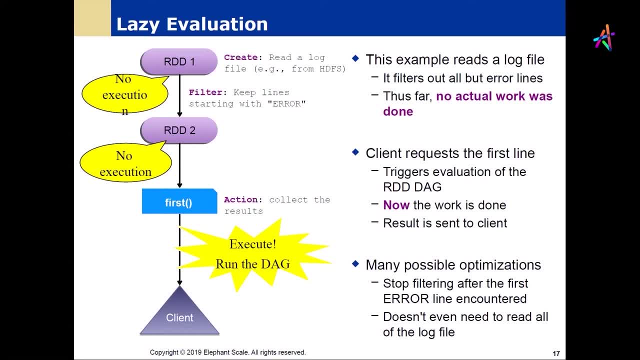 you know, get text and read a file in, but that file doesn't exist. You won't get an error because nothing's been executed at that point. And then you perform a transformation and everything looks good and everything looks good. And then you finally get to the end of the point where you say: 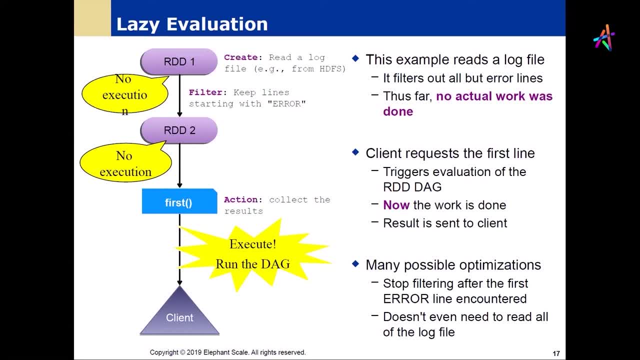 okay, now give me the first, give me the top element of this. Then it goes back and starts to execute the operation, And it's that point that you're going to get the error that that file doesn't exist. So this is: 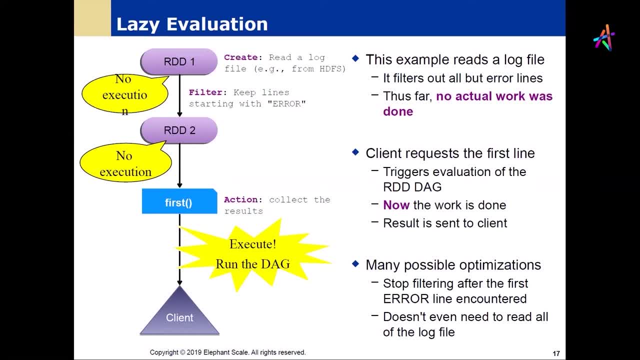 this is the, the manifestation of, of what's going on behind the scenes with these, with this, with this lazy evaluation, And this is this is a key concept. So the no actual work is being done in either of those two steps. 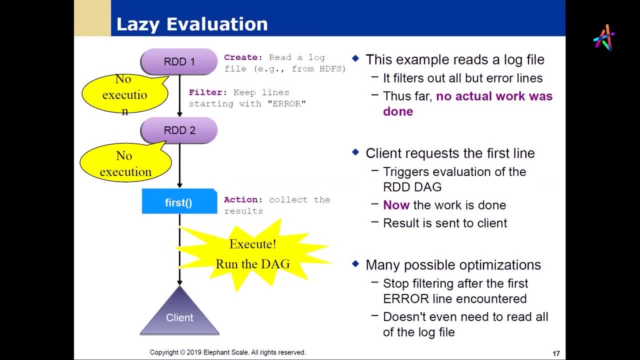 So there's no execution in either of the filters, because it's just talking about transformation. As long as the operation is only transforming, transforming the data in some manner, there's no need to execute it. It's only when we actually get the action that we have to produce something. 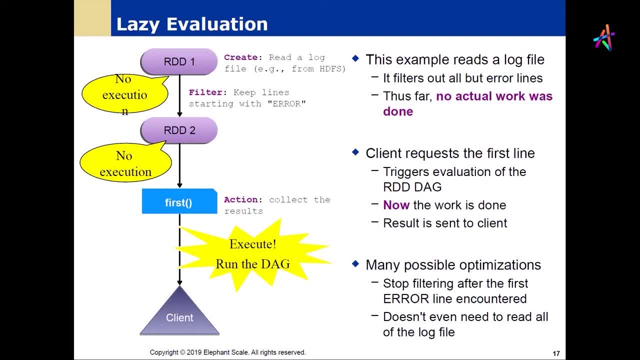 that triggers the execution. So, the, so the. there's a lot of different optimizations that can be made on here, So we could, if you notice that, that look at the look at the look at the sequence of actions that we're doing here. 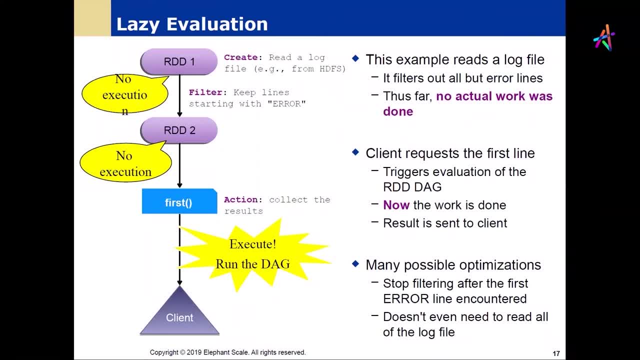 So we've got a log file, Maybe it's a couple of gigabytes, And we're going to filter out all the lines with air. So maybe now we're down to a couple of hundred megabytes And then we say we only want to find the first line of that. 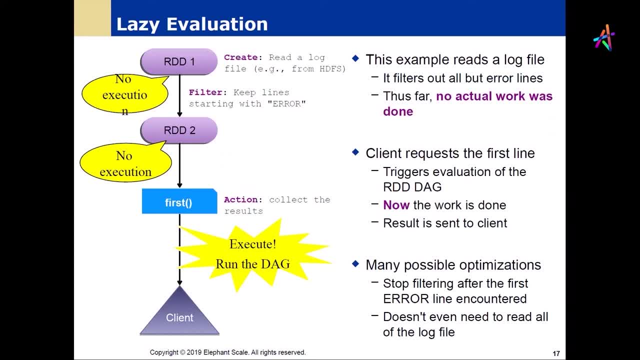 of that filter data set. Okay. So when you stop and think about it, well then, why am I applying a filter to everything in the log file? There's a better way to do this Instead of reading an entire multi gigabyte log file and then transforming. 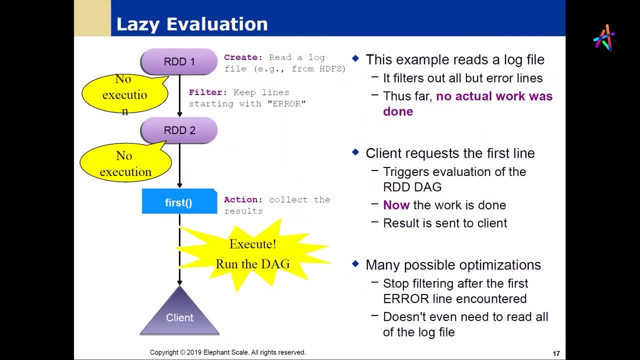 the entire file and filtering the entire file. maybe I can re-optimize this and just say: read the file in until I encounter the first error record And then just return that. avoid all of this kind of work. So these are the idea behind an optimization by analyzing: 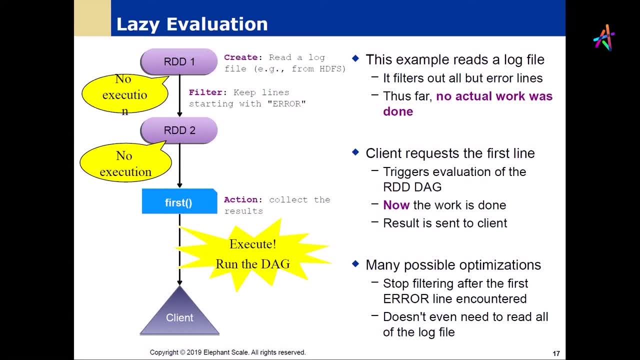 and that optimization is not apparent until you look and see what the action is that's requested. So now, knowing that we're only going to be getting the file, we're only going to be getting the first element back, Now we have to go back and rethink what these transformations do. 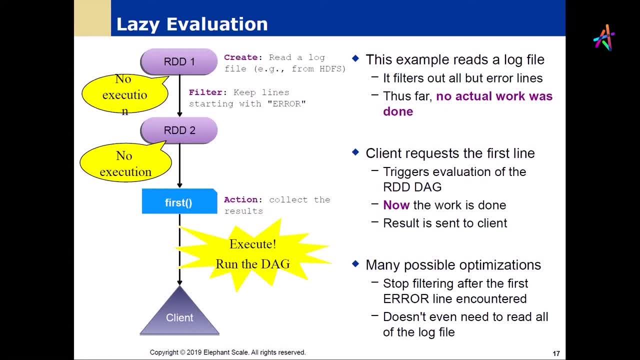 and we can get a much, much more efficient way of producing the result rather than blindly executing each step in turn. So this is the idea behind what the what this lazy evaluation does. So one way at first. so the sequence of actions that's taking place is that all of the 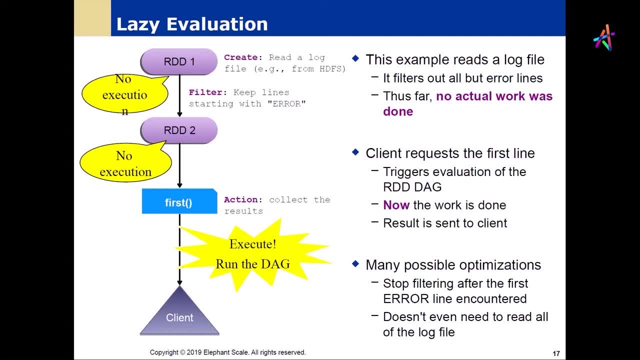 all of the steps up to the first action are creating a work plan, a list of tasks to be done, And then, once we encounter the action, we can look at the work plan and say: is there a better way to organize the work other than what was specified? 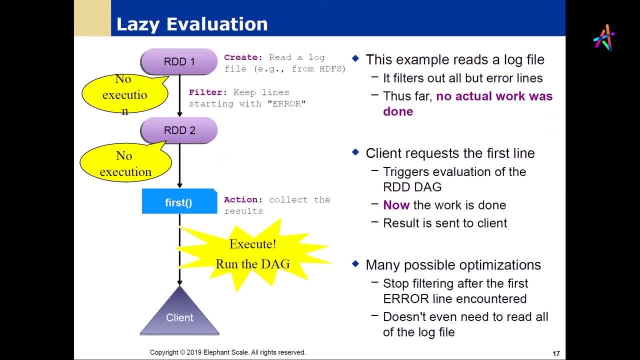 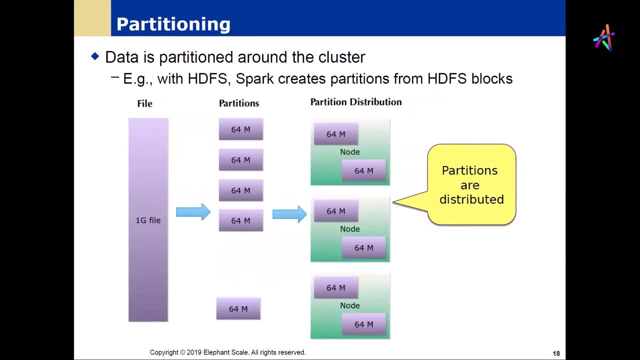 by the client, And that's where the optimization takes place with the RDDs. Okay, So that's. that's what we're talking about here. The, the data is partitioned around the cluster, So while we're doing this, we've got a bunch of partitions and they're distributed onto various nodes. 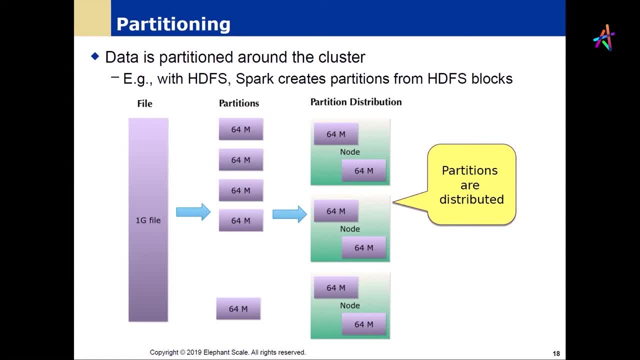 The partitions are distributed, How that partitioning takes place. Again, we saw from yesterday that Spark has its own manager, but it generally tends to sit on top of other other node managers, And so that's that's fairly opaque to. 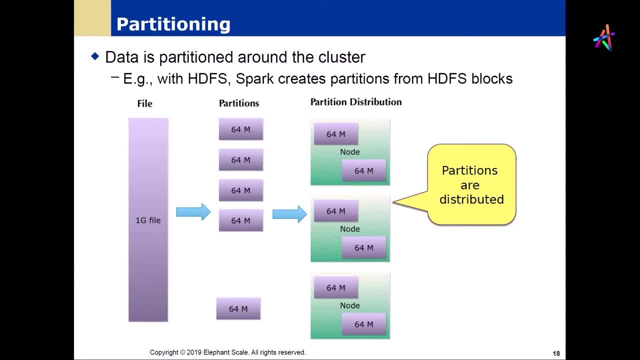 to to the, to the actual Spark engine when we're building it. But when we come into the optimizations these things are going to be taken into into account. So we've got distributed partitions. We take our file, divide it up into partitions. 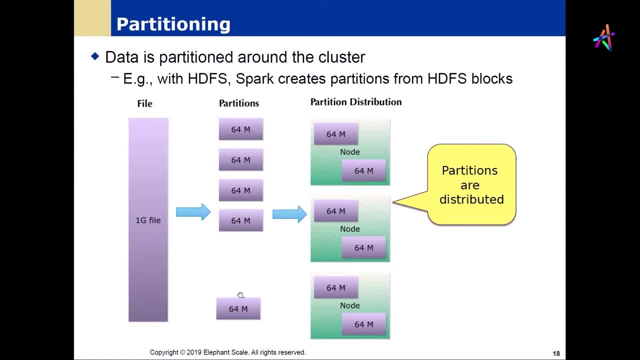 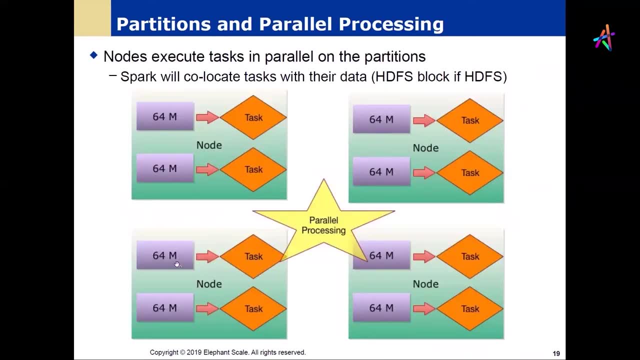 This is a fairly standard model- I'm sure you're all familiar with it- And we distribute the various partitions onto the various nodes. The nodes execute the task in parallel on the partitions, So we'll we'll basically co-locate the tasks with. 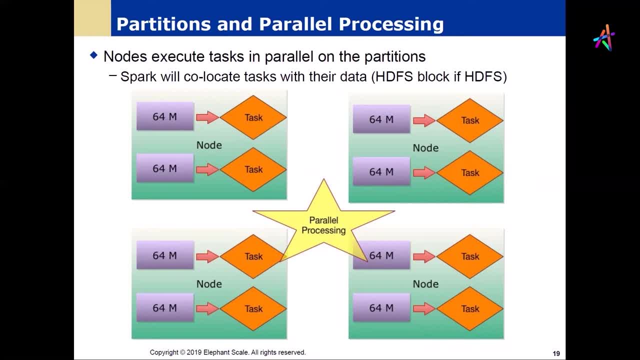 with the nodes. So, and then we perform a parallel, which is what we would expect. This is the whole idea behind the distribution, The distributed part of the resilient, distributed data set, is that we now have an underlying mechanism that goes and does the parallel processing, for. 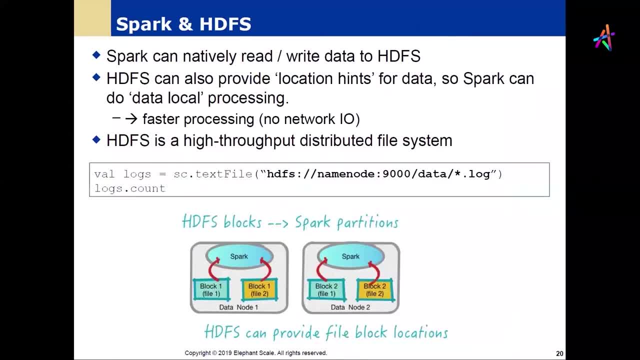 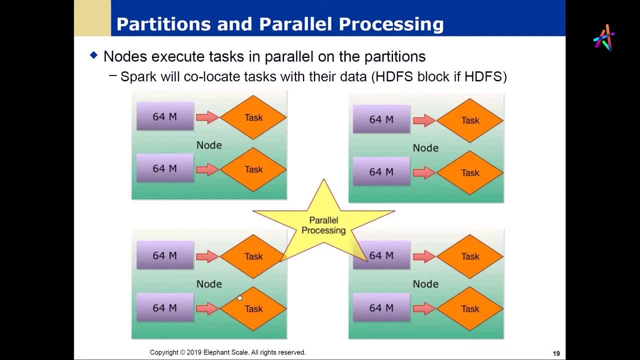 us Okay. So- and this will come to a point we'll look at later- is that this: when we're doing the processing, we may discover that the way the data is distributed after we do a particular set of, after we do a particular set of operations, is unbalanced. 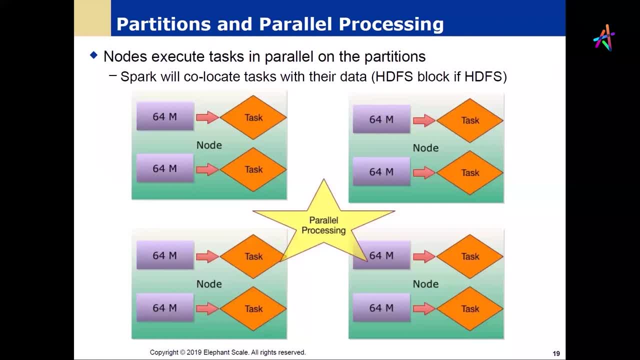 And we'll see an example of that later And at various points we'll execute something called a shuffle manager And that shuffle manager will go and reorganize the data so that we get a more even balance of load. So if we do some kind of filter and we wind up with no data on three of 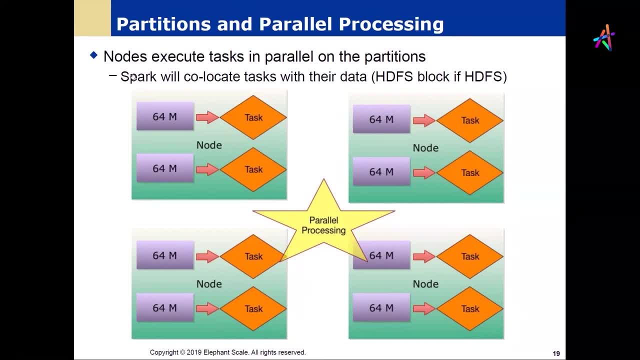 the nodes because we filtered it all out and all the data, for some reason, is filtered on this node. we're going we may want to shuffle things around to take advantage of the parallelism. So the parallelism and the shuffling is intended to improve efficiency. 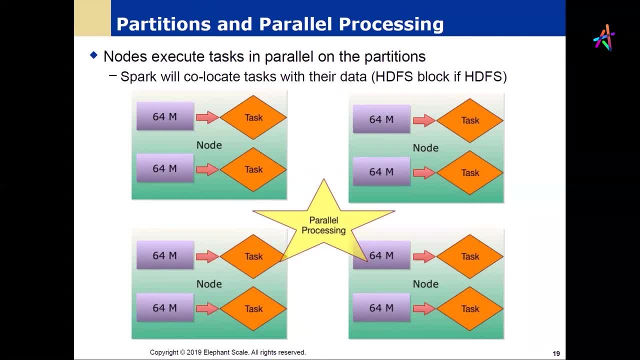 but it it can also be a drag, because shuffling may involve a lot of disc reads, disc IO, which ever again shows, slows it down. So one of the things that will happen is that while we've got this lovely you know- 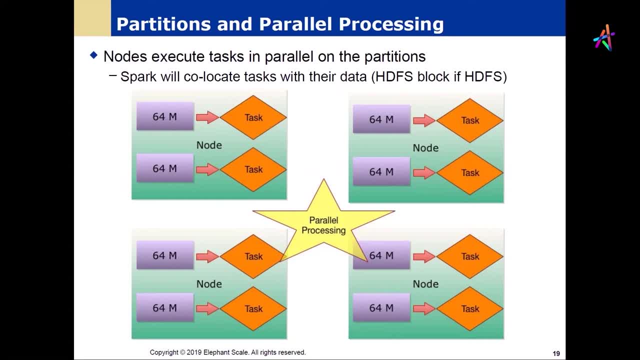 everything going in memory. that model can be a little bit difficult to to implement completely when we've got to do a bunch of shuffling. So we'll get into shuffling later and we'll get it. look into optimization on shuffling and we'll see how. 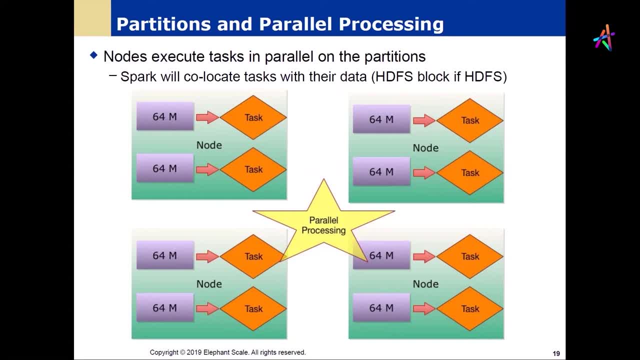 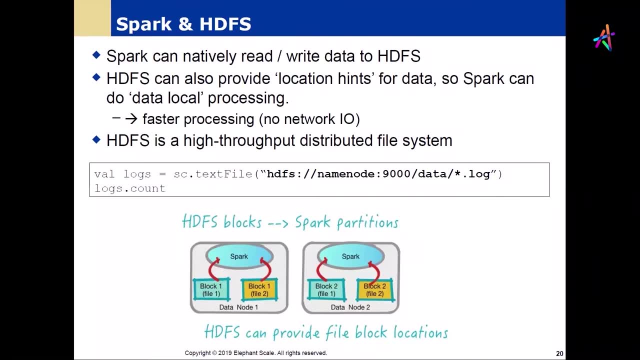 how we can optimize the various kinds of shuffling algorithms that are there. So we'll, we'll turn to shuffling. So Spark, again, is basically designed to sit on top of of a Hadoop file system and Spark can can take the hints from the 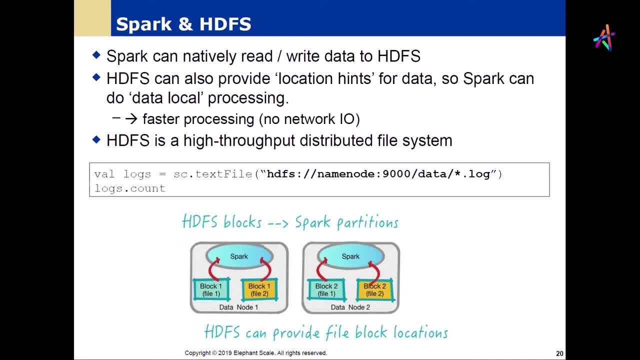 from the HDFS and do local data processing. So it the idea here is to is to is to optimize the operations based on on where the data is located. So if we take a look at that line of code, this is a work in Scala where we're using the SC. 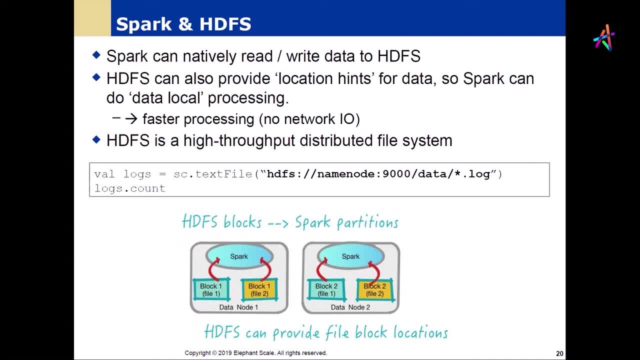 Now what the SC is- we'll get back to that in just a moment- is something called a Spark context, And I'm sure you used to using context objects in a number of different programming environments where the context object basically is an interface into a set of operational 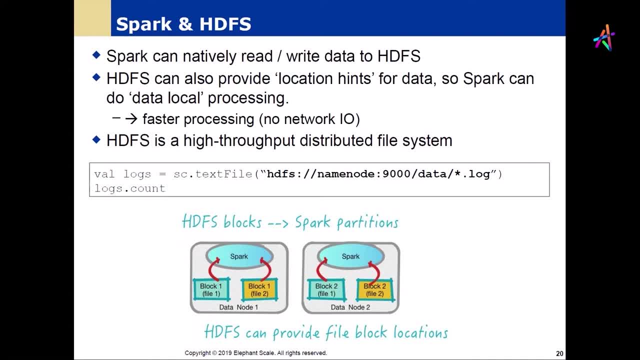 operational subsystems. So- and we'll see that this actually SC- has been replaced by a a, by an object called Spark, which implements this functionality but also implements other functionality as a result of having moved from this model to the unified data set model. 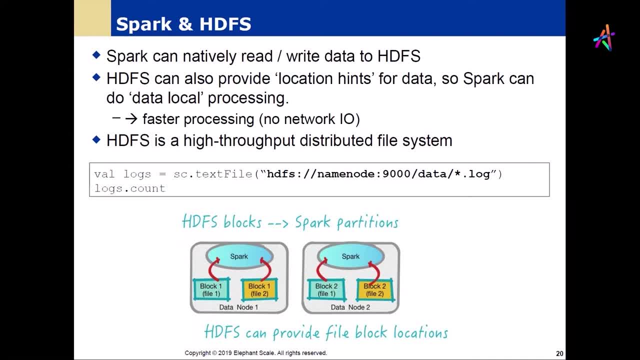 So the. so there is a, so the, the. so that first line logs SC text file goes and is reading in a text file from the Hadoop file system And that is not executed immediately, And then when you execute logscount. 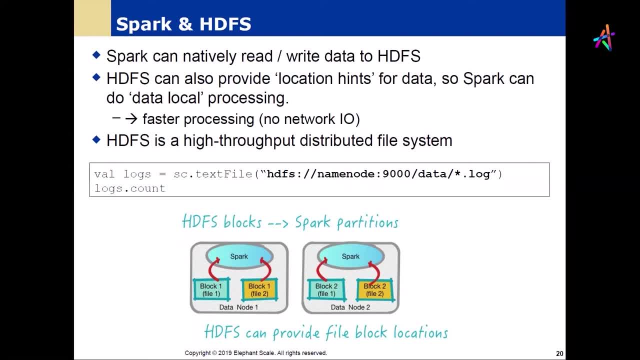 which is going to give us a count of the number of lines in the log file. at that point, the text file command is actually executed If you've given it the wrong URL at that point, if there's, if the file doesn't exist, in this particular case, 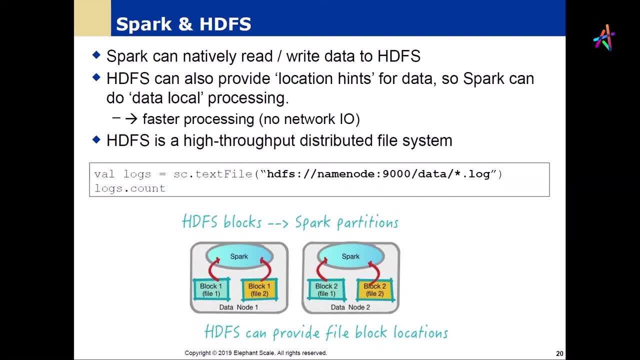 we're reading a collection of log files into one big. So we've got a bunch of log files sitting on a note and we're creating a single RDD. Logs in this case is a resilient distributed data set, So logs. so reading the data in and assigning it to a variable creates the RDD. 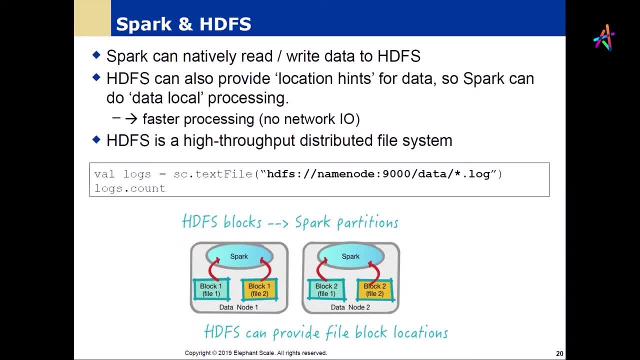 So logs is now an RDD and we can execute actions and transformation on logs. So in this case we're executing the action count, which is now has to return a numerical value which is going to count the number of lines. So the 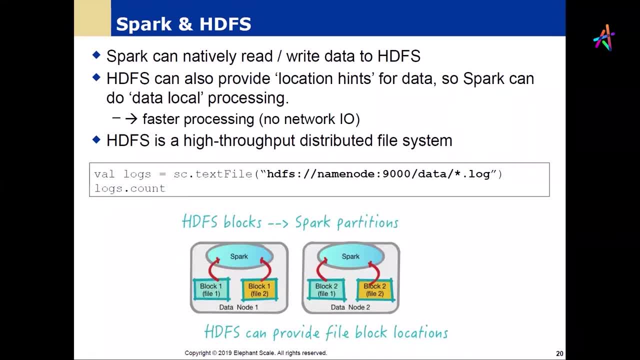 so again we, because Hadoop preceded Spark, Spark was able to leverage its interactions with Hadoop in order to take advantage of the information available from the Hadoop, in order to figure out optimal ways, or better ways, or efficient ways to distribute the data. 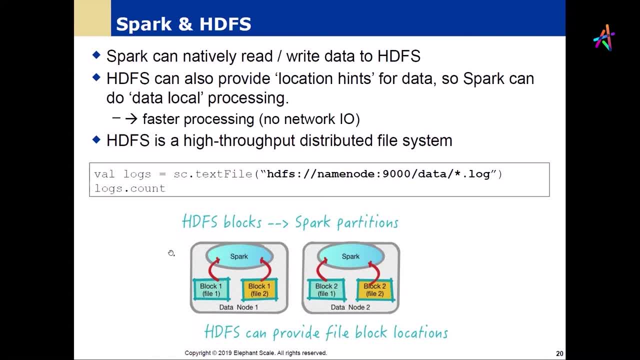 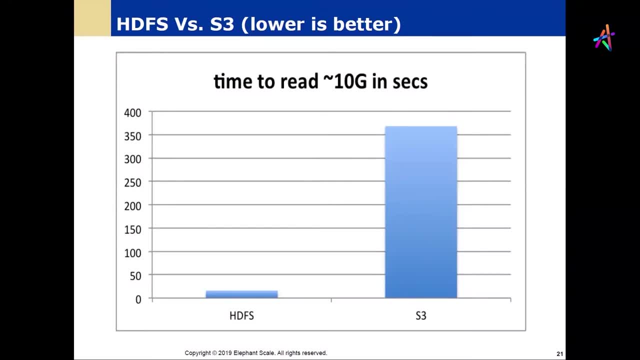 So when? we'll come back into those optimizations later on. Okay, So the the this shows up here. I believe S3 probably refers to an Amazon blob container And we got HDFS on the left. Okay, So what accounts for the difference in this? 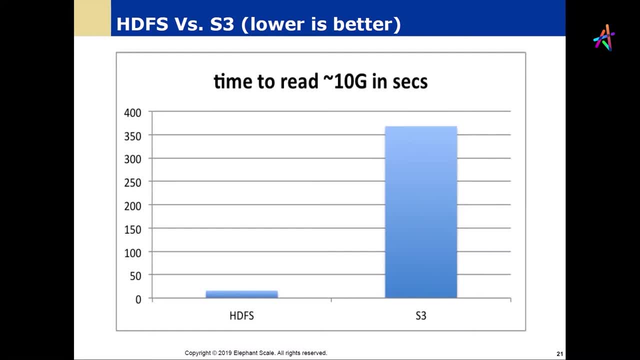 Well, when it counts for the different is is that, as far as the S3 is concerned, Spark is just seeing a big change. It's a chunk of data and the read time is going to be considerably longer. On the other hand, 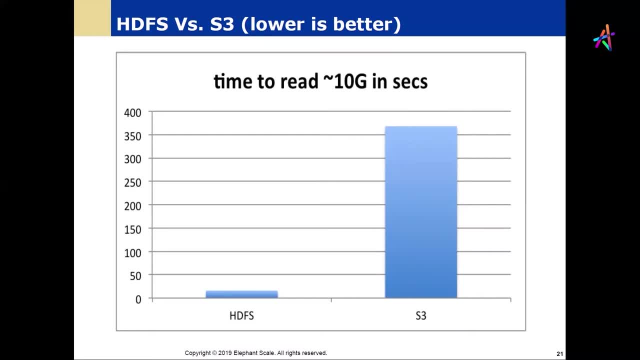 HDFS has a lot of information that Spark can access to read these things in very efficiently And, as a result, you get a much, much better, lower time. So one of the takeaways from this is that, while Spark can operate pretty much from data, 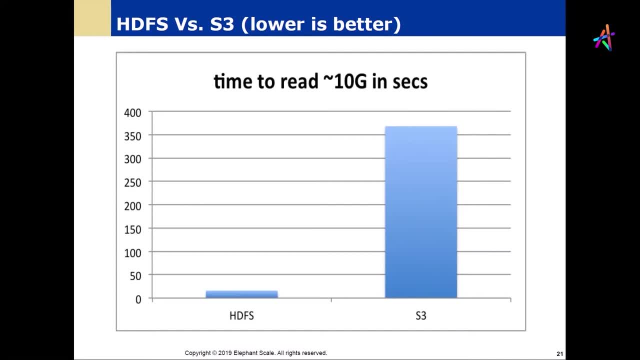 from any kind of data source. where we really really see good performance is that if we, if we are able to leverage some kind of distributed node cluster system like Hadoop in order to process our data, because Spark will be able to use that information to process reads and other. 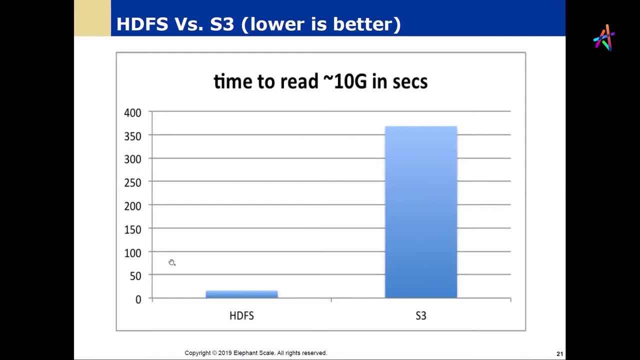 kinds of actions much, much more efficiently. So there's sort of a first optimization, pick a data storage that Spark's really going to be able to leverage, And you're going to see significant improvements in things like IDataIO, The, the. 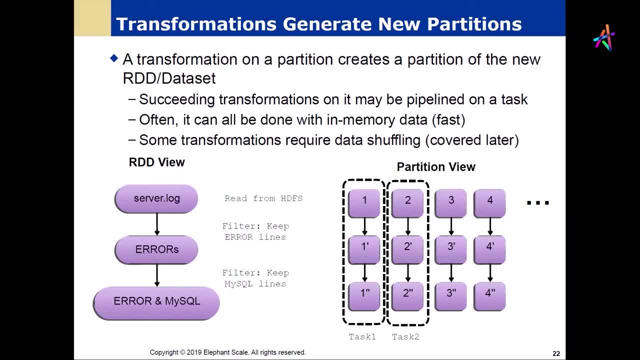 a transformation on a partition creates a partition of the new data set, And then the transformations on it may be pipelined in a task. Now, a task is a job that is run can be run only with only referencing the, the, the data that's in a particular partition. 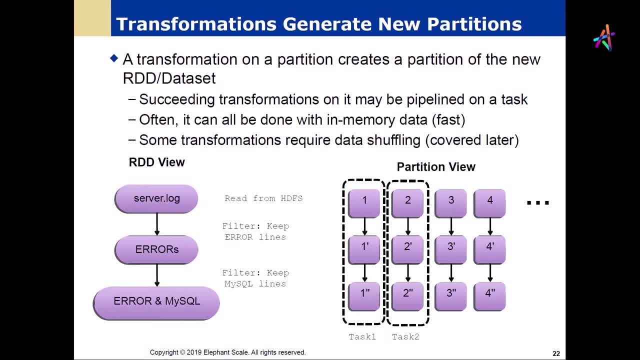 So the, when we look up the, when we look up the- I'm sorry- when we, when we execute the read, then we're, we're basically doing the distribute, we're we basically got information about how that data is distributed. 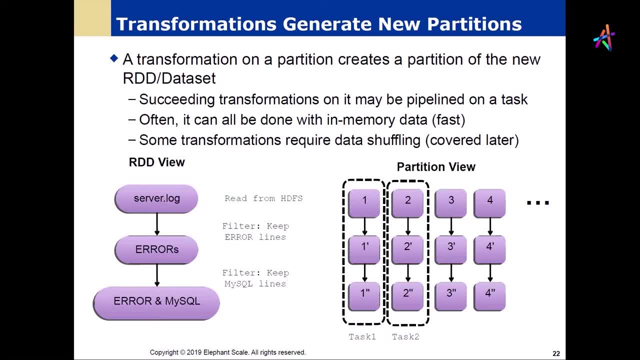 And that action that we're taking on on counting or doing a filter is is now broken down into tasks that run on on a on a single, within a single partition. So the idea is that, once we can break down the tasks in an optimal way, 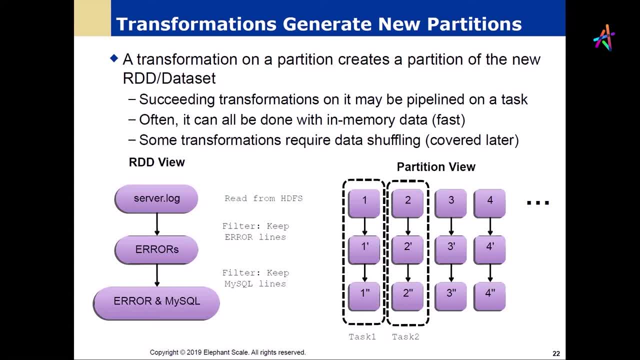 we can, we can, we can improve our efficiency by then doing all of this in, in, in memory. So, in other words, we're talking about the, the importance of staying in memory. Part of that has to do with how we organize the data on the partition. so 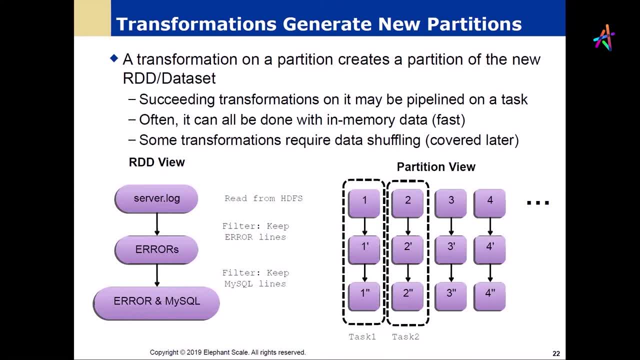 that we don't have to do things like shuffling. So if we can optimize our operations so that they can be pipelined in a task, so that our two options here the the two filters, if we can, if we can get it so that those two filters can operate sequentially within a 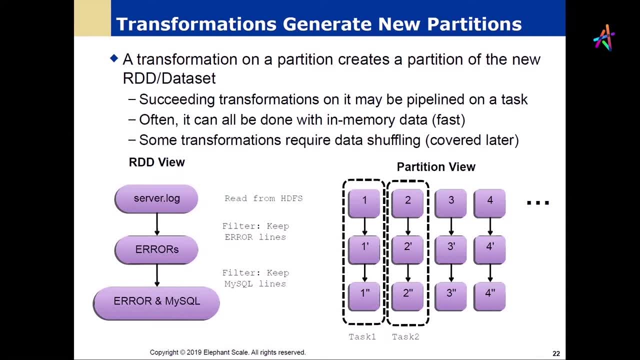 partition without having to refer to everything else as tasks, then we've got a really, really good optimization. So now, now we're seeing one of the challenges that we've got here. Okay, So we've covered a couple of concepts here and we're starting to get a peek. 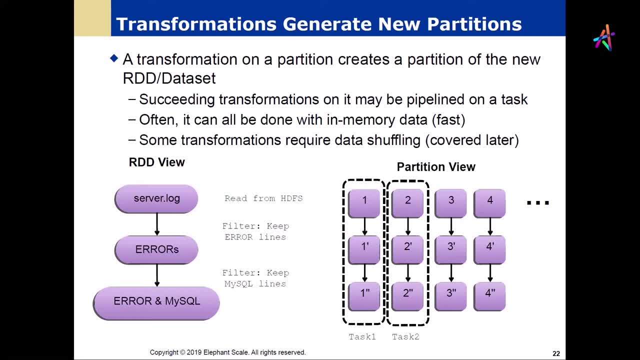 under the hood at what's going on with these RDDs. So, conceptually, when we write the code, it looks like we're just moving, creating all of these new RDDs and moving them around. What's going on behind the scenes? 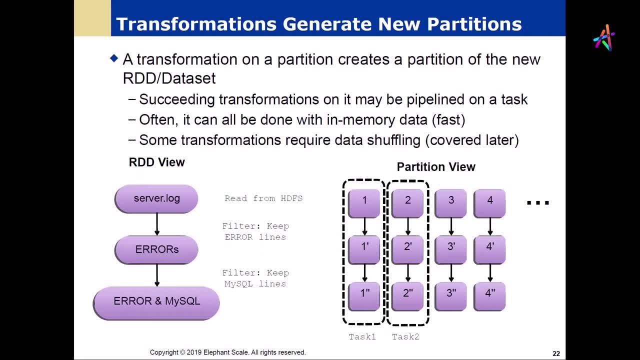 is that that acyclic graph directed graph has to think in terms of where the data is located and how can we organize these activities so that we can break a single transformation down into a bunch of tasks- each task running on a partition- and and pipeline it so that we don't have to stop and reorganize the data. 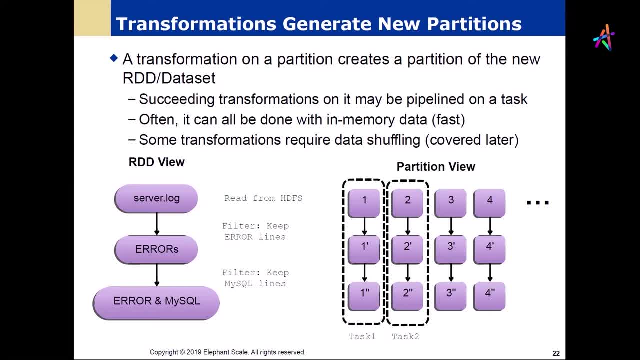 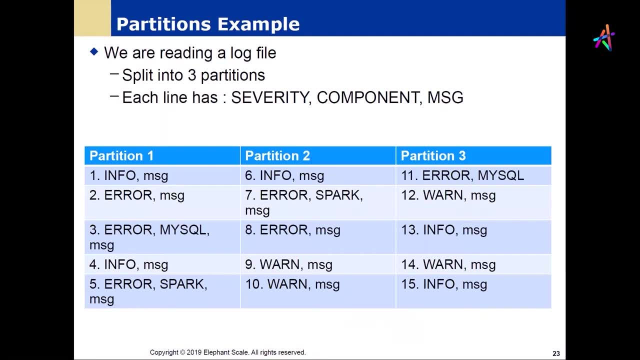 That's kind of our, that is our objective in the optimization. And again, if you, if you stop and you think about it, if we were to execute each step as it occurs, this kind of this kind of operation would not be possible. 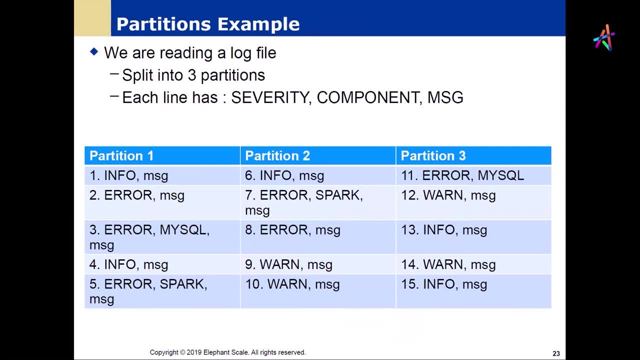 So we'll take a look at the example here. We're reading a log file and it's split into three partitions And each line has a severity, a component and a message. So the the severities here are info: error warning. The component looks like Spark. 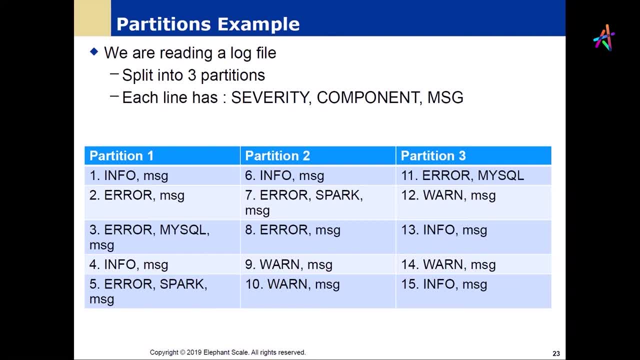 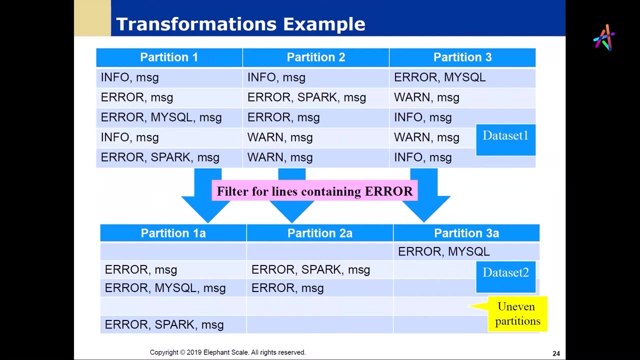 MySQL, some nulls, And we have a message which can be null as well. So we've got this data, We read it in and it's split into three partitions. So the okay, So the first transformation would be applied In this particular case. 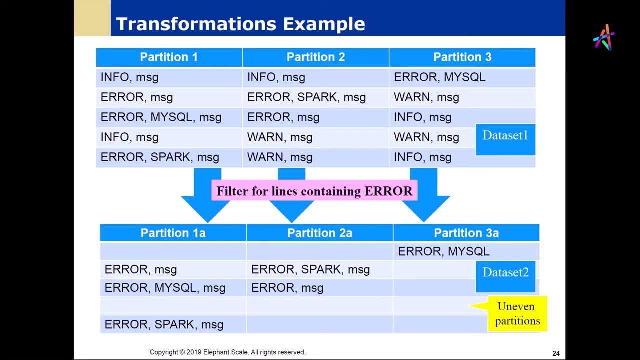 we have run three tasks. Each task applies that transformation to its partition. So, as partition one goes, all right, so let's go back. So we've got. so we've divided up the data, We've got this transformation. we're taking place. 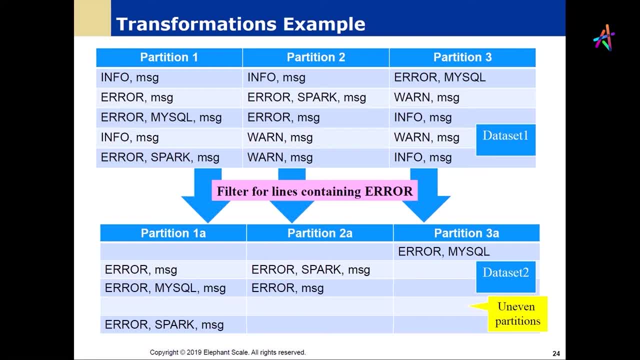 We're going to filter for the lines containing errors. That's broken down into three tasks And each task we'll just assume it's running sequentially at this point. So each task at this point goes through and and produces its output in our next. 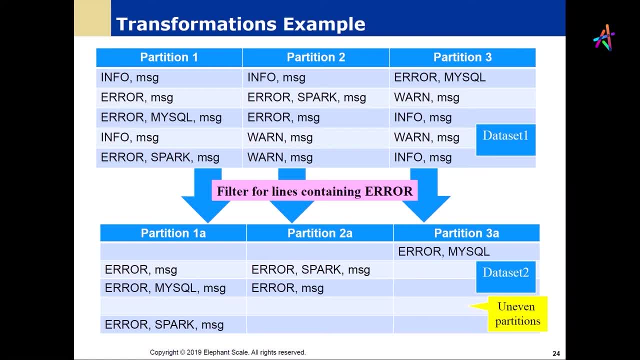 in our next phase And we have an what we call uneven partitions. The filtering is what I'd mentioned before. This is an unbalanced set here, which means that we're going to have performance bottlenecks because the work is is unbalanced. 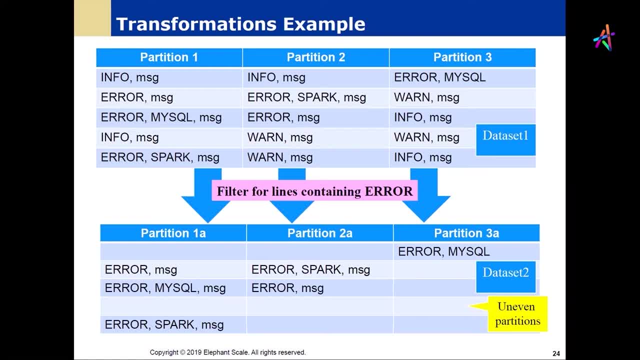 And the the model we're using here is if I've got three programmers working for me and I assign them programming tasks but I do it in an unbalanced manner, then my the programmer that gets all the tasks is probably going to break down. 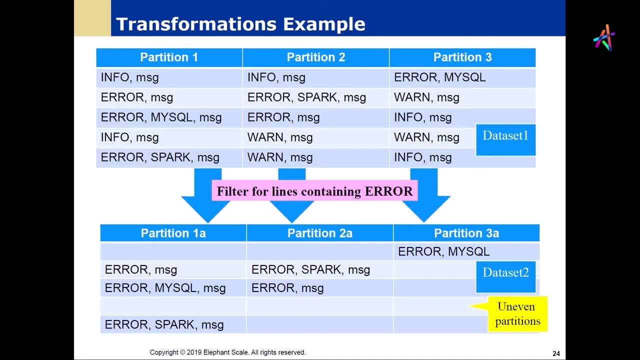 and quit and, you know, throw things at me Because he's so mad. he's doing all the work And I've got two other programmers to sit around just sitting around drinking beer and and watching a Netflix. So the obvious thing is: 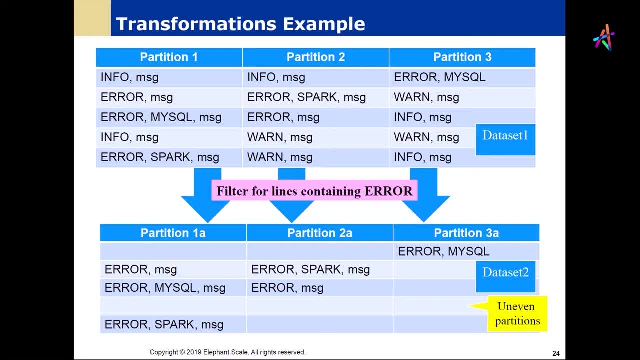 is not so much that I'm overloading one partition, but the question is: well, why can't I utilize all these other resources more effectively? So the real danger in unbalanced partitions is not that we're going to be bottlenecked because of partition 1A. 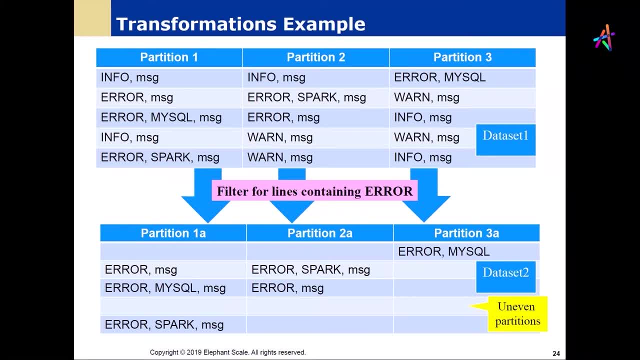 but that that bottleneck is unnecessary because, if we could proceed on, we've got all of this extra capability sitting in 2A and 3A that we're not using Now. this may wind up being a very significant unbalancing if we have a lot of. 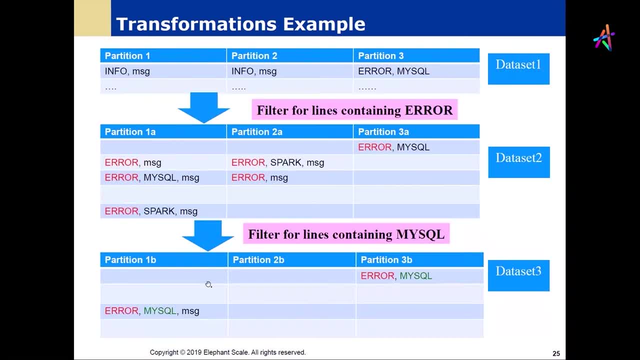 data. So we generally want to try and avoid our unbalanced partition. So if we continue on to what we're again, we're doing is looking at the individual tasks. We're looking for filtering for lines containing error, so that our first filter would. 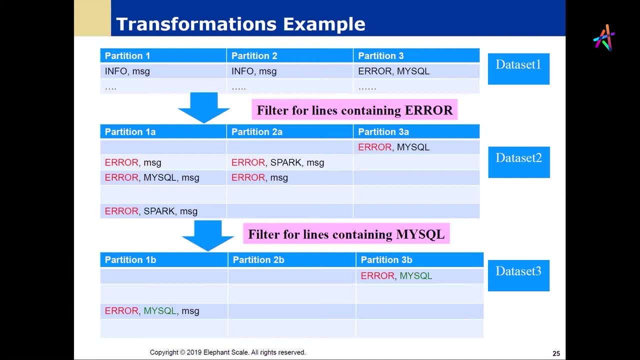 would result? our first filter statement would result in three tasks running in parallel. They produce the output that would be in that data set two, And then we run the second filter and that produces the outset and data three. So we've got, as we're reducing the amount of data, 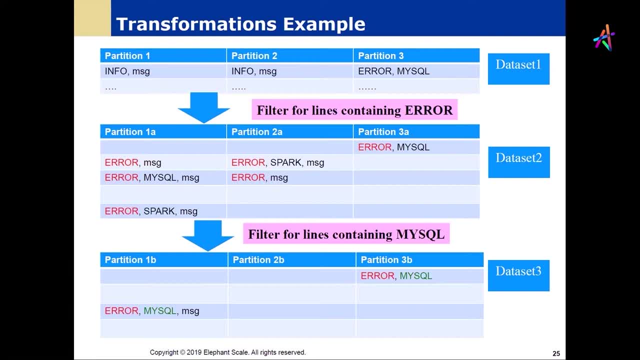 we're freeing up a lot of additional capability and storage. Now, the important thing to remember is that we're kind of cheating a bit here and saying that, okay, we apply this filter and we get this. we applied this filter and we get this. 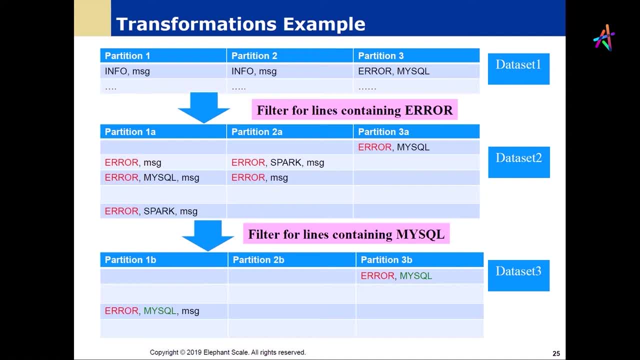 We're not really applying these filters. What we're saying here is: if we applied this filter, this is how the data would look. So we we have this, this operation here Now. this is going to be helpful if we have some sense of what the data is. 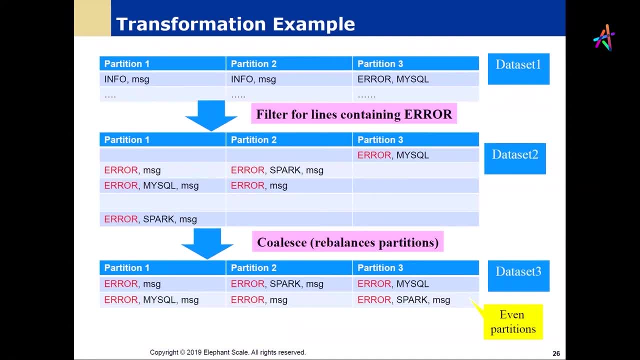 like. So what we want to do is do a couple of different things, And so we filter for the line containing error, and then we can go through what we call a coalesce operation. What a coalesce operation does is rebalance partitions. 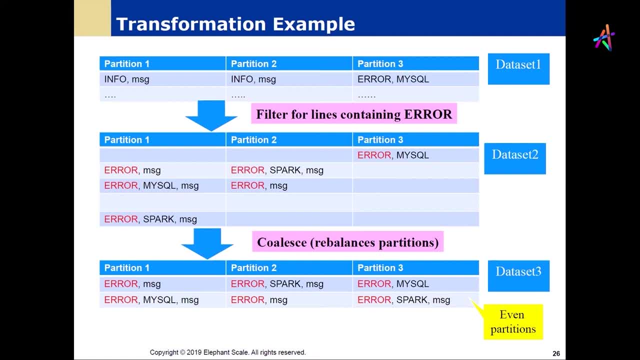 And this depending on on on on on the number of factors, for example, how unbalanced our partitions are. this can improve our performance considerably, But the problem is we're going to have to move data around, since each of 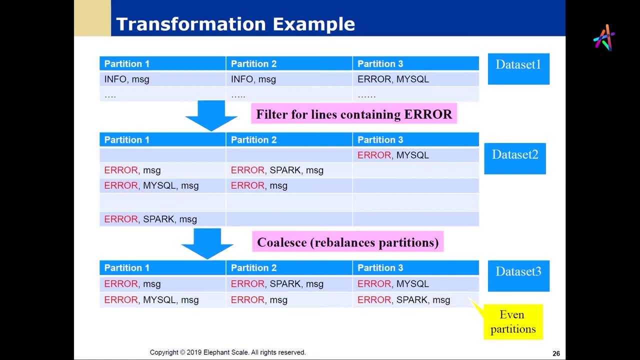 the partitions generally, is working in its own memory space. The often, the only way, the way that we often will do this is with some kind of of of disk, this guy in this guy in this link, like: how do we get data from one partition to another? 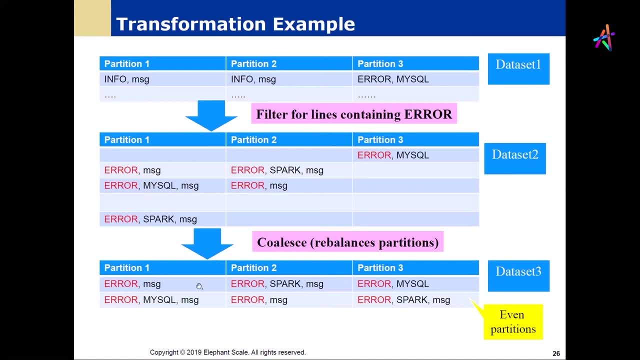 And so that'll become a topic of some of our optimization: optimizations as to how do we make this part really, really, really improve in performance, because it can be, in fact, quite, quite expensive, depending on the data in our underlying system. So the 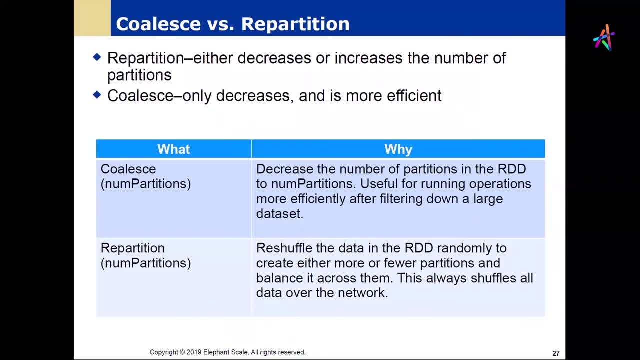 the idea here is that we've got a couple of different things, though, So we can repartition- we can create more partitions or decrease partitions- And coalescing, which is just decreasing partitions and is more efficient. So repartition reshuffles the data randomly to create more and fewer. 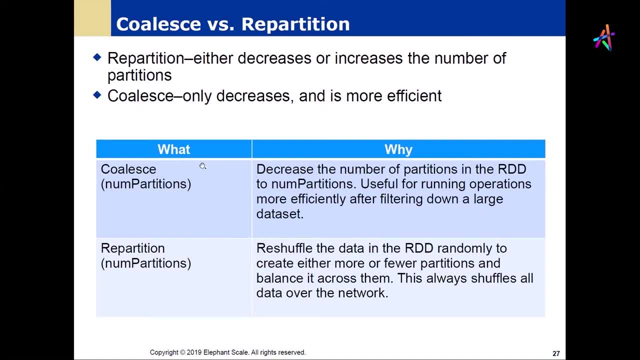 more, fewer partitions and balance them And the and so the. the idea here is that we let's go back- Whoops, Let's go back a slide here. Oh, there we are. Okay, So so now we can even think in terms of. 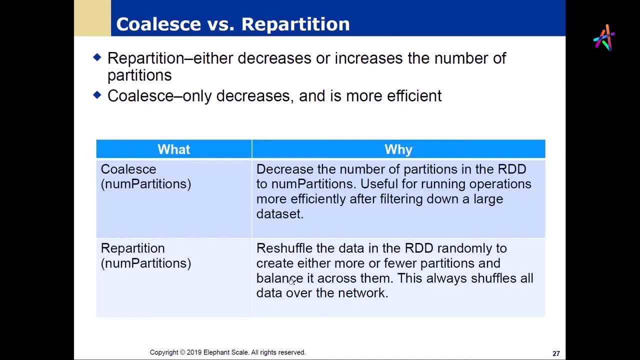 well, what are the costs of these two things? So we repartition, we reshuffle the data randomly to create more or fewer partitions and to balance it across them. So we shuffle data all over the network. So we could just reshuffle data or what we could do is coalesce. 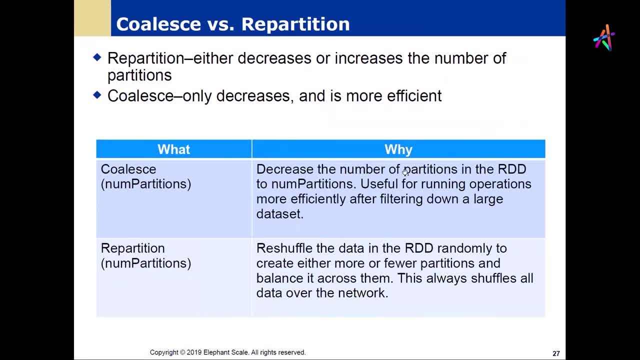 which is an optimization on that, because it decreases the number of partitions to these partitions. So, rather than than than just changing and resorting all the data out across the partitions, we're just saying: okay, so we've run a couple of filters and now we've got a whole bunch of 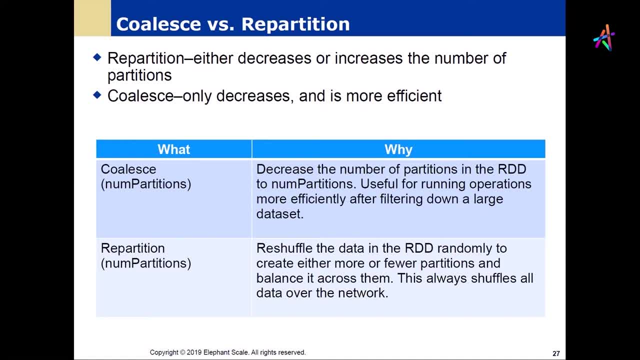 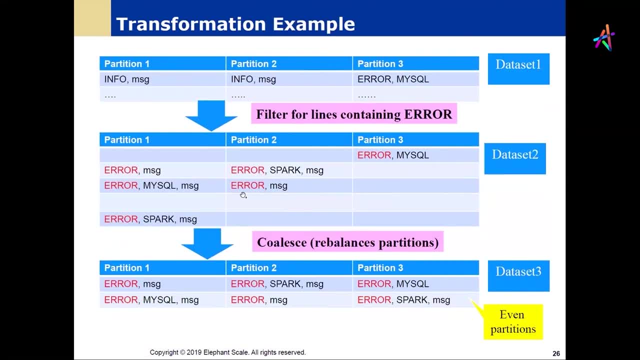 partitions really that are kind of empty. So what we'll do is coalesce them and and just make those partitions available for something else. So the idea here is that we, we can, we can rebalance the partitions we've got, and we'll get more into how these 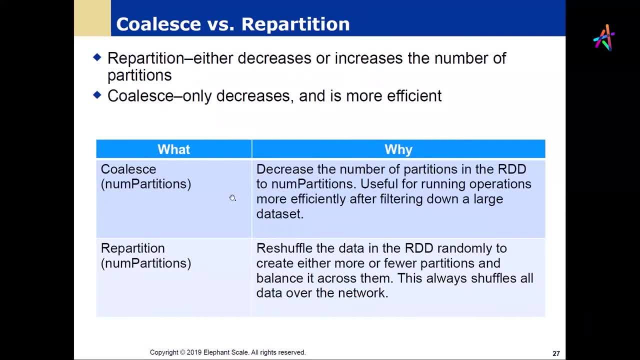 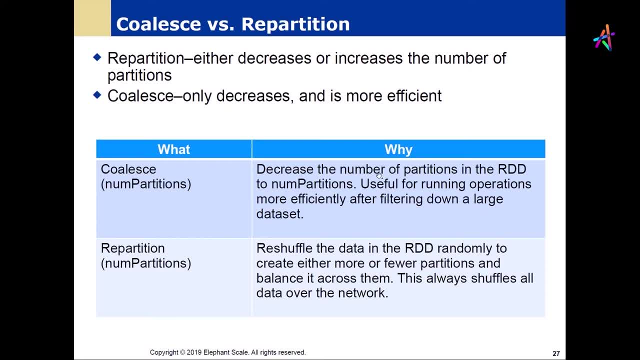 And so coalescing is one of the things we've got to take into account: The fact that we're currently using processing nodes to de- decreasing as the possibility of increasing or decreasing, and has to take that into account. its algorithm- we're coalescing- is only going to be used to decrease. 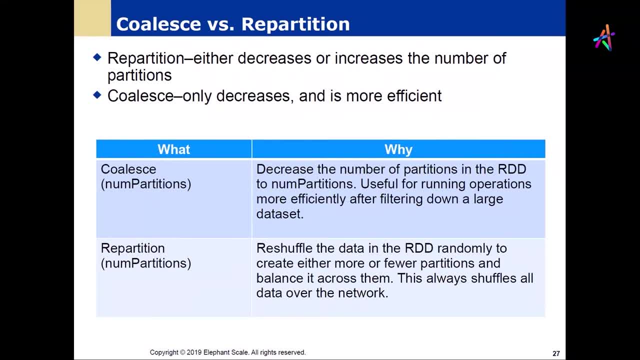 So we can have a much better algorithm for actually doing that And that's more efficient. So we're just decreasing the number of partitions So generally as we're filtering the kind of make return resources we no longer have available, that we no longer need, back to our 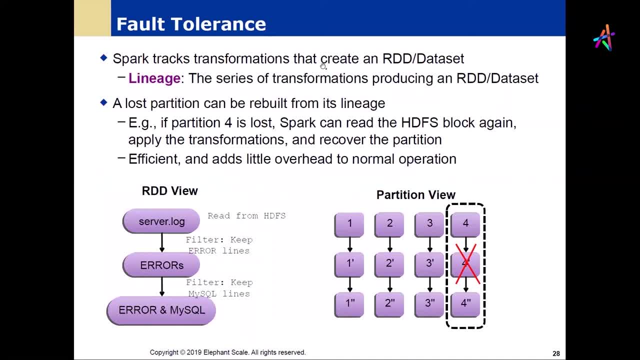 resource pool. So what Spark does is it tracks. it, excuse me, tracks the transformations. I've mentioned that before. That's at the ASIC directed graph, And the lineage that we've got is this set of transformations that produce the data set and the loss partition can. 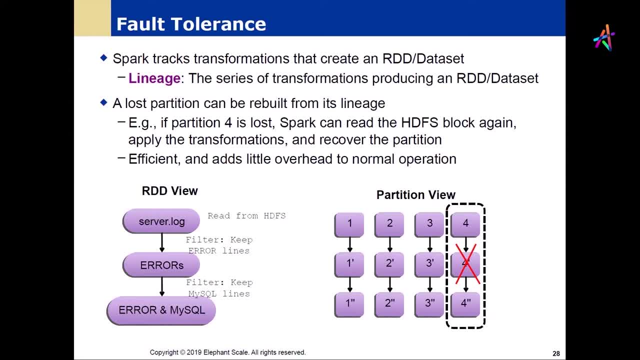 be reproduced from this lineage. So the example down here of partition 4 is lost. Spark can go back and reread the block again, apply the transformations and recover the partition Now, because we're just reading the partition again and reapplying the transitions and 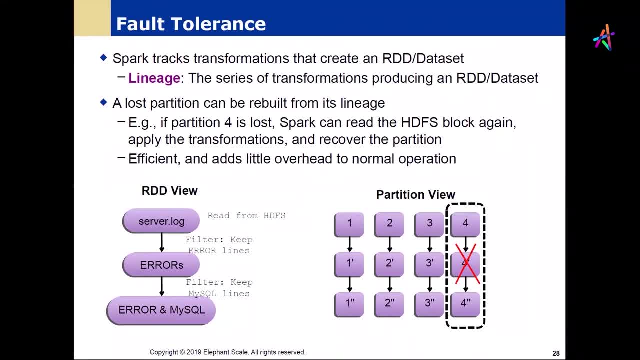 we pipelined the task as best as possible. it becomes a somewhat AWS flat which, during the time when the University of Washington, was very, very efficient. So the underlying mechanism that this works by is able to do a fault recovery because of the way the data is managed in the partitions. So it's very efficient. 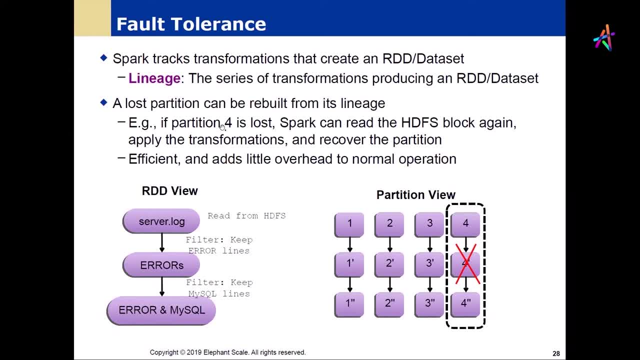 it has little overheads. and we can because, again, we have kept track of how the data got to this point through our lineage. we're able to basically back up a few steps and say, okay, how did we get here? and of course, you know that this is, though, so, this sense of knowing the history of what got. 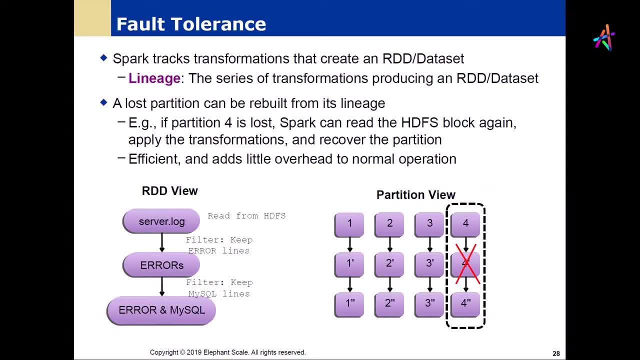 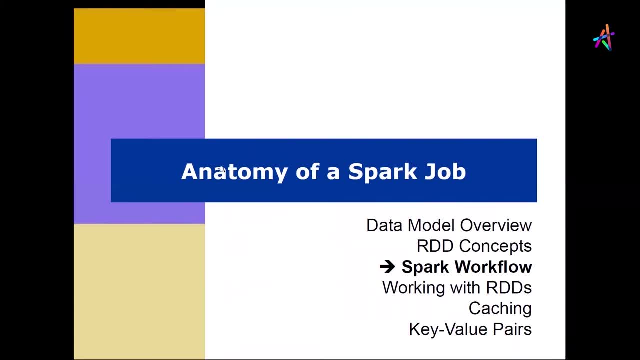 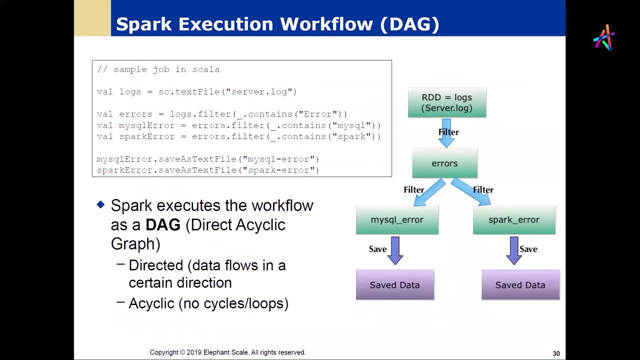 the data into this spot gives us this capability to look backwards in this lineage and say, okay, let's just restart back from over here. Okay, so let's take a look at what a Spark job does. So here's an example of Spark. Now this is using the older interface, which has got the 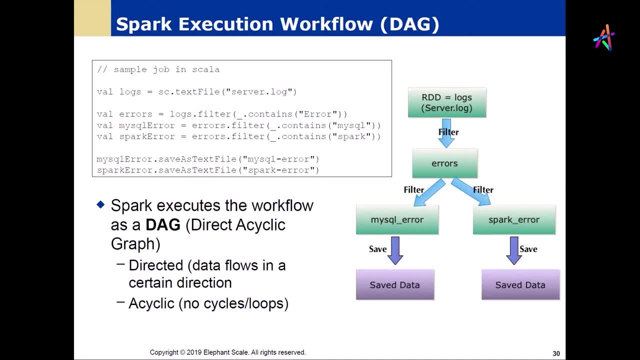 the Spark console. So you can see that the Spark console is running in the same context. So let's step through what what the code looks like. We've initially using the text file we read in a server log and that creates an initial RDD which is called logs. We then filter using our 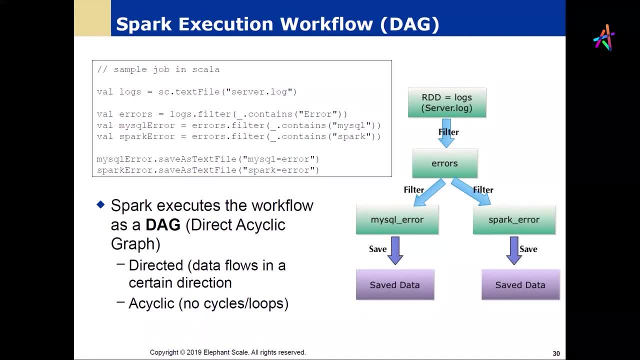 filter function for all of the lines that contain error and the result of that filter is assigned to an RDD called error. So after that line on that RDD data set errors, we filter out all of the Spark lines and we assign that to a new RDD called Spark error. So we have two RDDs that have been built out of this. 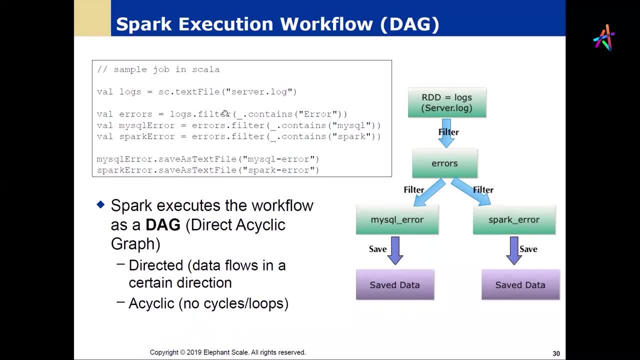 out of this operation. We've filtered the original line in two ways, So we have a graph here where nothing actually happens until we actually encounter the save as text file and we specify the RDD that's going to be saved. I'm sure everybody here is familiar with. 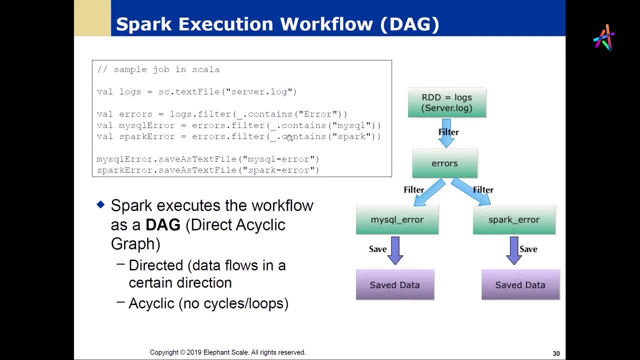 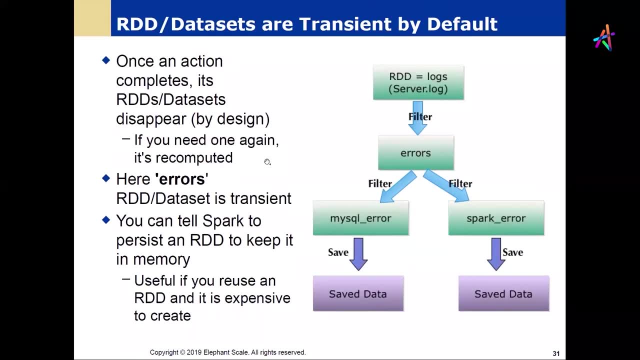 with the concepts of, of graphs and and things like that- Acyclic graphs, directed graphs and all of those sorts of things. So if you aren't, just let me know. Once the action completes, the data sets disappear and if you need one again, just go back to Spark. 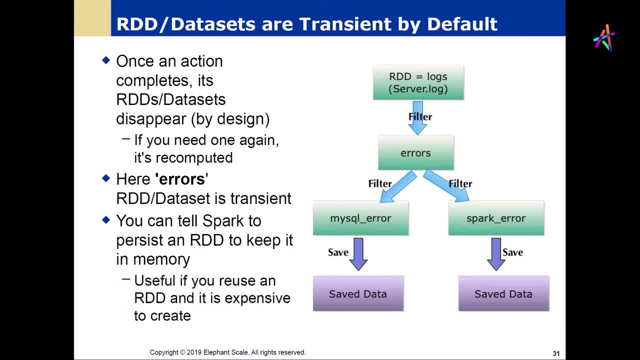 Keep looking for a single lecture or two, but number one should always be a search result. after that, Again, it's recomputed And again that's a little bit of a higher level point of view. Again, we do optimization here And it's easy to conceptualize that these errors. data set is transient. 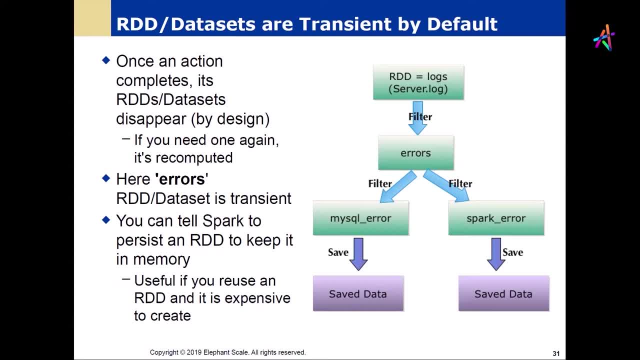 So basically, as it's executing it, it throws away the RDD, which is an intermediate result. So the way it's actually executing is a little bit different than we conceptualize, but it maps very nicely and we can use that conceptual model. 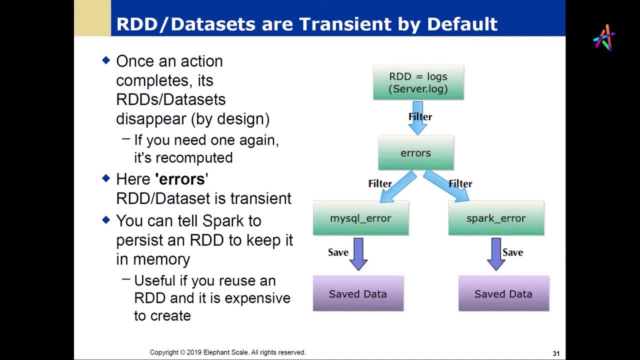 So in this particular case, if we didn't have the two filter operations out of the errors, we would probably get a different sequence of operations if we only had one filter. But now we realize the fact that we're going to have to branch at that errors process. 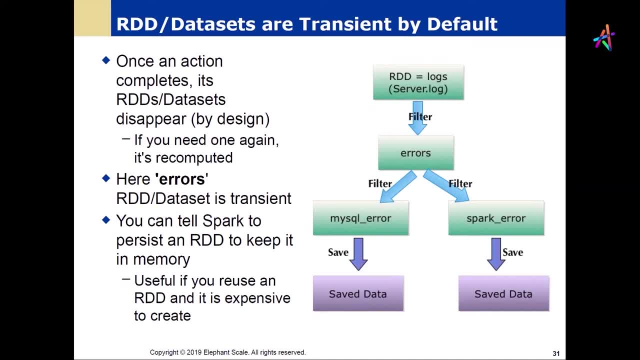 So the operations are going to be implemented a little bit differently. Again, this is the optimization on the acyclic graph. In this particular point though, that we're making, we can conceptualize it as this graph is running: Once we pass through a node, the data- the RDD- that we used in that node to create the new nodes, is no longer available. 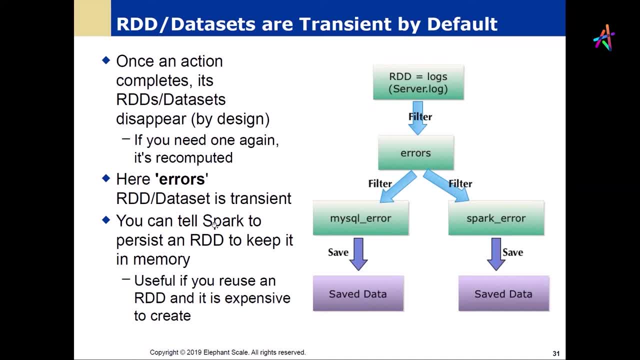 It's gone, So it's transient, And what we can do is actually suggest to Spark that it not be transient. We just want to keep it in memory And again, the idea here is that sometimes this initial operation, whatever it might be, might be extremely expensive. 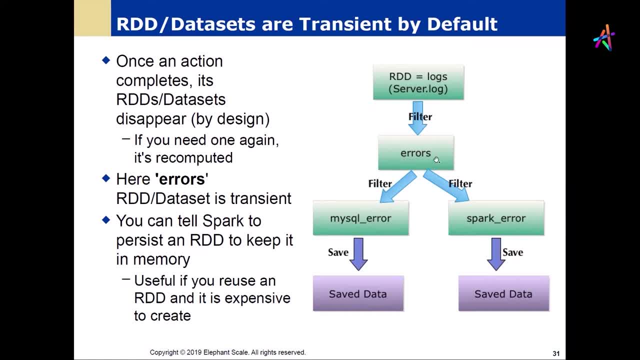 So to have to recreate this RDD might be prohibitive in terms of utilization of resources. So we can say: okay, when you get to this step, just hold on to a copy of that, and then we're going to use that in our further computations. 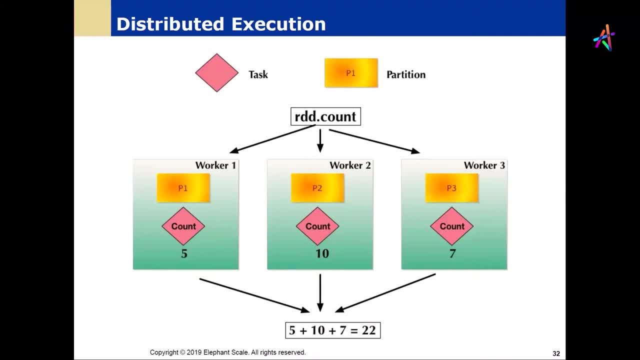 So here's our notion Of what we're going to be doing here. when we do a distributed execution, So we have RDD count, So we're going to count stuff in the data set And this is a fairly standard distributed model like a MapReduce model. 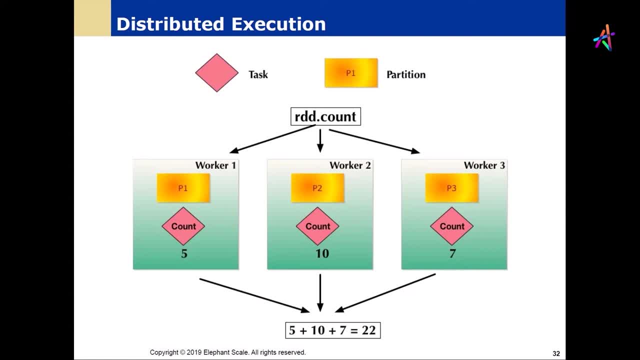 So what we're going to do is take our operation and delegate it out in terms of tasks. And again, the thing to notice about tasks is that the tasks themselves are operating pipelined within a particular worker node, So with an operator on a particular partition, so the so there's a fairly standard MapReduce type of idea here. 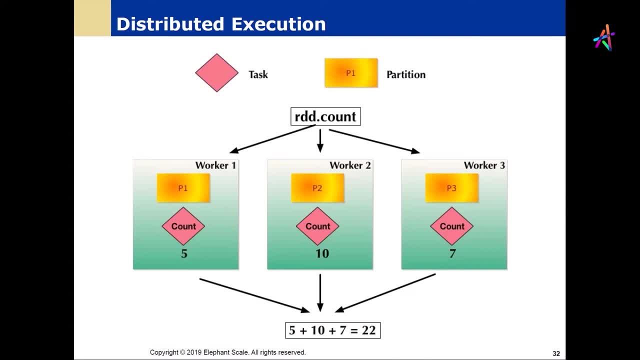 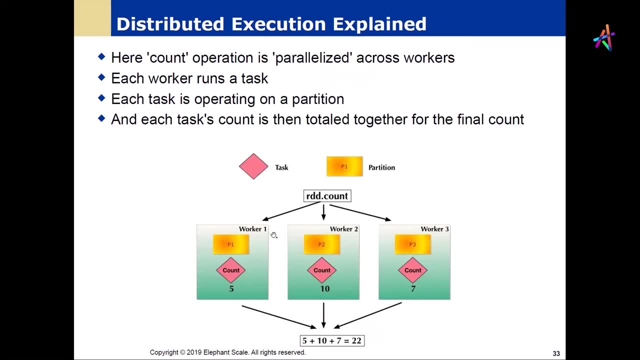 but it's far more efficient than a standard MapReduce by the way it's organized. So the count is parallelized, parallelized, parallelized, and we get used to this notion of the task. So each worker runs a task which is a subset, or the not a subset, which is the actual operation applied to that partition. 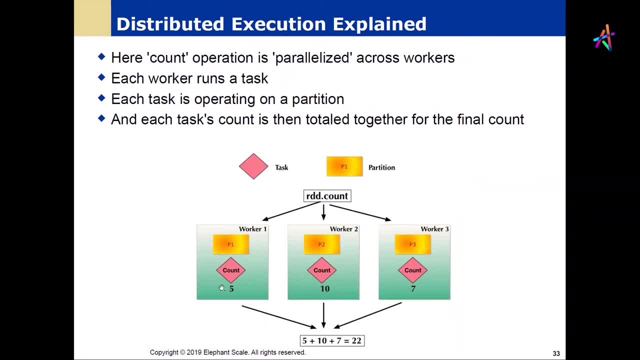 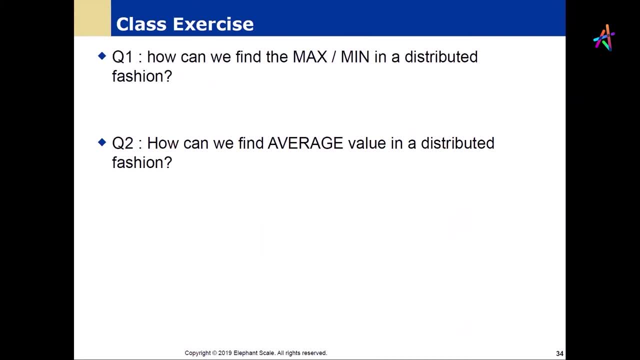 Okay, so this is the notion of the parallelization. So here's a question: How would we find min, max in a distributed fashion? Just, I guess, as a general thought. Well, we can find max or min in the each of the nodes or in the each of the partitions. 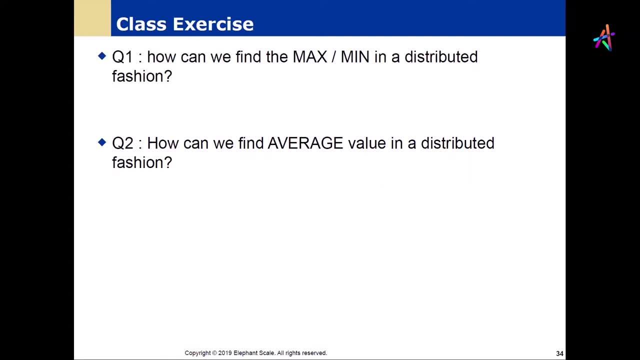 and then find max or min in in all the results that we've got from the nodes. I think that's probably quite right. So how can so- and I think that's fairly obvious- How can we find an average value in a distributed fashion? 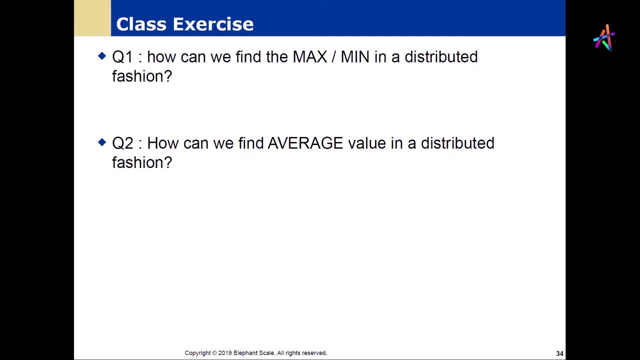 So cross all the nodes, sum up and count elements and in the end divide some by the number of elements. Yeah, I mean there's a couple of different ways you could think of decomposing. the problem Is is you could, you could return an average and then a count for each partition and then 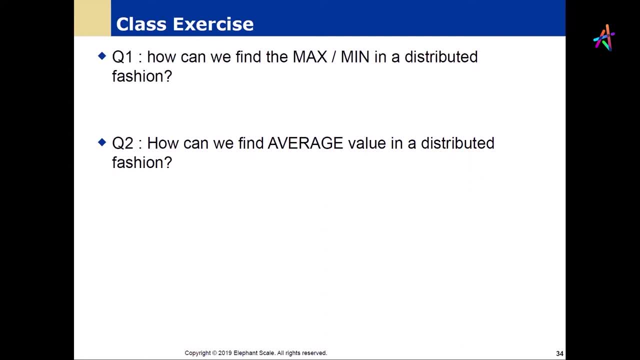 and then do a combined average, or you can do exactly what you say: Do a sum of whatever you're averaging for each partition, Okay, each node, and then do a master summon and do the same thing with the count. so yeah, i think these 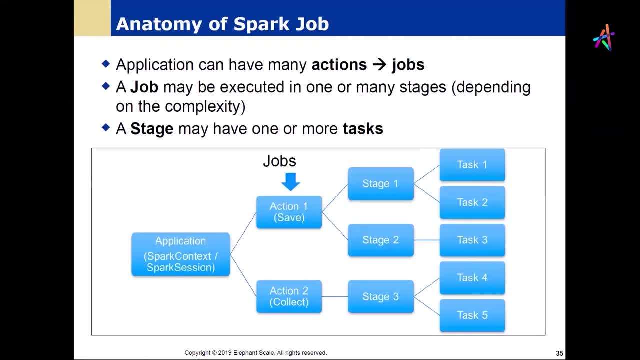 are fairly obvious questions: um, uh, so, uh, we're going to take a look now at the notion of the, the applications jobs, uh and a um, so we have a spark section and a uh- hold on here- and the job can be executed in one or many stages and the stages can have one or more tasks. 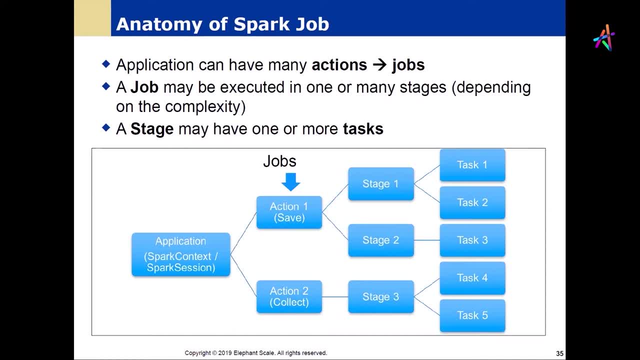 so what we do is we decompose down the action, uh like save and collect, and we decompose now those down into stages or steps, and each step then maps out to a set of tasks on a particular partition. remember tasks when we talk about, when we're talking about local. 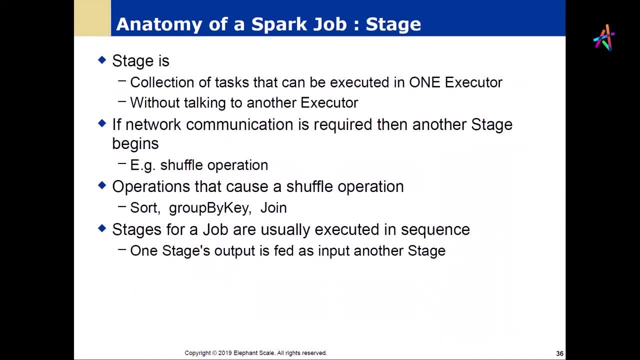 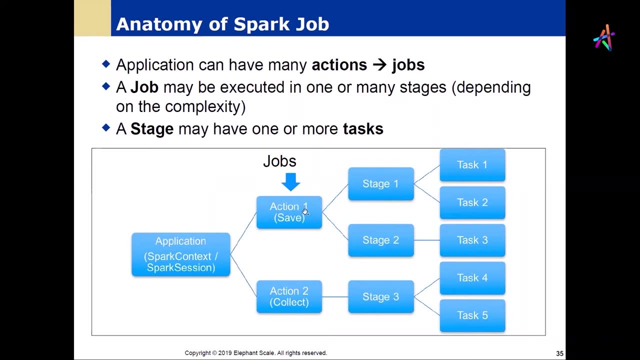 partitions. so a stage is a collection of tasks that be executed in one executor without talking to another executor. in other words, it can. a stage is a sequence of operations. let's go back over here. so when we look at this action, we'll say: well, what? how can we? what are the sequence of? 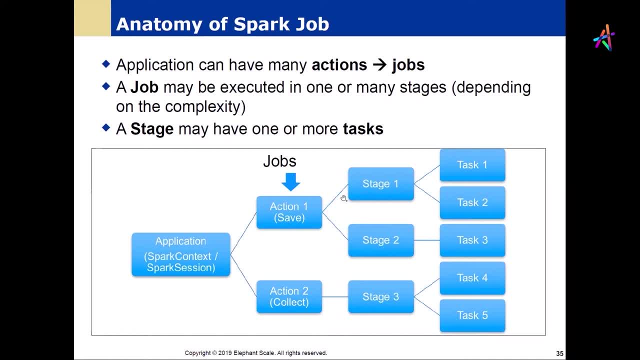 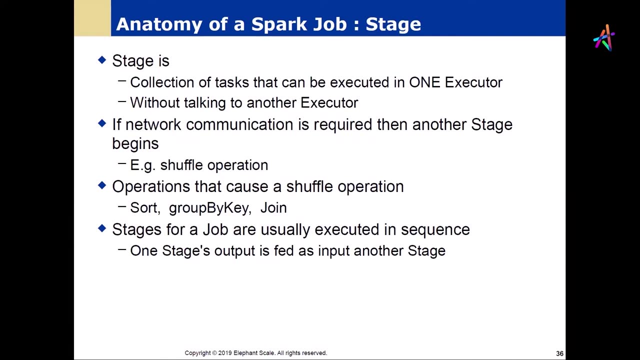 actions that we can do to get there, that can be executed within a single, within a single uh, within a single uh partition. and that stage then breaks down to the series of tasks that we can execute on each, each partition, the, the collection, so the. so the idea is that if we can, if we can execute all, 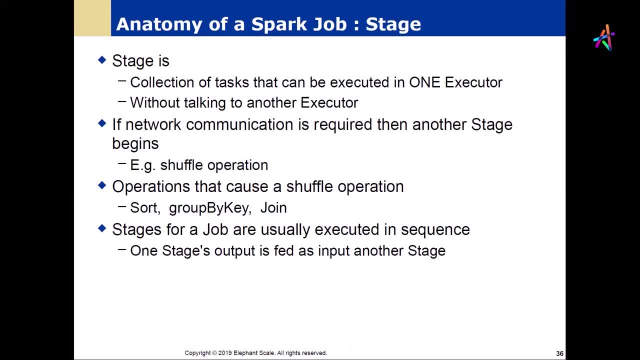 of this without having to do any reshuffling. we basically uh- you can think of it as having one uh uh, one, one task, but if, if we have to do some kind of of moving of data around or communicating of data, then we have to have a another stage. so we have to think about uh, uh, as long as 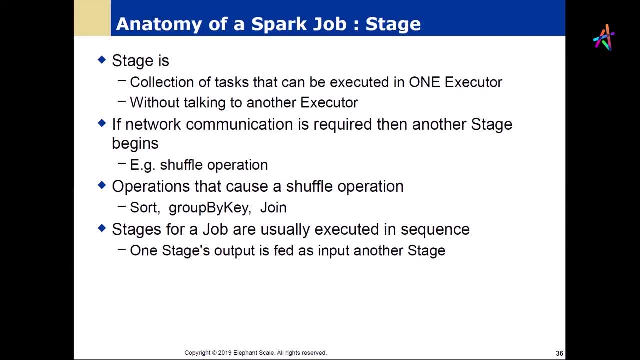 as long as the data remains consistent and and can work in isolation, uh, we're generally going to be working within the same stage, but as soon as we need some kind of of interaction, network, communication, uh, then we're we have to, uh, um, start a new stage. so what are the kinds of things that? 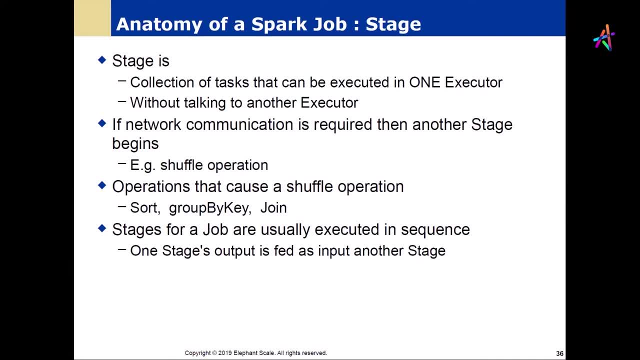 cause these uh well sorts groups joins, uh, so the um. so the idea is that is that when we we are doing some operation on the data set as well, and the ordering on the data set and how that works, uh, a whole that does some kind of transformation like this, like sorting. We can't just sort. 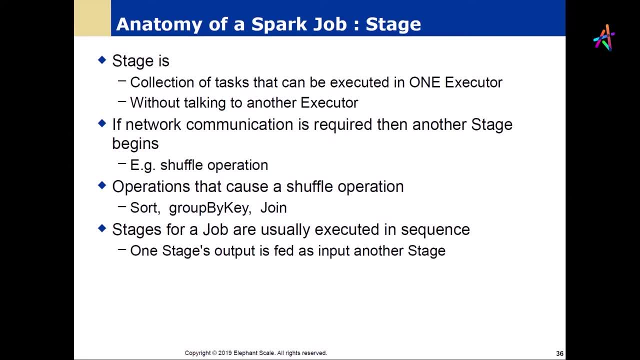 necessarily an individual node, because we're only going to be sorted on that node and so to get an overall sort we may have to do some kind of other operation to sort across the groups And similarly group by key. we can group on each node. 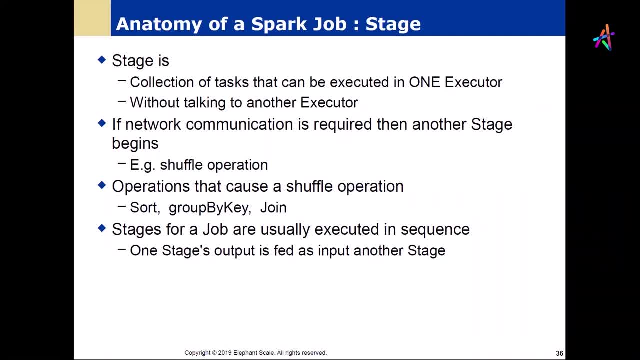 but we still need to group in terms of the entire data set, and joins, of course, are a similar kind of operation. So what we want to do is try to pipeline and stream our stages into tasks, but we also want to try and break down the job into the individual stages that can. 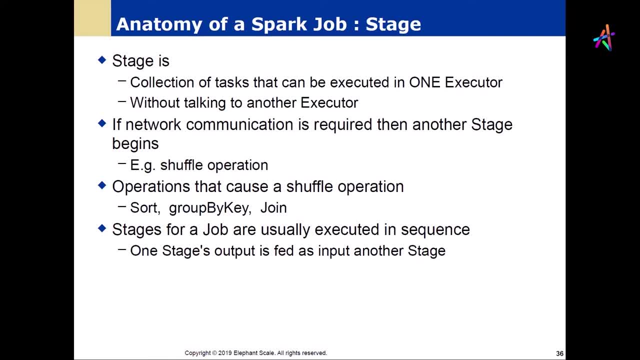 be executed in sequence. So again, we're looking at going back to a really functional model here, where we're looking at applying a job- and you can almost think of this as currying the job- where you're taking a data set and a sequence of operations and you're breaking them down. 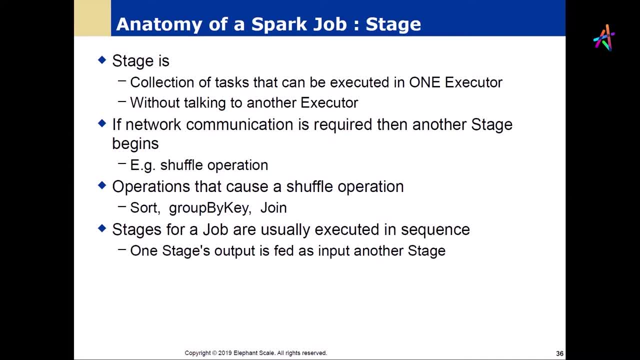 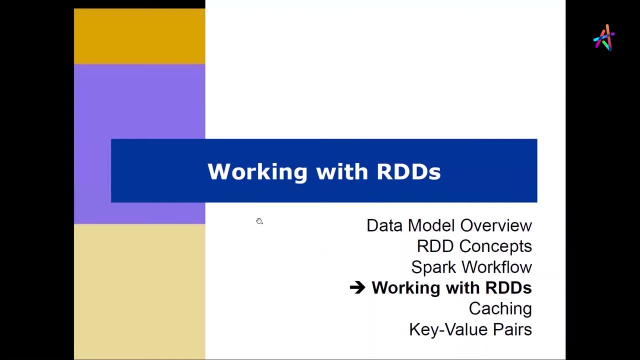 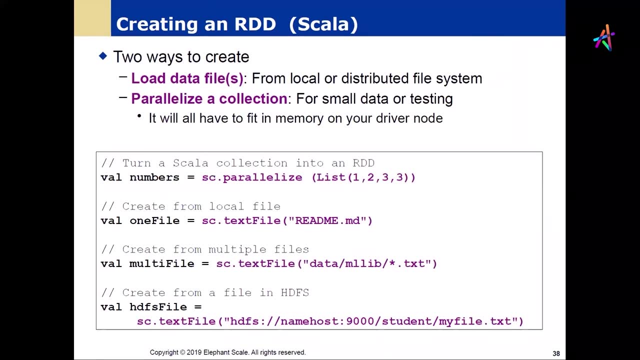 into a sequence of operations, each one feeding on the output of the other. So there's a way to conceptualize that. Okay, working with RDDs. By the way, we'll get into sort of the underlying mechanics after We cover all the basics, so don't worry, we shall get there. 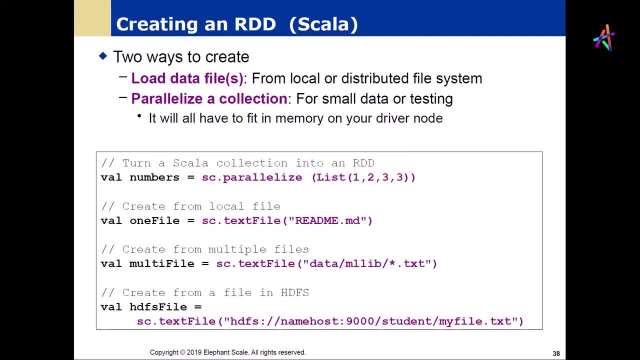 So the couple of ways to create data. we can load files from local or distributed systems, parallelize a collection, and this is often where we are wanting to work with small to medium-sized data sets. We're not going to get any significant advantages from parallelization. 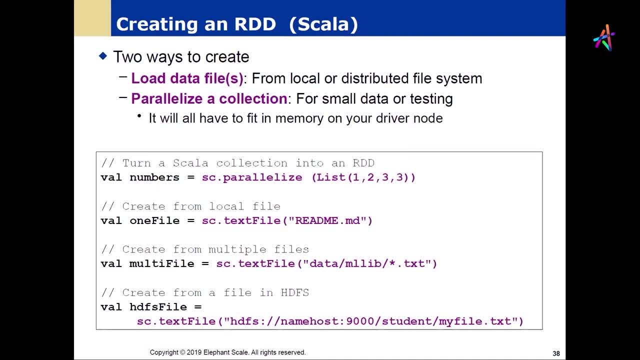 of the data or maintaining a distributed file system. The idea is that there are some applications where you don't need a massive amount of storage, but you still want to do the same kind of analytics that we're doing here. So if you're going to parallelize a collection, 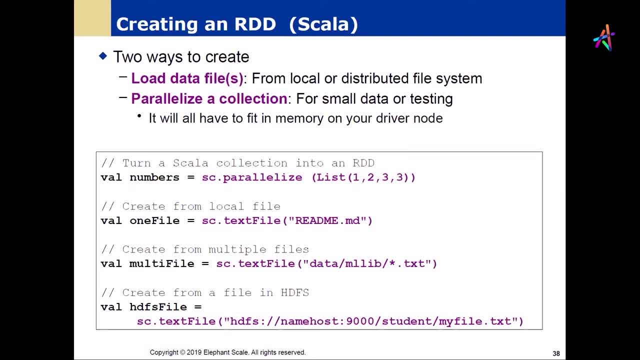 this goes back to kind of our workflow model. So, for example, if I am going to be developing some kind of algorithm to do some kind of analytics on a massively large data set, I'm probably going to take some sample of that data set and use that as a test data set. 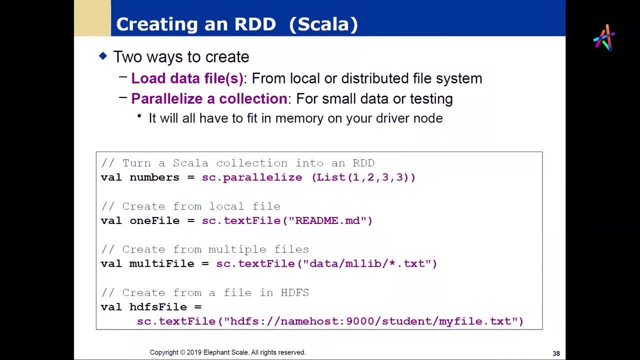 I'm going to start with a relatively small number of elements that are representative of the underlying population and I want to go and experiment with my Scala algorithms on Sorry Spark algorithms on that data set, Because the data set is small enough, I don't need to put it into a distributive 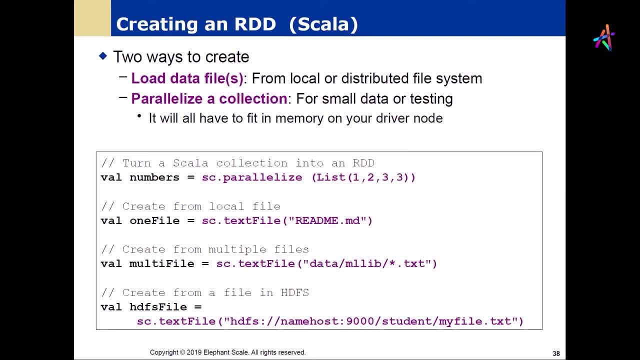 environment. So I'm really looking to see: is this algorithm going to give me the right result? Once you get the right algorithm, then you can start thinking about how I'm going to work with the larger, the larger data set in the in the data. but I know my algorithm is going to work, So this is. 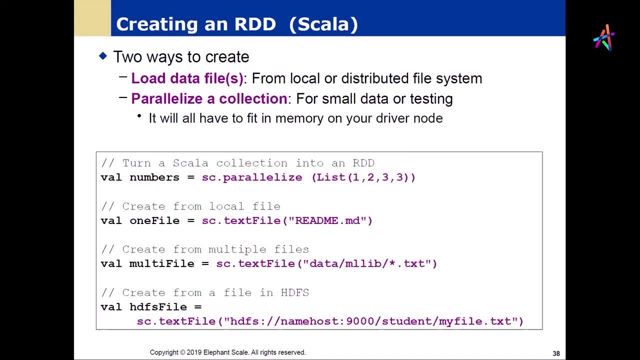 so the parallelize gives me the emulation of being in a distributed system. So I'm going to see how it's working and how it works And- and I can- I can work with small data that fits into memory that we can create from a local file. There's an example that we read it in. We can. 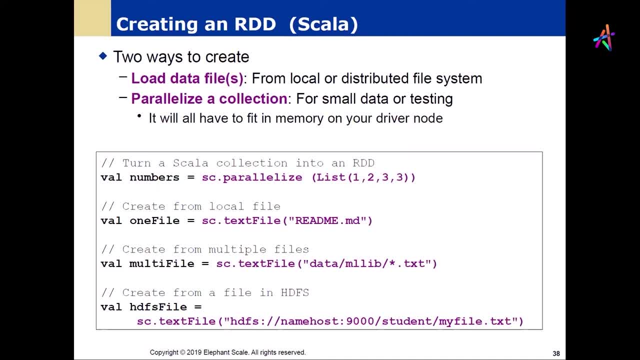 create from multiple files. We can create from files in HDFS And, as we get into other other ways of doing it, I think we get into the more recent versions of of of of things like data frames. We also are able to read JSON files and CSV files and other things that have structure. 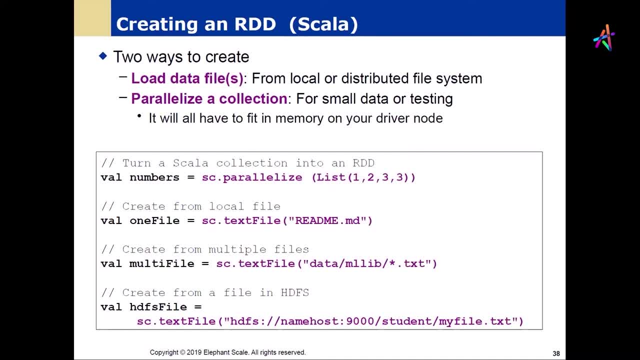 into it. The one disadvantage to the optimization routines for RDDs is that the data is is fairly opaque to the optimization routines It it there's no real sense of the underlying structure of the data, So it's not necessarily able sometimes to figure out what an optimal 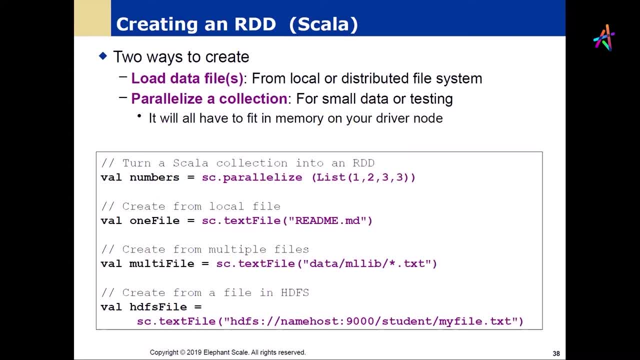 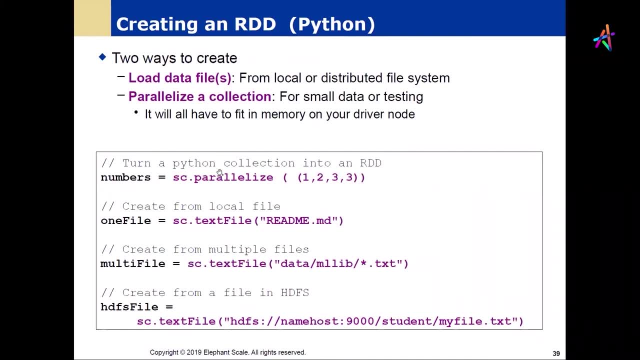 strategy is. That's what the data frames give us- is the ability to do a little bit more prediction as to what an optimal strategy is going to be. This is how we would do it in Python. Again, Python works here because we're working with RDDs. 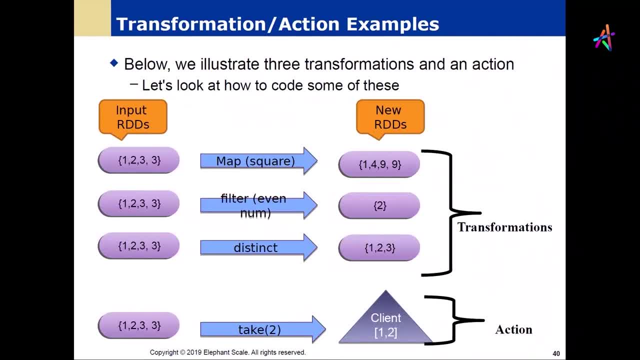 It's much the same as as the Scala And of course, we could do a number of of different different operations using different, or we can implement that in a number of different programming languages. Now transformation and action examples, And again, it's almost. 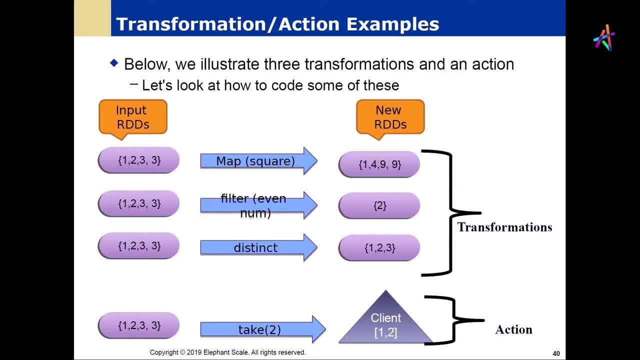 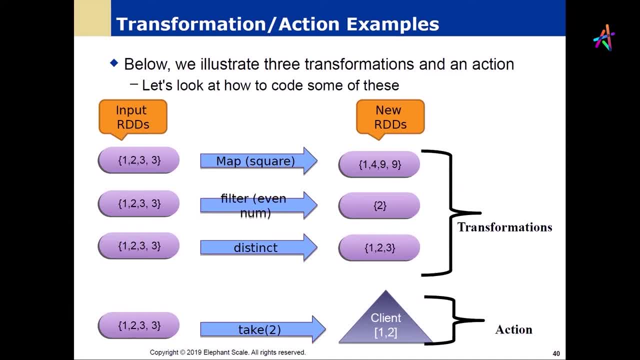 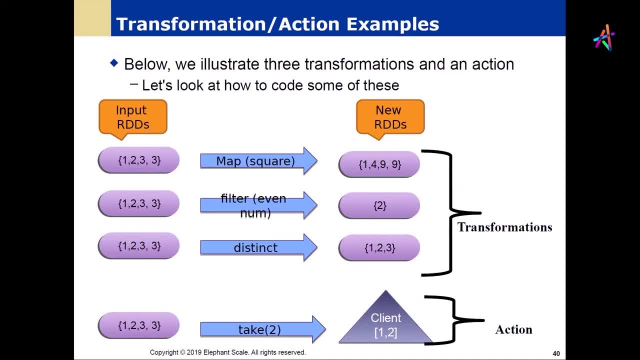 of thumb is: if you're returning a result to as a return value from your, your scale, from your Spark job, that is going to be an action. So there always should be an action, obviously, because what's the point of doing all this transformation? 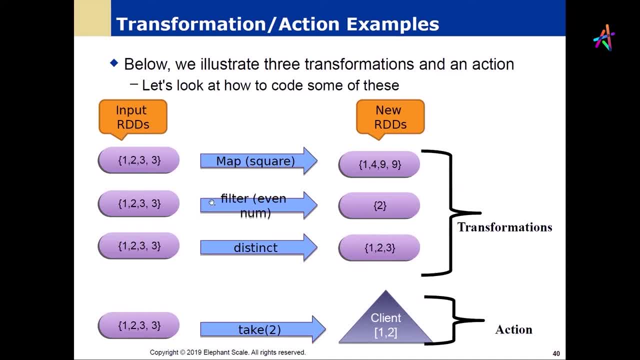 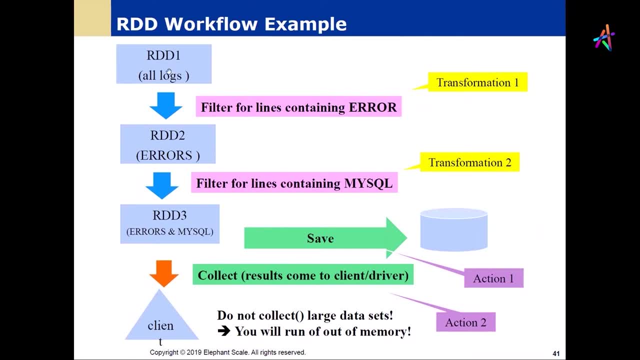 if you don't get any results from it. so we're counting on the fact that there's always an action, the workflow again. here is our, our RDD, and we again go through our filtering. do it's a couple of transformations? RDD 3, and we find the 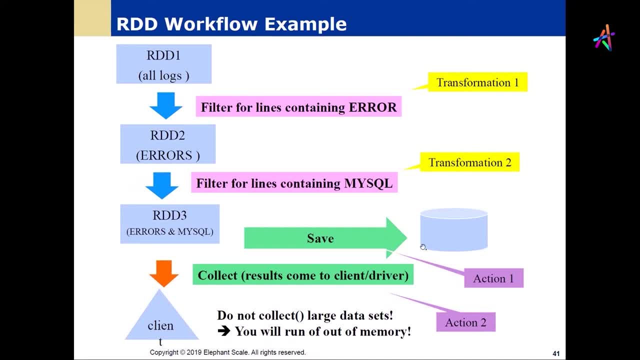 errors and then when we do a save, then we have an action and we can collect on that and also do the client warning here is: collect returns, all of the results of the transformations. there's other operations, particularly if you're testing that like first and top, and it's a top. there's certain you can, you can. 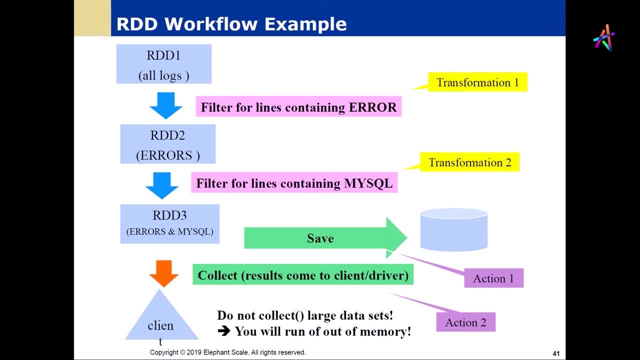 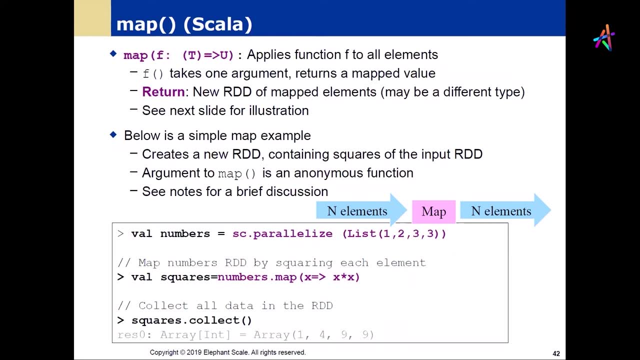 specify a certain number of records to be read and just to make sure that you're doing things correctly. yeah, if you're using collective, it's generally not something you want to do for a large data set. so the, the, the map transformation- this is going to be fairly obvious- returns the map value and the the there. 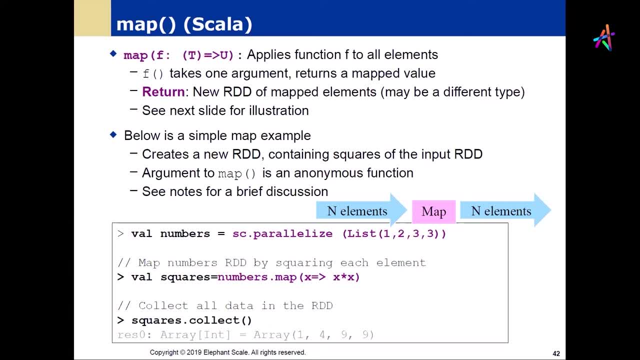 may be a transformation of type as well, but a simple map generally has the same amount of outputs- output records- as inputs. and now we, what we can do is look at that code down there, we parallelize a list of numbers, we apply the map function and then we collect it into and we get. 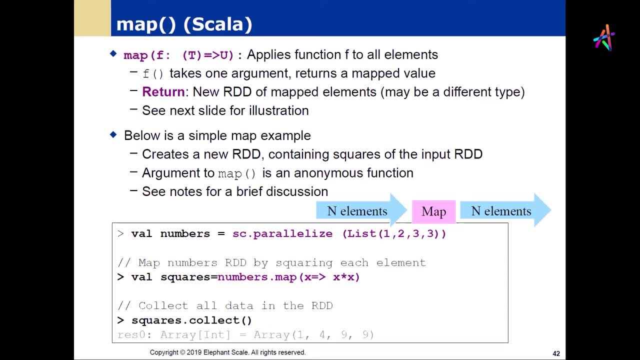 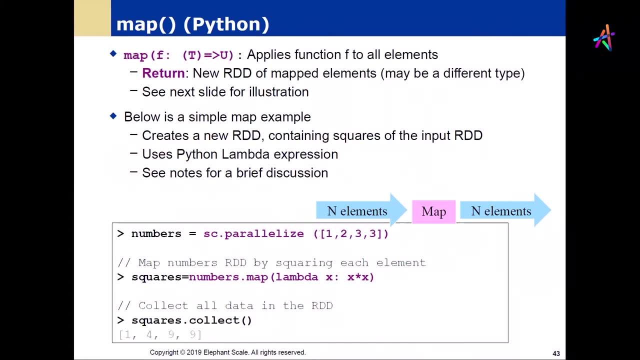 out the result, of the of the result. so it's when that collect is actually executed we wind up getting the the result. we do the same thing in Python. we're not really doing Python so much in this class, so I'll just put it up there to say you can see: exactly the same operation is taking place. we're just 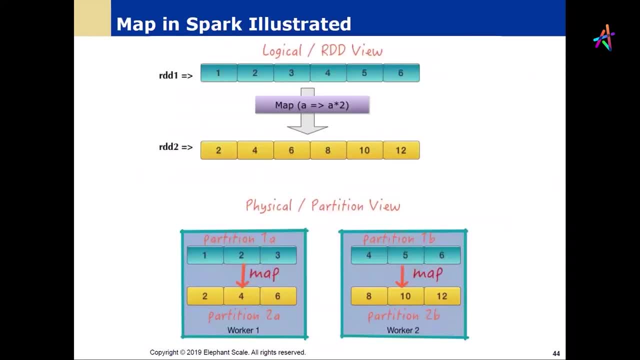 using a different programming interface. so what's happening in here is that when we parallelize the, the logical view- and this is now we're going to get düngstwen ini operational view and the logical view. so the idea is that every operational view of the data can produce multiple strategies. in fact, we 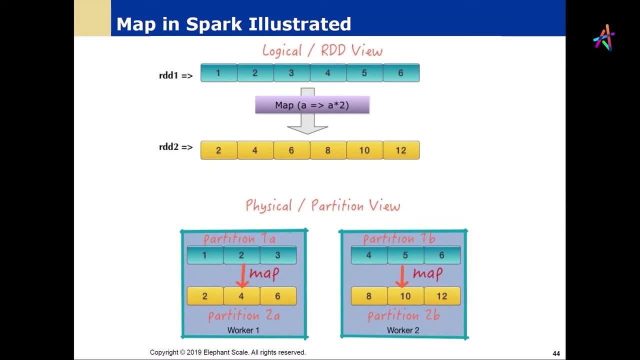 call this a logical strategy. at the top, the logical view is a logical strategy. it makes sense. I've got all this data and I'm going to, I'm going to molto. I'm going to multiply each element by two. That's the logical view In the operational view or the 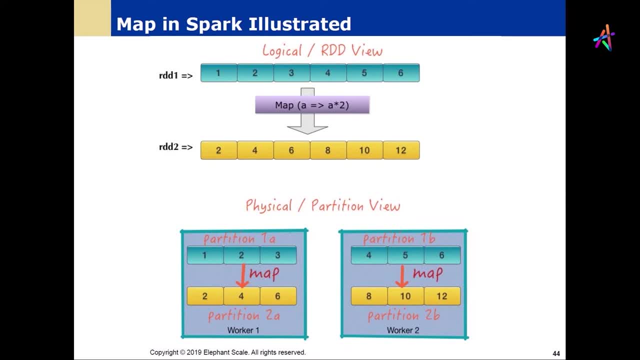 implementation view. I'm thinking in terms of how that operation breaks down into tasks. So from my logical point of view, from my analytics point of view, I create RDD2 out of RDD1, and I can imagine that's in memory. Now what happens is that the that operation has only got one stage. 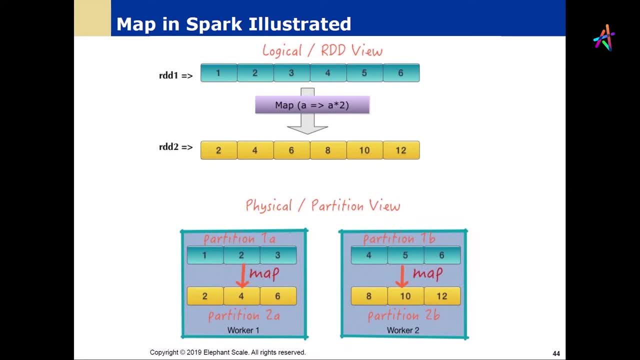 is then at the physical view, turned into tasks. So I've got this map task that's going to operate on each particular partition. So the so where we're going to get optimizations, is often in how that, how that operational view is implemented from the logical view. 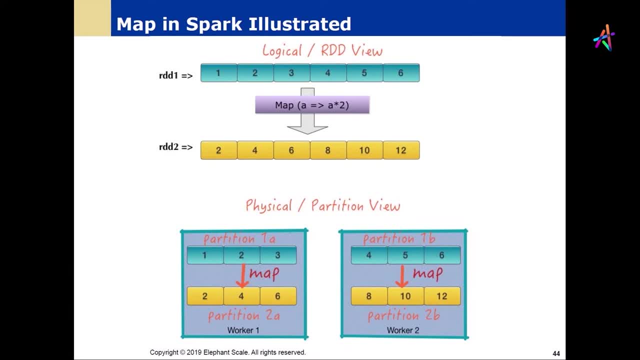 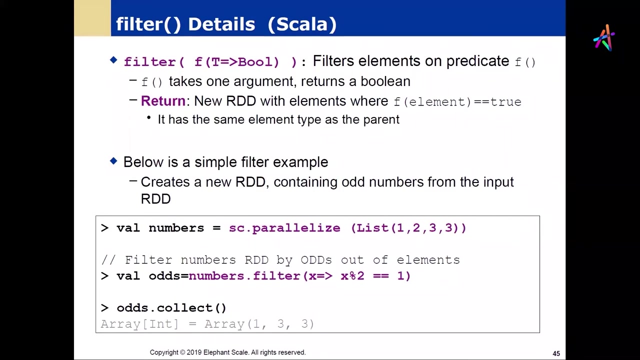 So the idea is that one logical view can have multiple possible implementations. Each one of them has an associated cost and our optimization routine is going to try and minimize the cost of that implementing that logical operation in a particular physical environment. Okay, so there's our the idea behind that. So a filter reduces the size of an RDD. 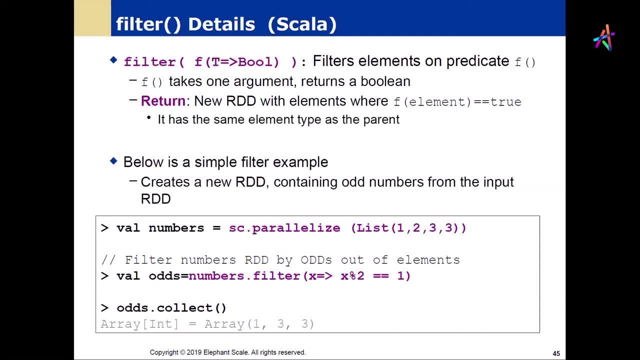 and it has does not do any type changing And we we have the same, the same operation here Again, fairly straightforward and simple. We're not going to get too, too deep into it. It's fairly obvious: you parallelize, you filter. I think everybody's familiar with that idea And you can. 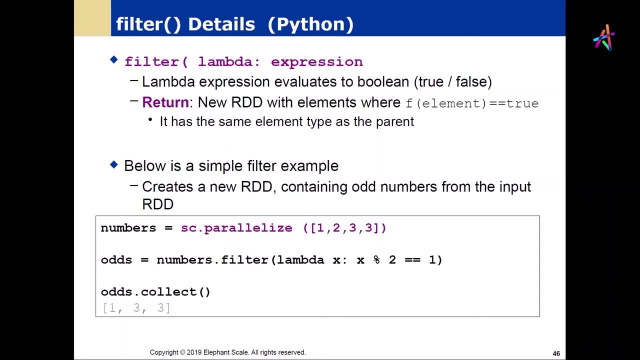 standard way actually is is to use use anonymous functions. So I think in Python we use the lambda keyword to get it in there. So I think in Python we use the lambda keyword to get it in there. So it's exactly the same as the slide before. 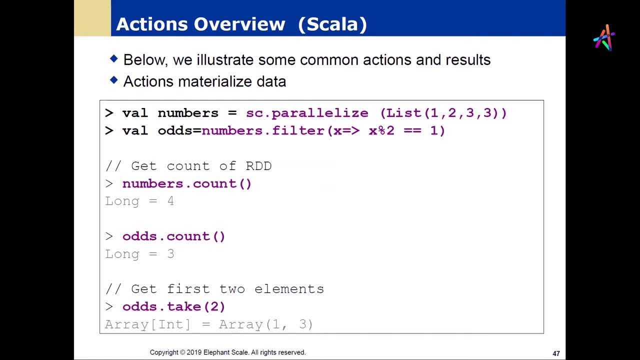 And we have a couple of common actions. Oh, it's take. was the the action I was trying to to? to think? I work in so many different environments. I get aphasia between, between the commands in different environments. I've actually sat down in a programming language. 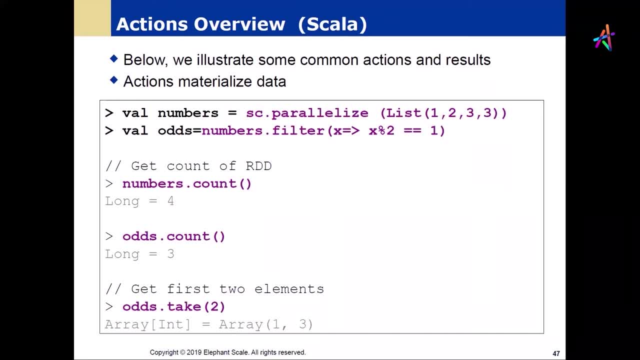 and written if, and I have no idea what comes next because I can't remember which way it's implemented in that programming language. So that's kind of embarrassing. So if you take a- let's take a look here at- at an action count returns the number of counts. 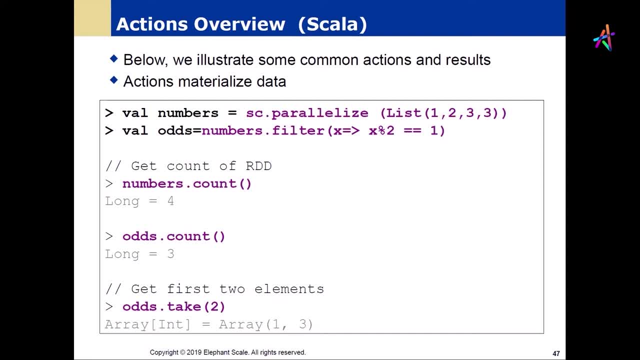 And, as you can see here it, by the way, could anybody suggest what a, what a an optimization might be on this? What? what are some of the different ways that we could do this collection? Pardon, Persist odds. collection between. 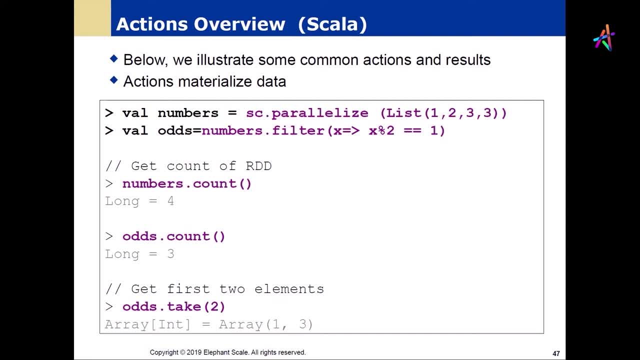 So count and take are both executing right. So if we could persist collection in before doing count, then we wouldn't do it second time. Yeah, so in other words, when you stop and you think about it, if you can think, there's a couple of different ways that I can. 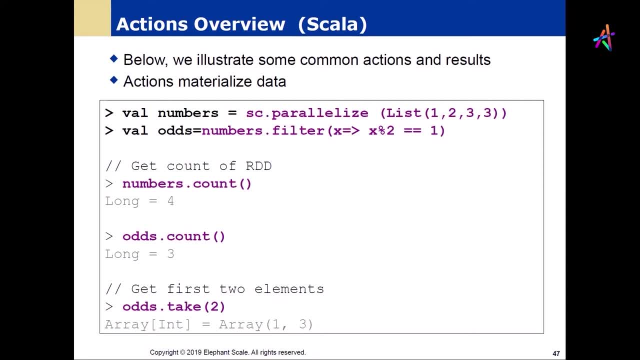 actually implement those two lines of code, some of which would produce results. So, if I Excuse me, So if I just executed this all sequentially, I would have to have both RDDs around. I would have to have both numbers and odds in order for me to 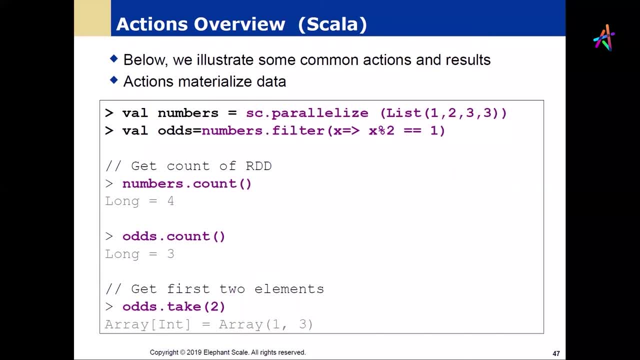 go and get a count of each. So it would seem really inefficient, even though the code says: due to these transformations, then do these two actions. When I analyze what the actions are doing, I can reorder it so that when I first create the numbers, I can do a count of numbers and stash. 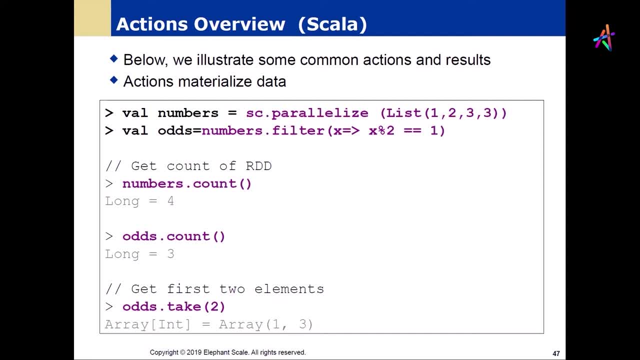 that and then do the transformation, get the odds and count that, And I don't have to keep numbers around. I can You know that, otherwise I might have to have it persisting. So the idea here is that what we're really doing. 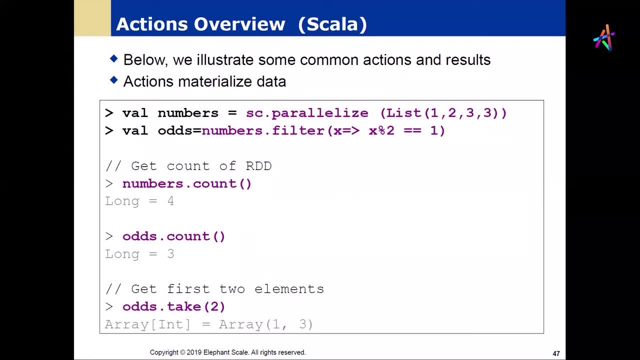 is doing a count. And not only that, but if I do the, the, the, the, the count on odds, I don't even have to keep the. if I'm only going to take the first two, after I get the count, I can. I don't have to maintain the whole thing. So the idea here is: if you stop, 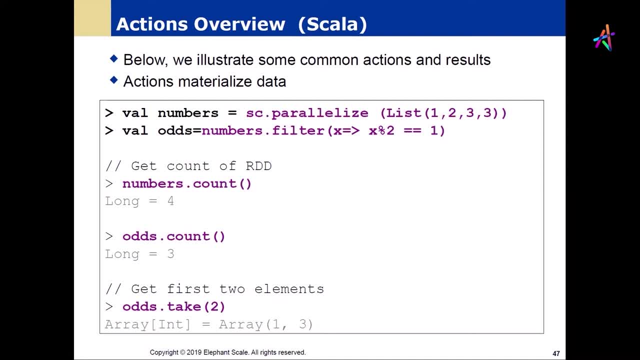 and you think about it. the question you're always asking is: what can I throw away? What? where can I? if I reorganize my steps when I'm actually executing them? am I going to get efficiencies? Am I going to be able to throw away data that I'd otherwise have to keep? 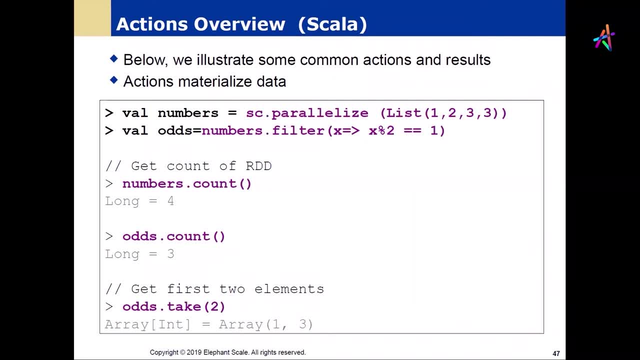 Or am I going to be able to do a couple of operations early, save the results and then not have to do certain kinds of transformations? So these are the kinds of ideas that we have between between this. Now, this, I think, is that's Python. we'll skip over that Reduce. 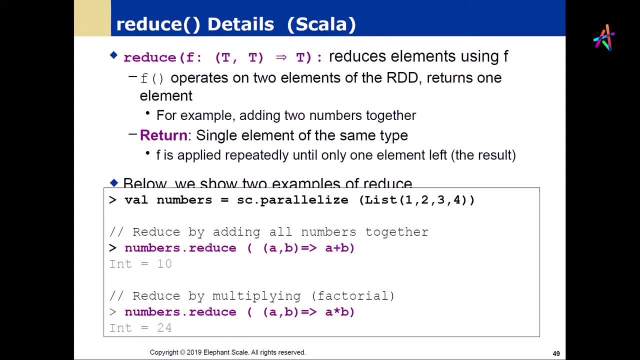 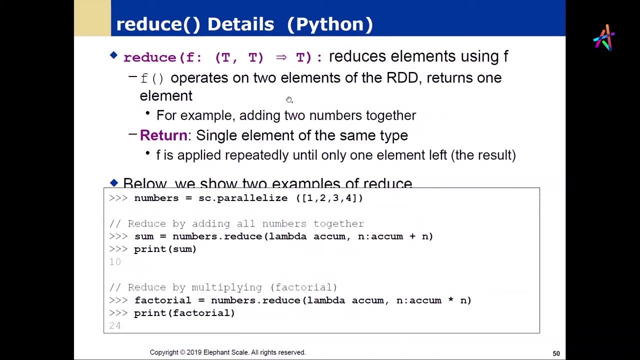 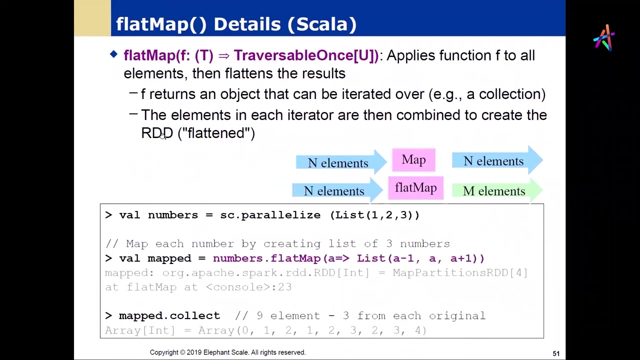 is a standard functional reduce operation returns a single element. so standard examples of reduce are multiplication, factorials and additions And again we do the parallelization and we, we operate it this way, The excuse me. Okay, so there's the reduction. We also have a flat map and this flat map, the difference between 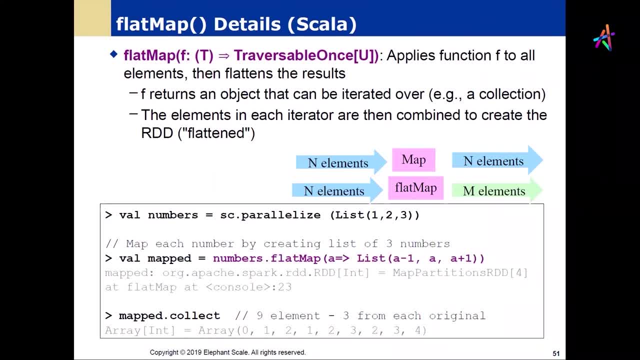 a map and a flat map is that it's a flat map and it's a flat map, and it's a flat map and it's a flat map. So what that means is that maps always the number of records in the output set is always. 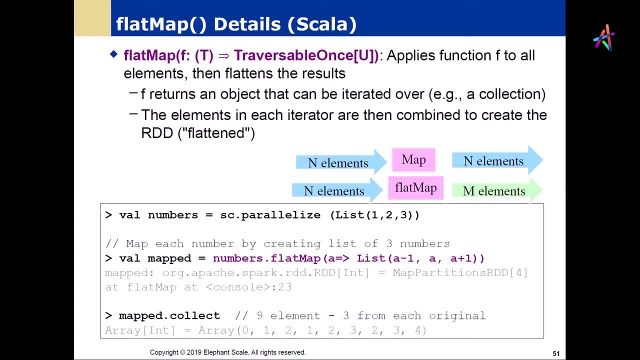 the same as the number of records in the input set. The flat map is the output is going to have. may have more or less records. For example, if I take a long string of text and I break it into words and return that that's a flat map, because I've got more records than I had before And so 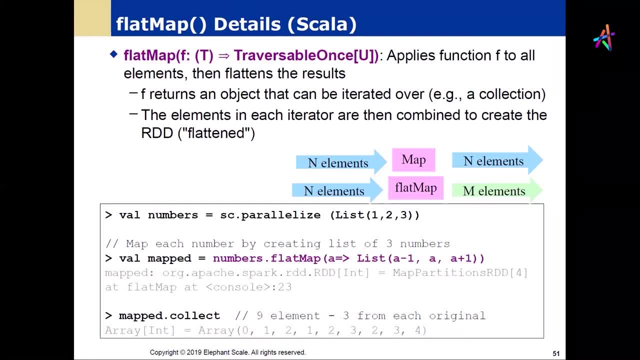 if I, if I also have a text, and let's see, well, if I take a, a, a, yeah, let me see. I'm just trying to think of another example of map. Another map might be that I have a string of words and I decide that I'm going to join all. 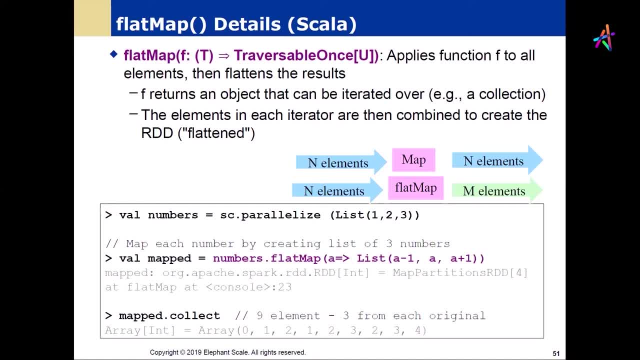 of the words that precede a punctuation mark to create a sentence. That also is a flat map, because I've got fewer objects coming out, So I have. so I always have a consistent size and it's important to distinguish these because that's going to factor into our optimization. 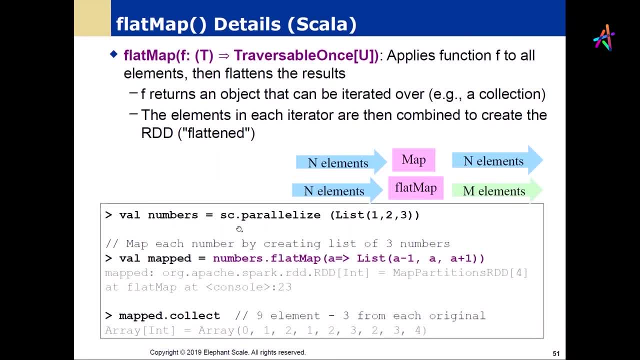 So here we've got- let me see reduce- flat map. So I've got my number of, I've got a parallelizing list of numbers and I'm going to create a list of three numbers out of each number. So I'm going 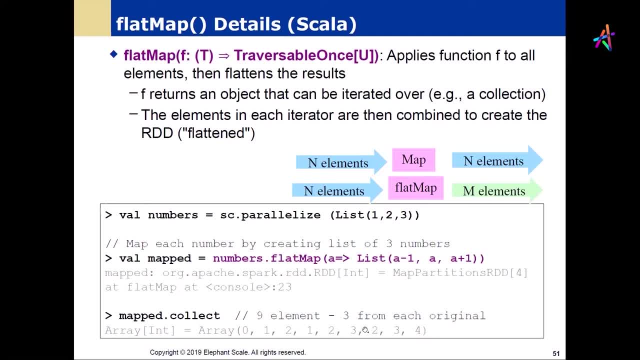 to wind up from one, two, three do zero. one, two, one, two and I wind up getting my my list of numbers, And so this is a flat map, because my original order three turns into an order nine list as a result of applying the map operation. 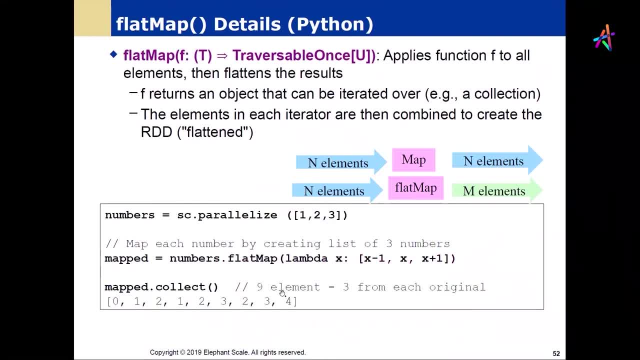 Okay, So where do we actually find flat maps? Flat maps often come when we want to break something down into finer structure or we want to coalesce structure into larger conceptual objects. That's generally. that's why I use the example of the sentence and the words. 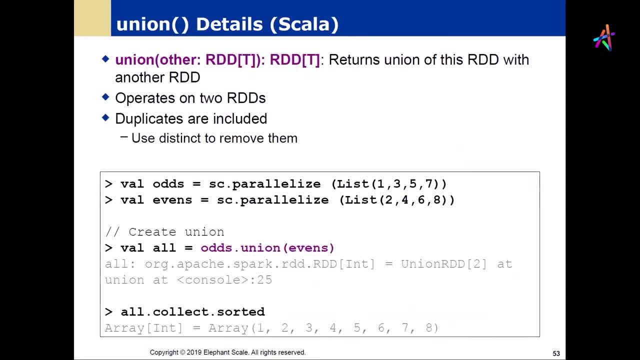 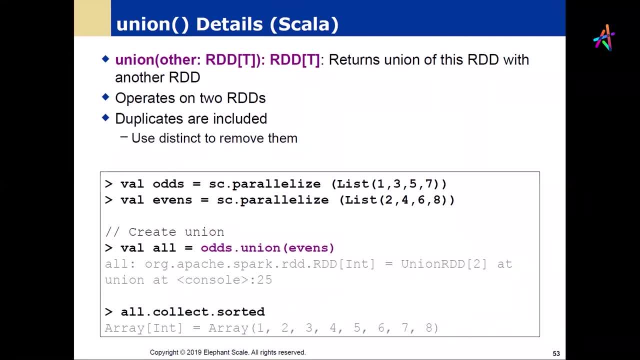 it returns to RDDs and creates a union for all of them. And again you can see that there's probably a couple of ways to actually optimize that as well. And now we're going to to do a collect on that and do a sort and we can use. 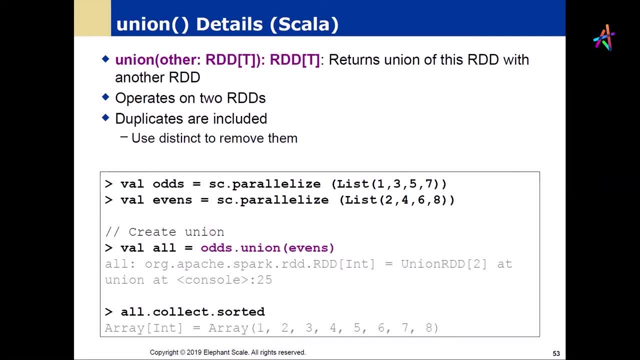 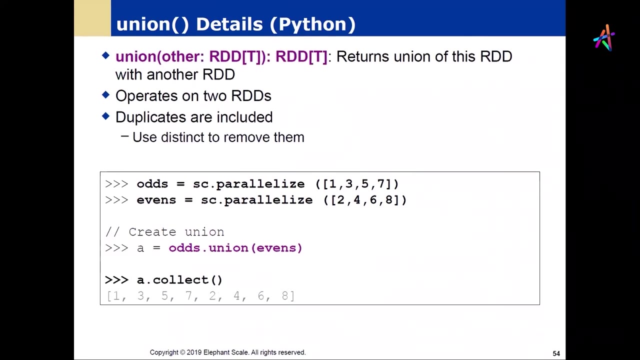 distinct to, to, to remove duplicates, And so so it. this is, this is um. this is um what we might call, uh, just a like an sql union as opposed to a set theoretic union. uh, we can also um return a union of this rdd with another rdd, so, um, we're. 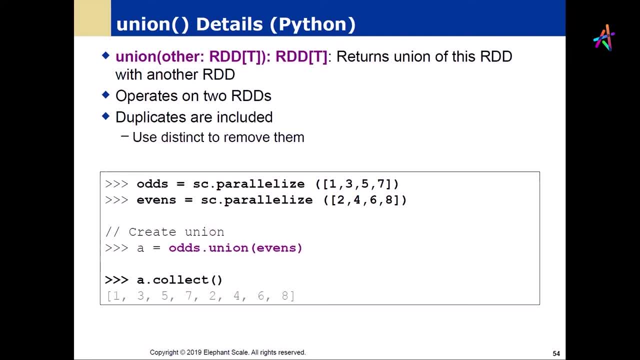 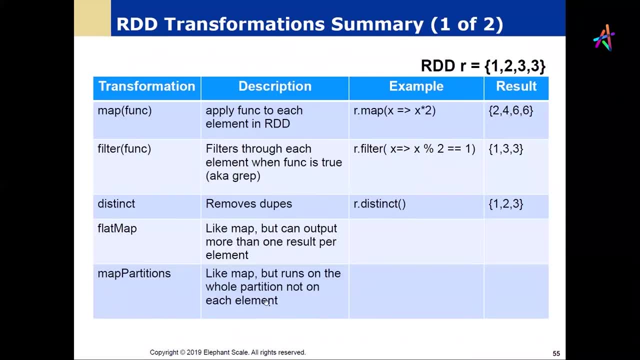 going to create a union of a particular rdd with uh, another one, a different uh in python, slightly different, so it's about the same. so here's our operations. mapping uh applies a function to each element in rdd and you get out the same uh, the same number of elements. each element may be changed. 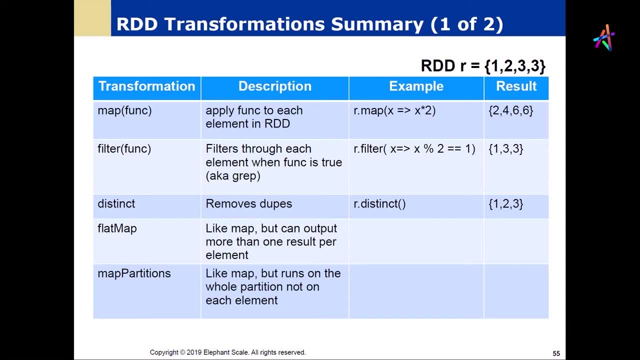 to a different type. so, for example, uh. an example of that is where i get a, a rdd containing string representations of of dates, and my map function turns them to into iso standard date objects- uh, or a date object of a particular type. or i get a um, a string representing a, uh, a numerical value. 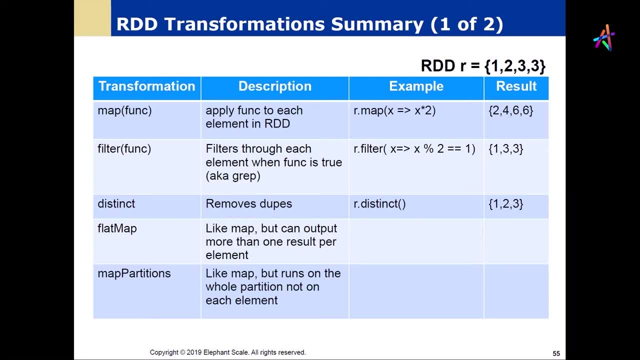 that's been read in from somewhere and my map turns it into an integer. so the map functions are not going to guarantee that the type of the object produced is the same as the object that went in, but it does guarantee that the number of objects is is the same. the filter, uh, throws away. 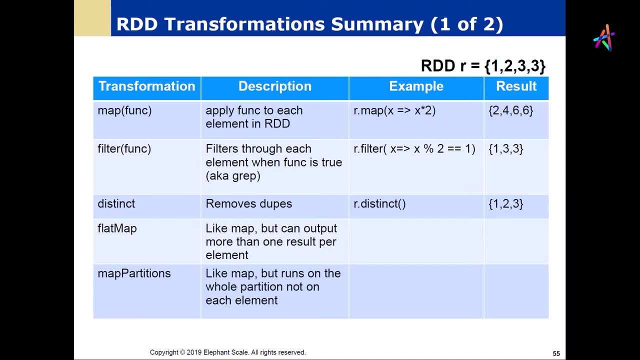 data always a useful operation to have. so the filter- the number of of records in the filtered set- is always less than or equal to the number of records in the previous set, and you're guaranteed that all of the data types are preserved because you're not doing any. 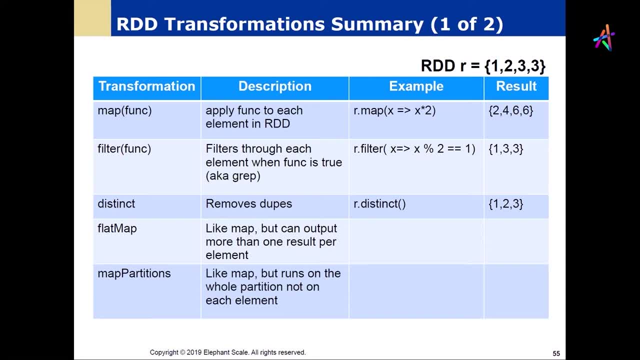 transformation of the underlying data. you can remove the duplicates of a of a set using distinct and flat map. uh is like map again uh. no guarantee that the output uh records are going to be the same type as the input records and there's no guarantee that the uh, that the uh. 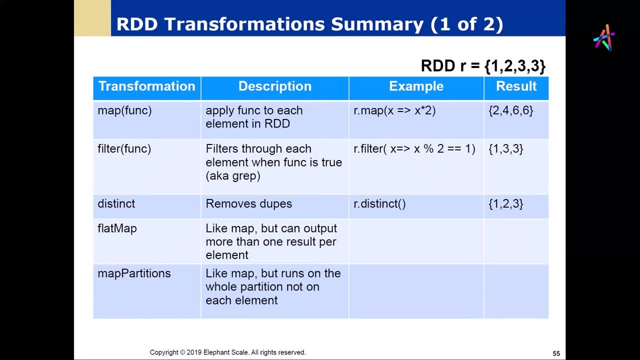 uh, guarantee that the uh uh uh data types are the same or the number of records are the same. all right, then we have map partitions, which is like map, but runs on the whole partition, not on each element, and i think we'll see an example of that later on. so it's a more of a group. 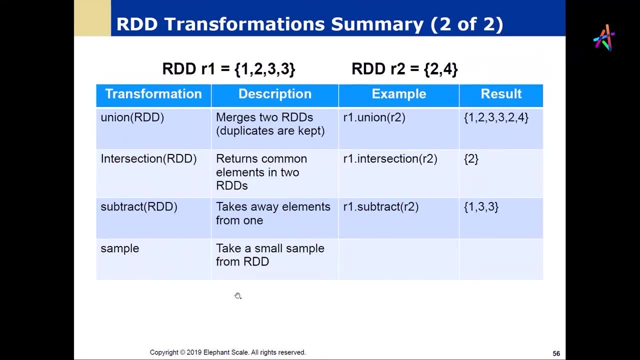 transformation, a couple of other things. we've got union. we saw that intersection. we didn't mention that, but it's fairly obvious what that does subtract. those are basically uh, the set theoretic, uh idea, uh, except for union. we have to remember we have to remove distincts because it is more of an sql. 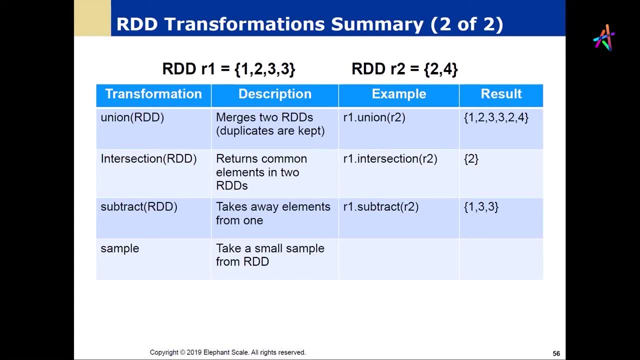 union and sample is a very useful one. we can take a small sample from the rdd. so, uh, if i want to know if my rdd is is going right and i just might want to grab a couple of quick samples out of it to say, did that transformation work properly? so we'll often sample as we go through as part of our data. 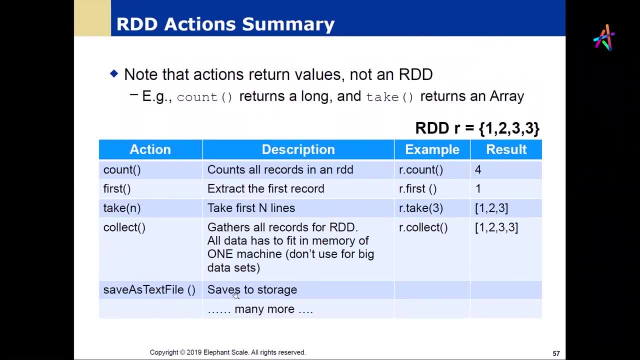 quality x, uh, um, data quality process, as the rdd actions, these return values that are not rdds and the ones we've seen here are, count first, which are fairly obvious: take, takes the first end lines, collect uh, gathers all the records, uh, which basically says uh, which basically takes all of the resulting rdd and and gives it back to you and then save. 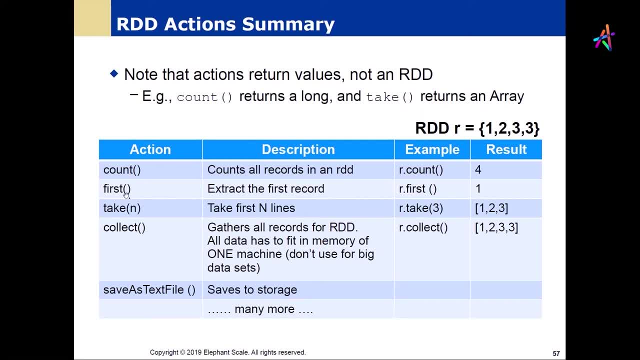 as a text file saves to storage, and there's a whole bunch of others but, but those are some of the more common ones. but again, notice that what we're getting back here is not an rdd. even with the rdd, we are not getting back an rdd. we are getting back a vector or a list or some other. 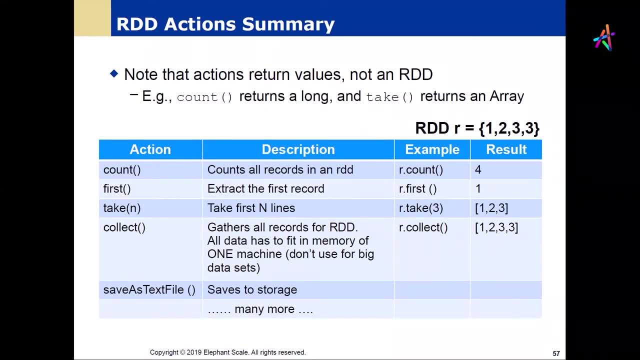 kind of of of construct that is not an rdd. so the rdds are only things that happen in the actual operations of the uh, of the data sets. all the rdds disappear after the last action has been, has been, has been executed. they do not exist, they're ephemeral. um, oh, let me see. 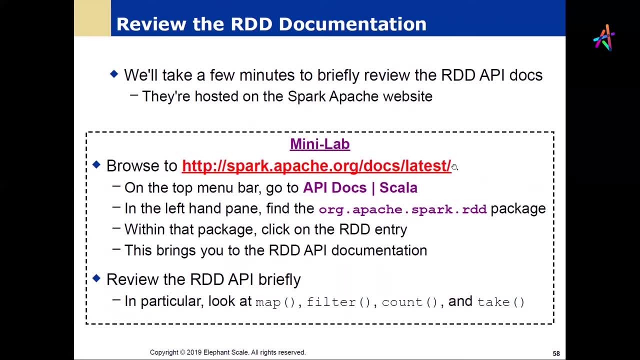 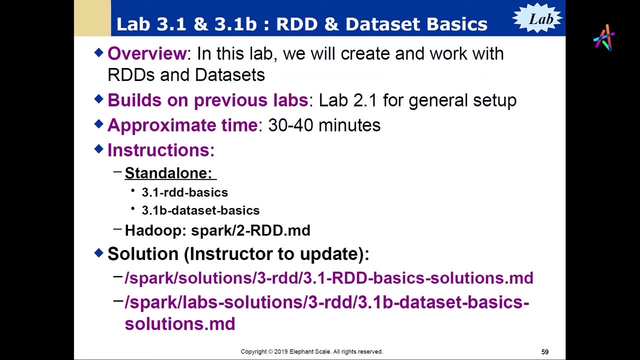 rdd documentation. uh, i'm not even sure if this is uh, this is still valid. um, so we'll come back and take a look at that a little bit later. uh, and we'll maybe browse on that. and now we've come to our first uh lab and, uh, we are going to uh um, do some some 30 to 40. 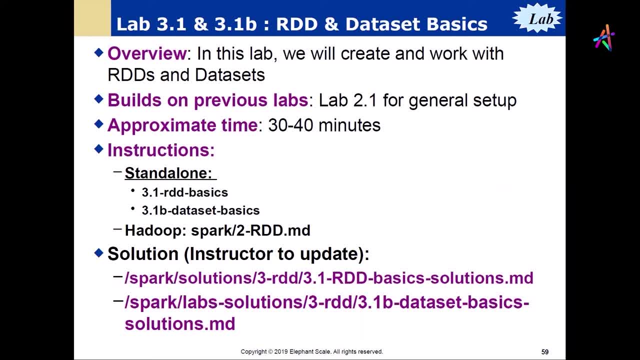 minutes. this is just going to be an opportunity for you guys to uh, uh, uh, uh, look at and uh, look at some of the things that are going on in the lab. and look at some of the things that are going on in the lab, and there are solutions to all of these things as well. and in order to do 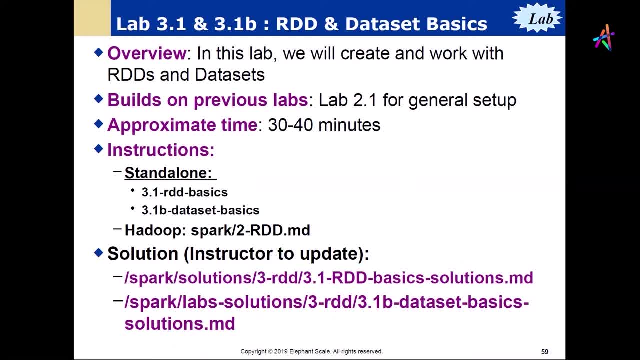 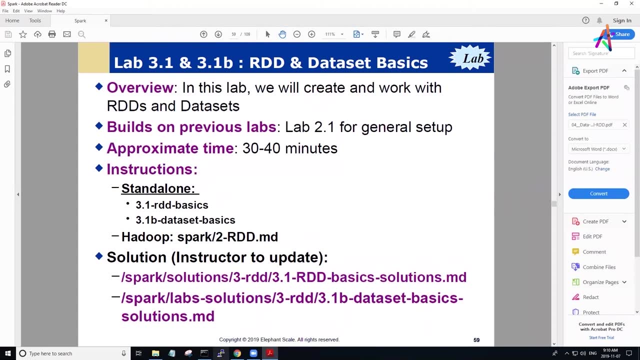 that we have to get you into that lab environment. so i have to go and find those and i'm going to be putting some, some things up here again. i'm still trying to work my way through all of this, this stuff, uh, so i'm going to go into my, okay. so first of all, any questions about the theory that we've 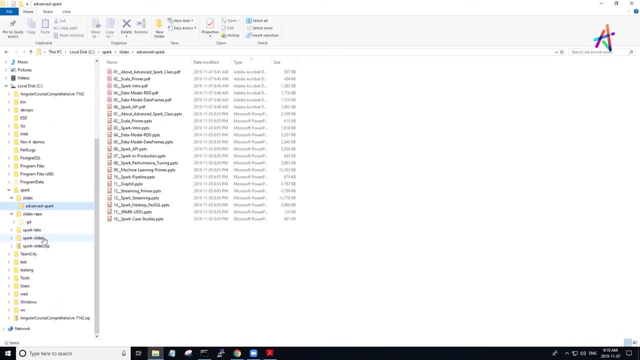 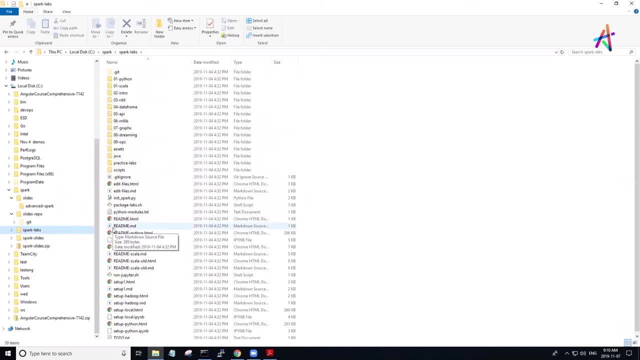 been talking about in the last couple of weeks, about the theory that we've been talking about in the last couple of weeks, about the theory that we've been talking about, uh, gerald here, different thing. so i i tried to connect. it feels like, uh, my ip is not reachable. 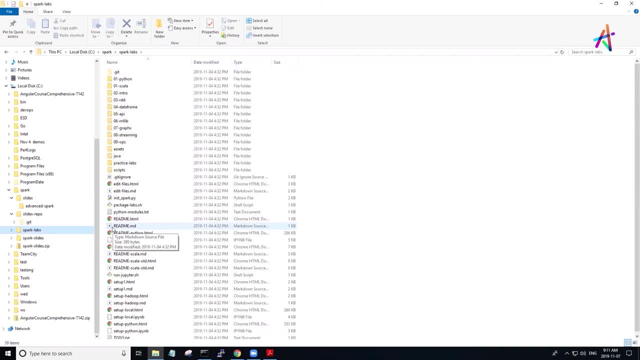 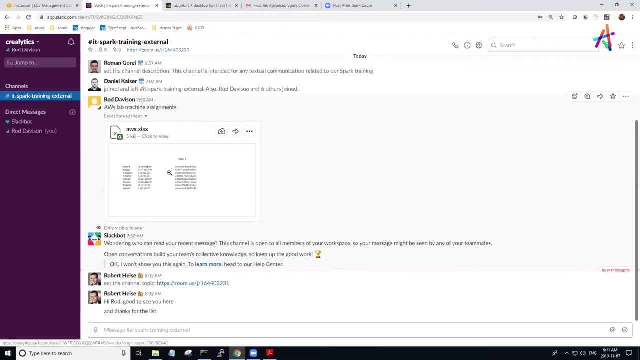 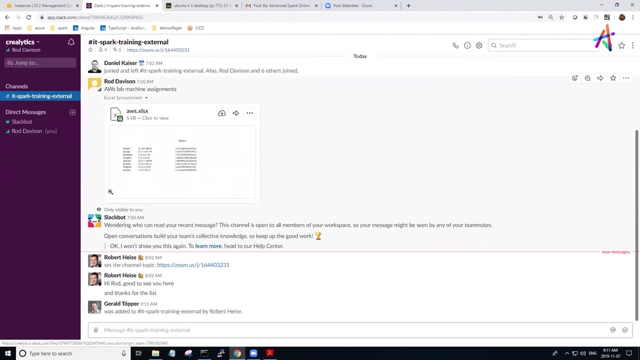 i mean the ip i had yesterday. oh yes, i, i gave you new machines, so there's a spreadsheet in the slack channel. you should get a new ip and, and it should, there's this spark training at the spark training. i think you missed to invite me. i, i'm gonna have you just now. yeah, so there it is. it's in the slack channel. uh, i tested my machine. 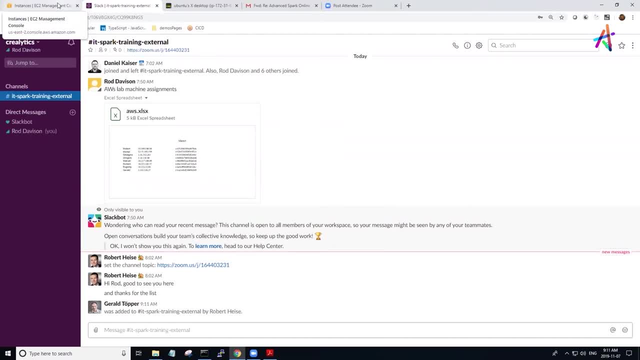 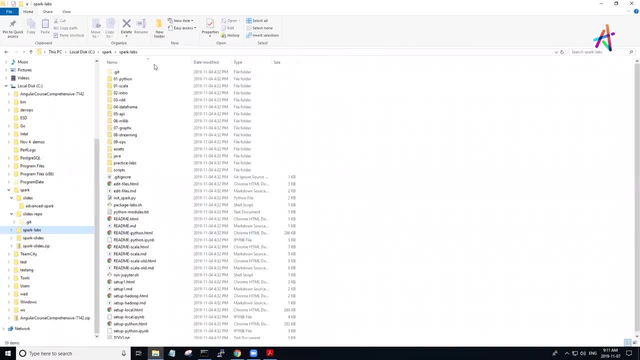 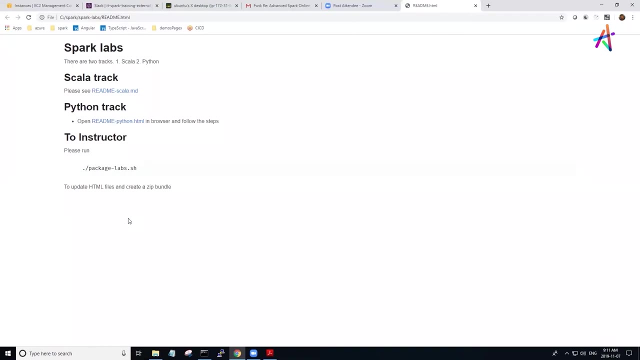 it works fine. i think somebody else took to their machine. it works fine, so we should be good on that. yeah, all right, thanks, okay, now i'll go over a couple of these files here. uh, these will be available to you in the machine and i'm going to try to make them available to uh to you all. uh, i'm going to. 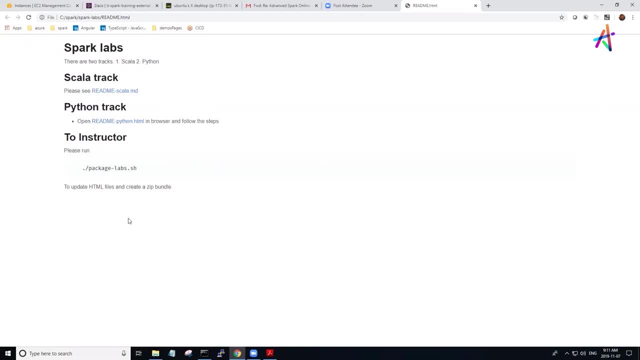 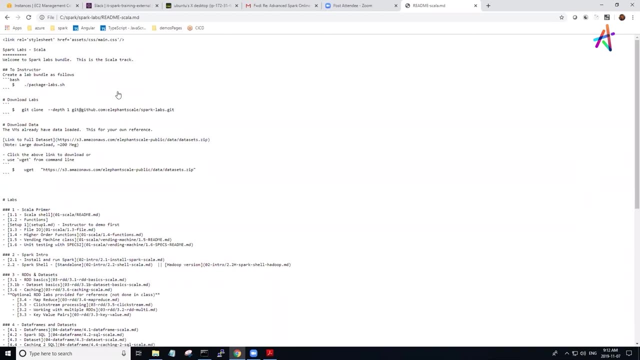 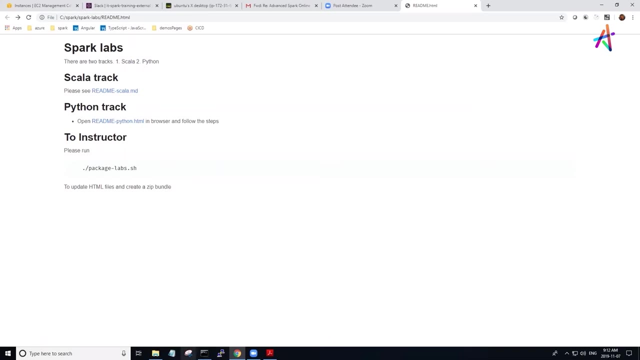 try to put them into an accessible repository so that you can also work on your machine with them as well. uh, so the um, there's some instructions here. uh and uh, okay, that's, that's where's our. there's a setup here i want to take a look at. um, read me, read me, read me. okay, so here's setup. 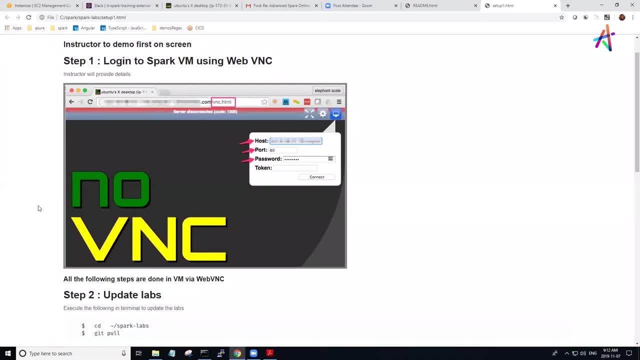 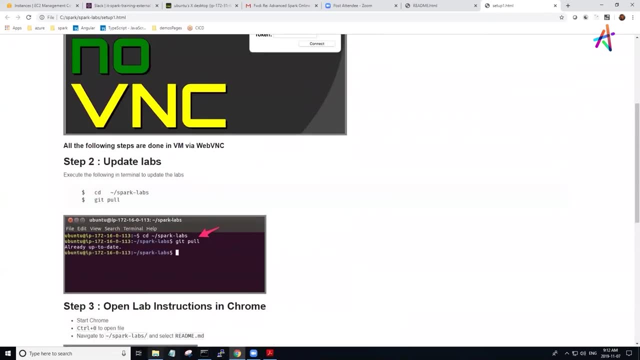 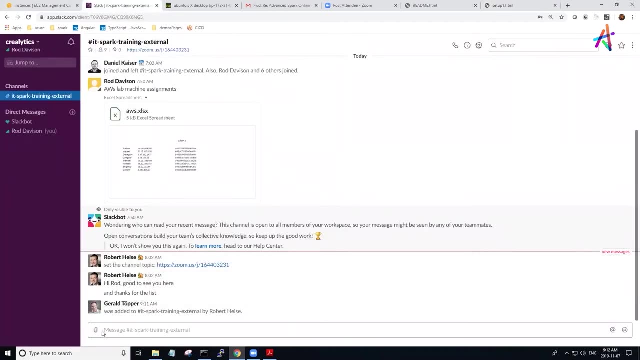 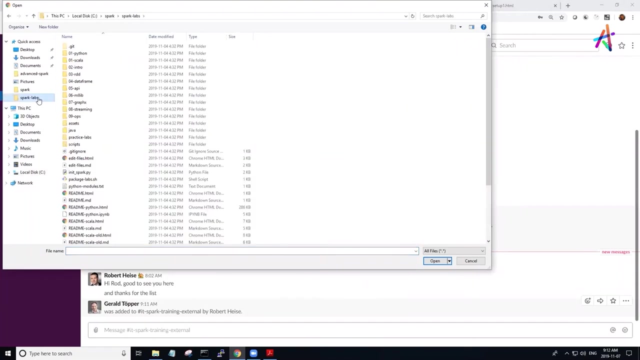 and this will- this will give you this information. i am going to put this into the slack channel so that you can, you can have the instructions, uh, and that'll be, that'll be useful. so, one of the slack channeling when you do set up. um, this, like whoever came up with this idea, the slack channel, you're brilliant. um, okay, and i'll just add: 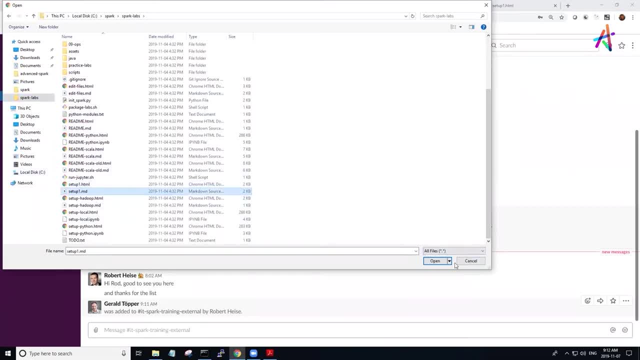 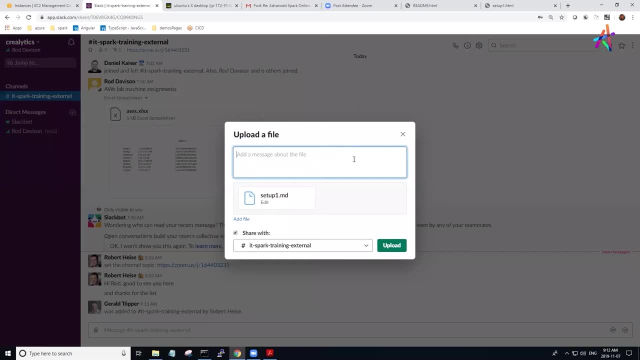 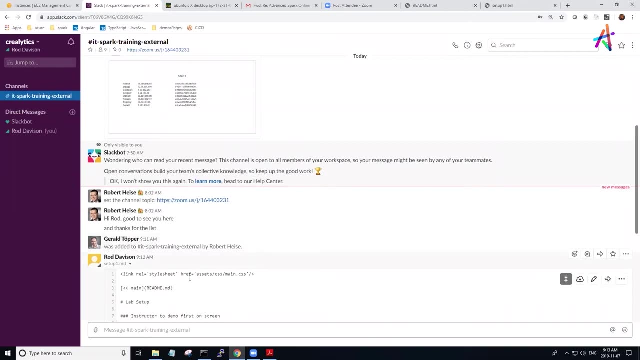 html to them. i'll give you the markdown. it might be a little bit easier to work with uh. so there's the setup. i'll put up some of the the uh. so this is the setup file. um, hopefully that'll you can open that into a uh, into a, an appropriate editor that will give 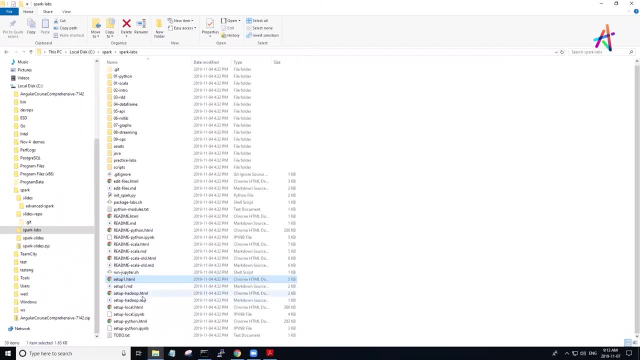 you a nice little markup. uh, i i'll put a couple of these setup files here so that you'll have them. uh, let me see. uh, we're. i don't think we're going to need hadoop at this particular point, but if you do, uh, i'll add the setup for hadoop and for scala and, um, uh, some of the edit files that are there. 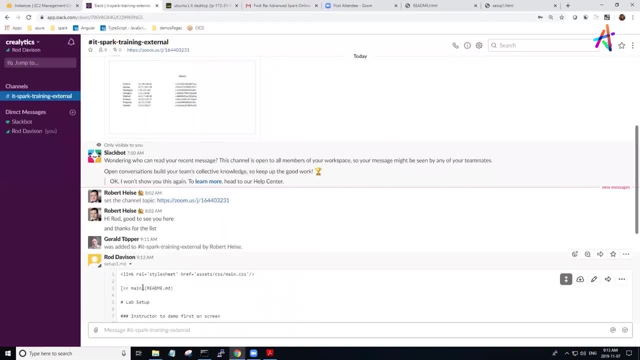 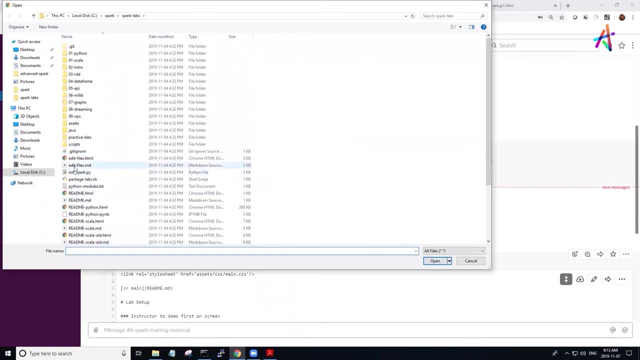 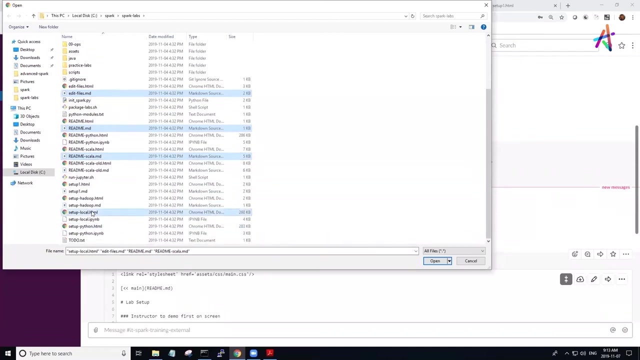 so we should have all of the setups that are there and i'll let you guys see if you can actually uh get into that environment. so the uh edit files, we'll add that one um, a couple of these files. we'll just dump them all into here. set up um. set up local. 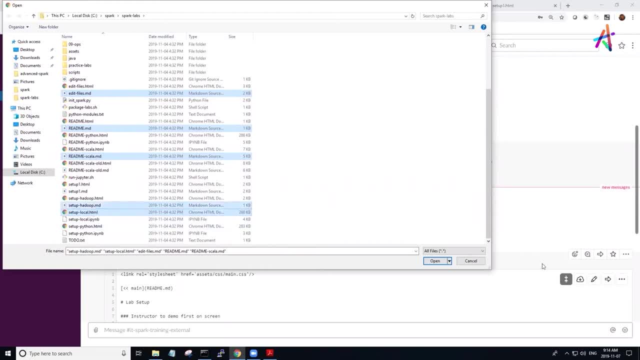 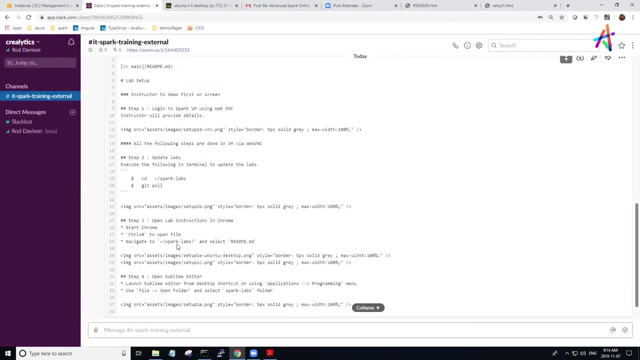 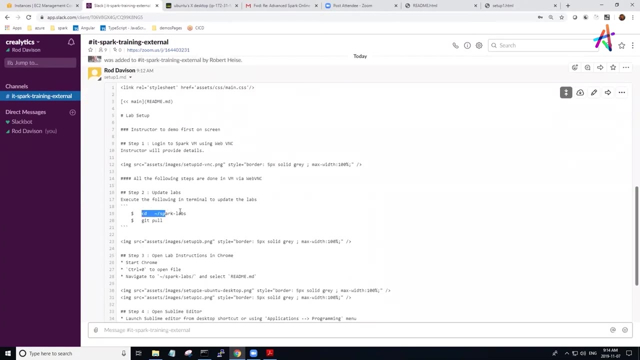 set up a dupe. i think that should be everything that you need, so i will dump those into there now. i will also. um, now in the setup, you'll also notice that you are going to be able to- uh, you're going to be setting up your environment so you can go ahead, and you can go ahead and set your car up to. 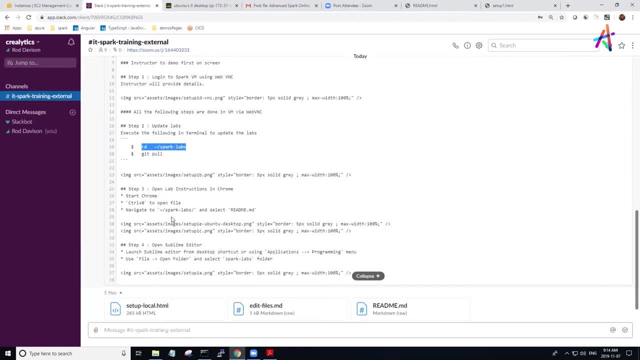 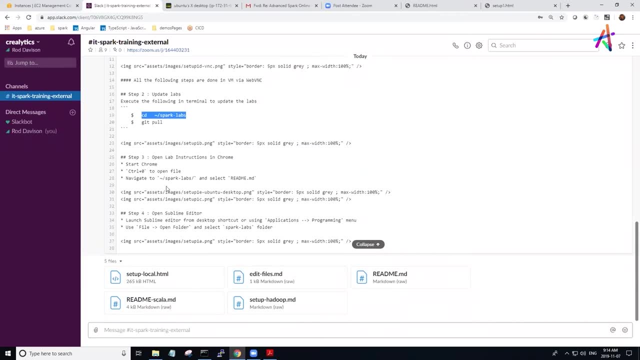 so you're going to do a pull on the spark labs, they are on your machine and, uh, you should be able to um to, uh, to to you, and this is what i think. one of the reasons why they wanted to have that desktop was because you're going to want to read the documents in the machine. so there is that. 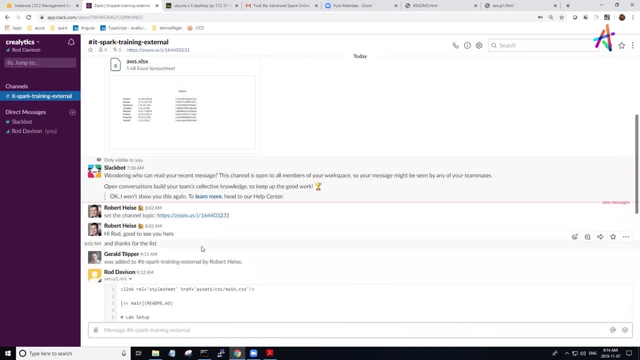 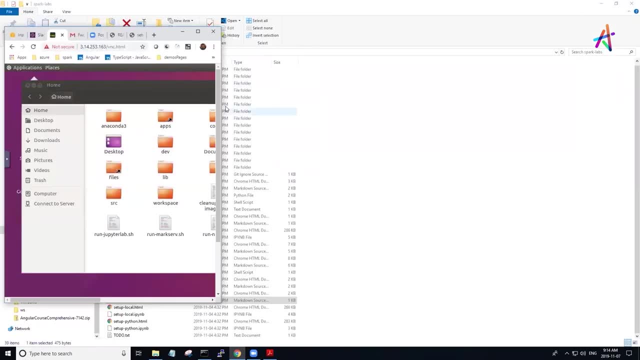 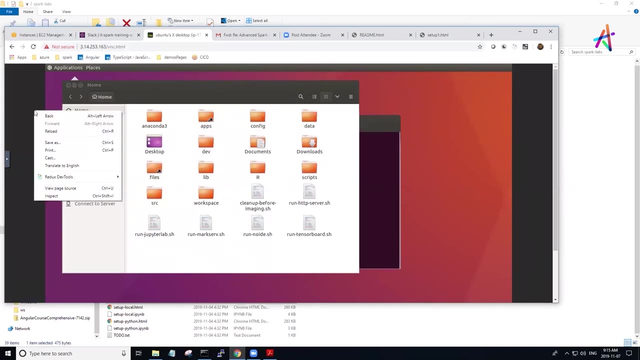 there is that as well. all right, so i'll let you guys see if you can manage the machines. um, like i said, i've i did uh so i could. like i said, i was able to get in and get the vnc started, so you should be able to get the various uh tools that you need here: uh, including the uh, including the. 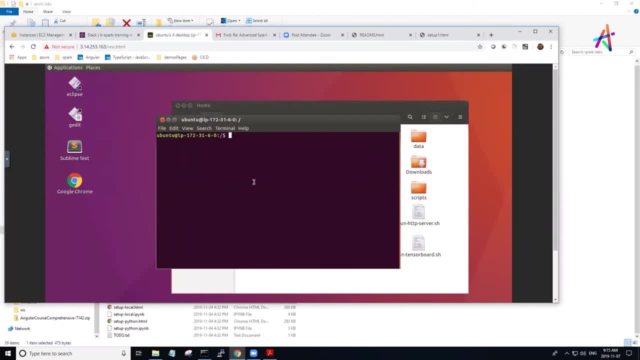 shell, uh, you should be able to get it. you've got a shell here that, uh, um, that should, uh, should, you should be able to manipulate with, or you can just sh into the shell until you need to edit something. all right, so, uh, you should be able to browse the various files. 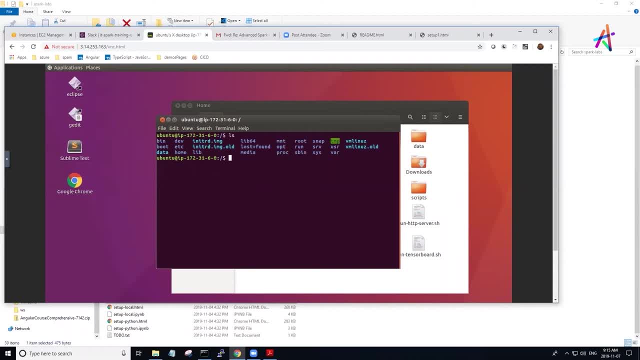 that are in there. i've given you copies so that you can look at them on your local machine as well, in case there's any issues. all right, so i will let you guys go to it, um and uh, we'll see if there's any issues and uh, i i hope there's not. i i i ran through this setup once before. 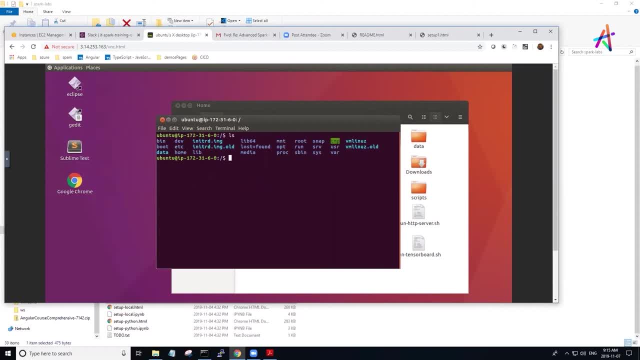 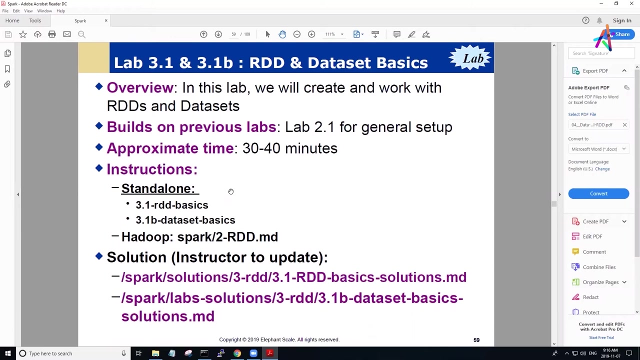 and i didn't have any issues, so we'll make sure that everything works all right. sound good? yep, okay, pardon, uh, yeah, just just read through the setup. um and uh, let's, let's, uh. actually it's a good question, i just wanted to give those to you. uh, so, um, uh so, the lab 241, lab three: oh yeah, we want to also go. 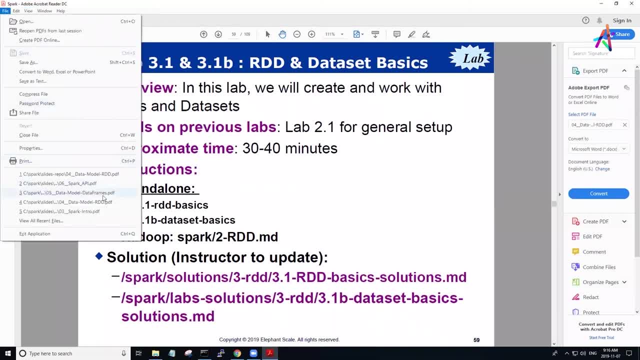 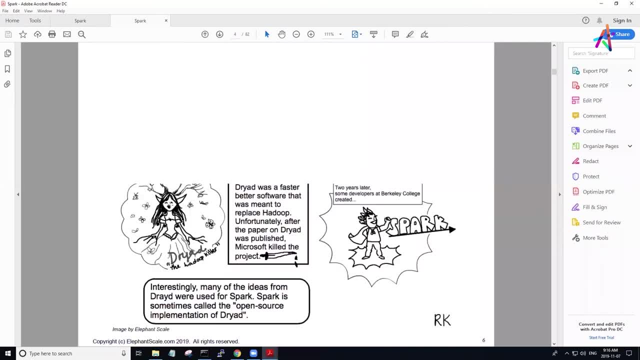 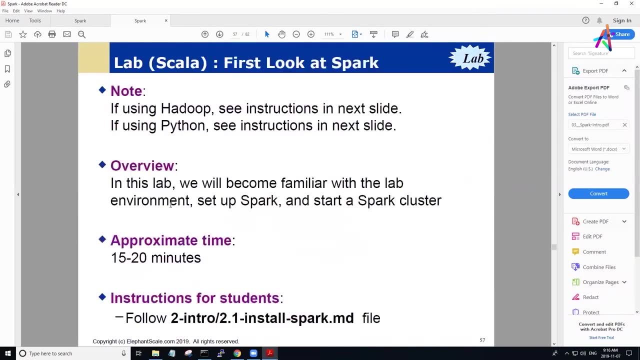 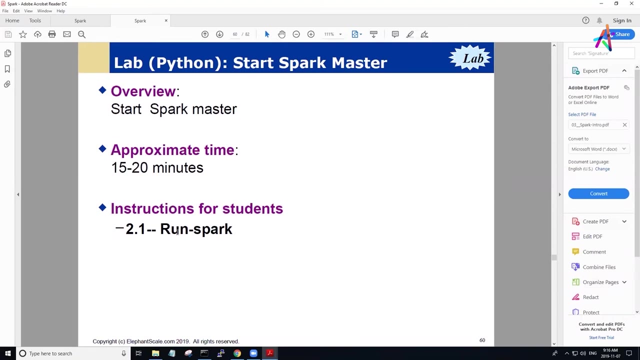 and and pull this slide up here. um, okay, and this is the one i, this is the one i said: we, we, uh, we'll come to today. okay, we ran out of time, so i will put this slide up on the screen for this lab too. there we go, uh, so so you want to to look for your run spark? uh, instructions, that should be. 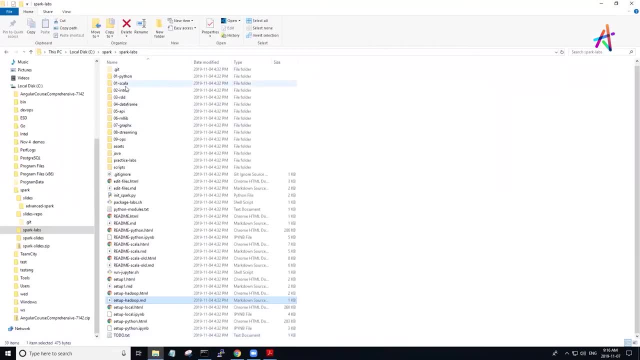 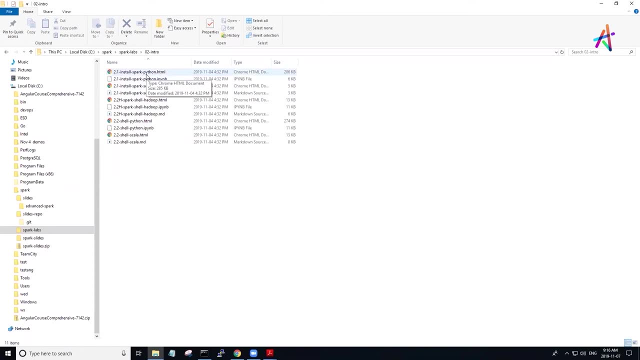 in your uh, in your setup. so i think that should be here, uh, and so you'll find the instructions in that folder. zero two: uh to install uh into all spark uh and in the other things. all right, so that should be in your once you do the setup. 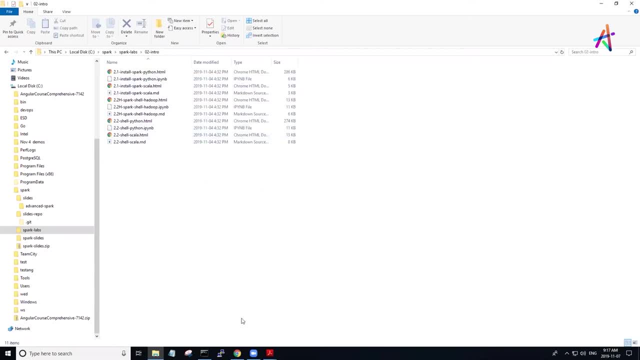 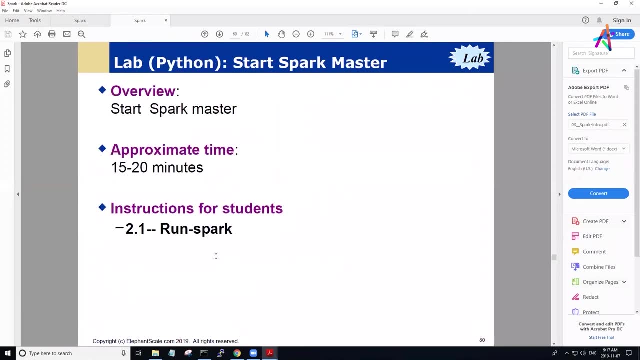 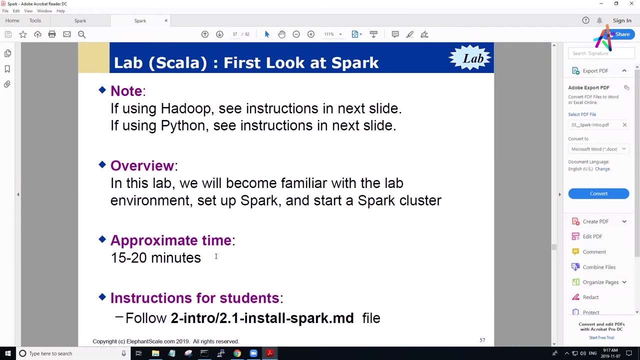 and you do a pull on that labs, you should have access to all of these things and the uh and uh you should be able to. uh to look at. uh, we'll do lab. that's python um scale first. look, there we go. that's the one we're using here. um and again, you don't necessarily have to use the dupe at this. 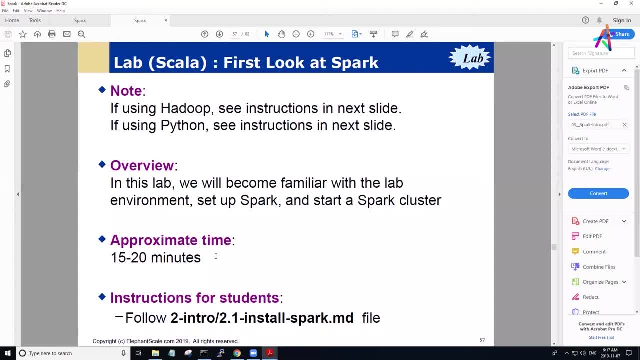 point. uh, you may want to use it later, uh, but uh, you want to basically set up a spark cluster. so there we go, it's 2.1 install spark file. that will give you the instructions to install. all right, is anybody confused? did i confuse it? yes, uh, so there's supposed to be a folder in the home directory of the user that. 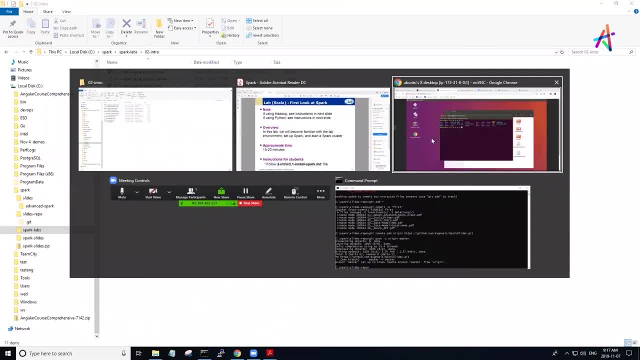 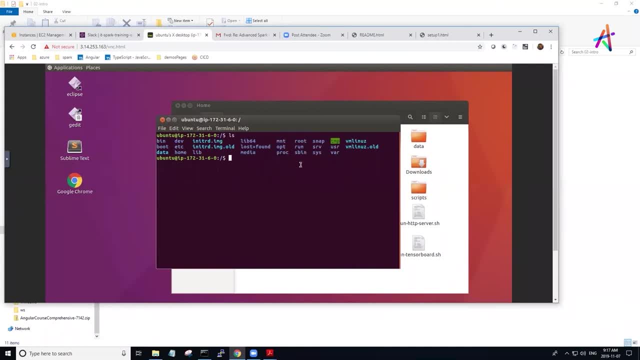 we log into the machine or there should be. um, so it's referring to a r dash lab folder- the instructions you send us- and i don't see it. okay, i think we may have to actually do a setup on that here. um, all right, let's take a look on that. good point. 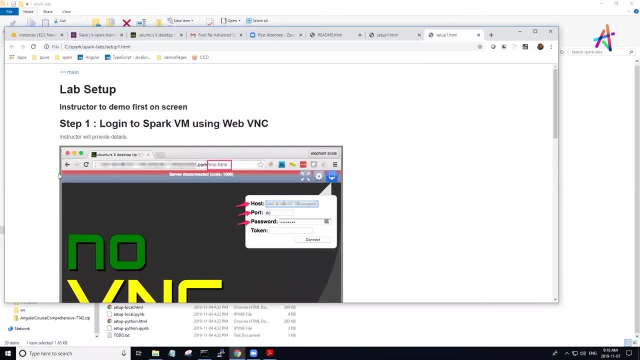 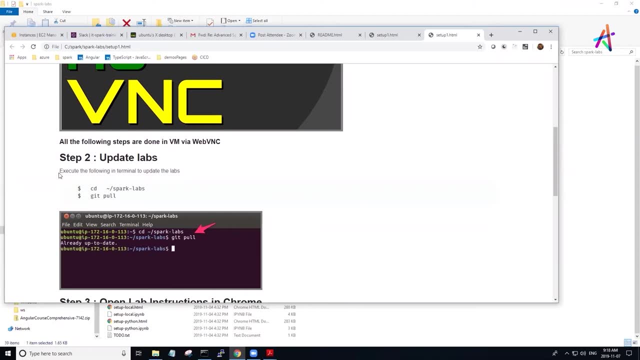 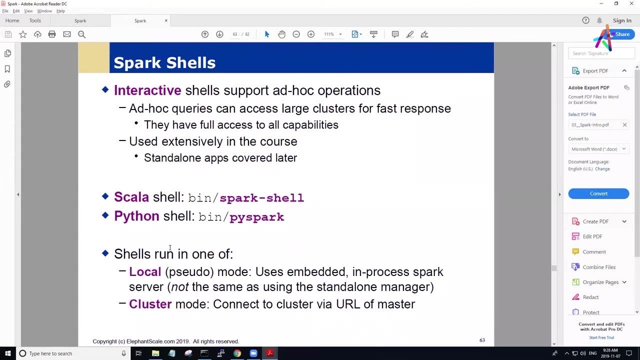 um setup. so let's take a look at setup. okay, so we log into to the spark vm. uh, we should see um terminal to update the labs. okay, so the two things that you want to do. i know, i'm, i'm. i find it a little bit confusing. 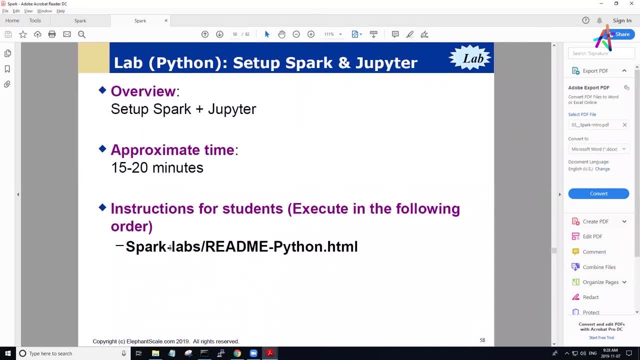 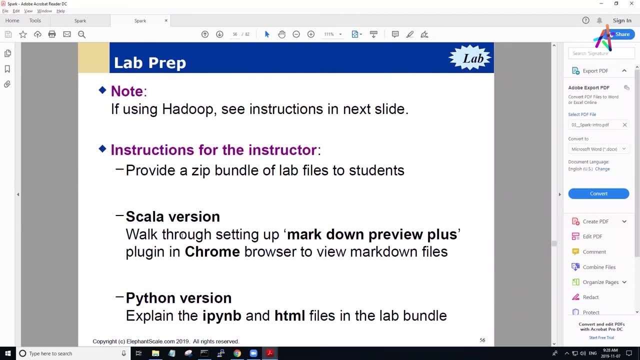 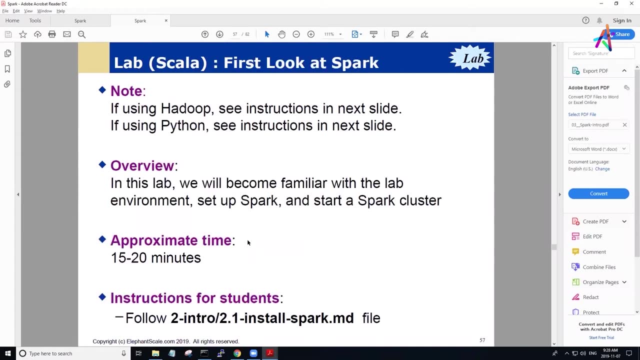 as well too, here. okay, so the um. there is the, the setup. uh, so the lab prep. so i've given you the zip fundle. uh, uh, you can mark down. uh, now we're not using python so we're not going to be working with that. uh, so the instruction is in in lab two. 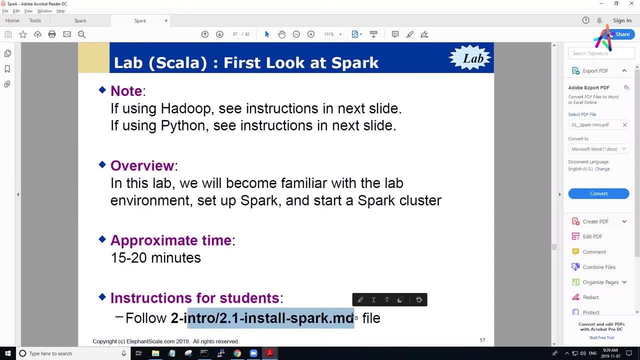 intro installs the spark file. that's the file that's in the instructions for this lab. okay, so this lab is about installing spark. all right, i cannot clone the electron scale data center. i have permission tonight. yeah, yeah, exactly, i'm in the folder. well, is that for the labs? 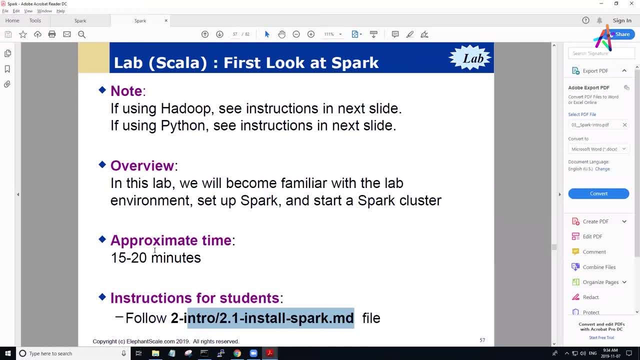 no, the lab is okay, it's after the data set. okay, so you're supposed to do this geek clone elephant lab data sets? but okay, hold on for just a second. no, it takes structure. actually says if the data direct directory is missing. for me, the data directory is present. 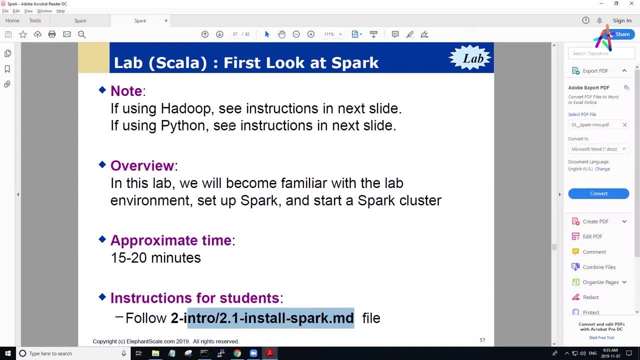 yeah, but i went now. but first i went to the data directory. i tried to pull. it didn't work, so i just deleted it and tried to pull directly from the home, which doesn't work as well. so those didn't. yeah, i think. i think that i'm sorry then i think the data directory poll is just done, in case. 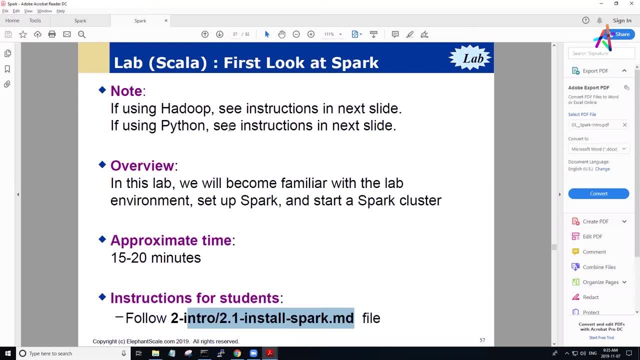 an update in the data directory. uh, i think the data is already there on the machine that you can use. i have a question. so this uh data folder, is that the same that is located on the s3 dot amazon awscom? is that the same thing? because, uh, i downloaded it from there and it was just fine. yeah, i, i don't. 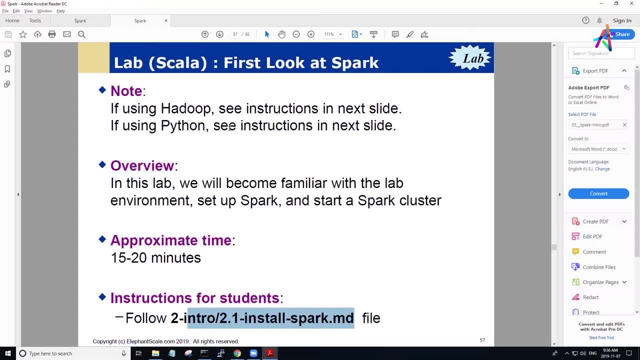 i don't know again, i just was given these, these kinds of lab materials just the other day, so i haven't gone through all of it. so, uh, let me take a look and see if i can figure something out. just give me a moment, okay. okay, if you go into the files directory, you'll see. 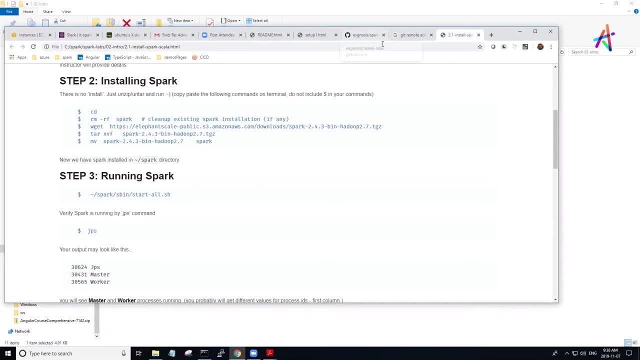 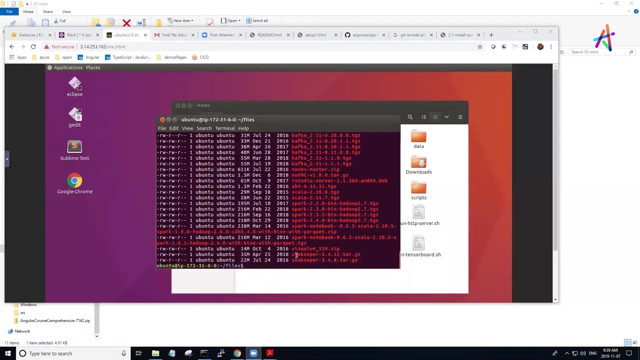 um, you'll see the, uh, the, the archives, the file archives in there. it looks like. well on the hand, i want to make sure those actually are there. yeah, so it looks like those are already in your files directory. a little easier to see it this way, i think. 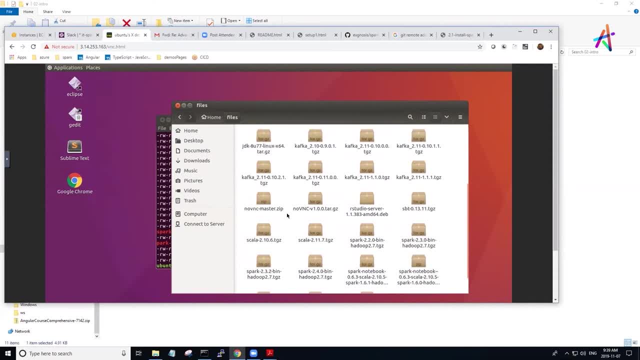 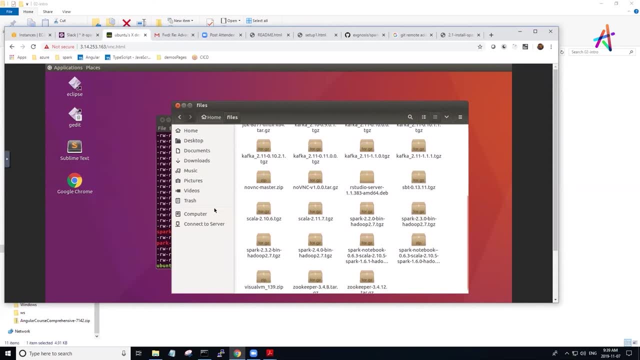 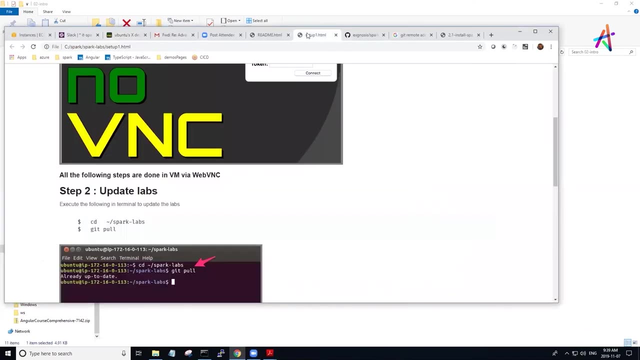 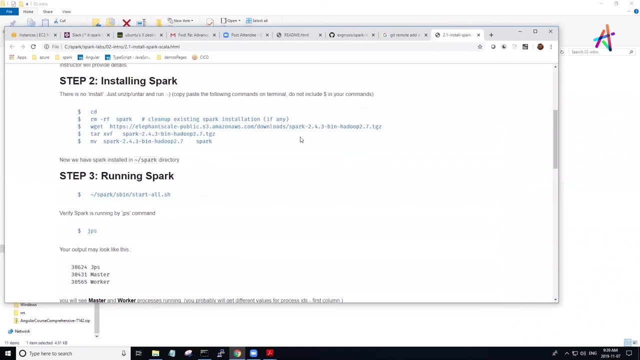 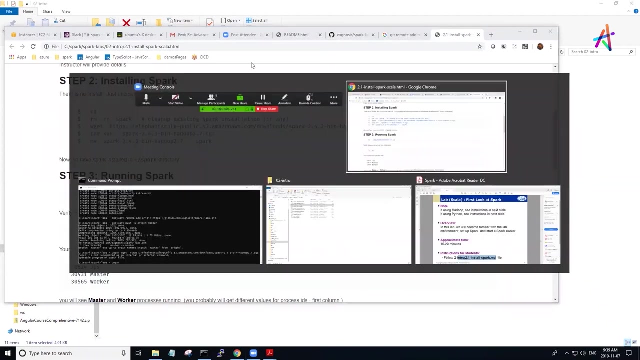 so you should be able to find it in that directory. okay, yeah, which one we're looking for? let me find out. we are looking for um hope. so we are looking for spark 2.4.3, bin hadoop 2.7. so that should be there, yeah. 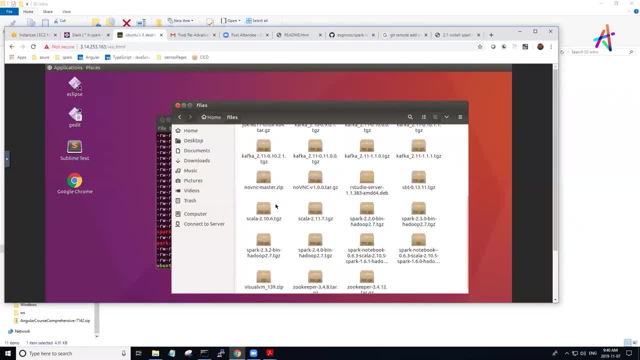 it's not this. i will do a date of it. spark two points. i think he deleted the data folder. yeah, yeah, thanks. so not the spark line is the problem, but the data folder. yeah, it's the last line of the installation, so data was present. we wouldn't need to delete it. but he deleted it and wanted to clone it again. 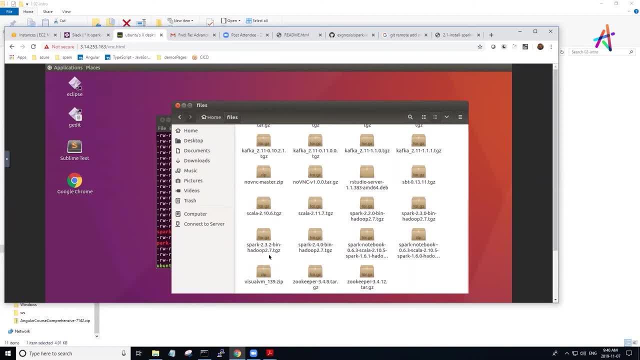 okay, who? who was that that had the problem with the data? that's me, gregory, because like, uh, yeah, okay, i don't know if we're gonna, i don't know if you're gonna, uh, we can actually get that back down, but what i'll do, gregory, is. 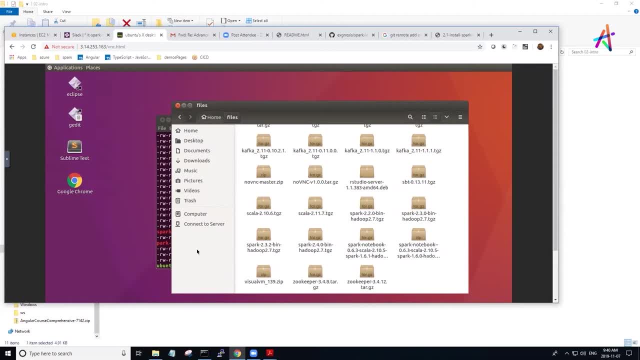 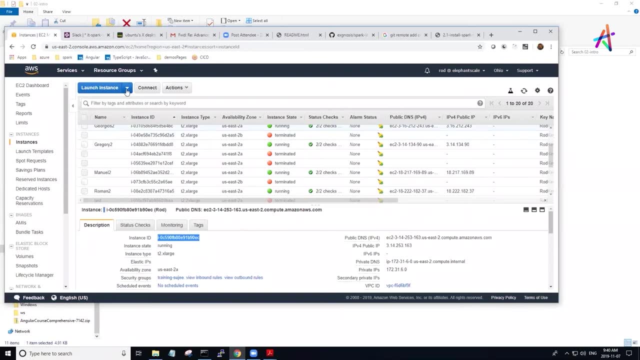 i'll spin you up another machine. okay, you'll just take a moment, you can. you can go back to, to, uh, so i'll just i'll just do a quick one. no, but i mean i, i can, i can sort it out with the link. oh okay, okay, because, because, like i said, these are no consequences. environments, if you, if you. 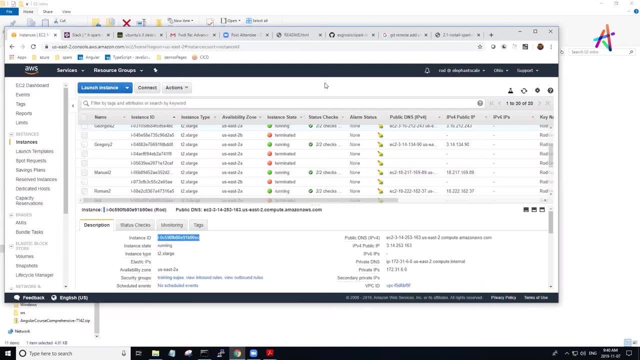 completely destroy the environment. don't worry about it, we'll just spin up another. no, no, no, but like i'll just get backwards. okay, let me know if you want me to do something like that for you. okay, just send me the link and i'll do it for you, okay. 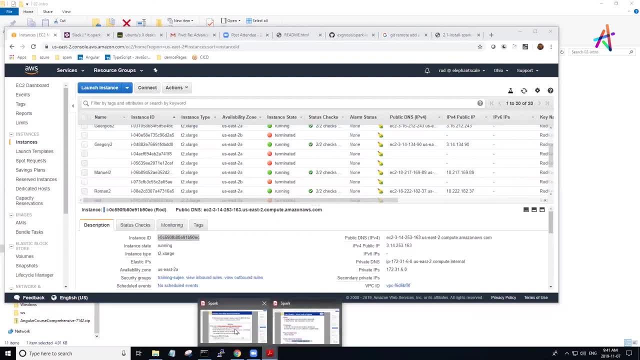 just send me the link and i'll do it for you. okay, just send me the link and i'll do it for you. okay, see if i can access to. yeah, define that romance and so be okay. so, yeah, i just wanted to confirm the link that i've sent in slack. is that the correct one? 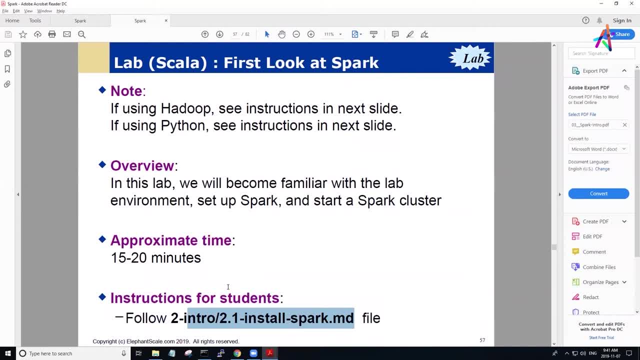 i'm sorry. the link that i've sent in slack. uh, could you please take a look at that. is that the correct one for the data? uh, let me take a look in slack. hold on, i believe it should be. i've got it from some other file, not from from the same one, but 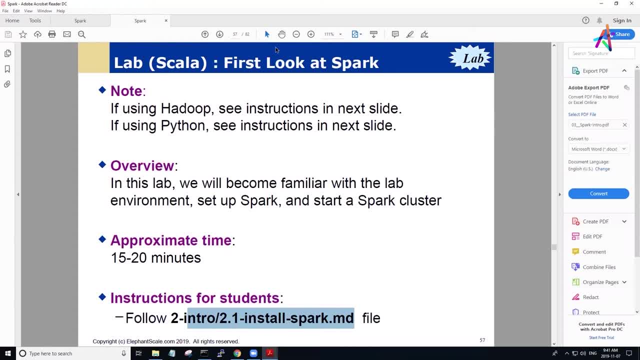 it seems like, uh, looking by looking at the structure, it seems like it's the same one as the one from git, but i'm not sure. yeah, i, i suspect it probably is okay. i, i think that. okay, i think, i think that elephant scale uses a fairly standard set of data sets, so they're probably located in. 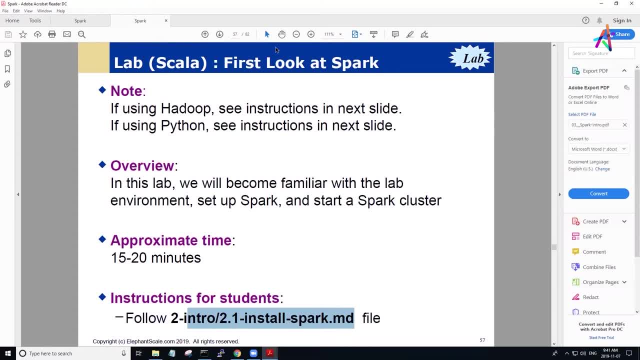 multiple places. i believe everyone is done. is anyone not done? i am done, okay, everyone else. anyone else done? done, okay. good, i think we're anybody having issues aside from deleting data sets. so i wasn't trying to be snarky there. it's actually a real issue. i have done far worse. 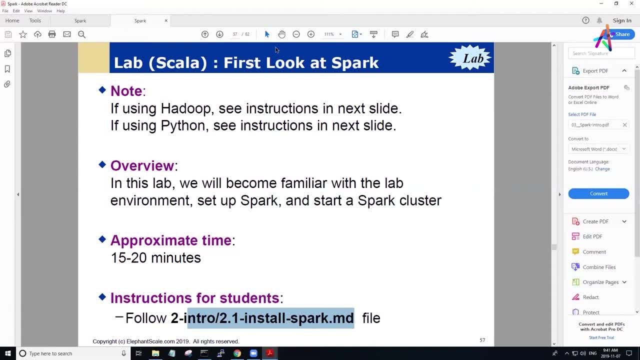 i've actually even done that rm minus rf slash by mistake, because i've left a space out of the out of a path name. took me two days to fix it. okay, um, okay, okay. so we've done the um, the general setup. so, uh, the, the next um. 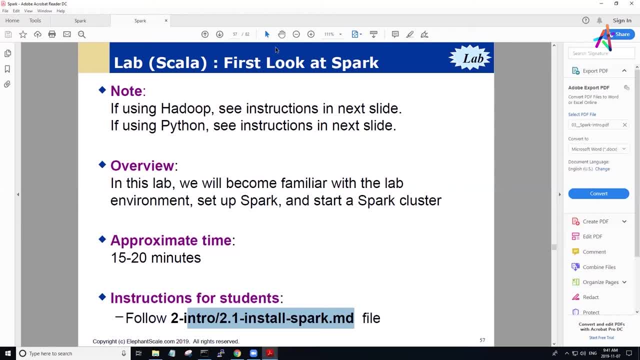 okay, i'll tell you about updating the solution here too. so, uh, but again, once we've done that, it's uh quarter to the hour, so what we'll do is let you guys move on to lab uh 3.1 and 3.1b. 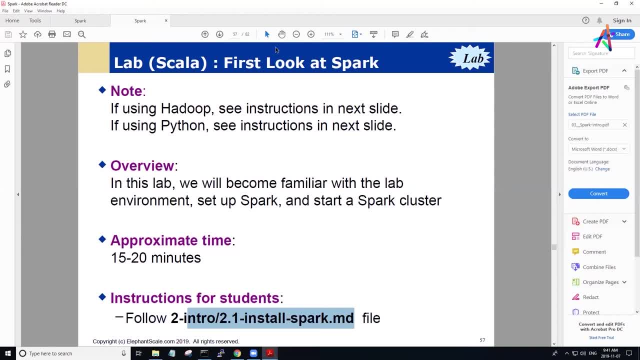 actually we do 3.1. i think maybe we can do 3.1b as well. well, at least let's do 3.1 and 3.1b. we'll come back. we're going to talk about data set basics as well, all right, 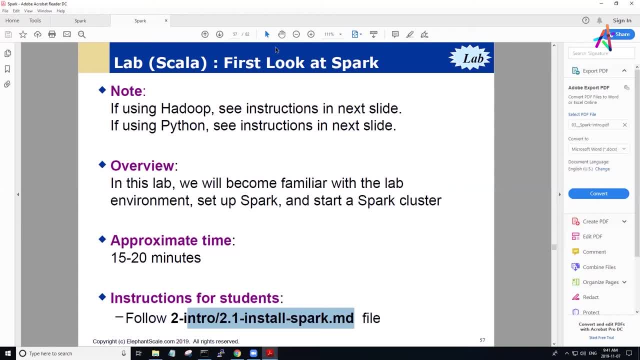 so we can get get us started on that. and, uh, we'll take a break at 10- you for 15 minutes and we'll come back and resume this and then we'll get on with the rest of the theory. okay, sound like a good plan. yeah, yep, awesome. okay, i will be here with my headphones. 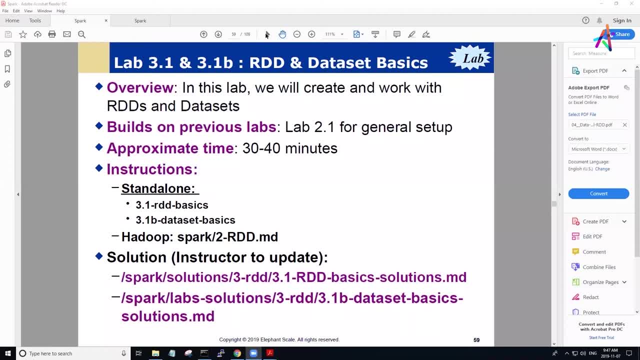 on, but i will be muted. so if you do ask me something, give me a moment to unmute myself. yeah, um, what's the reason why this? let's say it's a part of gel. yeah, it's implemented as two different tasks, even though it's a single text file. i have four cores. 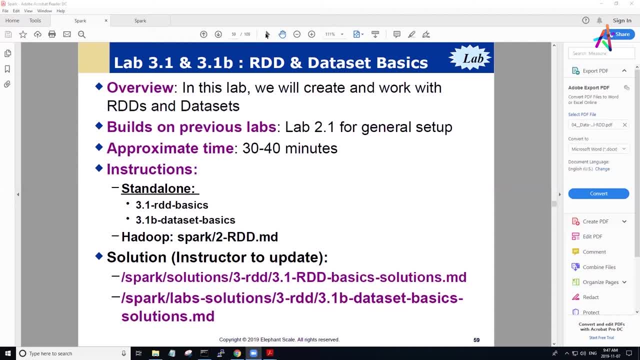 why so? if i look at the amount of tasks, yeah, there's two tasks, exactly. so the number of permissions for this text file. why is it two? probably because- good question- i have to like put in this one. this is the file b. what's the size of the file? 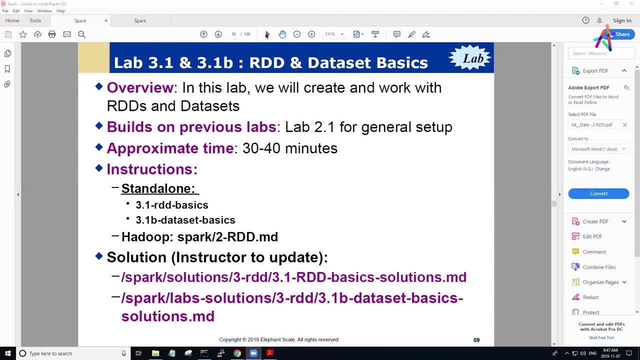 okay, so it's usually. if the file takes like more than two blocks, then i mean the file and the partition, usually in hgfs, would be minimum. the amount of nodes you have like if it's two blocks might be loaded as two partitions: just 134 bytes. and this is a file on the local file system, not in heroes. so at some point 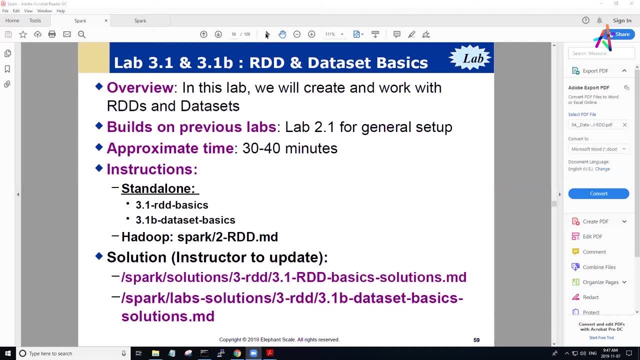 spark decides that if you create two, yeah, but like check this part, yeah, but the spark shell, uh, the spark shell basically, uh, uses local star, so which you should, basically, and you say it's four core. i haven't checked the machine, to be honest. so four cores, yes, and that's also what. 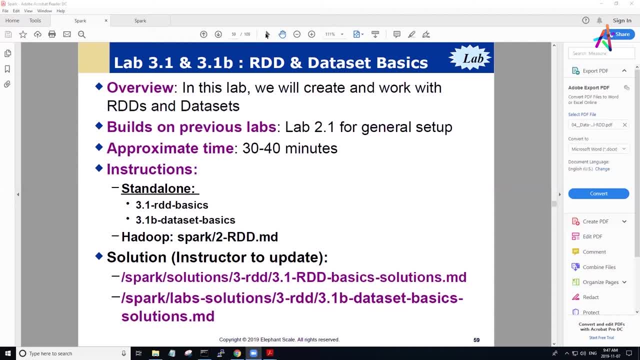 i see on the worker, so on the executor summary: uh, it claims to have it, for course, so, but the thing is, the thing is it depends, like the configuration also of the, the spark shell itself, because you have this mean, uh, like the parallelism which is usually 200 by. 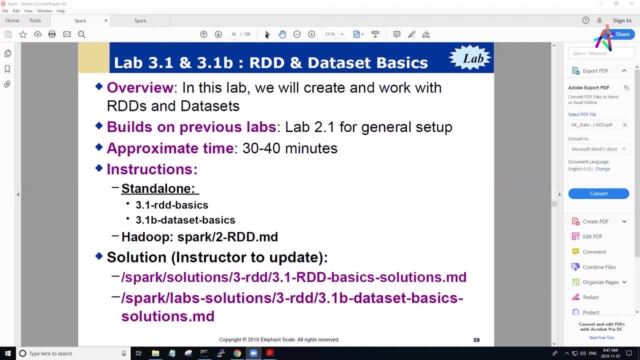 default, which means that it doesn't really care about the amount of core that you have. it will use 200.. if possible- and here, for example, like maybe that could be changed to two, or i don't know we have- you have to check the spark shell, uh, the spark conf that is used by spark shell, otherwise you 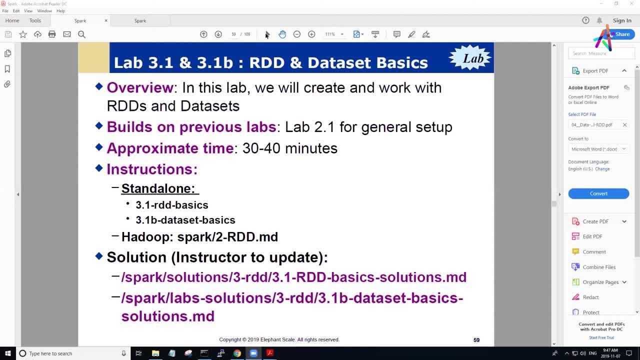 cannot be sure, because the default parallelism should be 200, but again, since it appeared to be a kind of a custom homemade uh bandwidth spark, then there might be something else here related to the the. so you were just talking about the simple word count. right, the first task, the count, uh, guess or just. 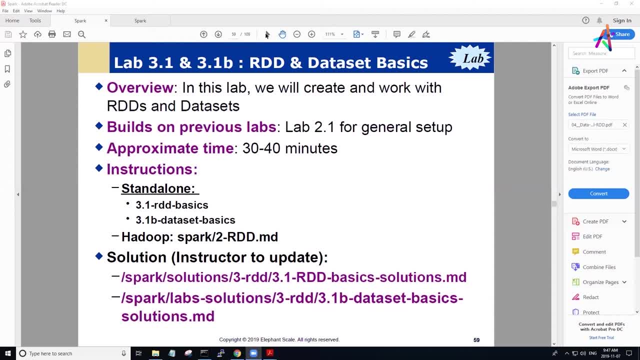 fill it on account and that's with a sample. finally, yeah, but you have two tasks, but you have none of. that is different. you have two tasks, two stages. is that enough? one stage, yes, but two tasks, yes, sure. two partitions: yes, for a file of one hundred. 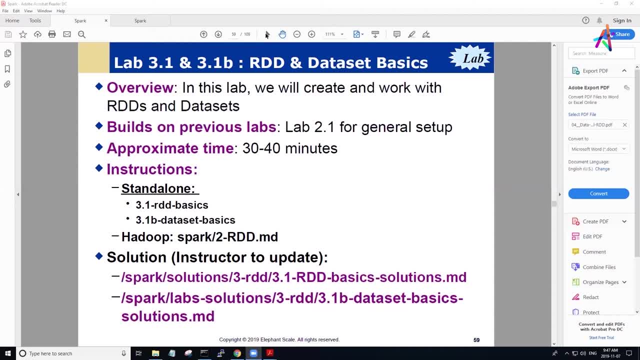 because you basically just leave the spark, the input star, so it chooses whatever is available and you just basically assume that two is a proper number. okay, so four cores are available. uh, then it assumes two is the proper number. and what i'm asking? what sort of mechanism is behind? 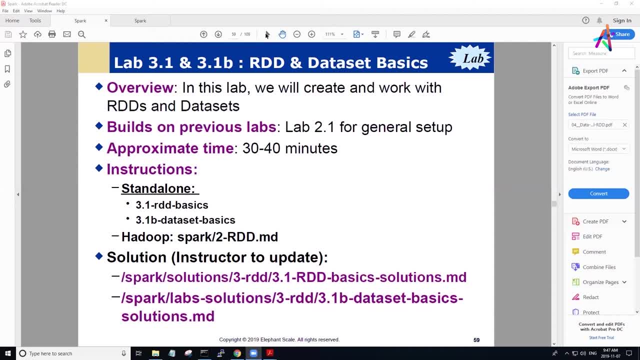 this because maybe that the partition is it's choosing doesn't have four. you can't have four partitions, so you have only the possibility to have just two partitions. well, there are four lines, so, like we might do, and there are four lines and i guess two and i guess two are the same, 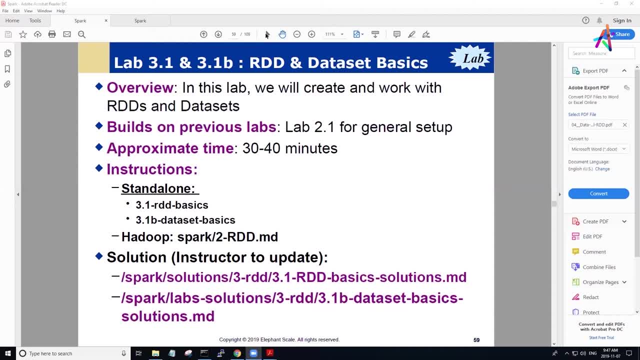 uh two contains: well, at the time you execute the counts, um, the spark doesn't know, right, no, no, but when you load- no, that's the thing- when you load the file, you load the file because of the count at that moment. but that's the thing. it doesn't do anything. have you tried to check the ui before? if you load the? 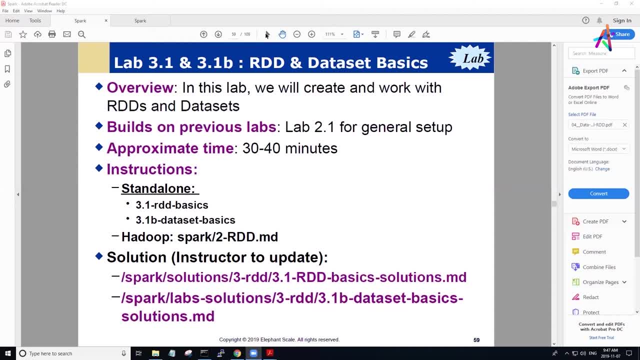 file. it refers to you, right? nothing happens. the thing happens only when you do this. i understand that. um, let me just do this. yeah, there's something like that. yeah, you will have to like: i haven't executed any account or anything, and already i am seeing two partitions here, and if i execute, 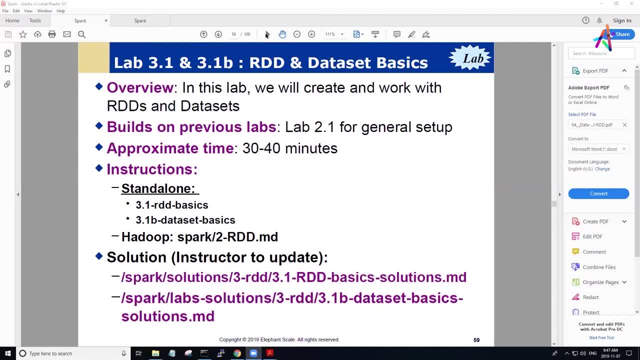 accounts, then i will see where do you do? i don't see two partitions, so there's this one you can see. so you get those partitions, yeah. get them partitioned, yeah. okay, interestingly, what you do is 500 megabytes. you get immediately 16. only will be loaded, so 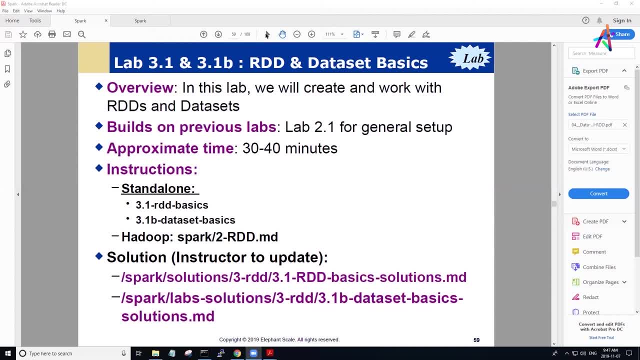 so to me this is unexpected. i would either expect one partition, because this is one file, or four partitions, because they have four cores exactly. so the question is: why? why two partitions? why spark is doing that. no, but that i think when you're running count, for example, will it create four partitions. 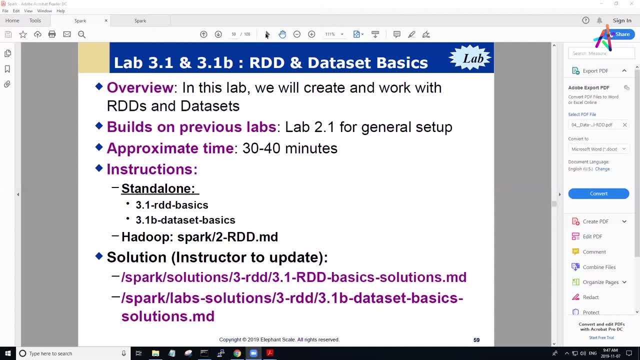 so what? what i saw is: um, just by defining the rdb uh from the info file and for executing any action, before running any action and then when i actually run the action and see the the outcome in the ui, i actually need two tasks and then i can execute it right. 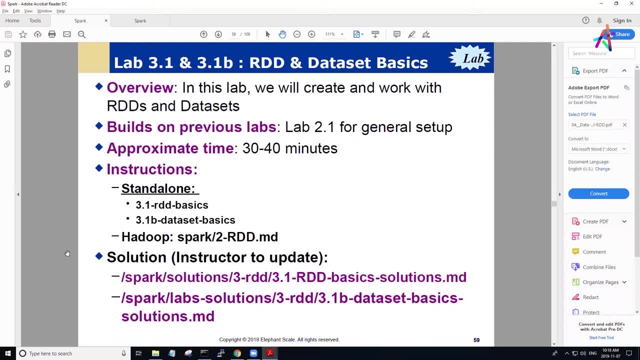 uh, rob, hello, are you here? yes, i am good. my question is: uh, is where, uh, what is free one b file? because, um, i'm looking at it and it looks a lot like free one without b. oh yeah, i think there might be some differences there in in just the interface, um. 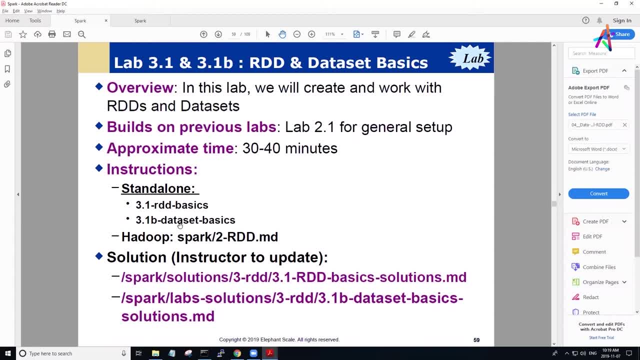 uh, again, i haven't had a chance to go through all of these files. i've been trying to to struggle with that um, so i think, without even looking at it, the probable difference is that there's a spark context, probably like an sc in 3.1, and an actual thing called spark and 3.1 b. do you see that? i'll. 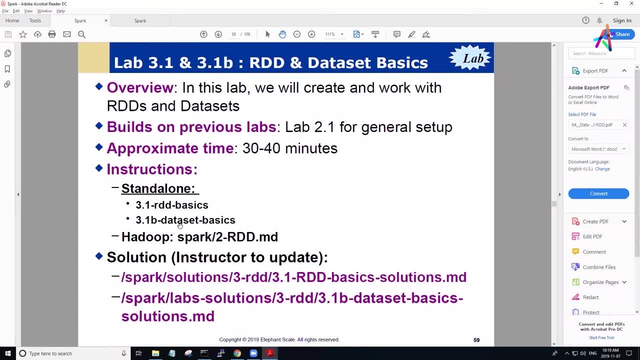 have to take a look. yeah, okay, so what that is is that it is the. that's the difference between the older version of, between the older version of spark and the unified um version. so almost everything is the same, except that spark object that's created in the b file, because that's the. 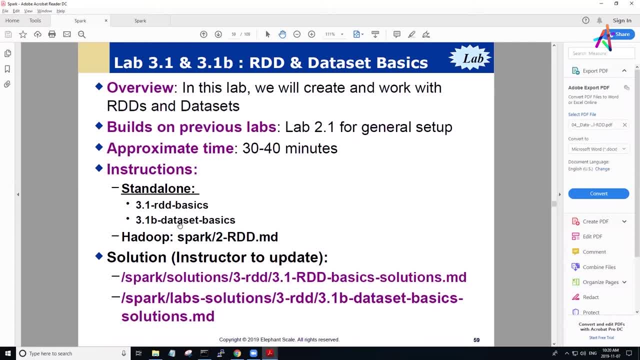 new unified interface to both data sets and five fields. but you i have a clue in here about the and foundation in this field. the friction interface p is the learn, looking at form and the encompassing, and to both data sets and RDDs. So SC is just the interface to a context. 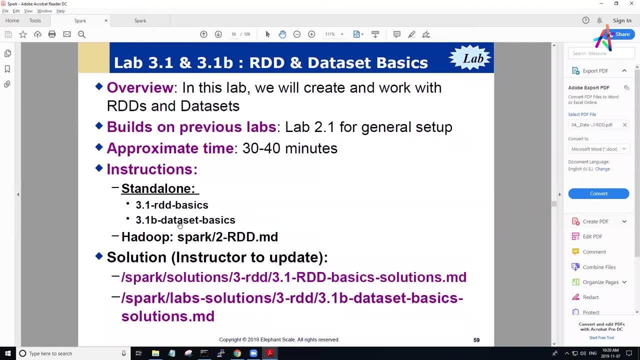 that just gives you an interface to RDDs. Spark gives you a unified interface. Does that answer your question? I will go through 3.1 or 3.1b. Yeah, yeah, and so the difference- I think believe the two of them- is just that they are. 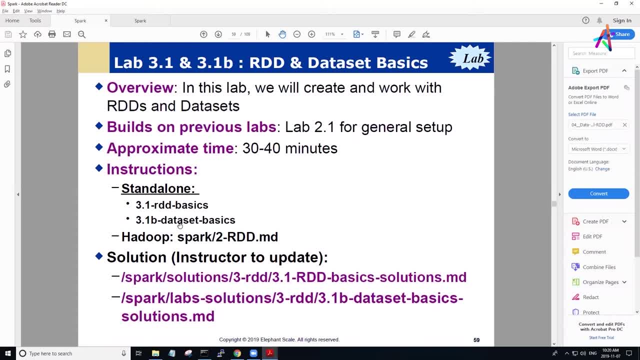 they're different in the and I haven't taken a good look at them. I'm still trying to sort all this stuff out. The difference is probably just that you're using a different interface And other than that, there should be a lot of similar things. 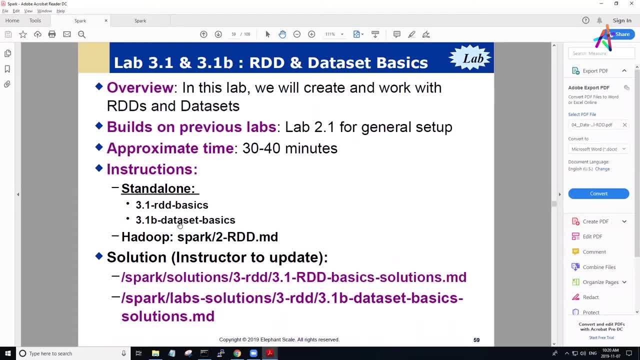 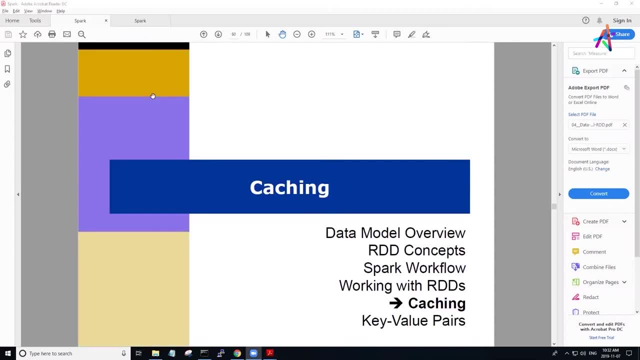 Okay, so it's not a continuation, it's not a No, I don't. I think it's again just a matter of using the different interface. Okay, got it All right. I have put in a query as to where the solutions are. 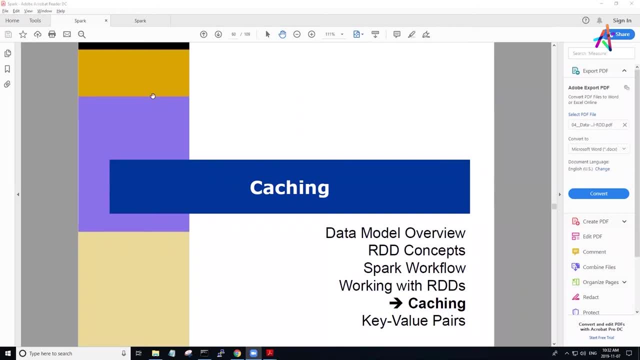 so I can share those with you. Now, how did the labs go? Is everybody having everybody doing okay? I said I checked in on that. Okay Are doing fine, yes, Okay, do you need some more time or do you want to carry on with this? 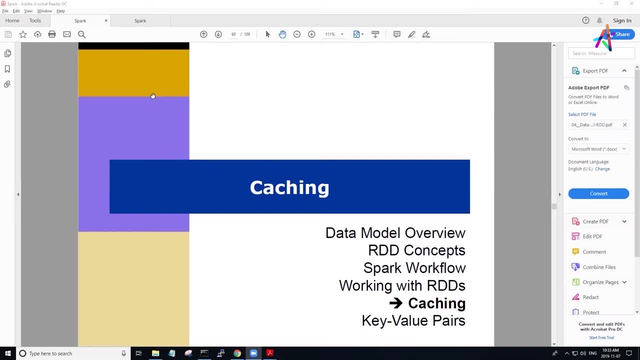 It's up to you guys. You're the ones that are taking the course. I would like to ask a question, if that's okay. Yes, of course. So when processing a text file and just doing some simple filters and counts? 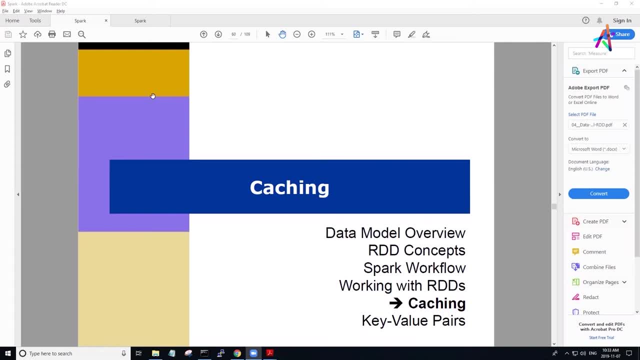 so there's this 100 megabyte file and there is one one gigabyte file, right? So as examples, we have this 10x difference. Now, when executing the same job, the same filter and counts, I see that there is not 10x difference in runtime. 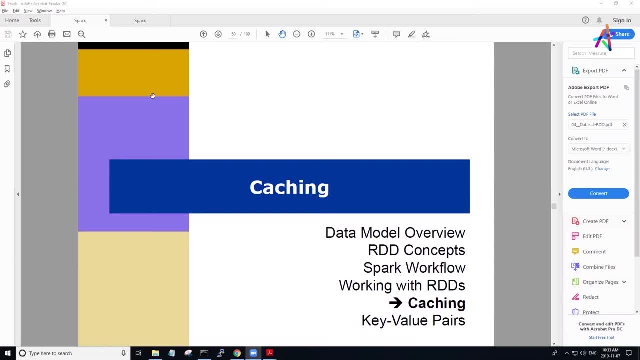 but there is a much higher difference. So the one gigabyte file takes much, much longer and I was wondering why is this happening? Which is the file that takes longer? So there's the 100 megabyte one and the one gigabyte one. 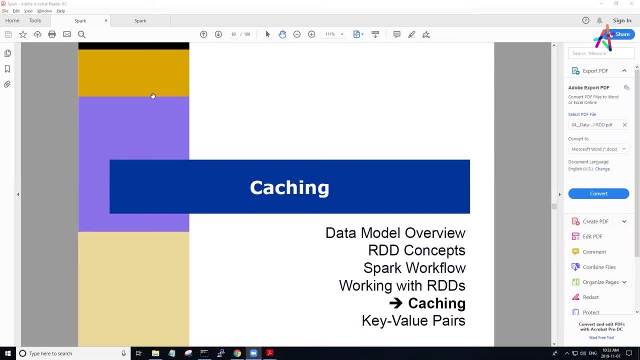 So I'm just comparing the runtime on both and even though the difference in size is 10x, the difference in runtime is closer to 100x. So why this difference? It's probably because you are running it in, you're not running it on a cluster. 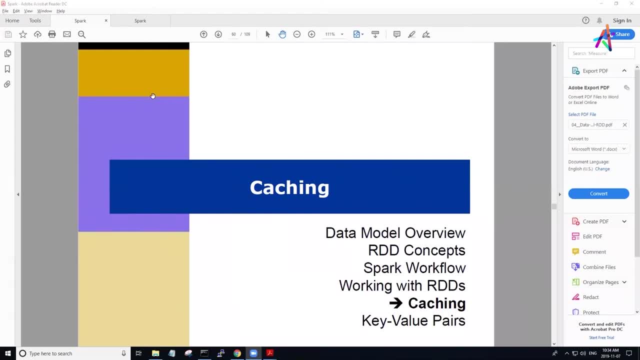 so there's a lot of memory issues going on there, Okay. so I suspect that there's probably a lot of disk reads and writings going on there, okay, That's my suspicion at this point. So then, because the file is much bigger, 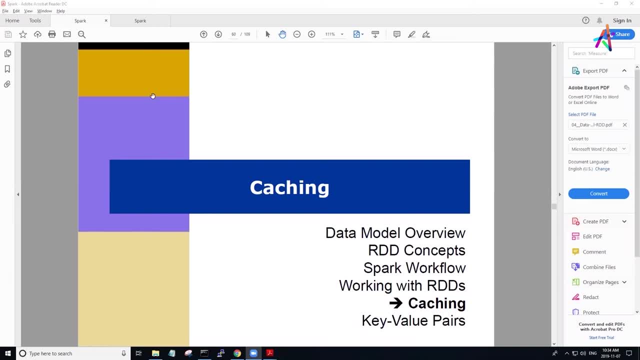 like the second one. it does not fit fully in memory and therefore there's a lot of read and writing. Yeah, there's a lot of spillage onto disk. Okay, that makes sense. And the problem with RDDs- as wonderful as they are. 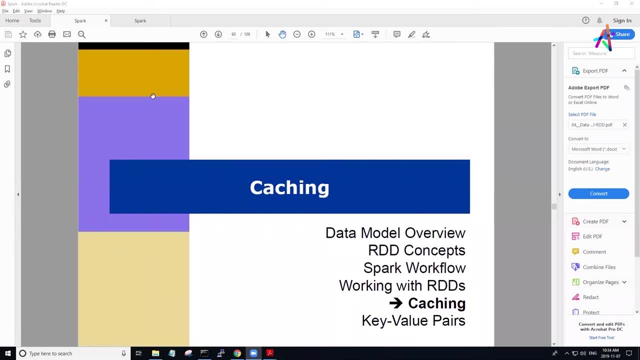 is that, again, a lot of that data is opaque, so it's not optimized when it's being spilled onto disk, and we'll talk a little bit about that. Yeah, Yeah, Yeah. So, while Spark does have a great in-memory model, 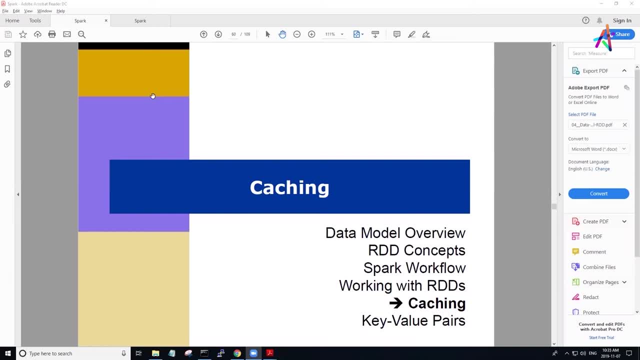 processing model. if we're generally running it in a relatively small environment, like we're doing here, when we start to get into really significantly large files, we're starting to really tax the resources, and that's where we often find that layer of clustering. 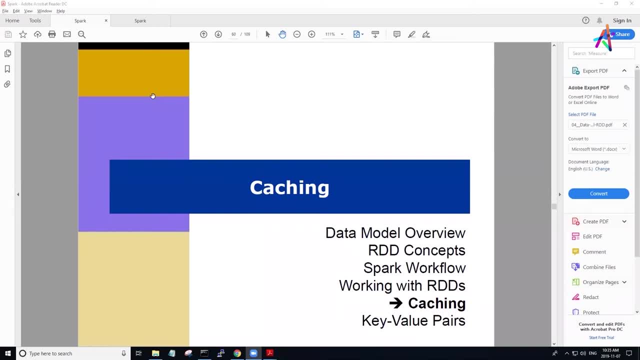 or the clustering that we use, really starts to help, because now we're spreading out the actual computational load into multiple processors with their own sets of memory, So that one file- so for example, if that one gigabyte file could- would partition up into 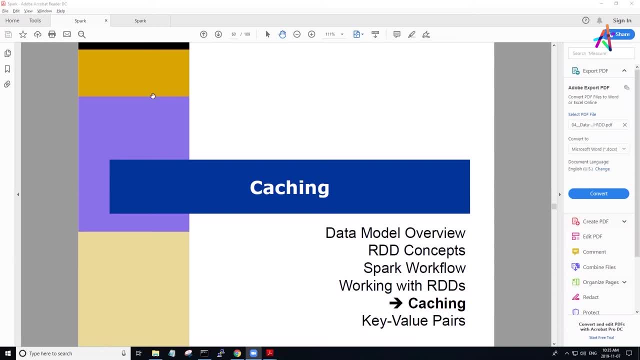 in a cluster if well. for example, if we partition up that one gigabyte file on your machine right now, I think these are all four-core machines, so you know there's sort of a physical limit there. But if we had a big cluster and we sent it out, 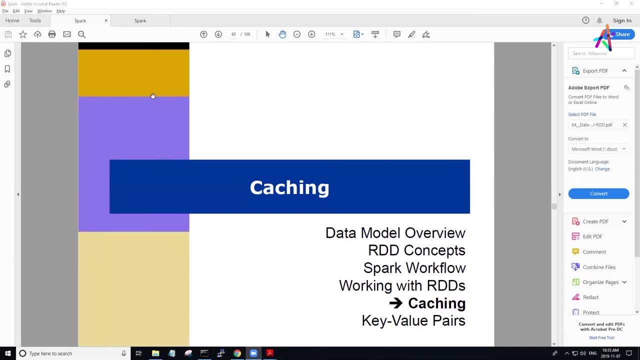 that would maybe go down into, you know, like 100 megabyte chunks onto different processors and then each one of those individual nodes would have the same performance characteristics as you would have with that 100 megabyte file on your machine. So this is an issue with scaling up. 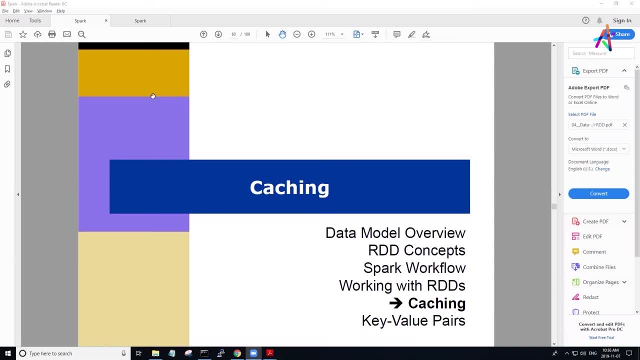 in terms of exceeding your physical resources. Does that make sense? Hmm, yes, thanks, Okay, good, Do you believe me? So far I do. I will check later. Yeah, yeah, yeah, the other thing too. 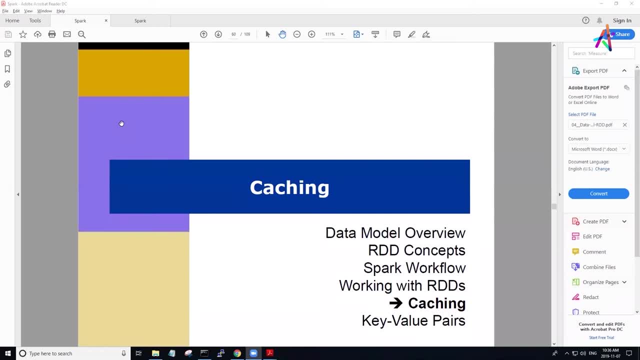 is remember is that the bottleneck for a lot of these things is just your computational horsepower and the memory that goes along that we have available to us, which is why we see increasingly movements towards GPUs and TPUs and things like that, as well as really significantly large memory models. 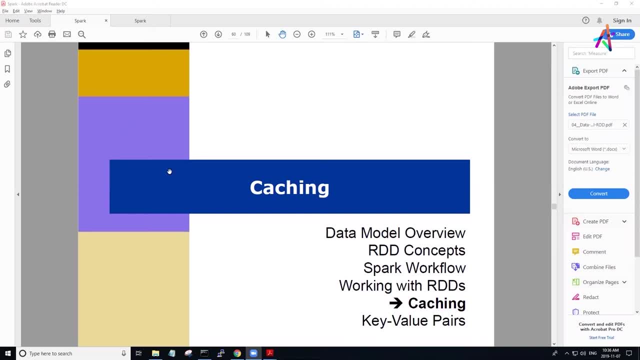 So, but you know, we all have certain limitations, so there are some things that work better from an architectural point of view. So, yeah, you are gonna see that kind of thing and I'm gonna suggest that most of that is doing to disk swapping on these machines. 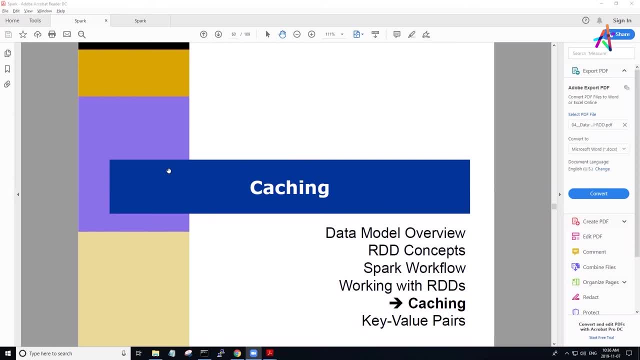 Okay, All right, So let's talk about AWS instances. I think if you ran up a larger AWS instance with maybe 16 cores and put a Houdoo cluster on there, you would see a significant drop in time. You know just, I mean really significant. 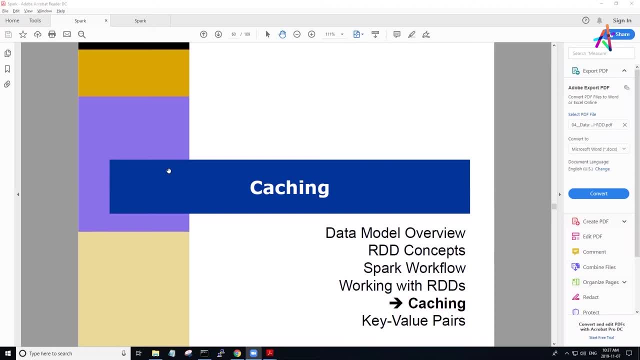 if you were able to use that cluster. But once you're done on Houdoo, you probably will see a similar drop in processing time. All right, So I just do have one announcement: I have been informed that I have to do something. 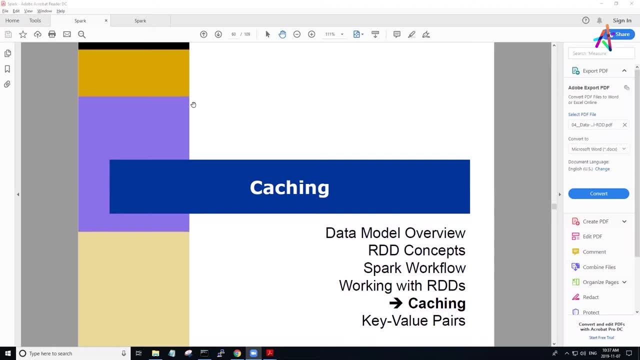 right at noon. So I am going to today only have to leave at quarter to the hour, So our class will finish about 15 minutes early. but I will make that time up by just kind of adding extra time as we go through the next few classes here and there. 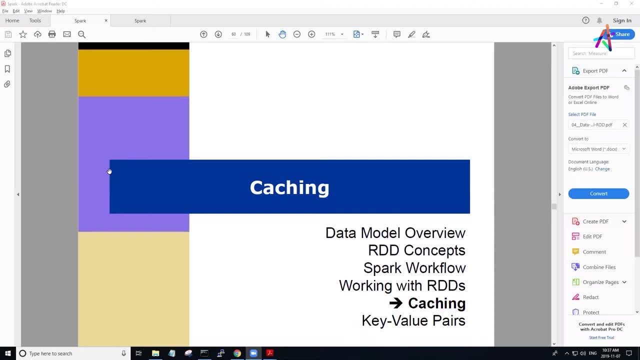 And I won't be. you know, I'll try and make up that time. Unfortunately, somebody sent me the wrong information. I'm supposed to give a lecture and they got the time wrong, So I just wasn't informed. So it'll be. that's just for today only. 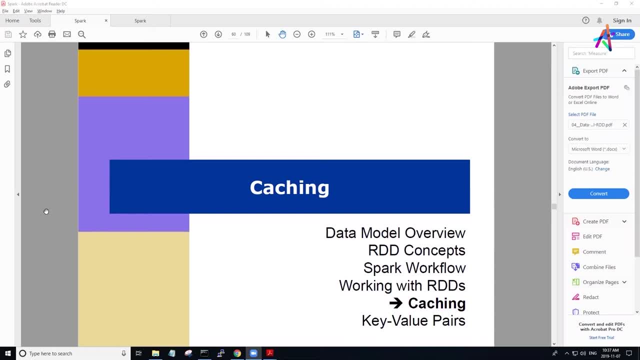 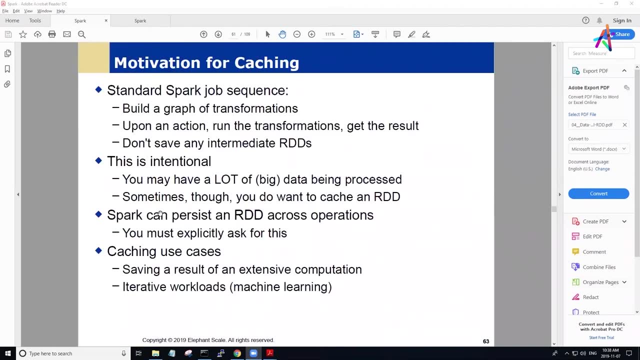 All of the other days. I'm prepared to stay as long as we need to stay. Okay, So we're going to move and talk a little bit about caching, And this is the ability to save intermediate results, because normally they are not intermediate results are not saved. 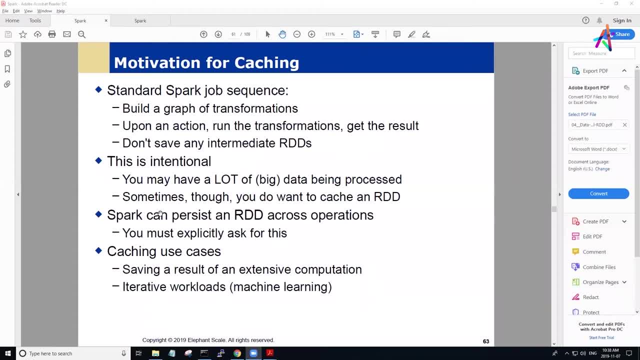 Now we looked at the acyclic graphs and we said that the graph is is built up as a work plan, a logical work plan, And then that's modified into an actual operational work plan And then, as soon as that action takes place, 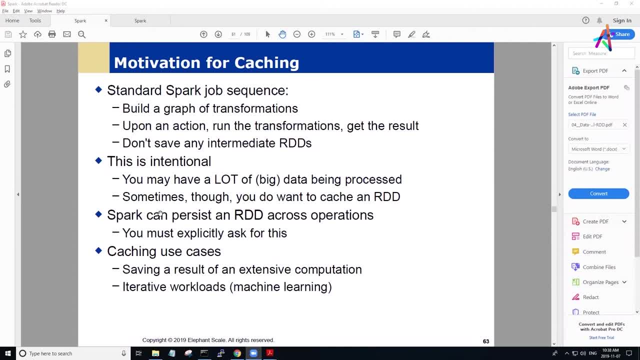 only then do we actually execute the plan, And there actually are no intermediate RDDs. So that is all a fiction that we use to think to conceptualize what's going on. Instead, the data is just processed in one big, long chunk. 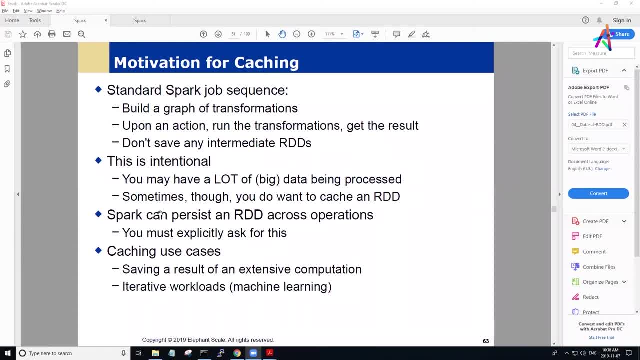 There's a series of tasks, So there is no intermediate RDD. There's a very efficient way to do the mapping. However, sometimes at certain stage in the processing we may want to save or checkpoint that results, So we are able to actually create an RDD at that point. 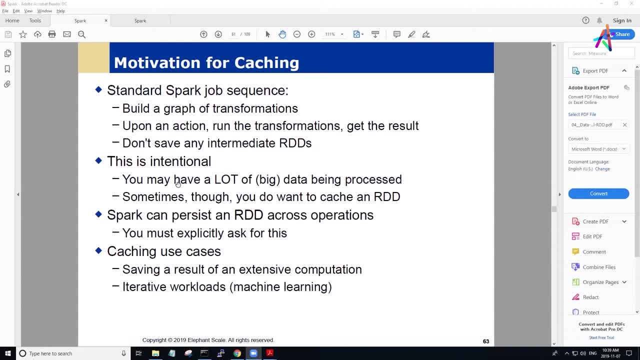 that is actually going to be there and persist. It's not just a theoretical construct. at that point We're actually able to grab it and snapshot the RDD at that point in the transformation And using that caching also is going to affect the optimization decisions that are being made by Spark. 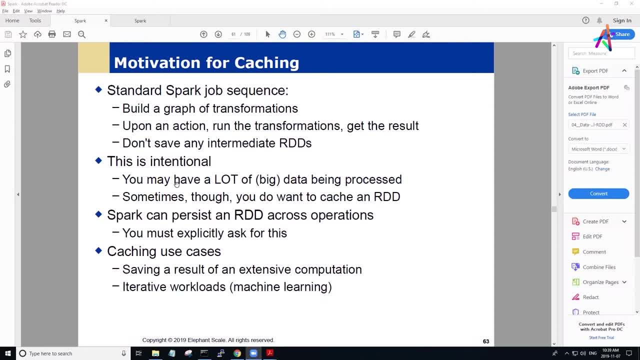 because it knows that this particular point is going to be caching out data And I couldn't tell you off the top of my head exactly what those are, but there are some there. We'll get into that a little bit later on in the class. 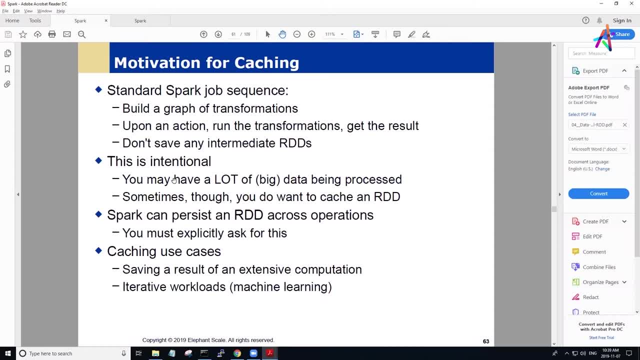 So what is the use case for this is is that we may have a particularly problematic RDD in the sense that it requires a great deal of computational power to get the raw data into a form we want, And we don't want to keep repeating that computation. 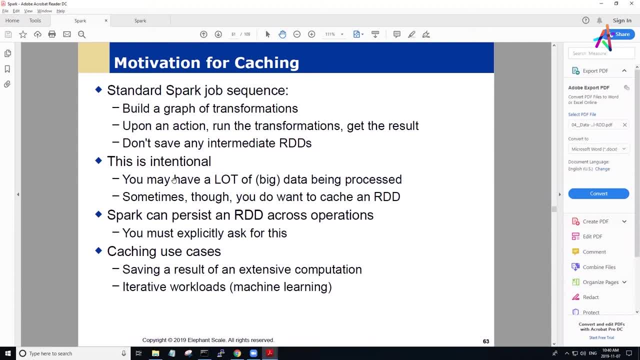 because we're then going to use that digested data in a number of different ways And we don't have to want to recompute it every time we want to use it. So we can basically put a checkpoint and say, okay, you know, save it at this point in this structure. 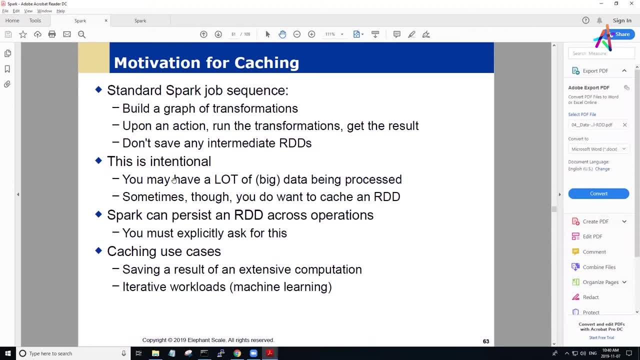 save the logical structure here so that I can pick up and use it again. So, because this is not the default behavior, those RDDs don't actually exist during computation. this checkpoints Spark to make Spark actually create the RDD in a form that can actually be persistent. 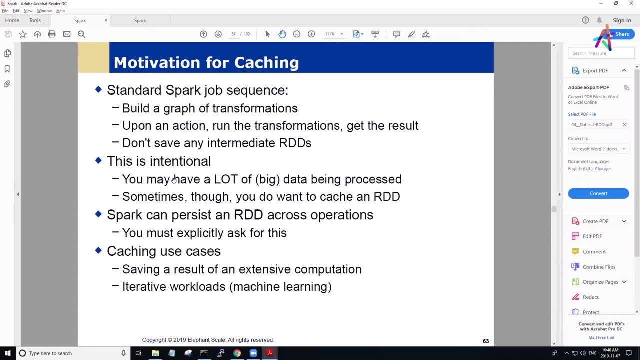 And we'll take a look on that. Okay, So the, the RDD, can persist across operations, because we're basically, like I said, putting a checkpoint in there and we may want to go back and refer to that work over and over again. 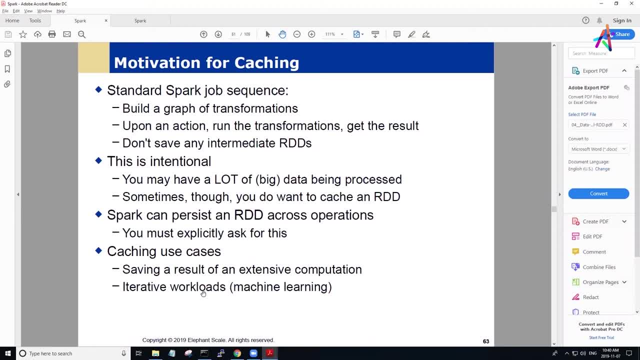 So those are the two use cases that we generally put out there. I'm going to use this intermediate result in a number of different computations going forward. I don't want to have to keep recomputing back to this point, So I'll just sort of preach it. 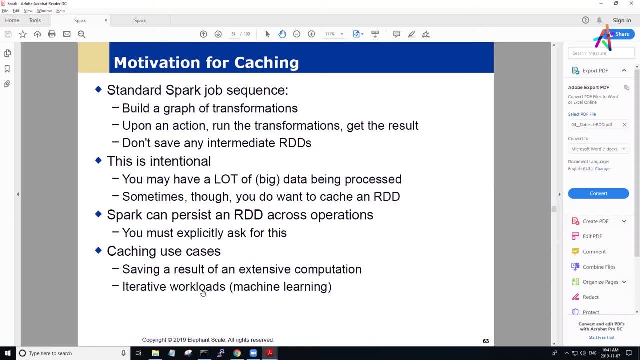 It's like it was almost like an ETL transformation getting it to this point. I want to start from this point for a lot of other work: or and or get to this point. Getting to this point is really, really expensive. 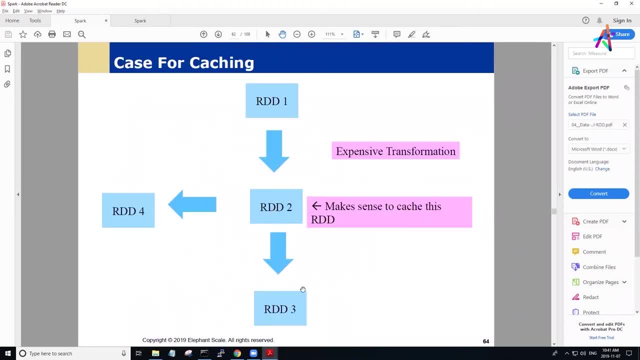 So I want- I don't want to have to do it again. Yeah, this is the the one of the use cases illustrated. I have an RDD one, I do a very expensive transformation and now I'm going to basically do two transformations. 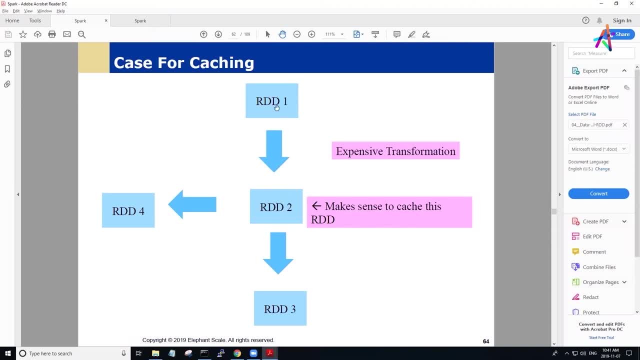 to get two different RDDs off of this one. I don't want to go through this initial step twice, So what I want to do is is basically say we've done this computation, cache this result and then proceed from there so that we can optimize and not have to to. 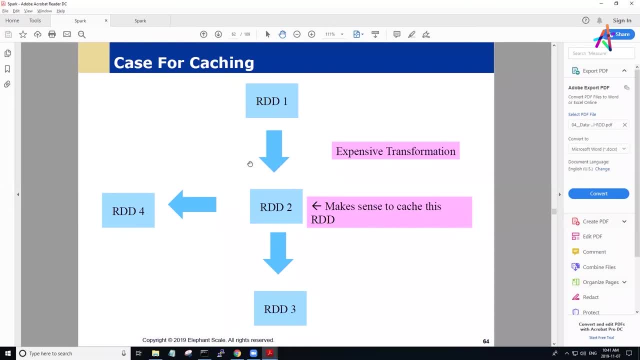 to do this again. So it is a trade-off. There's going to be a cost to this, And so we may have to make an analysis: Is it worth the cost of caching versus the work of, of, of, versus the resources that we have in the in the RDD? 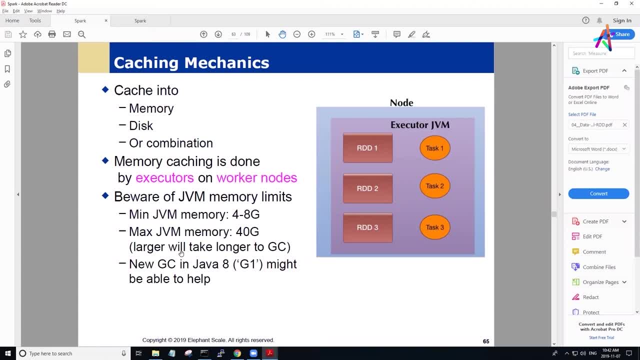 Okay, So let's take a look at how what the caching is actually doing. So we have several ways of caching disk memory or a combination, and the caching is done by the, the executors that are that are working on the on the worker nodes. 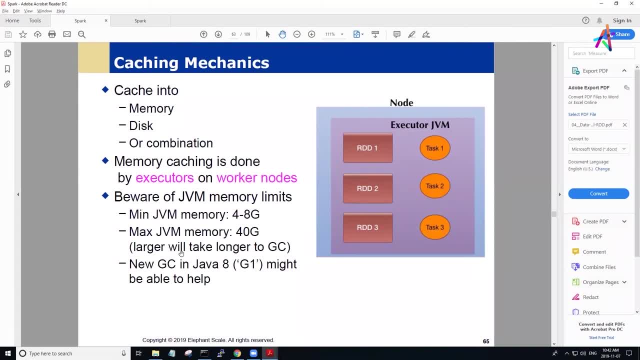 Now remember, these are all working in JVMs. So there's a JVM running there on the node, It's got a couple of RDDs that it's working on, And so we do have some limits of what we can actually put into memory. 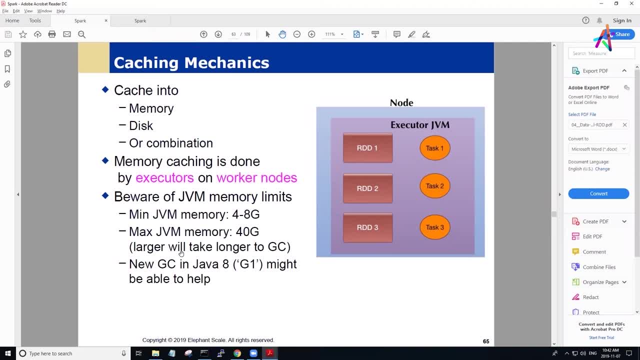 So we've got about a 40 gigabyte memory there, larger, if you've actually got that memory, I suppose The, the, the. so there's a, so there are memory limits. So once you exceed those memory limits, 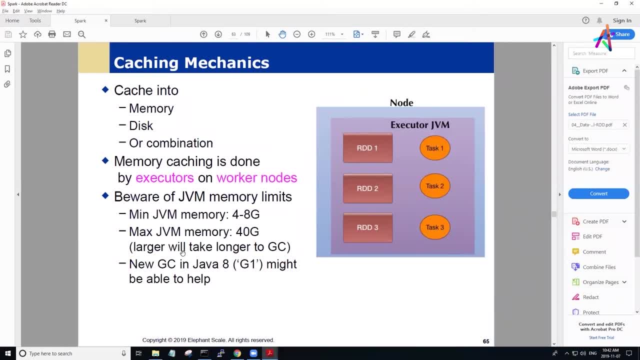 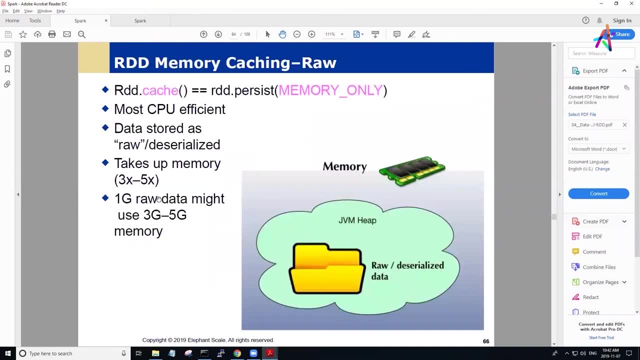 obviously you're going to have to go onto disk. Obviously, we don't have 40 gigabytes of memory, I think, on these machines. I think we've got only eight or four. So what we can do is specify that we want a persistence. 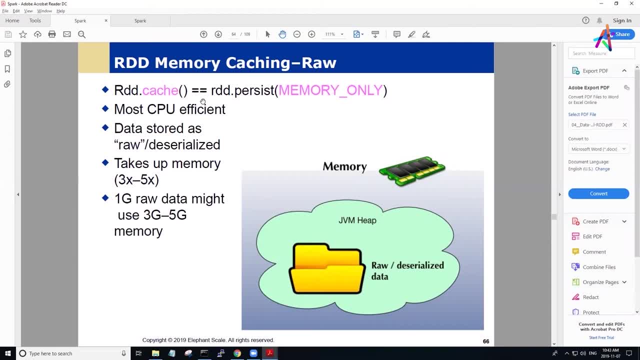 in memory only And so we can actually cache into memory And so we we can create a cache and again, most CPU efficient. Now it's most CPU efficient because it's not in, it's not intended for storage, So it's it's for stored in the form to allow low latency. 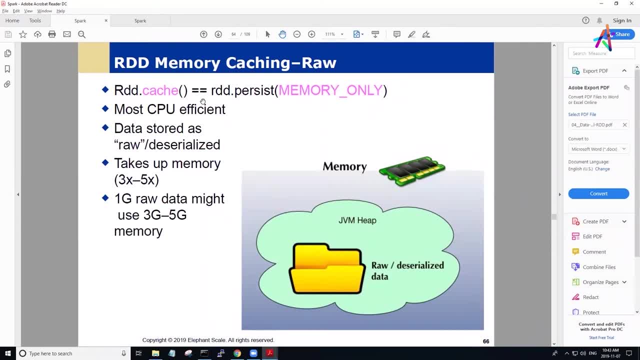 of access, And so this is the raw form. So we're not- we're not- performing any serialization on it, And when we're storing it in the raw form, that the one gigabyte of data might use three to five gigabytes of memory. 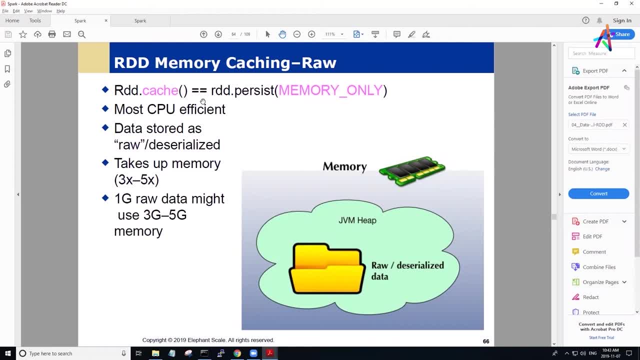 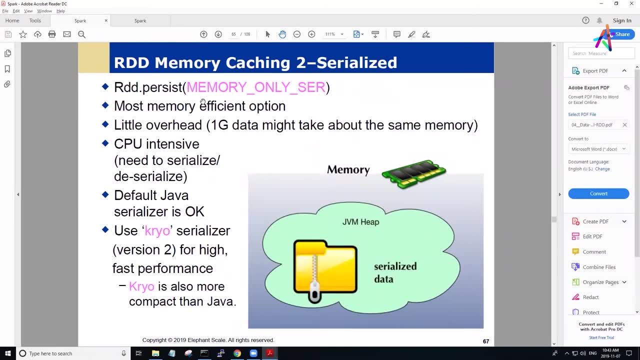 because again we're caching for low latency here. So this is- this is just something to keep in mind- The second time a cut type of caching we do as memory only serialisation. So we've got, so now we're serializing to memory globally. 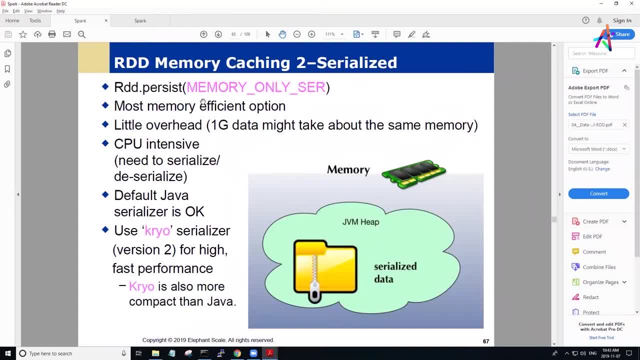 with serializing operations, writing data out the serializing operations. It is a trade-off between performance and memory again. So now we're saving on memory but again we've got computational costs because we're serializing and deserializing. Java serializer is okay. 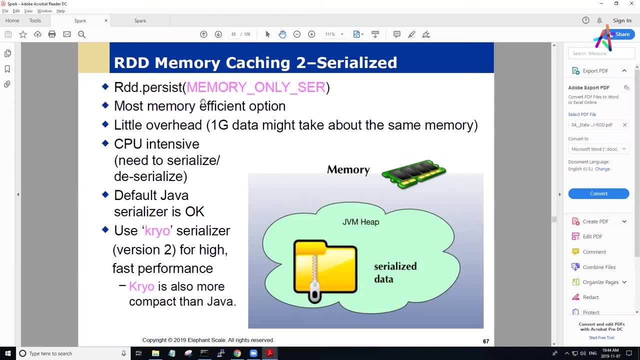 It's not that expensive. but we have another Creo serializer which is high-fast, performance, more compact than Java, And later on in the class I think we come back- we'll take a look at the Creo serializer. So already we're seeing that in caching and memory. 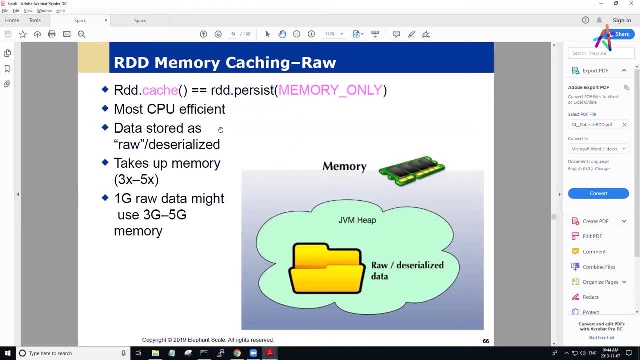 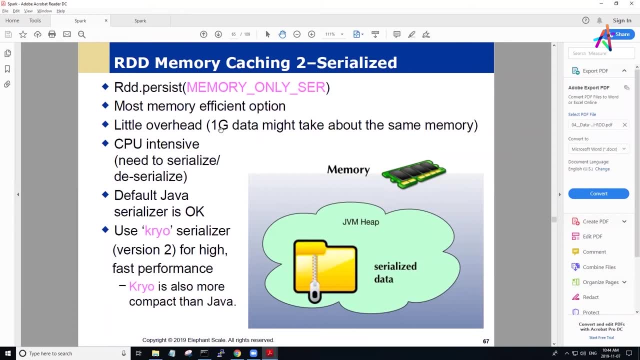 the two options we've got are to cache in a raw form, which gives us a pretty good latency. But if we want to save on memory, we're going to serialize, but that's going to require a latency time, as we do the serialization and deserialization. 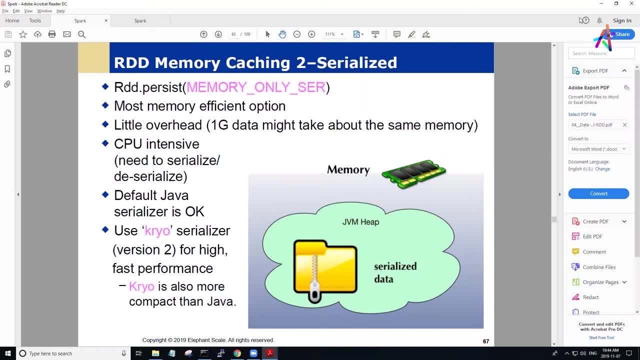 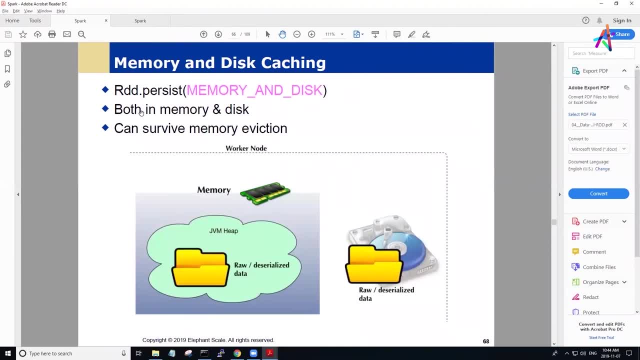 so there's some CPU intensive Hold on here. Then we have a raw form which is called memory and disk. Okay, let's talk about what memory eviction is. Memory eviction is where, for some reason, the memory that's been allocated to the storing, the RVM. 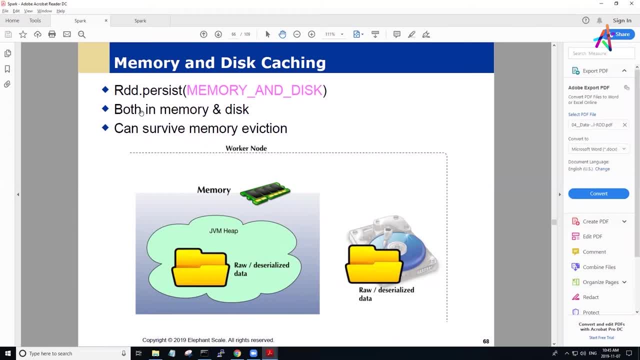 is is revoked and something else is going to take place. We're going to look at that when we get into Tungsten and how this kind of revocation and eviction takes place, But let's just say that there is the possibility. if we're doing memory only, 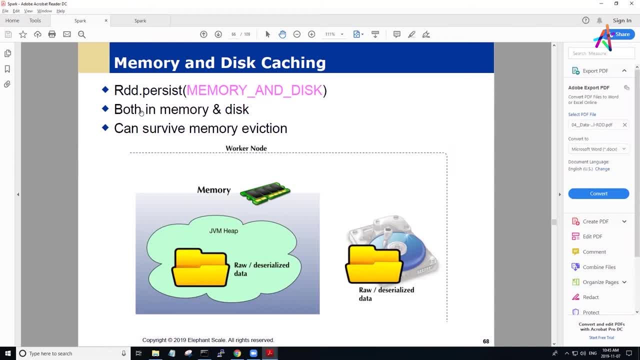 that we could suddenly find ourselves being booted out of memory and our serialized RDD will not be there. So what we can do is if we want durability. so notice that so far, we're now looking at another model, which is where we're actually going to store in memory. 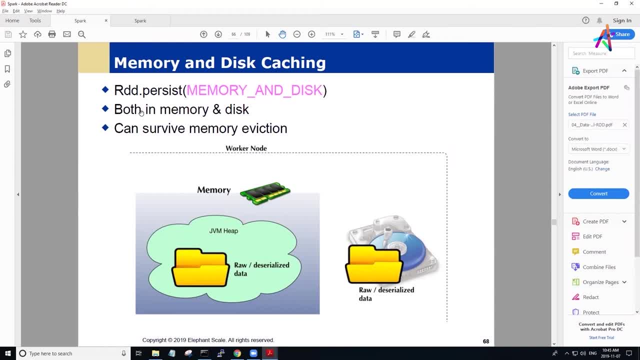 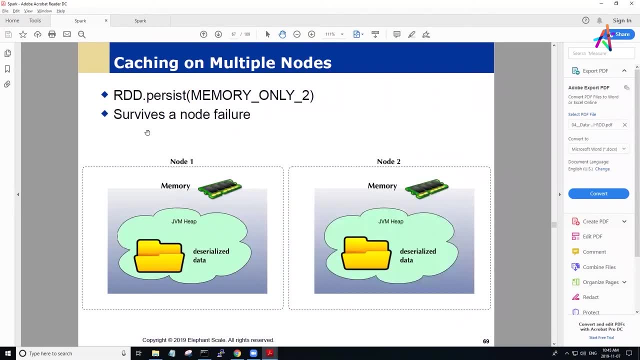 and we can. we can page it out to disk. So even if the memory is evicted, we're going to be able to still have it based on the disk or copy. So there's a couple of other sorts of things that we can do. 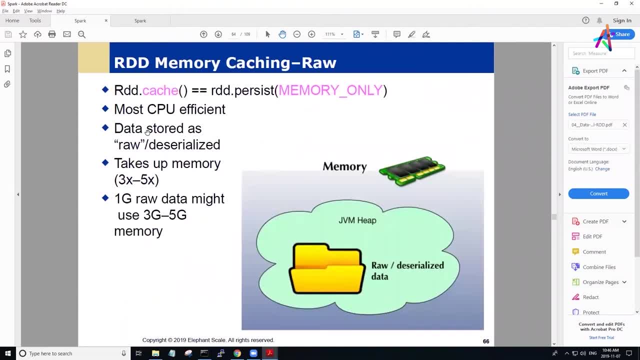 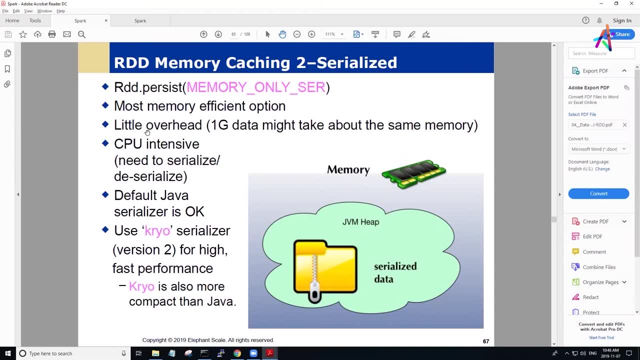 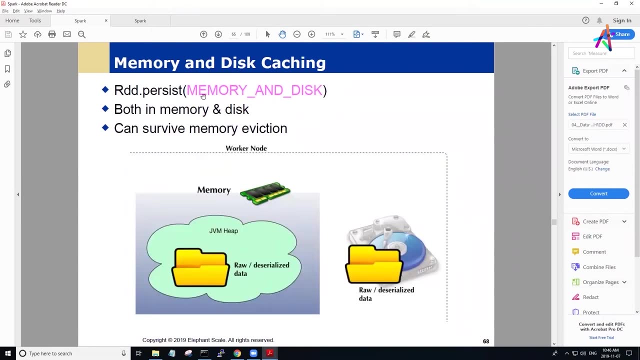 We can persist. So this is so notice, this is caching and this is persisting. In other words, we're, we're, we're. we're basically getting some slightly different accommodations here. So here's persisting with memory and disk. 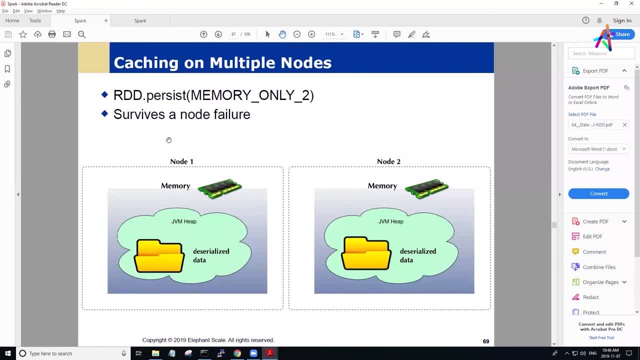 We saw that before. Here's a persisting with only memory two. So we're okay. Persisting memory two, so we have a node failure. So what's happening is again we're getting replication taking place. So numbers of ways to persist. 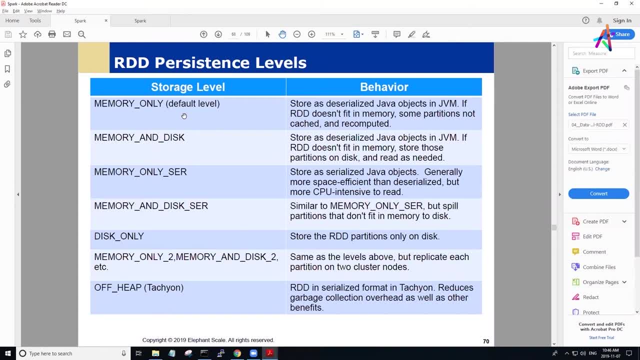 So let's take a look at sort of the persistence levels that we've got here. So we've got a memory only. So it's we've got deserialized Java objects. If it doesn't fit into memory, some partitions are not. 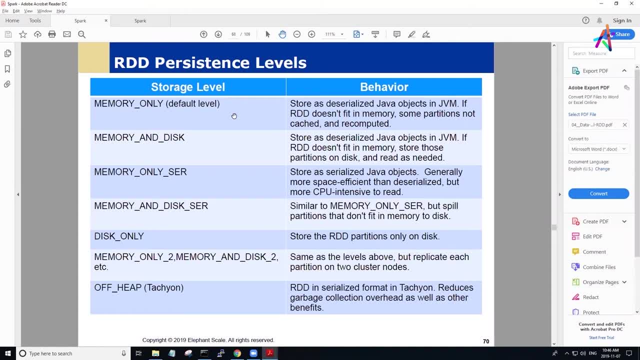 are cached and recomputed. So, in other words, if it doesn't fit into memory, it's not that we're going to lose the data, It's just the stuff that doesn't fit into memory we're going to have to rebuild. 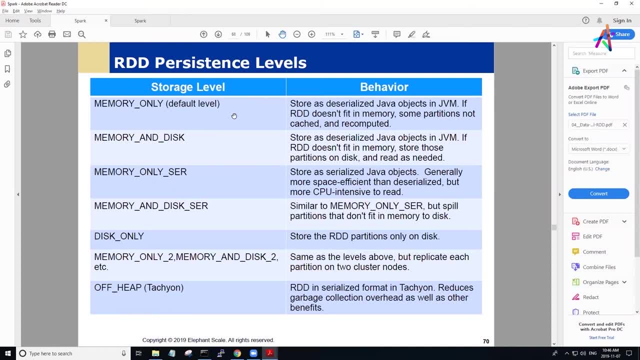 So you know that may not be optimal from our point of view. Memory or disk, sort of sort of deserialized Java objects. If the RDP doesn't fit into memory, those are stored on disk and read as needed. So it's a paging scheme to page out things from memory onto disk. 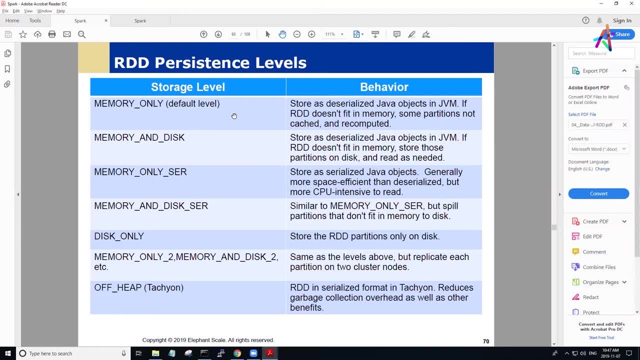 We'll get more into all of these different schemes later on too. Memory only serialization means that we're serializing as data objects And by the cache. by the way, is the just a shorthand for doing the memory only Stored as memory only serialization- stored as serialized Java objects? 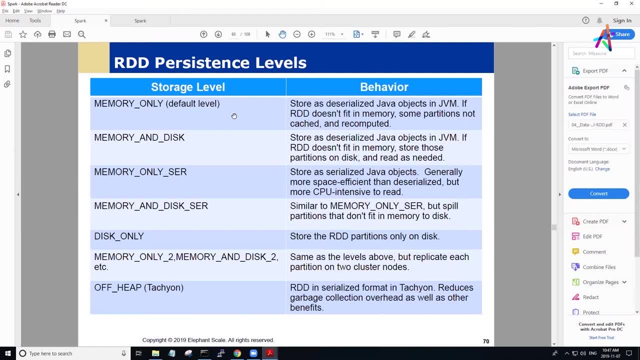 We saw that. but there's computational overhead, but better memory management. Memory and disk gives us the. it gives us the ability to page out- we call it spilling- partitions that don't fit onto disk. So you'll notice, the problem is if we don't have a disk. 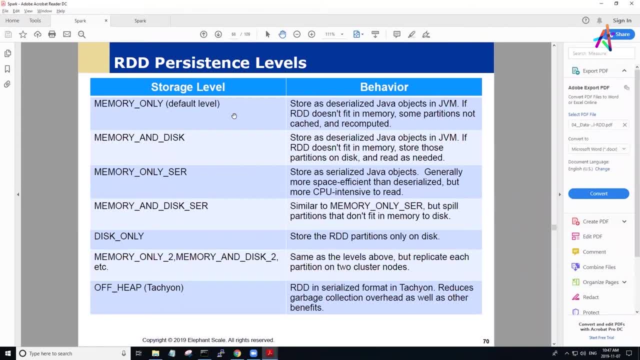 we don't have a disk model in our we don't have a disk option in our persistence. we have to recompute the stuff that doesn't fit into memory. This actually goes and pages it out into disk. So again there's another computation we have to think about. 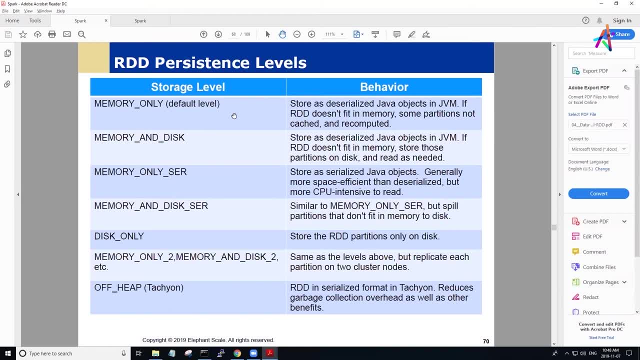 is which, from my point of view, is going to be more effective. If I have a really, really expensive computation, I'm going to start paging it out to disk. On the other hand, if I have a real bottleneck with performance and disk IO. 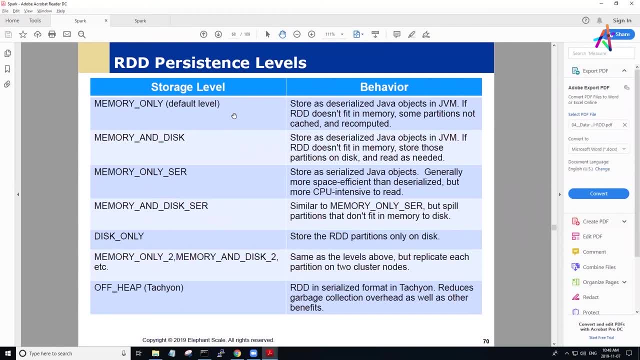 I may wind up thinking about: gee, it might just be faster just to rebuild the thing. So disk only is. we're going to sort the partitions only on disk And we'll see if we can find a use case for that one, And then we have the memory only two, memory and disk two. 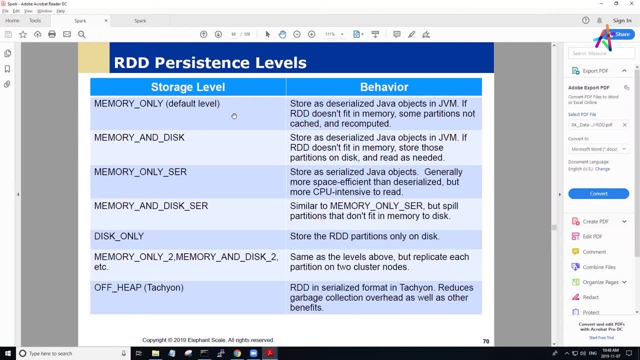 And this is where we're using the same. we're using the same clusters as before, but instead of using our redundancy failover on the same node, we're actually doing a replication scheme, so that we're replicating the partition on two cluster nodes. 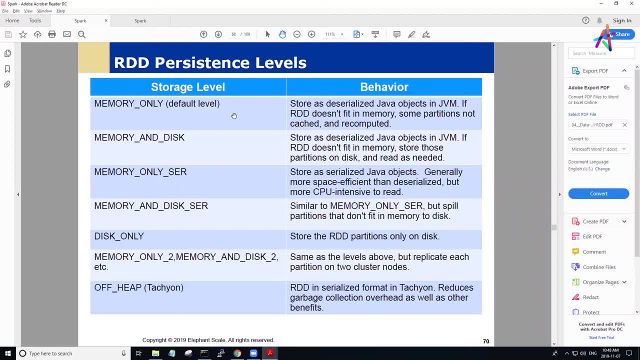 so that we can have persistence at that level. And then we're also going to look at later on off-heap, And that is a term where we're basically kind of doing direct memory manipulation, so we can even get better memory management. That's where we're getting into things like Tungsten and Tachyon. 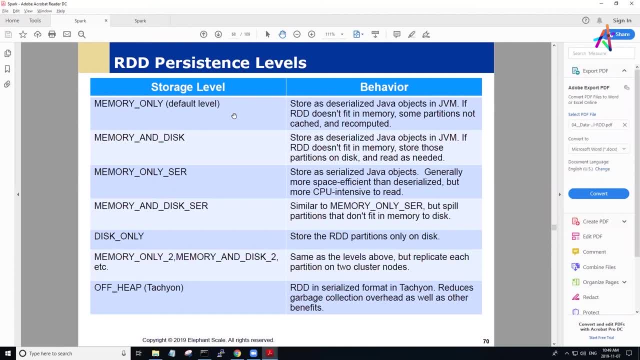 Some of the other things. Tachyon is the serializer, Tungsten is the memory management tool. So obviously, if we're putting everything in memory as a memory only model, then we're going to have to really really be concerned about how we're managing memory. 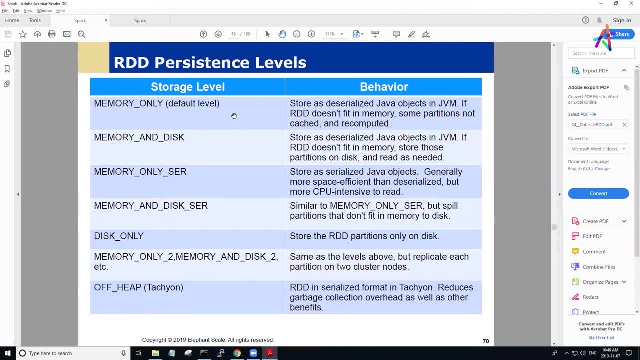 Did things fit into memory? What is my persistence model? What kind of failure can I encounter with my data when I run out of memory? What are the kinds of things that or if I get evicted from memory? what are the kinds of things I have to be concerned about? 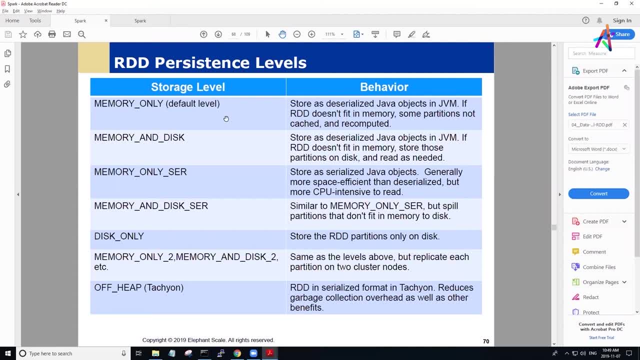 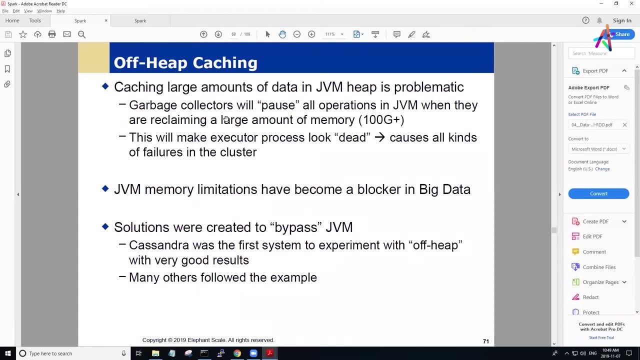 So all of that will come into play as we do our planning for these persistence levels. So I had mentioned off-heap caching, And so what off-heap does is tweak the JVM memory model. So when we put large amounts of memory on a JVM heap, 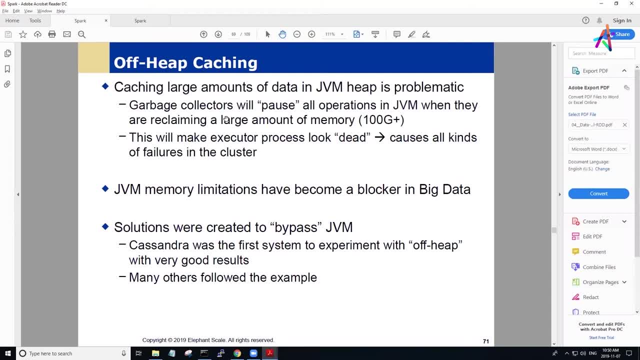 then the good old Java virtual machine garbage collector will go and do cleanup for us on a regular basis. So the problem is that we do not necessarily want this program running because we don't need the functionality it provides. So what we want to do is to say: well, how can we free up all this memory? 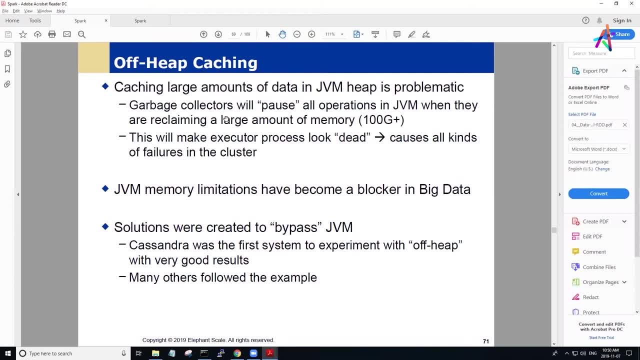 and tell the JVM just basically to keep its hands off our memory management. So what the off-heap memory does is: it bypasses a lot of these mechanisms And allows us to manipulate the heap memory in a way that's very similar to how C works with memory. 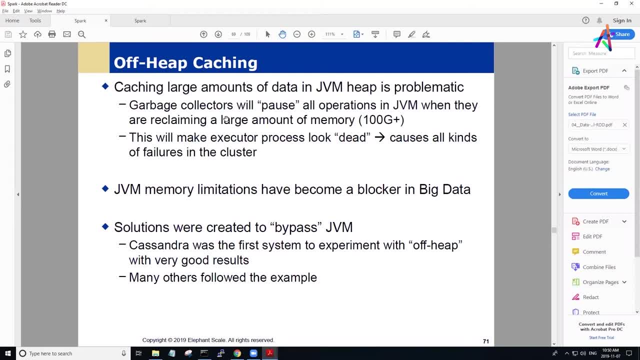 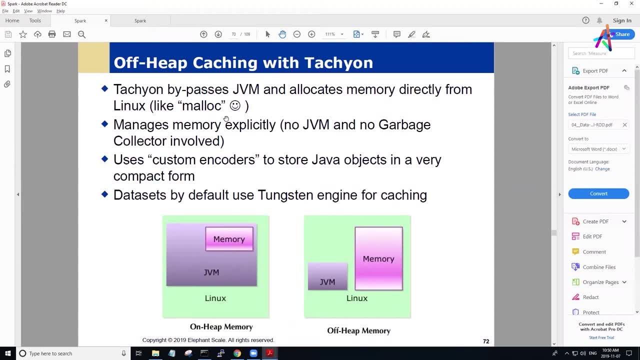 So Cassandra was one of the first systems to experiment with this, And there's a number of others And we're going to be looking at that as well. So Tachyon is an example of that, where we're basically allocating memory directly. So, in other words, if we look at the JVM standard memory model, 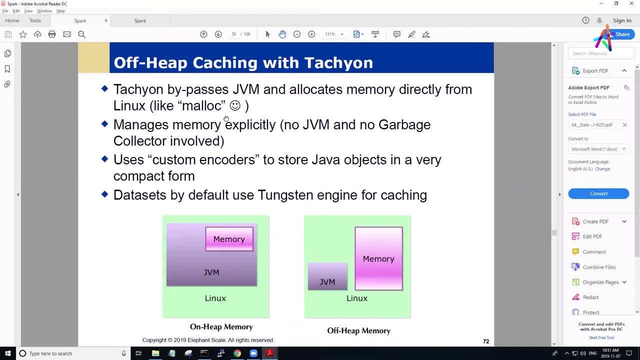 it is using the on-heap memory which is in the JVM, And anything that's not in the JVM, that's managed in the JVM, is going to be inaccessible. But the problem is once we put it in the JVM and manage it there. 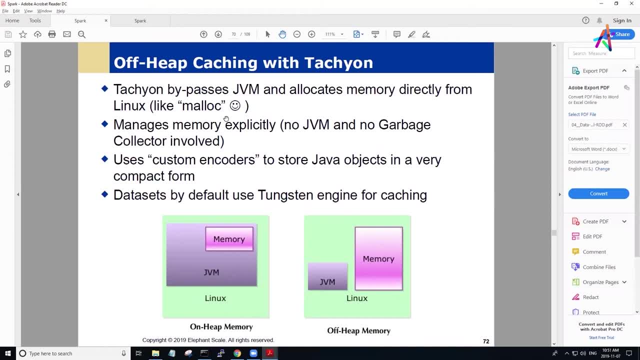 we've got all of this kind of overhead that's taking place like the garbage collector. So if we go back to C, what C does is it actually gets memory directly from the hardware using malloc. If you have never used C in malloc to memory, you've never lived dangerously. 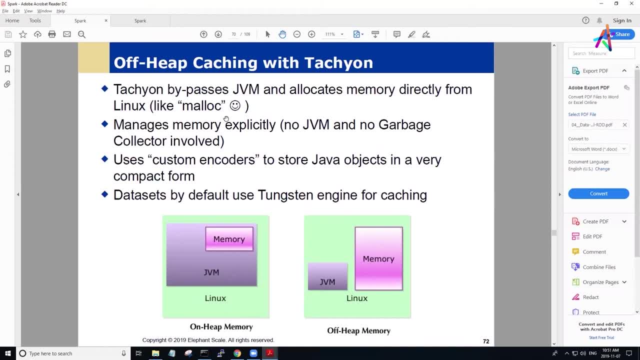 It's a thrilling experience. We used to malloc stuff all the time because that's all we could do to get memory. I have a question- Sorry, I have a question about the memory that you can use from the Linux system or whatever underlying system it is using. 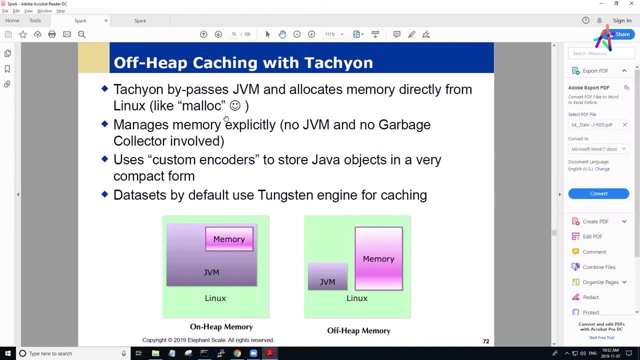 Is there a limitation on how much memory it can use? Because potentially, if you want to store something, if it's something too big, you kind of like blow up your cluster because the thing is like in the other scenario: you just blow up the executor, the executor dies. 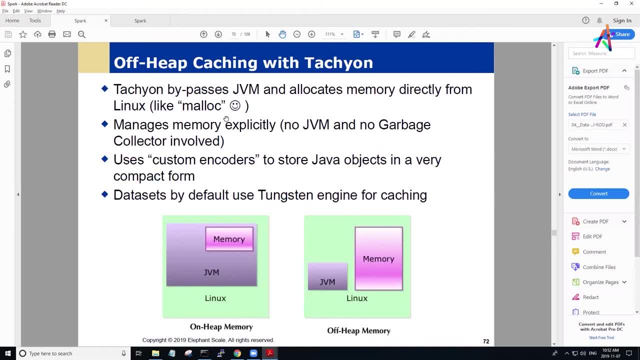 Whereas in this scenario you just want another one, But in that case you might completely destroy the node, right? Yeah, and I think you can tune the parameters for that. I can't tell you right off the top of my head. 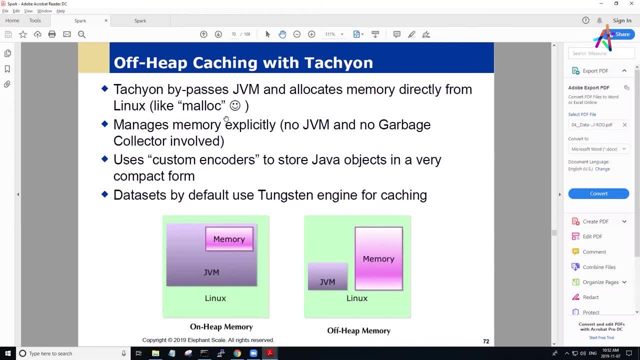 but I think there are some guidelines as to what you can access and what you can't access, And we'll get into that in the tungsten model in particular, which deals with those kinds of issues, And the memory that it actually uses is also split up into different areas. 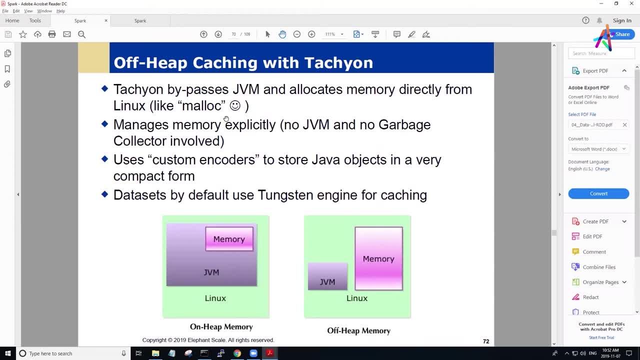 And there's a whole lot of memory management issues, So we will circle back to that when we talk about tungsten and address those kinds of issues. okay, Okay, thanks, All right. Okay, so the basic concept of offheap is: don't use memory allocation through the JVM. 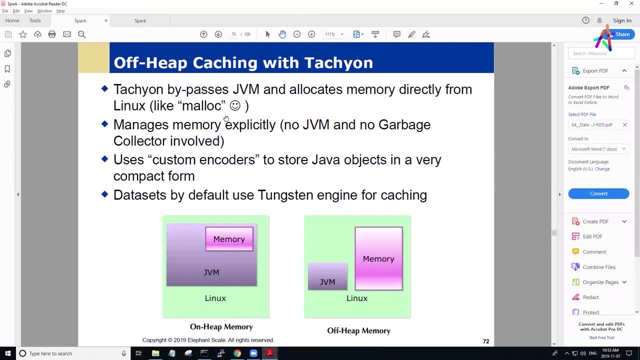 Just go outside JVM And manipulate the memory directly on the host node. Okay, so this is a really good solution. It gives us lots of more power in terms of being able to access the memory. Plus, we're not running all these processes that actually interfere with our computation. 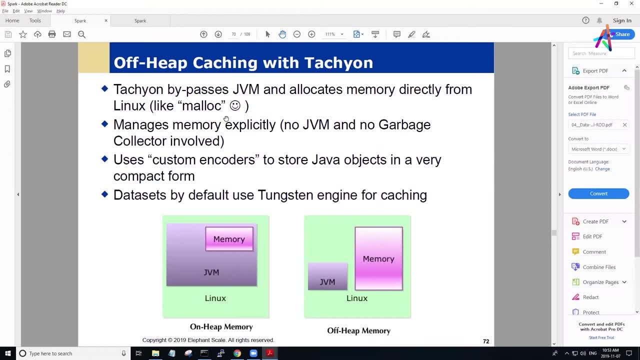 So, if you can see from the diagram, we're basically getting memory. that's outside the JVM And we also want to do. since we're now outside the JVM, we can also use what we call custom encoders And we can basically do very, very tight storage of the objects and serialization. 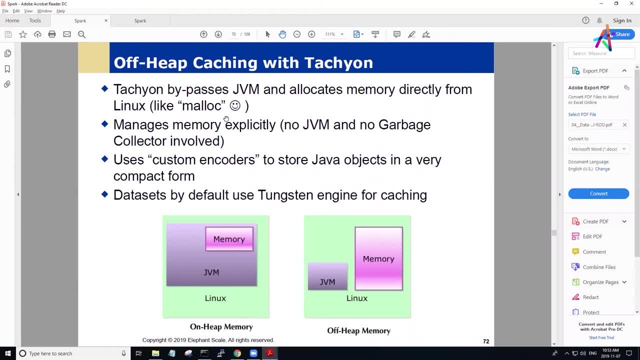 which gives us even better utilization of the memory that's there. So this all is managed through the tungsten engine, which is the standard way to do it now. So we have a big section on tungsten later on in the class, So we'll get into it and explore it. 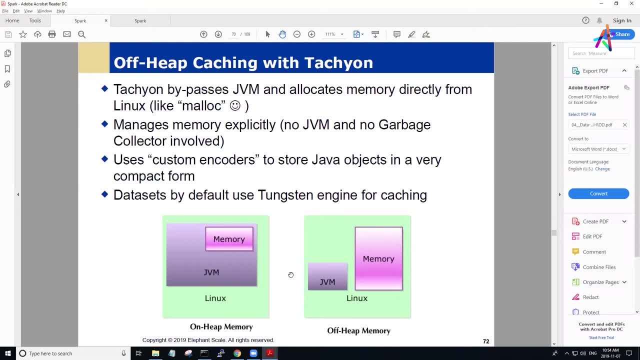 But at this point, all we want to understand is what is this? off memory or offheap caching? And basically, in a nutshell, it's the ability to bypass the JVM memory management and manage memory directly through the use of tools like tungsten. 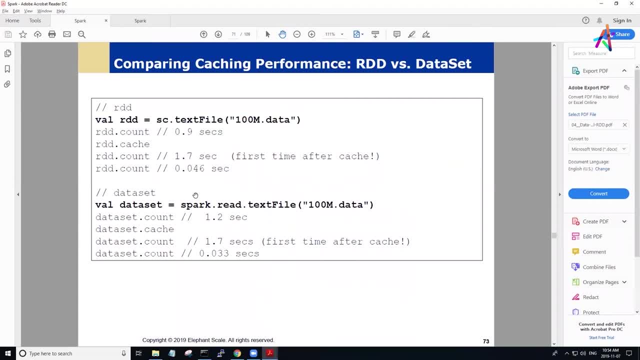 Okay, So one of the things that I was going to say. by the way, a couple of people asked me what was the difference between those two lab files, And I didn't look at them, but I have a suspicion that this was actually the kind of difference that we look at. 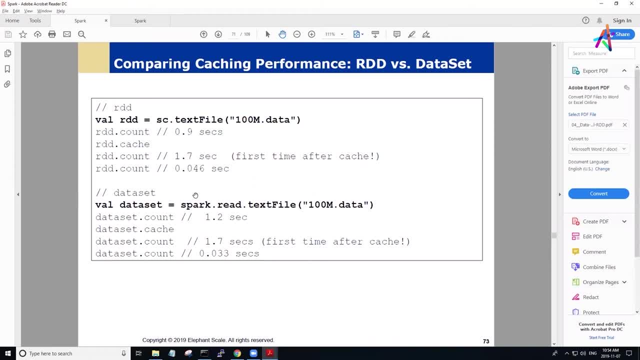 So the first one is a standard RDD. Now the SC dot is the interface to the original, the original SPARC, one point, whatever it was before they had datasets. So this is the called, this is the SPARC context, And it produces RDSs or RDDs. sorry, 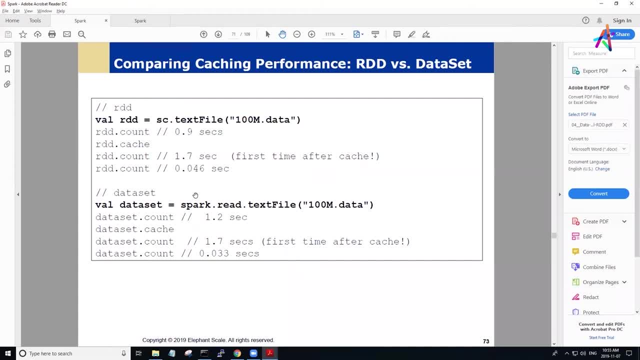 And if we take a look at the count running count on this: if we count it's 0.9, we cache it and count that it's 1.7 seconds after the first cache And then we count it again as 0.4.. 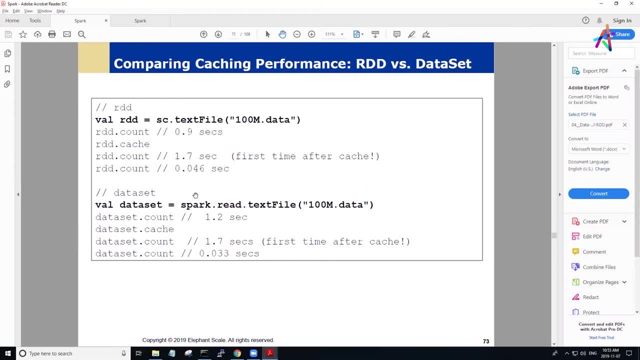 0.046.. Now the second one is a dataset, And what a dataset does is it operates. it's accessed through this. the SC is gone. It's actually been incorporated into this, So the dataset is going to read the text file. 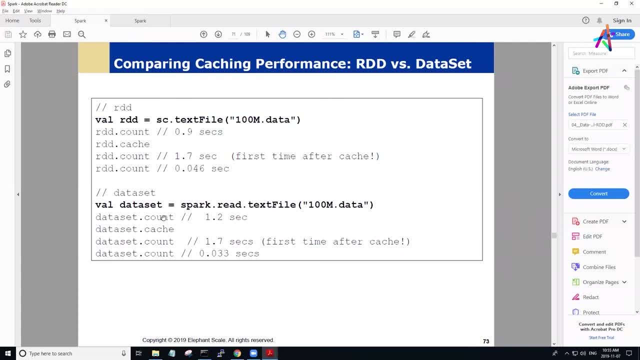 And you're going to see, it's going to take a little bit longer to count it. In this particular case, cache it. But when we cache it the count generally tends to work the same. But then after the cache the count is a lot faster. 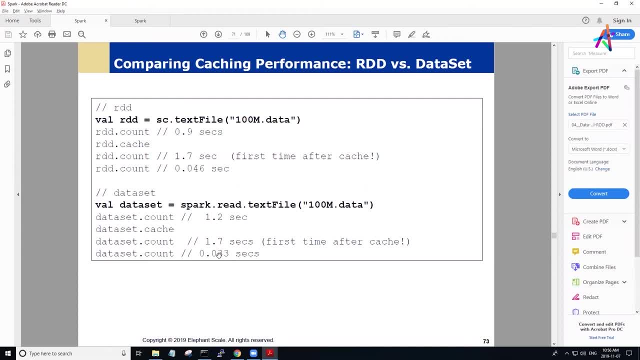 And that is because of what's happening in the, what's happening in the caching performance here. So, in other words, we're using a dataset, We're using a different kind of caching mechanism because we've got a dataset, And so we're getting a better performance. 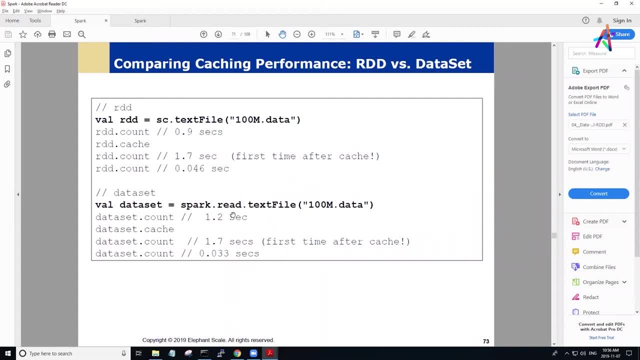 Okay. so again, we've got a little bit of a decay here And we'll start to get into looking at these kinds of stats, when we talk more about datasets, And figure out exactly what it is that's happening here, to account for some of the differences in these values. 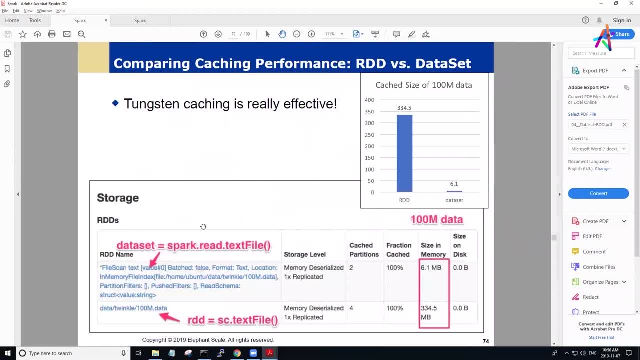 and how we're, why we're seeing the numbers we're seeing. So Tungsten is the, is the caching, And Tungsten, as you can see, take 100 megabytes of data And Tungsten uses a cache size of 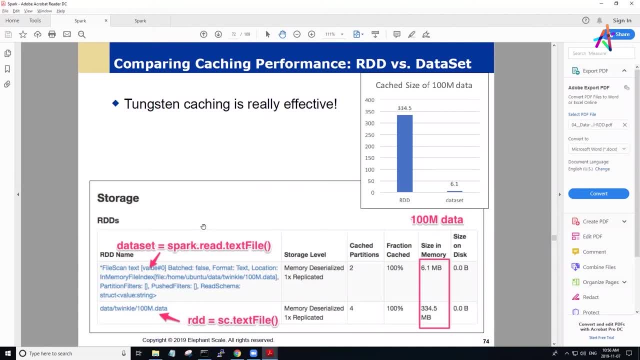 or the RDD uses a cache size of 334.5.. So I'm assuming this is all all megabytes here, or whatever. I'm not sure what that number actually is. Oh, there it is. Yes, it is So the RDD name. 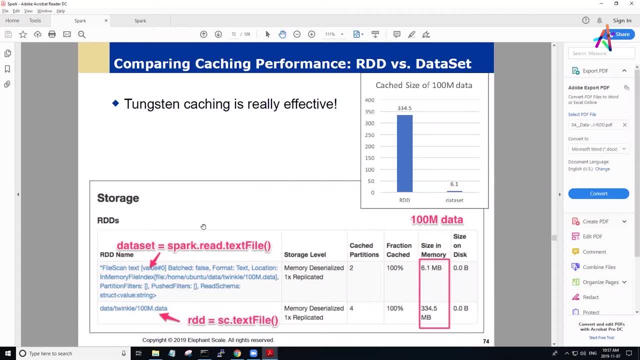 And we've also got a text file. So we've got basically the same operation taking place. We're caching the entire thing into a number of partitions, And what's happening is that the size in memory is particularly interesting. Now, why is the size in memory so different? 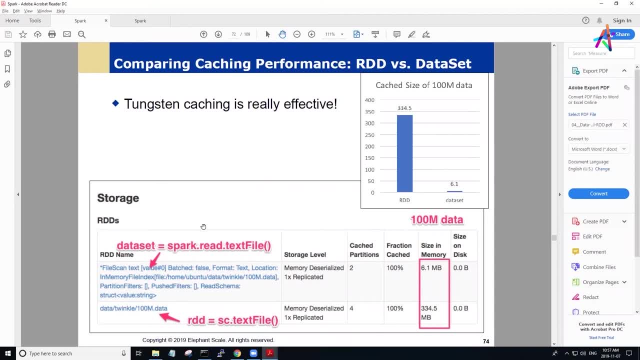 Well, one of the things is we've got a data set And so we have access to typing information, And because we've got that, we've got the ability to figure out more effective serialization. So what Tungsten actually does is it's able to go and figure that out with the data set. 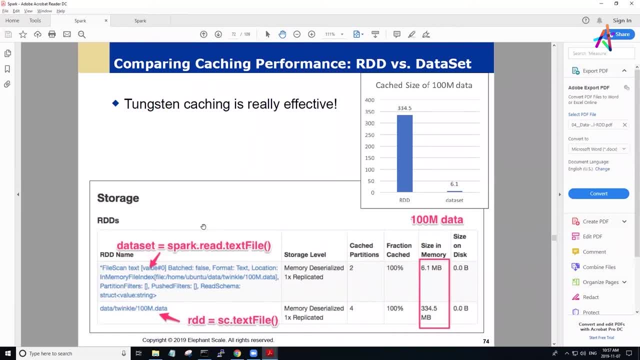 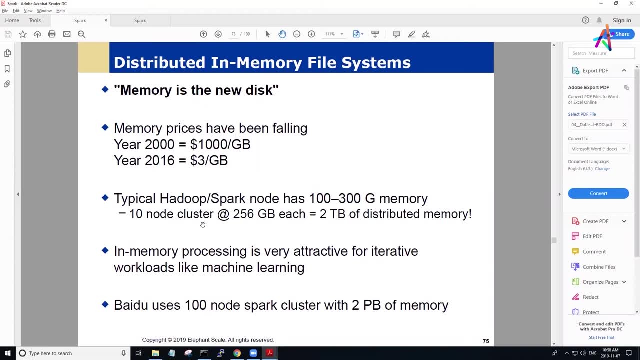 and get some very effective computations. This is one of the reasons why data sets are are so are so popular now in the Spark community. So memory is the new disk And again, I'm not sure how current this is. 2019 is probably current. So year 2000,. $1,000 per gigabyte, New disk: $3 per gigabyte. I'm not sure what they're measuring there in terms of what dollars, But anyway the So we generally can look up to about two terabytes. 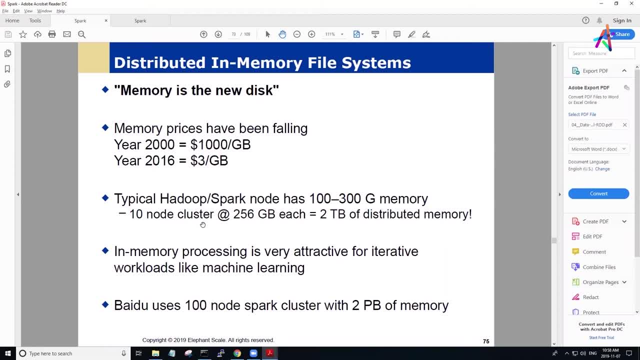 of distributed, distributed memory on a typical cluster, And so, because of that, because of the low cost of memory computation or the low cost of memory, it's starting to become more and more attractive to be able to add more and more memory. 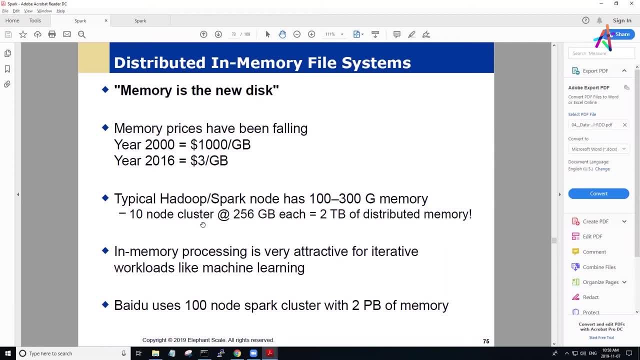 to do more and more memory in in, more and more processing in memory. So when I first started actually doing data analytics back in the 1980s, I had like a megahertz processor. I had one. I had one of them. 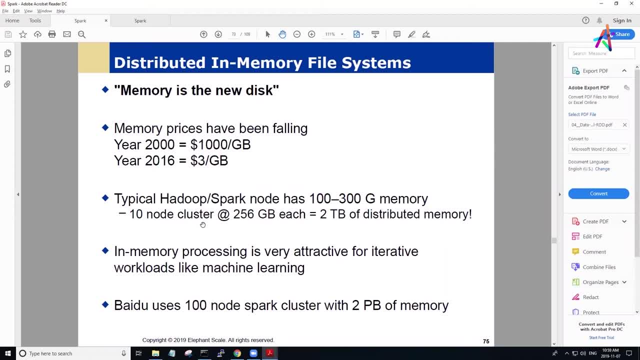 And I got a $10,000 disk drive which had almost 350 megabytes on it and weighed 50 pounds, And we had to wheel it in, you know. And so a lot of what we were restricted to doing was just sheer physical resource management. 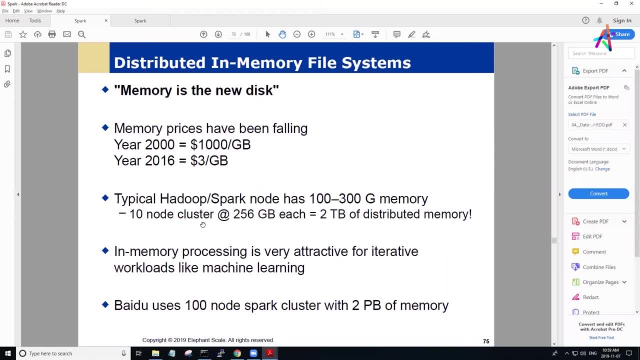 So the direction Spark is going is actually quite good because as memory prices keep falling and falling, because the Spark model is already in memory processing, we can take advantage of that And we get faster and faster kinds of computations, less and less spillage to disks. 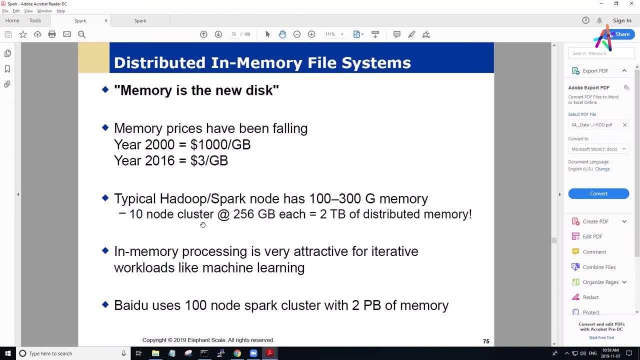 less and less need to actually store things and swap things in and out of disks. Let's also remember that Hadoop was also built at a time when we still had more expensive memory, So it might have biased some of the decisions that were made there. 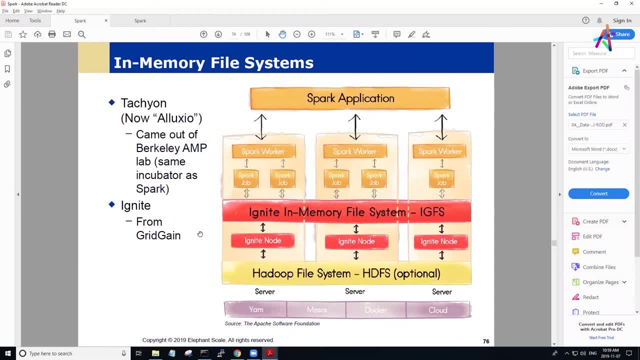 I'm not saying they did, but they just might have. So what happens is there's a lot of in-memory file systems, So Tachyon or Alexio- I don't know how to pronounce some of these things- and Ignite. 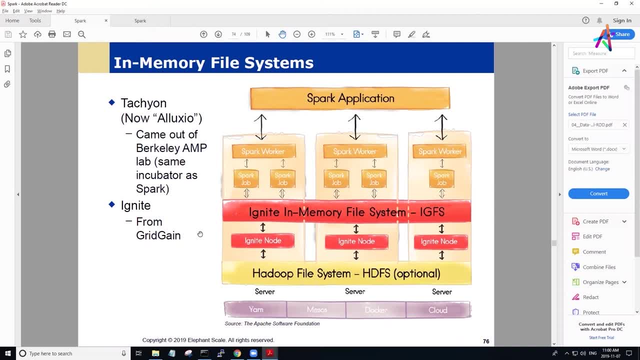 So there's a number of other things that we can basically put as layers on top of this file system. So, instead of talking to Hadoop directly, we can now basically do an in-memory file system caching, which speeds up our performance tremendously, And I do believe we'll touch on some of these things. 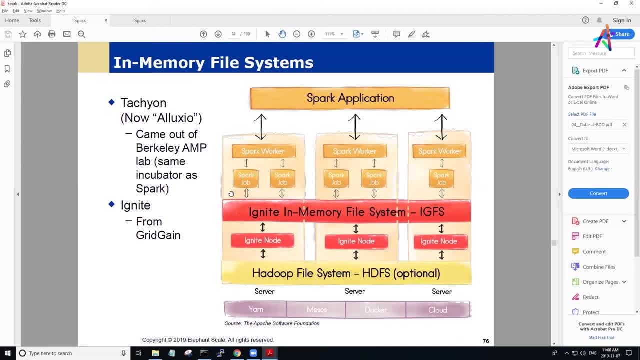 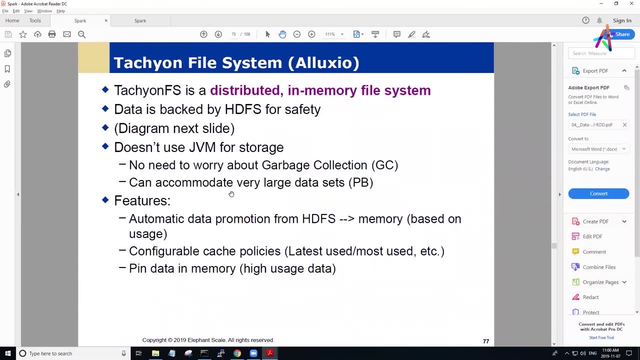 later on in the course. So we have a number of things. So we have a number of ways to continually take and leverage the increased amount of memory available per buck or per dollar for us. So Tachyon file system is one of them. 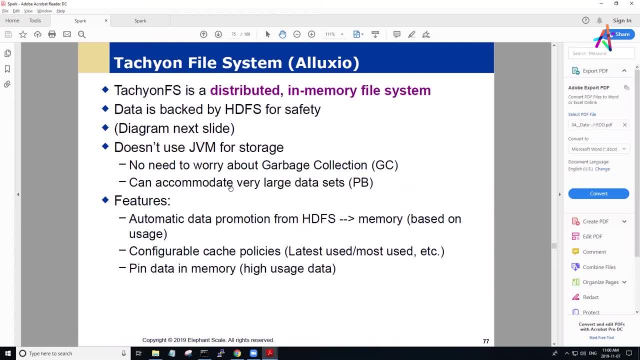 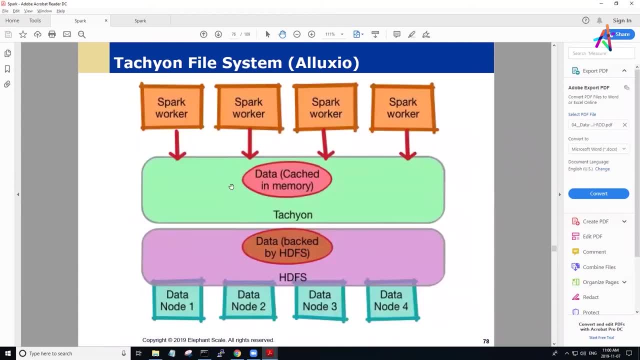 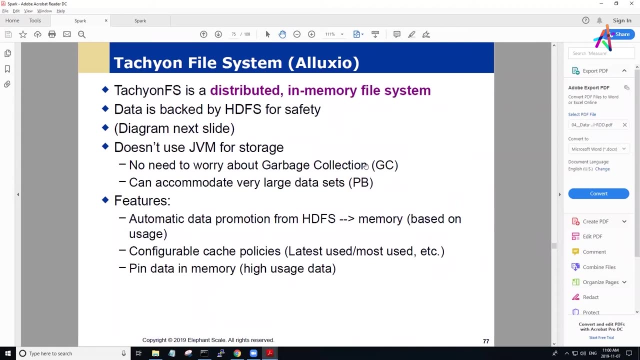 In-memory file system. it is backed by HDFS, which means that it's really a projection of HDFS. It doesn't use JVM for storage. There's the ID here. So in other words, we're bypassing JVM entirely, And so that gets us out of the garbage collection. 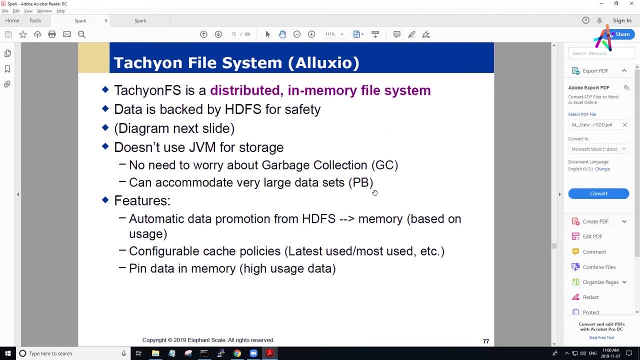 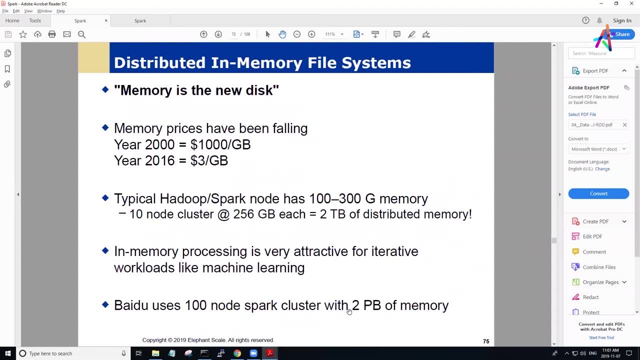 and it can accommodate very large data sets in terms of petabytes, And I think we saw something here about petabytes up there. So Baidu uses a 100-node Spark cluster with two petabytes of memory. I'm assuming that's complete. 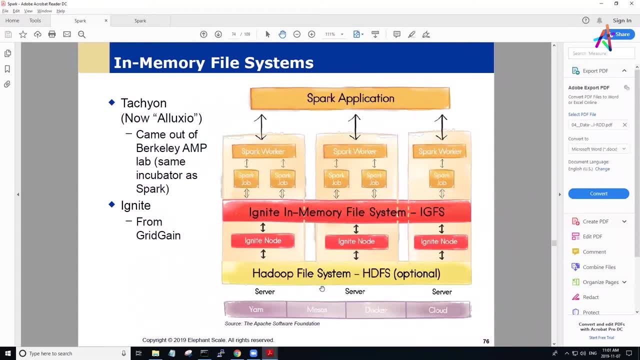 So we'll go back to the question about what's the upper limit. Again, I'm not really sure You know. it may be something incredibly, It may be the answer to just how much memory can you afford, And so, But there's obviously going to be. 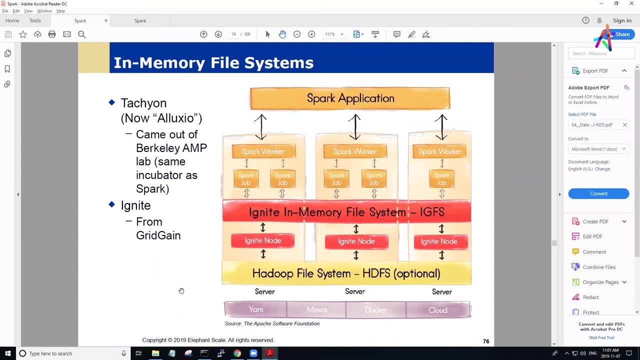 some practical engineering limits which we want to take a look at as well. Okay, so this is the idea is that we run this in-file memory system- And we've already looked at that. We get this sort of effect, So it doesn't use the JVM. 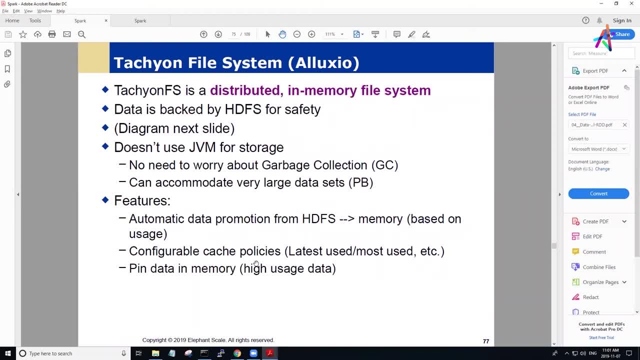 So storage bypasses all of that stuff. And again, this is what we call automatic data promotion, which is basically moving data out of the Hadoop cluster independently of requests, in order to populate the file system in using what we call cache policies. So there's a lot of different things we can do. 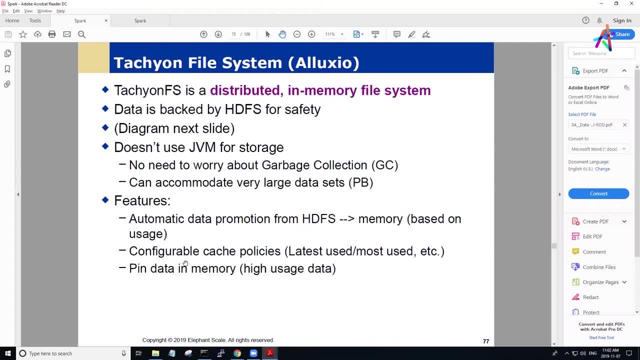 Pinning data in memory. In other words, don't move this out to disk. You know, we have a lot of experience with paging algorithms and that sort of thing, which led people to come into the Think about applying those kinds of concepts. 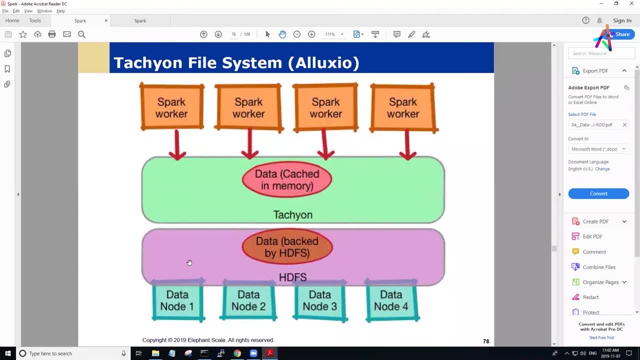 to these kinds of solutions. So there's our Tachyon Memory. Again, it's transparent to Spark. It's a layer that goes into here. So Spark is working with a file system. It just happens to be a cached file system. 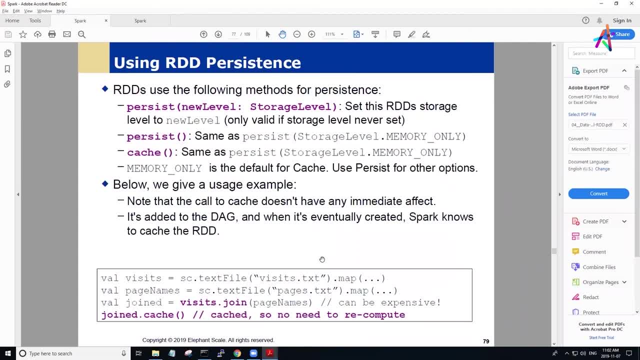 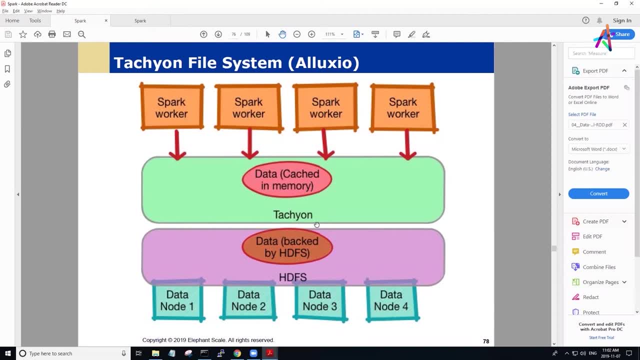 which is basically backed in memory. Okay, so it's. And, like I said, this is generally a presentation of this. And one person said: just think of this as being a virtualization of this. That's not quite right, But again, you can think of the fact. 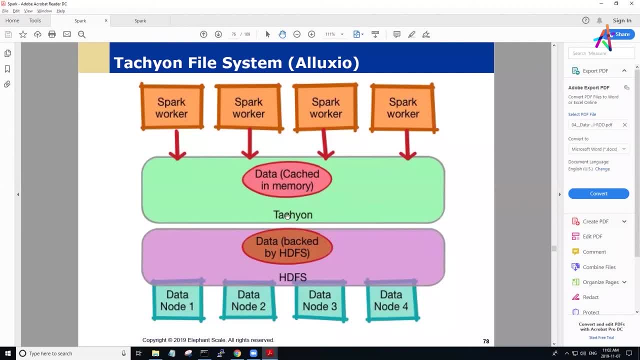 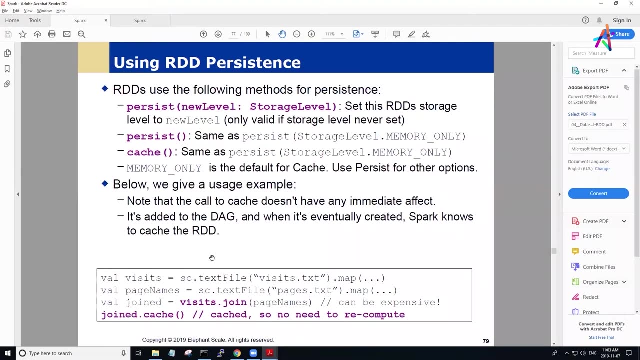 that we're introducing another layer of a staging area that speeds up the actual access, because now we can do optimizations on how the data gets into memory and when it goes into persistent storage- RDD persistence. So we do our persistence using the various parameters And we're not going to get too involved in this. 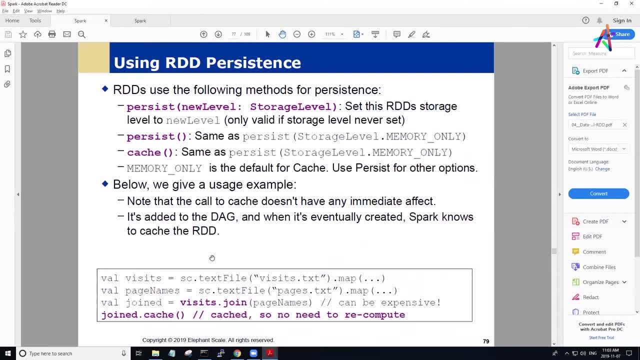 So we'll, Because we're going to spend more time on data sets and data frames. What we just should know about it is that we saw persist before And I'd mentioned that caching is kind of a shorthand for persist And so cache you can see there. 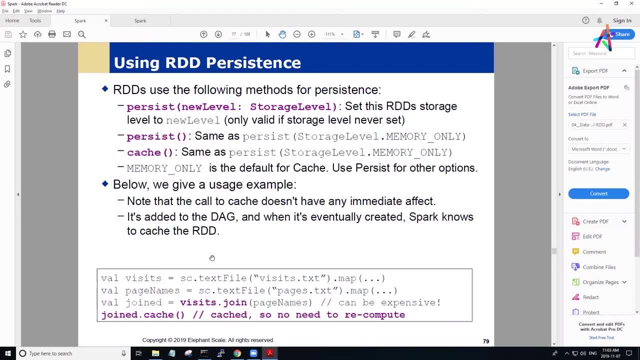 is the same as persist, storage level memory, only It's just a faster and easier way to write it. So our persist And so persist and cache are basically the same operation. But then of course we will use the persist with arguments to tune the actual persistence mechanism. 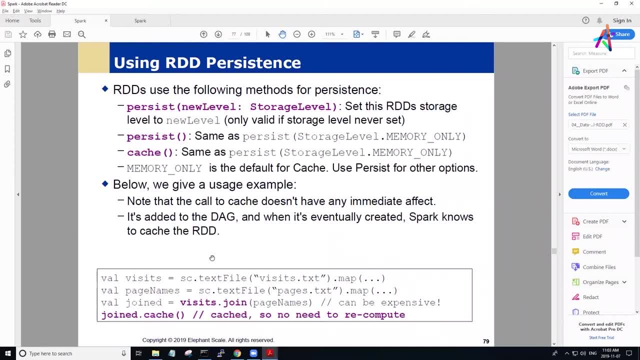 Example down on the bottom is when we actually want to do this. Again, we're using the SC context here, So we are working with the older interface. So we've got an RDD called visits, Then we've got an RDD called page names. 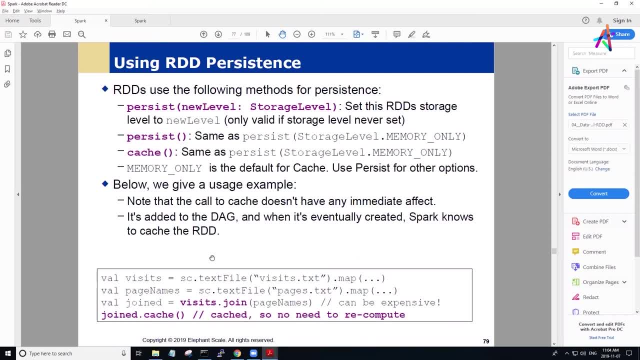 And we're going to do a join. So the join is a very expensive operation. So if we have other things that are going to require a join, we don't really want to recompute it. So we'll cache that join so we can reuse it. 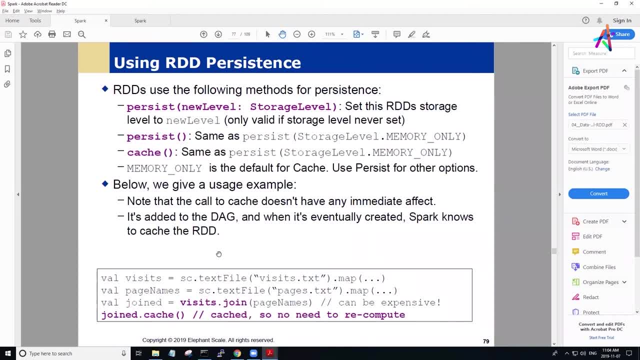 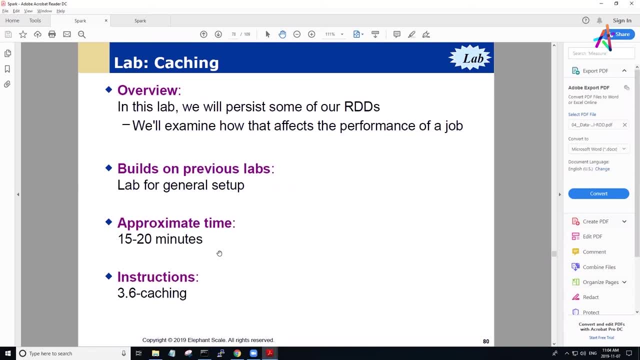 in subsequent computations. There's an example of where we just don't want to recompute something because it's too expensive. Okay, So we're going to try this out And this is our lab for caching, And this is going to be lab 3.6.. 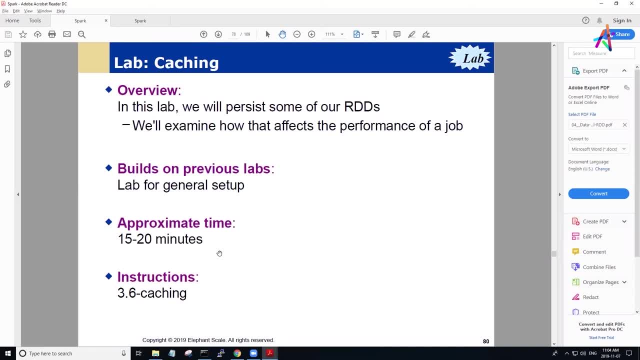 Now I haven't gone through these labs yet. I'm still just actually kind of getting all the logistics here sorted out. So I will take a look Now. I do have solutions for this, but not yet. I've asked Mark to give me the solutions. 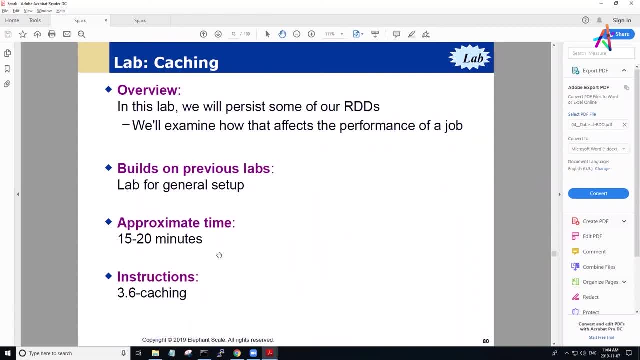 And I'll see about providing solutions for everybody tonight so that you can actually go and look at the solutions to all of the labs, as recommended by the course designer. Okay, Do we have questions about caching? I know I've deferred a lot of the discussion. 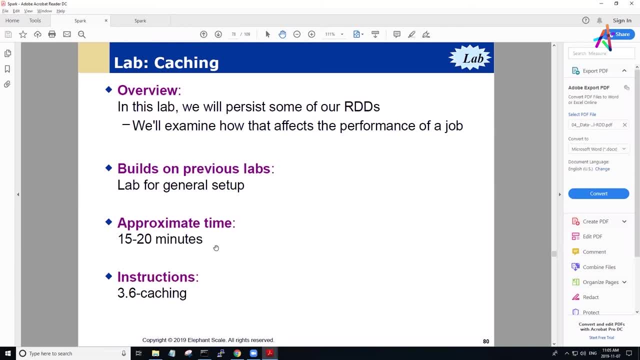 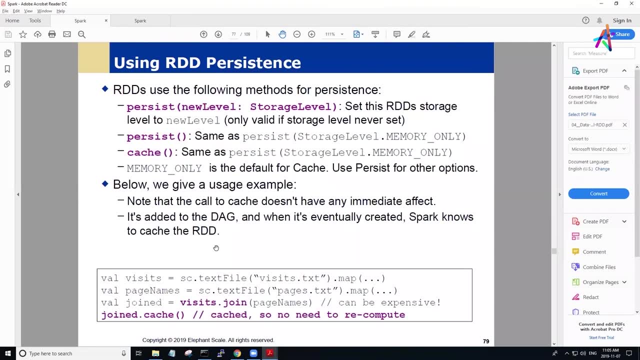 into our module on Tungsten, but this is really just sort of a high-level overview. Okay, So don't worry too much about the little details. Any questions about caching? All right, Yes, I have one question. Yes, go ahead. 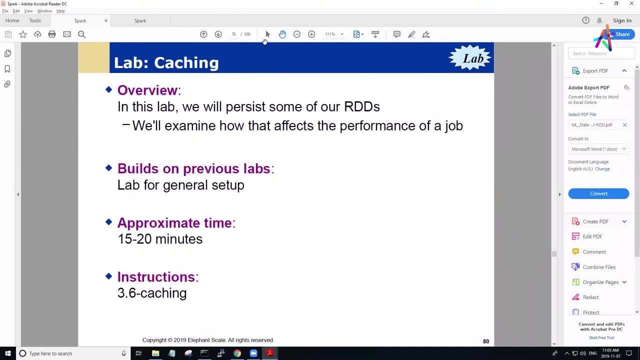 So there was memory and disk and then there was disk only. Why would you use disk only if there is memory and disk And whatever doesn't fit in disk is spilled into memory anyways? I think it's more of a use case issue. 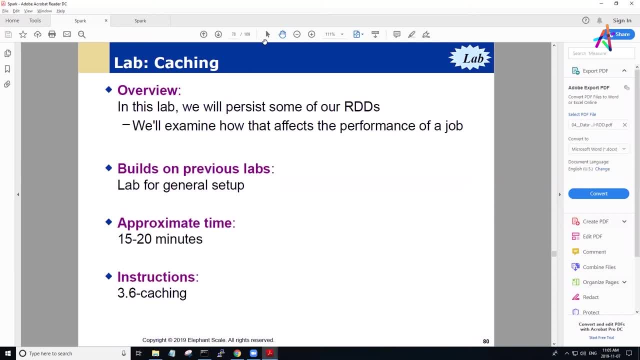 I mean, I think what happens is that, if you want, like if you're doing a really, really, really expensive computation- and, like I know, I was working with some people at Statistics Canada and they were doing a query, an SQL query- 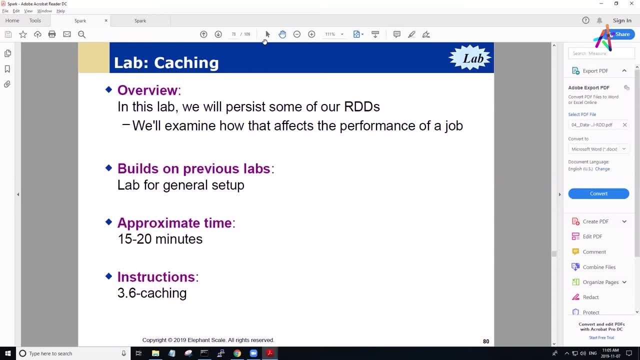 and it took three days to run the query because of all of the complexity of the data. And what they did was, once we had the results of the query, that became their operational database and everybody worked off that and it was actually stored in a separate database. 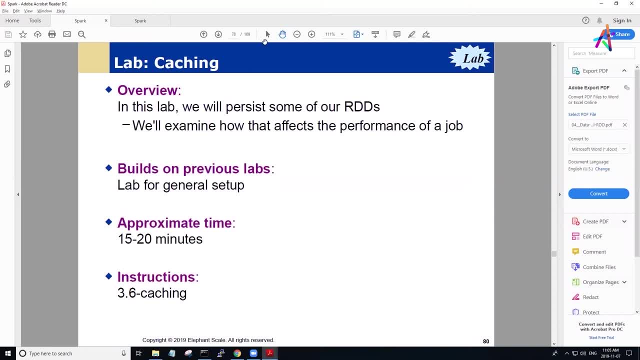 The use case here is that: getting the data into a form that we're going to use, we're going to want to use over the long term, not just in the immediate. that's something we're going to come back to over and, over and over again. 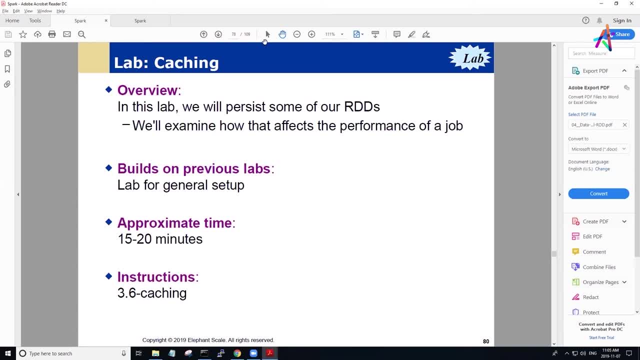 It may be more efficient to cache it to disk and then when we actually come back and get it out of disk, we're not burning up memory. So I'm suspecting the use case for that is that when you're looking at wanting to persist something to disk, 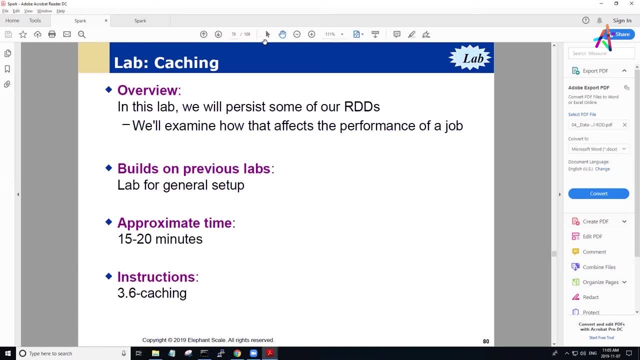 for a relatively longer period than the immediate calculation. maybe you want to save it there and use it in another problem. That's my take on it and I hope I'm right. I'm not sure if anybody I've ever talked to has actually used that. 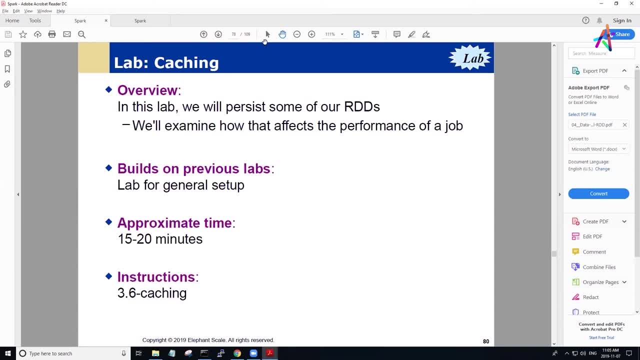 so I'll check for other use cases, But that's the use case that occurs to me when I first think about it. Thanks, Okay, Yeah, I don't really think caching disk only is something that you would normally do if you're just running like a Spark job. 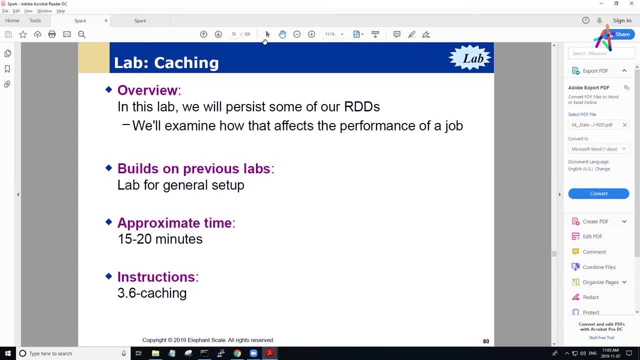 because I'm not seeing any advantage to it. but I can see advantages if you're caching stuff that you're going to come back to much later, but you don't want to occupy the memory in that intermediate time, Okay, So I'll let you guys get to work on that. 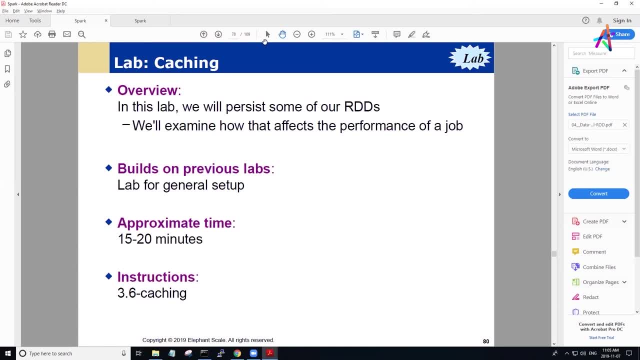 I'll check in with you in about 10 minutes and see how you're doing, and then that'll probably bring us fairly close to seven minutes after the hour. Yeah, we'll probably be able to finish this up and start talking about DataFrame. 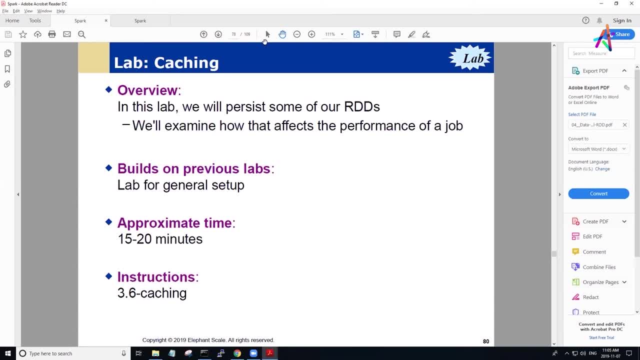 but we'll talk about DataFrames today before we take a break, So I'll give you guys about 10 minutes. You guys are really good, so I don't think you're going to need all of that approximate time that's required. You don't have anything to add memory on. 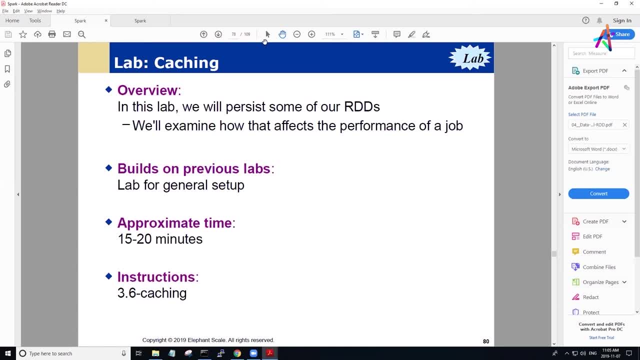 because it's a default. Maybe, yeah, and persist, But this is done. persist. It used to be a memory. This is the random data right, So it used to be serialized. Now I'm doing. Now you have to end. 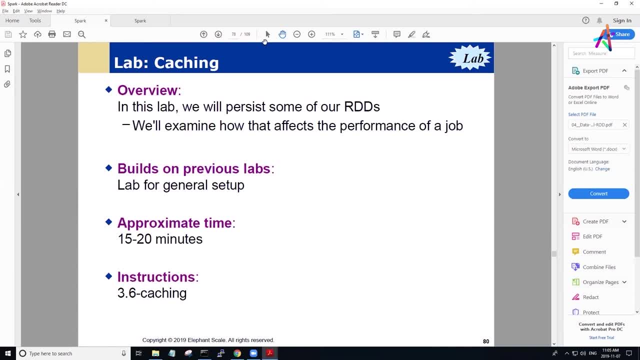 And persist with the brackets. Yeah, And now you have to count whatever Strings. what's it Internet Like? are they sort of cached as singletons within the JPM? So if I use the same string, like I just define two variables. 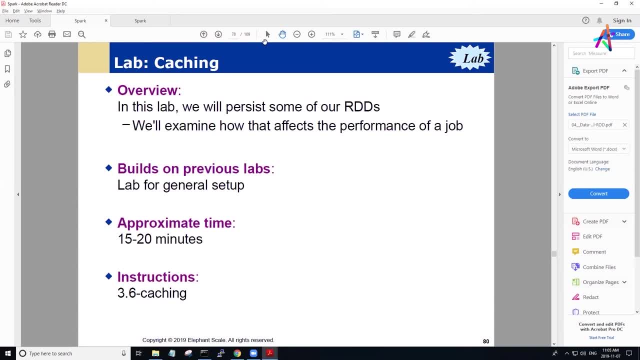 with a string, literal ABC, will Java create two ABC objects or will it be the same object in the end? That's a good question, Because I mean, I think Ruby kind of does that explicitly via symbols, And then I think Python does that automatically, or 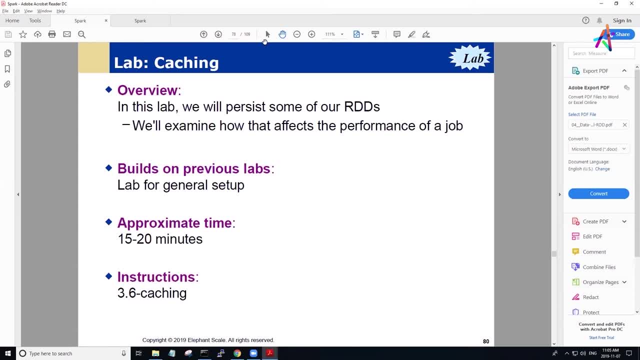 I don't know exactly. Excuse me, what was that question? I didn't quite catch it. So this is more of a JPM question, I guess. So I know that some languages, either explicitly or implicitly, they automatically define singletons. 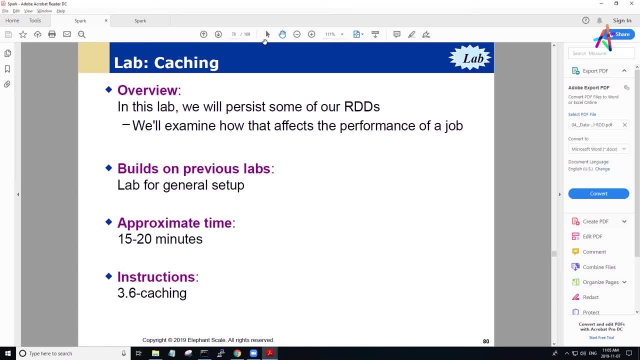 for some values like short strings. So if my application I use the same string literal a thousand times, it's not like it's going to create 1,000 string objects, but it will just reuse the same object as a singleton and just provide a reference right. 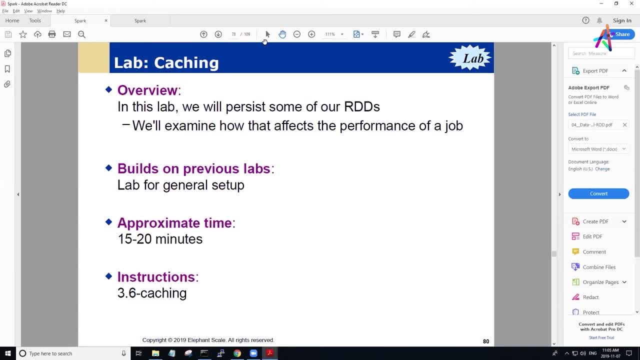 Yeah, I don't know if this is the case in the JPM or not, because we're discussing applications, The amount of Ruby that deserialized data structures with, But I think in Syntaxic Sugar it creates symbols like for each of them referencing the singleton. 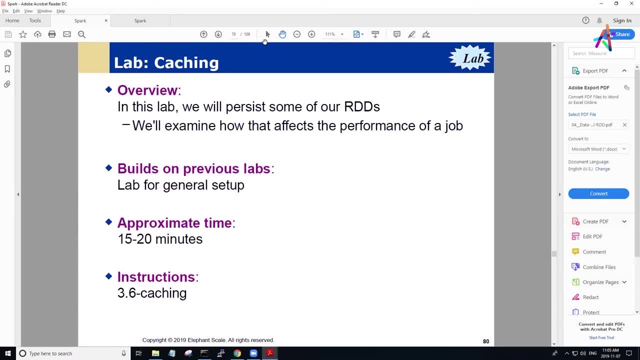 So I think Karsten read JPM first of all because he was thinking about the tungsten project. Yeah, so I mean this is completely unrelated to Scala or Spark. Just a general question about JPM, where there is this mechanism within the JPM. 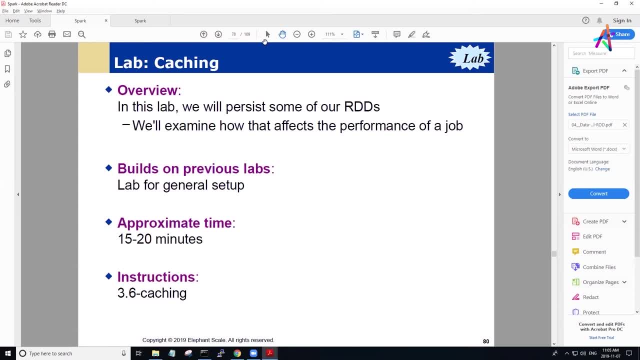 but it is sort of more tries to be smart in that sense. So I think it's a good question, but I think it's a good question to keep internally singleton objects for this repetition. Okay, You know, there's actually an interesting sort of answer to that. 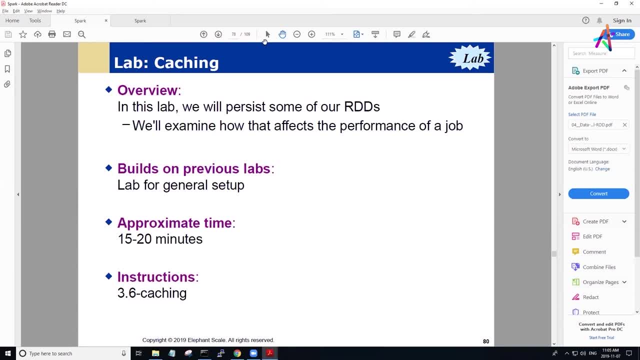 Yeah, In the sense that the original RDDs were opaque, So that kind of optimization could not have taken place with the original RDD interface but with the unified data set interface. there is a mechanism, like you're talking about the typing with the RDDs- that allow. 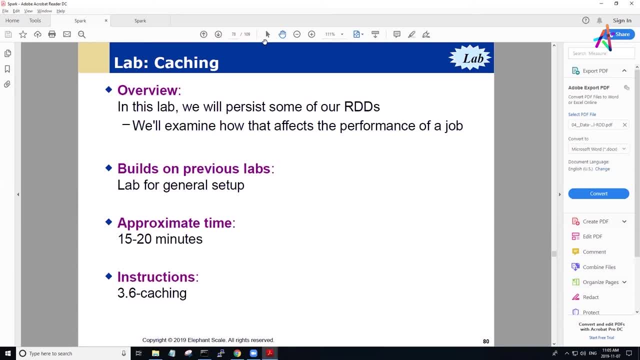 for that kind of optimization to take place. So a lot of it has to do with the introduction of typing into the RDDs, which is where the new RDDs are different than the old ones. They allow for kind of hooks into that, not that specific. 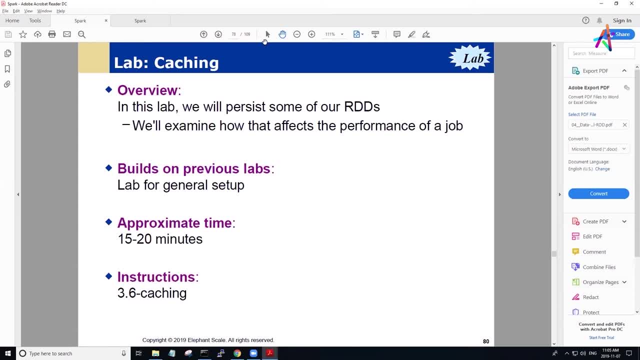 but that type of optimization. So what I'm seeing with these exercises is that they are very simple, right, Just run a couple of months, but the interpretation of what we see as an outcome. that's more challenging than I had anticipated And in that regard, 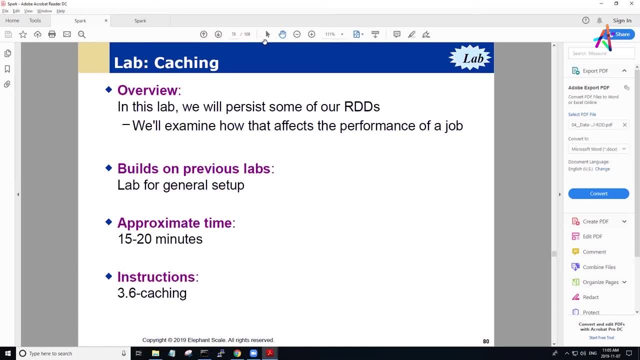 they are quite interesting, just to revisit later and really try to grasp what's exactly going on, Because some of the outcomes are not that intuitive, or So yeah, I guess there's some homework in this. Yeah, well, there's a lot of things going on. 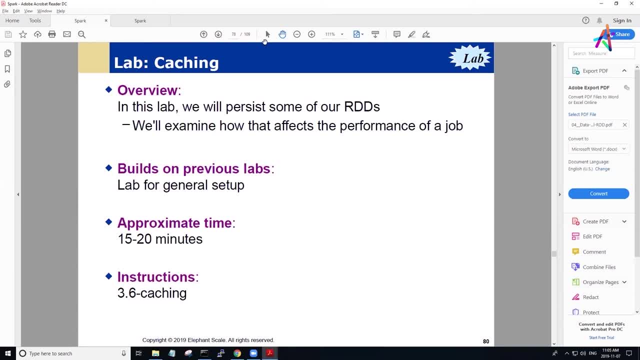 under the hood at this particular point too, that we have yet to explore. Okay, Well, I'm going to suggest that we take just a few minutes here to close off. I want to get off in about 10 minutes, but I'm just going to introduce kind of this section: 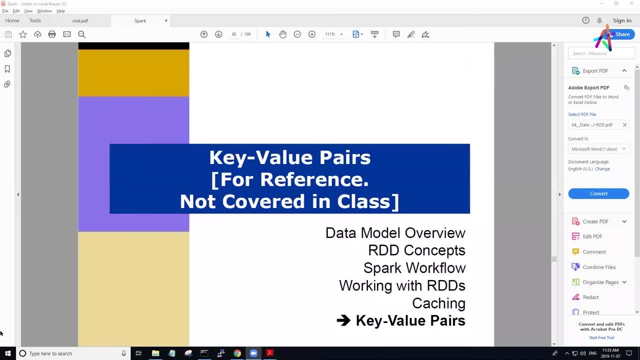 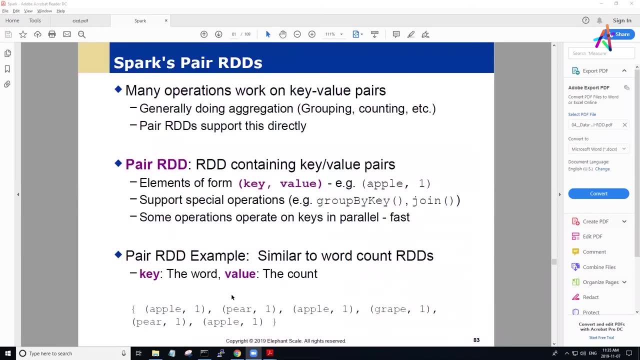 that's at the end of this module, as kind of a segue into DataFrames tomorrow. And this is this notion of key-value pairs, And this is kind of one of the motivations behind sort of the new, new kinds of RDDs where we work on key-value pairs. 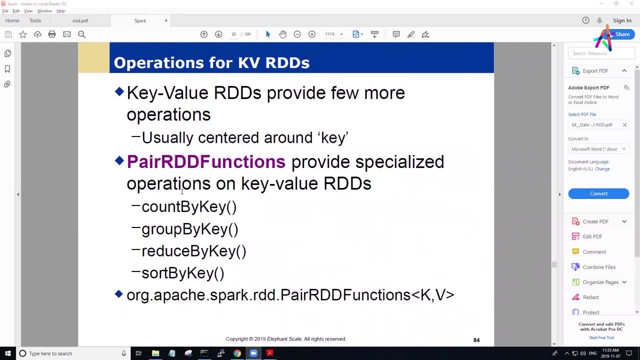 And we all know what key-value pairs are. So there's It's fairly straightforward, But we also can use the key to do various kinds of operations. So count, group, reduce, sort are fairly typical examples of pair functions or pair operators. 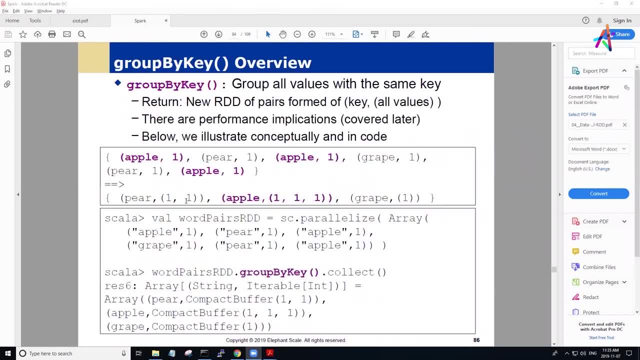 So we won't. So group-by-key does what you would expect: Groups all values to the same key. So we're grouping all of the elements together And we can do a group-by-key and then collect the results and get our arrays back appropriately. 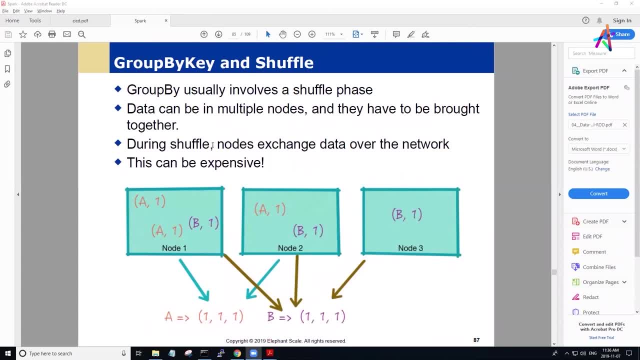 So we're going to just come take a look at kind of the underlying mechanism because group- And this is where we want to- And this is the point I just want to get to before we go, as an introduction to what we're doing tomorrow. 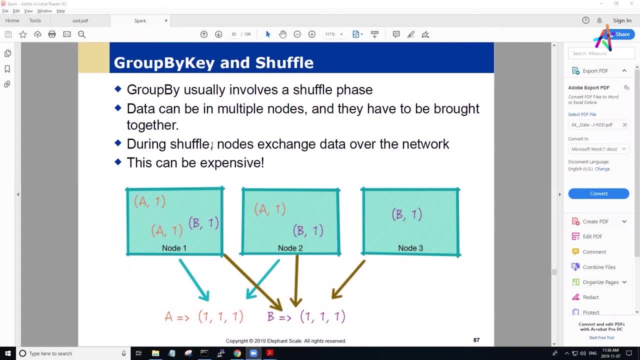 Grouping-by tends to involve a shuffle phase, because we may have keys in multiple nodes, So they have to be brought together through some kind of shuffle operation. So this is the. This is one of those performance hits that we take when we start to do. 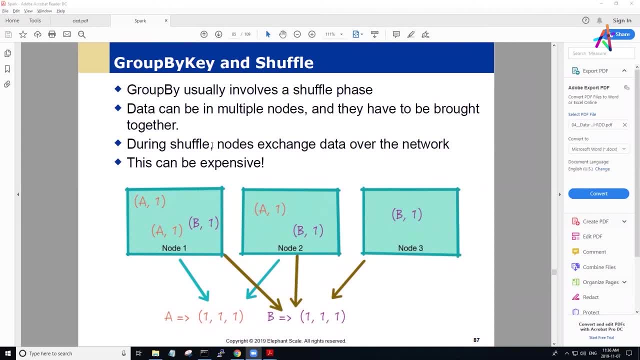 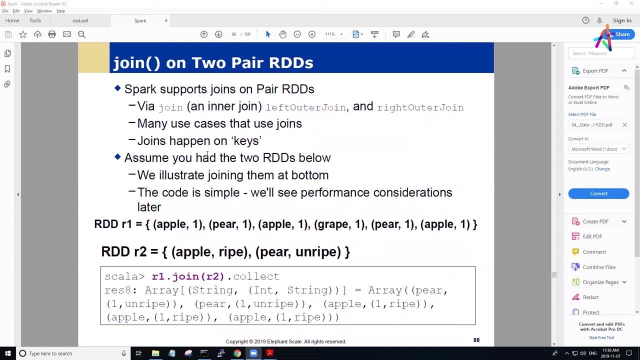 grouping kinds of operations, because now we're moving stuff over the wire and that starts to become a little bit more expensive. Okay so, And I just want to kind of go over just a couple of those points So we can join on a couple of pairs. 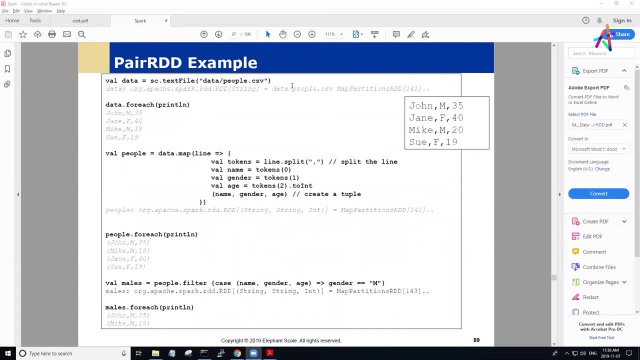 So we'll just take a quick look at a code example. We've got a bunch of people. This comes in in a CSV file. The format of the data looks like this: It is still, at this point, opaque to the RDD. These are just still strings of text. 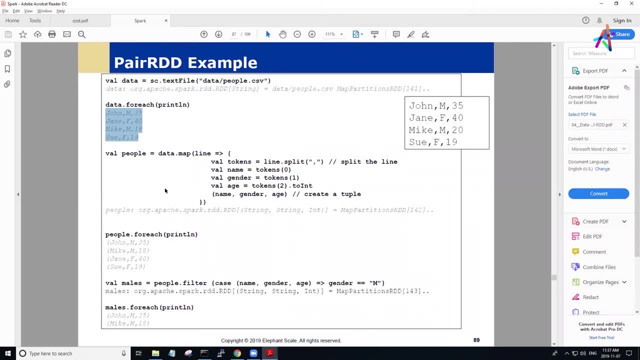 But what we can do is we can put it through a data transformation- create an RDD of people in which we tokenize these strings, and then we basically create a couple of variables or keys or a couple of key value pairs for all of the things, And then we take those two tokens. 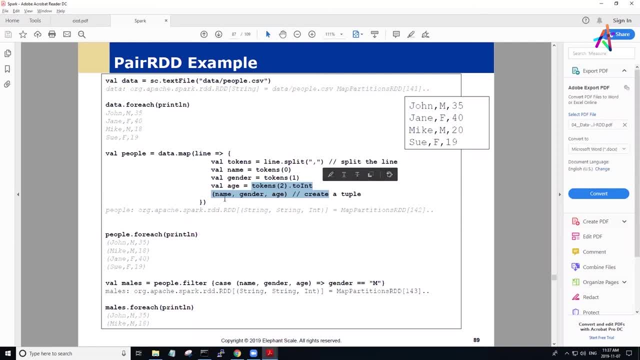 and we create them from int, And so we now have our name and gender and age tokens. So we take the first, second and third tokens and convert one and we wind up with a tuple Now, once we've got that structure, 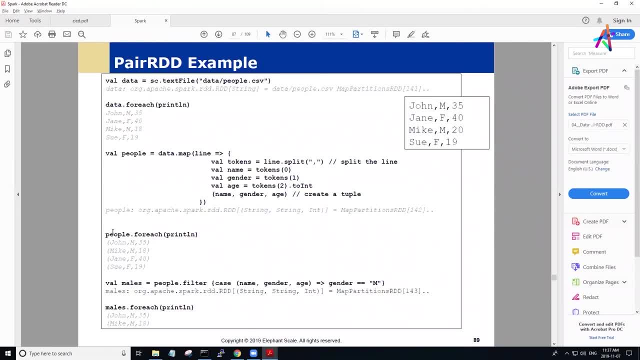 we've got something a little bit more easier to work with, because we've imposed some structure onto the underlying RDD, And so what we can do is now do filter, And in this case we're going to filter out all of the men, or all of the males. 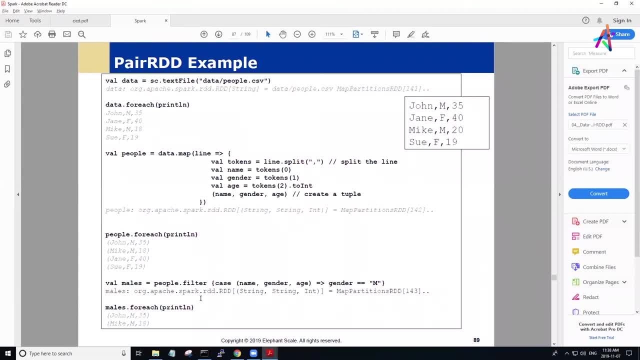 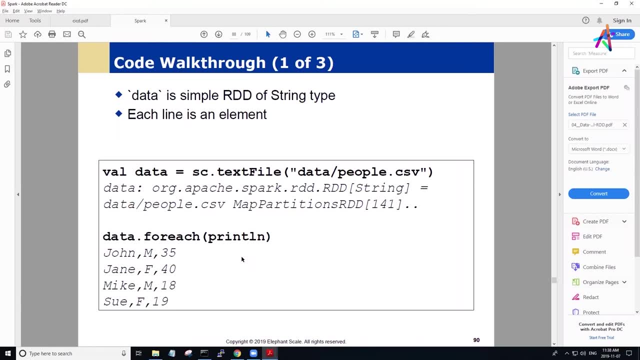 And we wind up with a new RDD which has that filter in place. This could not be done without a pair because again the data would be opaque. So data is a simple RDD of string type. Each line is an element And we wind up being able to tokenize this. 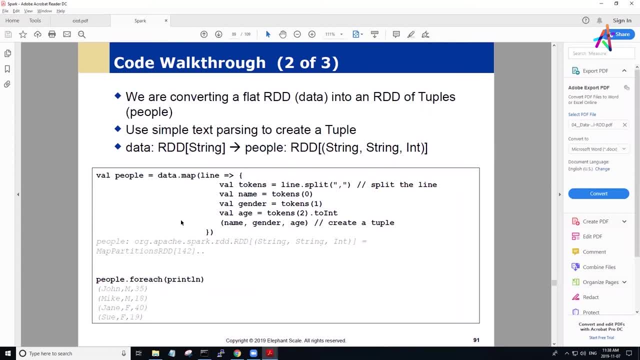 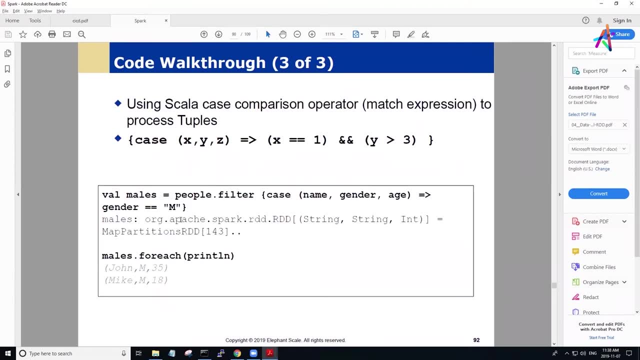 and take this flat RDD and put some structure onto it. Okay, so now what we can do is we can go and selectively do some comparison operators that we couldn't do before, when it was untokenized. We're actually able to do a reduction here. 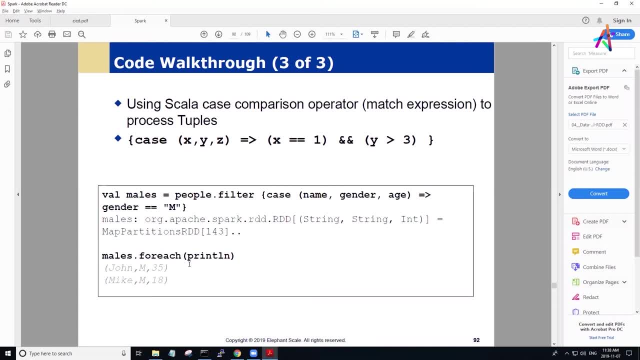 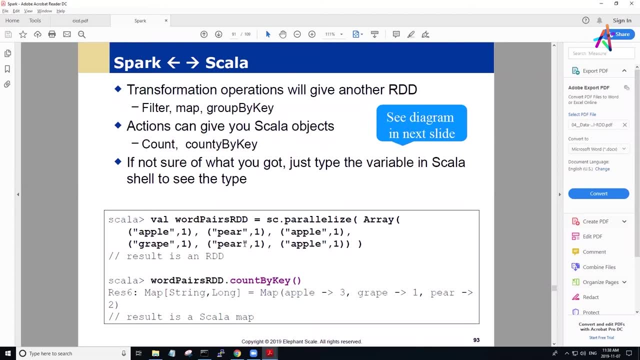 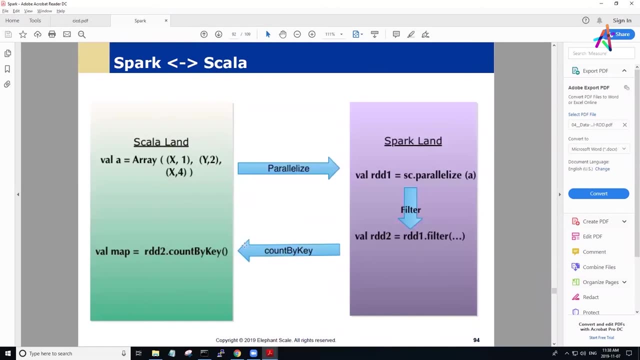 or a filter, which we couldn't have done before without a relative extensive computation. So in this particular example, what I just wanted to kind of close off today with is this idea that in Scala we're writing this code here and doing a count by key. 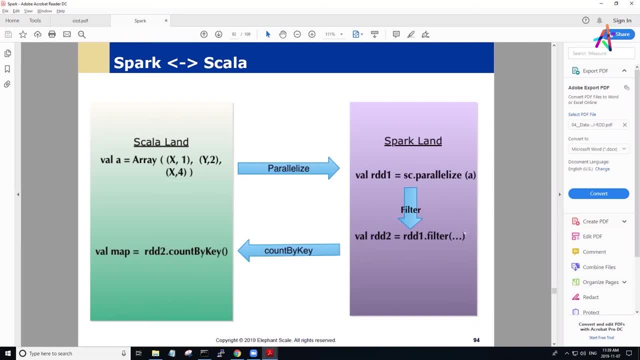 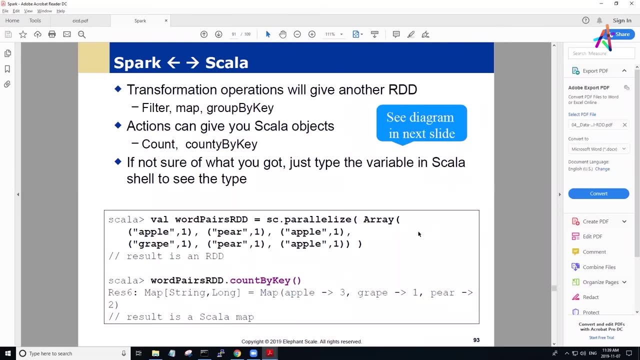 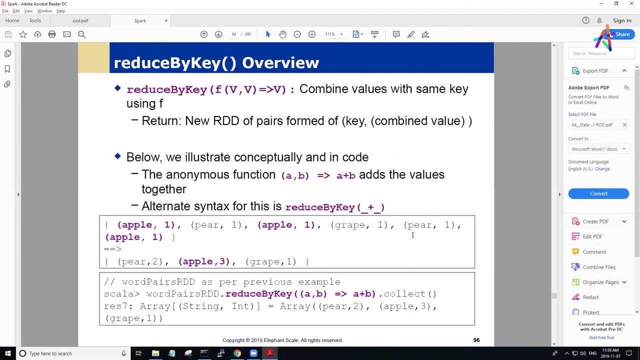 And then we over here have to parallelize things and then filter on each of the individual chunks. So the idea here is that- and we're not going to do this lab today- I just want to introduce this as a concept for tomorrow. 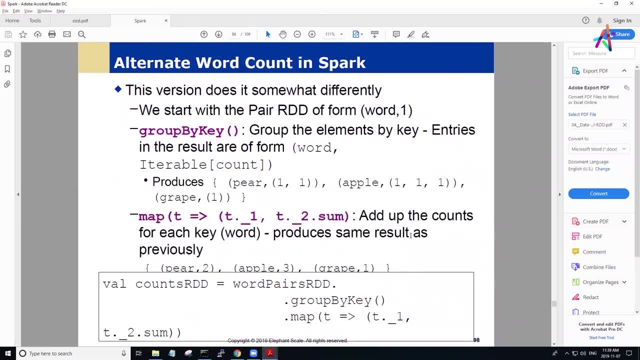 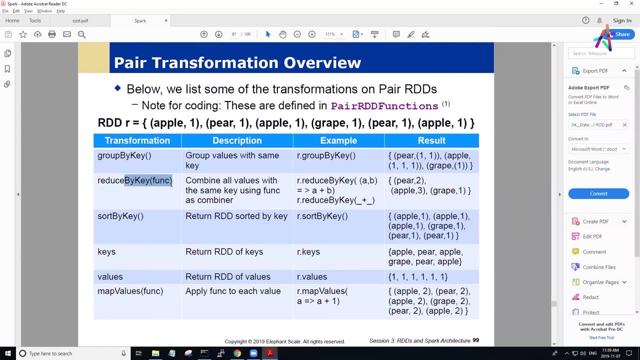 You can try to do this if you want. So there's a couple of other interesting things here that we can do, And this is where we're going to be able to. for example, reduce by key is a very efficient operation. Sort by key are operations. 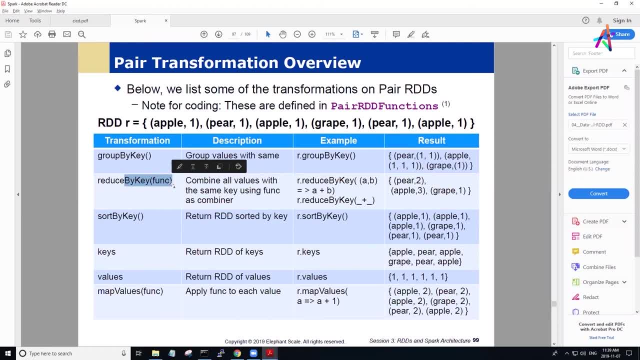 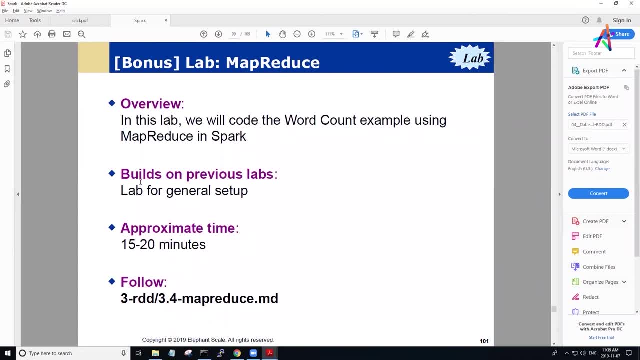 and some of them are going to require shuffles and some of them are not going to require shuffles, And we'll get into some of that kind of stuff later on. But I just wanted to introduce that as a kind of a concept for what we're going to do tomorrow. 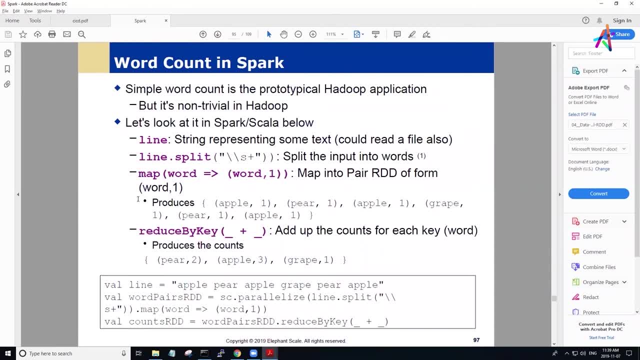 Basically working with these kinds of hold on for a second here, just one moment. Sorry, I accidentally muted myself there. Okay, so again, this is the idea of the transition from this. data frames is the idea of imposing structure on something. 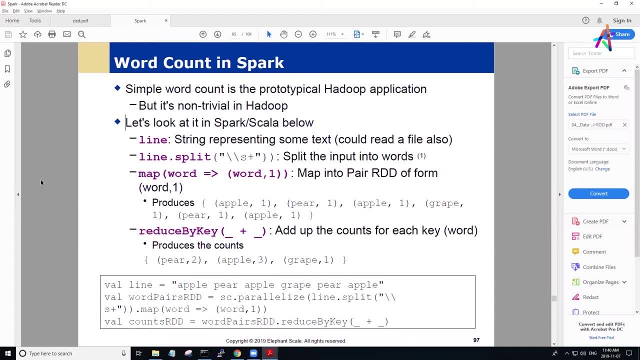 Okay, so tomorrow what we're going to do is we're going to come back and start looking at data frames, And that shouldn't be too complex. Then we'll get into data sets And as we get through that, we've kind of finished the initial architectural. 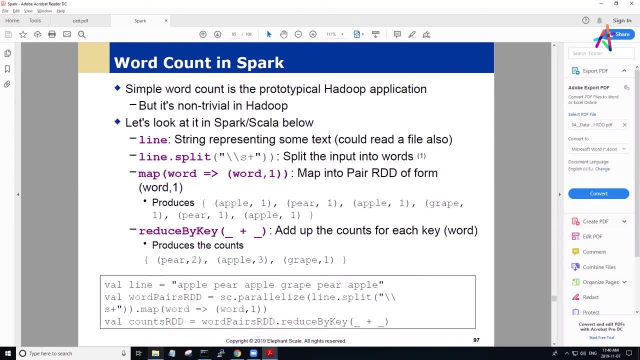 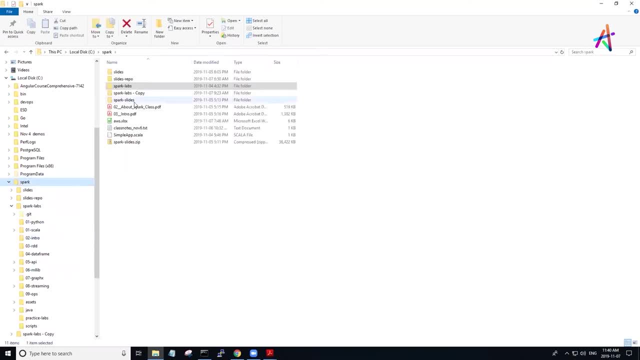 kind of position or architectural part of the course And we will be looking at. I'm not even sure where those slides are at this point, But anyway, we'll do a little recap on what we're actually going to be covering off tomorrow. 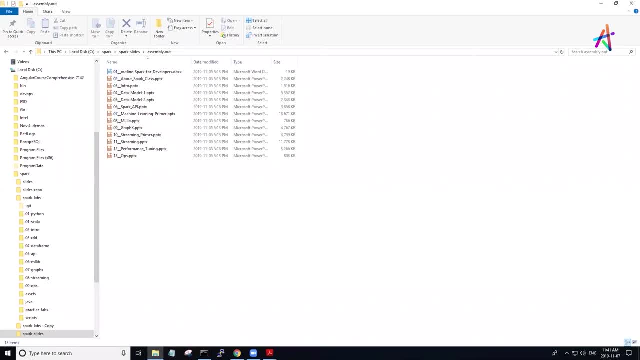 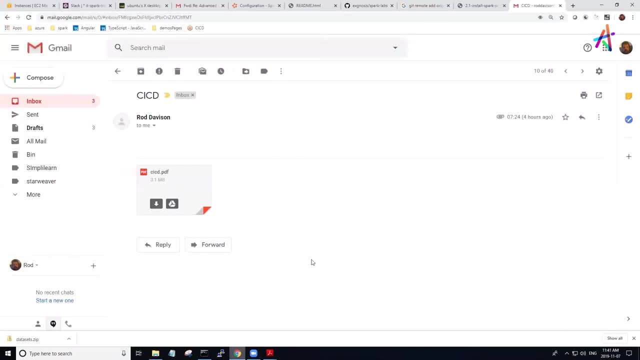 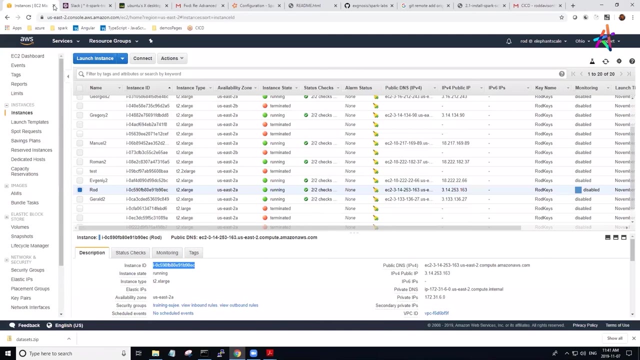 But what we're going to be doing. so how are you guys? are you guys enjoying things so far, Or how are things going for you? There's a little poll before we leave: Suggestions, Options, Opinions. Might be sorry. 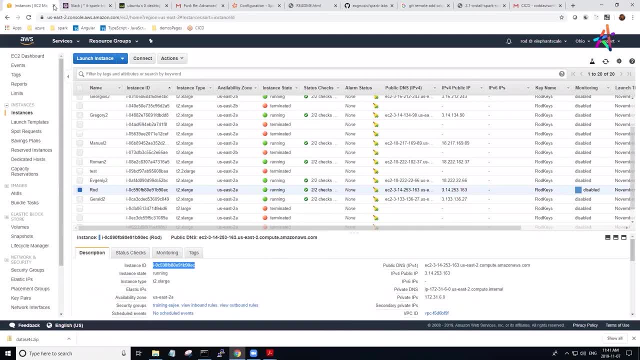 might be a little bit too late, but can I ask a question about the latest exercise that we did? Yeah, sure, Well, maybe another question, but rather I just wanted to confirm something. So, incidentally, I've tried doing the serialization. 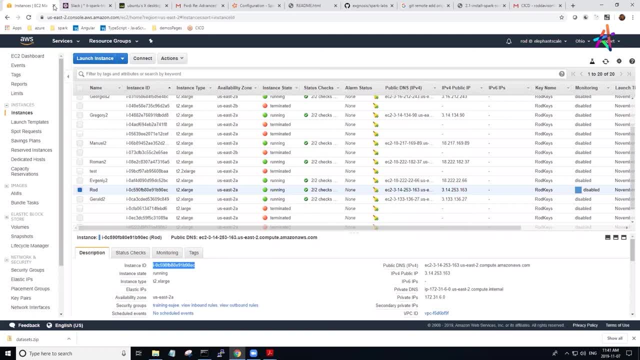 storing in memory only without the serialization, and with memory in memory, with serialization but not for the data, which was like the examples that we needed to work for, but with the random data, Okay, And I figured out that serialization doesn't really help. 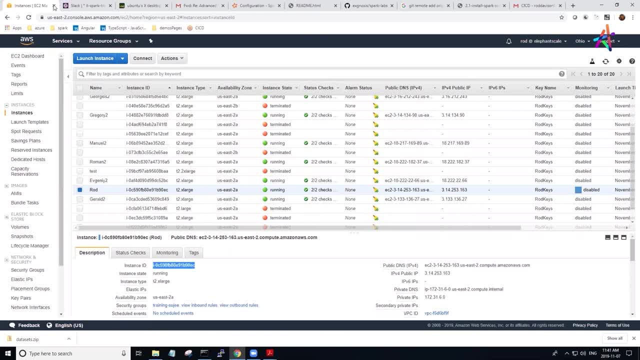 So it reduced from 105 megabits or so to 102.. So does it essentially mean that serialization here here involves like compressing the data as well? Yes, I believe it. Yes, That's a critical part of the serialization. 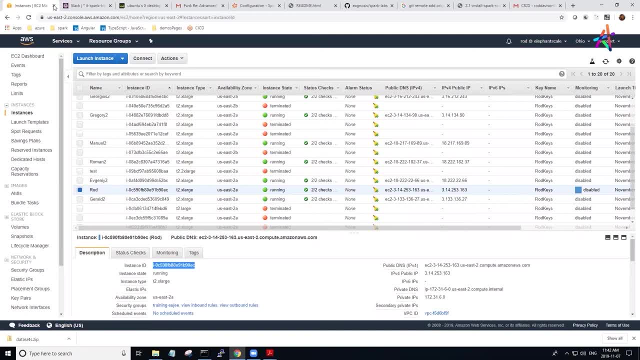 Yeah, That's why you're able to get that compression. So if you've got truly random data, then you know the serialization is not going to give you any significant data compression. Yeah, Okay, Thanks, Okay, All right. 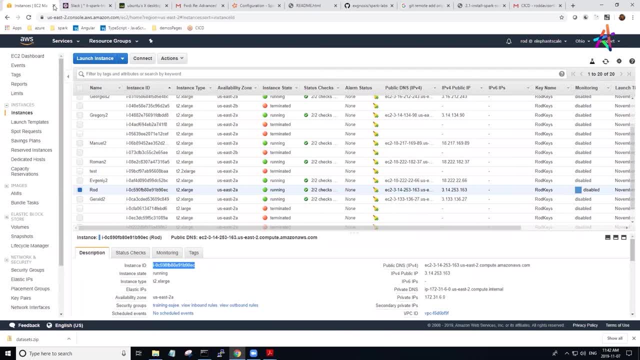 Well, I'm going to bail out now, in a minute, but what I'm going to do is I just want to get your opinion on something. I am going to be shutting down all of the virtual machines after class so that they don't get attacked. 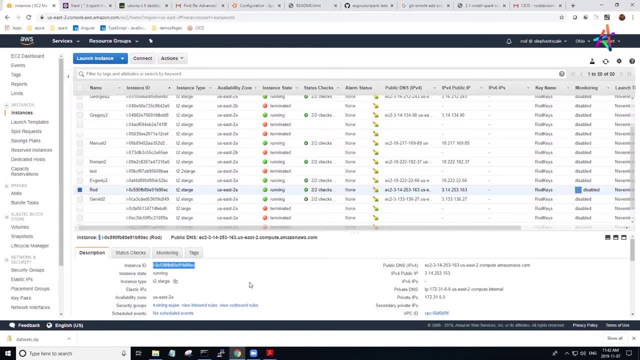 And then I'll start them up just before class. Now. if anybody wants me to start up the machine for them at another time, just contact me by email or on the Slack channel and I'll put your machine up for you. I just don't want the machines to be damaged. 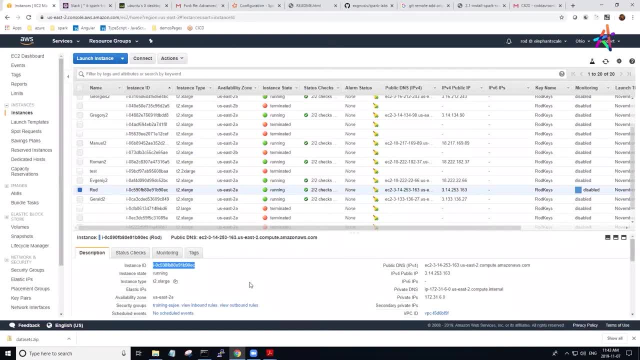 So I will do that in probably about 20 minutes or an hour, just to let you guys get a chance to kind of close up what you're doing. So it's about quarter to now. So let's say, within about an hour I will shut the machines down. 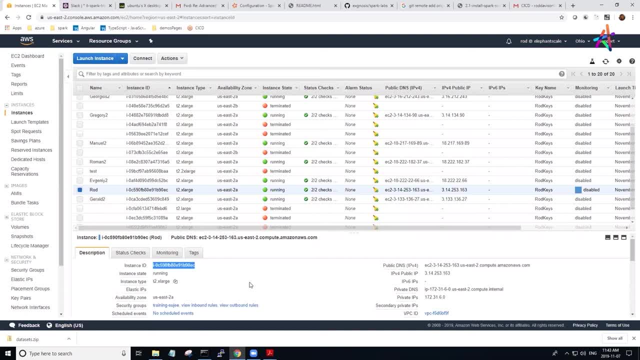 unless you tell me specifically you want your machine to stay up. All right, Does that make sense? Yep, Okay, good, Yeah, I don't want to inconvenience you, but at the same time I don't want us to do silly things. 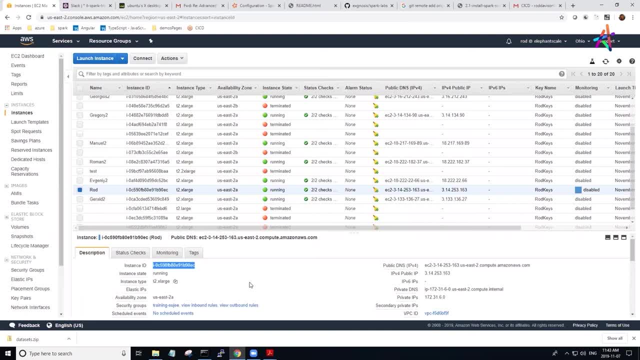 Okay, All right. Well, I will end it for today and we'll see you guys tomorrow when we explore the wonderful world of DataFrames. So hang tight and have a great evening. Take care everybody. Thank you, Yeah, Bye. 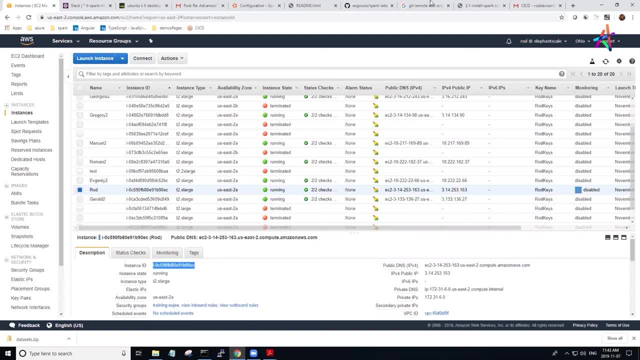 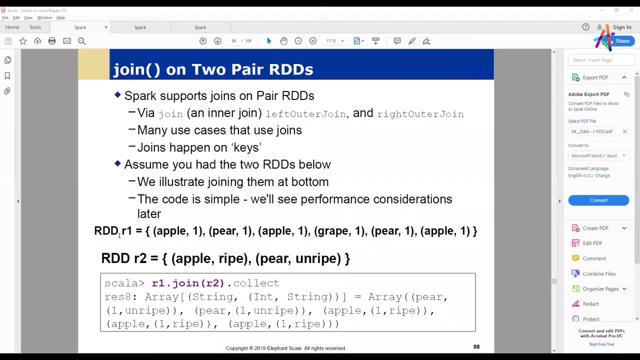 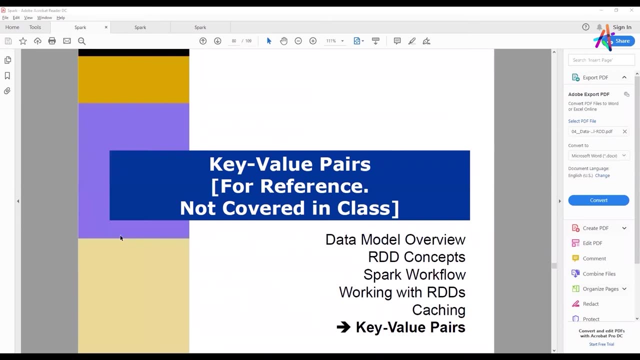 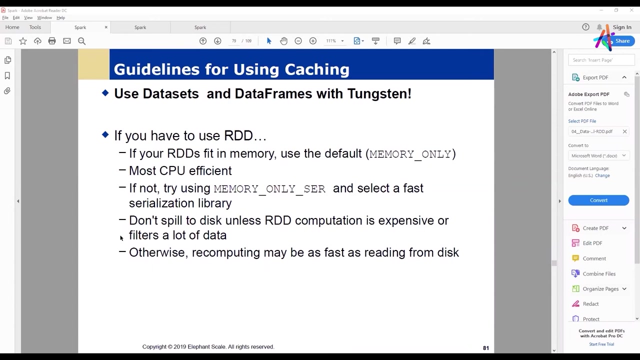 Thank you, Bye-bye, Bye, And remember I'm available on Slack, All right. So what we looked at yesterday was the RDDs and looked at sort of the idea of how they were conceptualized from the logical perspective versus sort of what was going on. 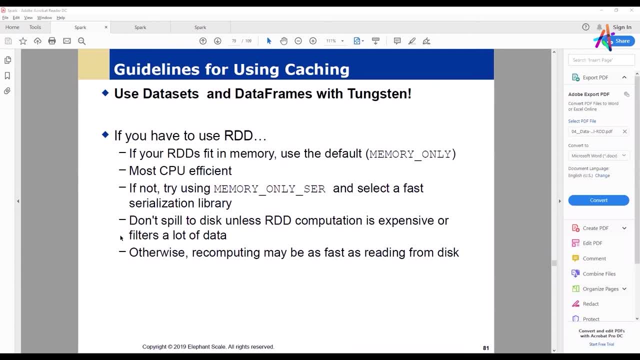 in the underlying implementation of them. And this gives us a basic idea that we're going to follow through with a little bit today as we get into DataFrames and work with the DataFrames of the idea that this conceptual model is opaque to us or makes the underlying implementation. 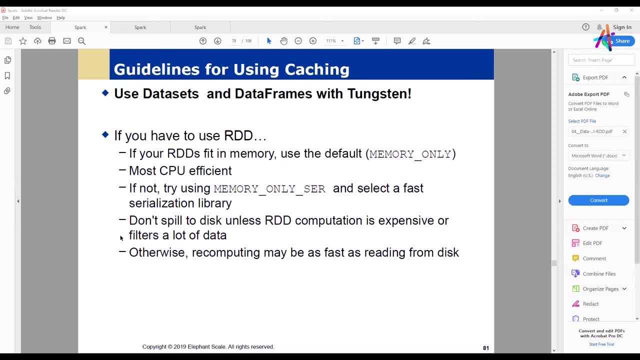 relatively opaque, so that we can model the processing from a strictly logical point of view, which gives us a logical way to look at how we can optimize this logical work plan. but then this logical work plan is optimized in some way, And then we also wanted to look at 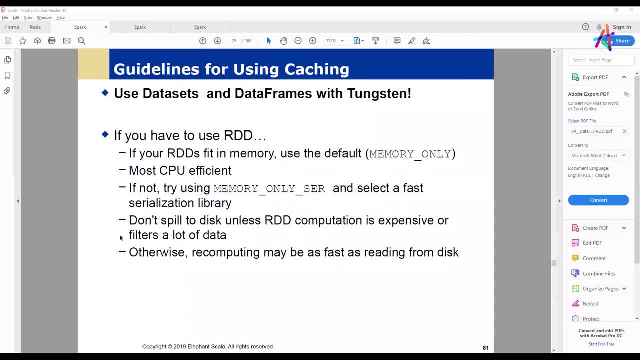 how we can optimize that even further. The one point that we did make about the RDDs is that they are relatively opaque to Spark, so that there are some optimizations that we could do that Spark can't because it doesn't have a semantic sense of the data. 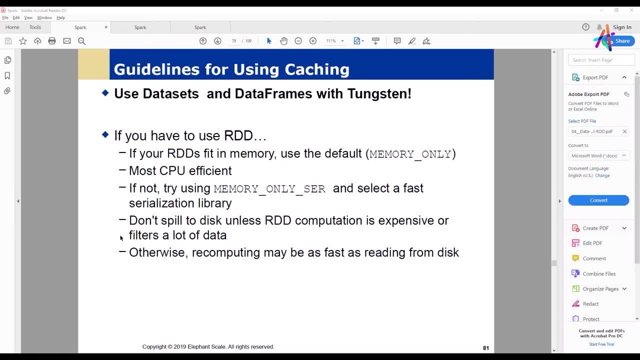 So the other thing we looked at also is this notion of caching, which was a fairly interesting notion, where we're looking at some things that are coming into optimization as well, where we're looking at being able to fundamentally save intermediate results for the processing. 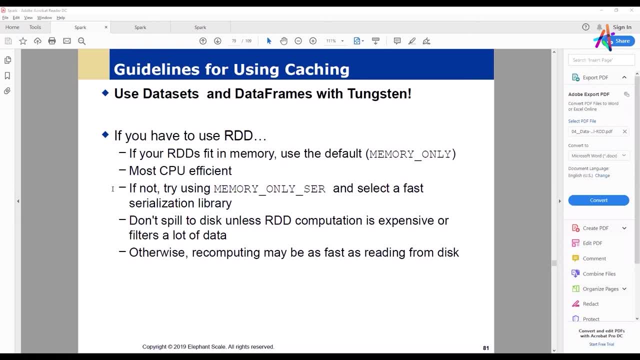 Okay, so any questions before we begin? So yesterday we were using data sets, not data frames, right, Yeah, well, here's the thing about that terminology, And I'm also guilty of sometimes being sloppy in my terminology. Data frames are basically similar. 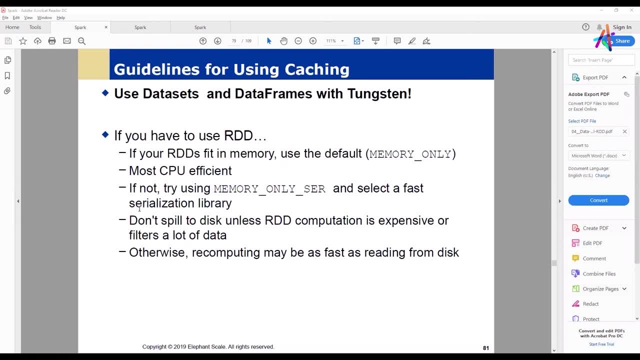 to data frames as referred to in other things like R. We're really looking at tabular data like SQL type of data Data sets. in Spark is a unified interface to both RDDs and data frames And that is where you were noticing the other day. 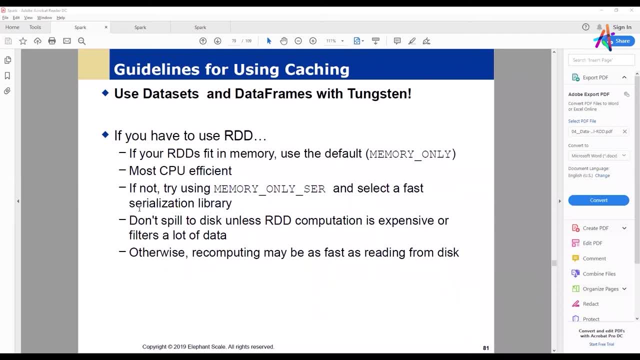 when you were actually working on it. There's two interfaces to Spark, when you were at the command line. One is the SC interface, which is the Spark context interface. That's the older interface, which basically allows you to work with RDDs. 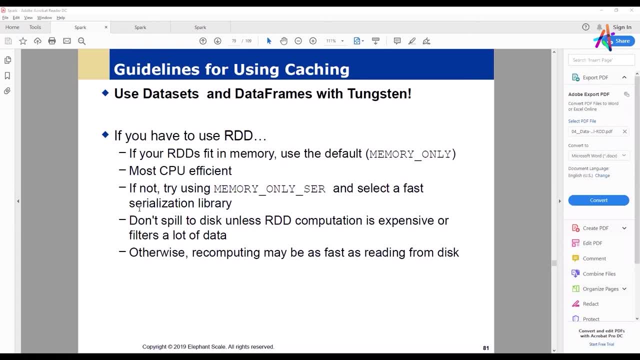 The other interface, which was the Spark object, is a unified interface that allows you to work with both RDDs and data frames, And that interface adds a little bit more functionality to the old RDDs so that they're easier, more efficient to use. 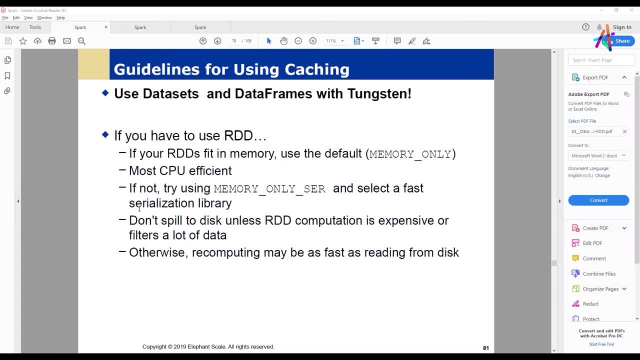 So data sets are a unified interface to both data frames and RDDs, And that's just the terminology. Does that answer your question? Yeah, thanks, Okay, okay, So I personally get a little bit sloppy, So if I sound confusing about it sometimes 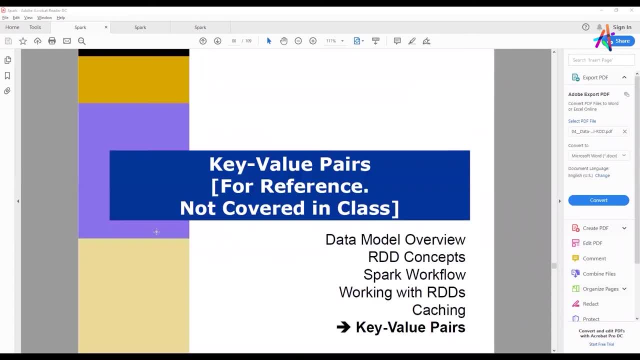 just call me up on it. Okay, so we're just finished off with this And I'm just going to take a look at a couple of points in here. Then we're going to jump into data frames And there's some various labs. 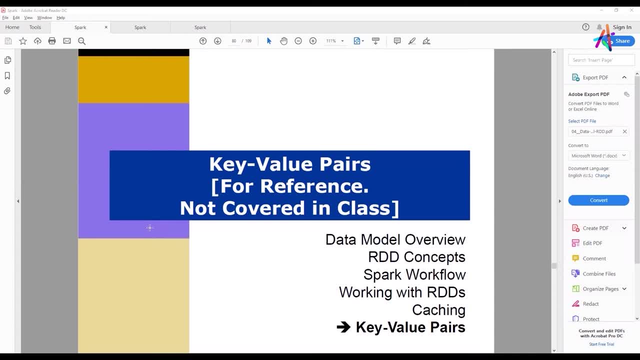 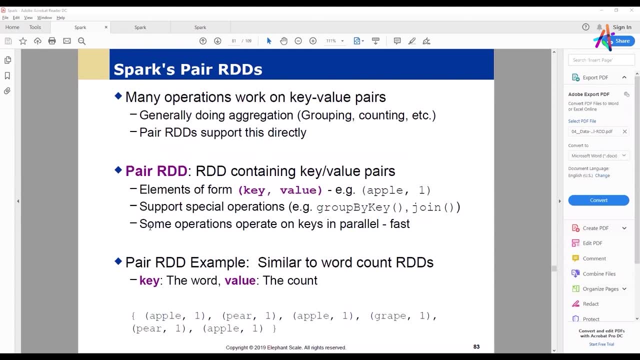 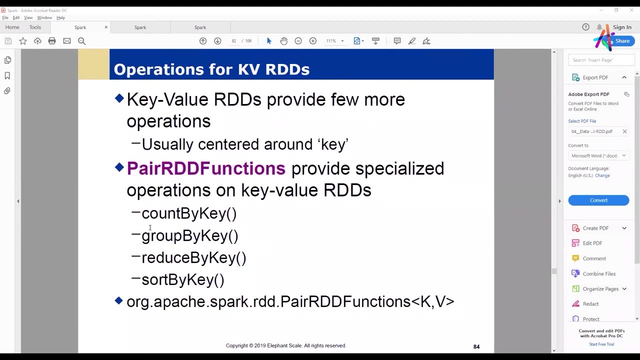 that we're going to do, just to experiment with the underlying model, And this is what we stopped with yesterday And this is where we were adding a bit of structure onto the RDDs. And I had mentioned this notion about introducing the pairs, And I think we looked at this example here. 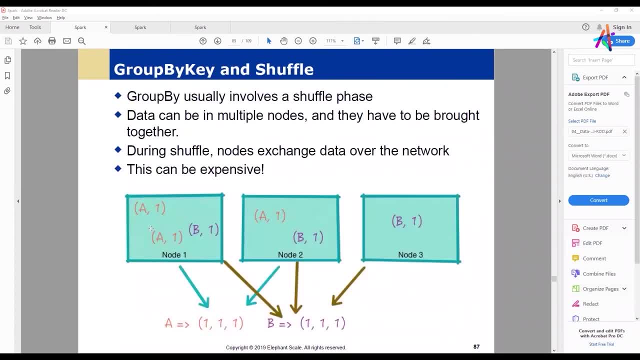 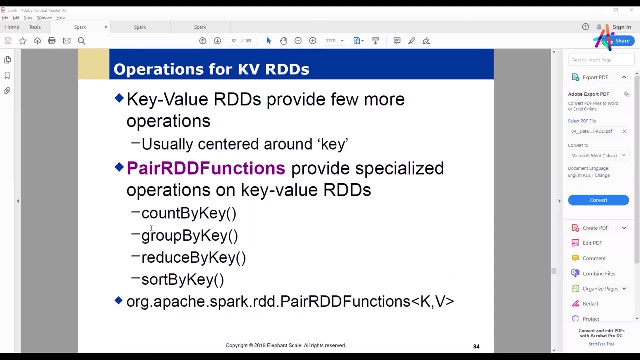 where we maybe there wasn't this one. I think we did a little bit further on. Let's go back here for a second. So we also introduced some idea of underlying shuffles here. So the key value RDDs, and this is kind of the evolution of RDDs. 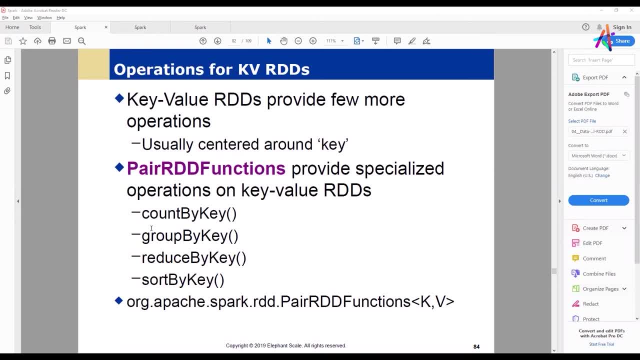 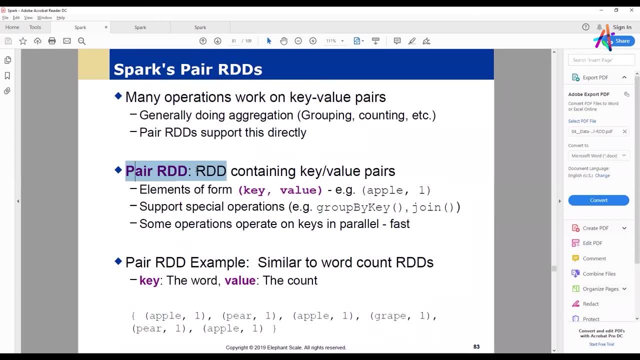 provide some operation centered around. the key- And this is kind of an evolution towards dataset- is the pair RDD. Now, once we've got this, we have this underlying structure, we have a little bit more power that we can use and we can get a little bit more efficiency. 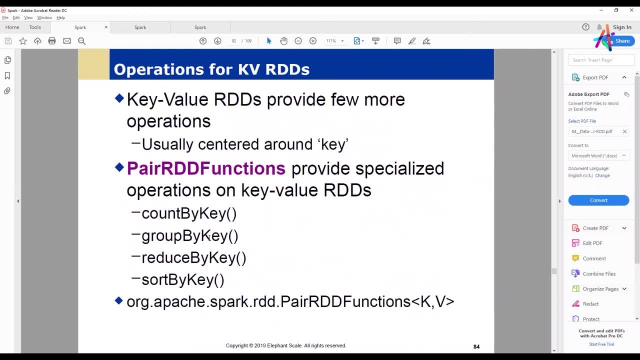 So the the standard kind of operations that we can now employ are: counting by keys, grouping by keys, reducing by keys, sorting by keys. you know kind of fairly, fairly typical kinds of things we would expect to be able to do. 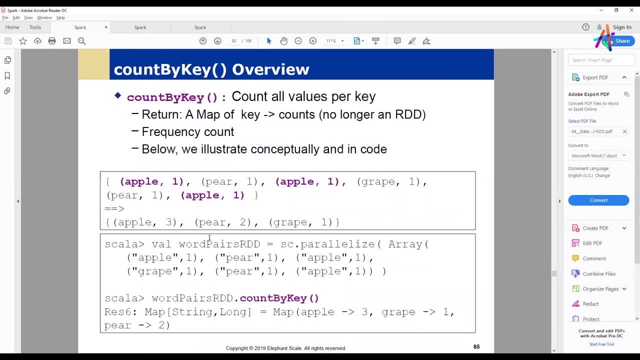 The count by key counts all the values by key. So we get a map of keys and this is would be considered an action, because we're not getting a, an RDD, we're getting a counts. So now there's the example of our pairs. 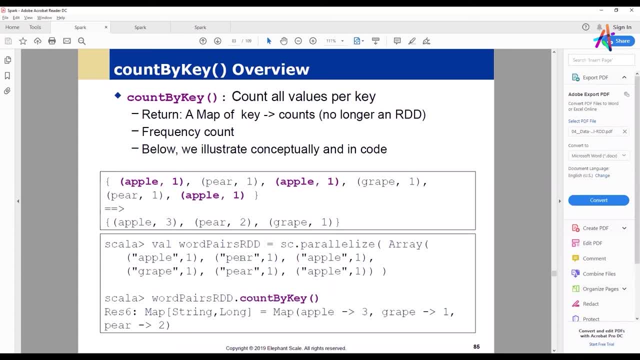 and we're doing a count by key. So we've got the fruit and and some some value of parallel, parallelizing it, And we wind up getting a a map of, of, of, of strings and longs, which is obviously not an RDD. 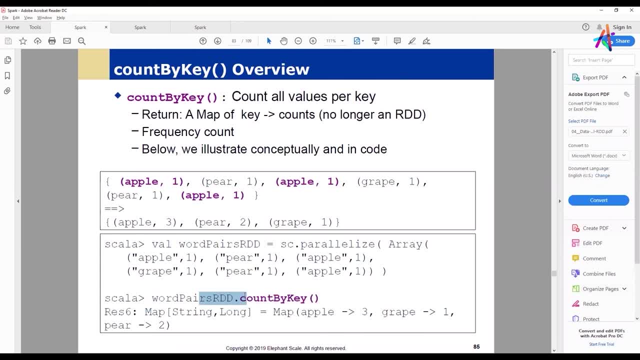 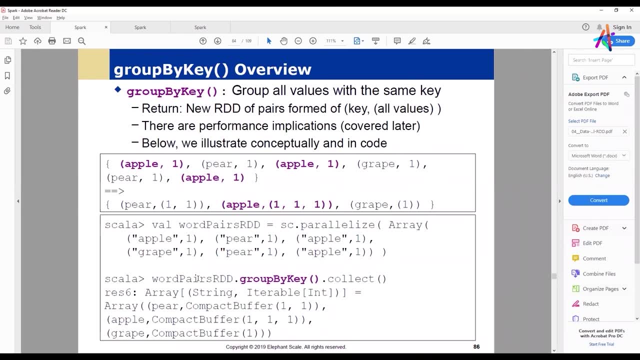 So this is definitively, this is going to be considered to be an action. Remember, the thing that distinguishes an action from a transformation is that transformations on an RDD produce another RDD Actions produce some other kind of data structure, which is really the termination. 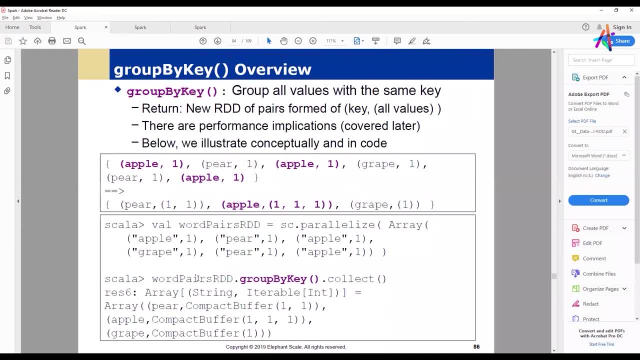 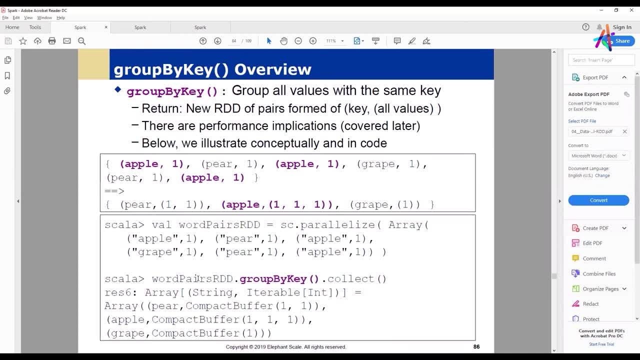 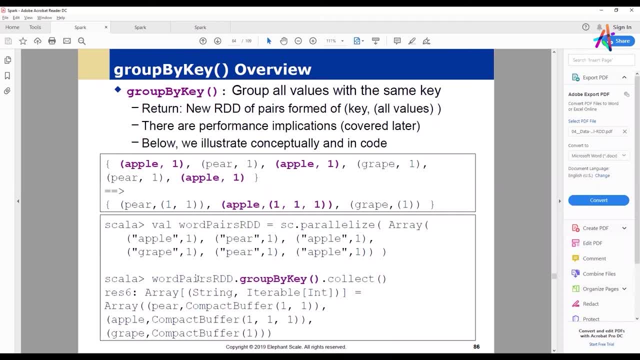 There are some significant savings we can get if we structure our grouping operations appropriately When we'll. this is one of the topics we will be delving into uh in more detail later on. so here's, in our example, we have a our um, our, our, our pairs, again our pairs, our, our pairs, um. i was looking at this one and saying that could. 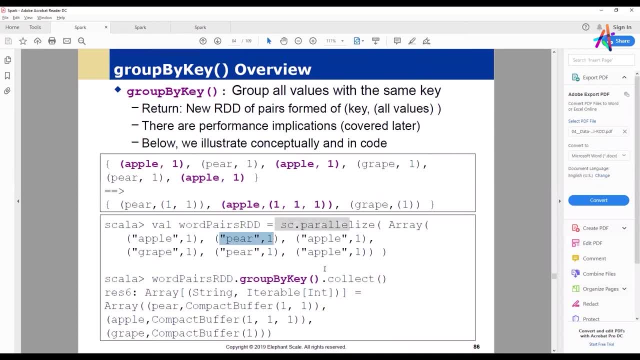 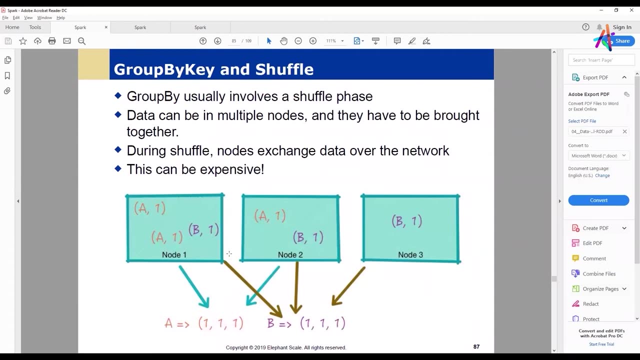 sound confusing, but we've got our pairs and the grouping by key collects them into again a an array of strings and iterables, but again, because this is not an rdd, this again is becomes- uh, becomes an action: the group by key. and this is where we start to look at the underlying issues. 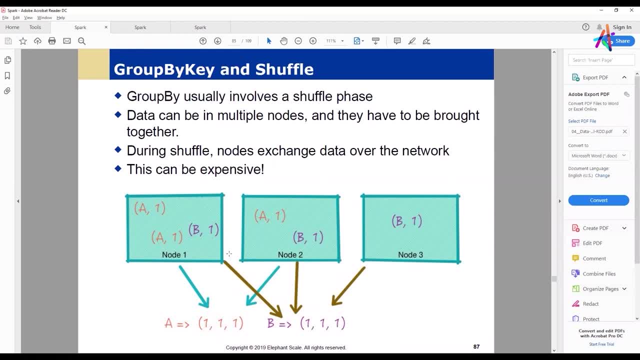 that we have with the, with the efficiency, is that because we've got this data distributed on the nodes, a group by key usually involves a shuffle phase, which means we're going to have to reorganize the data in order to get the grouping, because that data 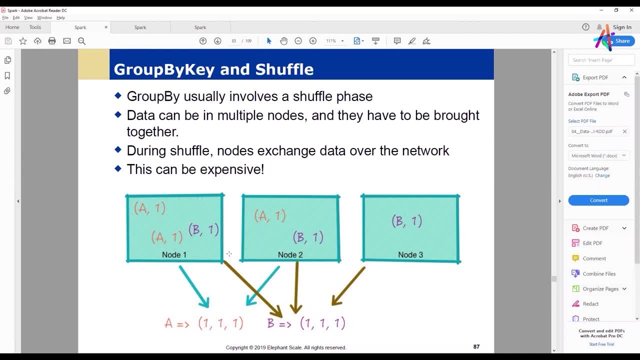 may be distributed and that's where we start to get a performance hit. so we're going to address this kind of issue as we go forward. but at this point it conceptually should be clear that when we start grouping data, we have no guarantee where that data is going to be. so we can assume. 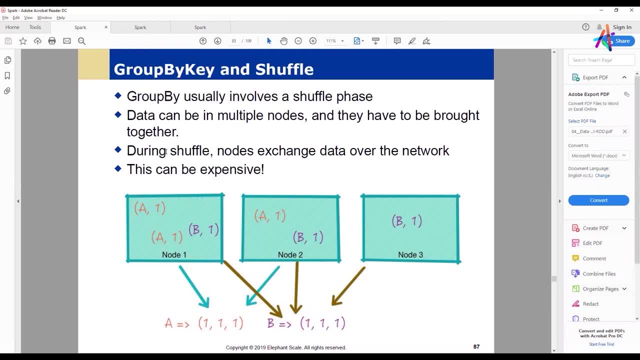 generally it's going to be random, and if it's randomly distributed then it's almost definitely going to be some form of shuffle going on. remember what shuffling is? the process of reorganizing the data on the nodes. uh, and that becomes expensive because we've now got network i o that that we have to invoke as 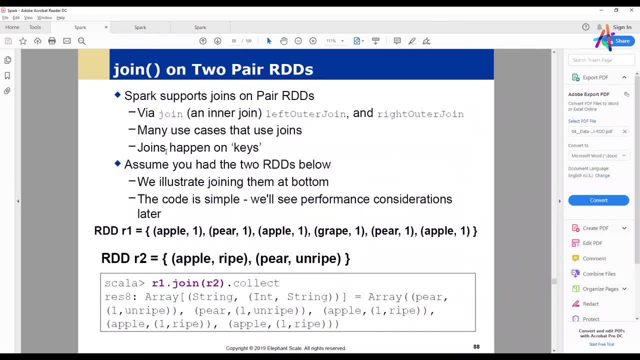 overhead. the other thing that we have, as that can be very expensive, is the use of joins uh. so we can now with our pairs, uh have uh, have a talk meaningfully about the concept of joining rdds and the example there is. we have r1, which 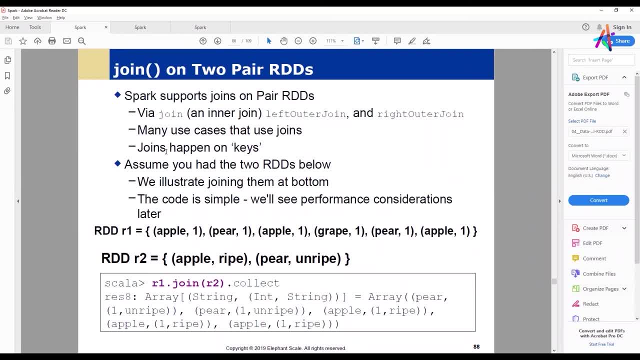 is a group of pairs, r2 is a group of pairs and we can join on the uh, on the uh, on the on the uh, the key value, okay, so that is is another example. um, but again it has uh optimization implications because there's going to be performance issues depending on how that data is distributed. 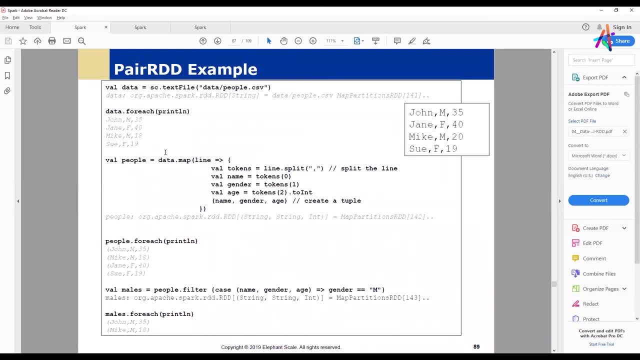 so we can see there's going to be a fairly significant example or fairly significant issues coming up. so here's the example that we had: uh, and this is: this is working strictly from an rdd point of view, uh, where we are imposing structure onto an rdd. the interesting thing, at least i think, is 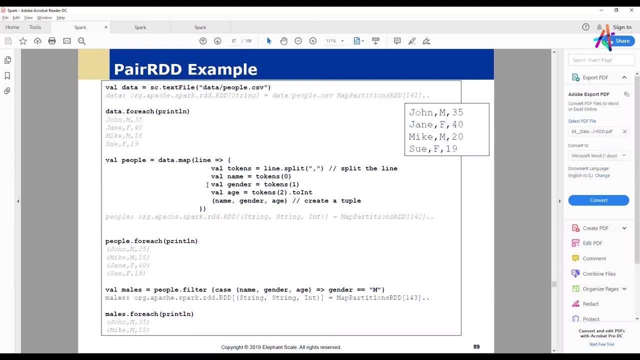 interesting is that, uh, there's there's no underlying spark um spark mechanism that allows us to, to, to, to uh, extract this information. we're doing it manually, but what that means is that if we are imposing structure on this manually, that structure is opaque to um to spark and spark cannot optimize on that. we may be able to optimize for some of the 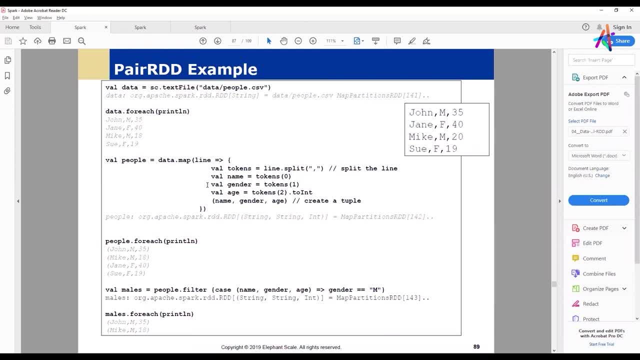 things that we're doing from a logical perspective, but spark does not know about that structure, and so it is not able to optimize the work. it can do the work because we're defining the structure for it, but there's no way that it really has on it that it actually is, and it's already doing the work that we want it to do, and so 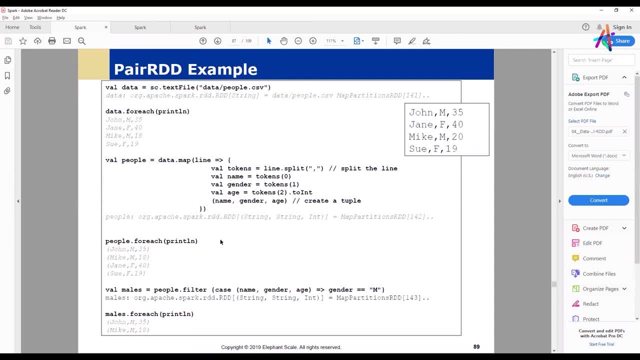 the best way to optimize is to do the work, which is the data frame, and then you can go use the uh to the data frame, which is the uh to the, the data frame, which is the data of the structure. so the data frame is going to basically take this concept of having structure. but now 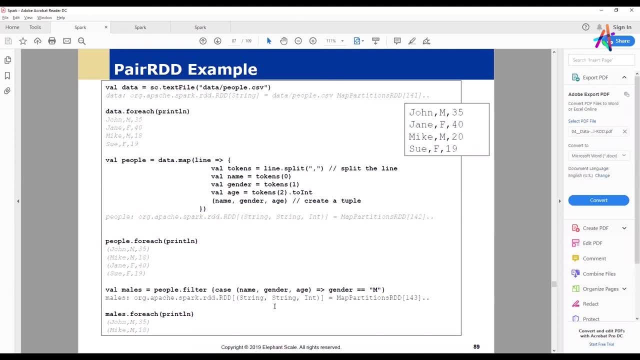 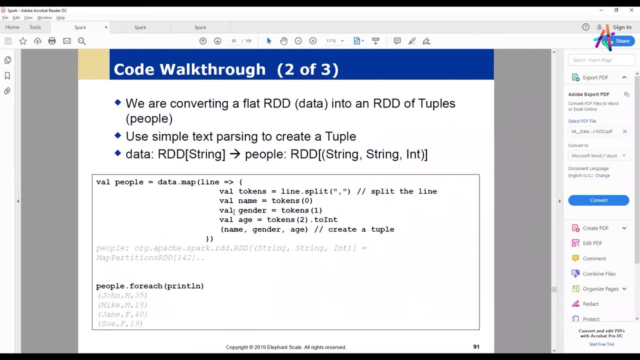 making spark aware of what that structure is so it can optimize, particularly with catalyst, the, the, the operations that are being done. so there's no way here that spark from got because it doesn't really know what this structure is. So this is where we hit the limitations of the RDDs And again, this is where we've created, we've 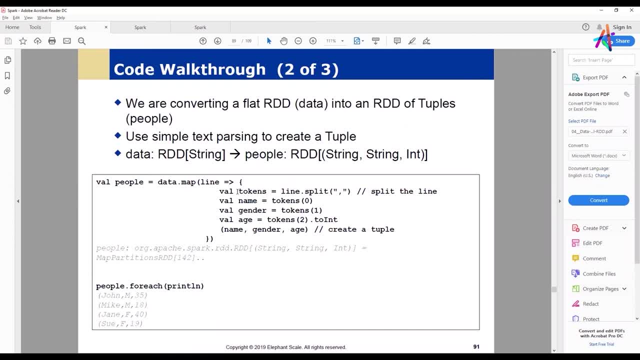 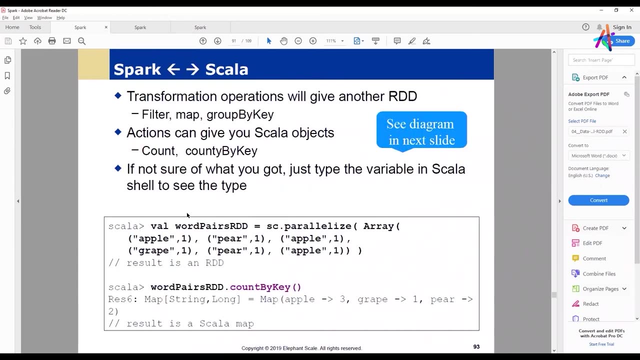 imposed structure on an RDD, but from Spark's point of view, the RDD is still basically a string that we've imposed the structure on, So our structure is not going to be particularly useful. It allows us to do a number of things that we couldn't do before, and we can do this. 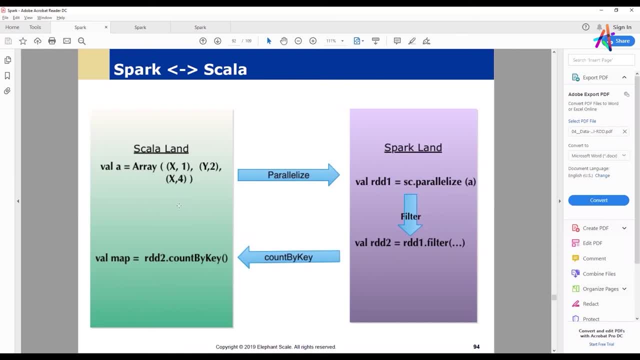 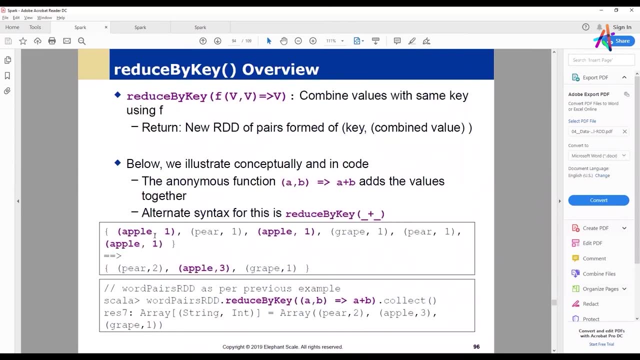 grouping with the pairs, but it's still not really adequate. So the idea here is that this is a better sort of approach. Now, we're not going to do this lab at this particular point, but I will mention just a couple of things, If you. 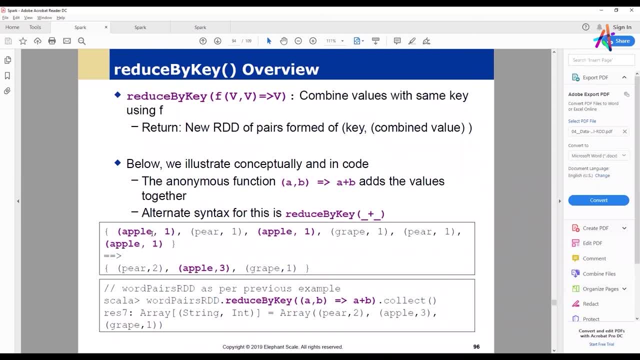 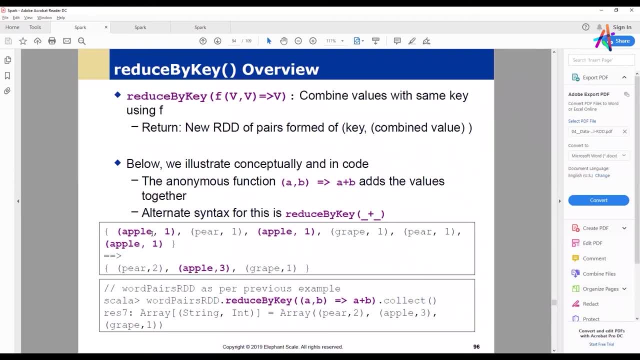 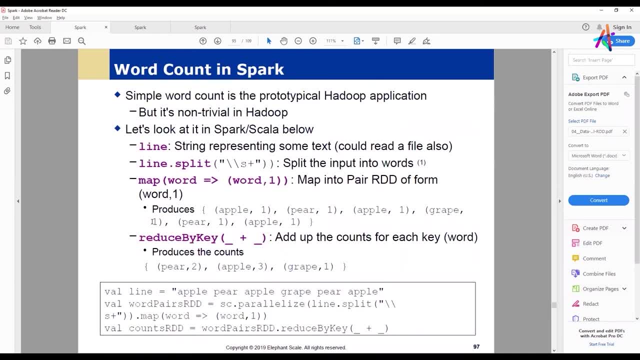 still rather limited on this, so I'm going to just go over the last couple of points here and then we're going to jump over to data first. So we have a just an example of where some of that optimization is taking place in terms of an actual task as opposed to being able. 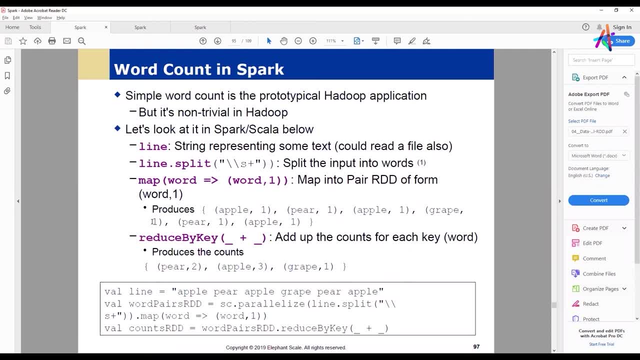 to work with the underlying data. This is just a little example that gives us the word count, The old word count, you know, counting the number of words in a string problem. So we've got a bunch of text, a couple of words, a lot of value. 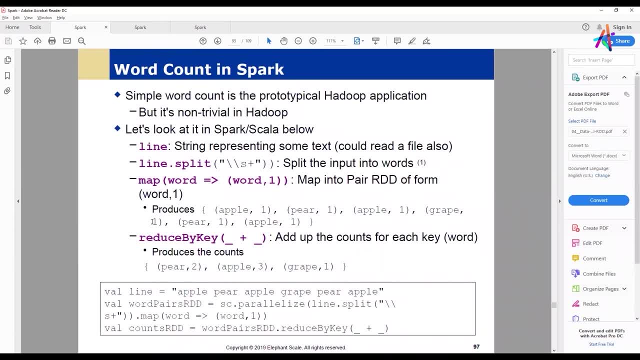 we split it into words and then we map these into count pairs and with an acute with it with the word value and then an accumulator associated with it, and then what we do is we just reduce by key, which goes through and accumulates across each of the keys, all of the values and coalesce and condenses them. 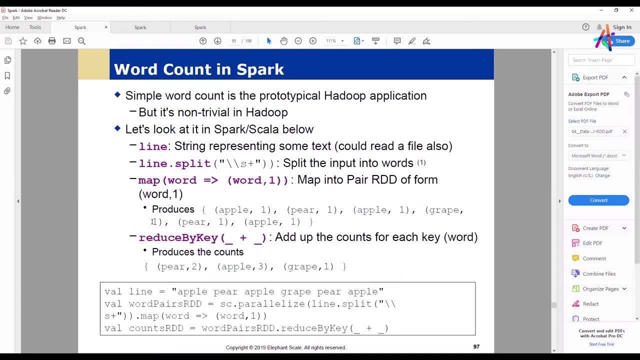 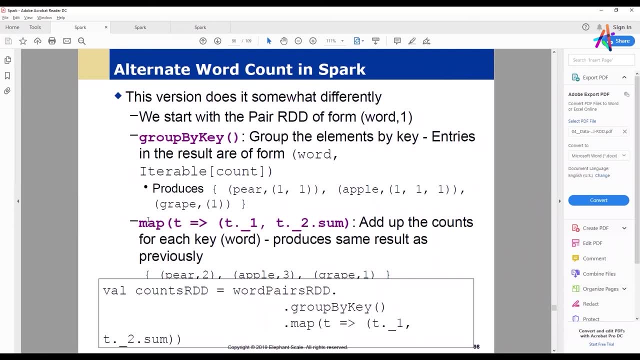 down into a into a final count. now that is, if you stop and you think about it, that is a little bit more efficient than grouping by key. so it was: stop and think about. why is it more efficient? any suggestions as to why a reduced by key wouldn't invoke these same kinds of overheads as a group of by key? 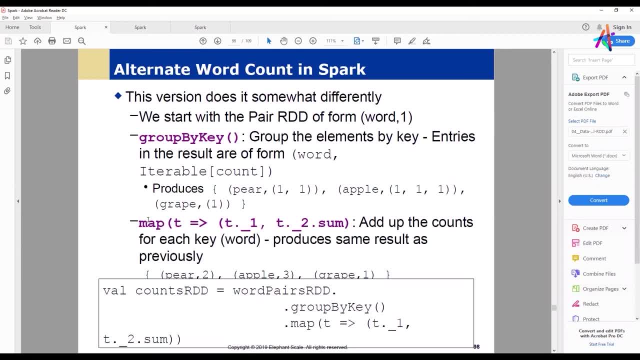 any ideas. well, grouping needs to know all the other right? okay, I think. I think I see where you're going with that and I think you're absolutely right. the partition levels were reduced by key. basically, does the computation on the node where it is, and then and then the driver. 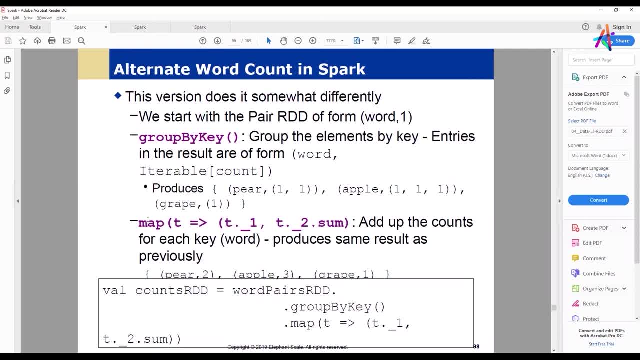 gets the computation and then the driver gets the computation and then the gets the result where group by key is to shuffle, because some driver might not have all the other key, so you have to, kind of like, do a shuffle before being able to do a group by key. that's exactly right. that's exactly right. so it's again. 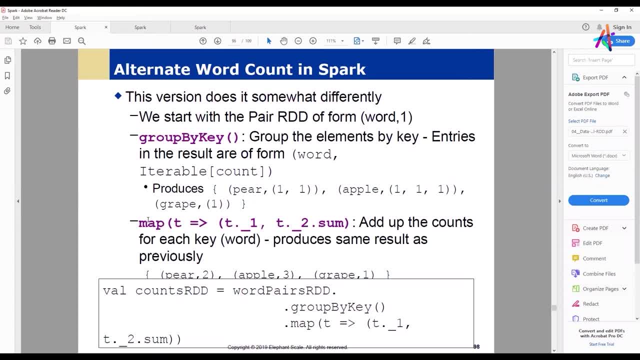 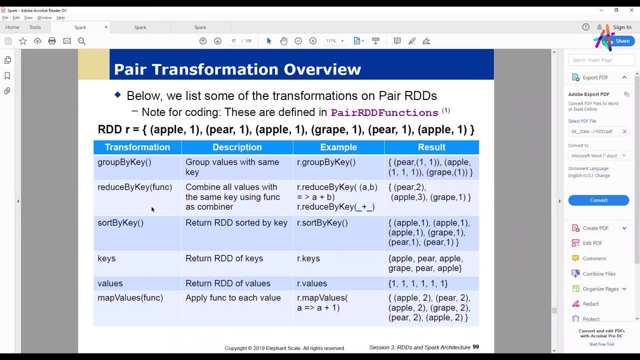 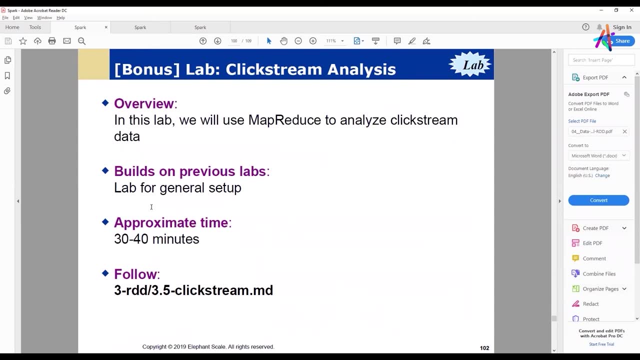 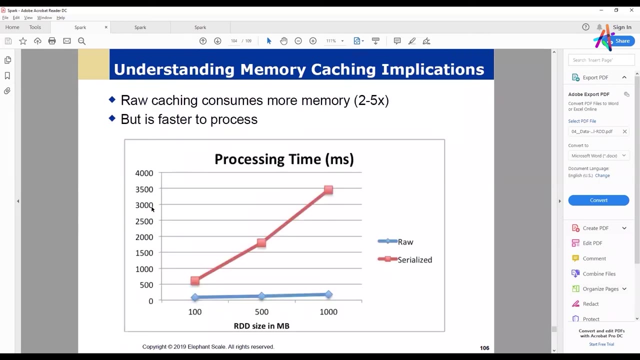 thinking in terms of of the implications on the data shuffling from the node. so so perfect, exactly the right answer. okay, so I'm going to just finish this up a section up, so we get the basic idea and I think we want to. okay, there's this one other thing here I think I want to. okay, there we go. so. 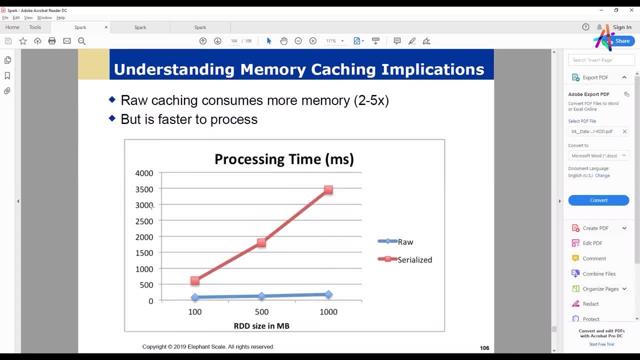 okay, there's this. one other thing here I think I want to. okay, there we go. so there, there's just a couple of things here about the bottom of the manifestation I want to cover before we get to data frames. this first one is this notion of implications of caching. so this is again at the- this is the classic time versus. 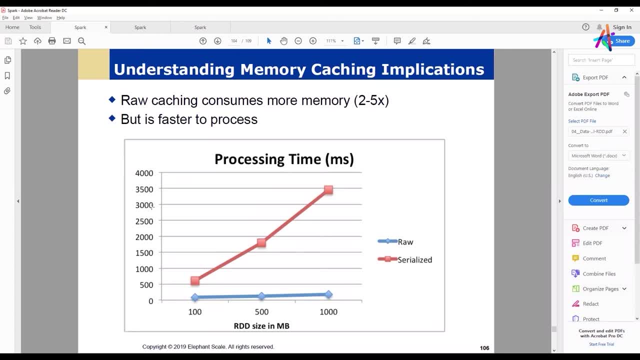 space trade-off. So if we take a look at processing time for serialized data versus raw data- and this is our latency- we'll notice that we get a very, very dramatic difference in performance as we go up in size in terms of processing time. But remember again the trade-off here to get 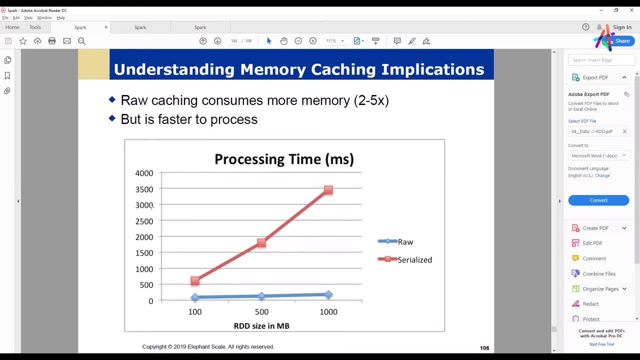 that raw processing time is that factor of using three to five times more memory than the actual RDD. So this is one of the things that we are going to take into consideration later on when we talk about optimizing is what's going to be my trade-off on the use of various kinds of caching. 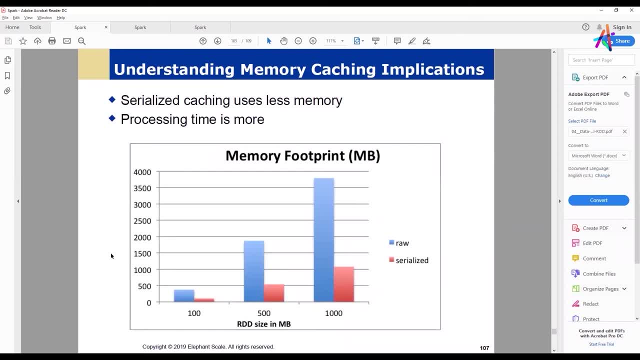 approaches. Here's the other aspect of it is serialized. caching uses less memory, but the processing time, So my RDD size in megabytes and then the memory footprint, which is the amount of memory actually being used in order to store that RDD as a function of size. And so there's our classic 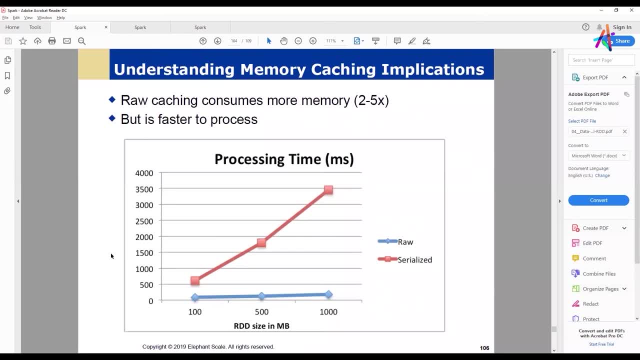 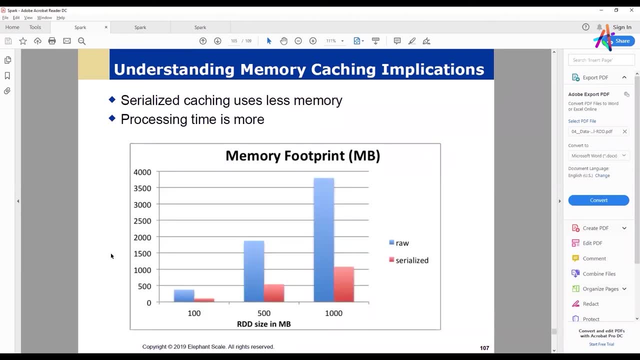 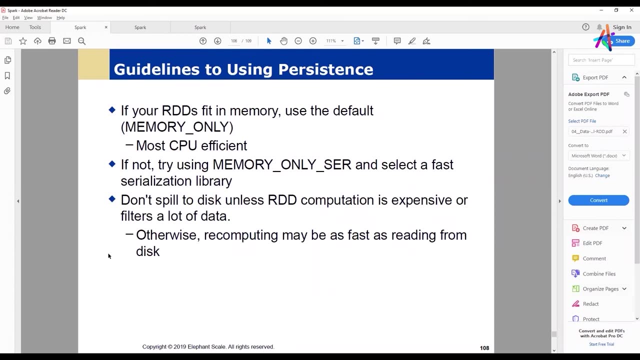 dilemma right there is that serializing data gives us slower access time but it takes up more memory footprint. I guess that's basically what we wanted to just really emphasize there. So a couple of guidelines. The first is that if your RDD is fit in memory, then just use the memory. only It's. 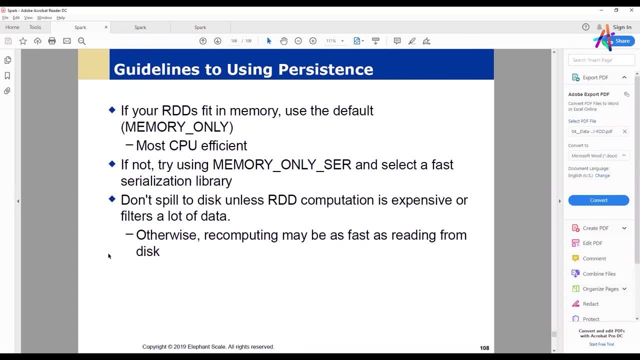 the most efficient of the techniques And if not, use the serialization. But then we have to choose, for our optimization, a fast serialization library. So things like the one we were looking at the other day. Yeah, Brian, I'm sorry. Okay. 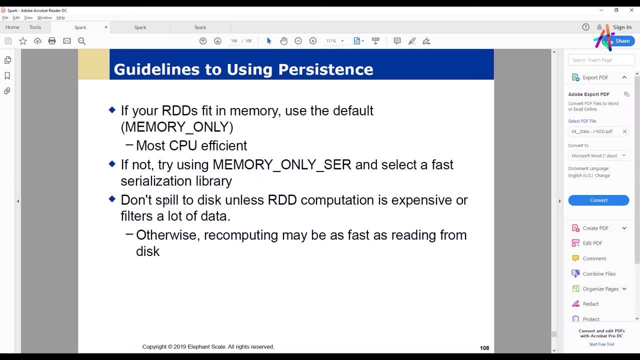 I thought you were thinking about the serialization library you were mentioning recently. You didn't find the name, or did I miss something? Yeah, it's Tachyon. I think I start to lose track of all these different names after a while. 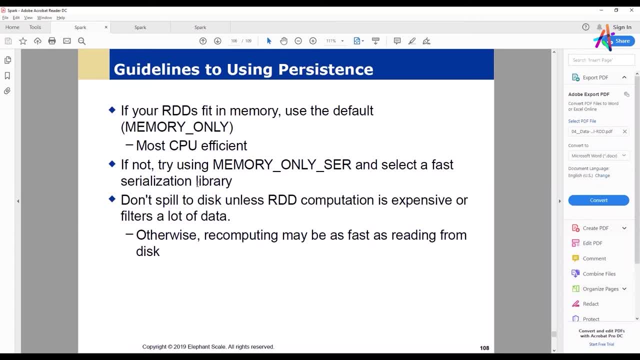 Yeah, but there's a number of different serialization libraries that we can use Java serialization generally. I don't think anybody really seriously considers just using standard Java serialization anymore, not with the availability of the other, more rapid serialization libraries and efficient ones. The term spilling to disk is 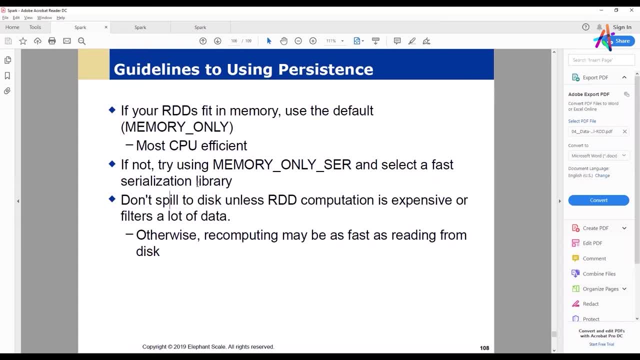 the idea that it is basically paging out the memory. So we want to try and avoid that as much as we can, And so the yeah, but if we have a situation where we're going to start imposing lots of of disk IO, it may actually be faster to. 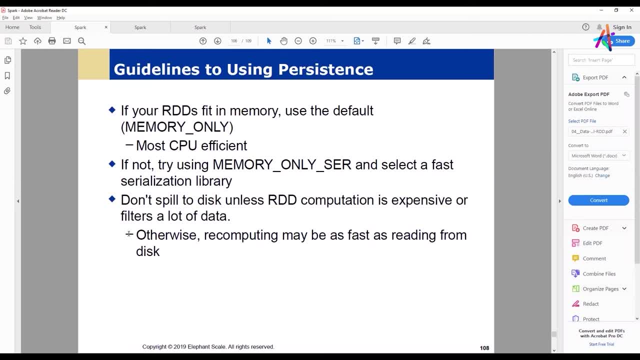 recompute. Any suggestions why It might be faster to recompute? Why would it be faster to recompute than going out? Because maybe you already have the source date in memory. Exactly Because very often it may be a lot faster to recompute because we're going to be just working with memory alone, okay, as opposed to disk IO. 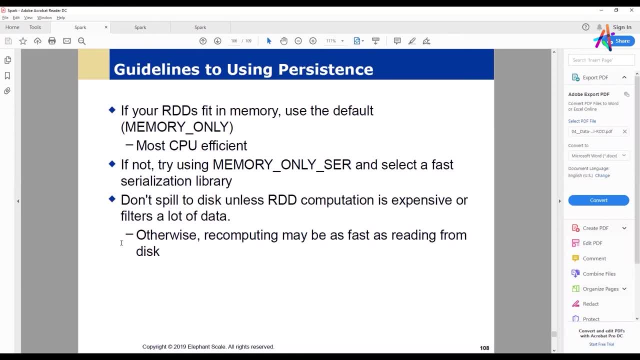 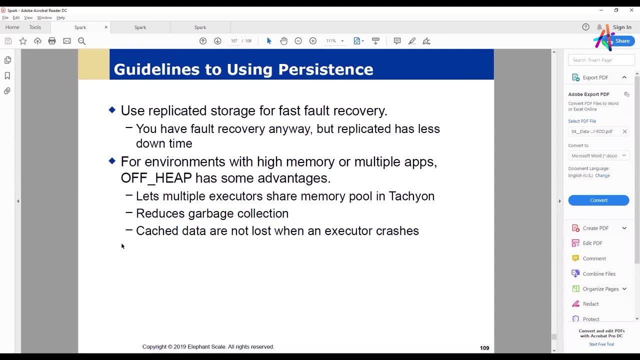 So recomputation, if it's all done in memory, is going to wind up being faster. Replicated storage for fast fault recovery- That's what we looked at when we had that multiple node storage recovery. Remember the notion of off heap is where we've got a tachyon. 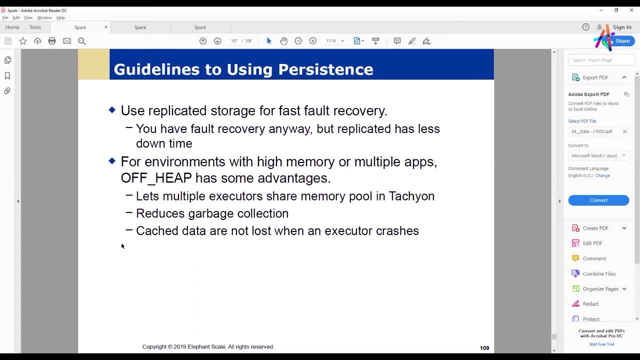 That was right. Okay, So we have multiple executors sharing a memory pool. This will be one of the themes we see when we get into Tungsten. is that optimization is efficient because we bypass all of the nice safe sandbox memory management facilities and work with the bare metal, essentially on our own. 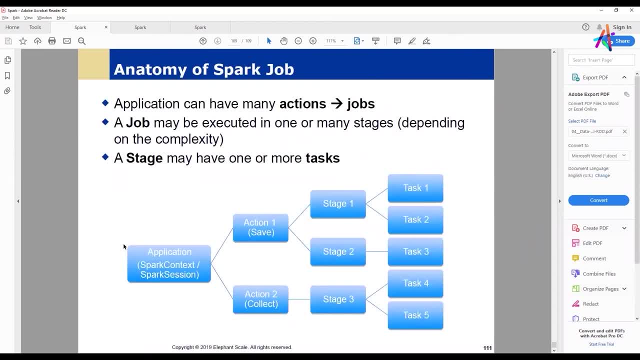 So the idea is we're about to go into review questions. We'll just do a A couple of. We've already got that, So just remember again as we go forward what this stuff is. We have a spark session, which has a number of actions. 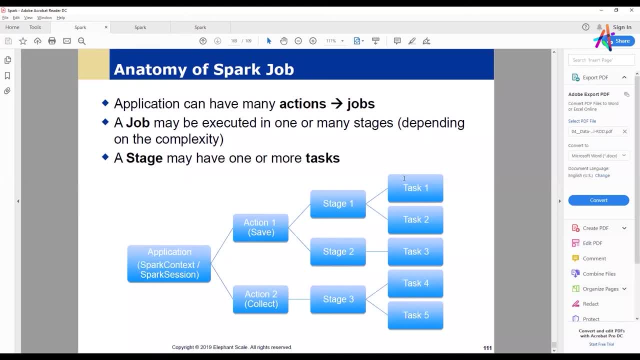 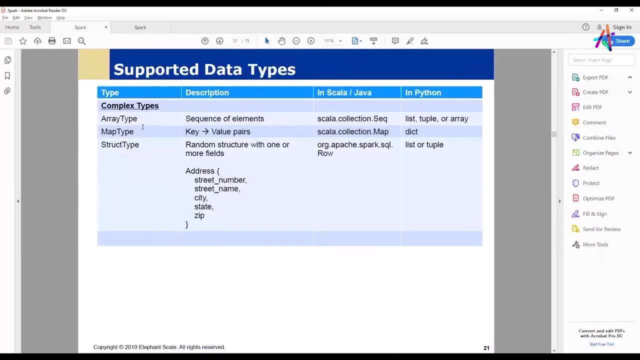 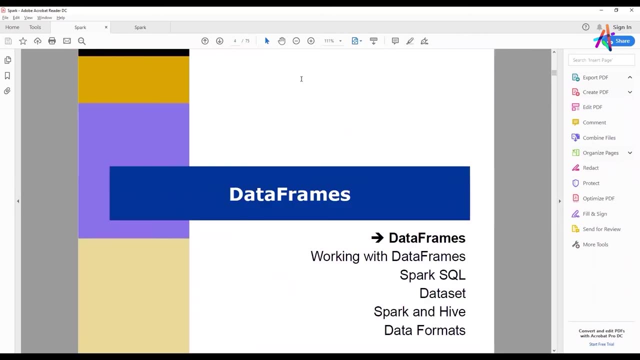 Actions are then broken down into stages, and these are then mapped out into tasks on the nodes. Just a reminder of some terminology: Okay, Okay, So now we're going to jump into data frames. Okay, So this is the model that we've looked at already before. 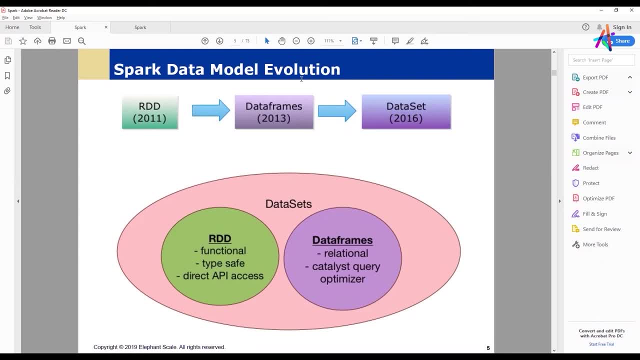 RDDs we've just gone through, And the advantage to data frames is that they are relational, so they fit very nicely with a lot of the data that we're already working with, And the big advantage we have is that we have this catalyst query optimizer. 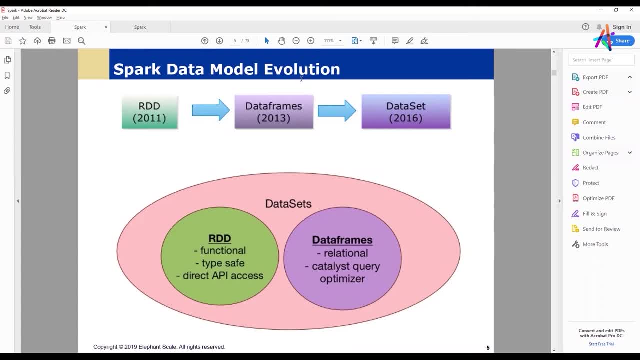 which enables us to get even better optimizations. And that data set unification is where we started typing the RDDs using type data And that allowed us to integrate a lot of more useful optimizations, both from a memory perspective and a performance perspective. And then the spark object gives us a unified interface to both of these underlying concepts. 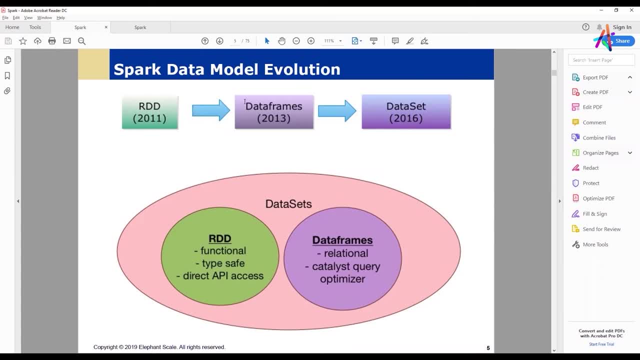 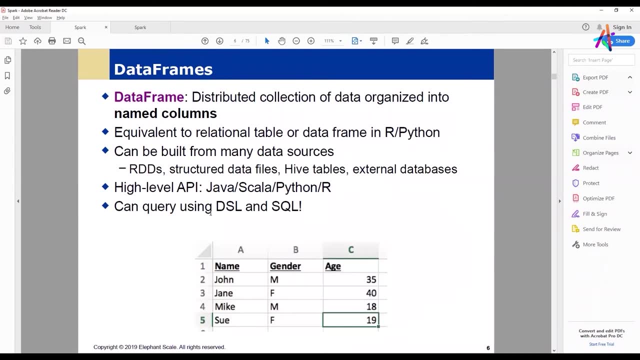 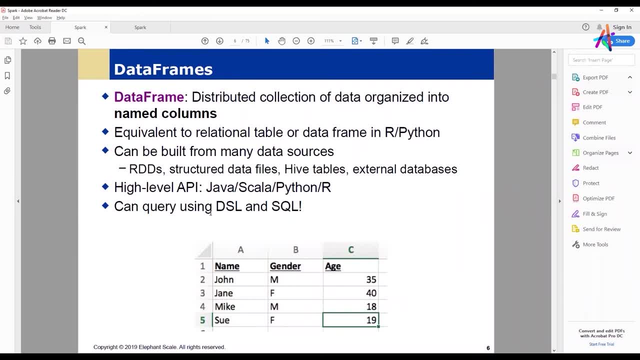 And we can build these from various kinds of data sources which also have some kind of structure imposed on them. We can build a data frame from RDD Using PEARS. we kind of saw a primitive form of doing that: Structured data files, hive tables, external databases. 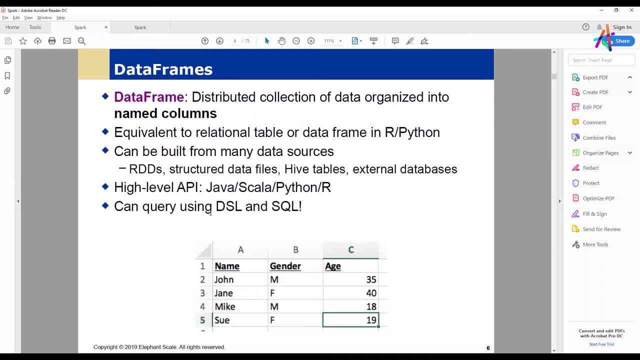 I think the issue for a lot of people is that this is so ubiquitous now in terms of structuring data that thinking in terms of a table does not impose any really undue constraint on our problem. So we can actually now start thinking in terms of querying using a data selection language and SQL. 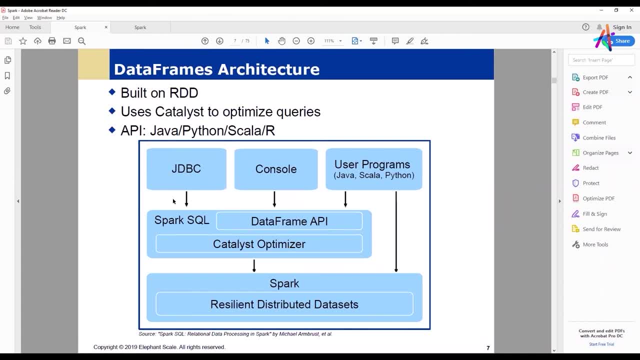 So the underlying architecture looks more like this. So we have RDDs, So the RDDs are still accessible to us. So using my Scala, I can still work directly with RDDs, But I can also work with the data frame API and the SQL query language. But where we get the performance is then we add this catalyst. 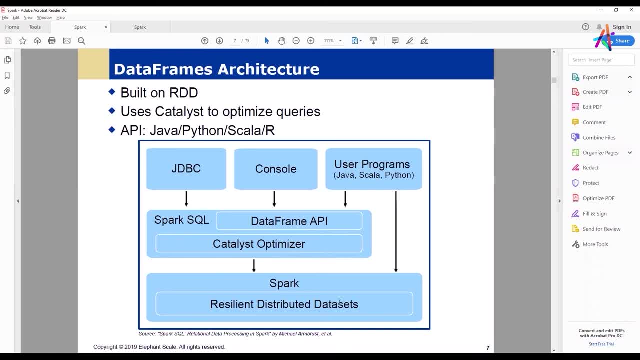 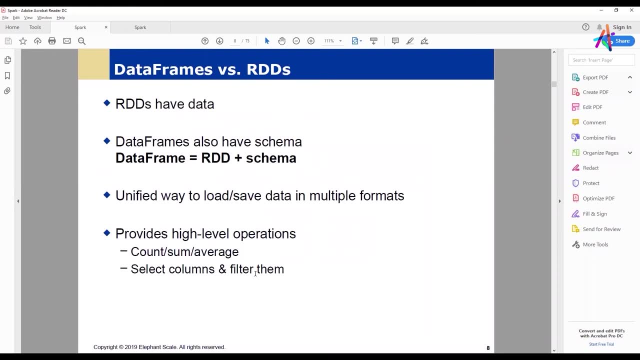 optimizer layer in here which we aren't able to access on our basic RDDs. So RDDs have the data, the schema, Data frames have data plus a scheme. So this is the way to think about. A data frame is RDD plus schema And, like we said, we are doing that. I started off a little demonstration where 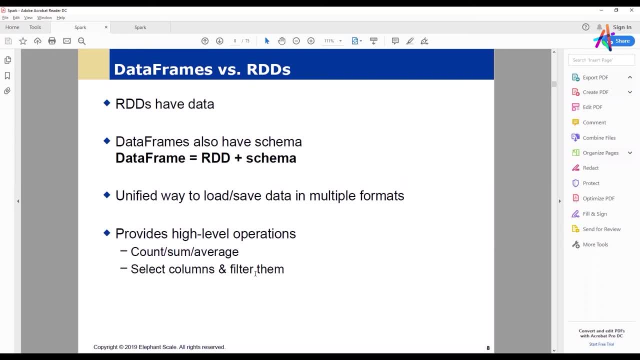 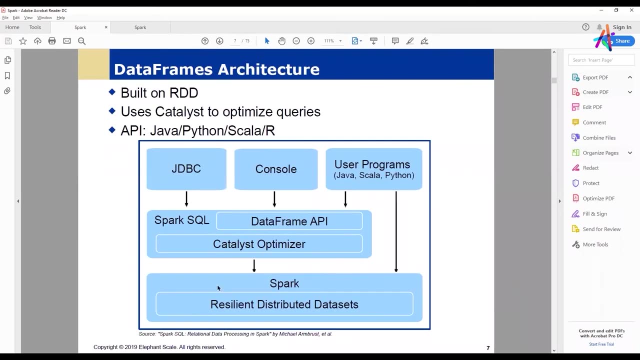 we had imposed a schema on the RDD but there was no way for Spark to know what that schema was other than our own code. So Spark was kind of blind on the manipulation. If you go back to this diagram here, And when we were looking at that pairs of data and the pair operations we were 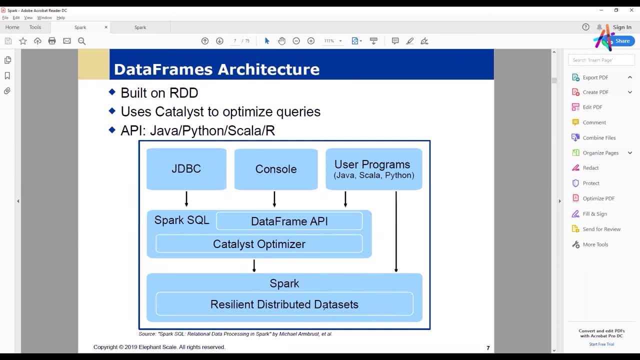 still operating down here. So that was not an acceptable approach from an optimization point of view because the structure was not known to Spark. So this introducing this layer of the Spark SQL layer and the data frames allows the Spark to become aware of the structure so that it can perform the optimizations. 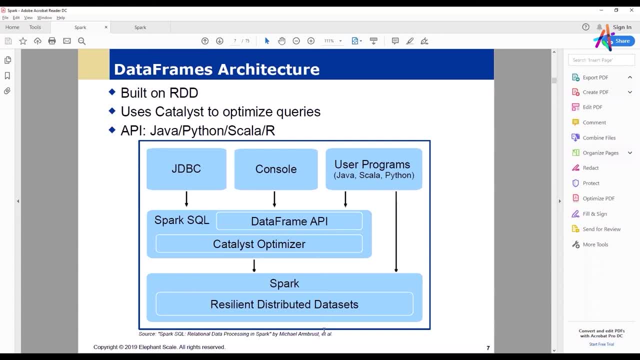 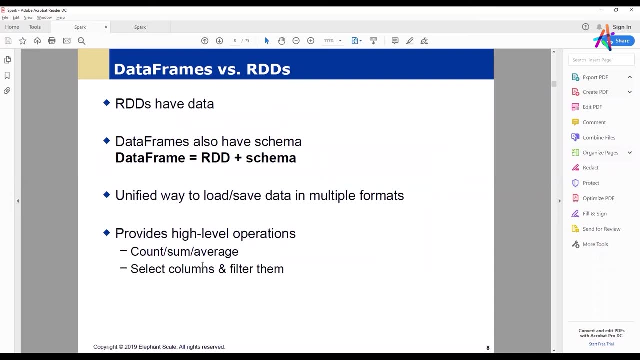 So we're still working with RDDs at the bottom level, but now we're making Spark aware of a structure that it can use to work with the RDDs. So the data frames now have a schema that is knowable by Spark And we now have a unified way. 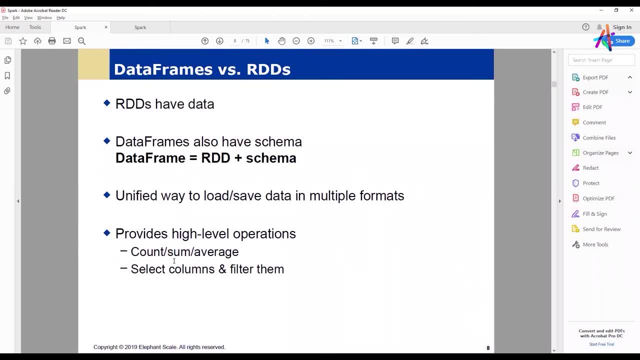 to work with the data And we can have the various kinds of things that would be functionality that would be appropriate from a or not appropriate but consistent with what we're used to in the SQL world And, by the way, that often means. 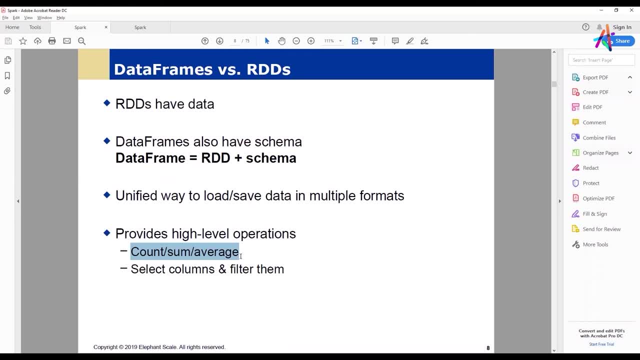 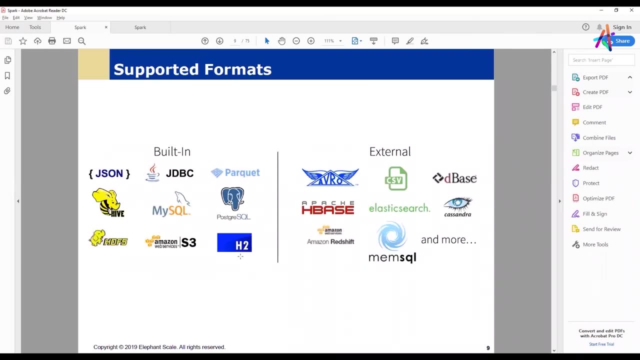 that we have the opportunity to transition a lot of query type logic that we may have somewhere else into Spark without having to modify our logic into managing just the underlying RDD. Okay, So a number of supported formats. So there's a whole variety of formats that are supported. 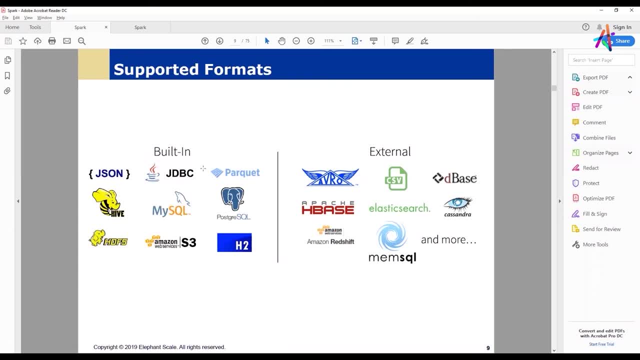 Built-in formats are ones that are supported directly by Spark, and then external ones which can be supported, And I believe those are means that's exported with an add-on And that pretty much covers a lot of the main sorts of kind of tools that we might actually be used. 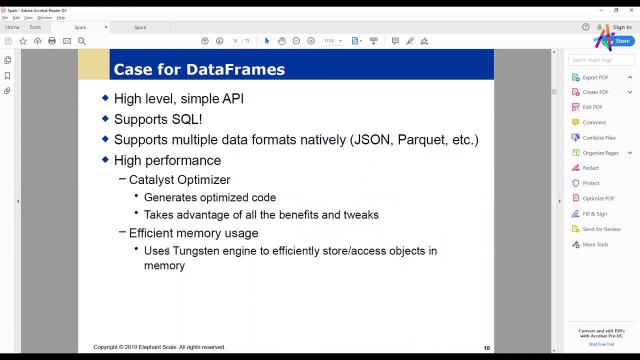 So the case for the data frames is number one. it allows us to access data from multiple sources. We don't have to extract data and then transform it into an RDD for processing. We're able to really import it directly. The high performance catalyst optimizer. 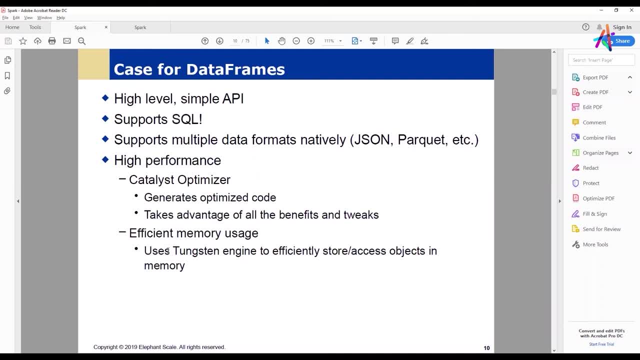 And we'll talk about how that catalog. I think we'll get into that in this lecture, but then we'll come back and look at it in more detail later on. The catalyst optimizer is going to construct similarly to the directed acyclic graphs. 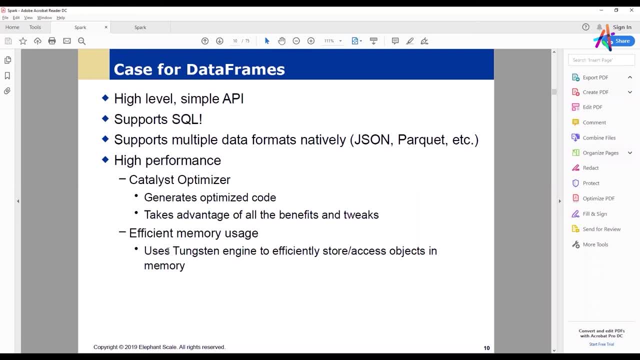 It's going to construct a logical work plan And then from that it's going to generate multiple possibilities for implementation plans and then choose the one that is optimal out of that. So it's actually a pretty interesting approach. I think it's actually 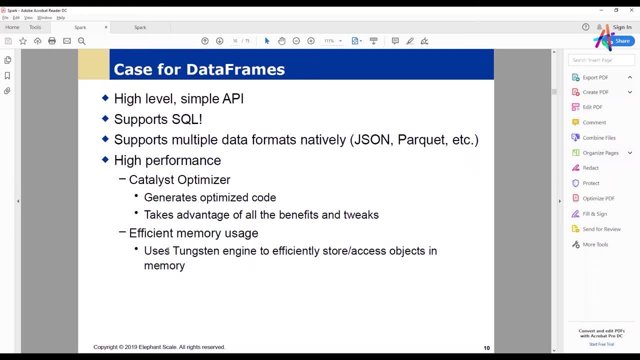 I was listening to a couple of lectures by the guys who invented it And I thought, wow, that's really, somebody really earned their money on that one. That's. it's really a lovely piece of engineering. I absolutely love it. 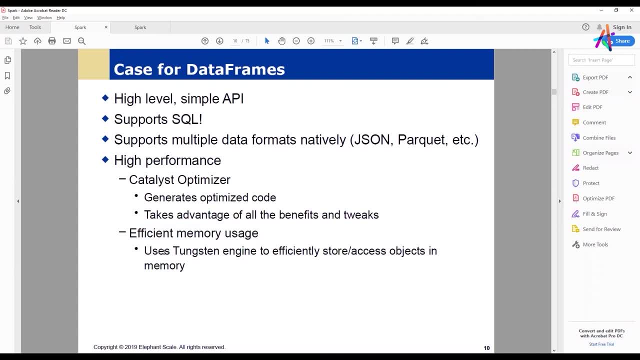 However, because we also have the structure, it also has implications for memory use. So now, instead of thinking of just writing data in kind of big chunks, we're actually thinking of being able to write data at an object At the time, so that structure gives additional things. 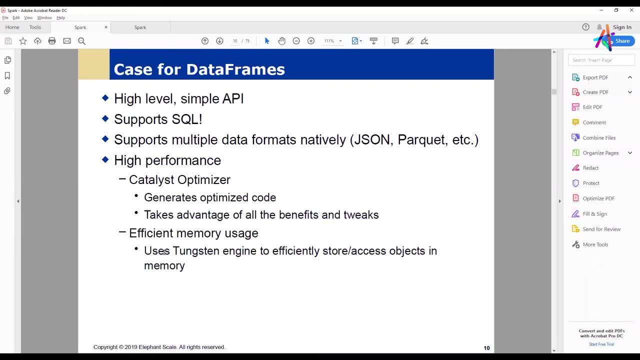 I think somebody noticed that the other day when you were doing random data, you didn't get a whole lot of savings in terms of storage because the data was random. There was no way to actually optimize what was going on there in terms of the compression. 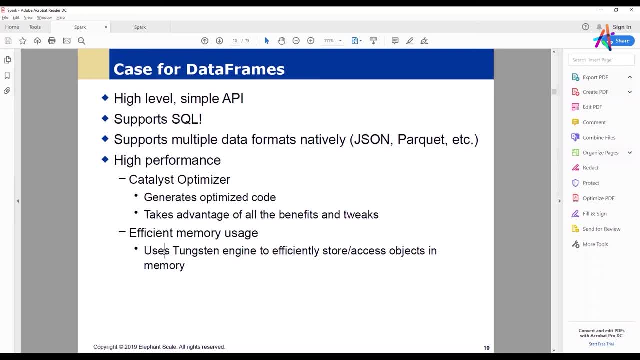 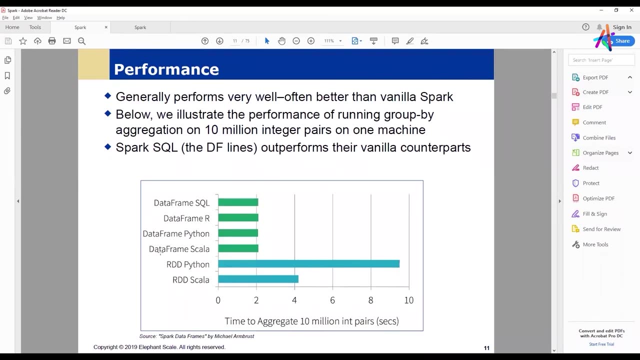 But once we start working with objects, then that gives the memory storage routines, and particularly tungsten, able to some hooks in which they can do a little bit more optimization. this will show up in the. this will show up in the performance numbers. so if we 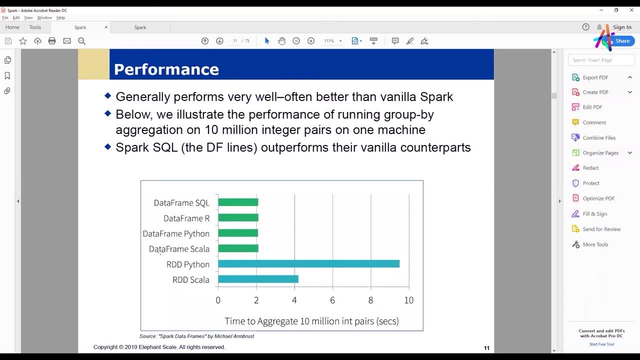 take a look at time to aggregate 10 million into pairs. so even using the pair structure that we had, you know, at the last section, those last two lines down there will only look at the Scala rather than the, the, the rather than the Python. so we're taking four seconds, just over four seconds, to do the integration. 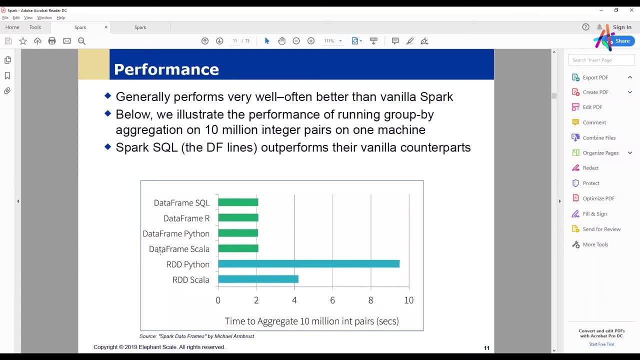 but if the if spark knows about the structure, then you'll notice we've cut our processing time in half. so this is where we get the the advantage from, from giving a scheme, a to spark that it can use. so again we come back to. the idea is that 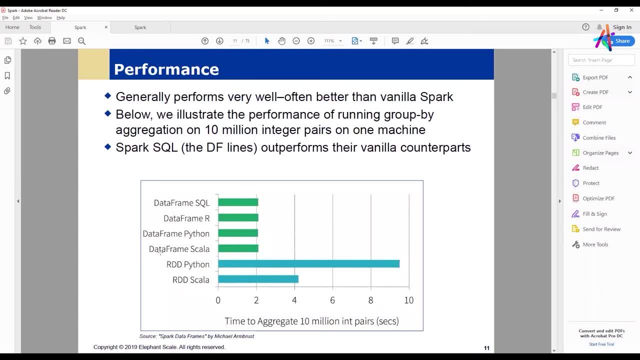 when we did that pair example before we knew the schema spark didn't know the schema spark was unable to take advantage of it. data frames gives spark an opportunity to look at the schema and be able to do optimizations based on the schema. so the- so this is this- was the the primary consideration for really. 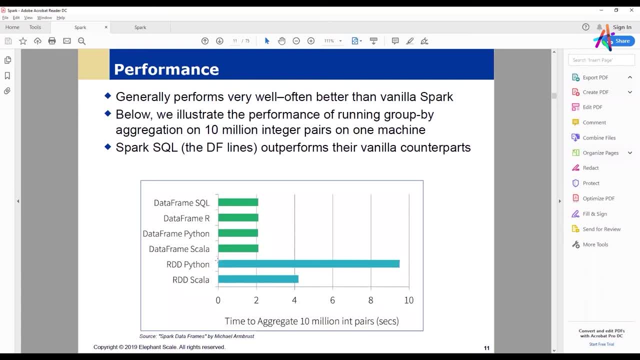 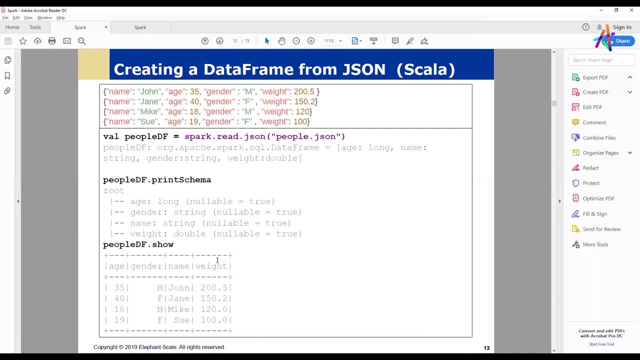 introducing the, the notion of a data frame. okay, so let's work with data frames. data frames can be created from any kind of structured data, so Jason is a perfect example from that we can do a data frame. now what we're seeing is the is the spark object, so we saw SC before. that's been replaced by. 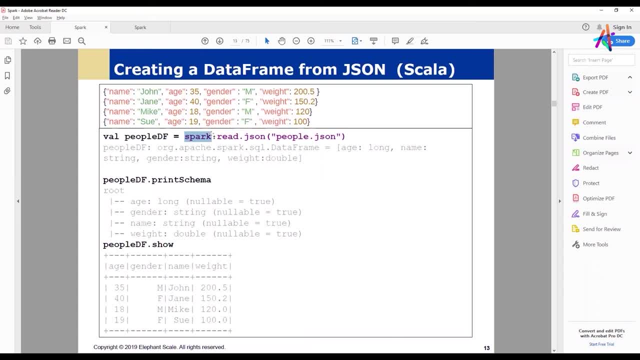 spark. so spark now is is, is the, is the unified interface into the data sets. so, reading a JSON file and we're creating a, a data set from our data frame, from the, from the JSON file and, as you can see, when we actually get the, the, the output. 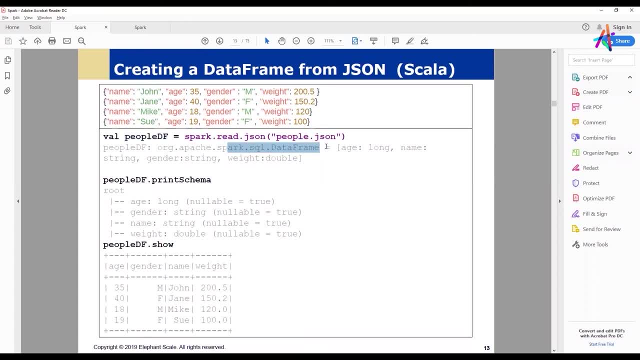 here we get a data frame that's coming out and the data frame has the, the structure. we can print out the schema of the data frame and we can show the data frame in which, in this case, is going to give us a table which looks pretty much like any. 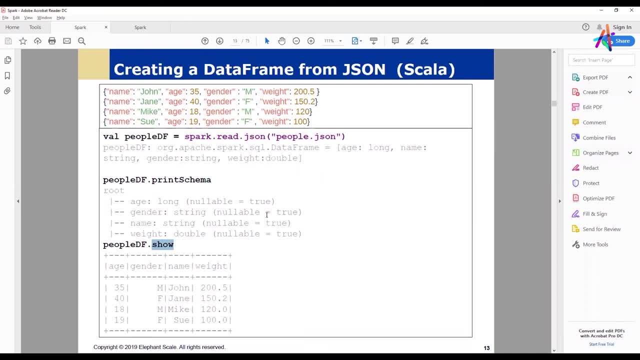 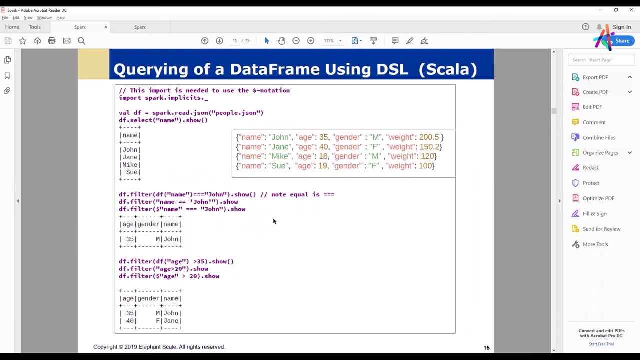 other table we would get in any other kind of relational system or structured system. we're not going to do the Python. there we go. so we can now query and use use queries on the data frame using a DSL. so so we can now query and use use queries on the data frame using a DSL. so we can now query and use use queries on the data frame using a DSL. so 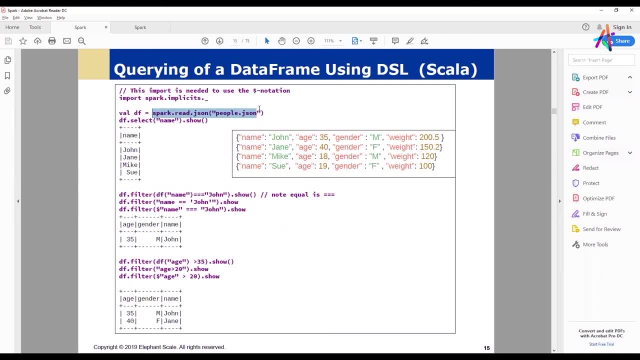 now we've, we've created a our file here and now we can do a select on name and show and show the results. we can filter on the subs. we can. we can filter, do a filter on on the data frame to to pull out all of the the. 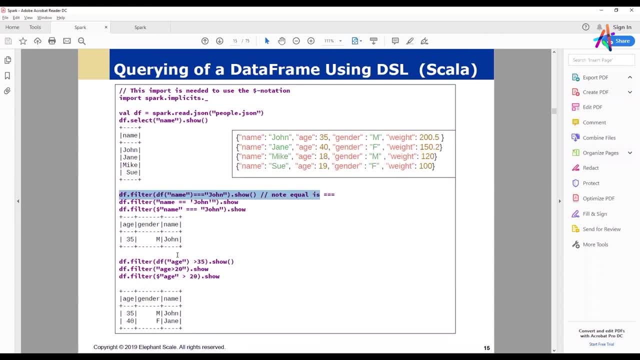 the names that are equal to John, and we can then show the result of the filter as well. so there we comes out, we've got John. so the excuse me just a second here. there we go. a little issue with my mic. there we go, so we can filter out the. 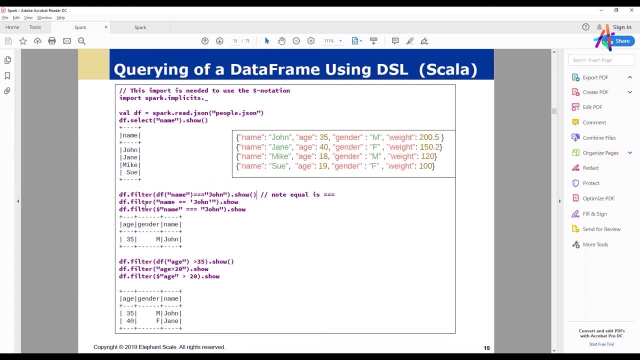 data, set the rows, and we show the, the rows that we filter out, we can filter on, and there's a couple of different syntaxes here, so we can do a variety of different ways of doing this. we we wind up with our result here, so, and we can. 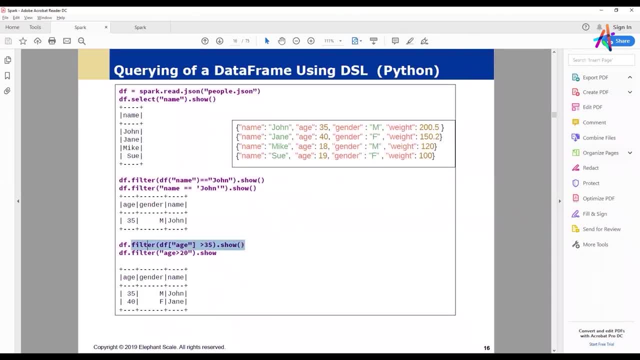 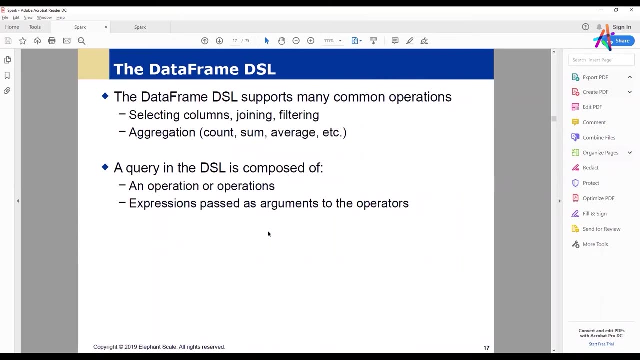 also filter on using other kinds of queries as well. so the idea here is that once we've got that structure, we're able to go and extract data in a variety of different ways. so there's a comment. so we would expect that the the data frames would support. 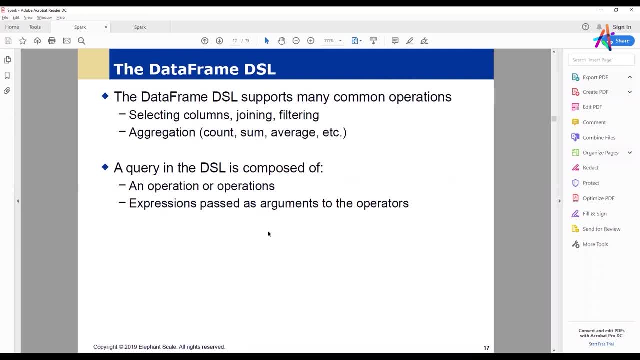 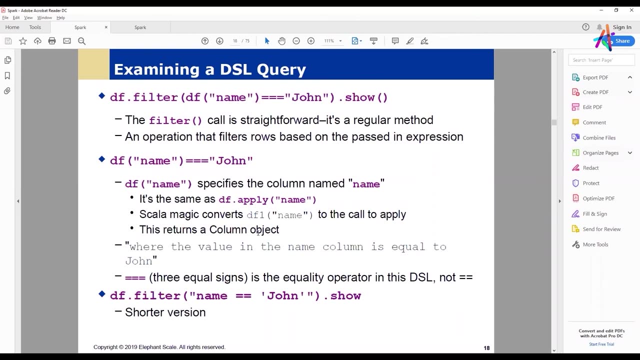 the the kinds of operations with it we used to. so selecting columns, joining aggregation, and a query is composed of the operations and the expressions are passes arguments to the operators. so here's a query. this is is what we were looking at before. so what we're doing is. 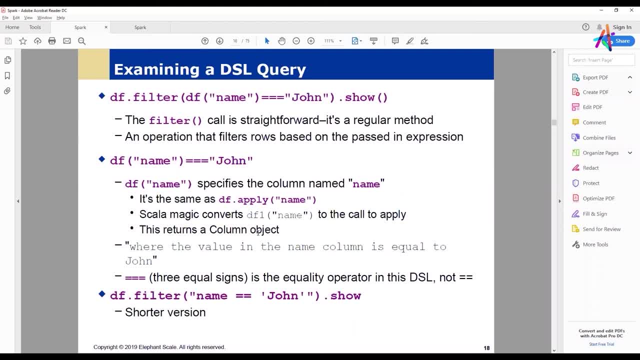 filtering through the, the, the data frame, and we're grabbing every row where the, where the name value is equal to John. so this is again fairly straightforward: the, so the, the DF Dame. it specifies the column and the is and the value, of course John, so the, the, the, this is. this is again the data frame we're. 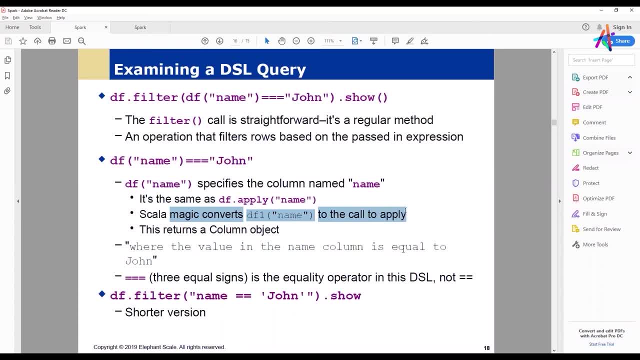 and done so that Hold on here. There we go. Okay, There we go. The connection to my microphone just keeps coming loose, so I don't want to suddenly drop out. So we're looking at again a standard query operation. We get a column object back. So again in plain. 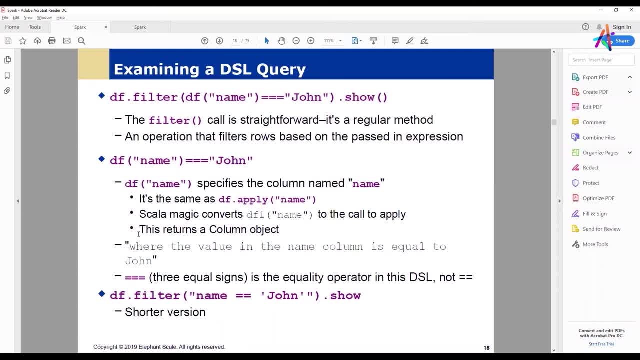 English it's where the value in the column name is equal to John. The triple equal sign is the equality operator, not a double equal. So this is also another syntax that we can use to do this, So we can filter on where name is equal to John, The difference being 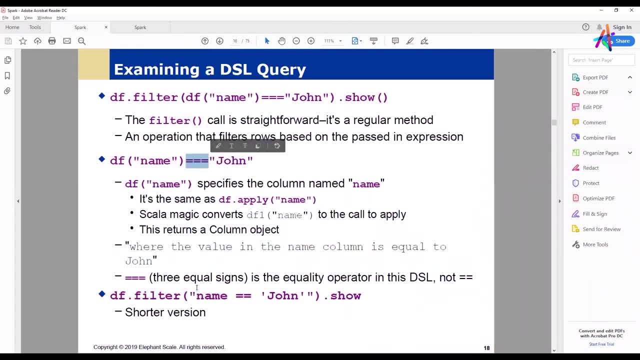 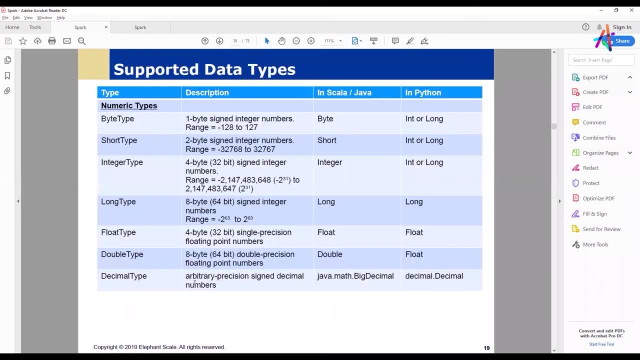 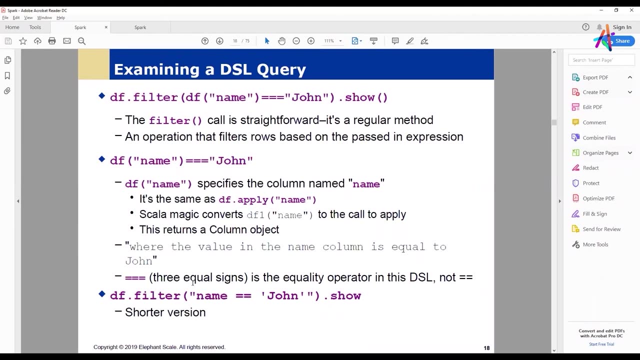 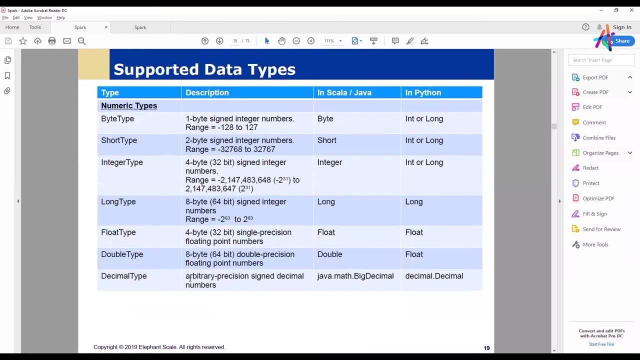 here is that the triple equal sign is used In this format, whereas we're using the double equal sign in the embedded format. So this is the shorter version, but we do also are able to do this in terms of equality, because we now also have the ability to use it with various kinds of type data, And so we've got. 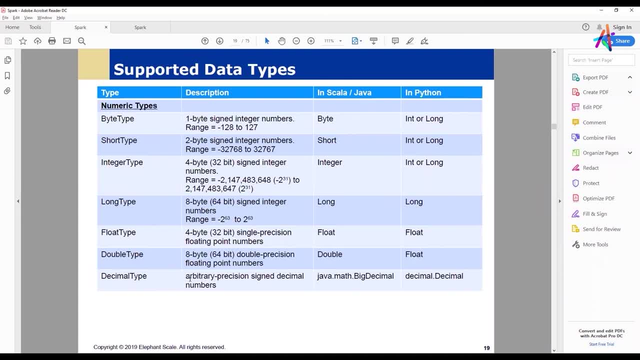 the standard kind of data that we would expect. Of course, we do have integer types, numeric types, long types, float types and double types, and also a large decimal type, which is also there as well. So there are a variety. 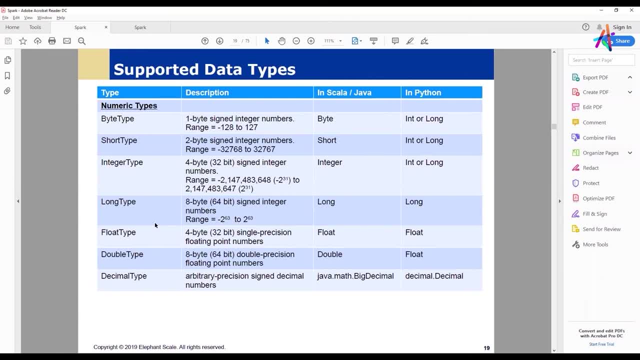 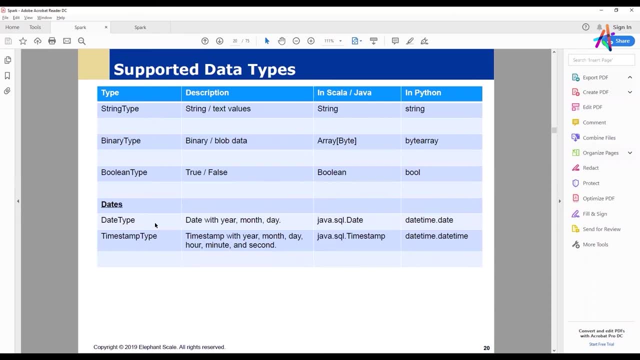 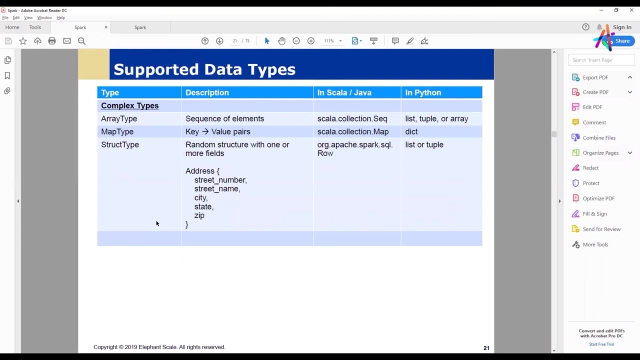 of different supported data types, which Spark is aware of: Strings, binaries, which are blobs, booleans, dates, timestamps- fairly standard, fairly standard stuff. And we also have various kinds of more complex nested structures, arrays, map types- exactly what you would expect. 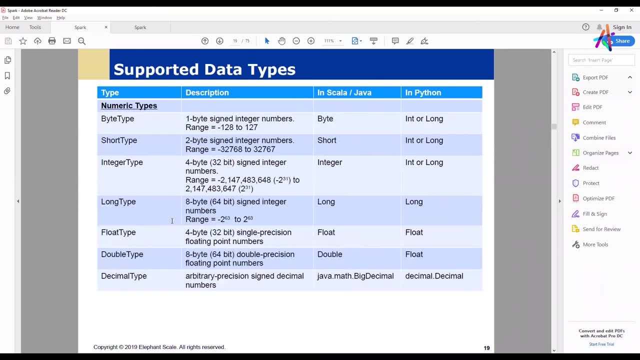 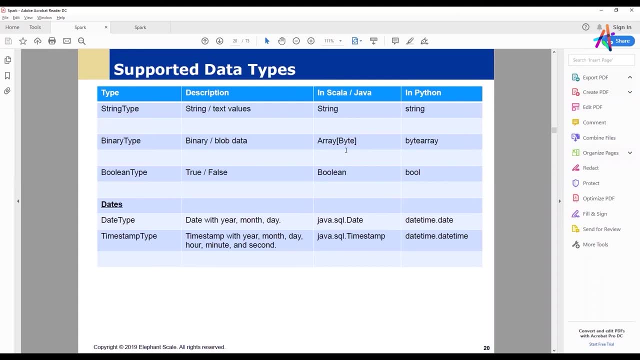 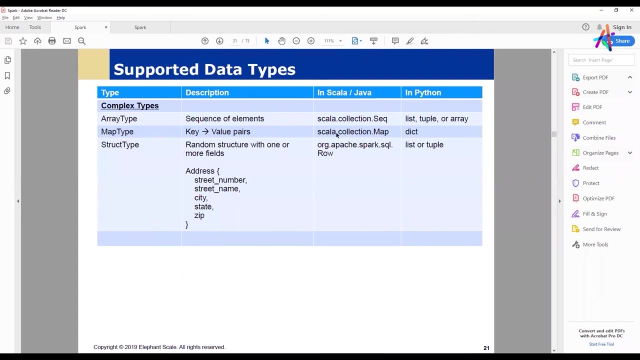 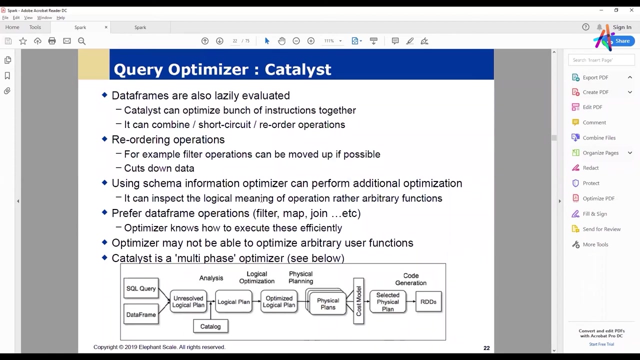 and this, this: these map up to the appropriate or or the the corresponding values in scala and java or in python. so we have arrays. there we go arrays, sequential arrays, map type structures and and general general structures, so the the supported data types. now is a rich is a rich. 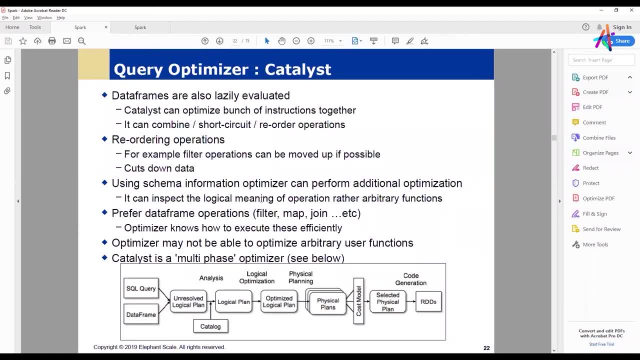 richer set of values than the, or richer set of tools than the original rdd, which was basically untyped. all right, this is where we start to get to the, to the interesting stuff, which is the, the catalyst optimizer. so, using the same idea before, uh, with rdds they were, they were. 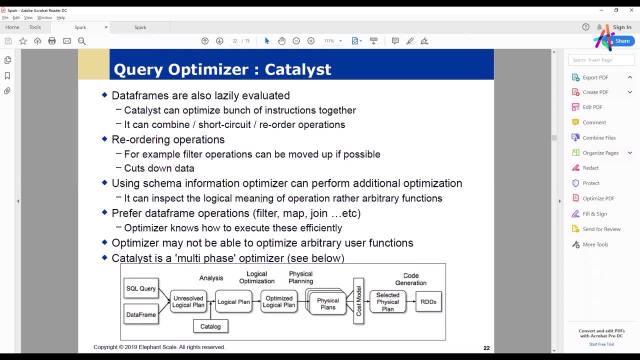 they were processed in a lazy manner, which meant that they weren't actually weren't actually processed until we hit an action. and, in a similar way, catalyst- uh, the catalyst optimizer, is used. uh can be used because data frames are evaluated the same way, so we'll have 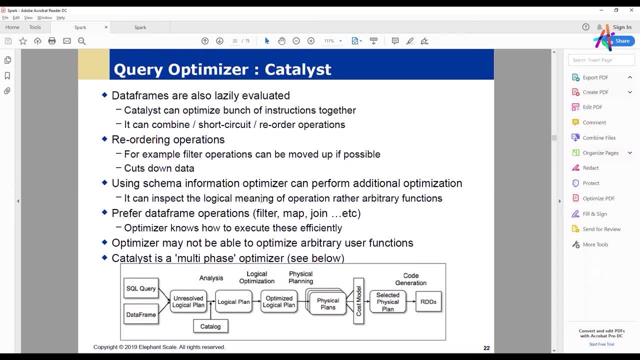 a series of transformations of the data expressed in the various in the dsl and and uh and uh uh that we're going to apply to the data. and then what catalyst does is? uh, optimize those in by looking at various what we call work plans or physical plans. so one of the obvious optimizations it has, 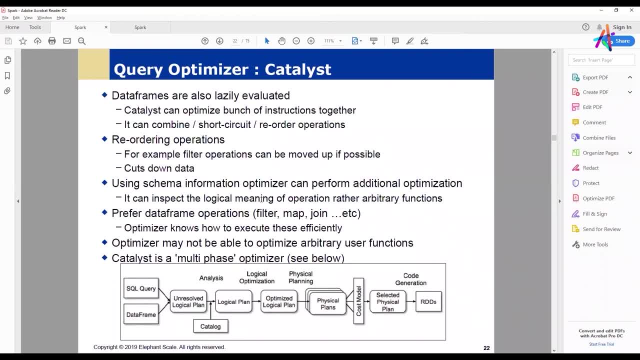 is to look at pushing filter operations up, which means you know the path. um, so it. there's a set of uh, Residential, Sean Hamilton, and also the search engine uh, and then, of course, performance analysis are use gdks to trigger a process of the data, Lat graveyard using the arenab После and through RDD, it filter data differently than filtering later in a sequence of events. it will filter earlier to reduce the amount of data and it does other kinds of optimizations. optimizations like expect the logical meaning of the operated arbitrary functions. that's something you can't do with our dds and it will know how to optimize specific operations like filter, map and join. now we can include, we can do almost anything we want with the data, but the ones that we haven't already covered, we want the use. that- and this is something that is doesn't necessarily it should actually be a trial request, so it's one in between and the main thing that's it should be the filter mapping step by step, but for which architect actually has to be the at this stage where he can ΔB, please the seam. 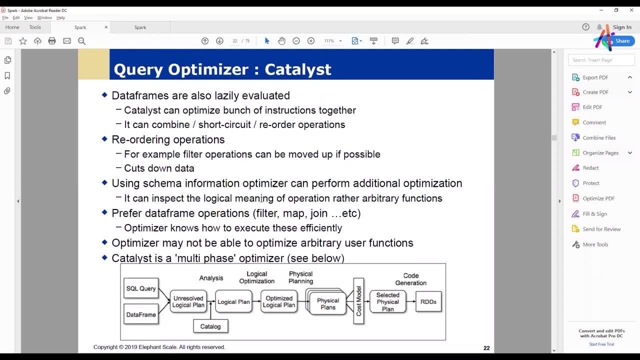 where we're sticking with the data frame operations. those give us the ability to actually let Catalyst do the operation, do the optimization. Okay, optimizer may not be able to optimize arbitrary user functions because it doesn't know how to evaluate the cost of those arbitrary functions. 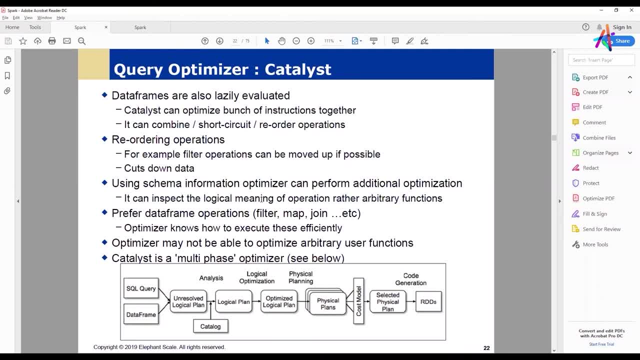 And I think we'll look at ways later on of working with arbitrary functions. But the fundamental idea is that there's a basic set of operations that Catalyst can figure out what the cost of those operations is generally going to be and it can then determine some kind of optimization on those operations. 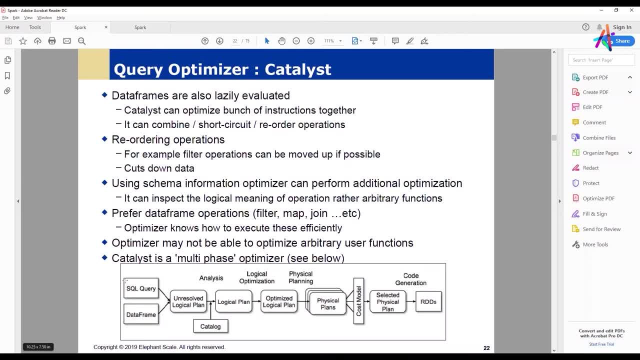 So this is the process that it uses. It takes a query that it's going to optimize and it takes a data frame and it has an unresolved logical. now that unresolved logical plan is basically what you've told it to do. It then goes to the catalog of the data plan. 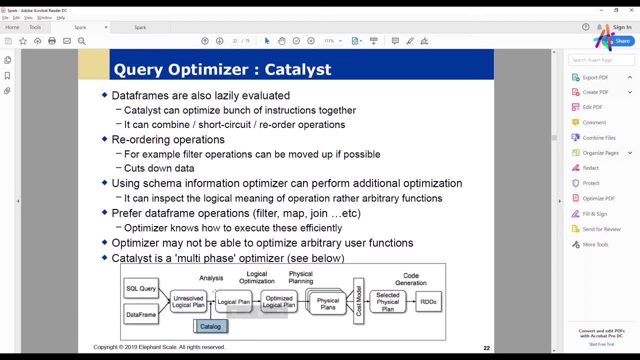 and then converts this and resolves this with all the different references that were made in the query to the logical plan. It then does a logical optimization, which means there are certain optimizations that can be performed on the logic plan, like pushing filters down And from that optimized logical plan. 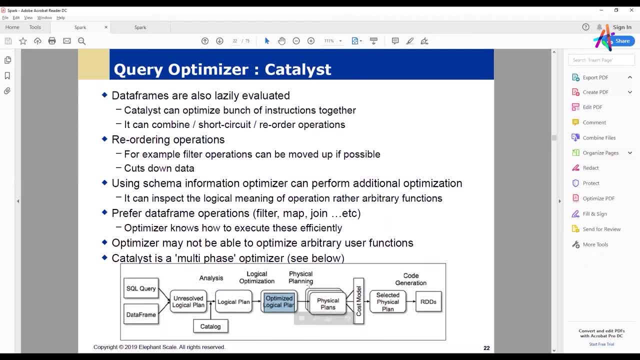 it produces a set of physical plans- I keep using the old term, implementation plans- but these physical plans are then evaluated in terms of the cost of implementing each physical plan. So each physical plan has an associated cost, which then goes through a cost model where we can choose. 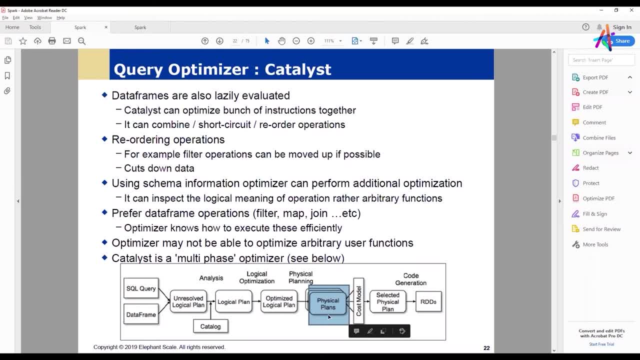 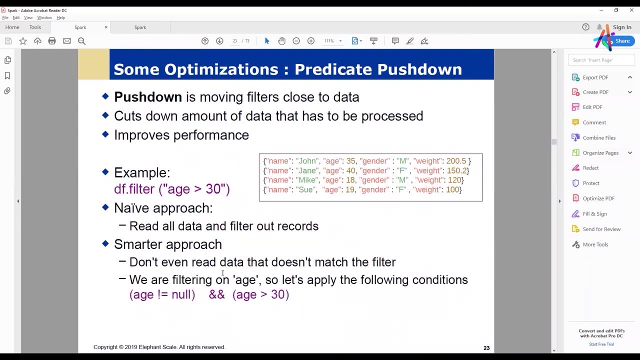 the physical plan that has the lowest cost, And that physical plan is the one that's selected, And then from that we do the generation of the code that produces the final result. Okay, so this is what Catalyst does. Now Catalyst also has some hooks in it. 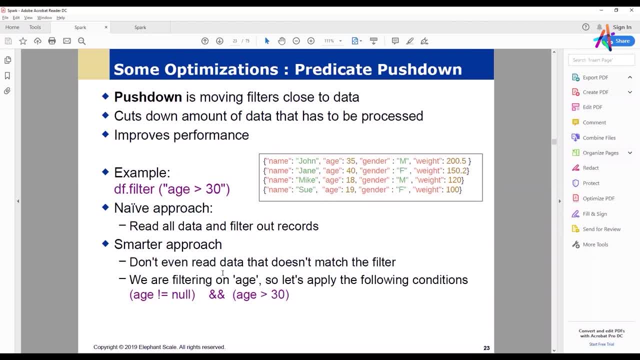 where we can plug in some of our own optimizations, which we will deal with next week. So one of the optimizations that it does is called a pushdown. So what a pushdown does is: Catalyst, looks for specific filters and it goes and does the pushes down the filtering. 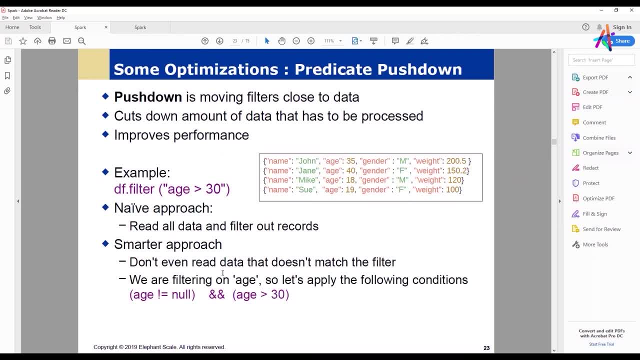 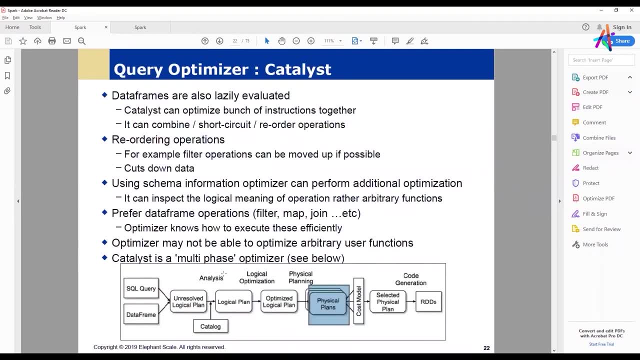 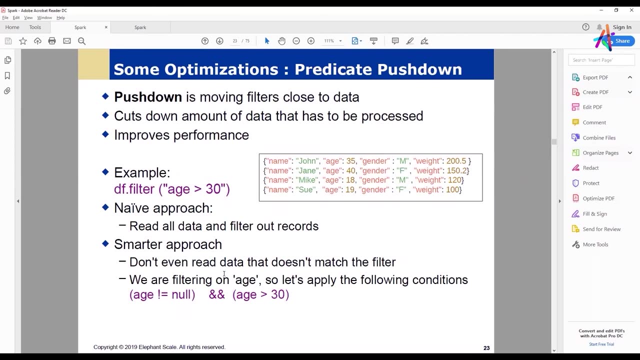 By pushing down we mean it moves the filtering closer to the data. So in a certain sense, let me see. can we see the diagram here? No, okay, So if we're doing a query and then a filter, that might be a lot more expensive. 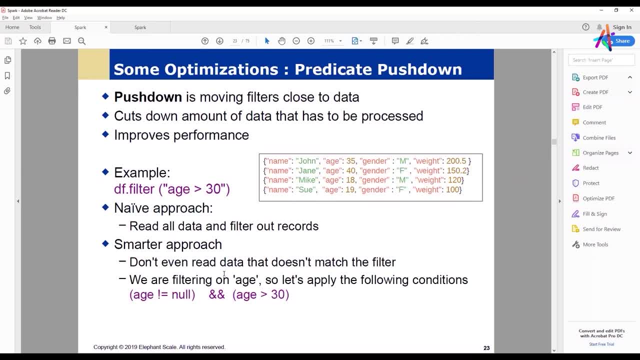 than doing a filter and then a query. So the. so if we do, or even if we do, a join and then a filter, it may be more, excuse me, it can be a lot more efficient to do the filter than the join. 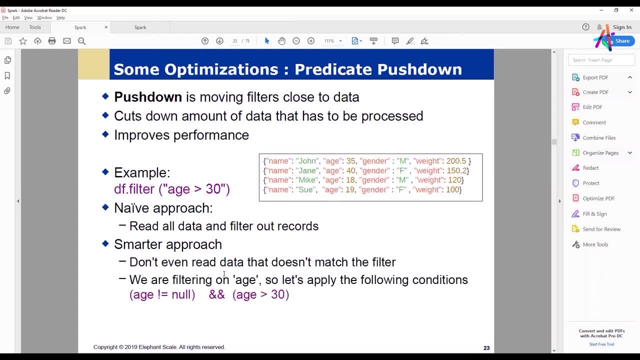 So here's our example: We have a, we have a dataset- small dataset- We have a filter. The naive approach is read all the data and filter out the records. The smarter approach is to say: well, look, if we're going to do a read and then filter. 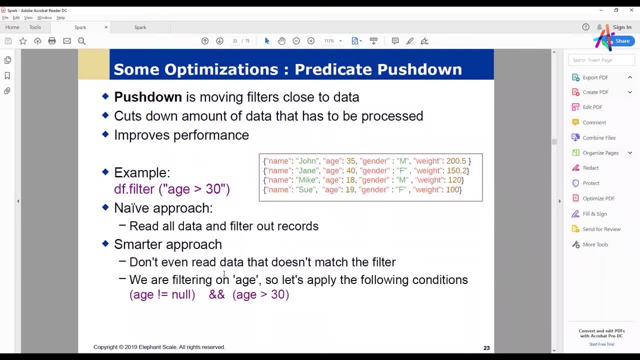 why don't we just, why don't we just read the data that only matches the filter, Because we're going to throw away the other data anyway. So we're filtering on age. So we apply the following condition: age is not null and the 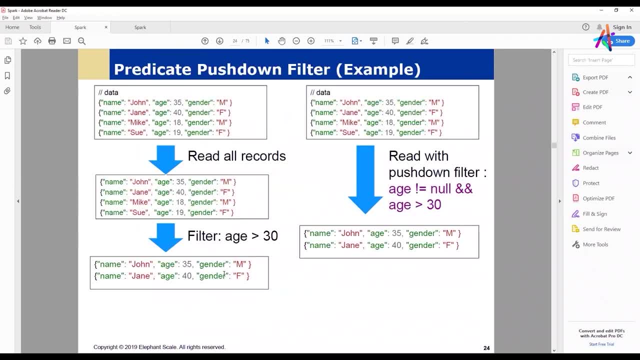 and it's greater than 30. So that's only the data that we're actually going to load and work with. So here's the optimization is that we've got the original data, We read all the records and then we filter, And that is a very natural way to write it. 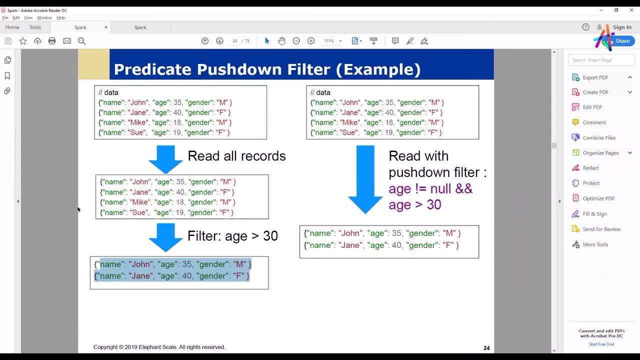 in terms of thinking about how the problem is going to work. But Catalyst says, actually the more simpler thing is to push down the filter. And by pushing down, ironically, it means kind of moving it closer to the data, which, in this diagram, is pushing it up a level. 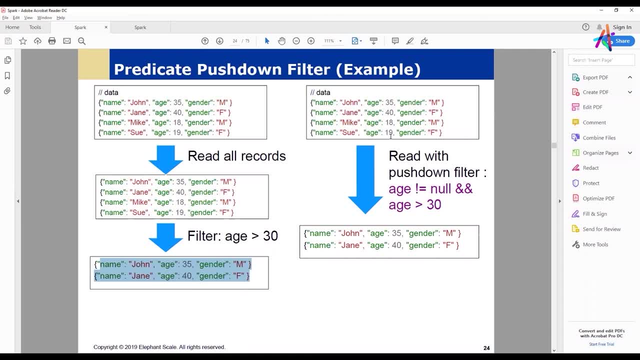 And so we're saying: only read down, only read the data that actually meets that condition. So as we read in a data record: if it doesn't match that filter, then we're done. If it doesn't match that filter, we don't even bother loading it into memory. 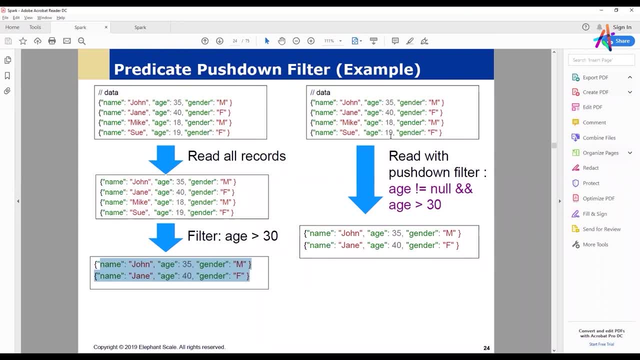 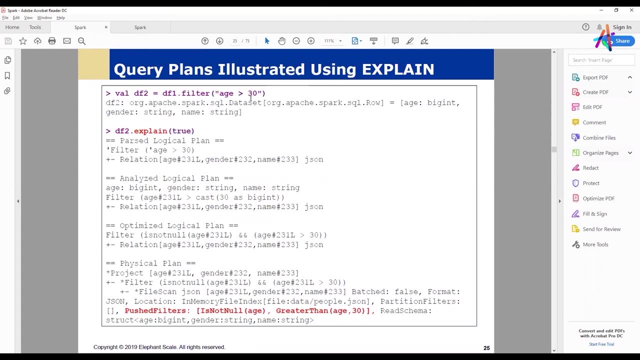 It just gets discarded and we just go on to the next one. So our data set winds up being a lot smaller when we load it into memory, when we read the data. So here is one of the options that we have with Catalyst is we can do an explain. 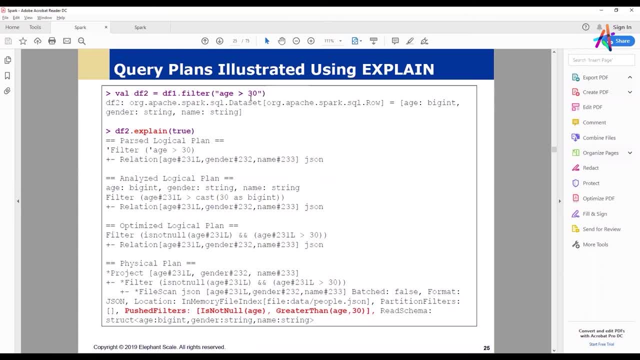 So here's my filter. So I'm taking my filter And creating a new data frame from it, from filtering my previous data plane, And then I can ask it to explain what happened, And so the output here gives me a little bit of a history. 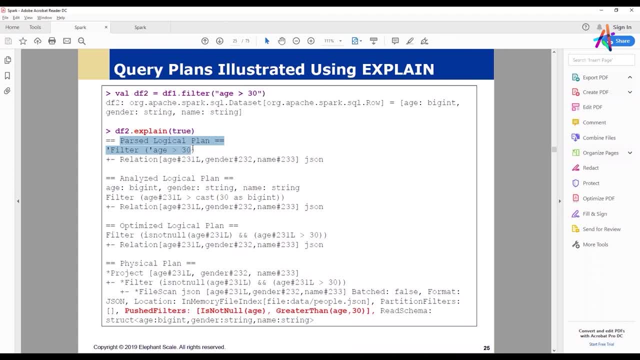 of what Catalyst did. So it parsed a logical plan filtered by the 30, and it analyzed a larger plan by looking at the various values and the various data types. It then looked at a couple of other aspects of what was going on. 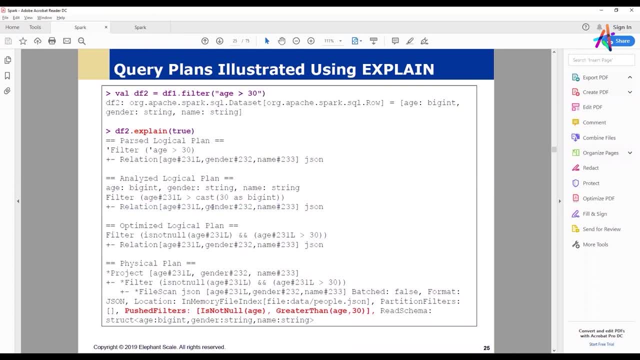 So this is a JSON file And there's a relationship here that it's looking at and these numbers here are indicating some internal record keeping. Then it does a optimized logical plan, which is what we just looked at. So now it's saying, okay, well, all right, we'll take this. 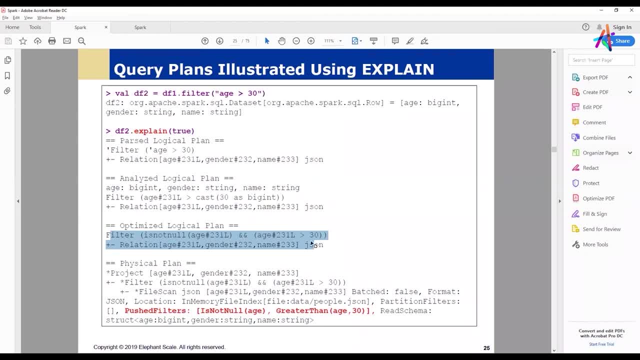 And transform it into this optimized logical plan. And then we have a physical plan which goes and describes what we actually did on this, And then we have the pushed filters, the filters that we actually pushed down, And so then it has the read schema. 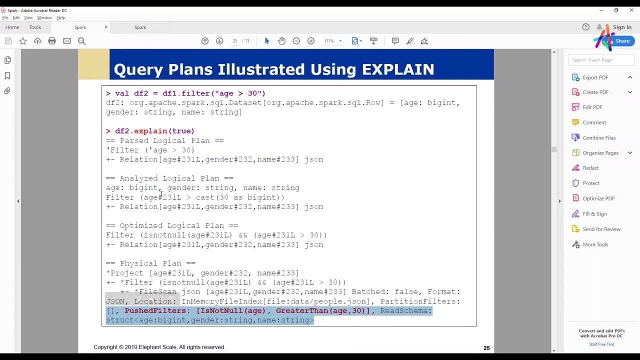 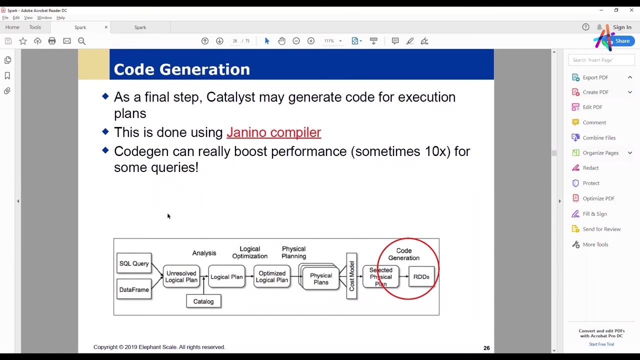 which is how it's reading the data in. So we can actually go back and ask Catalyst: what did you do to read in the data? And it will go. It will explain the steps that it used in the optimization. So Catalyst generates the code for the execution plans. 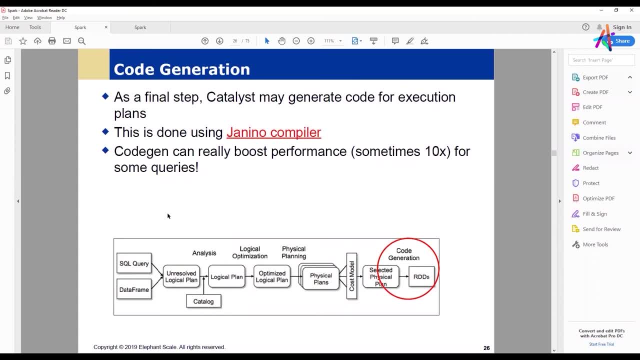 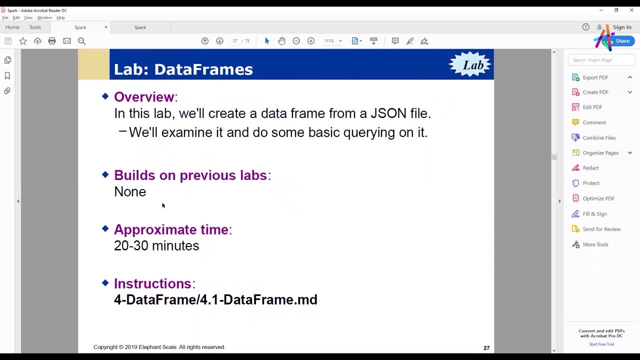 with the Janino compiler, and this can boost performance tremendously. Okay, so now what we're going to do is jump into our DataFrames lab, So I think we should be able to get into that. So we're going to basically create a DataFrame. 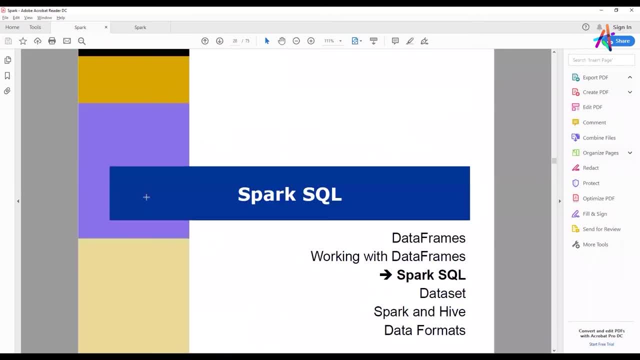 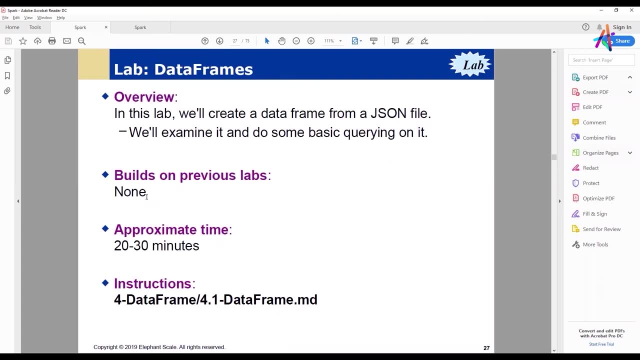 from a JSON file and do some basic querying, just to get some hands on with the DataFrames. All right, any questions? before we do that? All right, well, I'll let you guys jump to it. Same procedure we've before when you did the labs before. 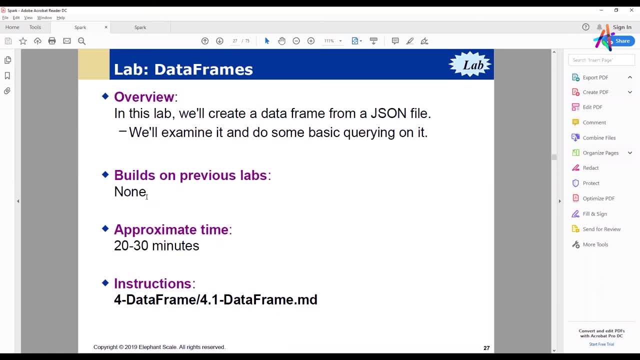 So we're in four. the instructions are in the 4.1 README file, And if anybody has any problems with the VMs, let me know. All right, and I'll check with you in about. I'll have my mic. I'll be listening in. 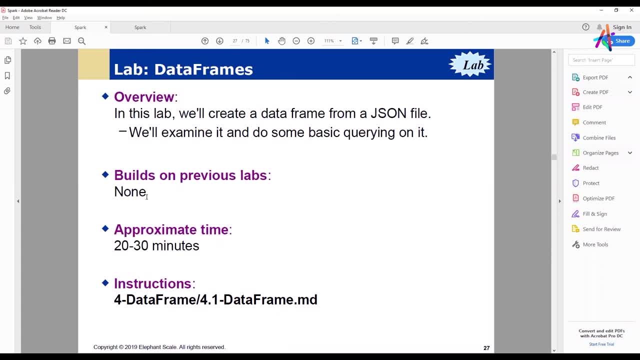 but I'll have my self muted and we can check in with you in about 15 minutes to see how things are going. All right, Because again, we're using the schema information, that, the schema information, that the schema information that is available. 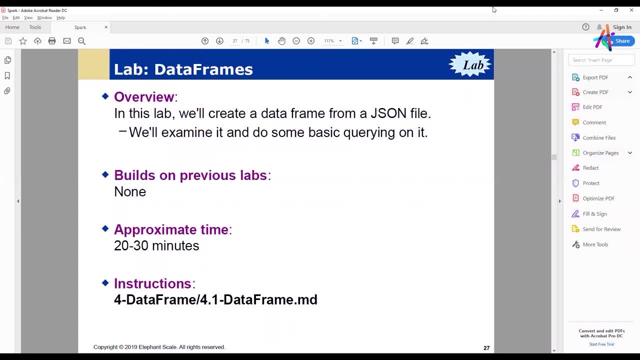 There's the diagram we saw before. So the the primary motivation here is that, while we have gotten some improvements over the Hadoop MapReduce interface, it's the RDD interface is still, you know, a pretty large API And it has the disadvantage 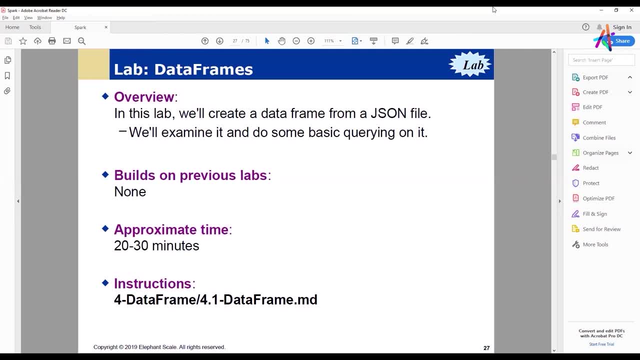 of the fact that we're still treating the data as big blocks of data, So we don't have a lot of things we can do with it. that would be really convenient with structured data. Hold on here. There we go. So the the other. 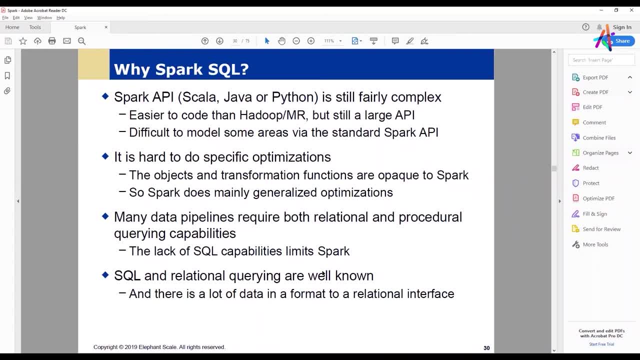 there's sort of the two different points that Spark is making. here is number one: we want to be able to have people use Spark in a way that makes sense to them, rather than thinking just in terms of RDDs. So the other, the other thing that Spark is making here is number one: we want to be able to have people use Spark in a way that makes sense to them, rather than thinking just in terms of RDDs. 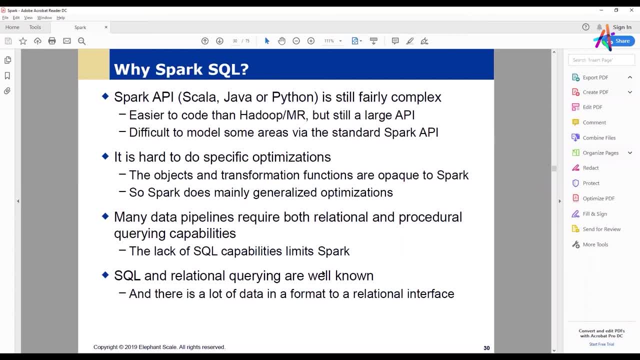 So the other, the other thing that Spark is making here is number one. we want to be able to have people use Spark in a way that makes sense to them, rather than thinking just in terms of RDDs. In the world today, everybody thinks in terms of structured data. 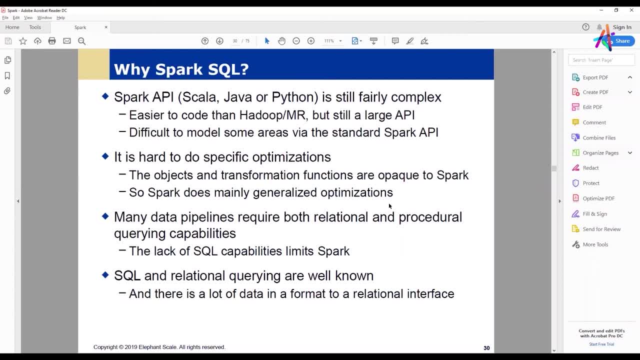 not everybody, but structured data is a fairly common kind of way of thinking about data. The data we look at as structured is one of those things that tends to be a self-fulfilling prophecy is that we use structured data because most of the tools we have are structured data tools. 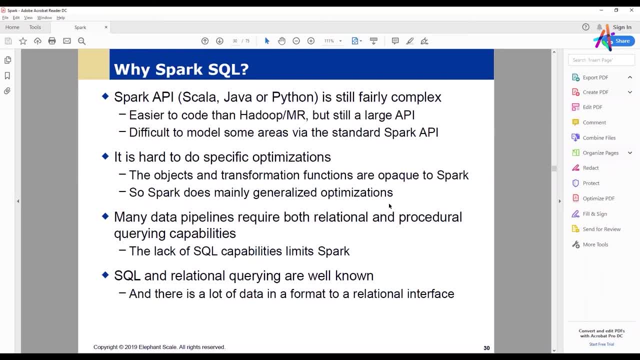 And because most of the data winds up being structured, then the most of the tools that we have wind up being structured data tools. So the data that we're going to want to work with is generally going to be in some kind of structured form. 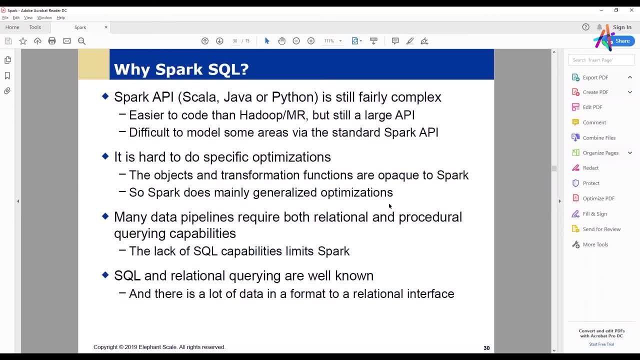 So the other thing that we do is we have a long history of understanding how things like queries are optimized. We can leverage all of that, that kind of general knowledge, to be able to do optimization. So, number one, we make a more intuitive and clearer user interface. 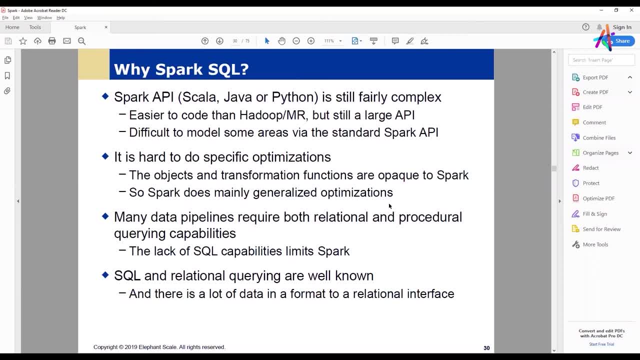 when it comes to working with data. But number two, we're also able to introduce optimizations that we wouldn't otherwise be able to be able to work with. The comment here is: objects and transformation functions are opaque to Spark, And that's the comment I've been making earlier. 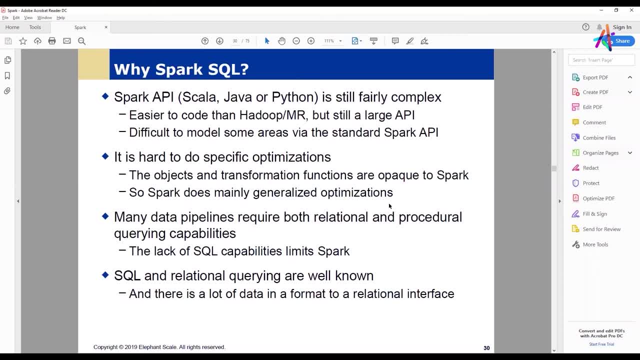 is that Spark knows that you're doing a transformation on the data, but the data itself is just a big black box. So Spark can make, in terms of RDD, some optimizations, but a lot of those optimizations just are not, are more general and they're limited. 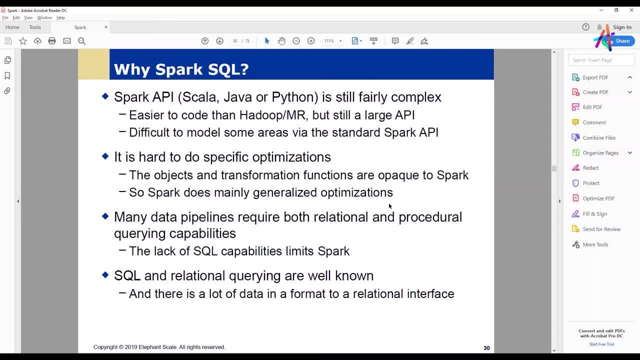 So the other, the other aspect of it is that we also have a use case requirements for being able to do various kinds of query queries into data And the fact that since, as I mentioned earlier, most of the data that we're working out there, 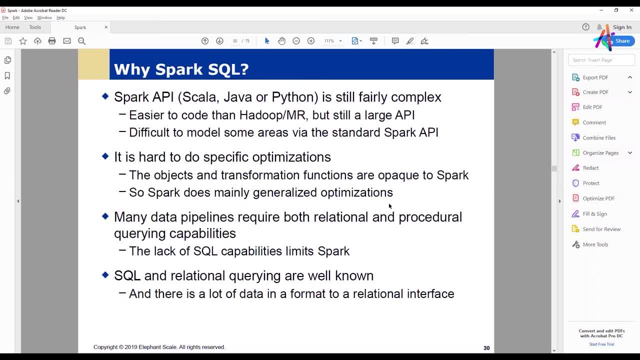 is in a relational type of structure, Spark is. Spark is unable to support SQL and relational types of of operations and it becomes extremely limited and is sort of the odd man out. So the primary, the primary motivation behind it, like I said, is twofold. 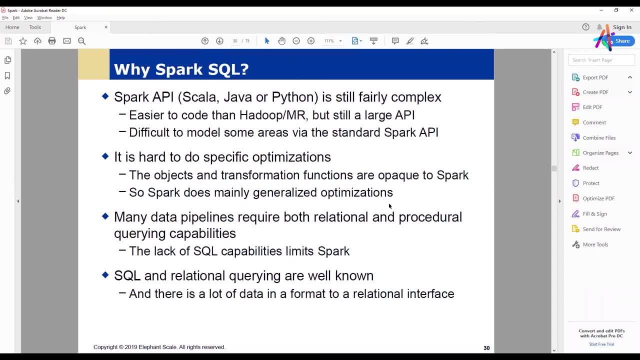 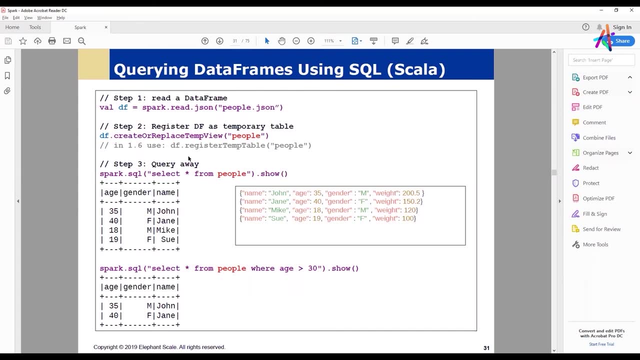 Number one: it is a a standard model, It is a well-known, we know optimize optimizations on it. And number two: it also introduces the ability to do to do more optimizations so we can query to do more data frames using SQL. 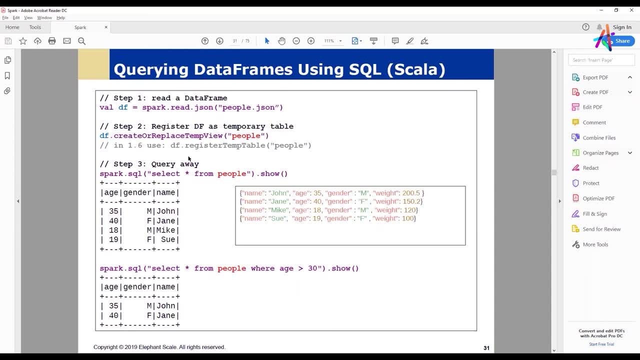 And here's an example: in Scala, We're reading an adjacent file. same thing as we had before. Now what we do is in step two, we're actually creating a view of the data, that is a essentially a table structure, And then we can start to query this. 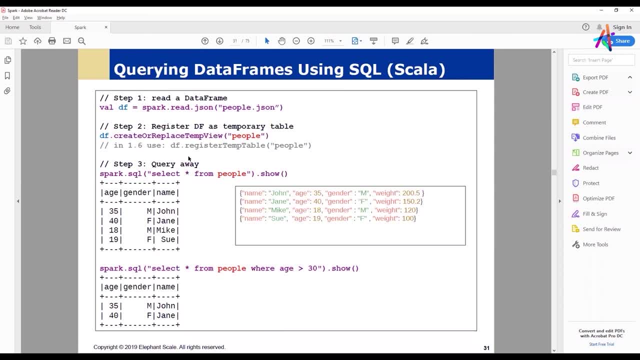 as we would any other table. So the example in step three is the. the string in the double quotes is a standard SQL query, and then we can show the results of that. And again the. the line down, farther, farther down here is also a standard, a standard query. 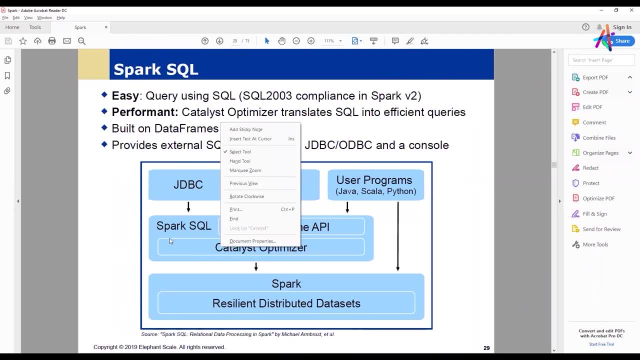 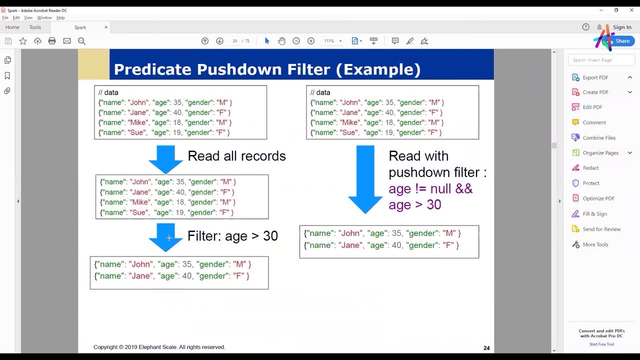 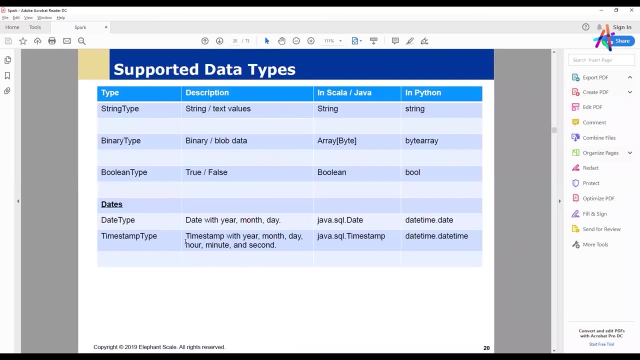 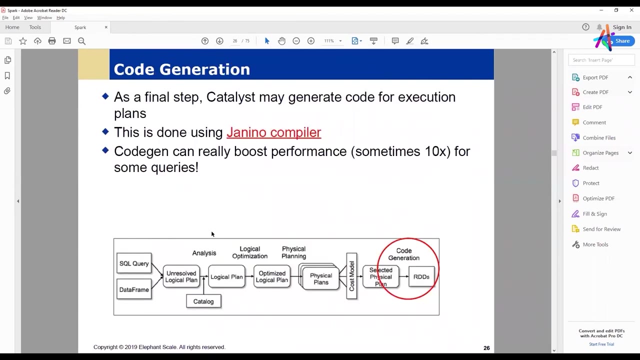 Now, the difference here- to go back from here, if we want to just keep this in mind- is that we have a more the operations that we were using here on filtering and these sorts of optimizations. while we were taking advantage of the relational structure, we still didn't actually have enough structure to be able. 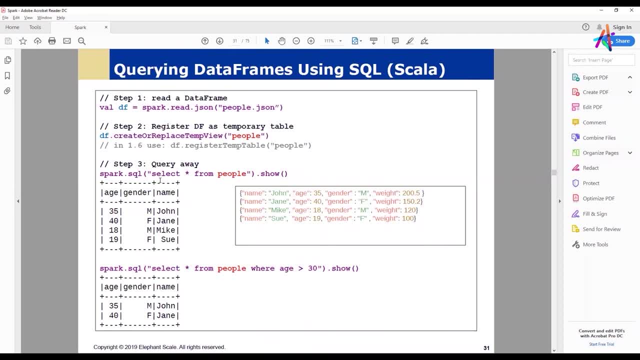 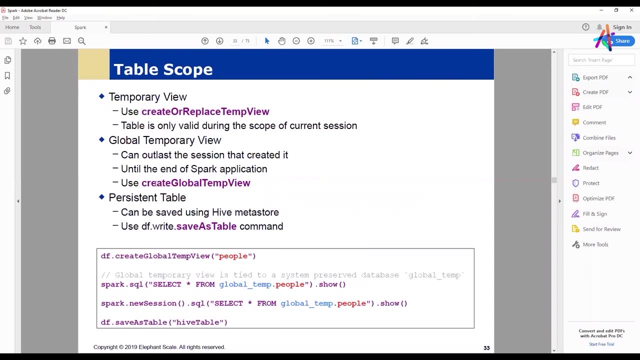 to do SQL. So in this operation here we're actually creating an intermediate form that allows us to do SQL type of operations. So what about this intermediate form? Well, the temporary view is like I said, it's just an intermediate form. It is a conceptual construct that is. 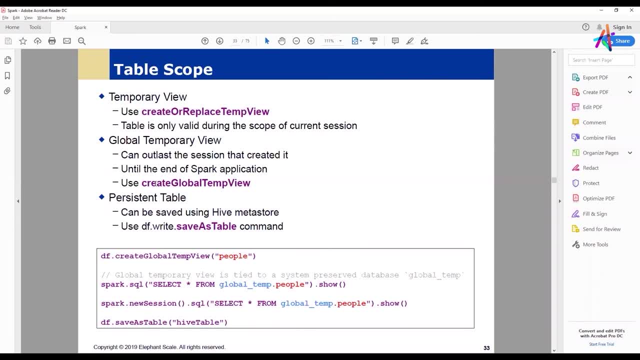 created for us to be able to interface with the data as if we had an underlying table. We can also create a persistent table and we can also create a temporary view, So we may have In our Spark application several stages that allow us to use a table in a transitory manner. 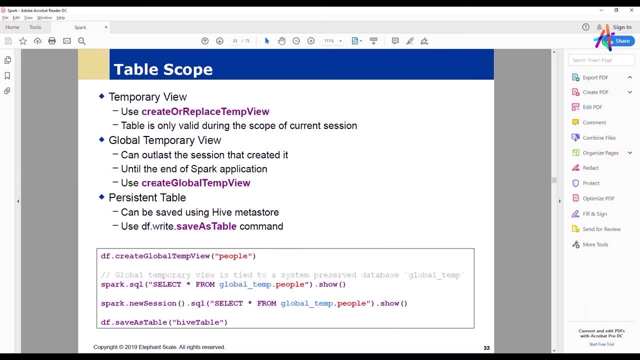 or we can generate a table that we're going to use consistently, which is our global temporary view, or we can actually restructure the data and save it out as a table using a save as table command, And there's use cases for each of those. 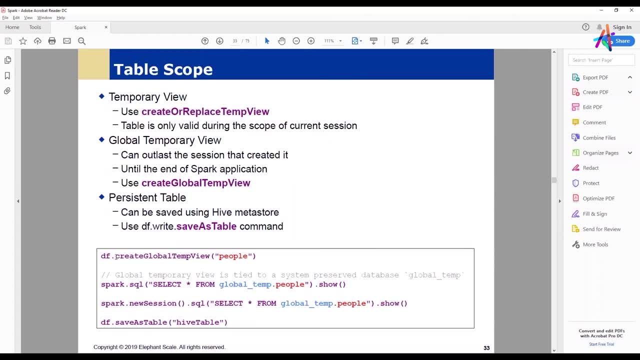 So here in the example we are taking a data frame. Now we've already got a data frame and we're creating a temporary global view from the data frame And we are okay. so here the global temporary view is tied to a system. preserved database: global temp. 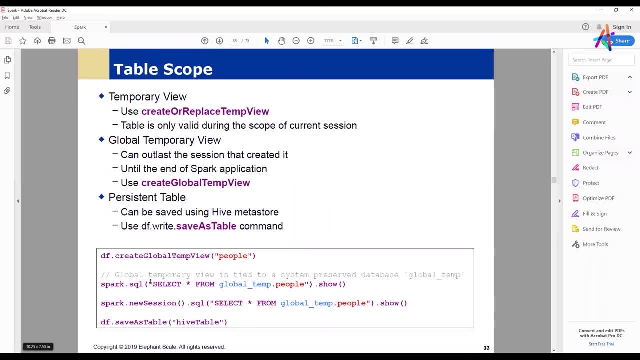 So, in other words, we are actually able to use this interface, but it's still tied to that underlying data store. So now here is our view, and we've specified that this temporary view is people, and so we've got globaltemp people, which is our intermediate view, on the table. 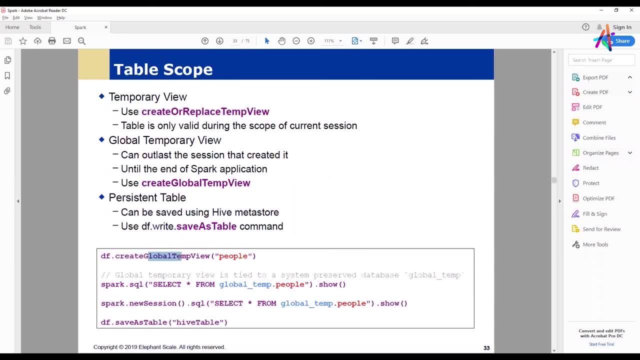 So we can also now, because we've created a global temp view, we're actually able to start a new Spark session and we're able to access that table again, so it doesn't have to be saved. It's saved more than once or it doesn't have to be created multiple times. 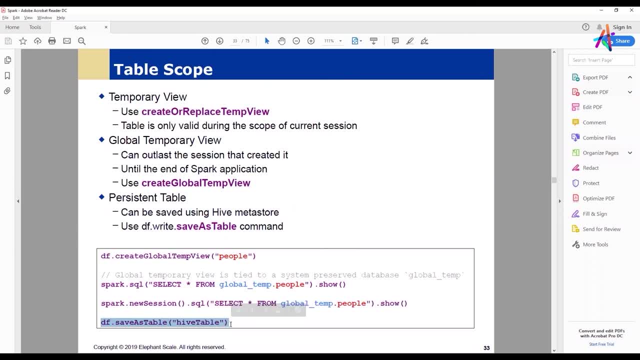 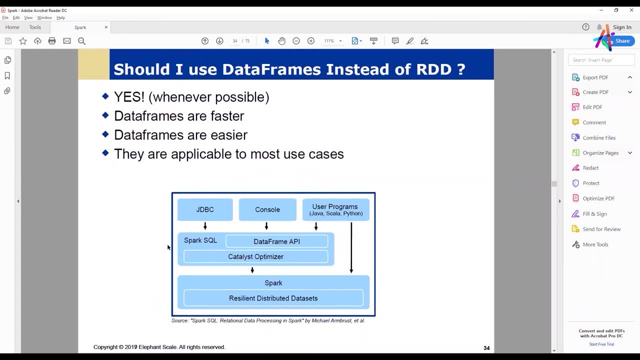 And then, when we're done, this table may be useful for reuse, so we can go and save it as a hive table. Question is- and this is going to be fairly obvious: do we use data frames in RDD wherever possible? They're faster, They're easier. 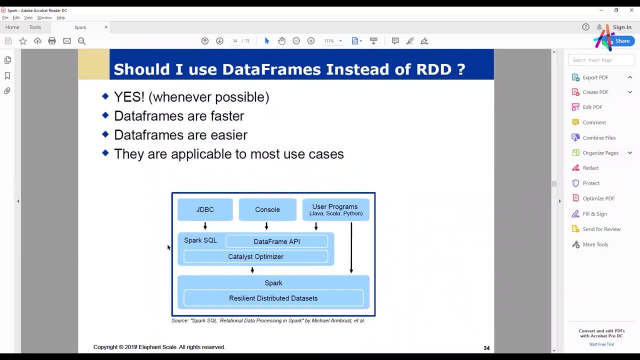 Why are they easier? The model is well known and that is Generally, as I've said before, those two points that we have with data frames. people generally conceptually tend to think in terms of tables, particularly because most of the data that we're using is in form of tables. 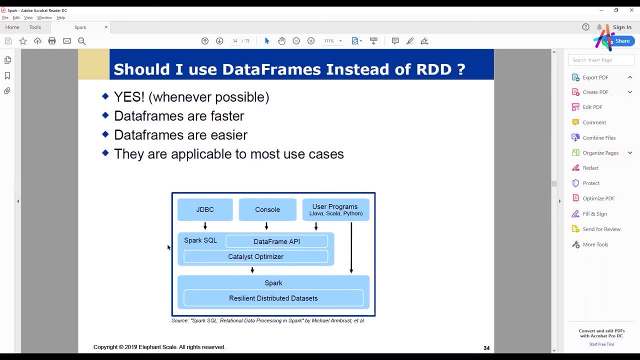 because most of the tools are tabular. There's a very natural relationship there. They're easier. in that sense, The fastness comes from being able to do the optimizations. but the other thing that we keep in mind is that, because of the nature of how data is maintained out there in the real world, 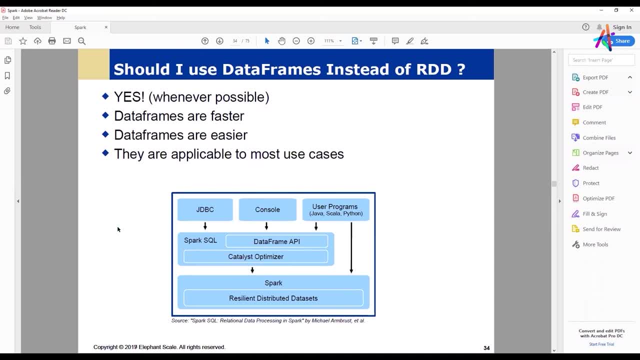 that most of the time tables in some form are going to be the appropriate tool for various sorts of use cases. Obviously, it's a little bit different when we talk about different kinds of streaming data and other sorts of things as well. 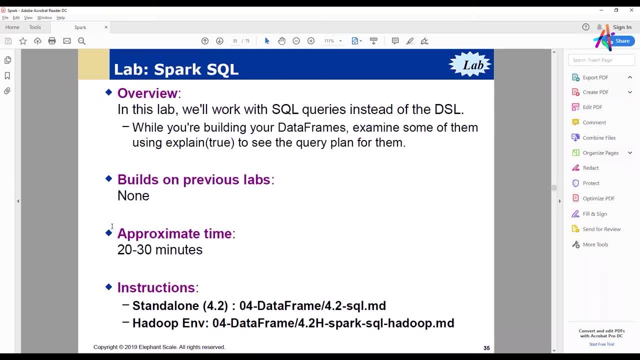 So now we come to our next lab, which is working with SQL queries instead of the DSL. So again, notice that there's two distinct ways to run queries here. One is with the DSL, which is the stuff that you were just using. 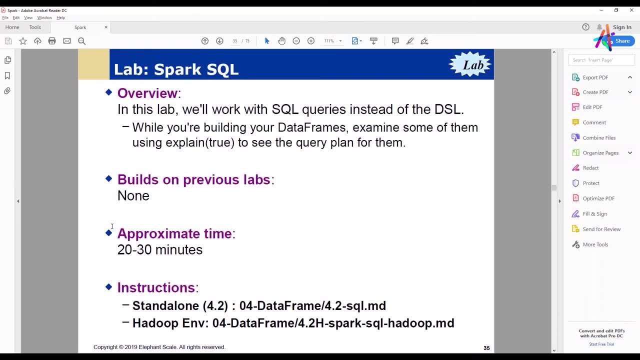 where you're actually not representing things as a table, but you're actually just working with the implied structure. In this one, we're actually going to be using the intermediate table in order to actually run the SQL query, So I'll let you guys get at that one. 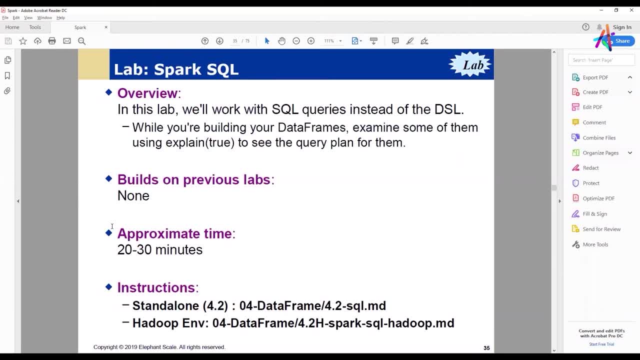 Are there any questions? Any questions before we start? Hello? Hello, Yeah, I'm here, I can hear you for some reason. So question, I was playing around because I was finished Tried window functions and things like that. Everything on first glance works. 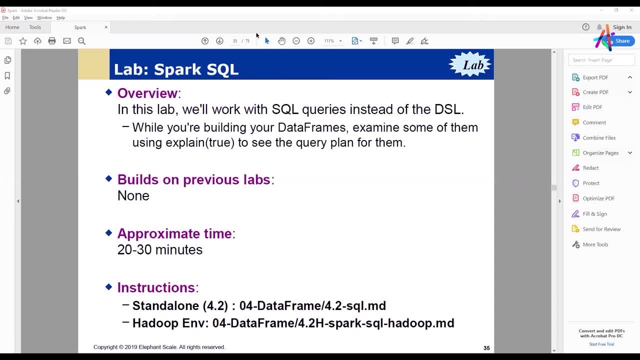 Question: Is it really full SQL that is supported, or are there things that are not supported from the standards? I think you're probably going to find that it's not going to be as rich an SQL environment as you have in other kinds of products. 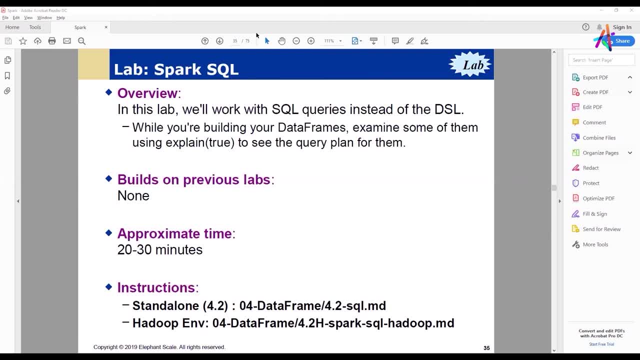 I'm not exactly sure, but the core SQL is certainly important in this sense in terms of being able to run queries. Were there specific SQL features that you were thinking about when you were talking? Ask that question. No, just things to look out for. 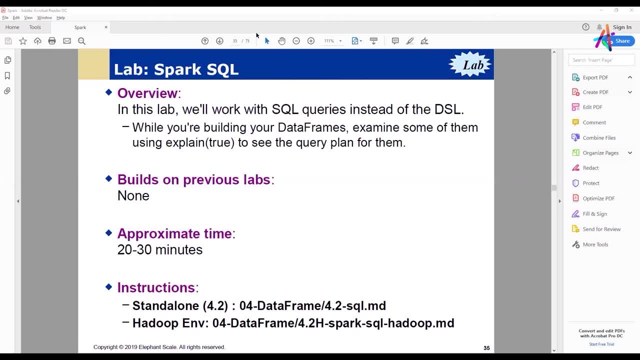 If you know of anything that doesn't work, that probably should right Things like group by low work. I was like, okay, window functions, do they work? Yes, they do. So are you aware of anything that is, let's say, outside? 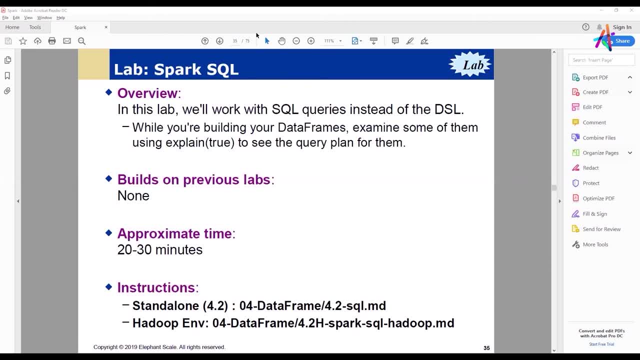 Not off the top of my head, no, But I'm sure that there may be some real peripheral kinds of things, things that are not that common, that may not be implemented, But most of the core sort of SQL type of structures and queries. 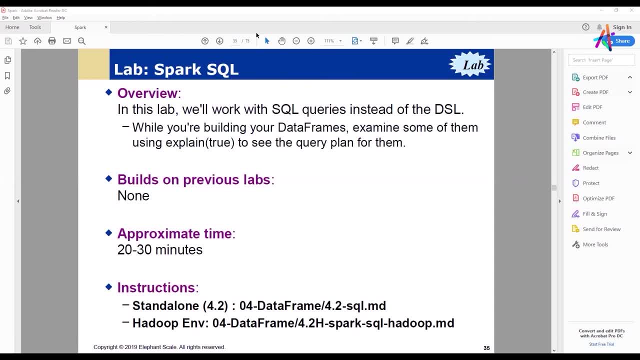 should be implementable in Spark. Okay, thanks. Okay. Different question: Is it really? Is it really widely used? Because I haven't seen it that much in any production code. You mean the Spark SQL? Yeah, the Spark SQL, yeah. 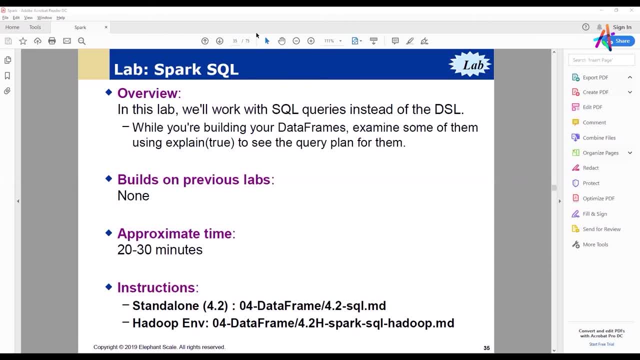 You know what? I really don't know what the usages of it are in terms of actual numbers, because I don't kind of follow patterns in the market, But the thing to remember too is that it's only been out for a few years. 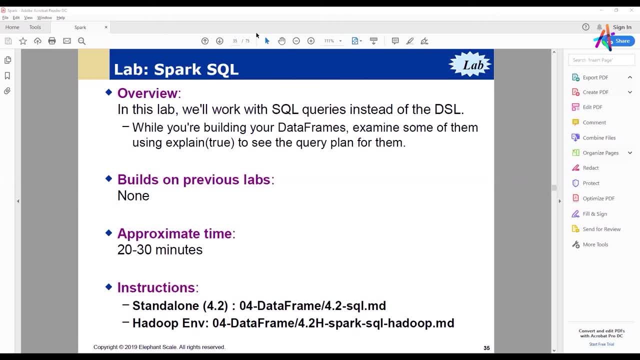 And what I encounter with a lot, A lot of people that I talk to- not just with Spark, with other kinds of products like this- is that they often, if they're early adopters, they wind up getting a whole bunch of production stuff. 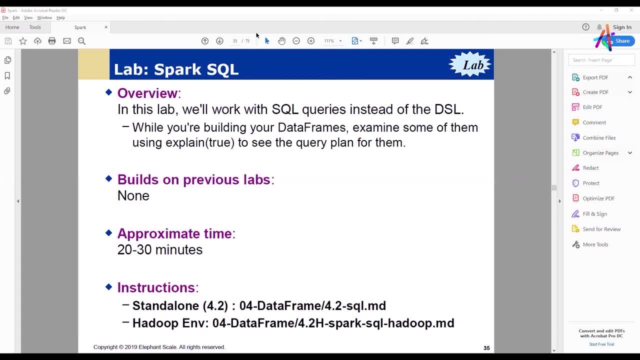 that's sort of in, you know, like an early kind of model, And then they really, If it works for them at that point they're often not quite that eager to make a transition into another sort of version. So I suspect that there are a lot of people out there. 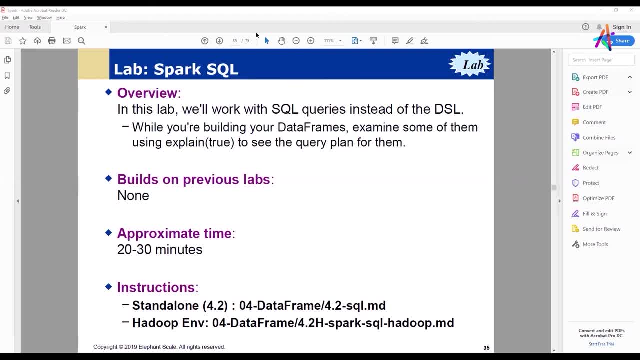 who have adopted Spark, who got involved with the RDDs and found it was adequate for what they wanted to do, and they haven't had the use case to want to migrate to SQL. I think we're probably going to see more of the SQL. 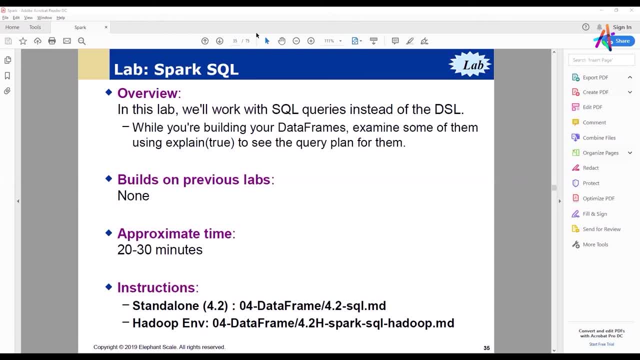 with people who are now currently adopting Spark, who are able to take advantage of that, And this seems to be characteristic of a lot of technologies. So, for example, Hadoop came out and solved a very specific problem and, even though there's been enhancements, 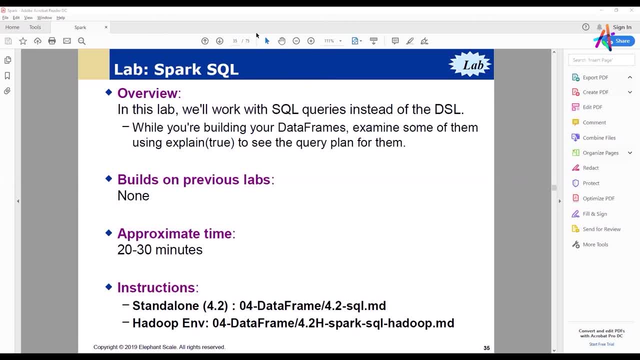 to the entire sort of clustering system. a lot of people are still using the model that came out earlier, simply because it meets their problem or meets their requirements. So that's the only such insight. I think I can offer. that for a lot of people. 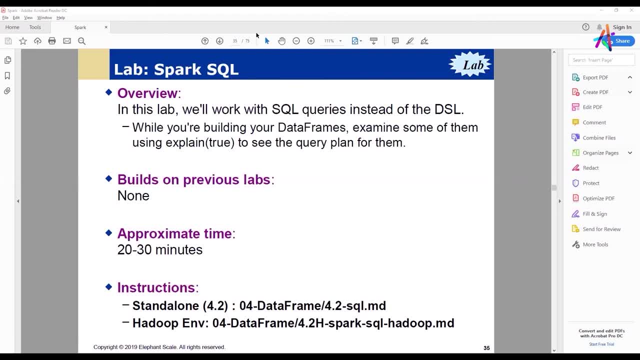 RDDs may be exactly just what they needed, And so they haven't progressed on this. But, but again, it's more of an issue where I think you have use cases where RDDs do not become, or for performance or other reasons. 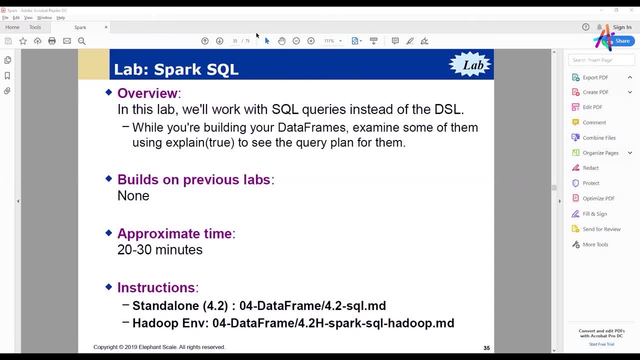 stop meeting the requirements that people look towards transitioning. I've discovered from my client base that people are very resistant to change, So who knows, Does that help answer your question? Yes, definitely, Yeah, Yeah, it's. I think that, like I said, 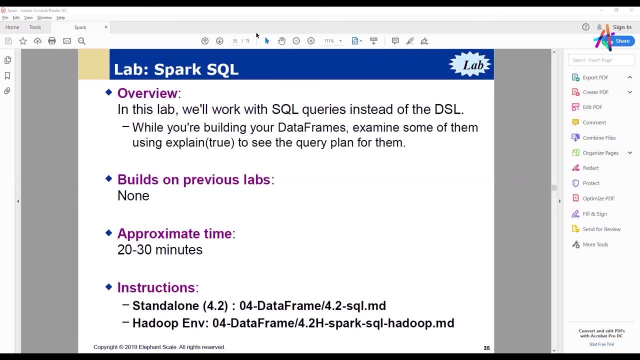 I think probably people who are adopting Spark now would be more likely to work in this environment than the old RDD environment, Whereas legacy users may not be All right. how are we doing for time? Has everybody got Anybody need a little bit more time. 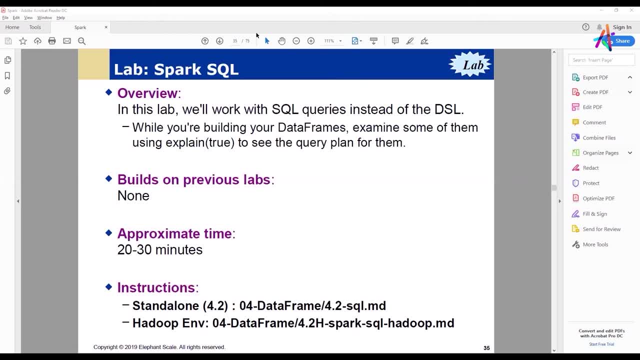 Sounds like a lot of people are finished. All right, I think we're good in Berlin, Yeah, good. Okay, you guys are really fast. You're taking about half the time you're supposed to for this, So we're going to be a little bit ahead of schedule. 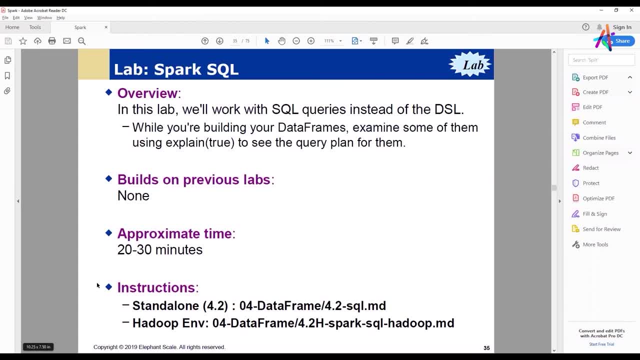 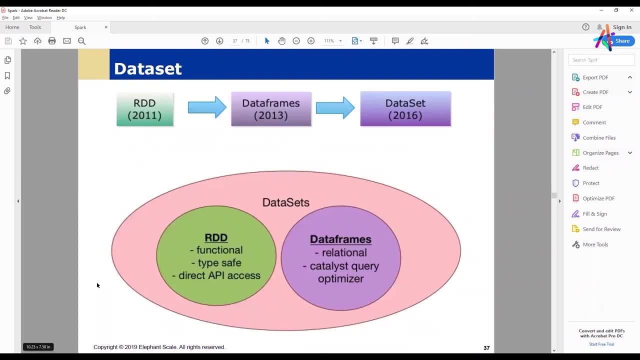 by the end of the day, which is Friday, So maybe that's a good thing. Okay, so now we're going to talk about Dataset. So Dataset is? So actually, if you look at this table just in reference to the previous slide, 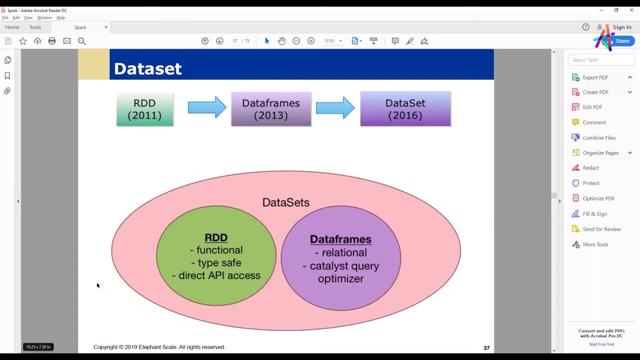 this is a very serious question. RDDs are 2011.. So that's about eight years ago And Spark, when it came out, was really sort of explosive in what it was doing. Excuse me for a second: It was explosive in what it was doing. 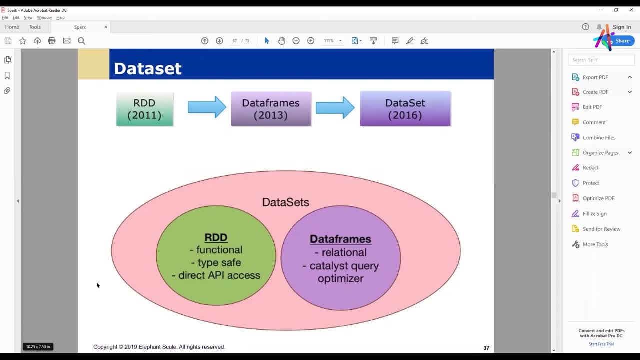 So I think we saw Probably would see a big wave of adoption at that particular time, At that particular point, And those are the groups that I'm thinking. maybe sort of it solved a particular problem for them, as they saw no reason to change it. 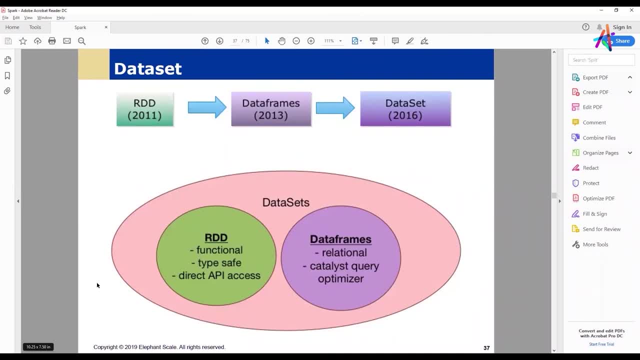 So DataFrames comes in 2013.. Now we have two different models that are fundamentally incompatible, So you are kind of using two different APIs into Spark And in 2016, they're unified under the Dataset API, So the Dataset unifies that. 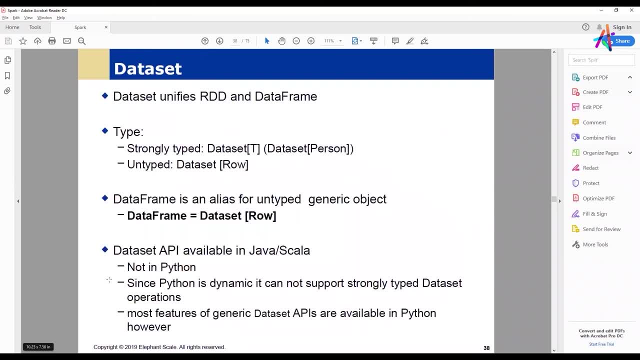 So the Dataset unifies that. So the Dataset unifies that. So in 2016, we have a new version of Spark And it has the typing. So we have strongly typed and we have untyped And the DataFrame is an alias. 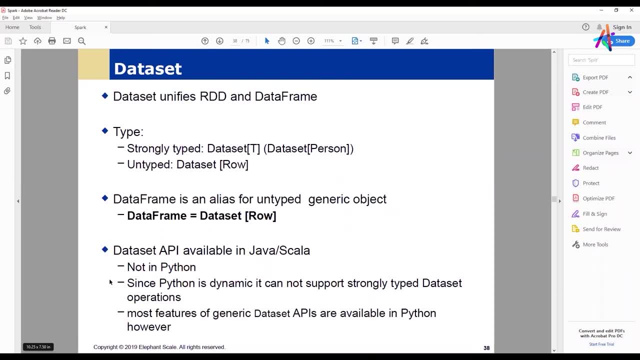 for an untyped generic object. So the It's not really clear from the side here, But the big thing that happened with Spark- and it's not really clear from the side here, But the big thing that happened with Spark was that. 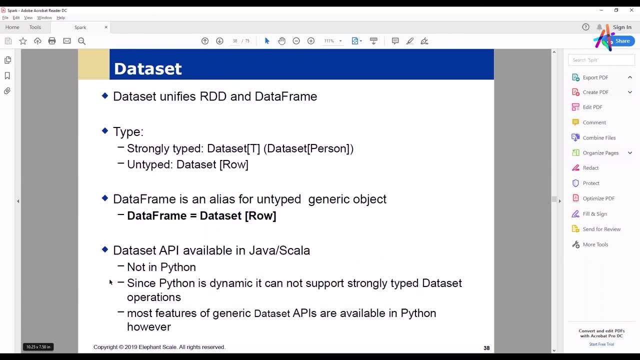 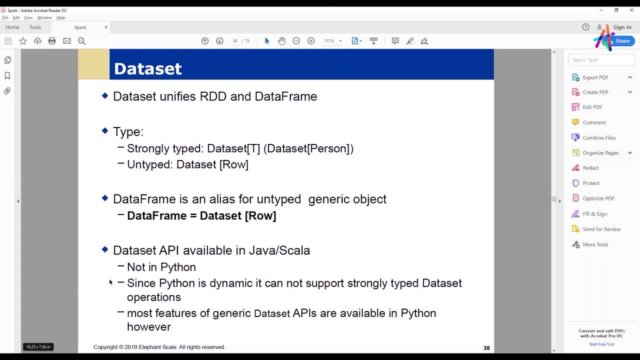 So the introduction of typing, whereas before with the RDDs, you had pretty much just kind of blocks of data And we saw before you could impose structure on it And you could impose structure on it, And then you start to get real good optimizations. 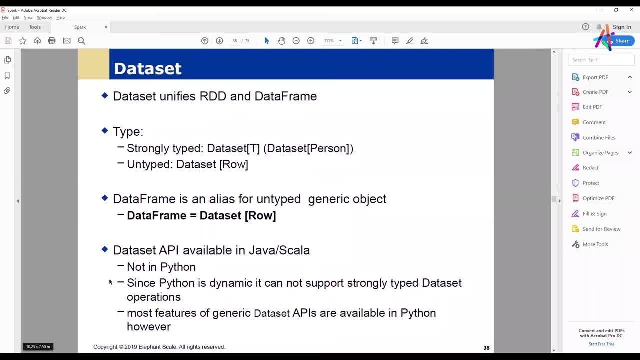 for things like serialization and other sorts of things, memory usage and execution performance, And that's why the Dataset API doesn't work as well in Python. Now, Python can still use the RDDs which use the older model, which use the older model. 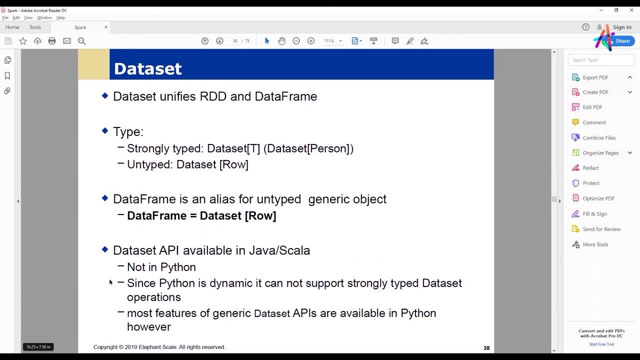 but the, but the but the modern dataset because it relies on this underlying typing. So this is an improvement that came into effect primarily for optimization reasons. So the dataset API is not in Python because it can't support the kinds of operations that depend on typing. 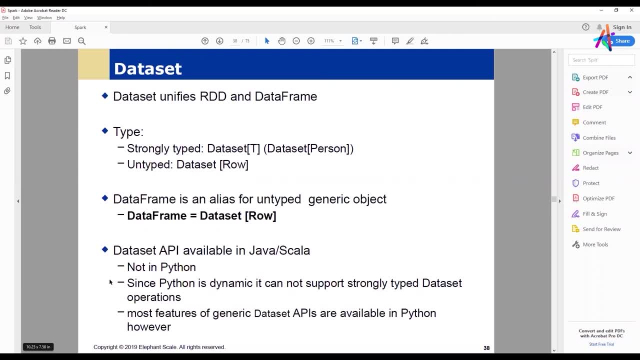 I'm suspect that somebody will come up with some kind of extension to modify that. But a lot of the features are available. But it's just not a full implementation for Python. So we can have in our datasets two kinds, which are the strongly typed and the untyped. 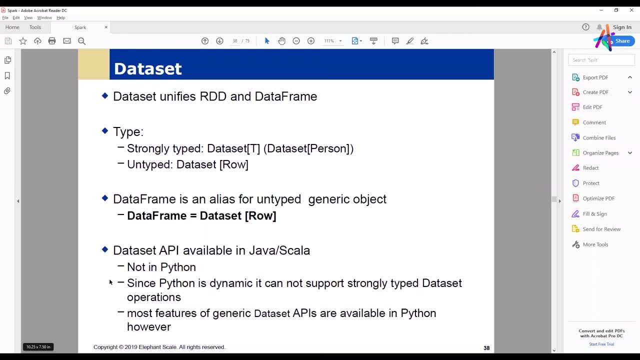 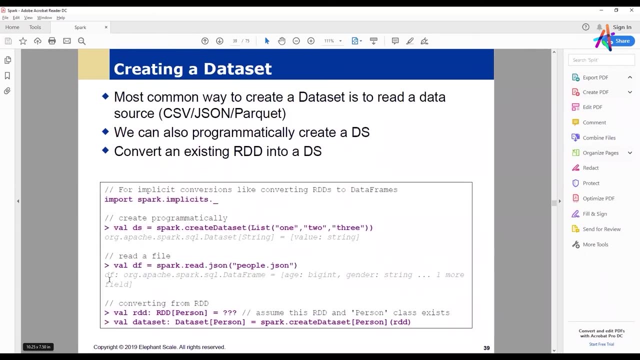 And the untyped are really more like the traditional RDD And the data frame. we also can use this for an untyped. So what happens is that the big innovation with datasets is the use of strongly typed data. So what we can do is read data from some kind of structured source and then 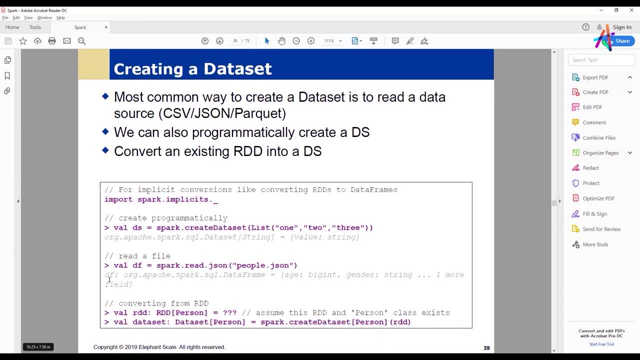 we can create a dataset out of it. So let's look at the example there. And we can also convert an existing RDD to Python. And we can also convert an existing RDD to Python. And we can also convert an existing RDD to Python. And we can also convert an existing RDD into a dataset, Again using the. 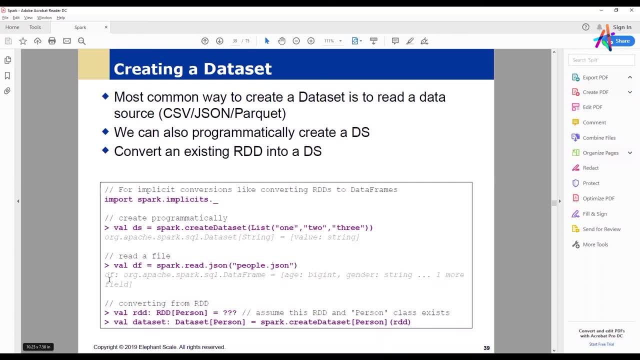 idea that we're introducing typing into a dataset. So we've got an example here of creating a data set from a list of things, And so now we've got a dataset from the list, We can read it from a file, So there's an implicit conversion to a dataset, because a JSON file can be parsed in order to 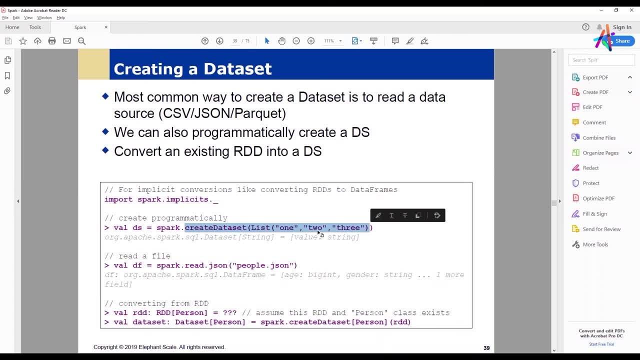 determine its structure, inherent structure in the json file, and we can also um go and convert uh, rdds, um, uh from uh, um or, i'm sorry, convert from an rdd. okay again, but again notice the comment here- assuming this rdd and the person class actually exist, uh, so what we're actually doing is is creating a, a typed. 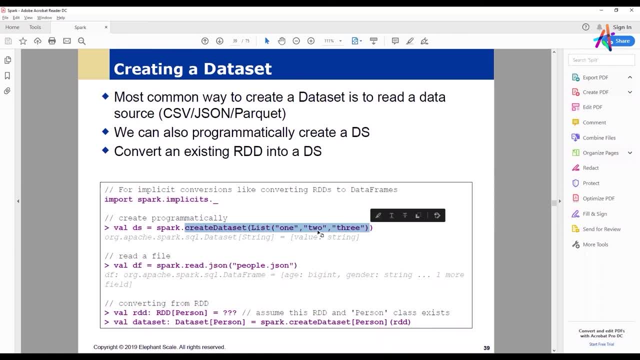 structure when we do create data set from the rdd in order to to create it now, if, if the class person, the typing, doesn't exist, then this isn't going to work. so just to to summarize to this point, we've enhanced rdds into data sets primarily by introducing structure. the data frame now is: 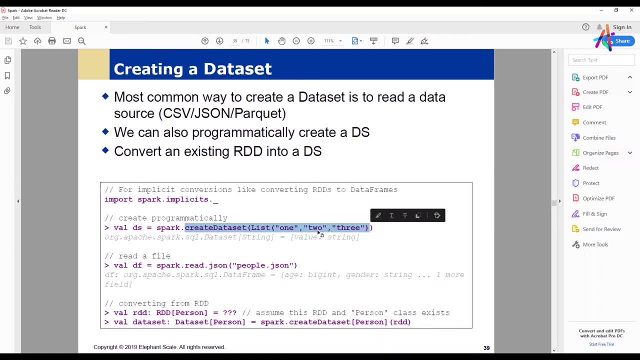 a variation on the data set or a subtype of the data set, but the data set in this strong typing, so we can utilize this notion of the typing in both the new version of the RDDs and the data frames. You got to think of this, as the data set is being introducing an underlying representation of the data which now can be accessed. 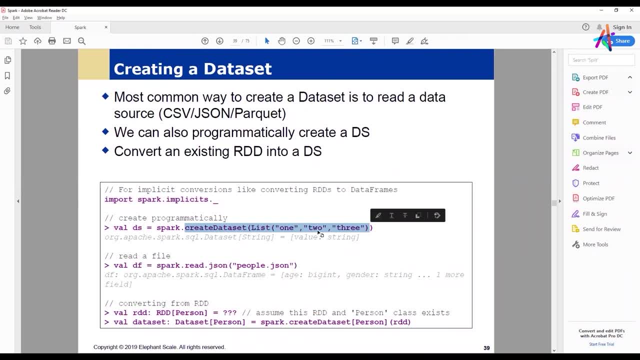 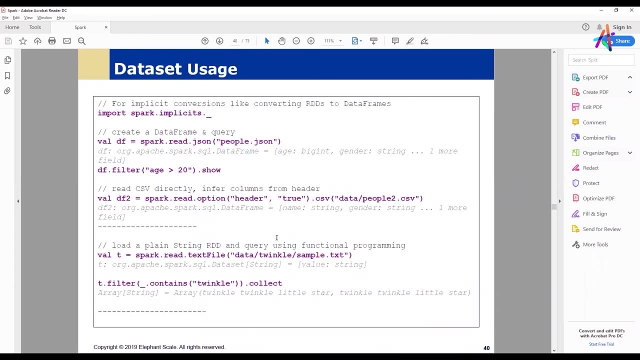 through a couple of different APIs, which is the data set API and the data frame, in the manner that we've looked at previously. So now it's become a lot more flexible. So if we take a look at this example here, in Scala we have the implicits, which does a lot of the implicit conversions. 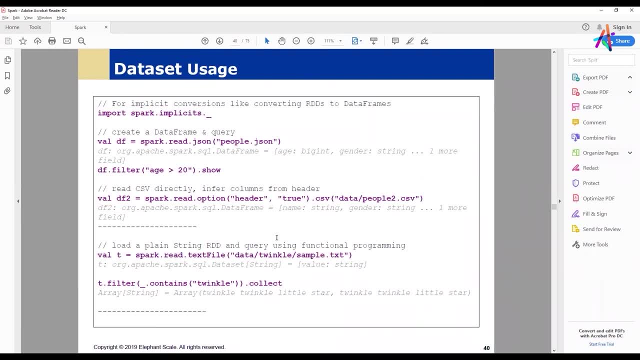 And so we can create a data frame and do a query. So we can read in the JSON file, so it creates a data frame and query, so that's a kind of data set. We can read CSV, which also has an implied structure. 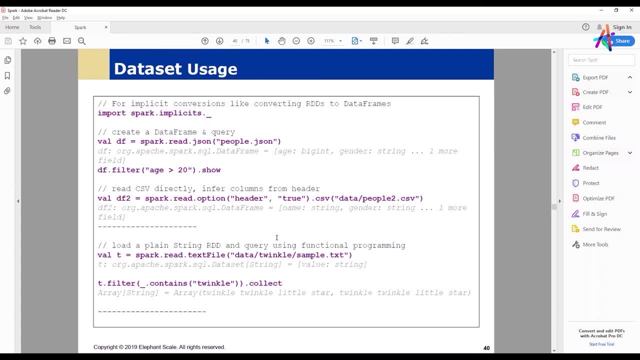 It tries to read the column headings or infer the columns from the header so it figures out an internal structure from that, so CSV files, And it can also load a more traditional approach, which is the text file, and operate on a more traditional level here where we're doing a filter. 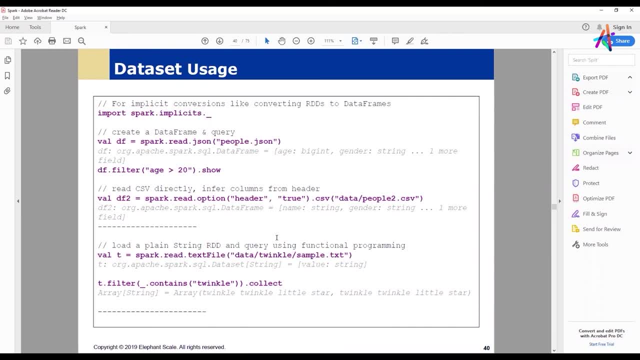 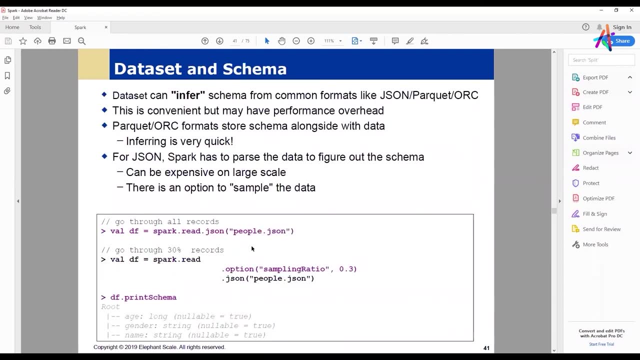 So we can, we can. so the data sets really cover the whole kind of wide range and usage. The thing that that that make data sets fairly powerful is this inferencing of schemas. So once we have a format like ORC, Parquet, JSON, you can start to infer. 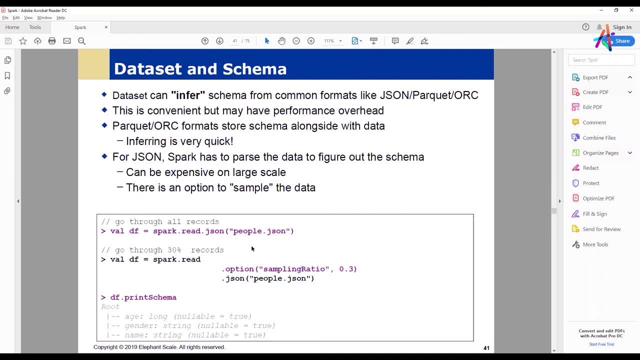 A schema from that. So the the there's. it says here there's convenience, but the the there. there may be, depending on the format, that we're using, some sort of performance overheads. So the certain formats have a catalog that go along right with the data. 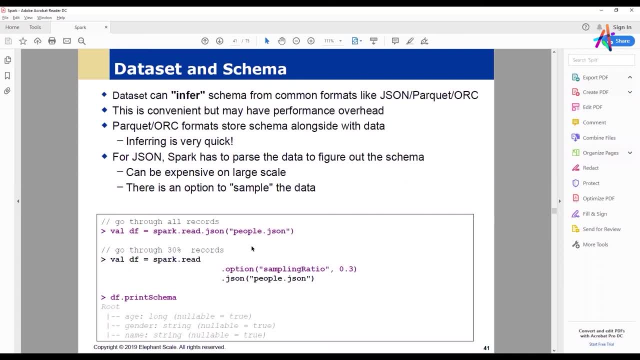 So Spark doesn't have to do any analysis of the data. Spark can just go and look at the catalog Or the schema And determine the structure right from there. So a couple of formats- Parquet and ORC- have that. However, the other kinds of formats you have to do some inferencing of the structure. 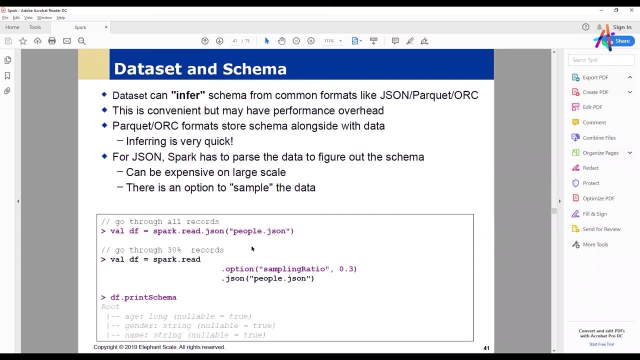 So the the cost of actually doing that can be very high depending on the size of the data set. So what we can add here, So what we can actually do, is sample the data and go and infer the structure from the sample. So, as illustrated in the example, we we could go through all the records. 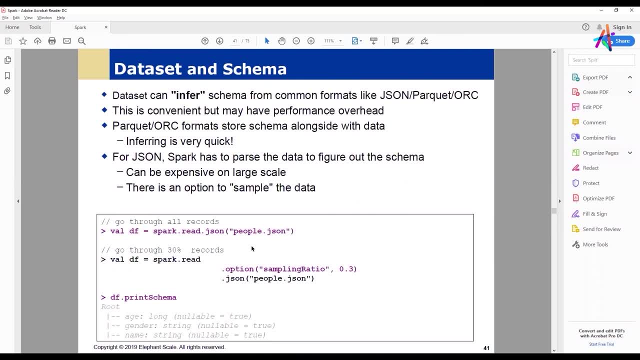 Or what we could do- and depending on the size of the data set, this could be quite expensive. Or what we can do is is just pull up 30% of the records and sample the data in that in that, in that sense, 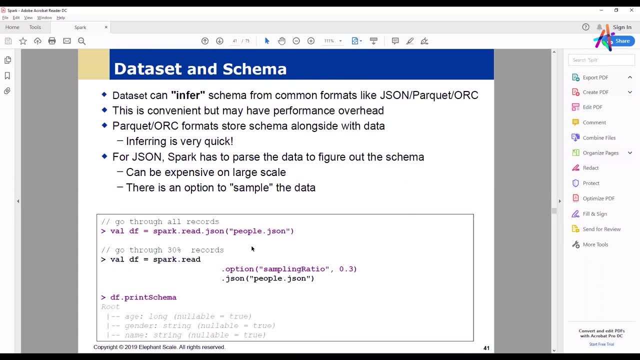 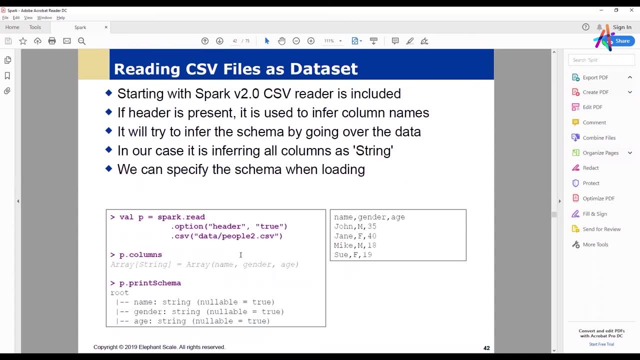 And and then print the schema that comes out of that. So the. so there are a couple of things that we can do to do that In order to- although I'm sorry, there's a couple of things we do to cut down on the overheads. 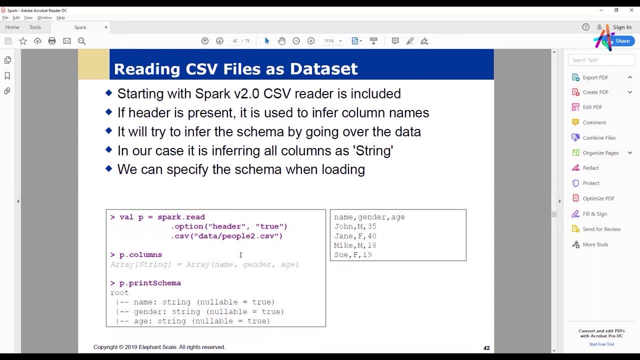 This is one of them. the sampling The CSV files as data set is an innovation, Which is where the header is used to inference from the column Column names And it'll go over the data. So it's, it's, it's inferring all columns as strings. 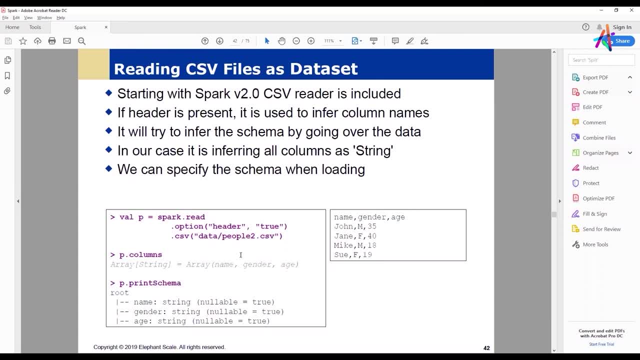 And we can. so it allows us to specify the the schema when loading. So there's our CSV file on the right With the three headings and the appropriate rows of data, And now when we're doing a read, we're reading the CSV and assuming that the headers are, that's that option clause. 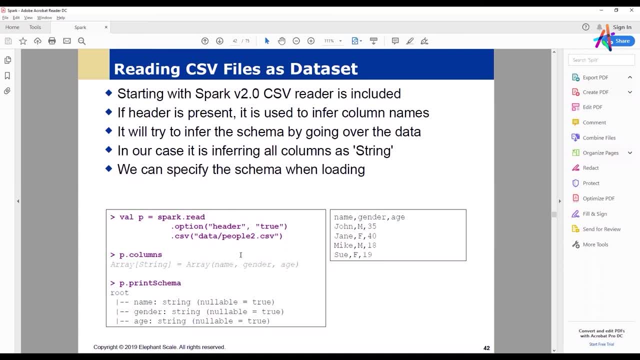 So we're we're reading our CSV file And we're saying: look for the headers, And then we can go and print out the columns and print out the schemas And we we have another way of inferring the structure, So we can also specify this. 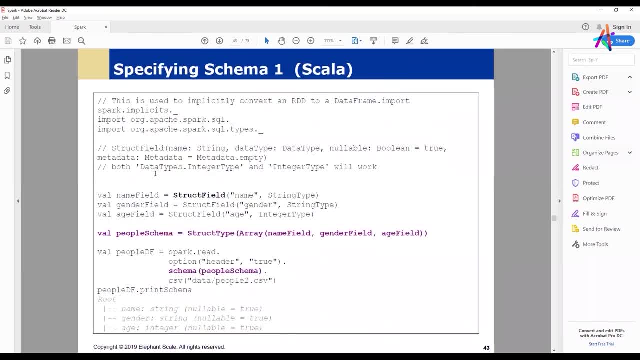 So this specify the schema when loading as well. Okay, so here's an example of specifying the schema So we can go take a look at this. So we are going to implicitly convert this RDD to a data frame, And so there's our imports. 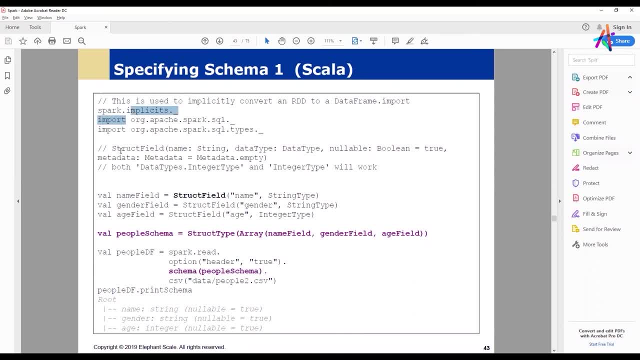 So here, what we're doing is we want to get this structured field And, let me see, this is going to be named gender and age. So we're we're talking about name as a string And we have some other information in here as well. 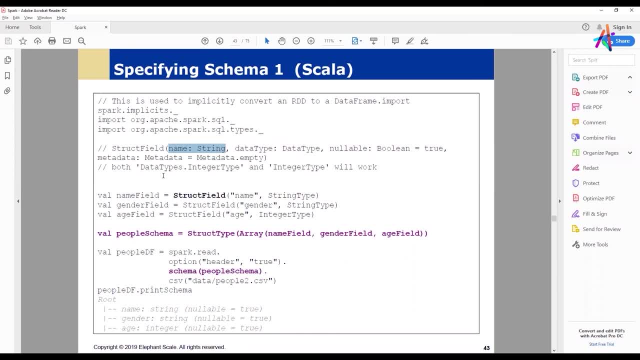 So we're, we're, we're. basically, I have a particular kind of structure And the the we're going to specify certain kinds of of typing on this. So now we're going to specify a name field And this is going to be. we're going to give it both a name. 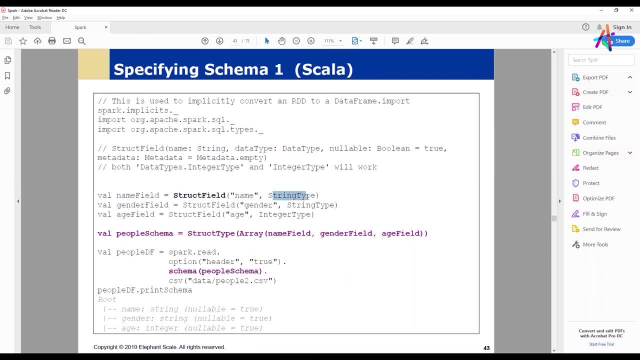 And and a typing for that name: Gender is also going to have a spring type And age is going to have an integer type. So what we've done now with our, our data set is we've we've actually started to put strong tags. 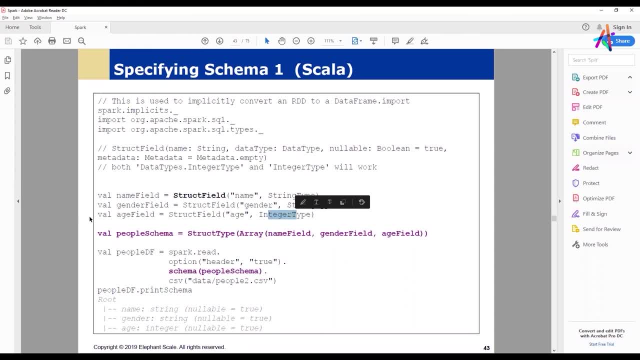 And we've put a little bit of typing on the underlying structure. So now we can create a schema Which takes the takes the name, which is which is it takes the name field, gender field and age field which we've defined here in terms of structure. 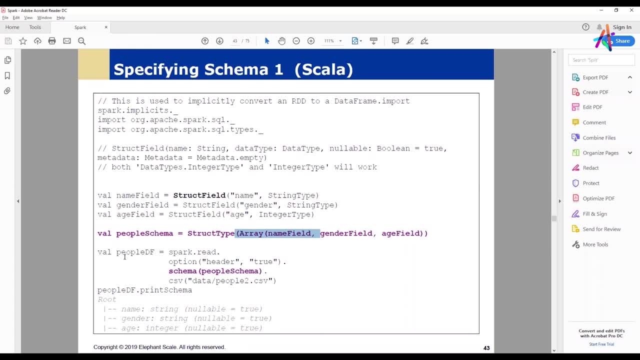 And now that we've got our structure, we can go and read This, this data, in a very, very efficient, a very, very efficient way. So here's read operation: the option header is true, but we're also now giving it the schema. 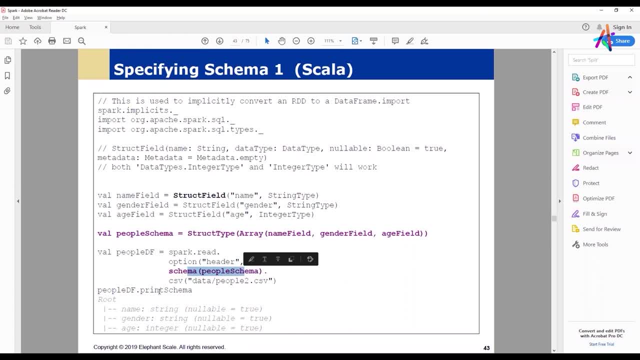 as we go, as we read through the CSV, and now when we print out the schema, we see that we've got an appropriately typed, typed object okay. so this is a definite improvement over what we were doing before, because now we've got a really solid structure, we've got typing in the structure and because we've got typing 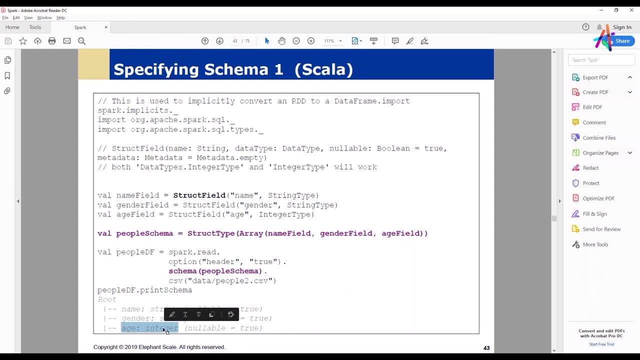 all of our serialization routines and a lot of the other routines we're looking at are gonna become much, much more efficient because we know exactly what kind of data we've got, instead of just looking at really a blob of characters or a blob of bytes. so we're gonna skip over the Python here. here's another. 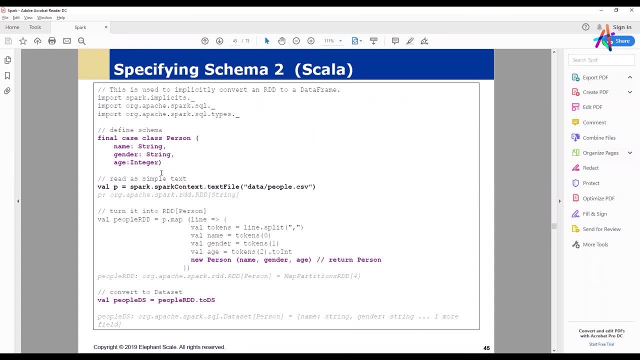 example of structure. in this case, we're defining structure in terms of a class and a class, and, but it's actually not necessarily the case if we look at the data itself. but it's actually the case if we look at the data itself. but it's actually the case if we look at the data itself. but it's actually the case. 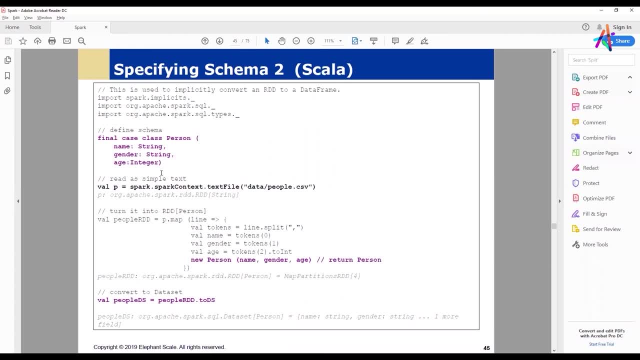 last definition and we can read the data in now as simple text. So we've got our CSV file, we read it in as a simple text. But what we've got here- unlike before, when we were just doing this with RDD and we were just imposing a structure on it- that structure was opaque to. 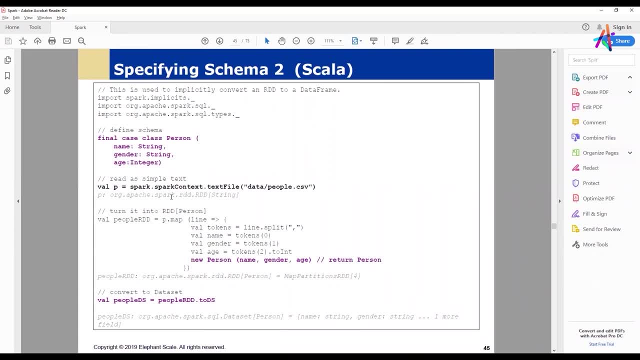 Spark. Spark didn't know about that structure. But what we're actually doing now is we're able to actually communicate to Spark exactly what that structure is. So we're putting this into a data frame by using this class definition, We're reading the text file and then we turn it. 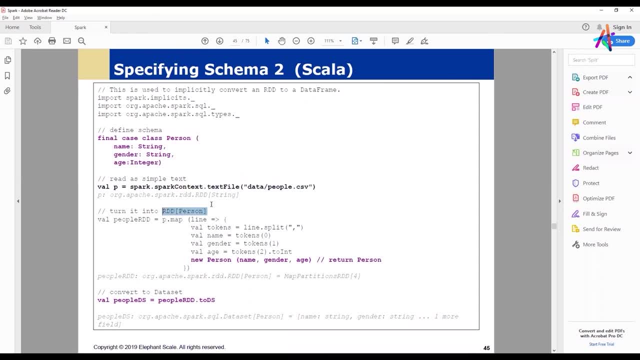 into a RDD person by going and splitting up the lines and creating a new object. Now, this is what we did not see before. Before we just actually split it up and we had the data in a form that we could manipulate, But it was, like I said, opaque to. 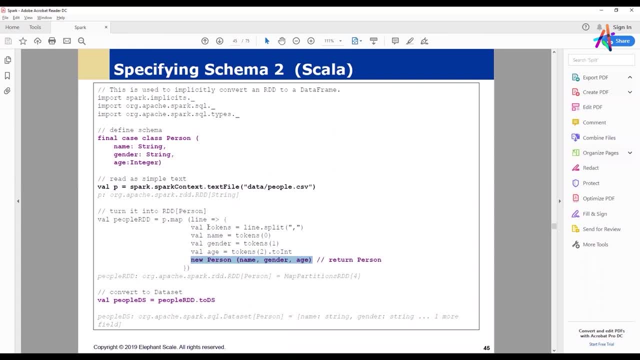 Spark. Spark didn't know what we were doing. Now that we've got this person object, we are actually able to construct this structure. So we're still not completely done, because even though we've defined the structure, we're still not completely done. So we're still not completely done. 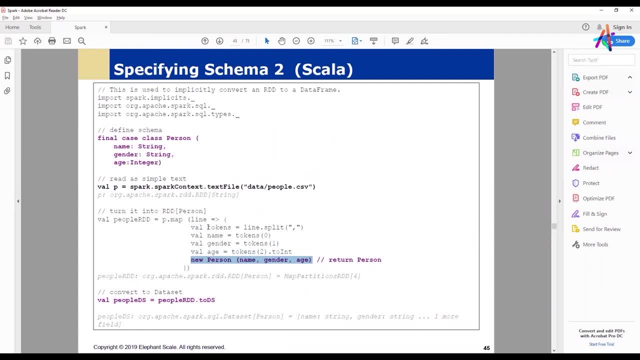 because even though we've defined the schema, defined the object with a strong typing, and even though we've turned it into an RDD of persons, we still have to convert it internally to a data set that can be utilized by Spark, and that's what happens here. So we've kind of imposed some 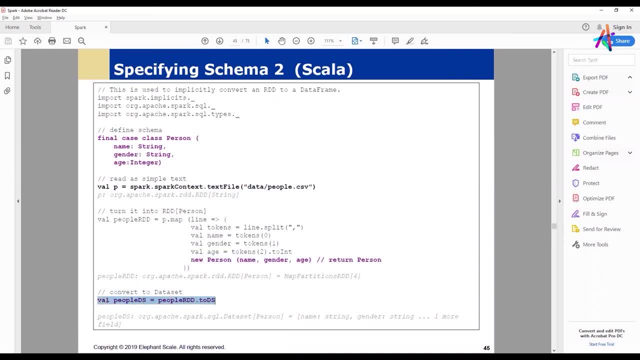 structure on the RDD, and now we're basically converting that into a data set so that we we are able to access the full ability of Spark. Okay, so here's the. it's a subtle point, but again, this is worth repeating. Spark cannot do optimizations on type data unless it knows. 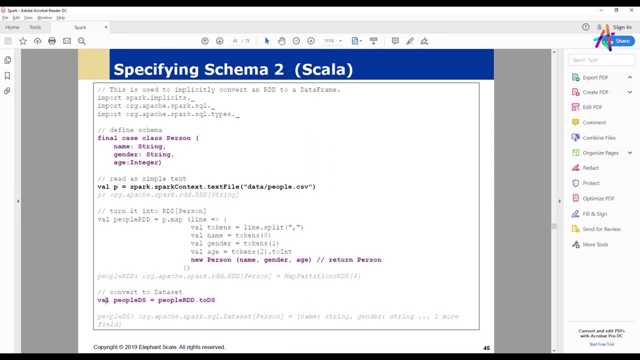 what the type is, and this is our ability to be able to communicate that to Spark. So this is where the data set is an enhancement of the RDD, because again, we're creating an RDD which has been been been been typed, and then we put it into into a data set. 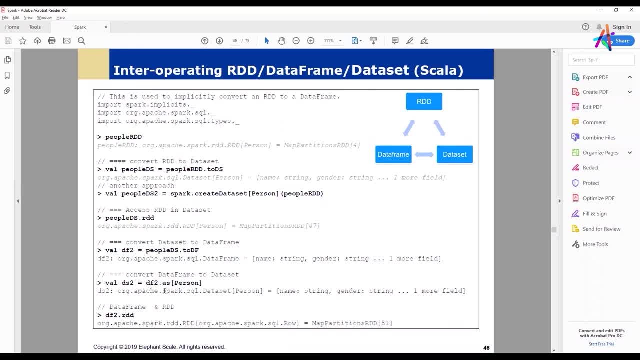 Okay, so here is the. so here we have the ability to move between these, these different formats, And again, we want to move between these formats because we may want to operate on the data from multiple, multiple points of view. So we have a people RDD, which is, which is an RDD of persons. 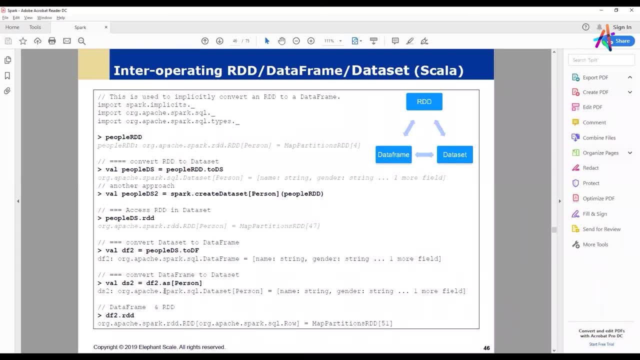 Now again the. the difference between this and the older RDDs is that we have, you'll notice, it says people RDD, because we've got a RDD full of people, person objects. That's the big enhancement on the, on the RDDs in the data set in, in, in, in the data set world, We can convert the. 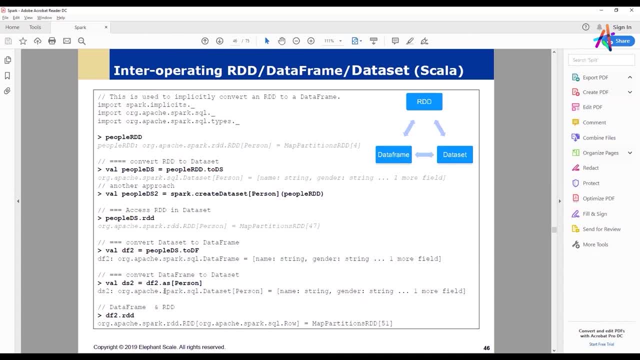 we convert it to a, to a data set, so we can work with it as a data set, And we can. we can do a number of different ways of doing that, that conversion, And we can also go back and still access the underlying RDD. We can put it into a data frame so that we can use data. 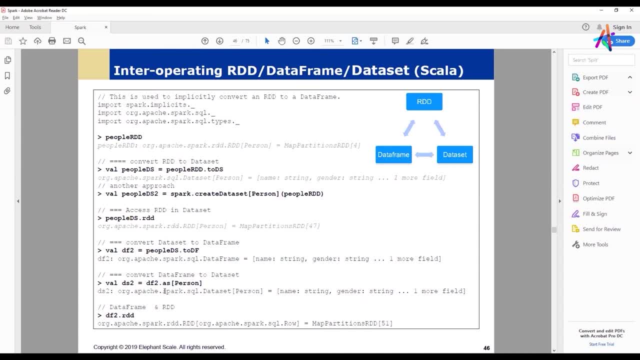 frame kind of operations, And we can also take a data frame and convert that to a data set, which just means that we're we're now using that standard interface with the data set And we can do do this kind of version. 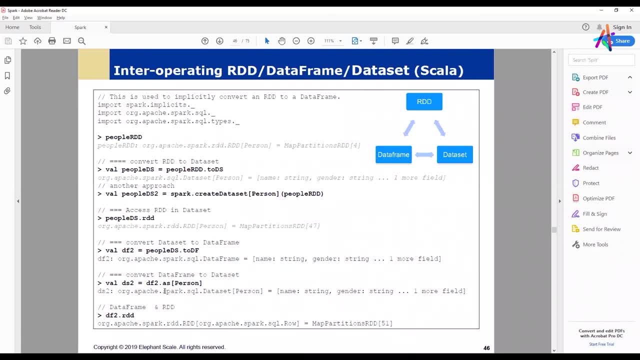 So what we're looking at is we're looking at a data set and we're looking at a data set and we're looking at here as multiple views into the underlying data. We can look at it as a data set, a data frame and an RDD, depending on how we we want to work with the data. So it's it. 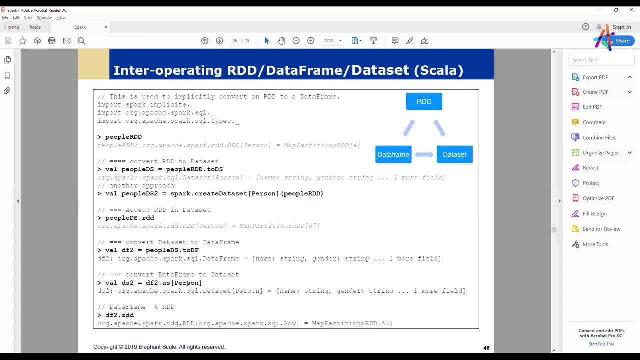 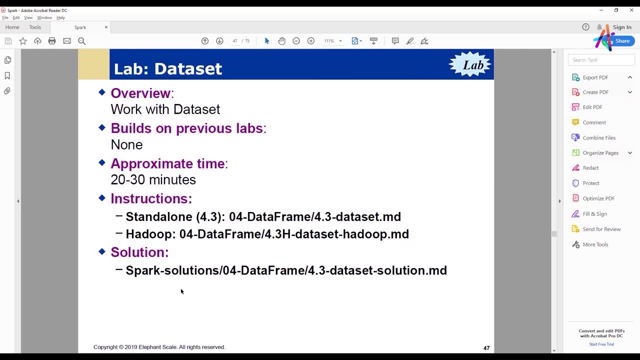 it. this, these conversions are are shifting basically our views of the of the data. Okay, So any questions before we we jump into a lab here. Yes, So in all of these conversions, like from RDD to data set, 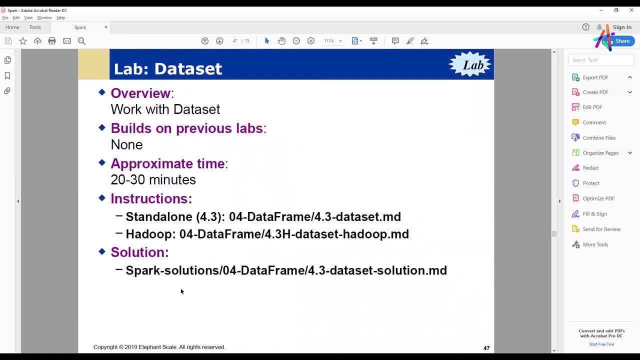 or data frame and back. is there any cost on those conversions or is this just like very thin wrappers around each other? Yeah, there is a cost, but the cost is really minimal because, as you said it's, it's kind of like different views of the underlying data. 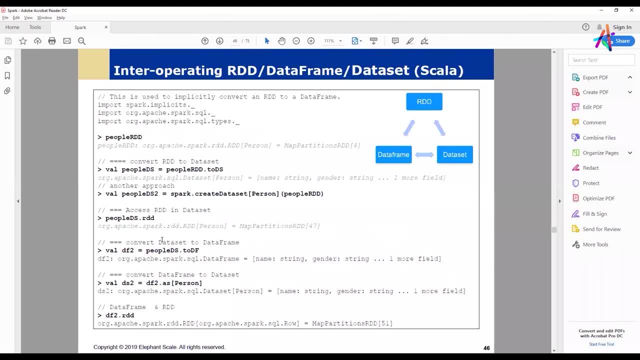 The thing that makes this really work is the is once you've got the, the data structured in some way, and you've you've got an associated schema. it really is representing different ways of looking at the data. So, yeah, you can, you can implicitly convert one back to another. um, if you think about how, how spark is, 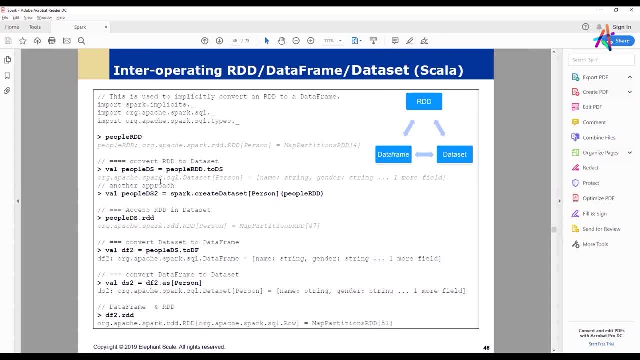 actually working. um, the, the, um, the um, the uh, uh conversions are basically just referencing different uh. we can think of it as templates that you're looking at the data through. so you're looking at the data through multiple lenses and uh. so i think you're correct- correct in saying: 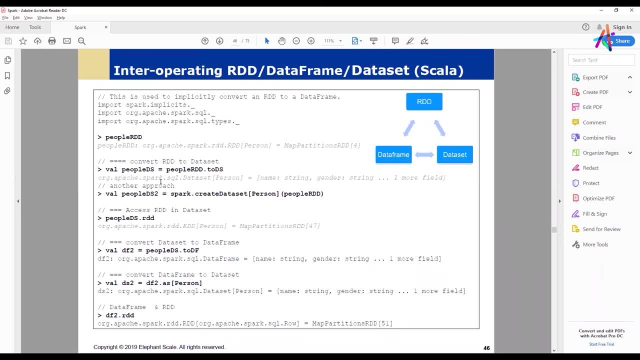 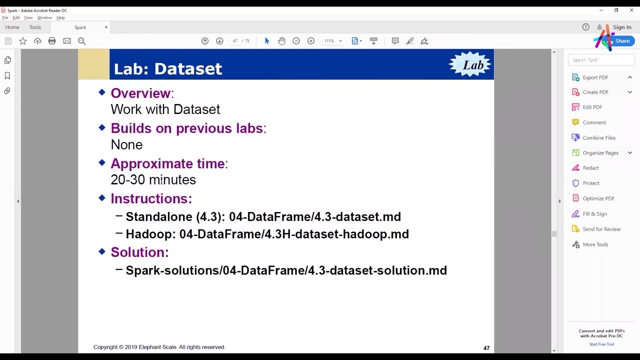 it's like wrappers, um i i think of it more as as being just different, uh different, uh kind of um views into the same underlying data. so, uh there, yeah, you're not convert, you're not moving the data around. uh, what you're doing is is, uh is taking different views of the data, the, so there, 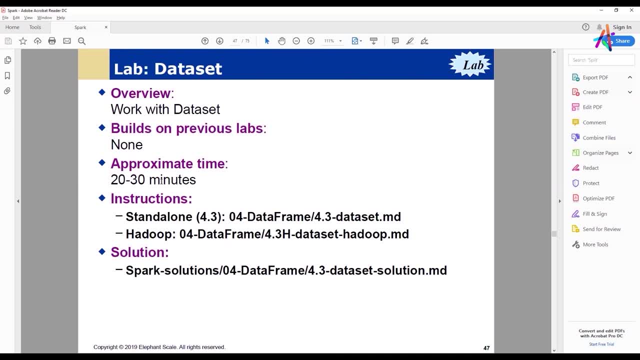 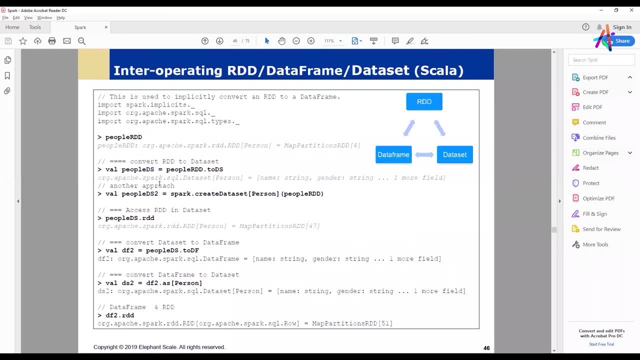 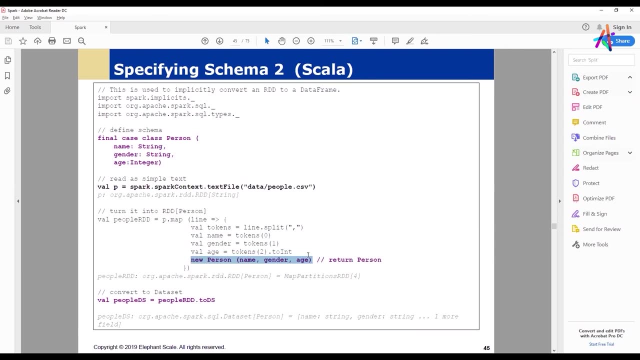 is a certain cost, uh, which is computational, but the cost doesn't involve restructuring the data. but the key point here is: is this, uh, typing of the data that allows this, this conversion? okay now, if we just had a raw rdd full of text, uh, we would have to do all kinds of work on it to try. 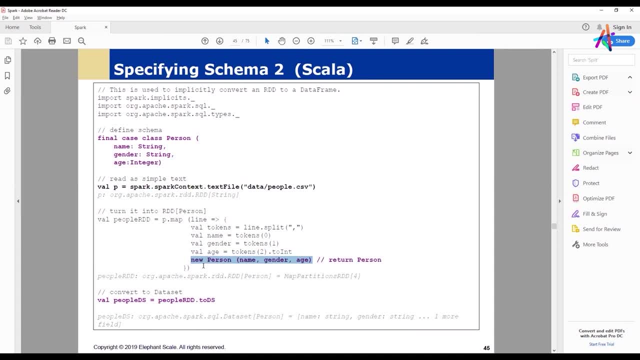 to get it into a form. we could look at it as one of these other things. but once we've got this underlying uh kind of structure in place- and remember, the schema is nothing we do to the data- schema is a description of what is in the data. so, uh, we're not really doing any converting of the 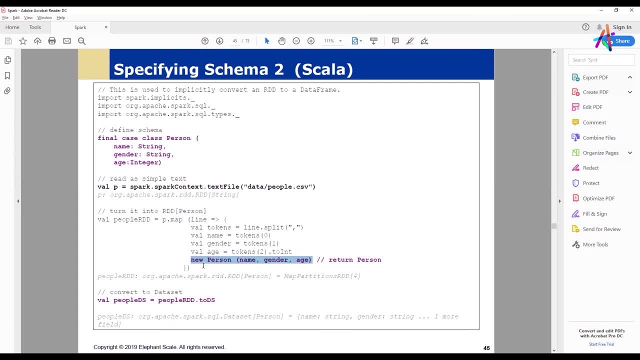 data into a completely different format. it's kind of in the same way that a view into a relational database doesn't actually um, doesn't actually create new data or do a transformation of the data. it's it's basically just giving us a a different perspective into the data. does that answer your question? 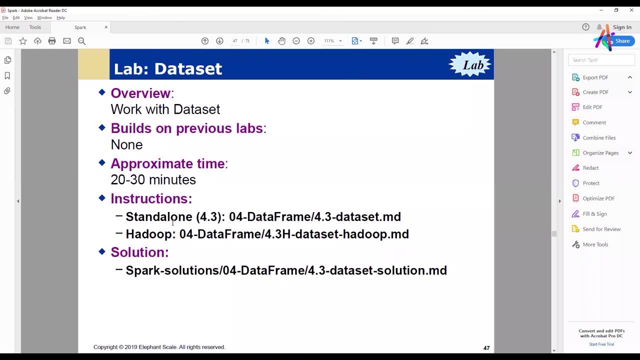 yes, and i have another one: go ahead, go ahead, um. so if we have a data set and we have this, uh, what's people or person type? um, so we are giving spark, uh information that it can leverage to, let's say, optimize, for example, uh, when encoding data, uh, to give you memory, um, do we have the same? 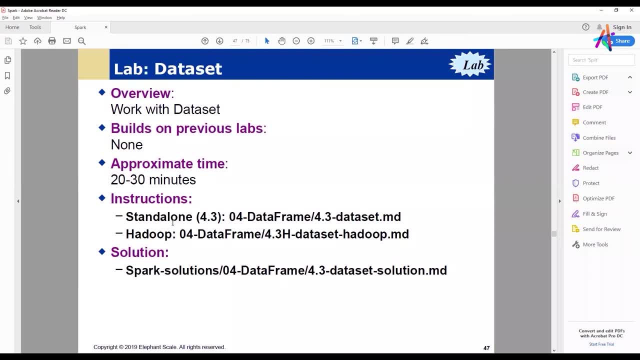 benefits of the data set uh. to give you memory um. do we have the same benefits of the data set um? do we have the same benefits or similar benefits or a subset of those benefits when we uh type an RDD with this person case class as well? I mean by having this case class in there. can. 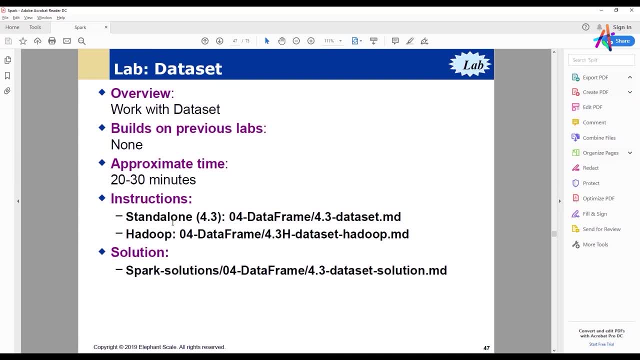 the RDD become more efficient, in terms of cache, for example, than just a string rdd. yes, yes, and that is that is one of the main motivations behind this, this notion of, of, of having the imposed on the, on the RDDs, is that it allows for significant performance and 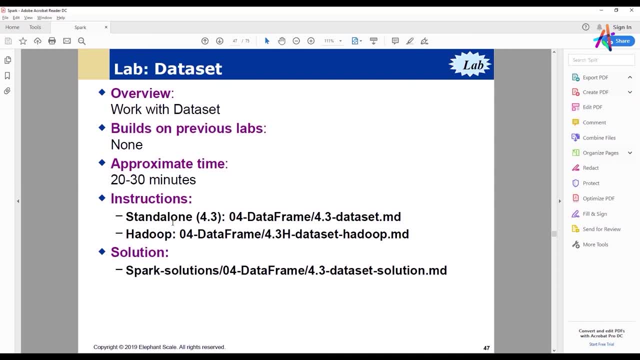 improvement on caching and other things, because now there's structure and data typing, so appropriate optimization decisions can be made and in that sense, is there an event benefits in moving from the personality into a person data set? in terms of optimization, no, because the underlying data is still the 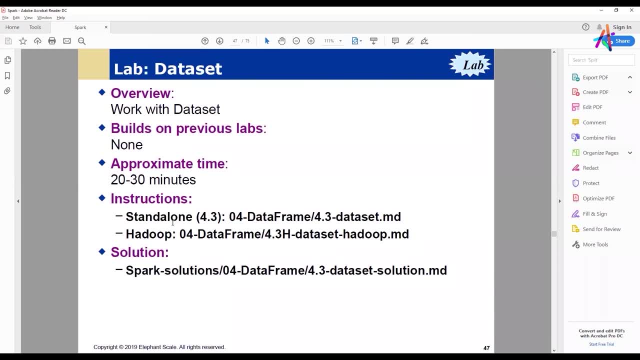 same, just just, but the the it's. it's the fact that we have now typed that underlying data in in in terms of persons- whether we're looking at a data frame or as an RDD is just our view- into the data, but the data now has a way of. 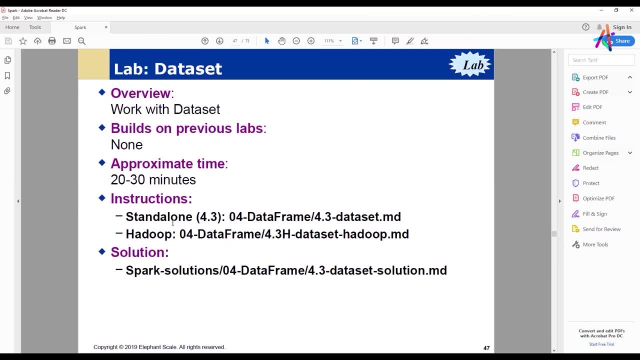 being chunked into structures, and this is chunking of the data so that that makes things efficient. so, for example, now, instead of looking at, this is just a long string of text. each row is this: each row is a string of text with the name and, and, you know, age. 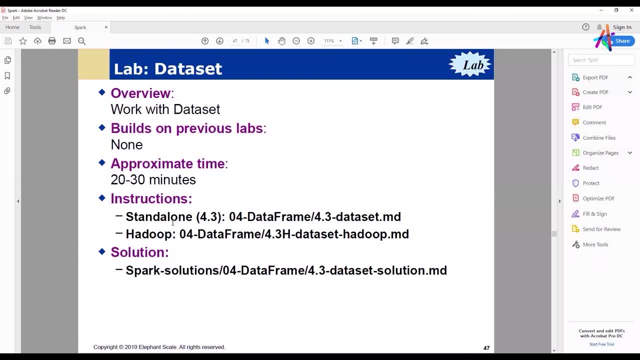 and and whatever, and gender, instead of just looking at it as text, each, each one of those, those, those chunks, is now been been typed with a small schema on it. so the the idea here is that once we've kind of schematized the underlying data in in terms of these types, it's very easy. to get a lot of data out of it, and it's very easy to get a lot of data out of it. it's very easy to get a lot of data out of it and it's very easy to get a lot of. it's very easy to get a lot of data out of it and it's very easy for us to go and. 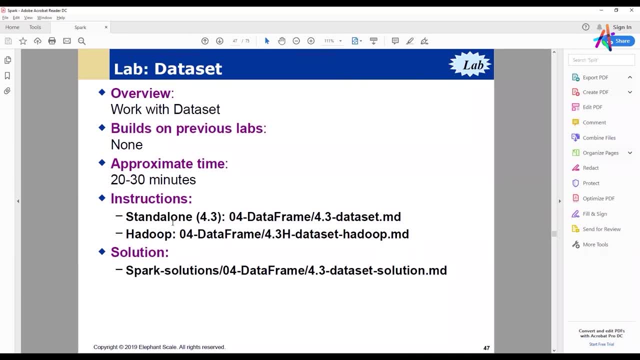 to get a lot of data out of it and it's very easy for us to go and build a representation of that in the tabular form and also we can go and just look at it as an RDD. but now the optimization really starts to take place. 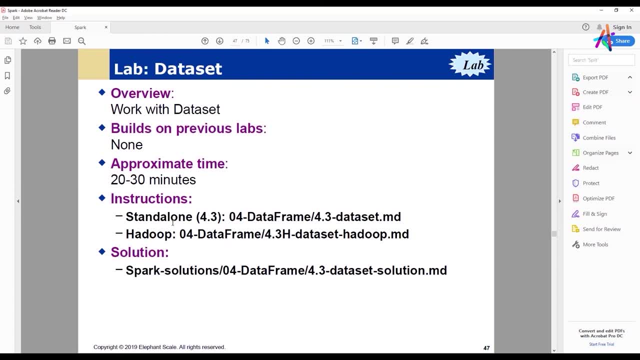 when maybe it's something to go and cash that or to serialize that out, because now we have a lot of information about the underlying types and that can be used to make optimization decisions. so this is really kind of a an approach of an optimization decision. so this is really kind of a an approach of 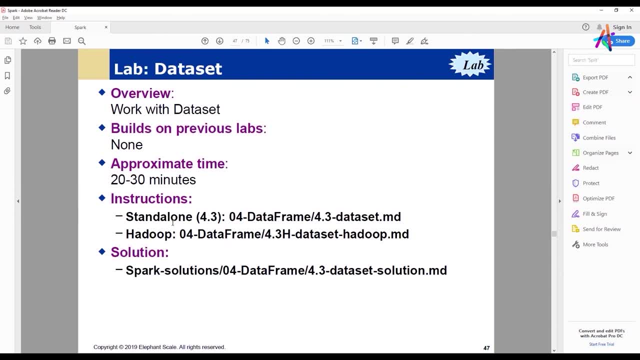 of imposing a certain kind of structure, And once that structure has been imposed, it allows these multiple views, but it also allows us to do a lot of optimization that we couldn't before. I think did I answer your question or did I kind of go off on a tangent there? 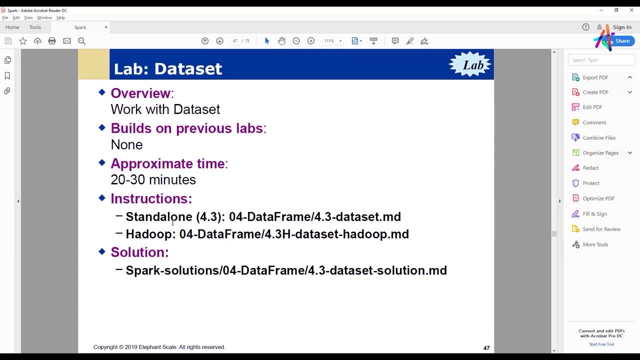 Yes, that's clear now, thanks. Okay, good, So then it is my understanding that the conversion from the RDD into the dataset- assuming that RDD is already typed, what it gives us is just access to higher level APIs, right? So data doesn't change, optimization doesn't change. 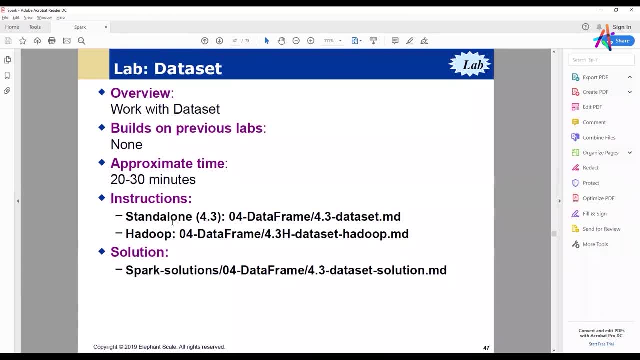 but it gives us access to again maybe this SQL interface or group by operation or all these higher level API. So that would be the reason why at some point, we might want to move from RDD to dataset. Is that right? Yeah, and I think that one of the two things. 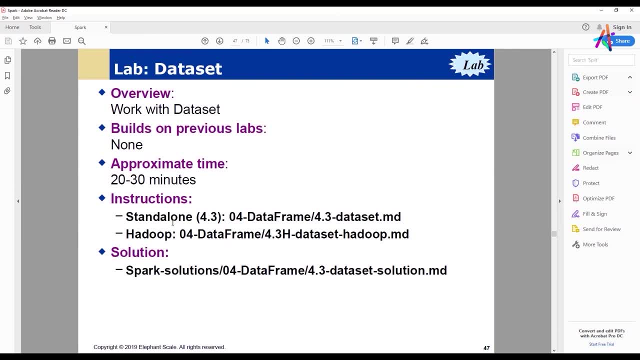 you have to look at in deciding to do that conversion are number one performance issues as you start to think about caching and serialization and we can start to get better performance in the dataset. That's one argument. The second argument is: what are people using the data for? 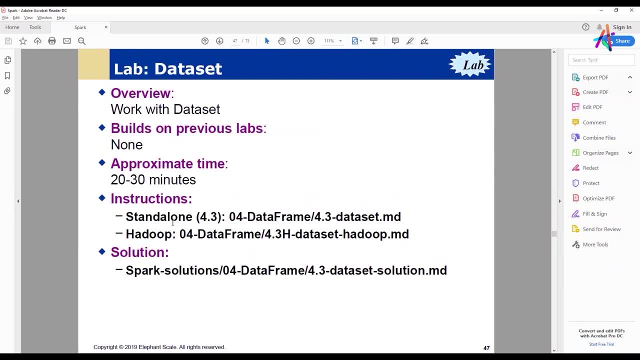 So if there's a lot of data analytics and a lot of people experimenting with queries that you clearly want to get into it from a user perspective on the approach of you know what's going to be easier for my users to use, What are their requirements for the use cases? 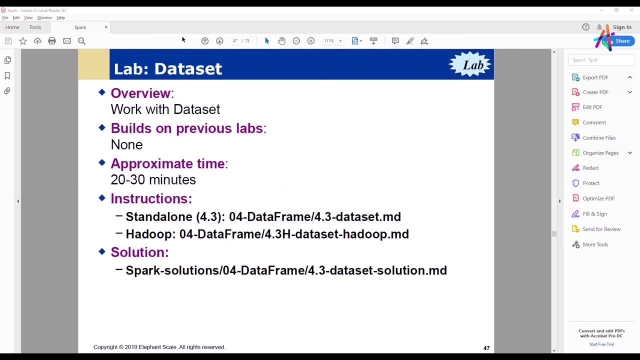 Does that make sense? Yeah, so I think in Brilliant Group we finished with the task and we had a discussion on how exactly performance or memory, or both performance and memory, are optimized with predefined schema using the data frames, If you work with them as an RDD. 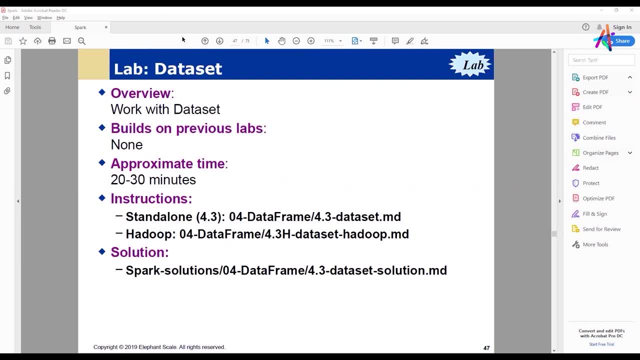 Okay, I'm sorry. can you repeat that? There's a lot of echo. So we're loading data using data frame API or dataset API, right, And then we convert it to RDD and continue working as an RDD. Do we still have the transitions we got? 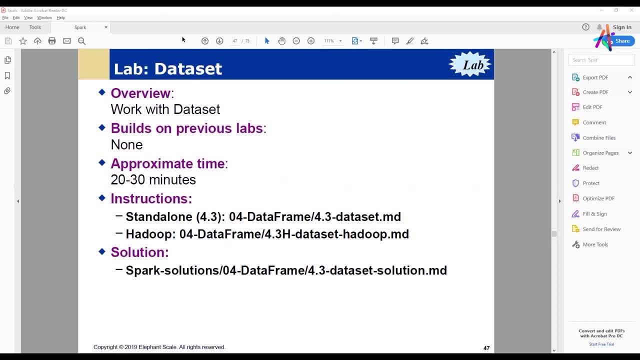 for data frames and datasets. Do you still have the what you got for data frames and datasets? Transitions, like not loading everything, Okay, good, Yeah, in terms of the, the caching and optimizations: yes, In terms of the optimizations of queries. 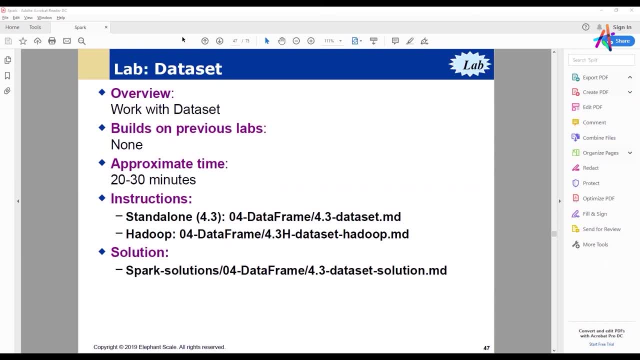 and operations generally. no, Because now the operations you're performing are in a form that can't be optimized through things like Catalyst. But the other kinds of optimizations which are based on the underlying structure of the data, like the typing, yes, you do get that optimization. 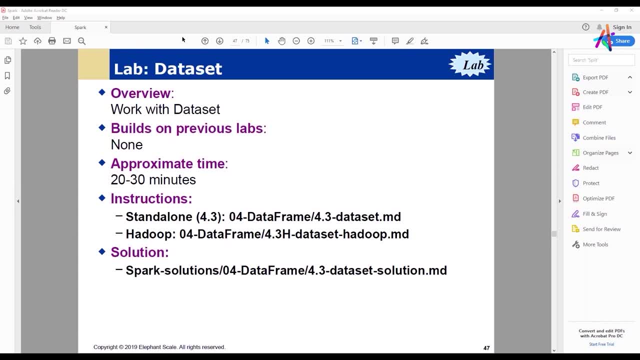 So what exactly are these memory optimizations we have, we're still having? Well, this comes from the typing and the fact that once you've got that structure on the underlying data, that can be used for the optimizations Now, whether you view that data as a table. 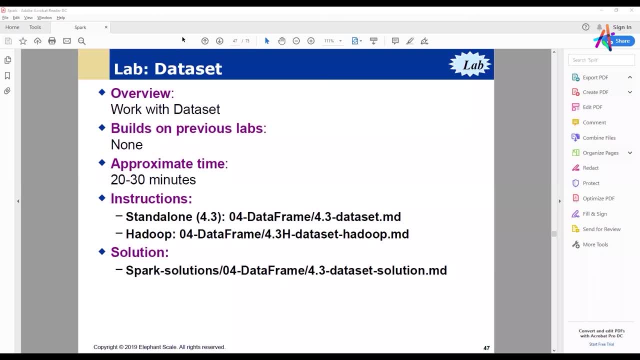 or an RDD is a different interface into that data. okay, Let me simple. Do I make sense? I guess it does. Okay, But I still didn't get the part about the memory optimizations. what exactly is optimized this way? Okay, 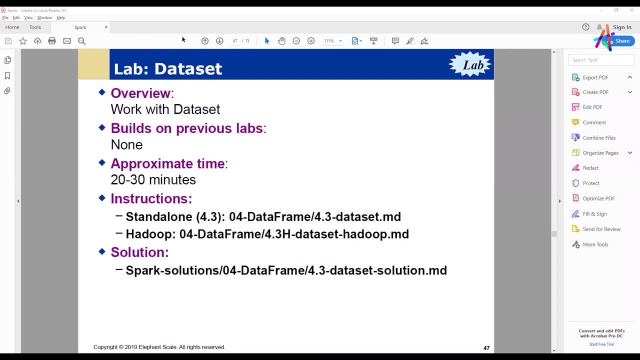 Well, when you talk about things like serialization, for example, okay, Serialization, if you know what the data structure is, is and the type of the data, you can make choices about serialization which you couldn't otherwise, and that's just sort of an example of that. this is something we're getting into more detail next. 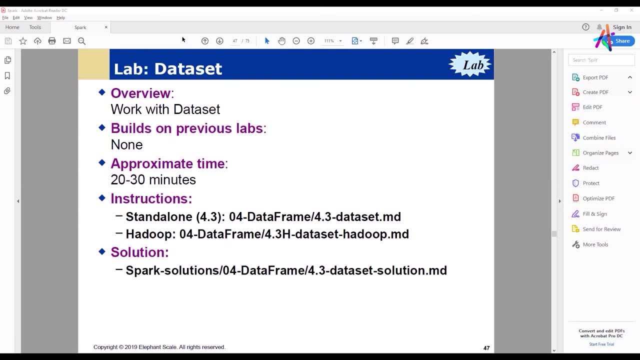 week about those particular optimizations and how those optimizations work. okay, but generally, if i know that i've got, say, integer data versus string data, i can, i can think in terms of optimizations of how i'm going to, to, uh, to, uh, to uh to, to work with things in memory and also. 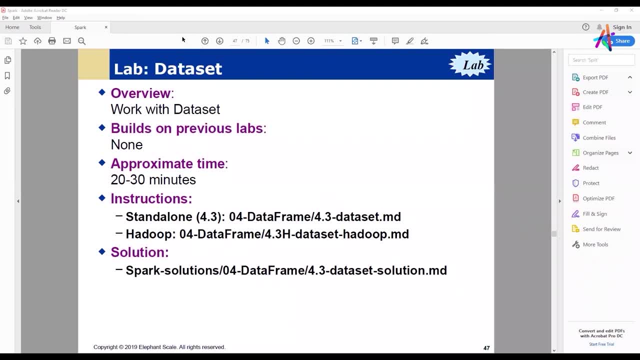 storage, yeah right. and the other thing too is, if i've got, if i've got structured data, then you know it's, it's, it's there. there's a certain access efficiencies. so if i have a long string, uh you know, and i want to access something, i'm often doing some kind of linear search through. 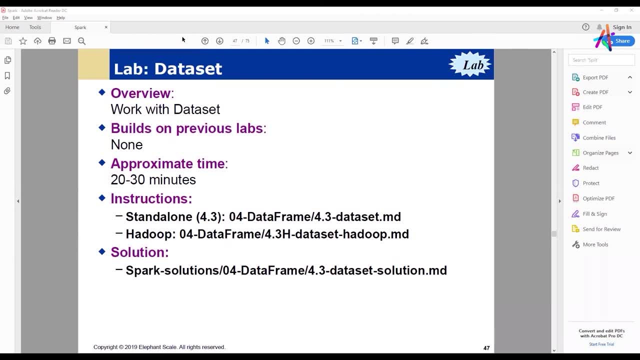 the string, uh. but if i have, say, chunks of data that are of a known size, it's easier for me to do that. so i'm going to do that, so i'm going to do that, so i'm going to do that for me to to get to to a particular point, uh. so let's suppose i've got a bunch of person objects. 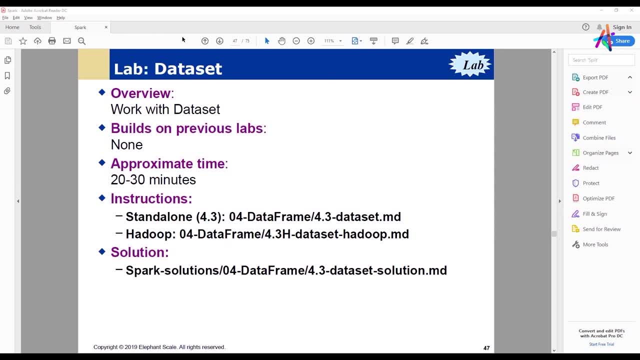 and i know that the person, objects have, have, say, a fixed size. i'm just using this as a hypothetical example and i know i want it. i want it to search for a particular uh element in the string. and this is not necessarily with spark, which is an example, if i, if i, if i don't know that underlying structure. 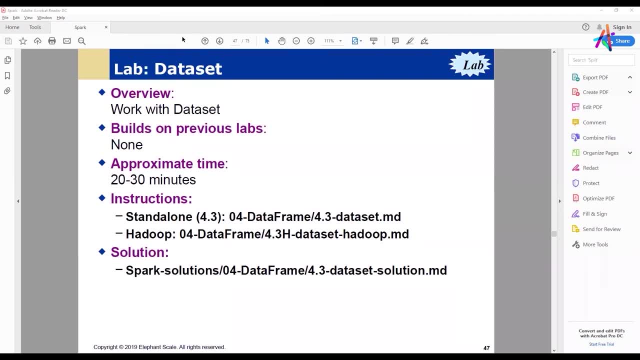 i have to start at the beginning and kind of search all the way through from beginning to end. but if i know that every n positions on i'm starting a new object, i can. i can optimize my search by looking at position one and then position one plus n and the position uh, one plus two n, and i can. i can speed up a lot. 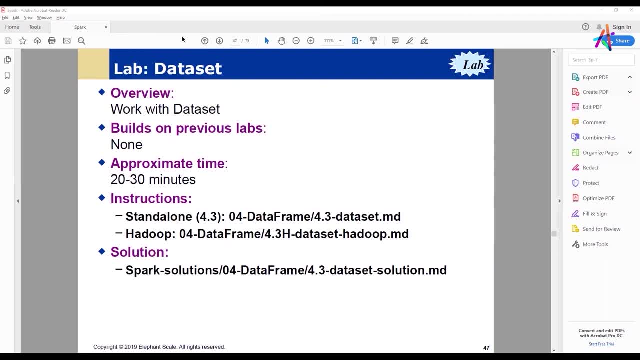 of optimizations. so knowing something about the structure of the underlying data, knowing something about where things are, sort of positionally, enables me to do various kinds of optimizations. okay, does that make sense? absolutely, okay, all right. so this is why that typing is so important and this is why python. 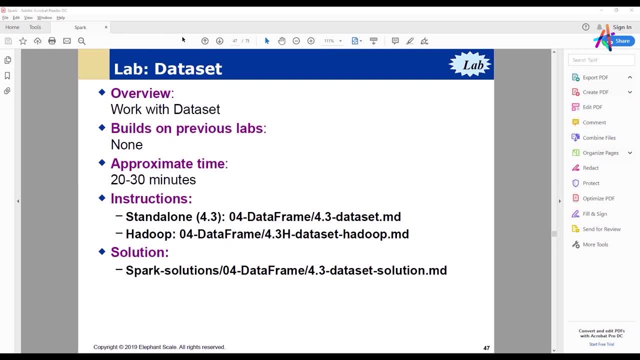 has such a problem with it because python is not really intended to to do that kind of typing. so python can do some of it, but python has struggles with a lot of a lot of it. all right, so Can I ask one more question? It's kind of related then. So I see we are sort of providing. 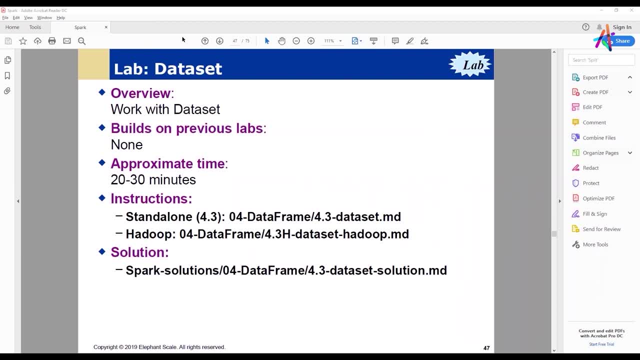 types in two different ways. So one way is, let's say, when we read the CSV and we provide this schema, right, Like this: yeah, extract fields and so on, right, Okay, So here we are providing types for the data frame or data set And then like, separately we are applying a case class in. 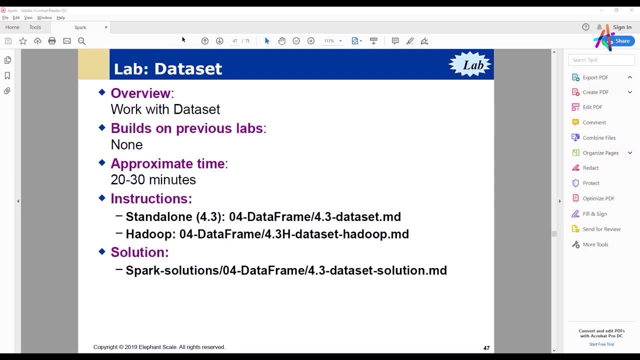 color right? Don't we already have the types, if we provide this set of extract fields already? Yes, There are two different ways of doing exactly the same thing. In the first one, where you're inferring it, you're doing an implicit typing, In other words, you're reading: 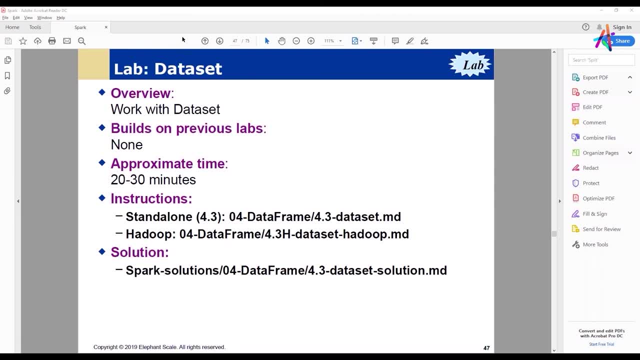 the data and you're doing an implicit typing. In other words, you're reading the data and you're doing an implicit typing. In other words, you're doing an implicit typing. In other words, you're reading the data and inferring the typing from the data And generally that kind of operation. 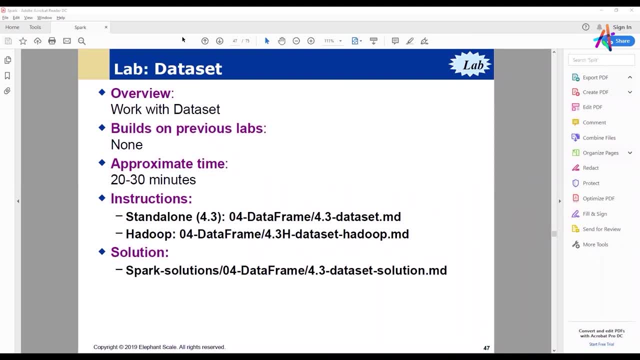 can be expensive because there's an inferencing component involved. okay, So in that view, we're saying we'll let Spark- well, in the data is an implied structure and we'll let Spark figure out the structure and pull out a schema from that. In the other way, what you're doing is: 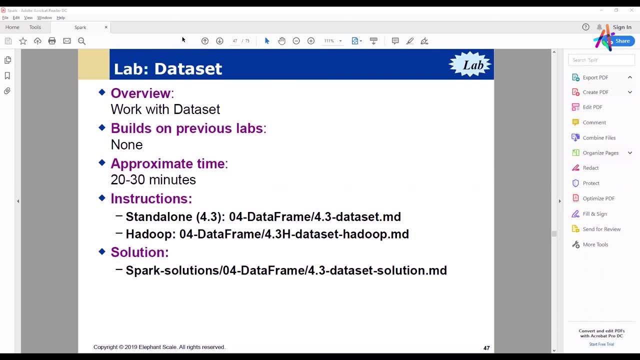 you are explicitly typing the data, You are defining a data class and then you are explicitly putting the schema into place to do that data class. So one's explicit, one's implicit. You can use either approach. Some use cases. the implicit approach is going to be easier, particularly if 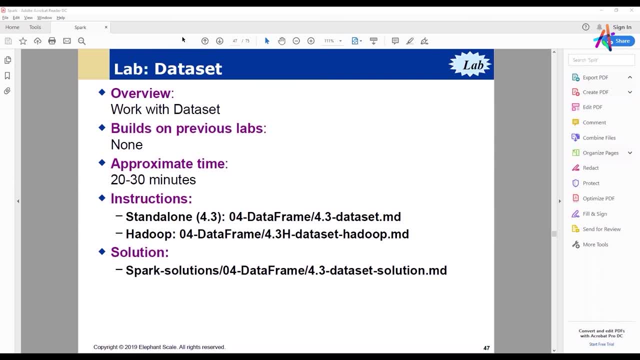 using data that is really really well structured and has associated schemas. The implicit approach is going to work really really well. But you know, if we're working with, like I said, JSON data or CSV data, it may just be expensive to do it that way. So we can switch over and do it explicitly. 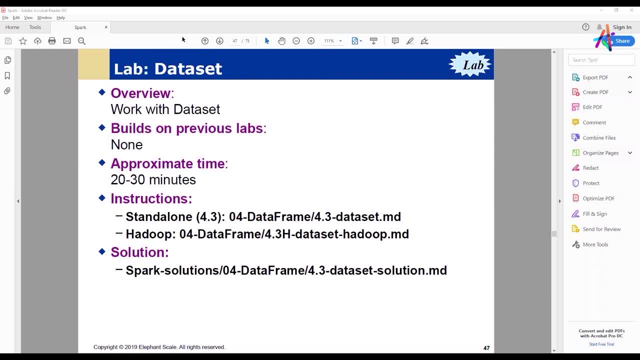 Or sometimes we may do it explicitly, simply because we want to have that explicit declaration there, so that it's something that is well-documented. Does that make sense? And if we think, for example, from the Python perspective? I can from Python read a CSV file. 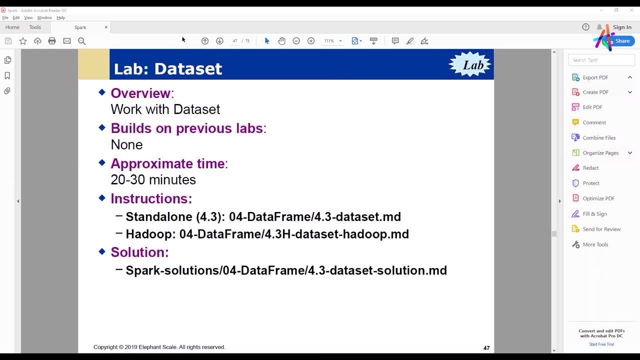 And, at the time of reading, I can provide this array of struct fields providing a very explicit types, And therefore I can get a data frame that is typed And therefore I can get all of the optimizations that we are talking about. The only thing that I'm not getting from. 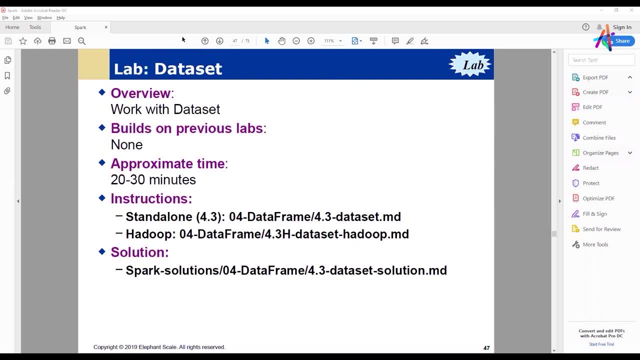 this dataset API is the compile time safety right, But in terms of optimizations, I can get exactly the same thing from Python, just because I can provide this schema via these struct fields. Okay, Yeah, Yeah, Optimizations are not dependent on the language API that we're using. 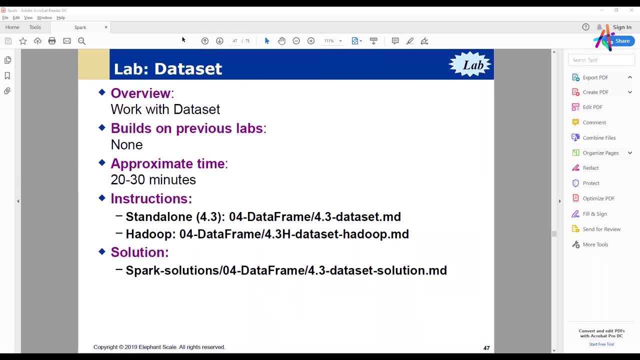 The problem with Python is that there are just certain things we can't express in Python, Or I'm assuming this. I'm not sure of the exact details, but my inferencing is that there are just certain things that we just can't express in Python that we can express in Java. 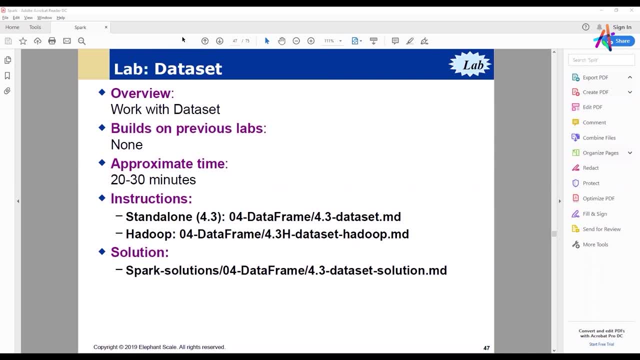 and Scala in terms of typing, which makes just the API for Python somewhat problematic. So whether we're using Scala or Python doesn't change the underlying optimizations and things that's happening within Spark. It's just that the Python API just doesn't have the full 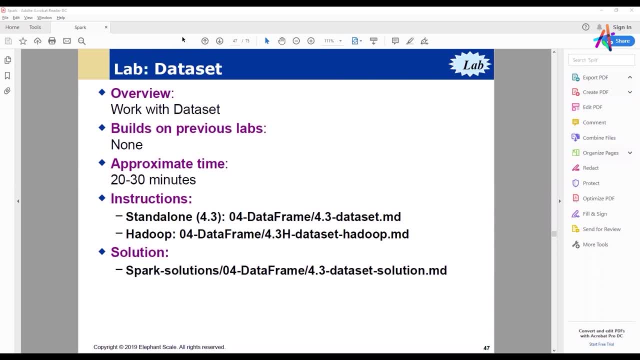 functionality implemented And I have a suspicion, based on what I was reading, is that that may change in the future as somebody puts some work into it, But it's more an issue of trying to figure out how to do the language bindings to the underlying API. 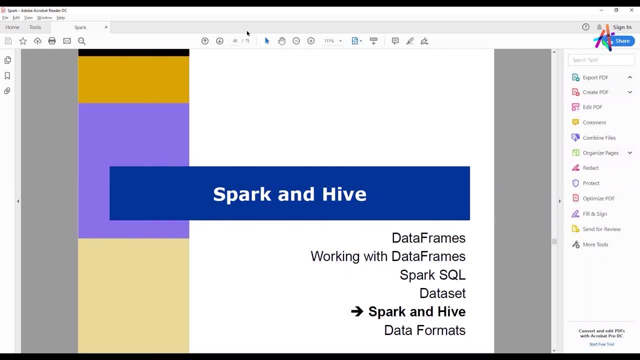 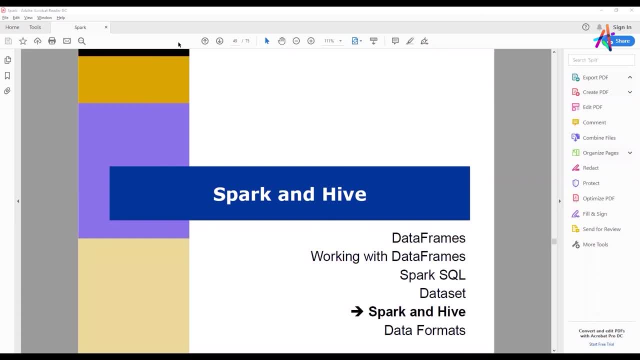 Okay, Yeah, Yeah, We're all here. Okay, good, I was just worried that Berlin may have gone off and got sidetracked with something there. Almost, Almost, Yeah, well it's. you know the problem with taking breaks if you're actually in your. 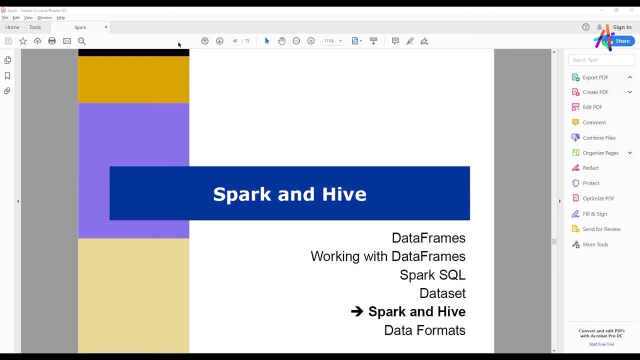 office is that, Yeah, as you're going to go and get a cup of tea or a cup of coffee, somebody always comes up to you and says: could you just have a moment? you know, i know you're in club, but could you just have a moment? 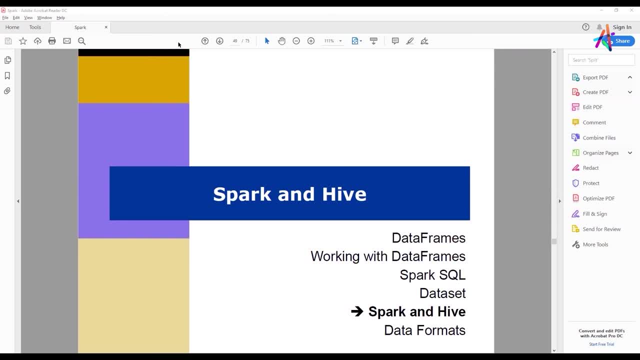 and then you spend your time just trying to get rid of that person so that you can, you can get on with your life. so, um, it's it's always an issue. it feels like we are the only ones. okay, all right, okay, so, um, now, are you guys familiar with hive? 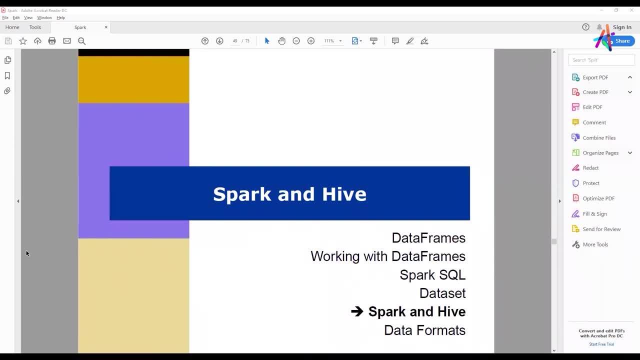 no, no, okay, okay. well, i- i i'm not a big hive person either- uh, because i really haven't had much opportunity to use it. so basically, just to give you an idea of what hive is it's. it's basically a data warehouse that is kind of built on top of a hadoop cluster and um. 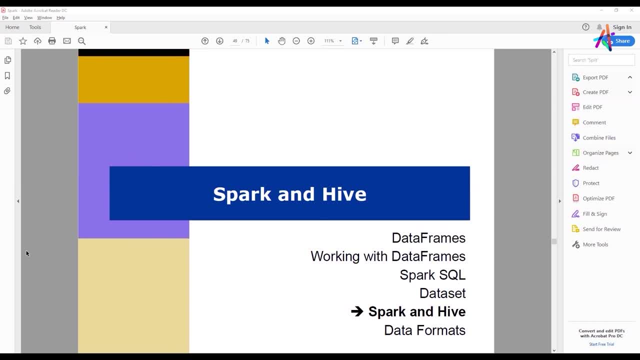 it allows you, uh, with, with, uh, with all of these kinds of of of things, with, um, uh- and we'll go back to that question before- about sql: um, when we're looking at these kinds of analytics, um, with data, there is a subset of sql that really isn't applicable. you know things. 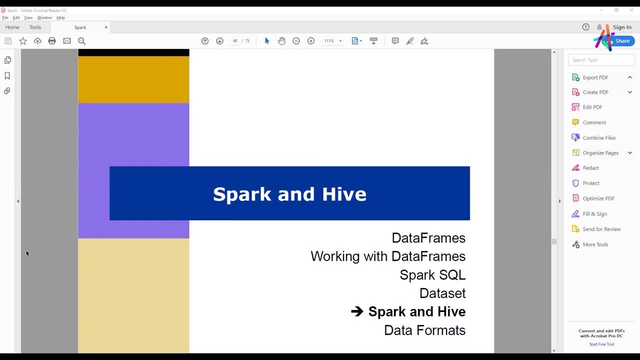 so. so sql itself is primarily um useful for transactional data, you know, with normal ized forms, and, and, uh, you know you, you want to make sure that you don't corrupt your data, uh, when you, when you, um, when you insert records and delete records, and there's this constant. 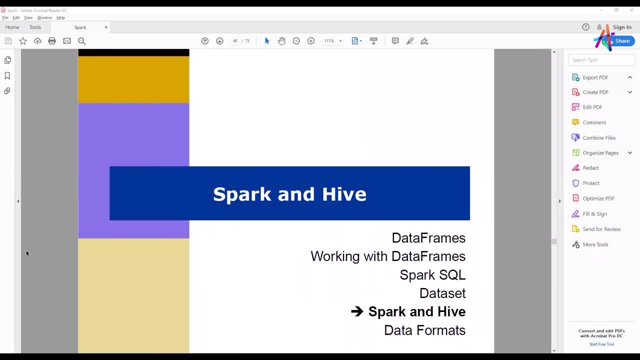 notion of data in motion and data data shuffle- i don't like to say shuffling- data constantly being being modified and so we have things like normal forms to present. against that, in fact, i was just talking to somebody, a class, a couple weeks ago and they said: why should we? 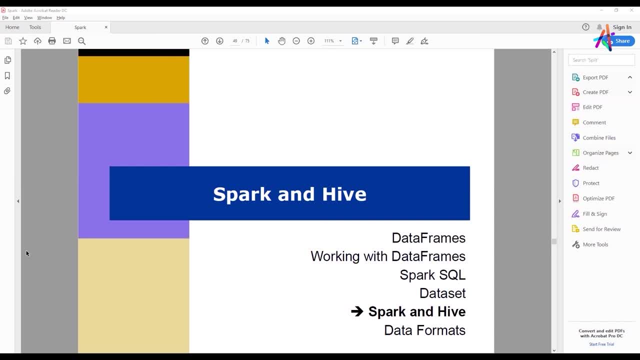 have normal forms, and i had to quote mitch hedberg who said: uh, computers, um, allow you to make mistakes faster than possibly anything else in the world, with the exception of handguns and tequila. and if we don't have things like normal forms to control that, then we, we, um, we, we don't. so a lot of the sql model is built around not queries, but is 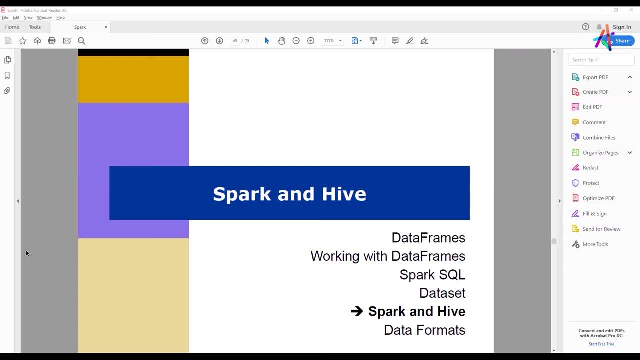 built around the data update and the, the building these, these structured data forms. the data that we're working with in spark is generally not transactional data, so a lot of the sql stuff that deals with updates and deletes and normal forms it doesn't apply here, so so but 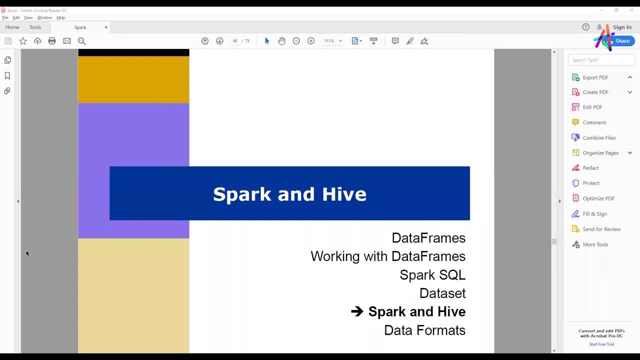 we're primarily focused on queries. so when i was making that comment earlier, i was trying to think: you know, is there anything about the querying that that really is is different in spark sql? and i guess i should add there is that. that is that spark is not really going to to to be, if you're. 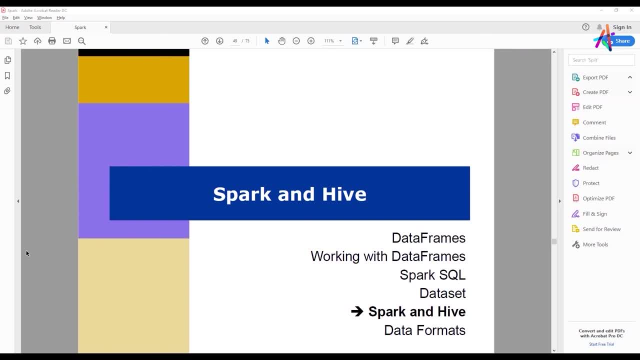 if you're running update queries on using spark, you're using the wrong tool. uh, it's just not. it's not what spark is for. so, uh, i i'm thinking in the context of um, of, uh, you know, just being able to query data is primarily what we're looking at, and being able to transform data, but we're not necessarily 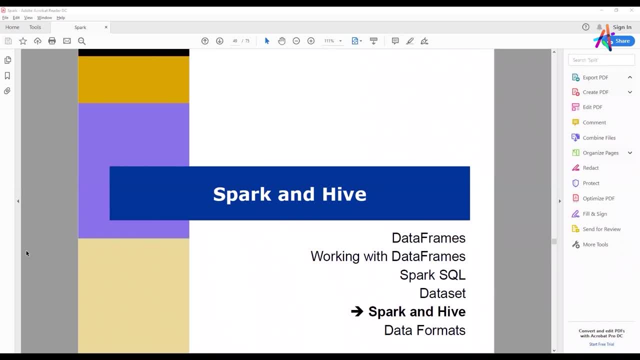 interested in transactional types of operations. so anything that that sql does that's highly transactional is generally not supported in these kinds of of sql, like environments, and if they are supported they're not. they're not very effective. so hive represents a data warehouse type operation or data warehouse type structure that's on top of the dupe and it has its own version of. 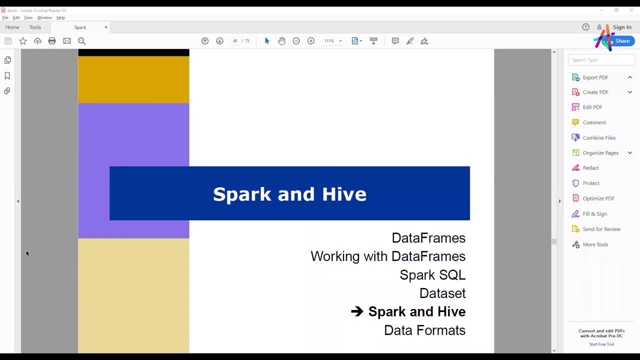 of of sql, which, um, which, again, because we're working with a sort of analytical kind of data rather than transactional data, doesn't really do a lot of of the updates, and because it's also a data warehouse with sort of uh the all the implications of, we're not going to be modifying. 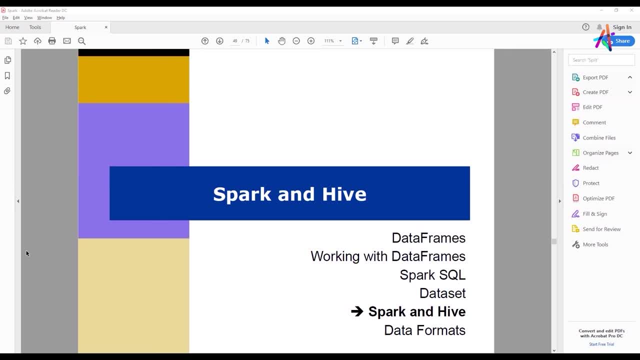 data. once it's been stored, uh, all we're going to be doing sometimes is restructuring it and looking at it in different ways. uh, we can throw out a lot of the sql stuff that that need has to be that's associated with with the data data modification. so, uh, the the hive ql is a subset of sql which is primarily query. 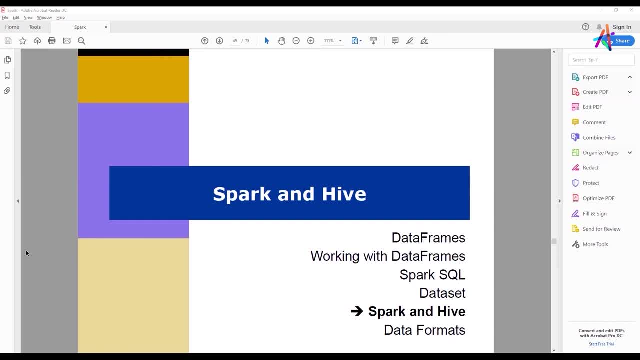 based and it also has a couple of of of uh, of other um parameters and commands that that relate to the fact that it runs on a hadood cluster. so there's there's a little bit more that you can do with it, but it is. it is uh, primarily a. 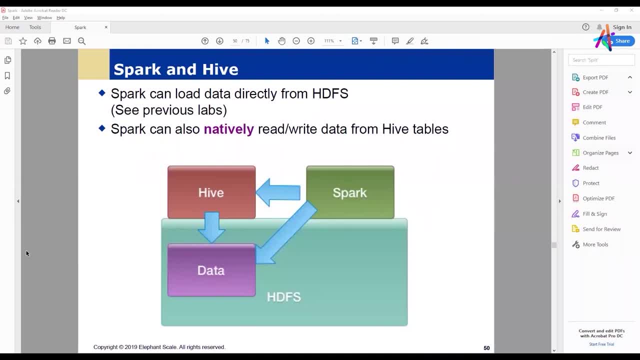 primarily a data warehouse, um, uh model, um. one of the things that hive does is um, is, uh. it also um creates tables and, like i said, i'm not a big hive person, but i do know that i'm not sure if the tables are actually structurally created. i don't believe. 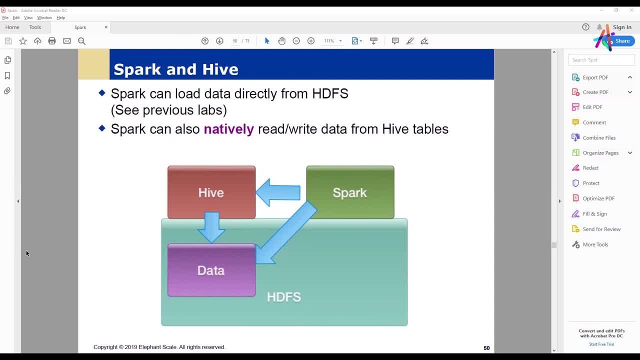 so, uh, what i believe is that table descriptions and schemas are kept in a separate database, uh, and that database, basically uh, contains a schema and structure descriptions which are then used to to format the queries which are then executed through a variety of map reduce kinds of of operations. so spark can manage the data directly in hadoop or it can utilize hive uh. 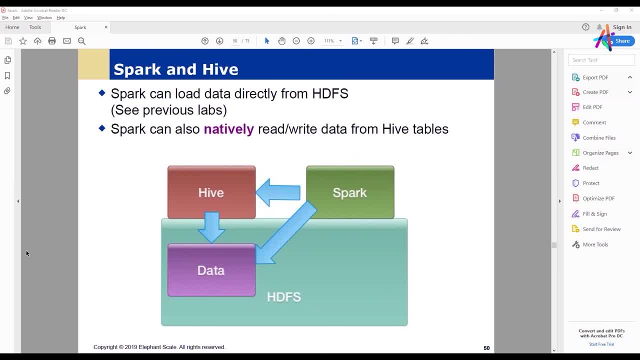 tables um, which is an, a structure imposed on the underlying data. so, uh, it depends sort of on the use cases to as to how you've got stuff. if you're using hive, then this is this is an appropriate way to do it, and if you're not using hive, um, there may be an advantage to actually thinking in terms of. 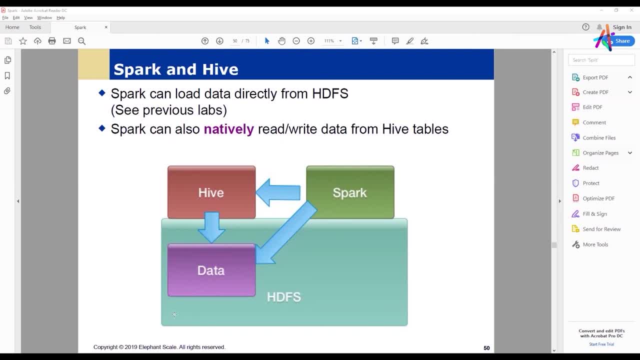 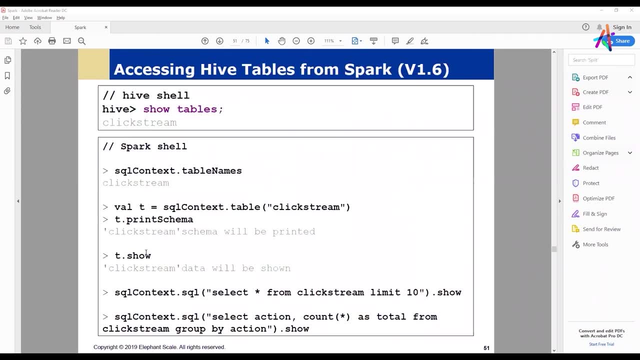 of using it, or there may not be. so, uh, hopefully, by the time we go through the end of this stuff, you'll have a sort of an idea of whether or not it's something that's that's useful for you. so hive tables can be thought of conceptually as tables like everything else. uh, so we're, we can go. 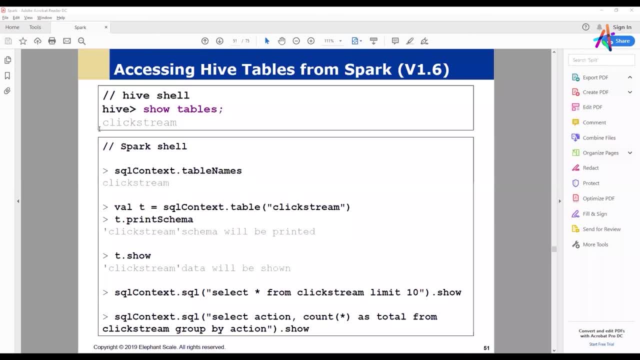 into the hive shell and this is going to look very much like any kind of standard sql type of shell. so we have show tables and it shows a table of clickstream. uh, it gets the sql context and this hive context is available in that spark object. you can. i think it's also in the sc. i don't know if. 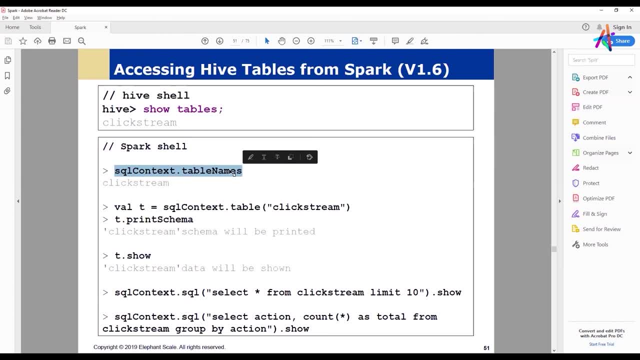 it's the object, but it's certainly in the in the spark object you get in the spark 2. there is a hive context inside that, so you can actually access a hive context in that spark object. uh, so now, if you're working here in a in a hive shell to the show tables, um, now in the in the 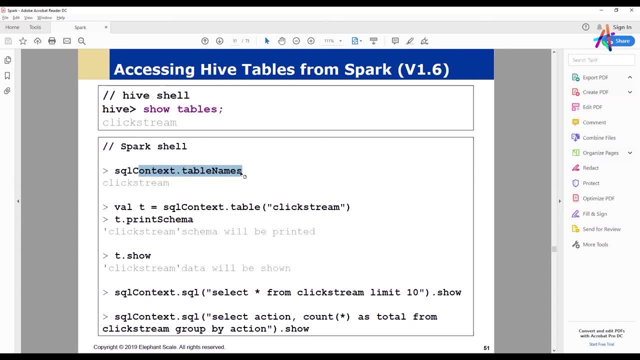 spark shell, you've got an sql context which can uh do a similar kind of operation, and this sql contact is the interface into the into the hive, uh, into the hive, uh, um api. so we've here created uh t which is a uh which is a uh, a reference to the, the underlying table of clickstream. 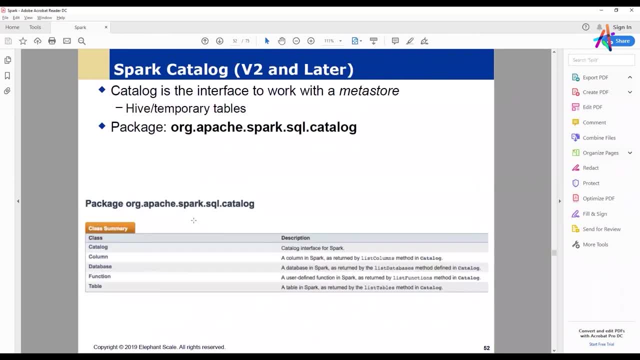 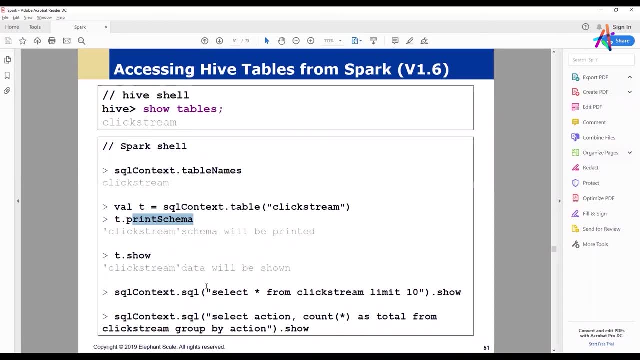 and we can now print the, the schema from that table and we can show the data. that's there and now we can use these queries. now that we've, we're attaching ourselves into that hive context, we can execute basically the hive ql query now for for things like select statements. 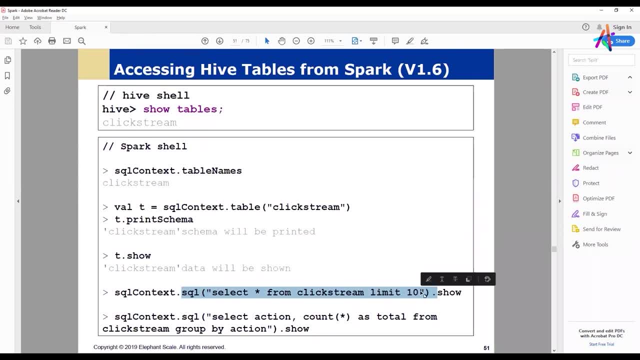 most of these, these data warehouse, like hive and everything else, generally support um select statements in in a pretty much standard way: um, so, the so, uh, so so the the queries are fairly standardized across it. it's in the other stuff where where we start to get some variations and 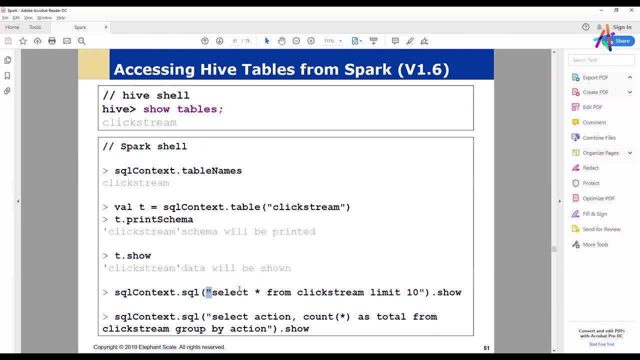 differences. so now we've got a context. we execute an sql command: collect, uh, select all columns from clickstream limit 10 and then we can show the results and we can do a count and again, fairly standard sql kinds of queries. again, the hive ql is intended to look like sql. 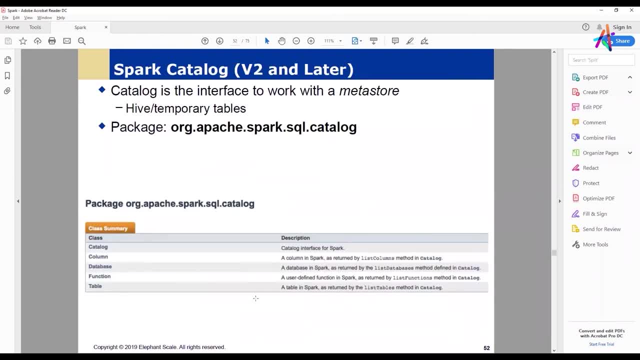 for most of your basic query type commands and uh. you also have uh the catalog, which uh is the uh uh, uh uh interface to work with the metastore. now, the metastore is the um actual descriptions that hive maintains of the, the conceptual table structures that are there. okay, so let's take a 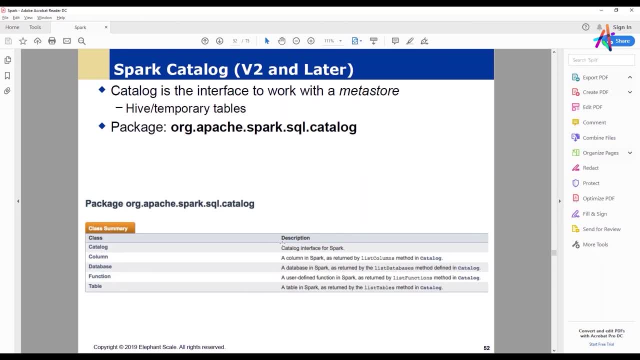 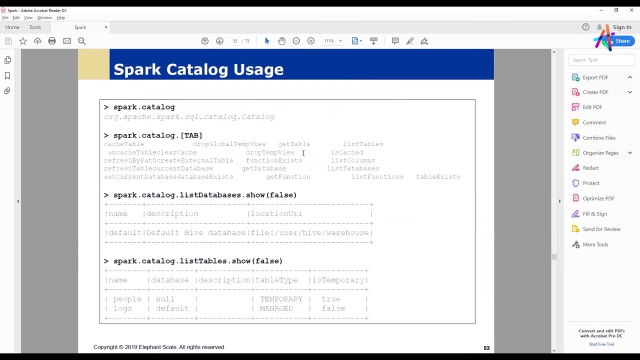 look here is that we have a catalog, which is the catalog interface, for spark a column- uh, which is a column, and spark a database, a function, a table- uh. so we do have those particular build, those particular options, okay. so here's the example of using the catalog. 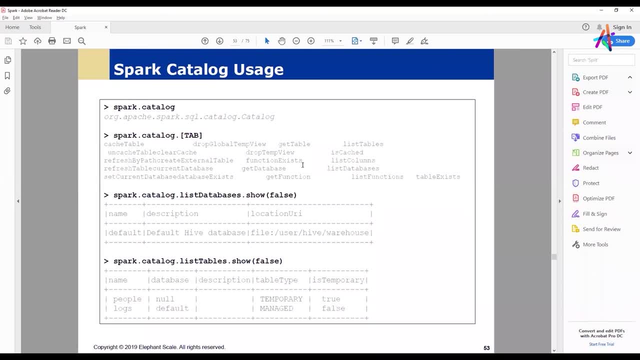 so we've got the spark catalog and now we can go and in the smart catalog, uh do tab and we get uh, the, the, the kinds of commands that we use- drop, temp view is, cache, list, tables, get table. so we do have a number of of fairly standard uh commands that we can use, so we can take one here. 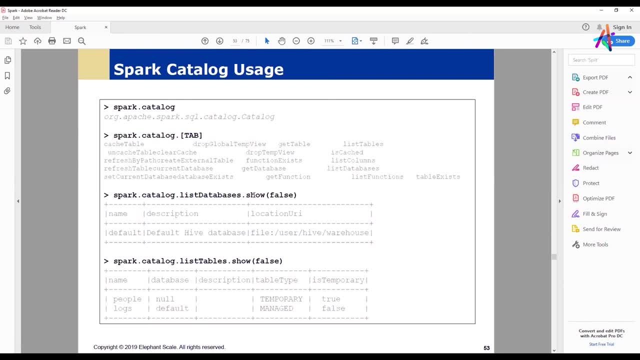 it will say uh is going to Spark uh web or it'll do, why not? and this will give that uh past, because your biggerTER version will be a far better version and we can scan that for our power table. so those that timeware are seeded. however we can, you can use numbers here so you 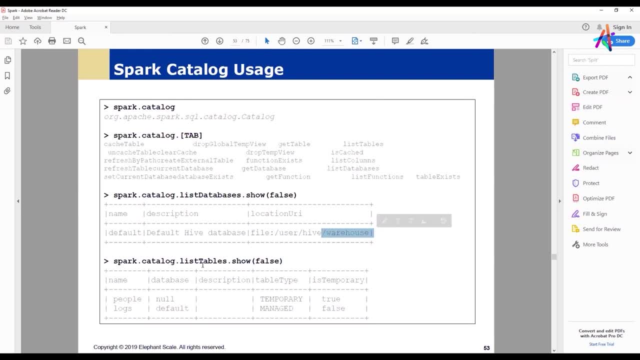 can use it by input processes, you can use uh numbers on it and then you can start exactly as you go. so here's um the ways that we've uh set up the uh, the tables about how many uh or numbers. again, that's more of a a hive kind type of thing, uh, and whether or not the table is is temporary. 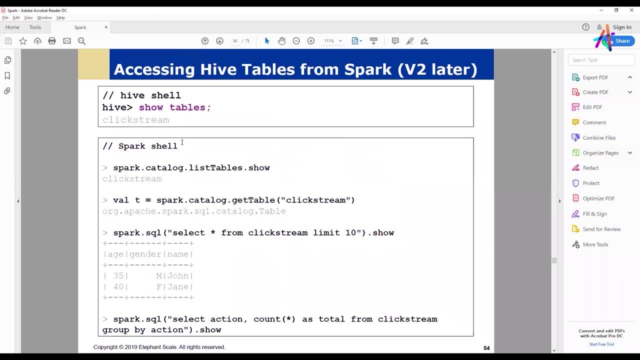 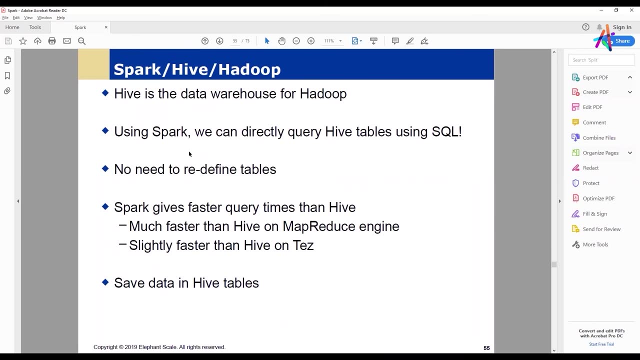 okay, so, um, so we can. we can again use our spark shell to do the same thing that the uh that we've got here. we just did that, i think. there we go. so a hive uh data warehouse for hadoop uh, we can directly query the hive tables using sql, so we don't have to switch over. 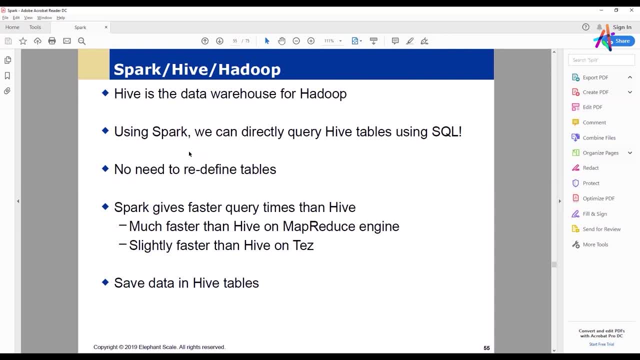 to hive. we don't have to redefine the tables because we are able to access all of the metadata and catalog data that hive maintains using the tables uh, or using the, the tables that that hive sets up in the. in terms of the metadata, hive does have. um, as you think back on what we were looking, 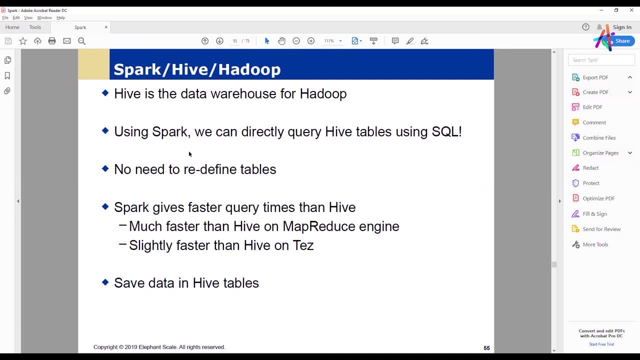 at before when we're looking at parquet, on some of these other formats, because they have attached schemas, spark is able to work with them much more effectively in this particular situation, uh since hive maintains uh a database of metadata, uh spark can utilize that metadata uh to get the 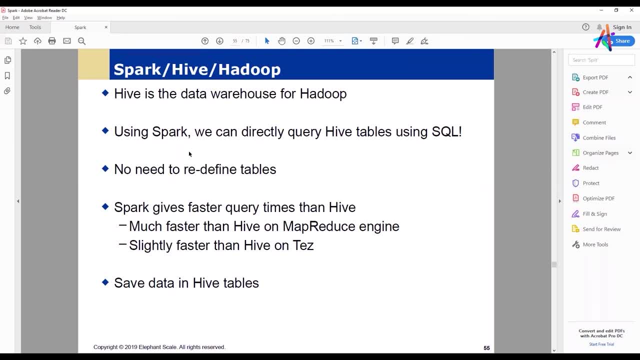 same kinds of of uh, of uh efficiencies in terms of getting information about the structure of the data and the nature of the data that it got when we were using some of these other structured formats. okay, so, um, so. so, basically, spark gives us a, a context, which is a hive context. 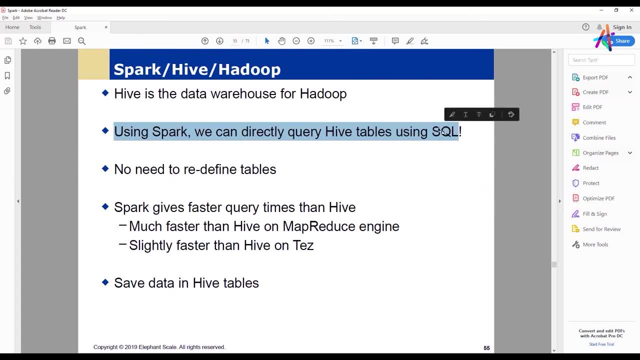 which is an interface that we can use uh directly into uh into the, into uh into hadoop, into uh into the, the underlying data warehouse. there is no need to redefine tables, in other words, there's no data transformation involved, and spark gives a faster query times than hive, and again, that's. 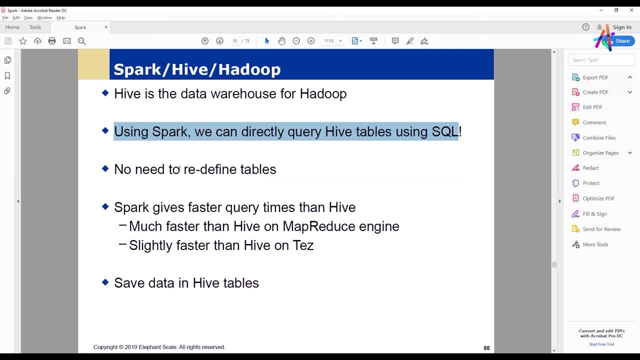 because, um, hive is using the underlying hadoop, the system which is mapping these out as mapper, and so the uh, the requirements that are uh, uh, com that her um is telling us is that, um, if we have Moderate Bet on the disk, that needs to be reproduced. so Divide is using the work couldn't be broad enough to uh. 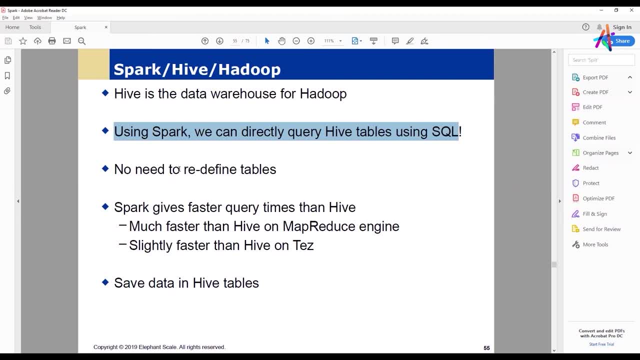 a more effective way, or a more efficient way of processing stuff that's stored in Hive. One of the use cases for this is that a lot of people went to Hive as a way of dataware, as imposing a data warehouse structure on top of their- you know- kind of big data solution. 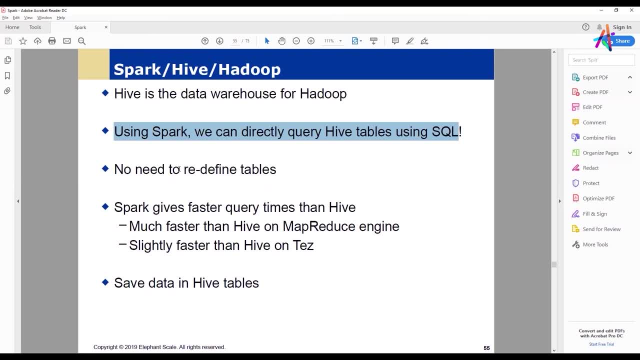 So they have all this stuff in Hadoop and you want to know. well, how can I access it directly? Well, let's conceptualize it as a data warehouse. So Hive comes along and gives us that structure, that interface maintains all the data we need to work with the underlying data as a data warehouse. 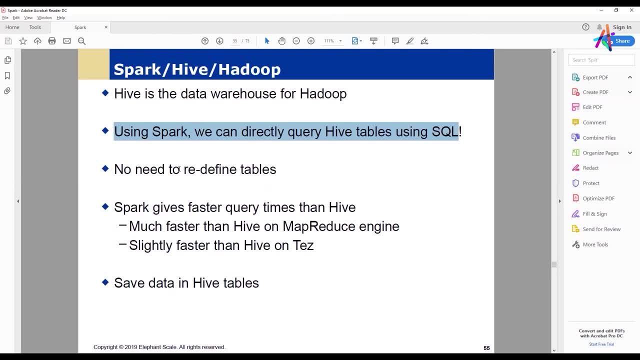 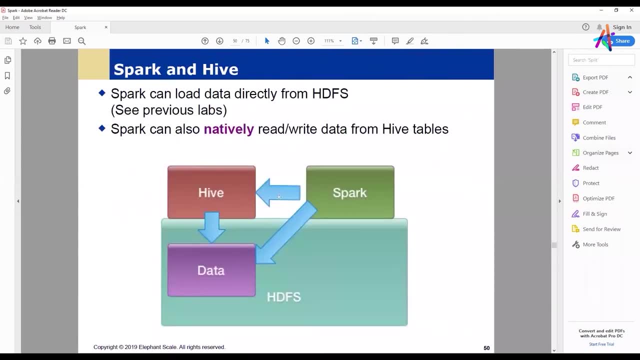 And now what Spark does is: Spark gives us a way of optimizing. So in this diagram, while it looks like Spark is actually going through Hive, I think it's a more accurate representation to say that Spark is sort of short-circuiting some of the stuff that Hive does, but it's using all of the information in Hive. 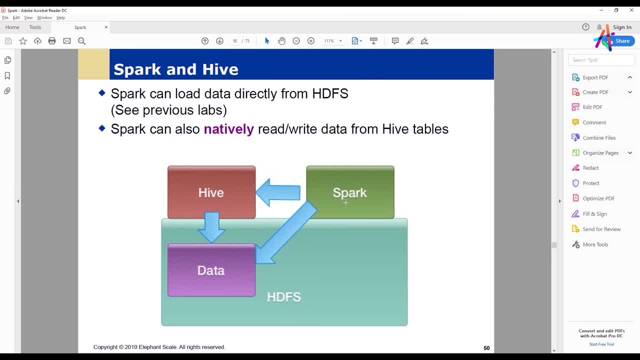 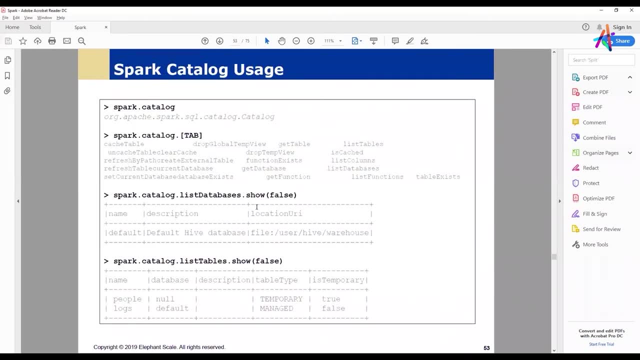 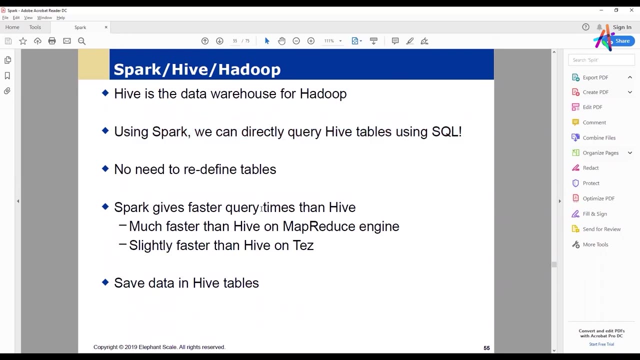 to be able to structure its queries. So I think it may be a more accurate representation to say that Spark is actually bypassing generally the slower parts of Hive and kind of giving us those performance introductions. That particularly shows up when we're bypassing the native Hive. 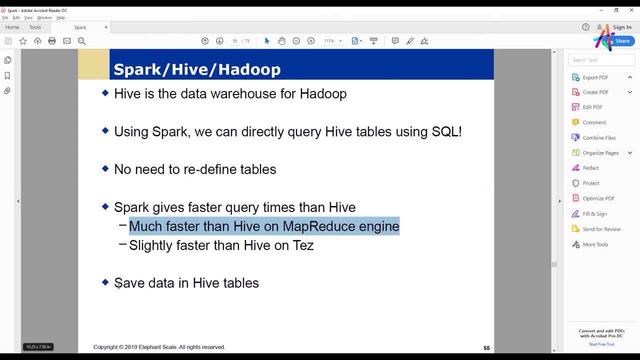 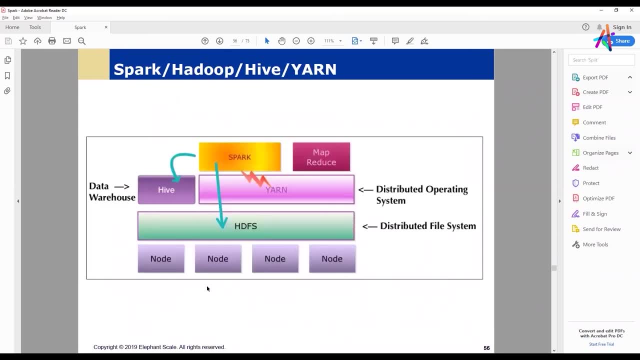 However, we can also save data in Hive tables, So we also have the ability to do persistent data. So there is a couple of operations here that are not generally native to the Spark world. We're not thinking in terms of saving tables in Spark. 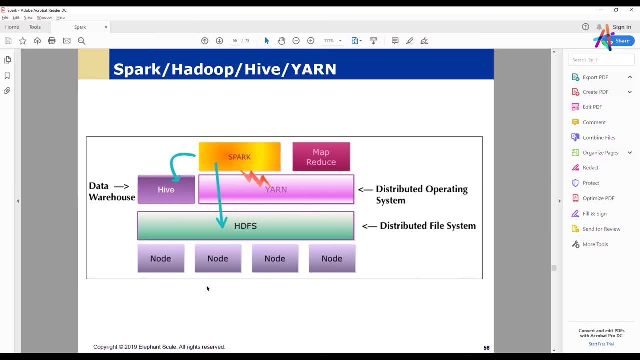 but we can basically reference saving tables through Hive. So here's our model again. This is our HDFS, Here's Spark, And the Hive represents a view into the HDFS system, the underlying data that Spark can use in order to execute various kinds of data warehouse type queries. 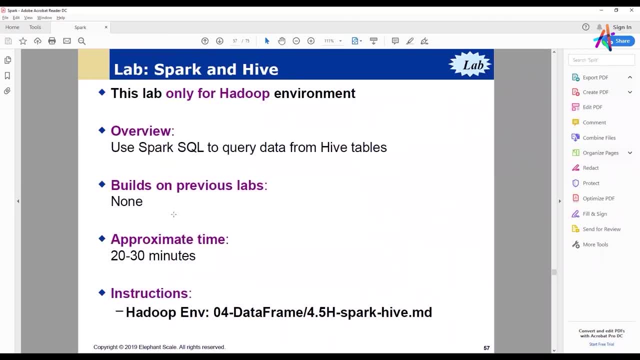 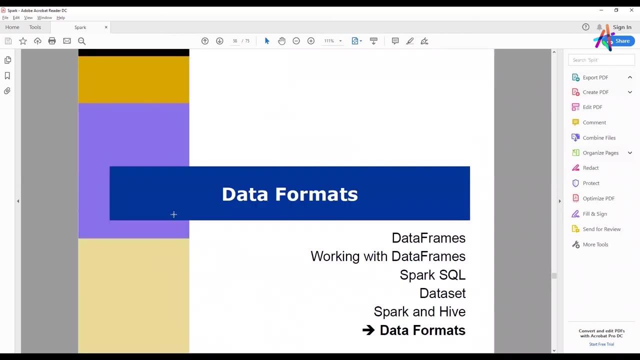 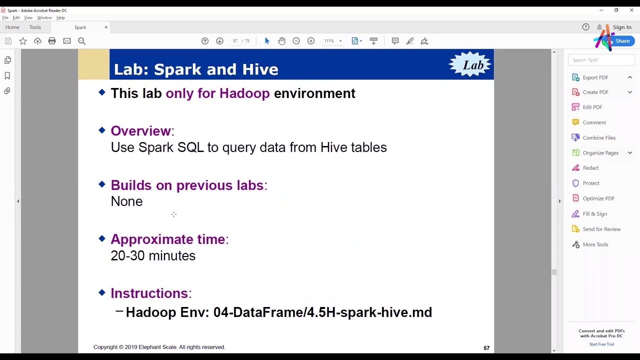 Okay. So now this will be a really quick And simple lab which will let you look at using Spark SQL from a slightly different perspective, And then we're going to be closing up a lot of stuff with the data format stuff, And that'll give us a bit of time to start talking about some of the other topics. 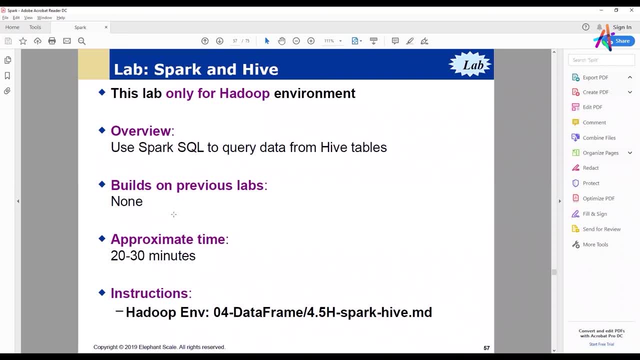 This will represent the end of kind of the basic stuff that we want to talk about Spark, And then we'll get into some of the more interesting stuff that you guys are particularly interested in. Okay, So I'm going to let you guys do this lab. 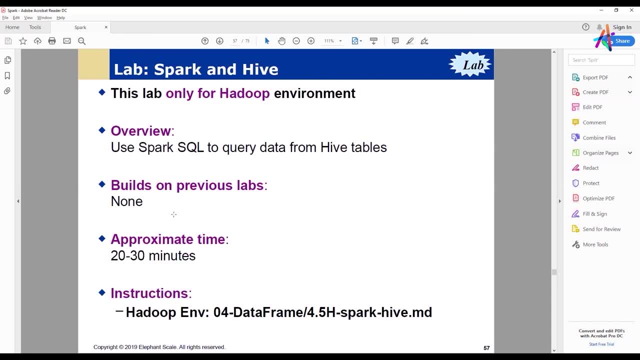 And one of the values of doing these labs is just to become more and more hands-on, familiar with the environment. So are there any questions before we start the lab? So step one says: open two terminal sessions to Hadoop node and instructor will demonstrate how. 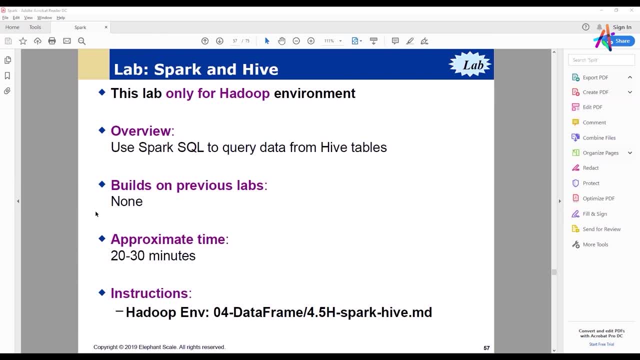 and I think we need these demonstrations because I don't. I don't have that demonstration here, So maybe the nation would be fine. Pardon, Maybe an explanation would be also fine. Yeah, there, there's okay. Again, I'm still sorting through all this documentation. 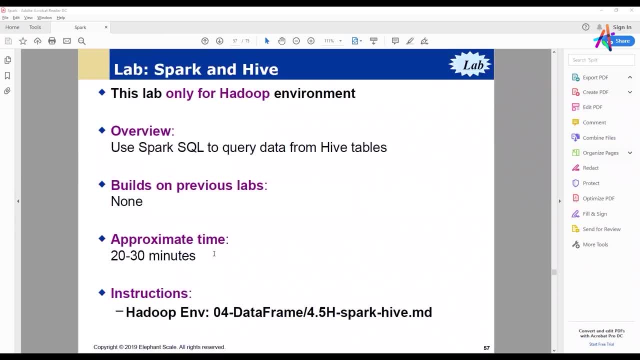 Let me check on this. They're there. to tell you the truth, I don't have that explanation on how to do it on there, So maybe what we'll do is we'll defer this lab until I find that documentation. I didn't get a lot of this lab stuff until just a couple of days before the class. 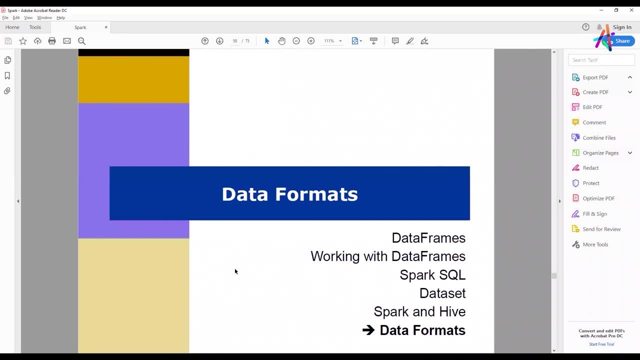 So you know, I didn't get a chance To do that. Okay, So how about if we just move on? we'll move on for now and then we'll come back to this lab later, If you want to do it. 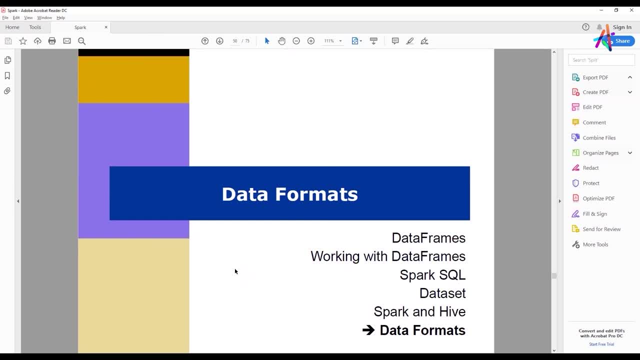 will that work? Yes, Yes, That'll give me a chance. That'll give me a chance to hunt stuff up. Okay, All right, I apologize for that. I'm I'm trying to, to, to, to assemble all of the stuff as we go along. 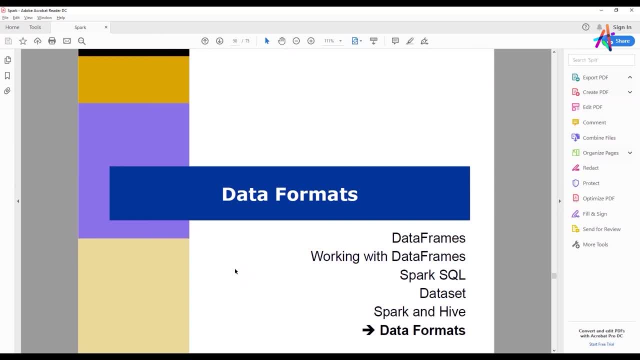 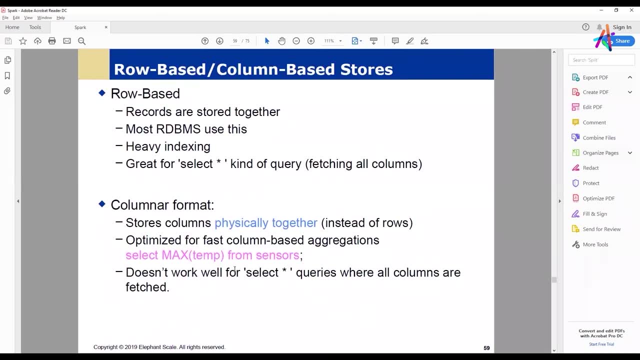 So sometimes it can be a little bit tricky. Okay, So let's work on with data formats for a bit. Okay, So the the notion of data format is that we think in terms of how data is actually being stored, in terms of tabular data, and how records are actually stored together. 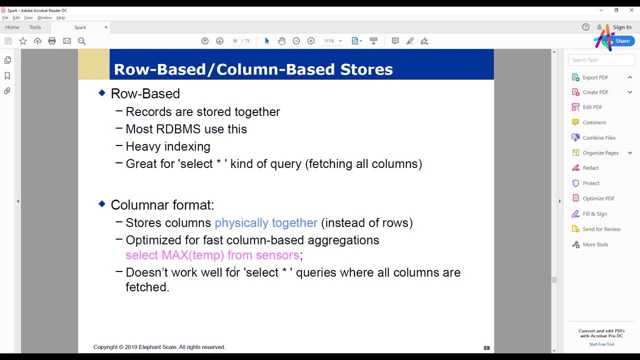 So, or how records are actually stored. So in most systems we use role based storage, where records are stored together, And so we have. this is the model that most, most relational databases actually used, And this is is generally because we're 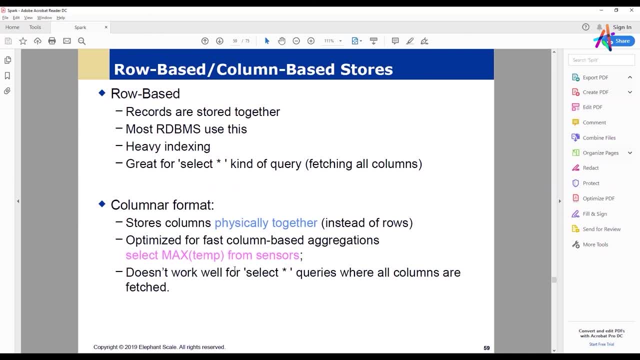 we're. the granular level that we're working at is the individual entities that are represented by the individual rows: The, the. the advantage also is that our select queries work kind of nice because we can kind of collect a select all of the columns And just kind of go down the row and select columns that are. to go down the table and select the, the, the rows that are appropriate. 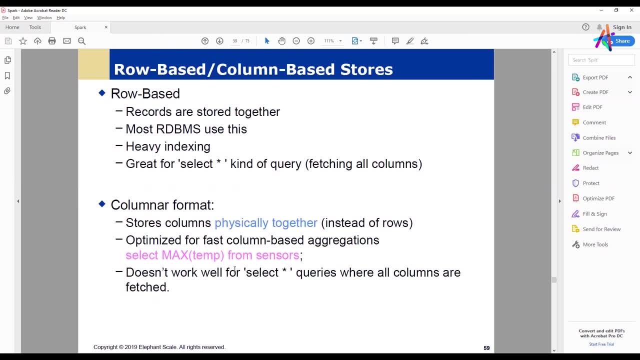 So from a from a an advantage point of view, it it makes working with the data very, very nice. The disadvantage is that if we're actually searching for things based on on some kind of role, some kind of column value, are our search time. 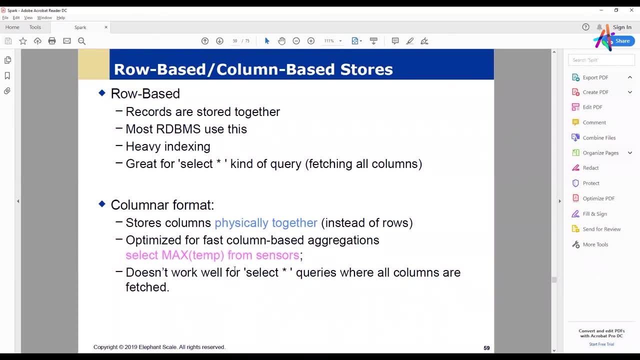 Tends to become at least linear, And so we we have to index the various columns if we're going to search on the column. So the indexes are a way of actually compensating for that. Now, in the, in the column, in the column format. 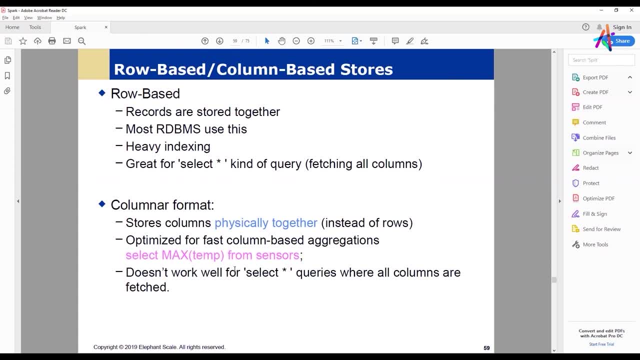 we're storing it column by column And there this is. this is the reason why we, we, we, we don't do relational data this way is because because when we're adding records, It's very difficult to insert records, Whereas with row based, you just add another row to the table. 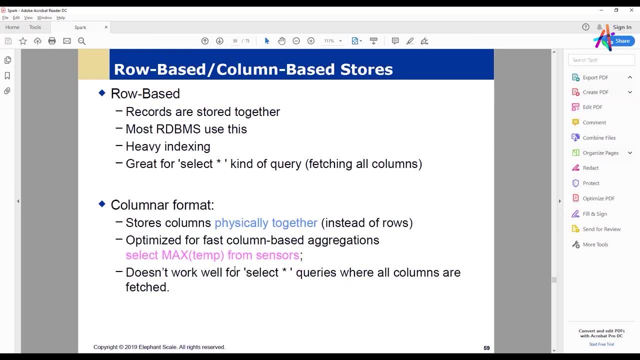 However, the column format does have a a some some significant advantages Because we're often doing some kind of of column based work. likes example, there are select the max temp from sensors. We basically can do a very fast access into a chunk of the data. 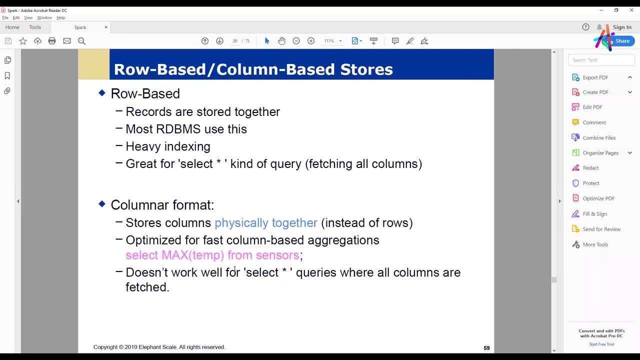 Which is the, which is the- All based on a column. It doesn't work well for select queries because if you visualize it, you're going to have to basically kind of jump from from chunk to chunk looking for that particular record. so if we, if we have, if we have, say, 10 records and we want to select record five, we have to jump from each column chunk to each column chunk looking for. 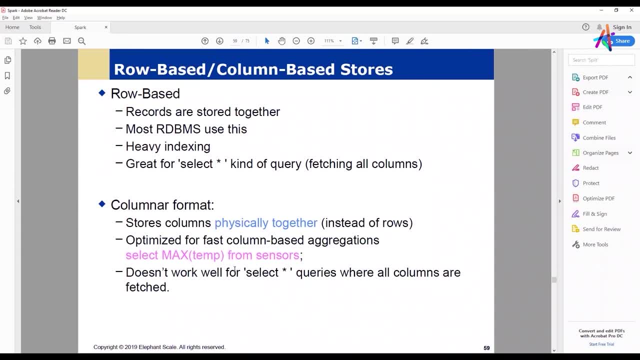 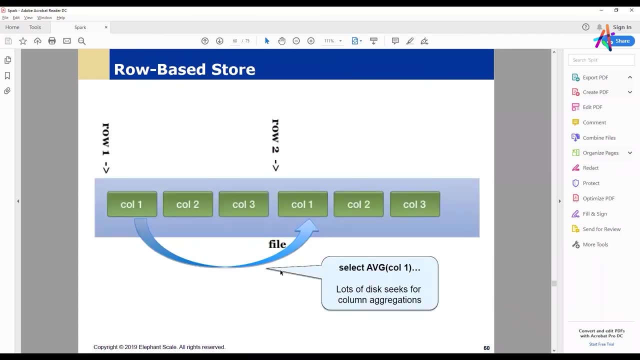 for for what part of that column is? it belongs to record five, And so we get a much, much more difficult process of assembling a query. So, like everything else in life, there's advantages and disadvantages to column based row. so here's our role based store. 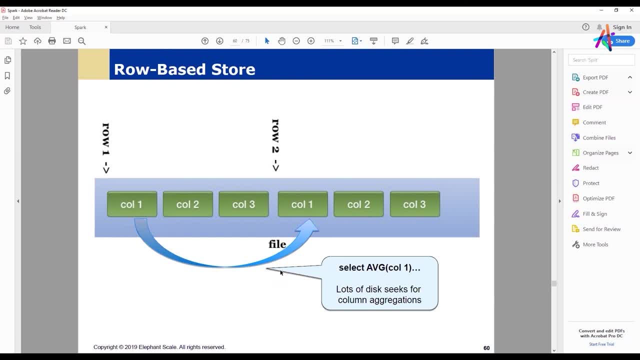 And, and the disadvantage here is that when you want to do aggregations, there's that, there's that a set of. So I want to sum up column one. I have to kind of jump from place to place and pull out the values for column one and assemble those into some intermediate form and and then do the do the operation on those, on those forms, on a column store. 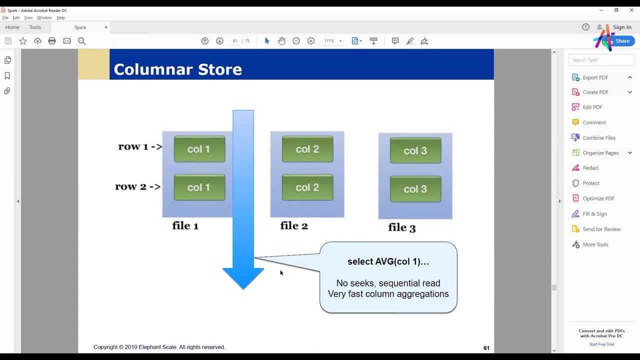 When we've got something like this in the various files, It's very easy for me to to to go in and do operations on the column. Very often for data Warehouses This is often a very effective thing because you're not interested necessarily in in individual records. you're interested in in various forms of aggregate data. 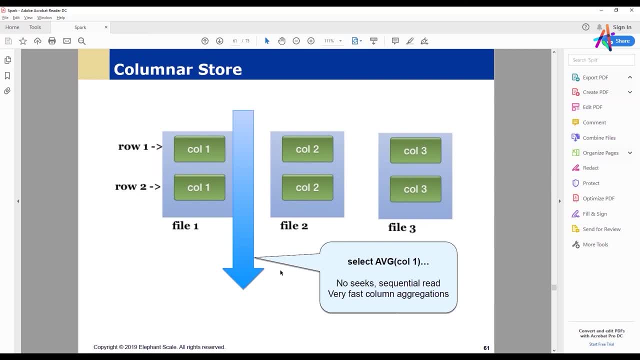 So you're interested in total, total sales by region or something like that, And so a lot of the operations Jackson and be performed are doing operations on columns of data across the data set. So in doing a column store you are getting very, very fast access to the data. 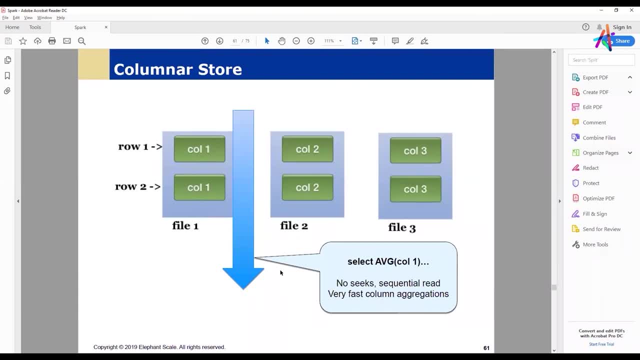 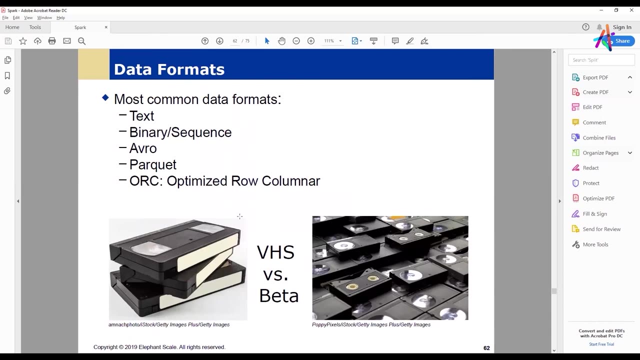 Barbara sometime observe it last time that there were some kind of Ha ha ha. So that that's one at one aspect of storing data. Now the other, the other Aspect of data source, is the actual formats that also interact with this, And each one of them, again, is going to have their own. 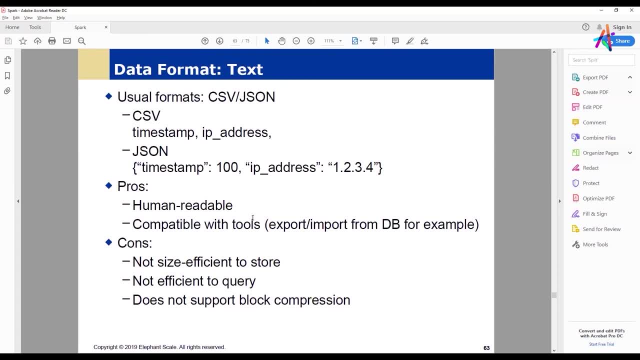 particular advantages and disadvantages. The standard, what we might call pseudo-tabular data, which is CSV JSON, which we also might consider to be sort of Excel-ish kinds of stuff, involves more or less explicit relationships between a key and a value. 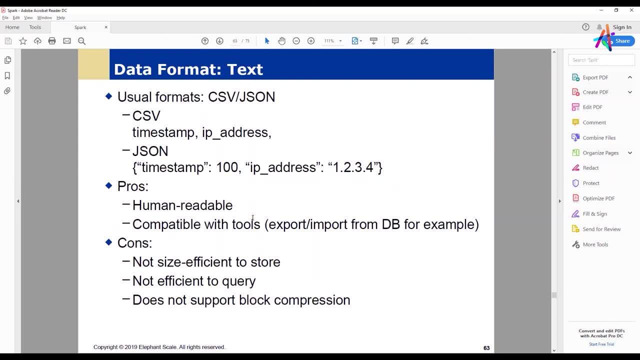 The advantages that this has is that they're human-readable, which is one of the big reasons why JSON is also preferred over XML is that it's much more human-readable, which is an advantage with various kinds of things like configuration data and other things. 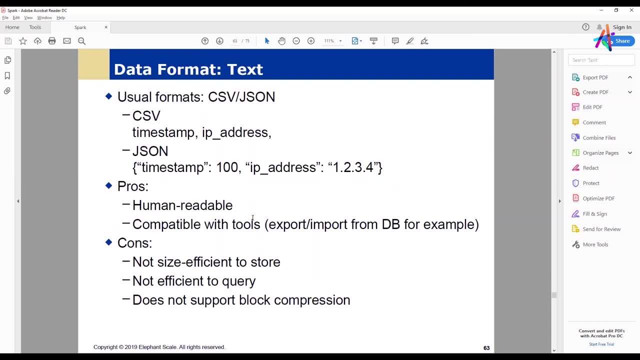 we've talked about, But it's also an advantage with various kinds of things like configuration, data and other things we've talked about. And it's also an advantage with various kinds of things like where you want things to be human-readable. It's compatible with tools. There's a lot of tools. 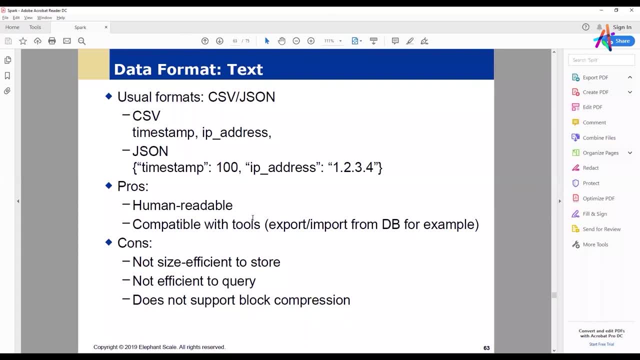 out there. It's a schema-independent store so you can move stuff from databases to data warehouses, to other kinds of environments. So JSON and CSV might also be considered kinds of transitory or transport tools that you would use to move data around. And because that's one of its strengths, it also is one of its weaknesses, Because it's human-readable. 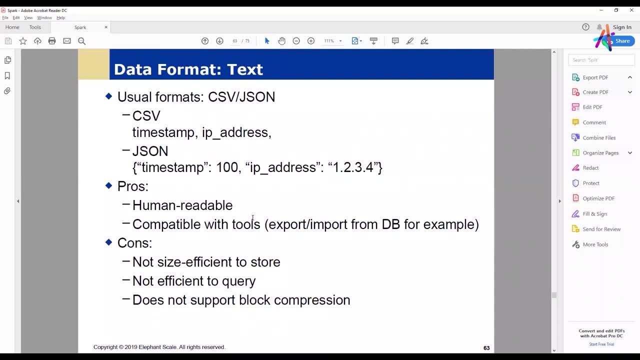 and because it's sort of in a neutral format, it's certainly not size-efficient. It's got a lot of redundancies in there. The other thing that it has is that it's really difficult to query this data. There's no optimizations that we can really perform on it. So, in order to work, 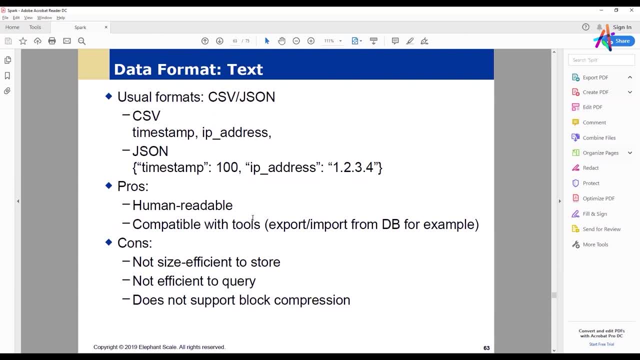 with this data, we generally have to convert it into another form, And it does not generally support some kind of block compression, So it's also something that doesn't lend itself well to various kinds of compression algorithms and things like that Binary sequence. 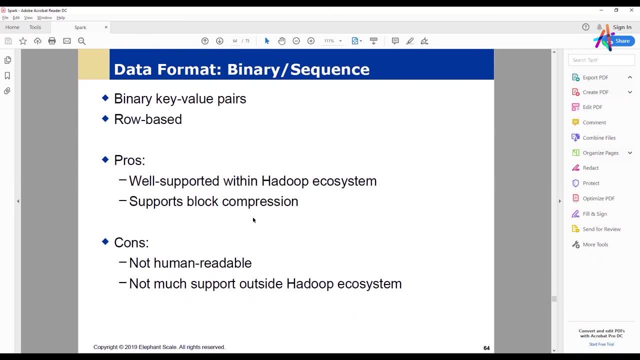 a binary key-value pair is role-based. It's got the advantage of that. it's supported within the Hadoop ecosystem which we're building our Spark and other things on. sometimes It supports compression, which is really good because that's what we're doing, So it's got the advantage of that. it's supported within the Hadoop ecosystem. 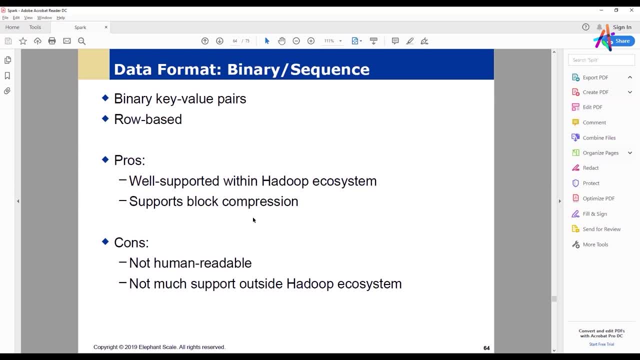 which is really good because that gives us various kinds of optimizations, But it's not human-readable. And again, I'm not really convinced that that's much of a con, Because if I'm looking with a lot of this data I'm not really going to be reading the data, I think. I think I'm going to be more looking at. 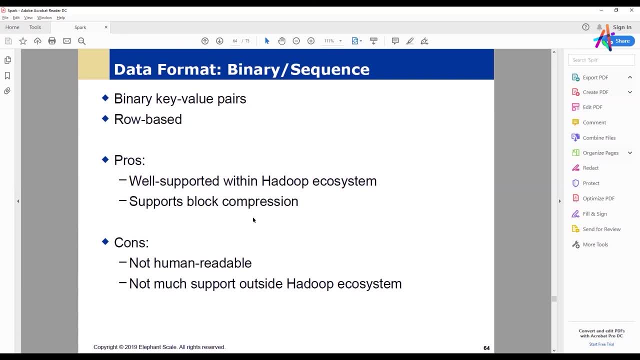 the results. in particular, if I'm doing any kind of analytics, You'll get some kind of representation of the data. The problem is that outside the Hadoop ecosystem- this is the big con- that if I'm doing a lot of analytics, I'm going to meet some of the data- The problem is that outside the Hadoop ecosystem- this is the big con- is that if I'm doing a lot of 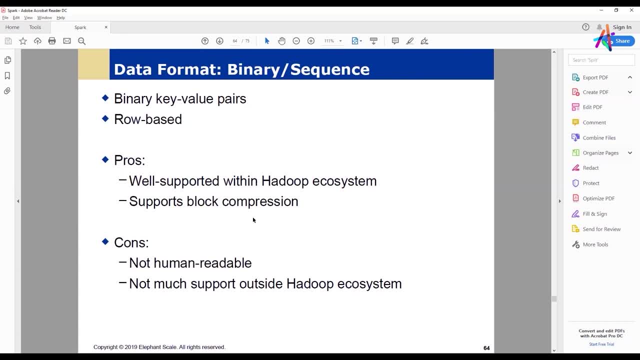 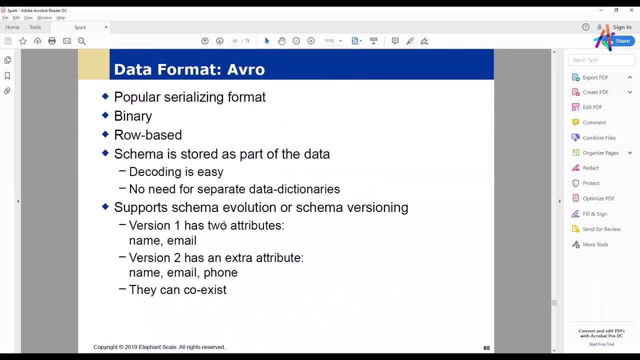 I want to start using data that's not really Hadoop-based, then I might start running into problems with this format. Avro is a serializing format, It's a row-based and it's got the advantage that the schema is stored as part of the data And, as we've seen before, having access. 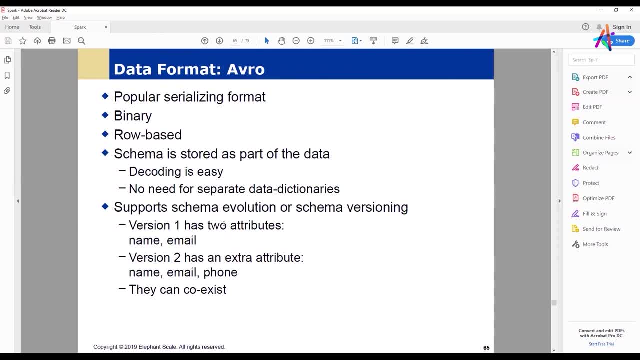 to the schema makes a lot of easy decoding taking place, so we don't need separate data dictionaries. And again, it's a serializing format. Okay. so if you have a schema when you're serializing, your serializing becomes really efficient. And if you want to think about how this works, 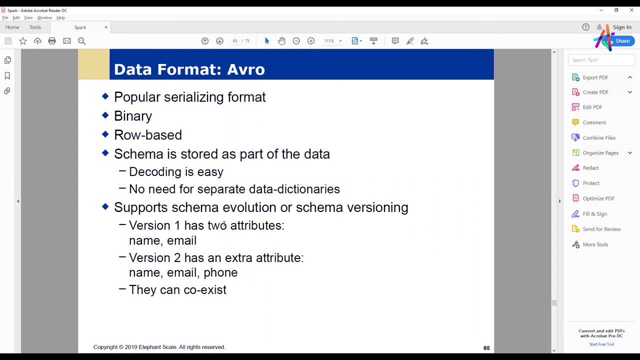 the place you really get the efficiency is in the deserializing. So if I know that when I serialize a number of data structures, each one of them is going to be marked in some manner, when I deserialize I can generally chunk up the byte stream much more efficiently. when I'm 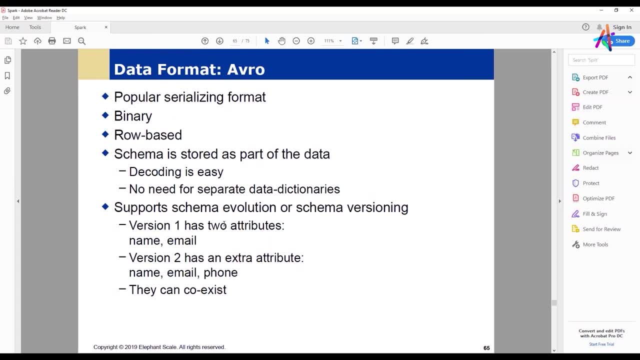 pulling it back in. So the idea here is that when I have a schema that's available, I can do a lot of more appropriate, a lot more optimizations, particularly when I'm deserializing. Serializing is generally not going to benefit too much, necessarily from some of these. 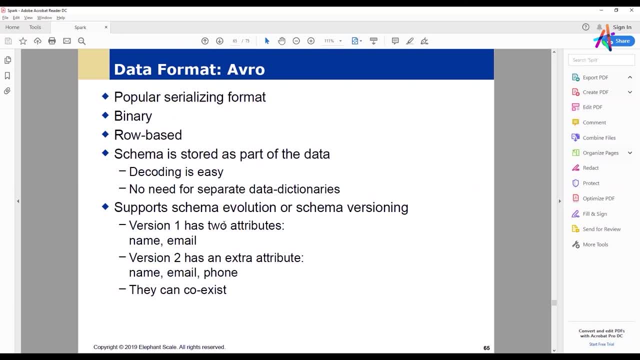 in this context, from this kind of operation because I still have to do all the serialization. but a lot of the deserializing problems are sometimes involved in trying to figure out, you know, like reading it, enough to know when to stop. So when a bunch of serialized data, 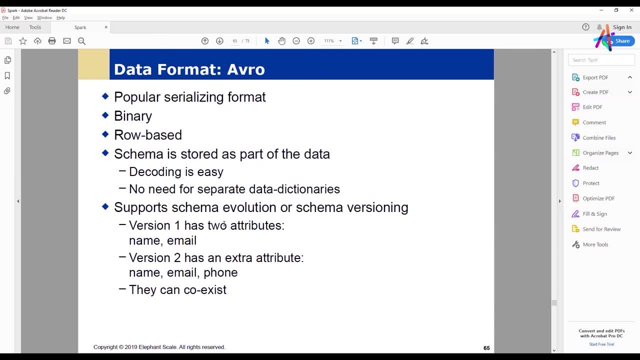 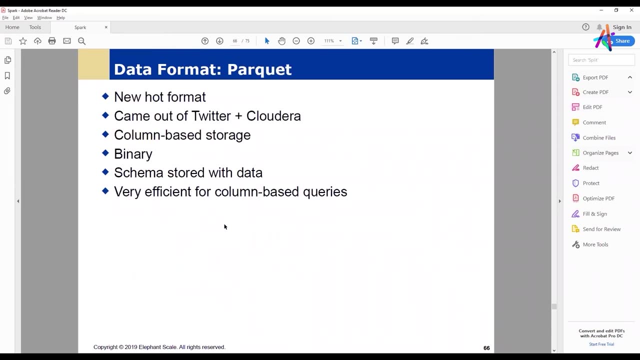 actually represents something, So you can have some optimizations in there. It does support schema evolution and versioning, So it does enable multiple versions of a schema to coexist. Now, parquet is something that's coming out of Twitter and Cloudera. 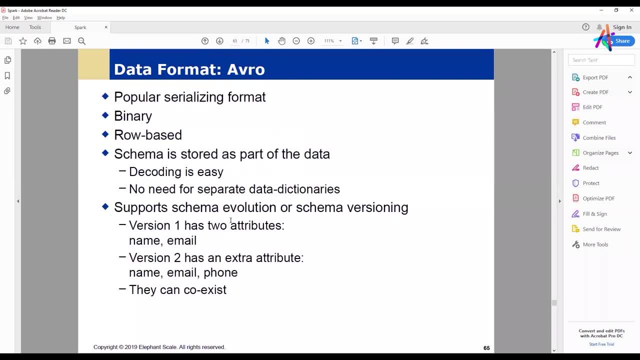 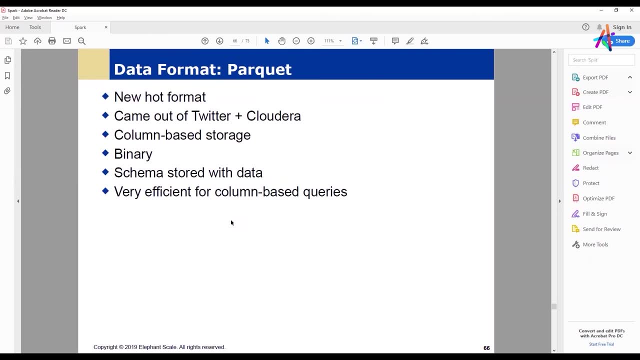 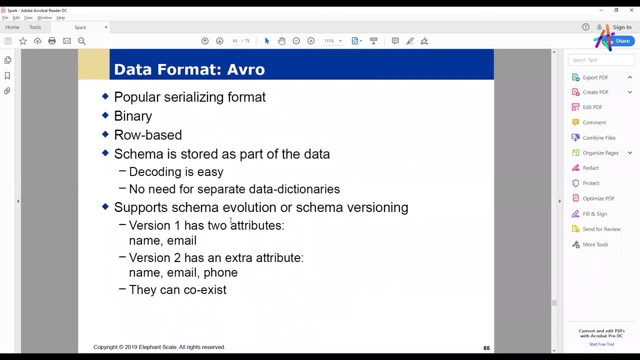 It, on the other hand, is column based, whereas these other things are rule based. It's binary and the schema stored with the data and is very efficient for column based queries. So we have a couple of different data formats which are usually using different. 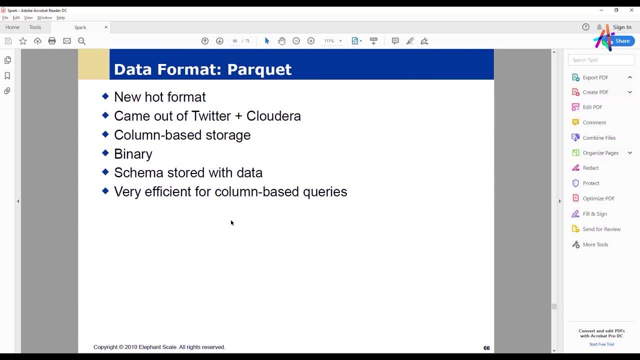 storage mechanisms. So parquet schema, again stored with data, but now we're looking for very efficient column based queries. Okay, so now we have another data format is ORC, optimized role, columnar, And this is evolution of something called RC file, And it's a hybrid format where it stores rows and within. 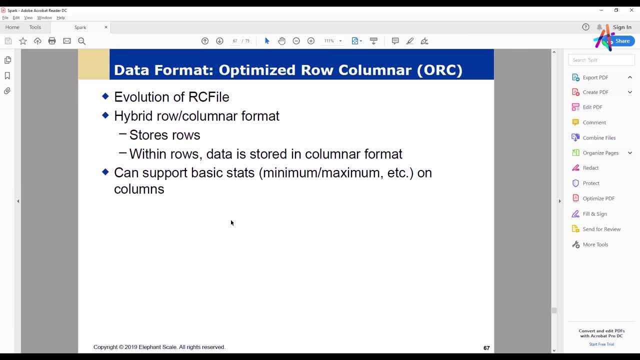 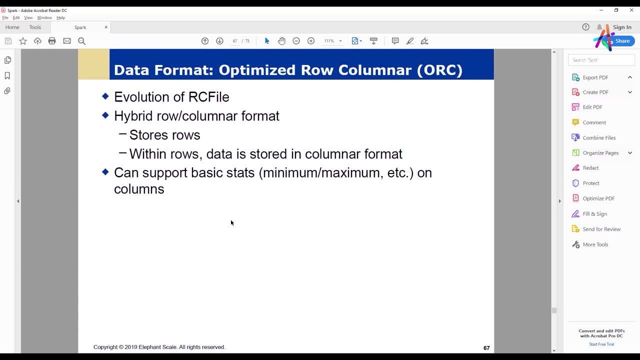 So what we're really doing here is, in the optimized role columnar format you think of it this way- is that the rows themselves in a normal row based format tend to be hard to find, or the columns tend to be hard to find, because we're really thinking in terms of rows. But if we can overlay, 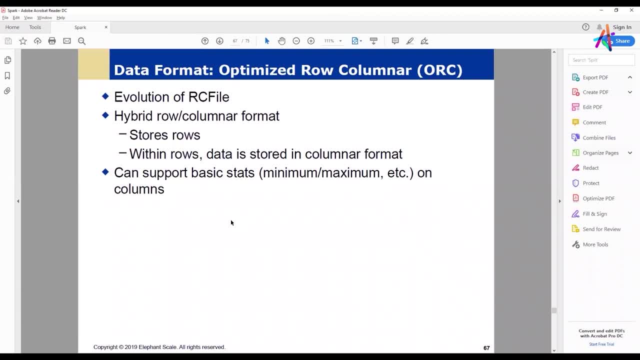 if we can overlay, on top of that, a structure so that we can easily move down a column with rows through some kinds of hints as to getting into that, so we can go from row to row, navigating through a particular column, from row to row through a column, then we get things a lot easier. 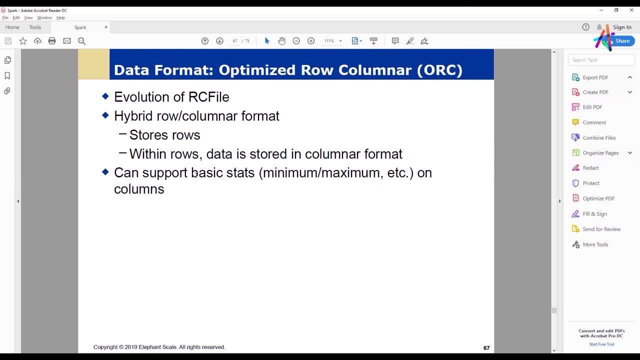 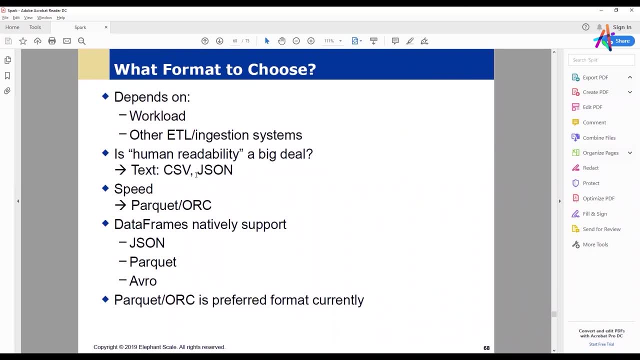 So this gives us a much better performance on column based operations. So how do we decide what we're going to do, what data format we're going to choose? we come down to to a number of considerations. Hold on here, Sorry. 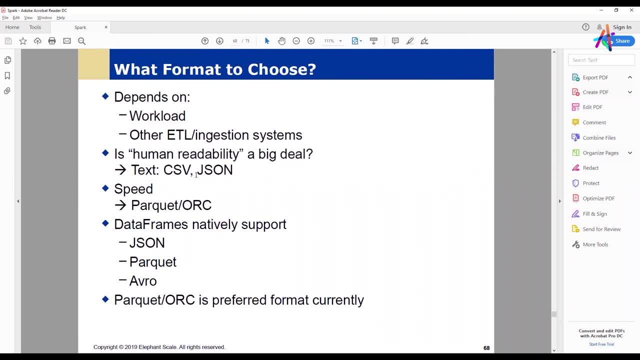 That was my timer to have you stop your lab. So the workload, ETL ingestion systems. obviously, if you're using Hadoop, that's going to be one of the most important things. So one thing: if you're using a different kind of system, you want data formats that are going to be compatible across those areas. 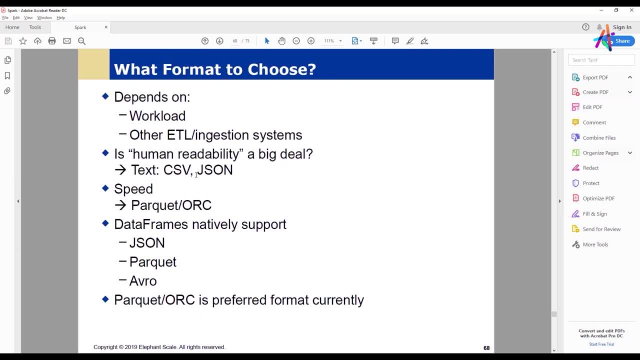 Is human readability a big deal If it is, and you can develop use cases for human readability. So there's there's there's times when you may want to look into the data and and have human readability. And again, I- not my, my personal feeling is that when we're operating in kind of a SPARC environment, 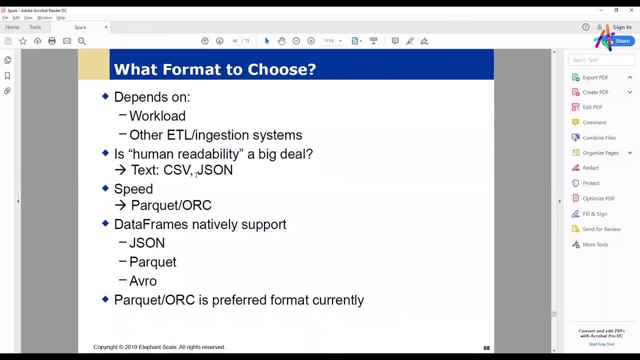 By that time we should really have a good sense of kind of what our underlying data structure is like and how it's working. So human readability generally, I think it's probably not as big an issue, But if it is, then we want to use some kind of human readable format. 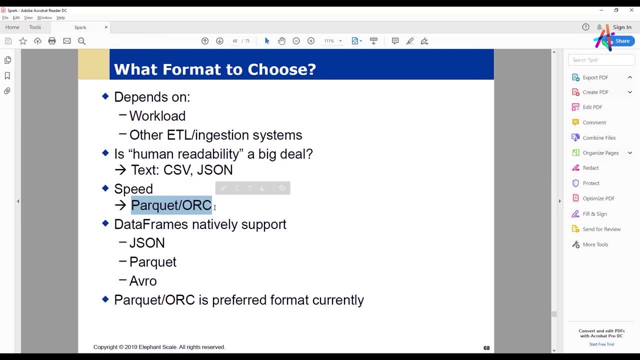 Speed Parquet ORC because of the way in which the data is organized. If you want to be able to use data frames that are supported natively, then the things that have that structure associated with them is JSON: Parquet Avro. 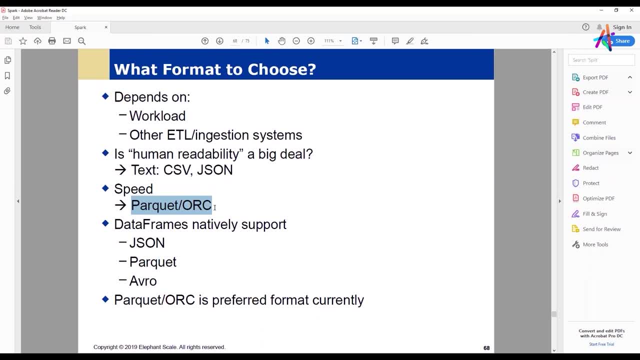 And apparently right now- and I'm not too much up on what the current trends are- exactly what everybody's using. it looks like Parquet and ORC is a preferred format And I think that's a good thing, And again, I think the ORC looks like it's got some really, really good advantages. 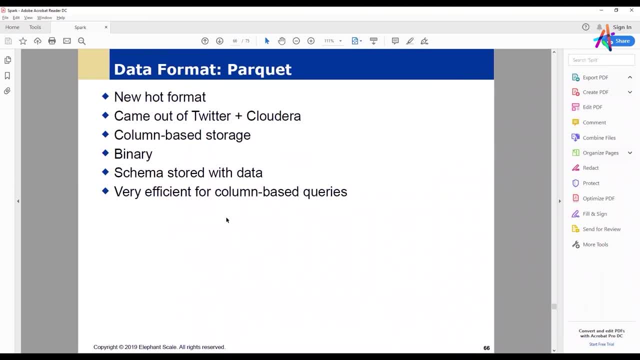 And Parquet again because it's column-based storage, And part of the reason for that is that we're also, if you stop and think in terms of a query, you know a lot of terms of our query are being done in terms of searching through a column for particular values in a particular column. 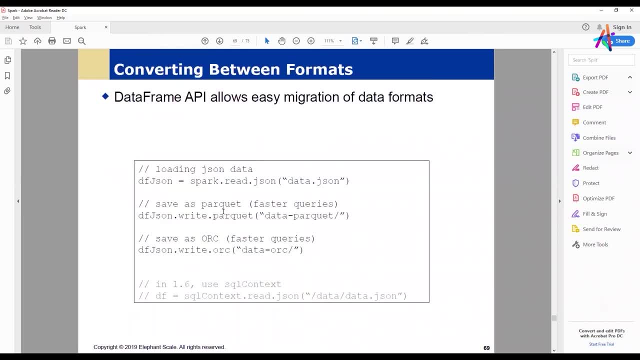 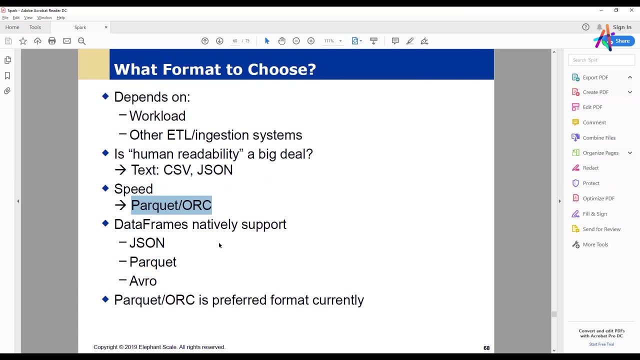 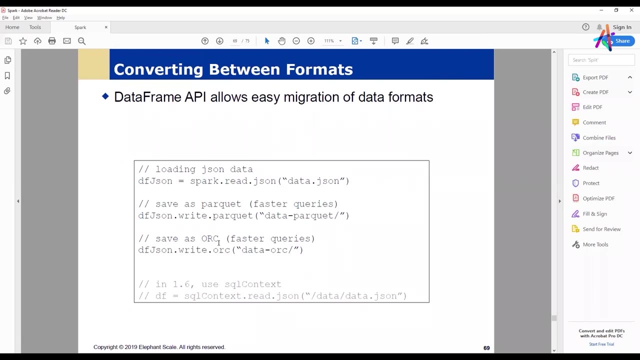 So you can see where optimizations would come up from that format, From using that particular format. Okay, So Parquet and ORC preferred format. I don't know who says they're preferred format. I'll just trust what the guy who wrote this said. 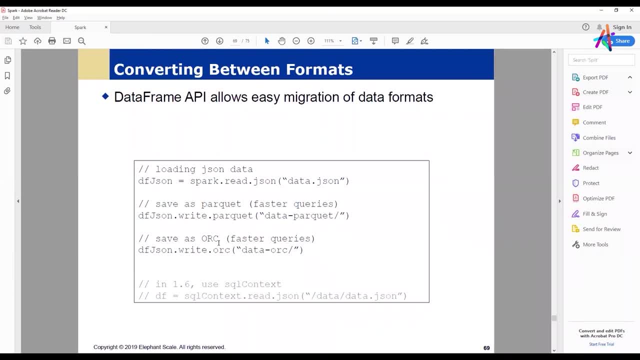 But what happens is that we do have the option of being able to convert between formats, So we can actually- as the example shows, we can- do migration from one data format to another, And so we've got a JSON data frame. 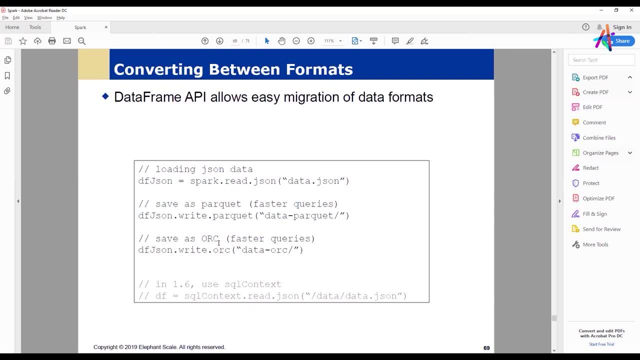 We're reading JSON, We're getting a data frame, But now we can write it as Parquet. My understanding that what this writing does is it's actually creating all of the metadata in a Parquet format- And also the same thing with ORC- is that it's also doing a lot of the metadata work. 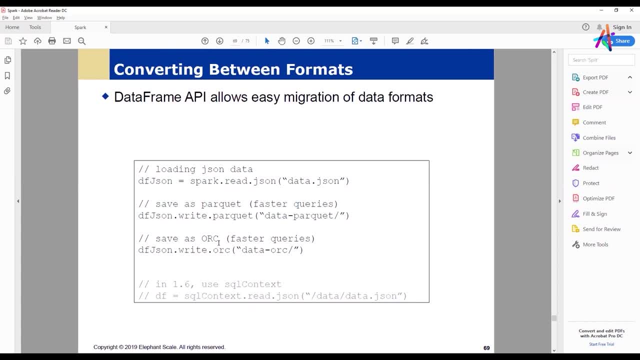 I have to go and check and find out exactly the amount of what we're doing, The amount of overhead that's involved, And easy in doing this Because I don't have those values right offhand. But the idea here is that from an operational point of view, I can generally go and create various formats. 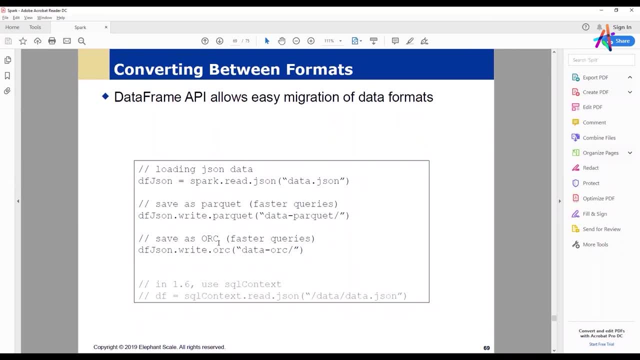 Now I'm going to suggest that the choice of migrating from one format to another may be dictated on how we are going to do this. How are we going to be working with that data? So we may have data. It's one format. 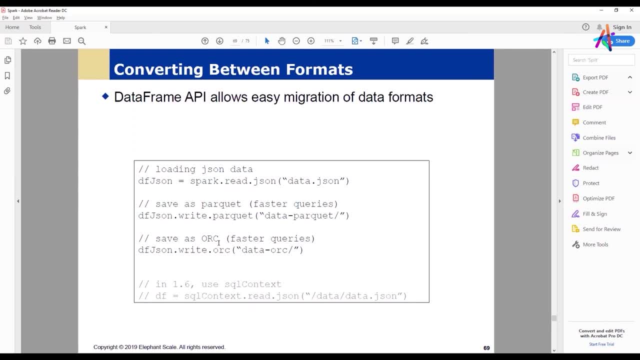 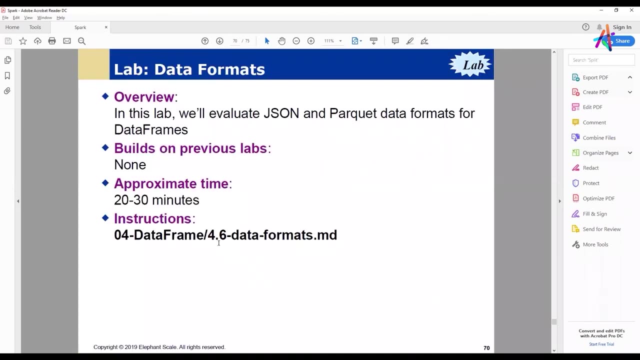 We read it in, But now we realize that the operational stuff that we're going to be doing this isn't really a great data format. We can switch it to a different data format And we can get some easy migration. Okay, So now we can hopefully be able to do some good labs. 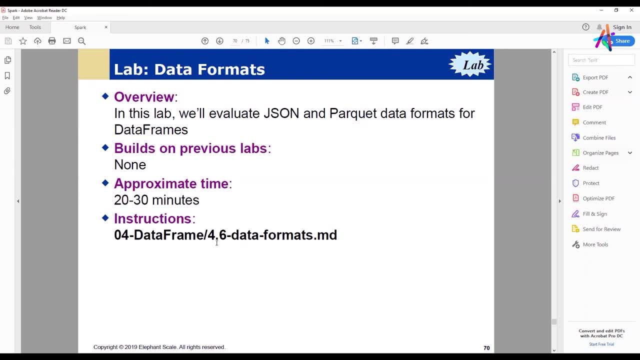 And I'm going to go while you're doing that and try to find out where that thing I'm supposed to show you is located, Because I don't know how it's actually set up on that system. But I will do that, Okay. 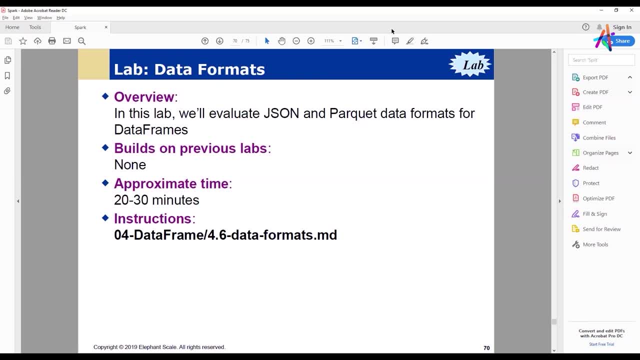 So we've got another 50.. First of all, questions about data formats and things like that. All right, One thing to remember is a lot of these data formats rely heavily on how the metadata is structured, So there is a lot of the conversion that can take place is actually conversion of metadata and doing mappings of metadata. 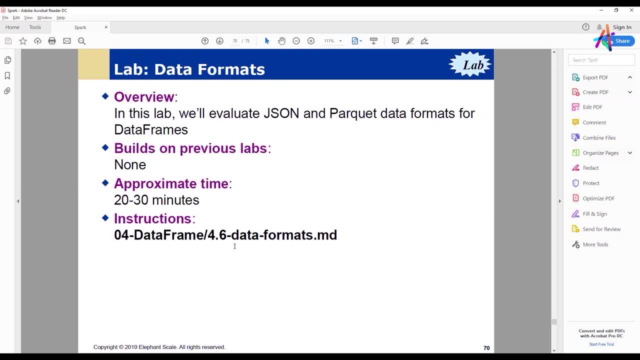 Not all of it, But a lot of it. So there are efficiencies in that format, in that aspect of it. Okay, So I'm going to let you guys do 4.6.. I'll give you 15 minutes. 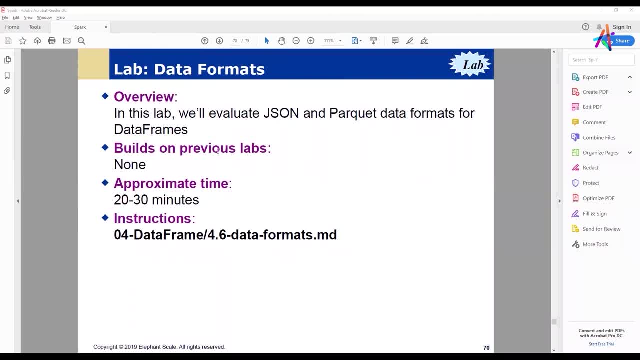 There's no questions, So it looks like we're fairly good. All right, So let's see what we're doing now. Do we need a bit more time or are we good? Some of us are good. What about Gerard? 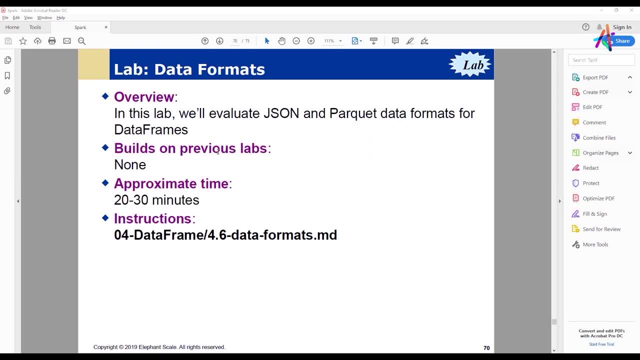 Are you okay? I'm still good. Okay, Yeah, Some of us are not. Okay, Well, another five minutes. We're in no rush here. We're really far ahead of where we should be. So you know, I don't want any of you to feel a little bit rushed. 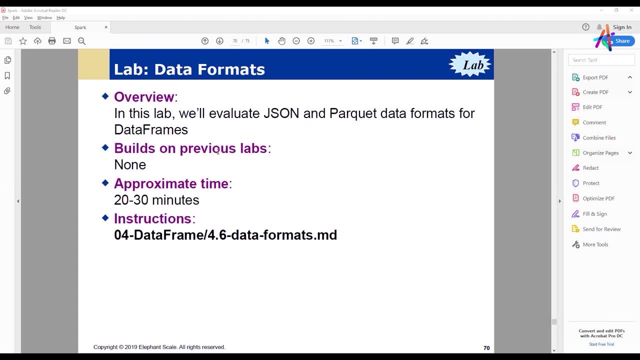 So those of you who need more time, you can take it, And those of you who don't need more time, you can stare at the people who need more time and make them feel uncomfortable, or something you know. But I have a question. 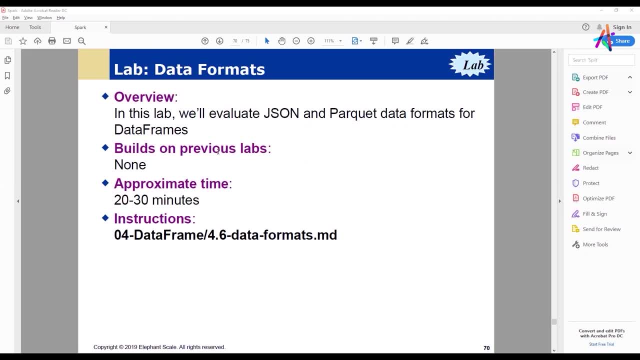 Do you have any questions? Yeah, I have a question. So it says so. the lab description says that we need to record the load time into the spreadsheets. However, this is a little bit complicated for us. I don't want to see, because it doesn't explicitly show the load time. 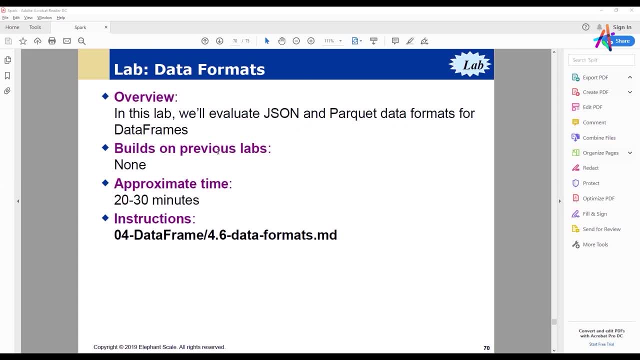 Okay, Or at least I'm just unable to see where it is. Okay, I'll take a look at it too, And I'm taking a note of some of these things and I'll check on to them over the weekend and see if there's something I can come up with. 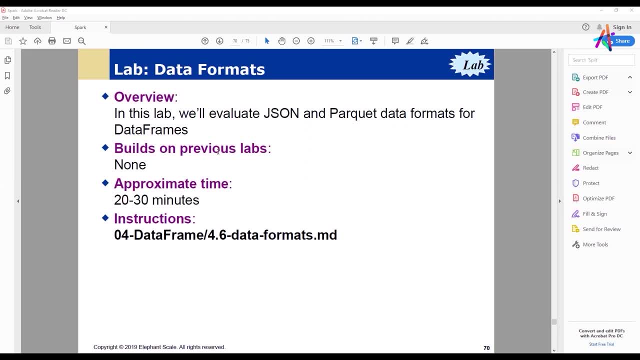 Okay, Yep, All right, Anything else? So do you want to take another little bit of time or do you want to kind of move on a bit? It's up to you guys. Okay, Thank you, I still didn't finish. 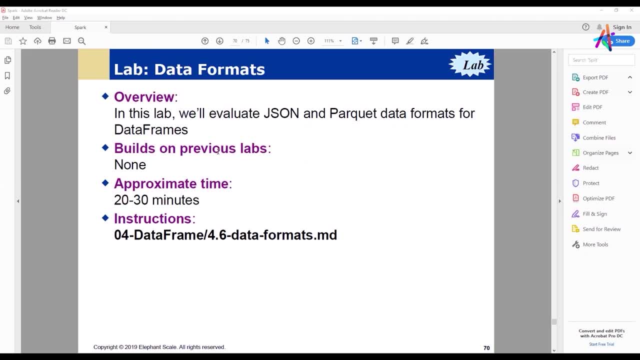 So Okay. So I'll come up with, We'll say, another five minutes for those who Five minutes, Yes, Okay, Good, We'll do five minutes and then we'll get back to it. Okay, I have one more question though. 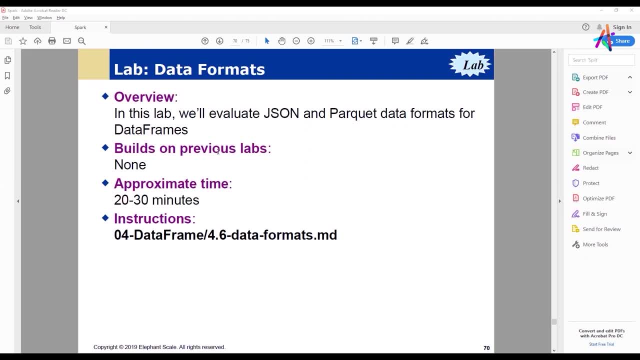 Okay, Go ahead All those five minutes. So at the end it says you should sort of well, you should- be looking at where is your resource ceiling, whether or not this is the memory, CPU or disk. I was sort of trying to monitor the. 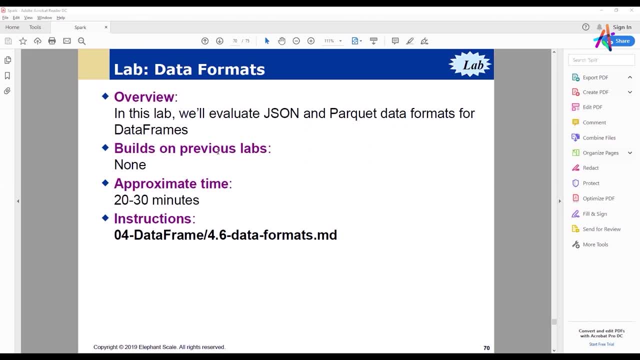 ATOP output, but apparently the sampling rate wasn't very good, So I didn't really get any answers for that. I mean, I have some hunches, but What's your hunch? You'll get some actual results, for which ones were bound by. 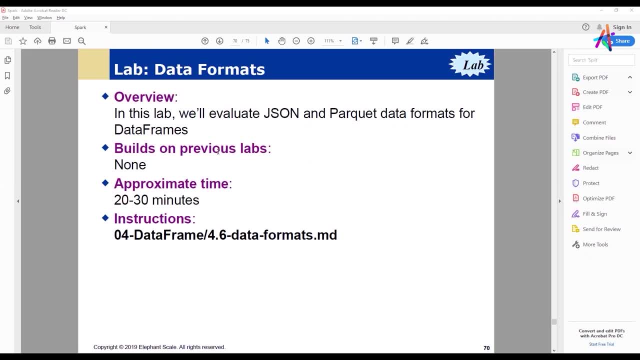 which? So what you said? you had some hunches. what were they? So like my? as far as I understand it, if you read JSON, that's a big file format. It's even apparent when you do, when you list the files and look at how big they are. So 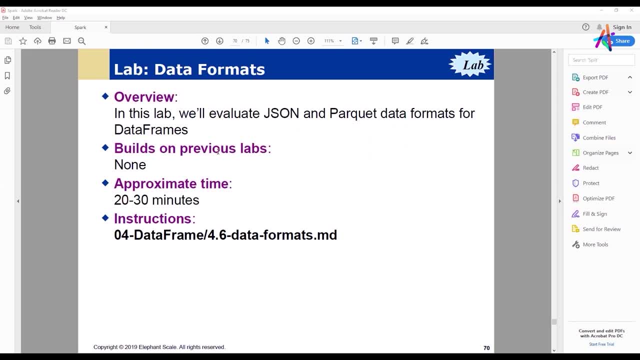 it's going to be both disk bound and CPU bound because it has to parse both. So like there it's. it just depends on how fast your disk is. If it's an SSD, it may be CPU bound because it takes so much time to actually parse it. If it's a slow, 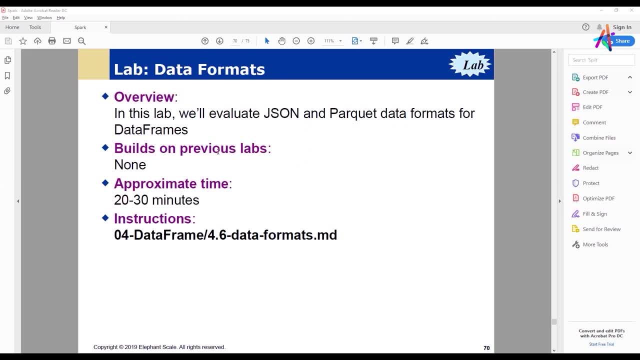 spinning disk, then your CPU is probably fast enough, so their disk is going to be your C long. Yeah, I think that's fairly true, but but again, remember part of the part of the part. the thing that is always going to be true is that the parsing JSON files is going to be much more CPU intensive. 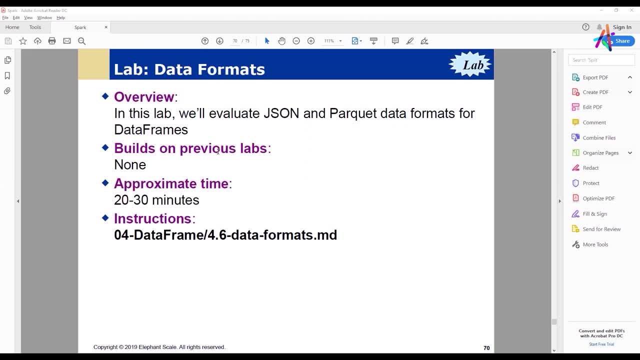 than parsing some other format because of the fact that it's basically Yeah, no doubt, no doubt, Yeah. so that always is going to be true. but your comment about the disk is quite true and I think maybe one of the questions you might look at is that in even if you have a slow disk and you move up to a fast disk, you still 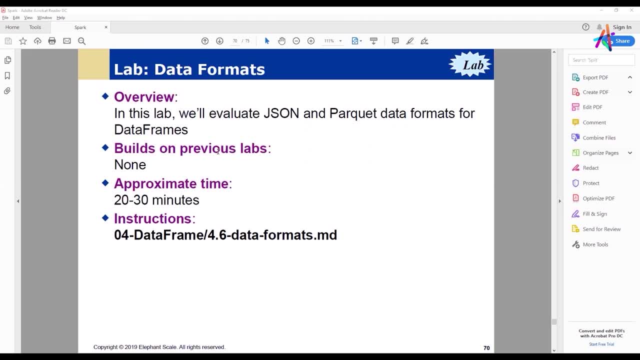 are stuck with the, the, the parsing problem of the file, of the, of the data format itself. and you know, even if you keep everything in memory, you still wind up with that CPU intensive operation. Yep, yeah, that's exactly what I, what I thought, right, so you still are. 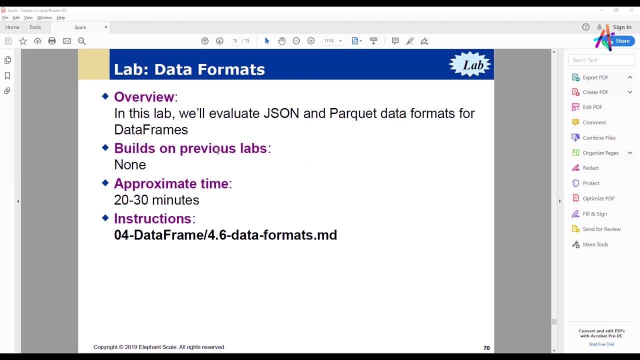 stuck with that task. uh, it's just. uh, depending on your disk speed, it, your bottleneck basically shifts to from one to the other Right, and even even if you're using an in-memory disk, you know um, you're still stuck with that CPU problem. Yeah, definitely, Okay, all right, good so. 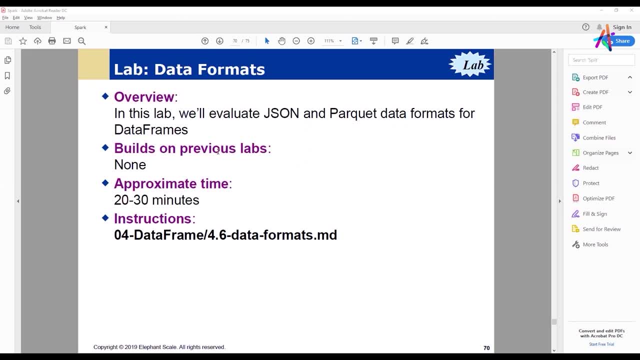 we'll do the five minutes and then we'll do it and and uh, just for you to. so you guys know we're two-thirds of the way through a three-day course in terms of content. so we've got a little bit of flexibility today in terms of what we're going to be doing. so we'll check in in five. 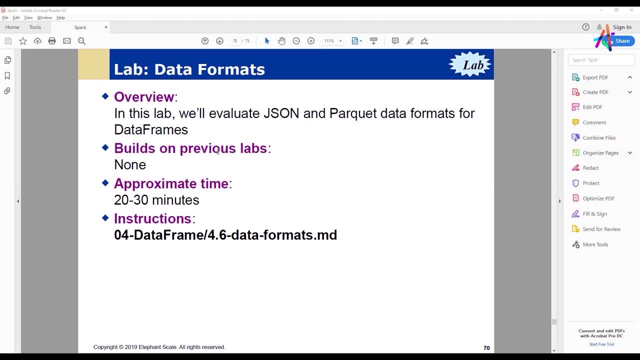 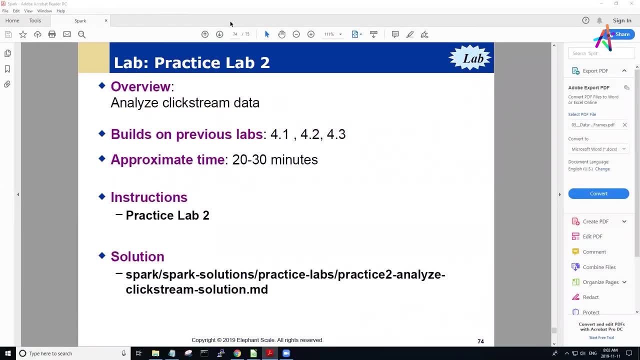 minutes and see how we're doing. okay, Okay, good, all right, uh, I was just explaining a moment ago that, uh, I may have made a mistake. um, I didn't explain that. I'm sorry about that. I'm sorry about that part. I was, uh, last Thursday and Friday. I was very 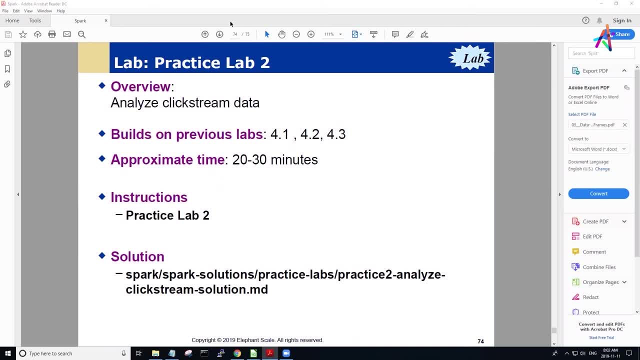 sick, so I was kind of stumbling through my, my classes, uh, focusing as best I could, and, uh, I went and shut down the, uh, the virtual machines on Friday. I saw them all changing state, but for some reason when I came back this morning they were all still running. It really surprised me. 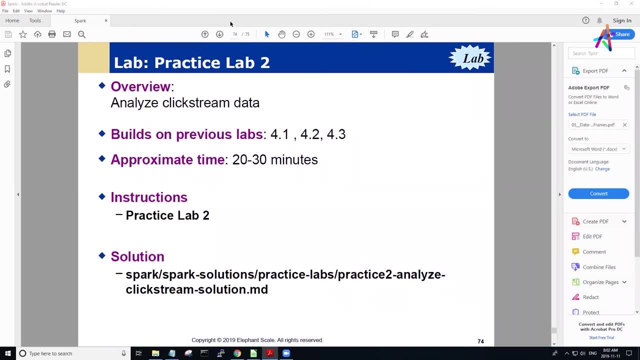 so I thought, oh gosh, this is great. so they probably have been compromised. so I've I've spun up another set of virtual machines, but they're in that kind of initial state. so I'm going to give you kind of the option here if you want to. uh, just uh, if you're just working at. 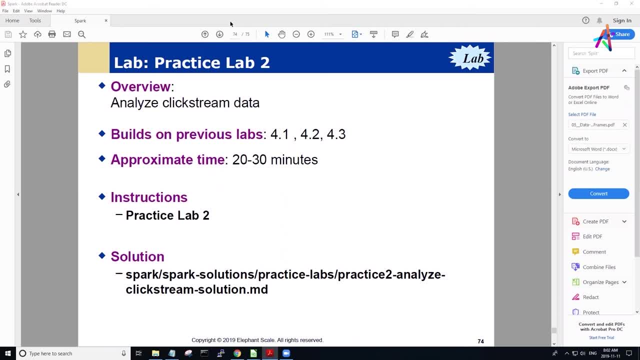 the command line and you want to play with the previous one, or if you want to pull some stuff off the previous one. um, you know, I've left them up with the same IPs, but I've also put up some other, some brand new ones this morning for you, and I'll I'll I put up a new spreadsheet which I'll dump. 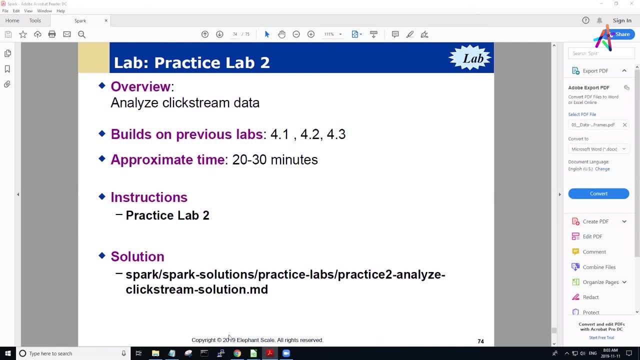 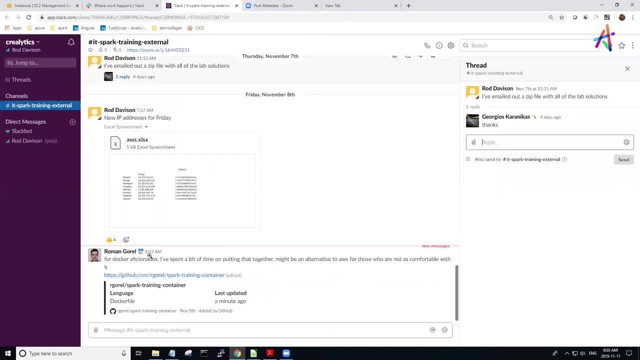 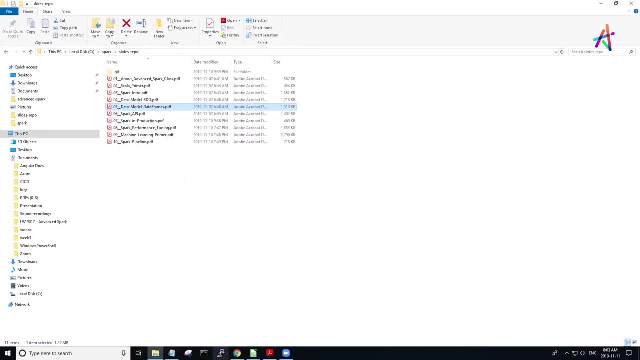 into this Slack channel right now, so I do apologize for that. uh, like I said I was, I was definitely not, uh, not completely, completely, should we say, sane, I guess, um, when I uh, when I was, when I was doing this. so, um, I'll, I'll let you, let you guys, make your choice, uh, as to what you want. 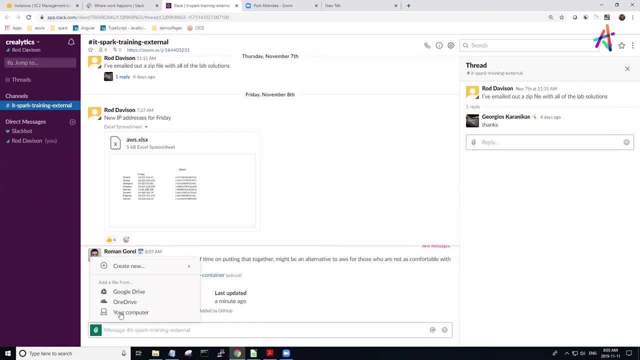 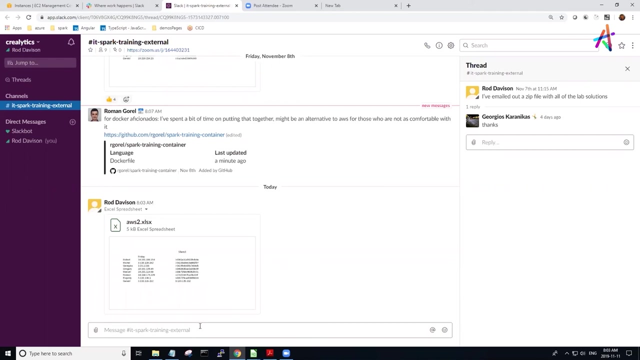 to do for me, the BNC. it says too many authentication failures. yeah, yeah, so I am going to to to put into the uh, into the uh. okay, so I put, I put the new spreadsheet in there. so I'm going to look, I'm going to give you guys. 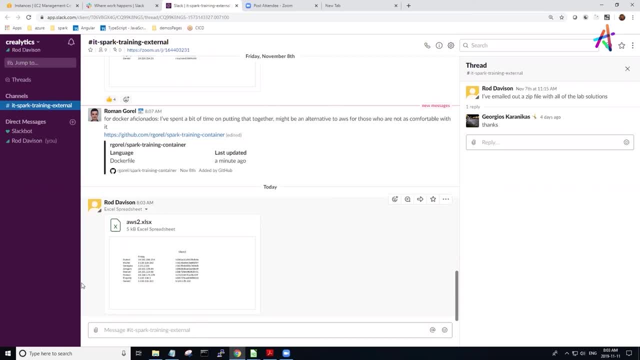 the option. as, as for those of you who just want to use the new machines, I will shut down your old ones, uh, but if you want to uh work on them a little bit, so I do apologize, it was entirely my fault. um, it was, uh, it was. 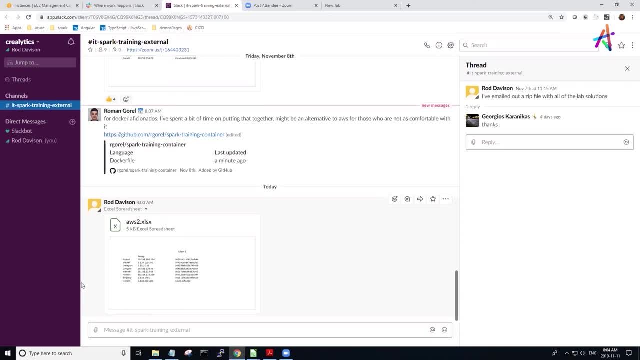 else other than than me not not ensuring coming back later and ensuring that they've been shut down properly. all right, uh, general speaking, uh, I would also use a new machine, but the, the, the password is not there. I mean, the IP is listed twice for me. oh, okay, okay, let me, let me. 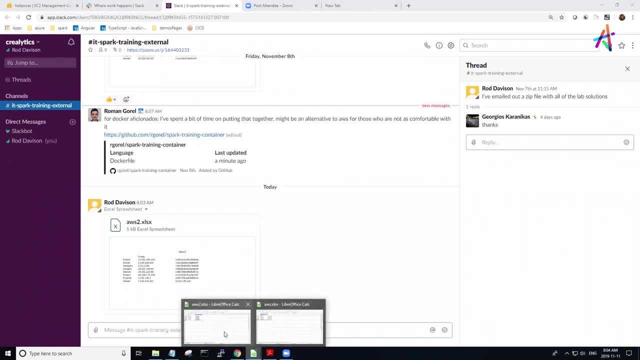 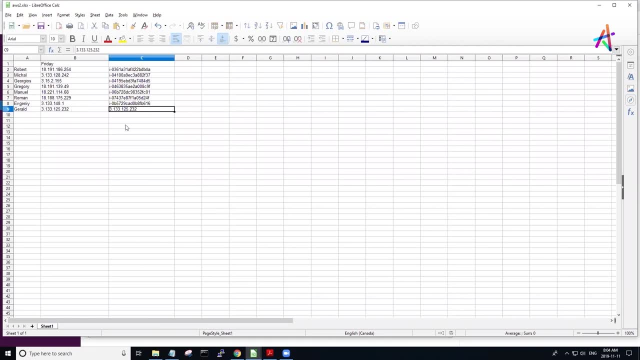 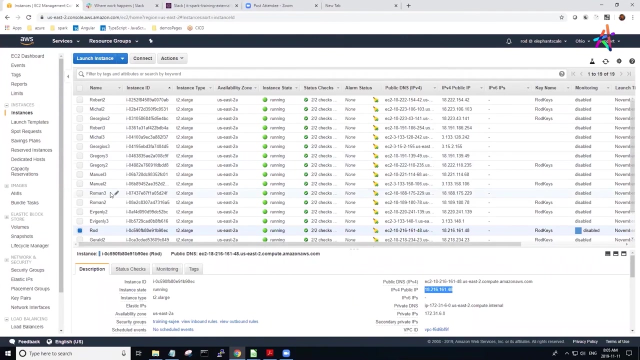 see if this can be fixed. I don't know, i can't see them. okay, go ahead and do it. which, which machine was that? uh, gerald, the very last entry. they want anything? oh, I didn't put the IC, IC, gosh I here. I thought I was actually doing better. okay, uh생, let me, let me. 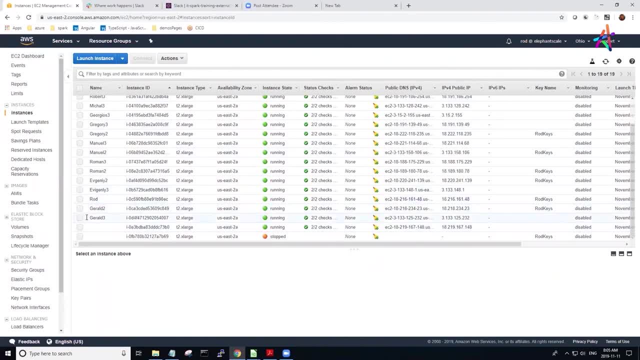 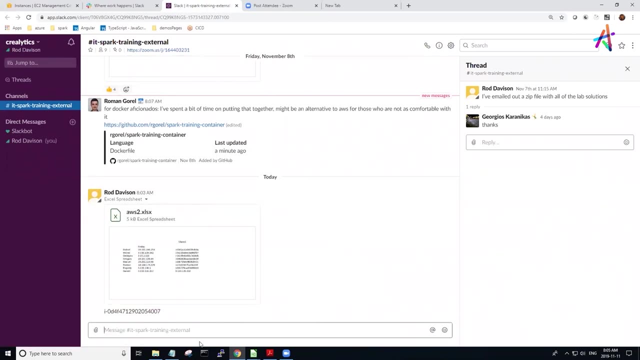 fix that for you right now. that is, Geralt, we'll grab the instance ID on that. and Gerald, I'll just pop that instance ID into the slack channel so you can. you can grab it from there. my apologies on that, there we go. so there you go. if anybody else is in any of the issues, let 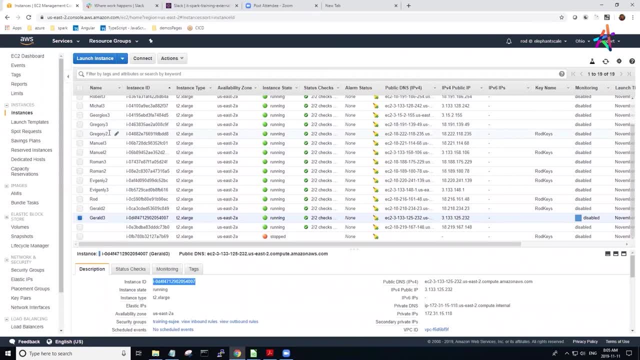 me know. okay. so, Gregory, speaking here, I'll keep my old VM. thing works there. I connect, okay, so your old VM is fine, all right. yeah, 235, no, what which one know it? then just me check the IP I used. yeah, the IP ends with 235. yeah, so this one I. 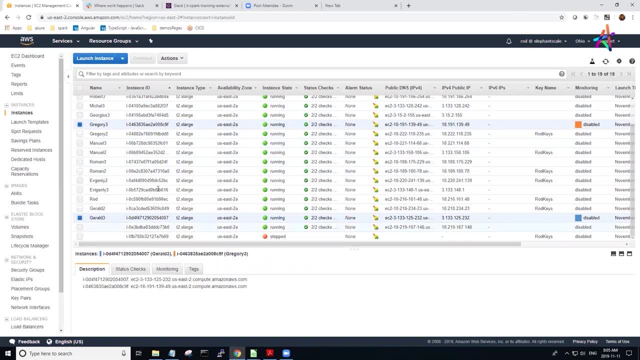 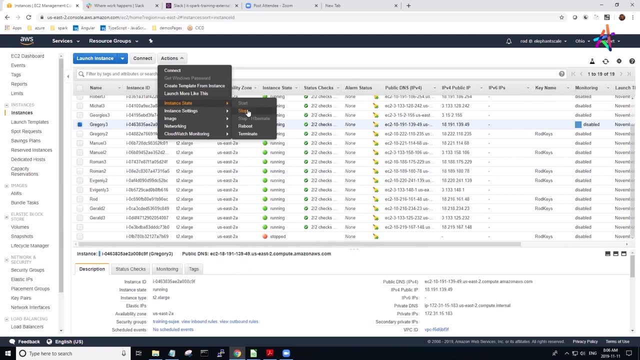 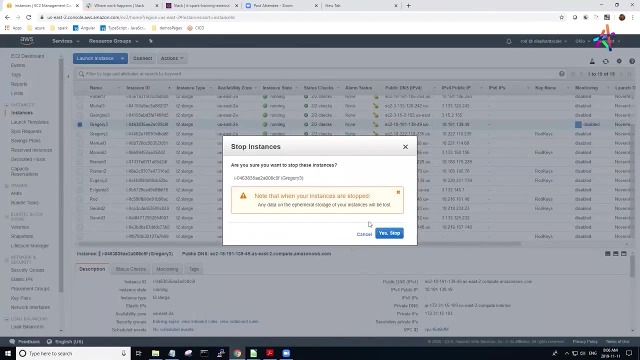 keep, okay, okay, so I'll just shut it out. I'll just check which one is only. yes, yeah, absolutely off. your old one for now, Or your new one? Yeah, the new one. yeah, All right, Roman speaking, and doesn't let me in. actually, 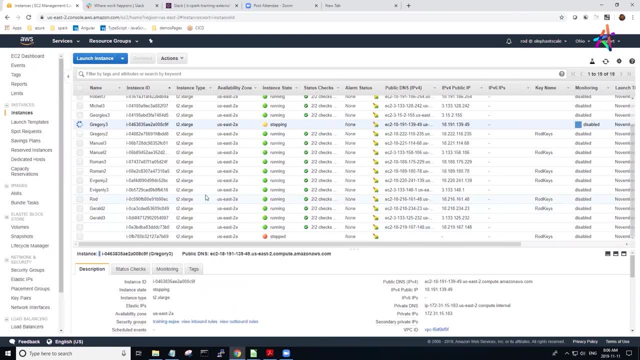 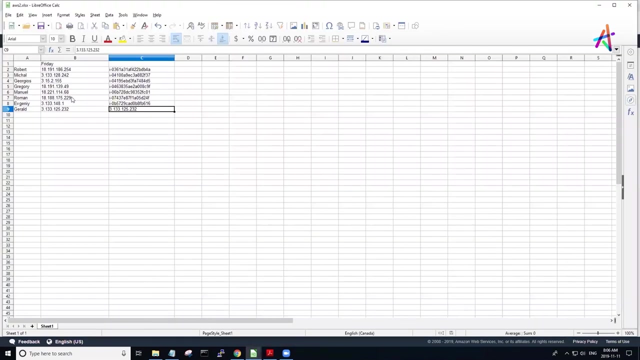 so I entered the password and it asks me for a password. Who is that Roman? Roman. This is for the new one. Yes, Okay, let me see if we got the made a mistake here. We may have. Let me double check this Roman you should have, uh, 18. 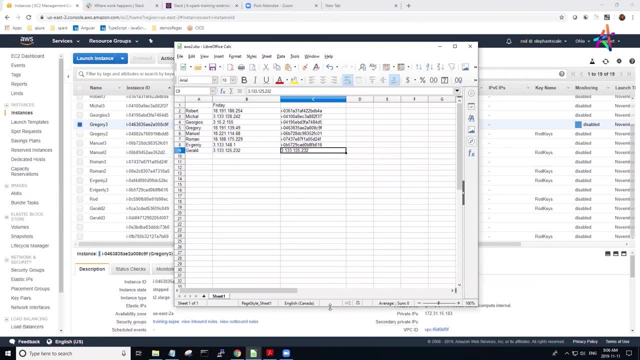 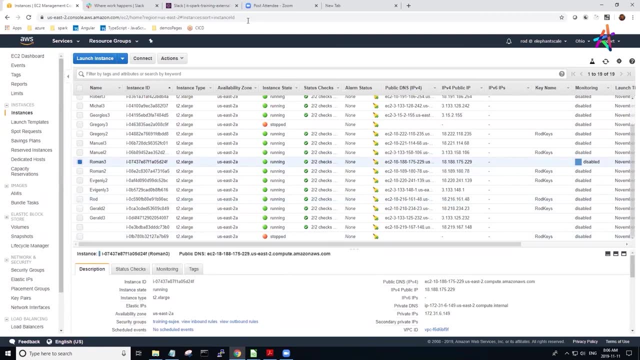 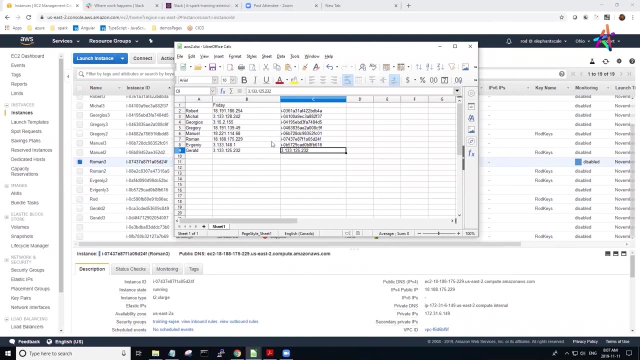 so for Roman, hold on here, do it this way. Okay, So for Roman, we should have 18883 and we should have, okay. uh, looks like the information I sent you was correct. Okay, And the username is still Ubuntu. right, That's right. 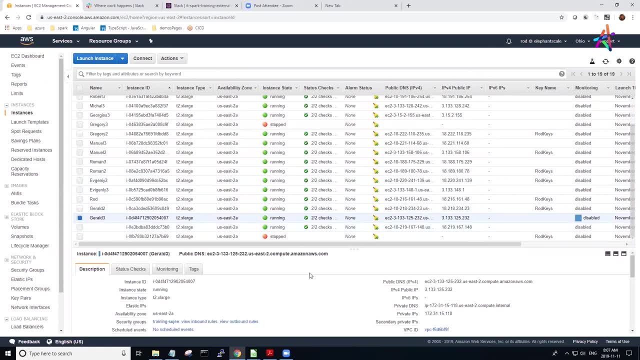 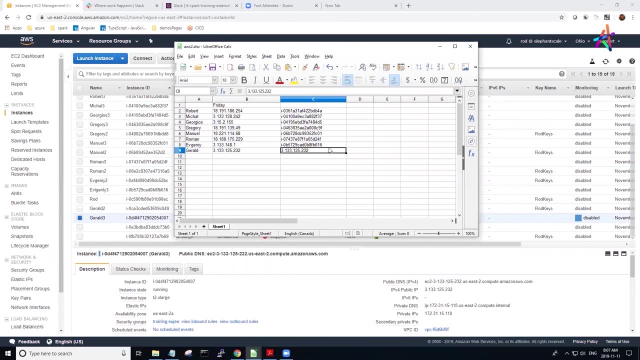 Okay. Oh, now it was successful. Oh, it was okay. It just heard us talking: Yeah, I don't know what happened, but now it's okay. Yeah, I know that happens a lot with technology, doesn't it? It's supposed to be our servant, not our master. 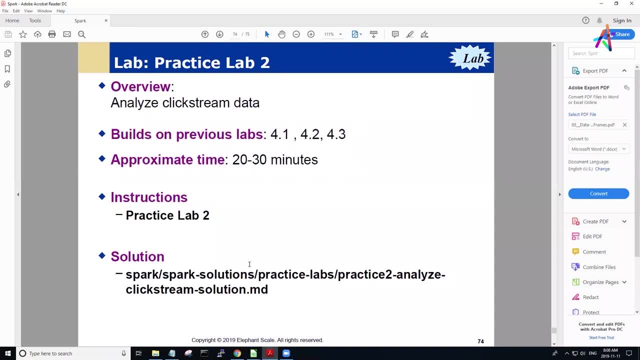 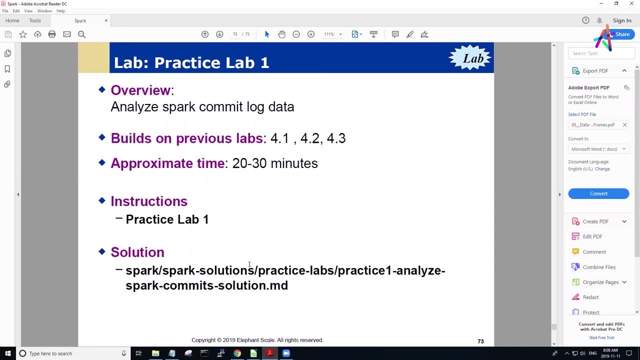 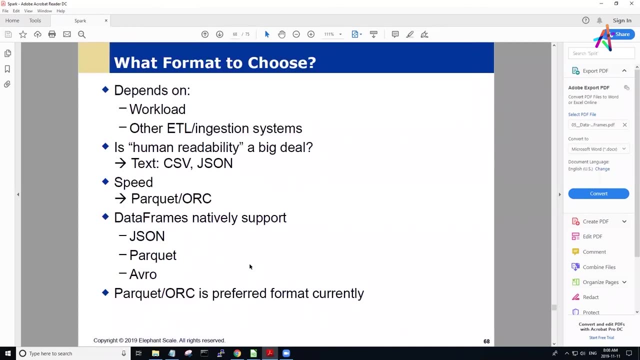 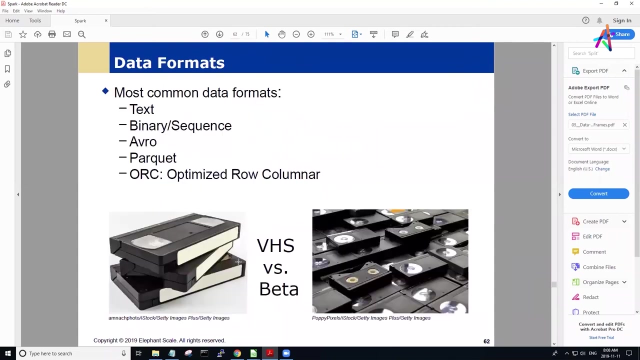 Okay, all right, Uh, okay, so now, uh, uh, well, we're gonna. we're gonna start with kind of a little sort of review of where we, where we picked up. uh, we've had a lovely weekend, uh, and uh, we all just gonna kind of do a little bit of an overview before we jump. 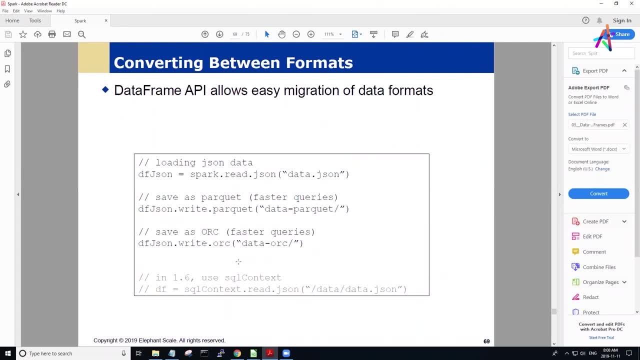 on to our next section. um and uh, we also have some opportunities to play around a bit more with labs. now I, uh I am obligated um by the nature of sort of my, my, my obligation um to my people paying me. I have to uh give at least a cursory coverage of of the components. 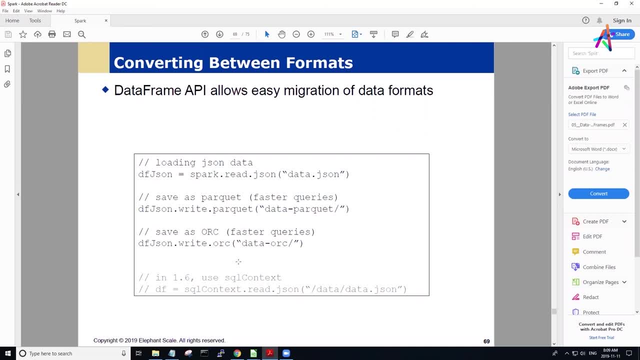 of the course, but you'll notice that we haven't been spending a lot of time on things like Python, um, so there are some sections about applications. we're going to go through those really quickly, because what I am intending to do is to introduce material, uh, particularly around the interest. 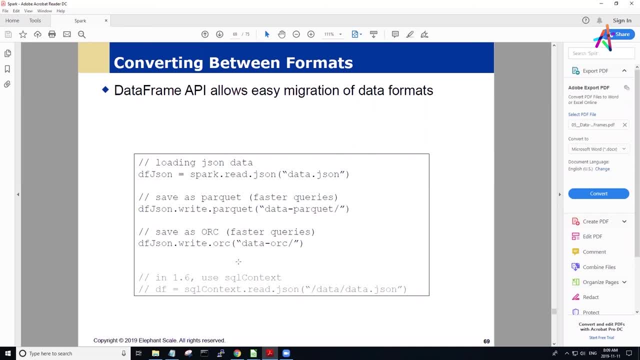 of you guys on on uh, Catalyst and and tungsten. so, um, that is stuff i'm going to be be sort of adding, pulling off of some, some different sources. uh and we'll. we'll talk a little bit about some of the other things, like bucketing and. 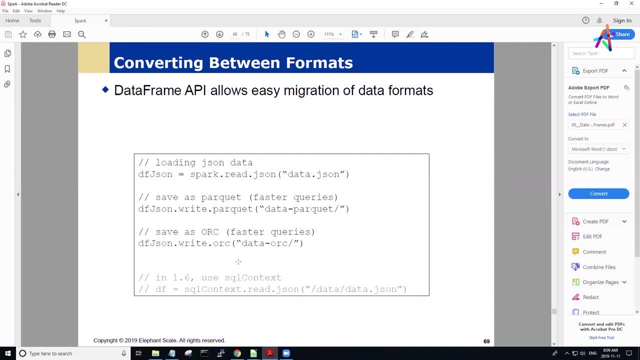 and uh, some of the uh, some of the procedures that are kind of circulating out there in the world around, uh, some of the things we do to avoid certain kinds of shuffling and uh, how to manage things like large joins and and some of the, the pain points that we often get in there, but uh, 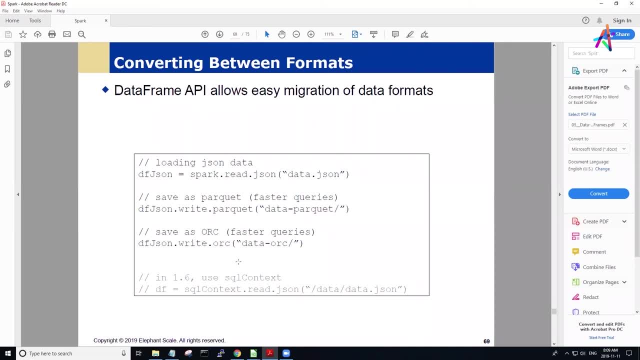 we're, we'll, we'll, we'll kind of add those over the next couple of sessions and uh and uh make sure that we cover off a lot of those topics like: so that is up, hopefully by the end of this session, uh, on wednesday when we leave, you'll have a pretty solid understanding of what's going on with. 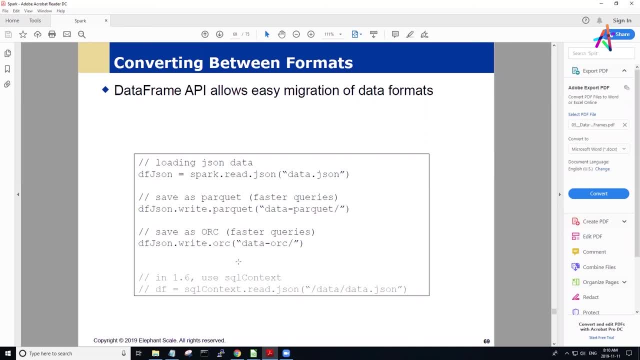 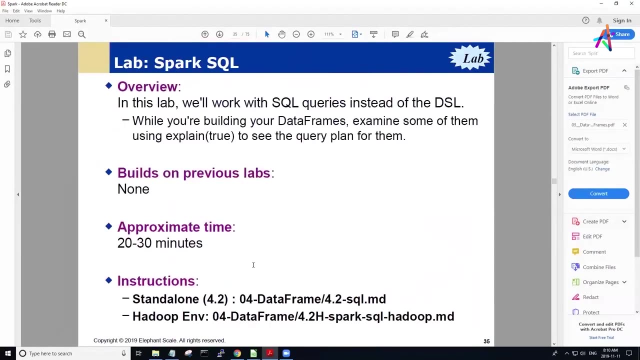 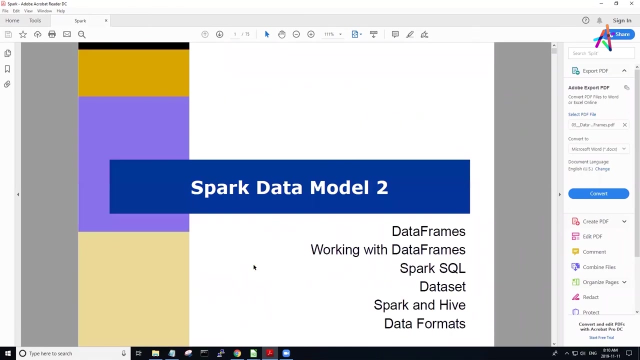 tungsten and catalyst and what all of the things are that are happening under the hood, so you can sort of build an experiment from there, all right, so, uh, the first thing that that i was just going to to. uh, well, i'll just going up to the one up here, to the start here, um and uh. uh, we had talked about rdds with the 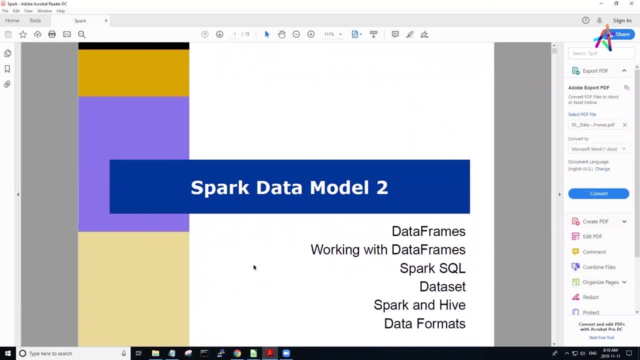 and i'm not going to go back and pull up the slides on that, but uh, we talked about rdds as this kind of structured format, now rdds. um, i i've uh, i've been kind of curious as to as to the amount of support that they actually have, and 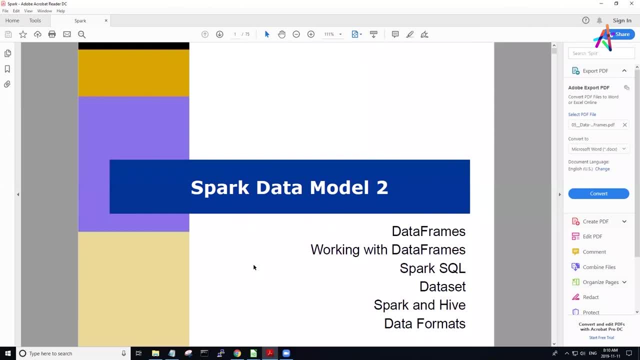 generally. uh, there are some special use cases for the classical rdds, but but normally they're pretty much uh, um, deprecated in the certain sense that the kind of uh data set, uh uh that that has been evolved, uh pretty much does everything that the rdd can do. 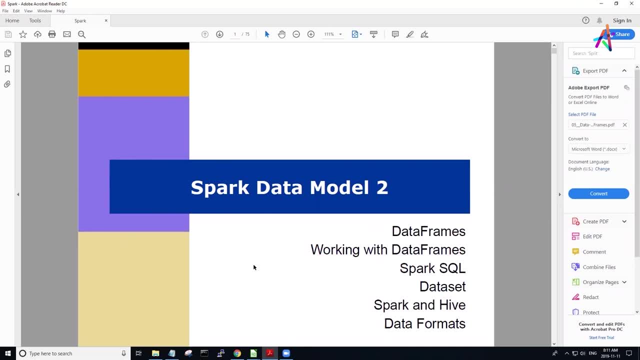 it offers the same interface, but it operates much more efficiently. so the uh, but the underlying concepts there are are are very different, and i'm going to go back to that and i'm going to are- are fundamental in terms of how we interact with them. so the, the things that we discussed- 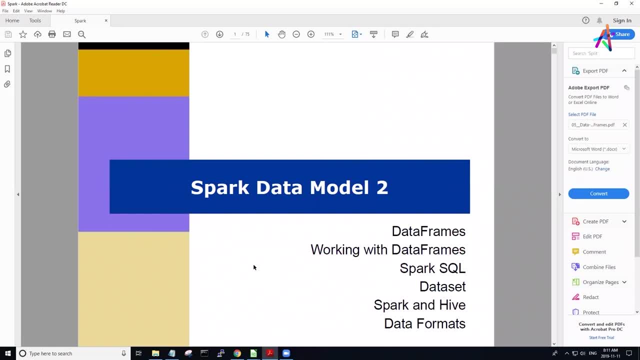 earlier were, were the important part about uh, about how spark was functioning. that we talked about was the um, the directed acyclic graph, and this idea that the transformations are not executed until an action occurs, action being defined as anything that returns something other than an rdd, so that there's an optimization play uh process that can take place. 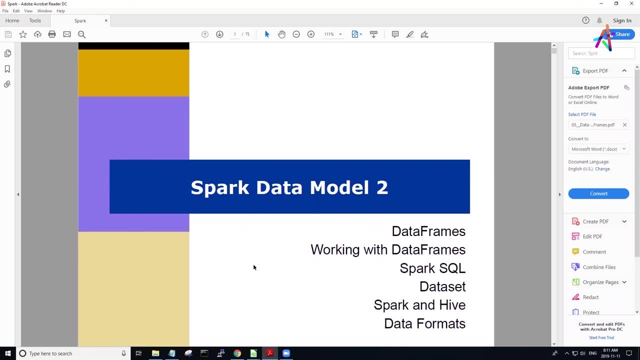 so that is fundamentally uh, the, the, where we introduced the basic architectural idea that that spark had up until about, i think, was spark 1.4, 1.6, then we, then we, then we implement this, this uh data frame, uh, uh concept, uh, which is the idea of rdd plus schema, uh, one of the one of the. 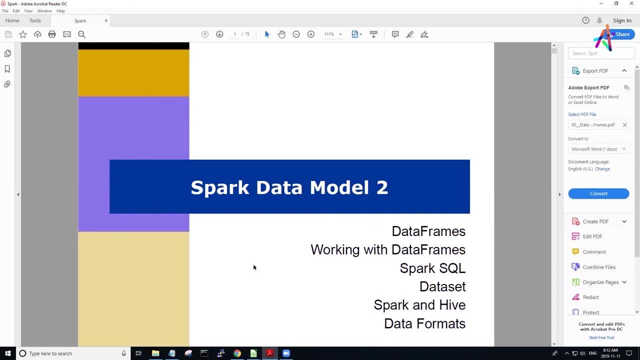 drawbacks to the rdd was that you couldn't do certain kinds of optimization because the rdd itself was open to the rdd and the rdd itself was open to the rdd and the rdd itself was open to the, to the, to the uh, to the uh, to the optimizer. 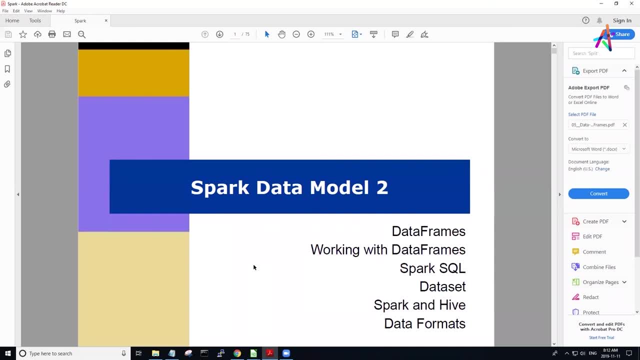 so you were limited in what we could expect, uh, spark to do for us. the other problem that spark was running into- uh, you know, or this, was this notion of being in memory. and again we have to keep in mind that there's two different things we're talking about memory. one is: is the memory. 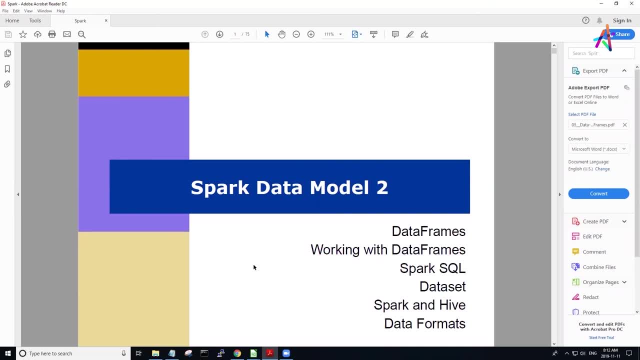 that we're we're we're talking about in our uh, master node, where we're running this soprac Spark from, versus the memory in the various worker nodes And we are given the fact that it's all running in JVMs. we had problems with actually being IO bound And one of the papers 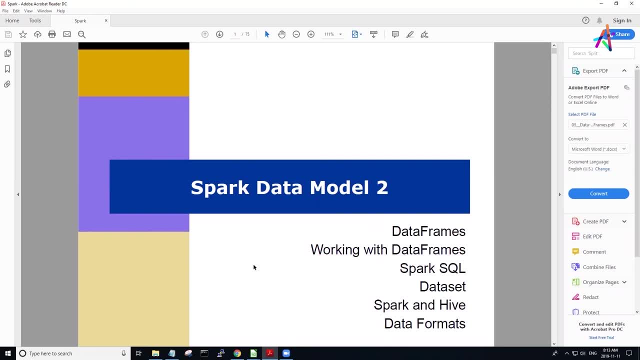 I was looking at a while ago was pointed out that, even with memory only, even with memory only storage, one of the bottlenecks that Spark was running into was the latency between moving data from memory into the CPU, And so one of the things that Tungsten does- 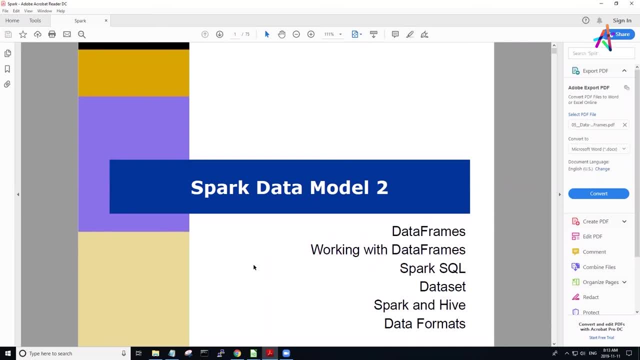 is utilizes caching memory, the L1,, L2, and L3 caches. It actually optimizes the storage in ordinary order to cut down on the transfer time between memory and and and the CPU, which is which I thought was a really interesting little innovation. so, as we 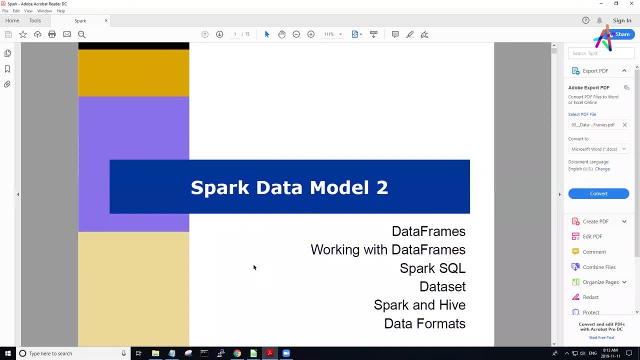 come into data frames. we're now putting structure on there which allows us to be able to start doing optimizations. this is where catalyst comes in. and then, with the introduction of typing, which allows us now to do much better allocation of memory and much better serialization, and again with the, with this, data sets. 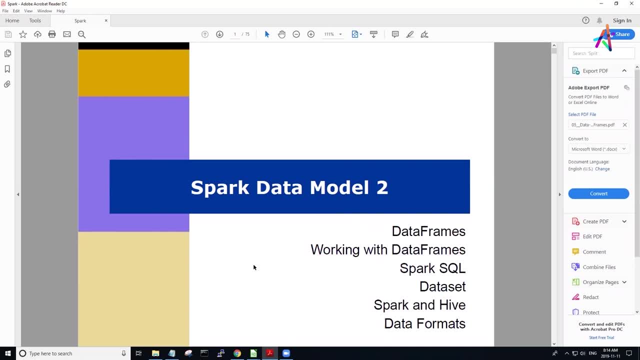 we're now really looking at two. we're really looking at two interfaces into an underlying structure which is being used from either the point of view of a data frame or a, or the point of view of a of an RDD. now you can see here that we've got a lot of data, that we've got a lot of data. that's. 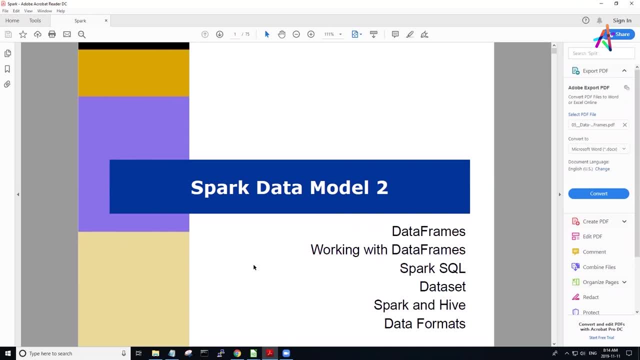 the excuse me. the overall approach to, to to a spark is to is to look for places of optimization, keep as much things in memory. avoid. avoid relying on a lot of disk IO but also being able to delegate a lot of the. the actual distribution of the, of the, of the partitions of the. 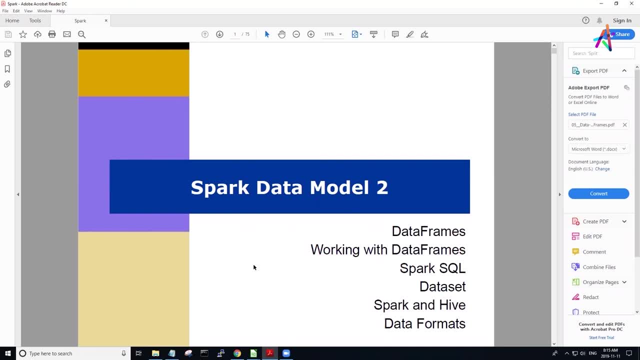 data out to the various nodes. so there's a number of places there we want to look at where we can optimize performance. so the idea has been to keep the API fairly consistent, or at least consistent and easy to use from a user's perspective, but at the same time allowing us to to to have opportunities to optimize under. 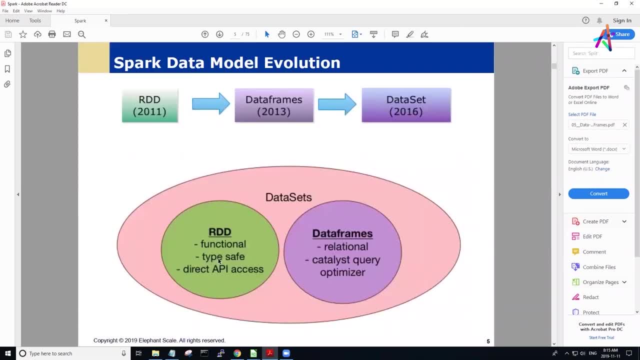 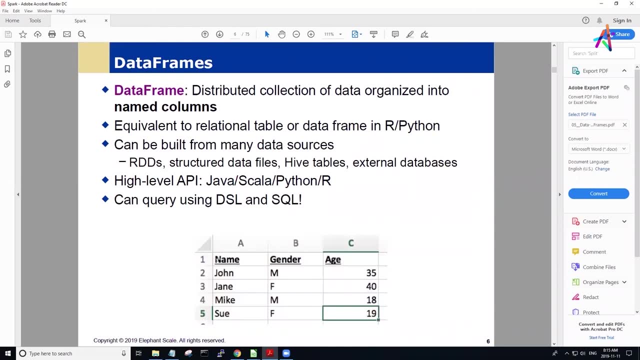 the underlying architecture. so this was the idea of data frames, then data sets- a um data sets- coming along to provide the unified interface. i was watching one one video at one of the spark conferences and somebody was saying that if you ever decide to go back away from data sets, 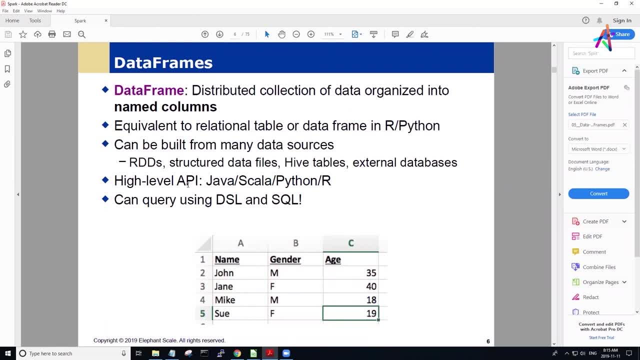 you should be consider retiring and just taking up farming or something. so this apparently has got a lot of um, this is, this is really sort of the the uh, the, uh, the, the direction in which future optimizations apparently are going to be built. um, so we discussed, uh, the data frames. 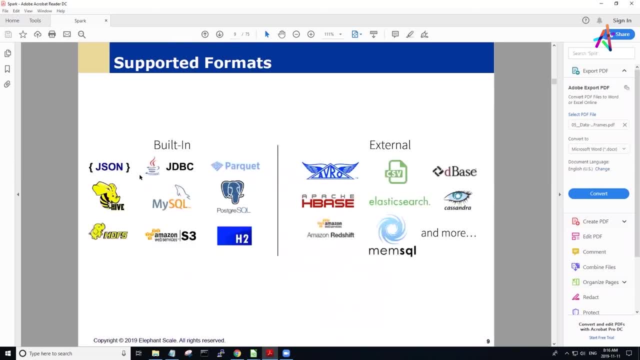 and the um and the uh, the uh um ability to um to be able to start to use sql type queries and manipulate data based on columns, the, the um. everything that i've been seeing uh suggests that this uh parquet data format is increasingly becoming the recommended one for. 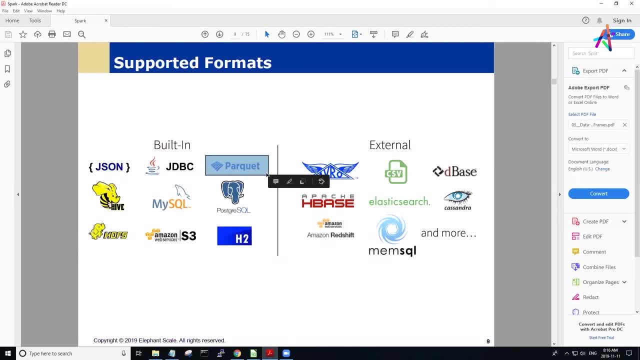 um, uh for, uh for spark. now, uh, when i actually started this course, uh, i had not actually used, uh parquet and i didn't really know an awful lot about it. so i went and i started looking, uh, reading up some of the technical docs on parquet and i was very impressed. 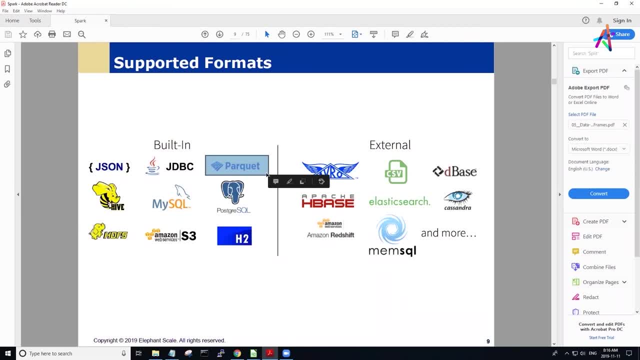 uh, this is a data format that has got an awful lot of of a very impressive design to it. uh, and the way it stores the columns and the data, and how the data is serialized and deserialized. uh, so one of the the optimizations does certainly seem to suggest itself, and one that i was not fully 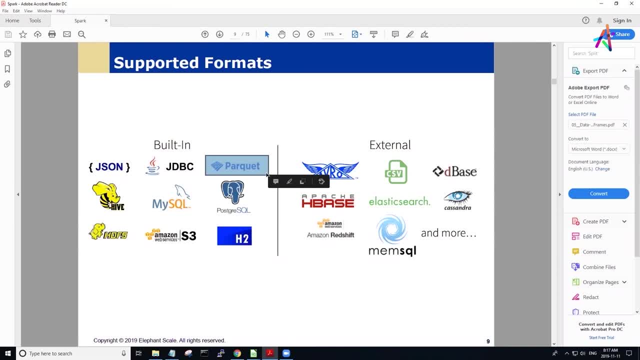 fully aware of uh is that the choice of the, and i've been also coming across items where, where the, the real gurus in spark, are suggesting that, if you want to look for certain kinds of optimizations, that parquet may be a data format, particularly with regards to serialization. 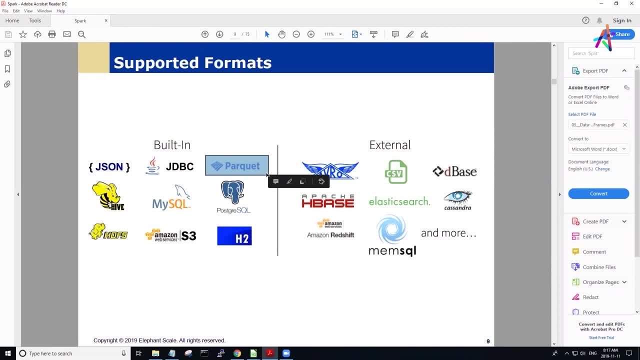 uh has much better serialization than than some of the other data formats. while all of them work well, parquet does seem to be one that has uh. that has certain uh uh advantages that can be utilized by by spark. so just keep that in mind as a little. 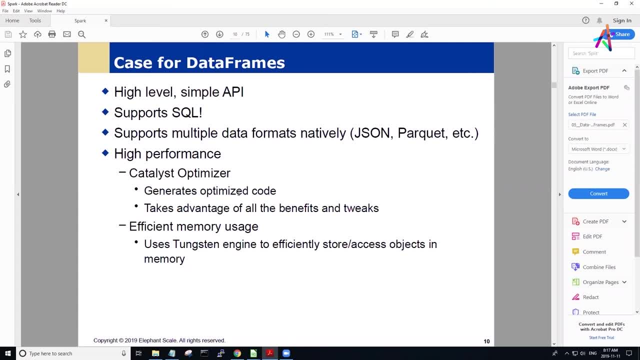 tweak. hold on here, i've got a. one of my devices is beeping at me. i'm going to have to turn it off. there we go better. uh, so oops, we're going to get more into the, into the details of tungsten, uh, either today or tomorrow, but we'll certainly take a get into it by tomorrow. 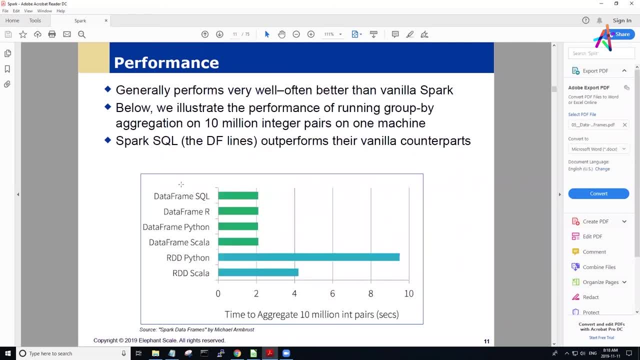 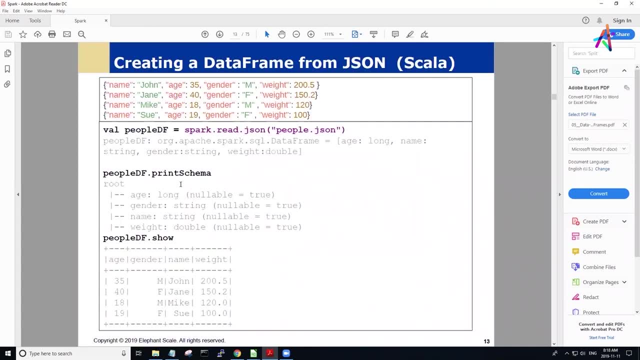 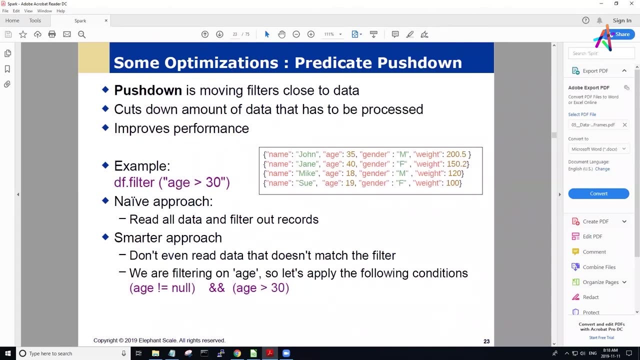 uh and uh, then uh again. when we look at at the at the, uh, at the, at the performance- uh again. we've seen that before, so we don't have to worry too much about that. we took a look at the at uh, basically the data frames, data typing, um. and then we started talking about some 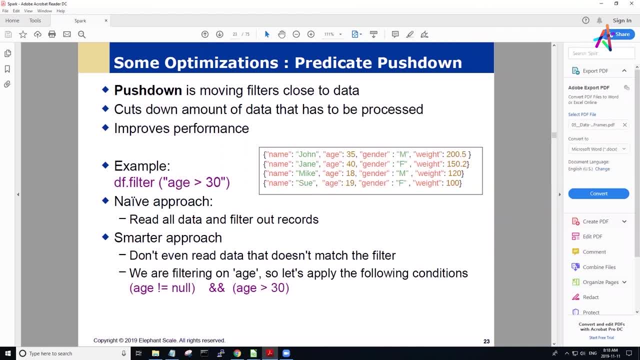 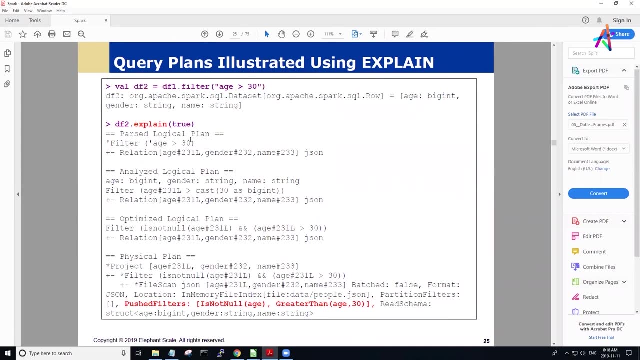 of the optimizations and and how we can do optimizations, uh, particularly through catalyst that does things. in the example we looked at as predicate, push down uh, where we were, instead of reading all the data in, we, uh, we filtered the data so that we cut down on the amount of of data we actually keep stored in memory. 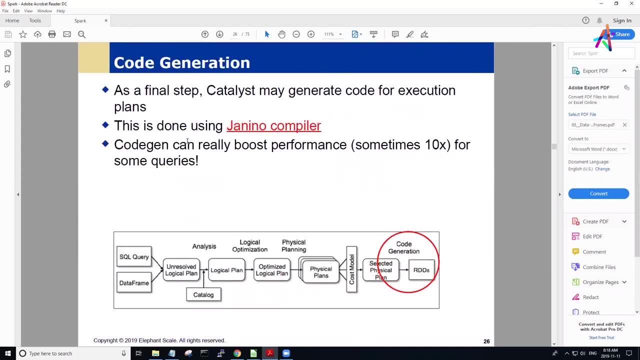 um, uh, and then we actually have uh, have, when we have uh running through catalyst, uh, and we'll just remember. this is a point we're going to come back to. so just worth remembering is that we we wind up with an unresolved logical plan, and that unresolved logical plan is just basically. 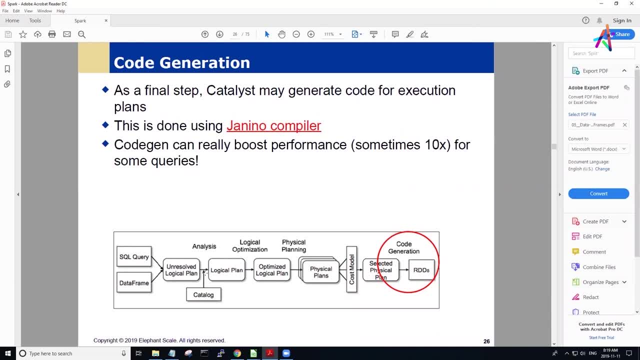 your statement. the resolved logical plan is when you go and you add in all the information from the catalog about the structure. that's optimized- and we'll take a look at some of the optimization rules that are used a bit later on- and that produces the physical plans. 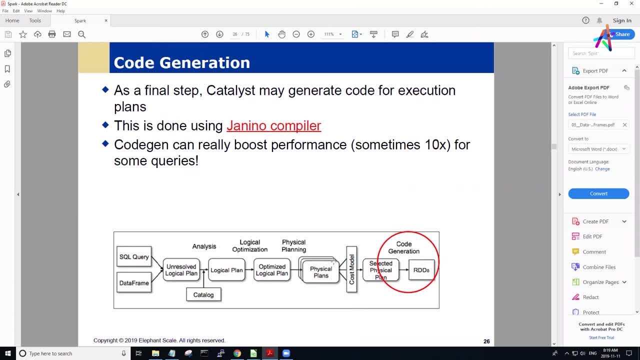 each one of them is then run through a costing model to determine how, uh how expensive each plan is in terms of execution, and then from there we wind up with a selected physical plan and then from that plan we actually generate the code uh, which is uh often by done through this genino compiler. 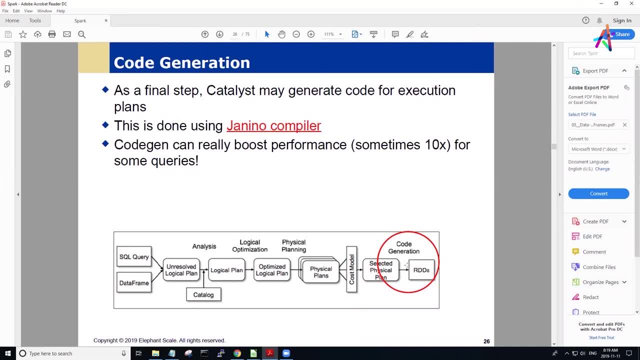 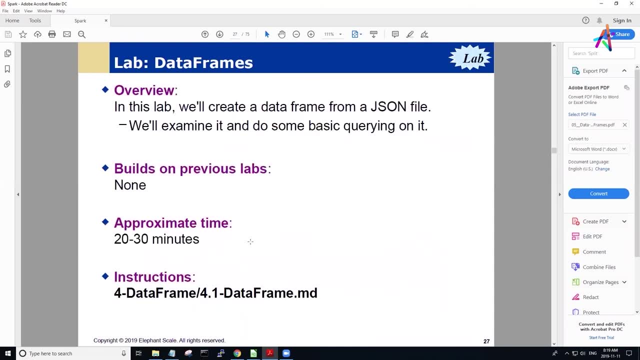 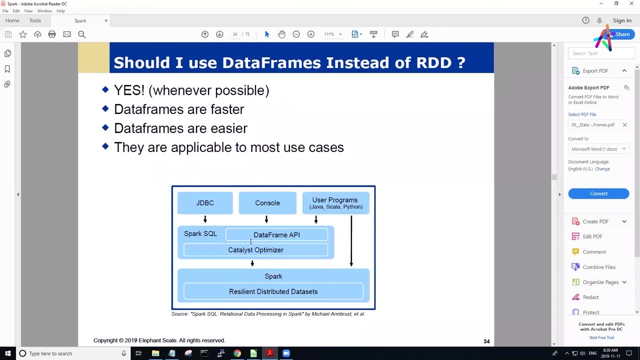 uh and that produces uh, the appropriate uh, rdds that that results from the query. so the idea here is that we have this other point of optimization. i think we did that one quite nicely. uh, we talked about uh, spark sql. um, uh, should i use a data frame instead? 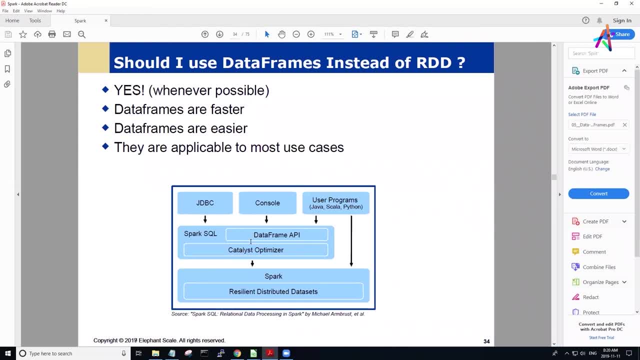 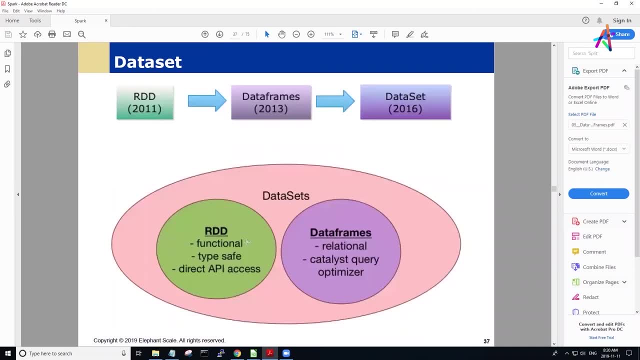 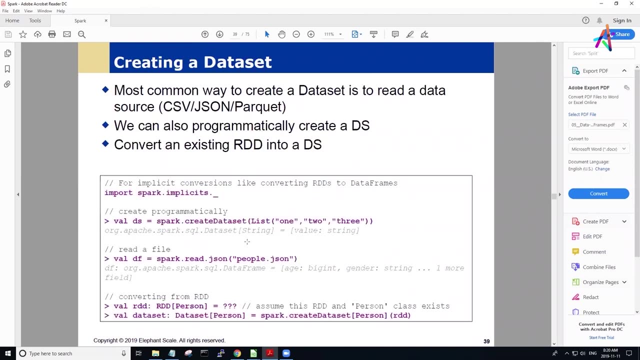 of an rdd. uh, this is not a theoretical thing, this is just a practical issue and this is yes, uh, wherever possible. and again, it remember that this point, the data frame is a, uh, as an interface into our, our underlying data set. uh, uh, approach, um, so, um. 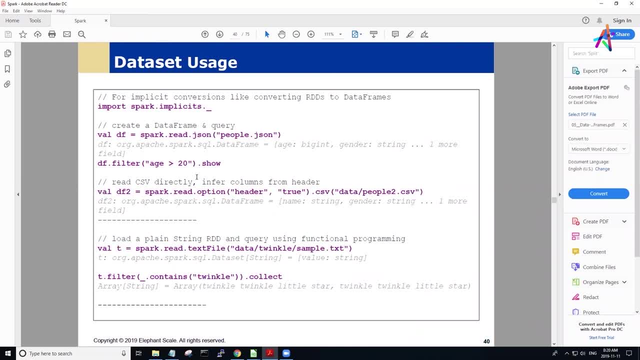 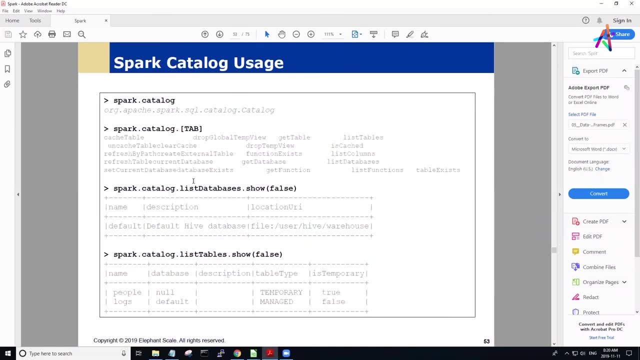 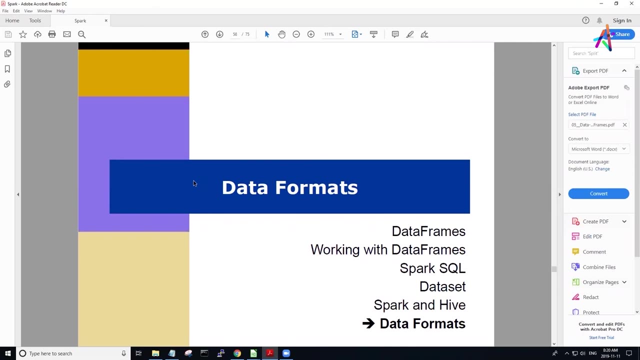 the one. uh, here we go, and we talked about creating data sets from various kinds of things. we're not going to get into into all of that kind of stuff again. uh, we talked about using the various uh, um other other, um other data. uh, you talked about using the other. 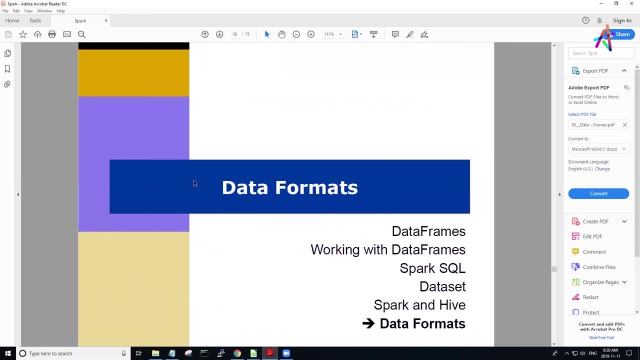 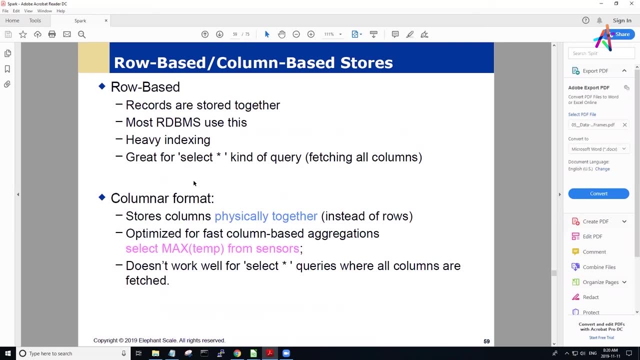 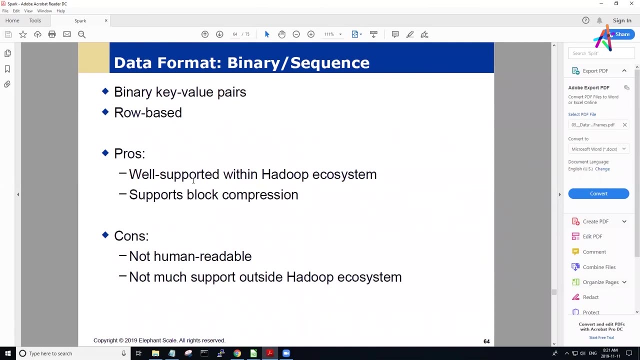 um, or interacting with hive. uh, and it's, uh, it's a data warehousing sql type of language. uh, for data formats. we looked at those again and then i'm not gonna to to go over all of this again, but, uh, just just remind us where we are when we left off. um, now again the. 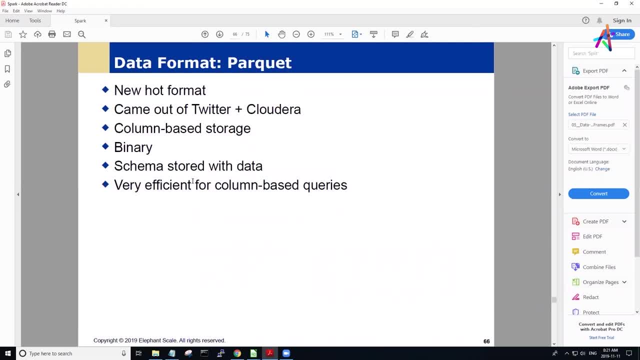 again, parquet, um, this is, this is the one that seems to keep coming up over and over again, uh, from at least the, the kind of technical things that i've looked at, that suggests that this is really, if you have a choice, uh, to at least experiment with parquet. 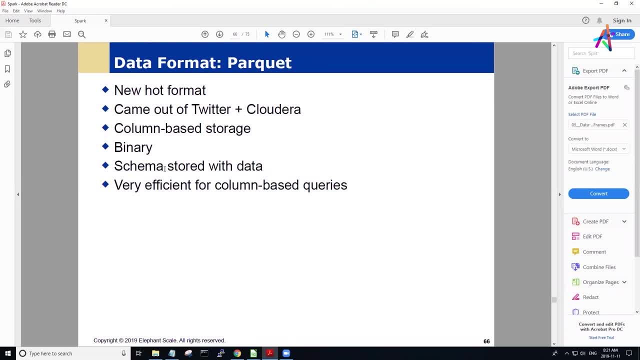 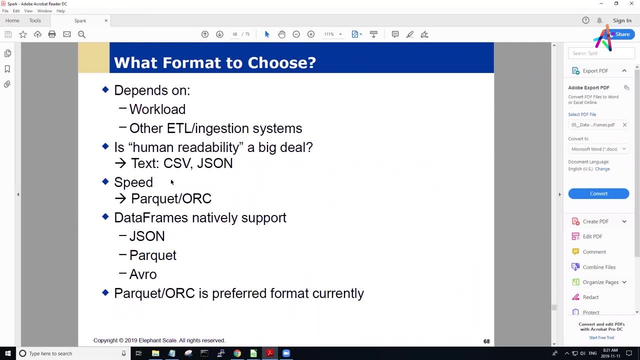 and see if you can uh and choose some optimizations on that. okay, um so, um. so it says parquet and orc. now, unfortunately, i don't know an awful lot about orc, but uh, but i bought parquet, like it seems to come out as being the preferred format. i just didn't realize how. 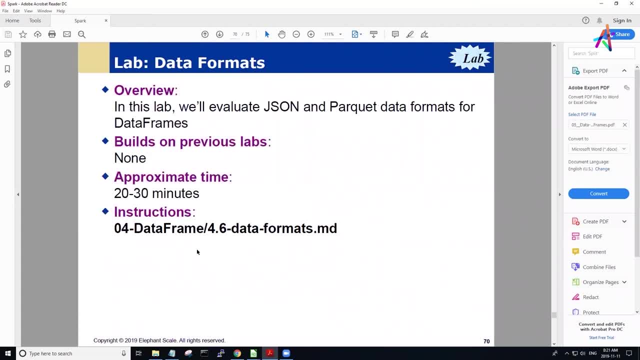 much uh until a little bit of uh, uh, until we got into into that. now, i think we did this lab at yesterday or on friday, didn't we? i think this is the one where we we ended at i i, i think we kind of concluded our day on friday with this one. if i'm wrong, please. 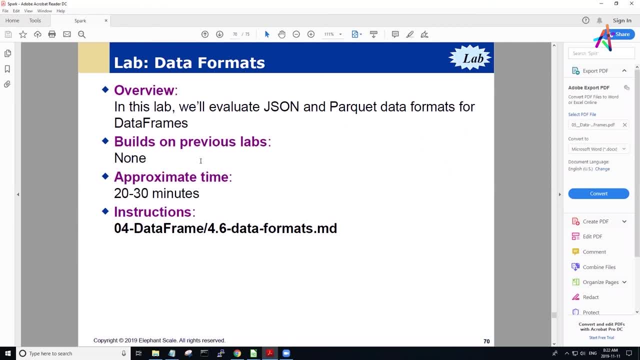 you know, let me know. yes, we did this one, but you wanted to look into the previous one, the spark hive um class, because that didn't work on our machines. yeah, i, unfortunately i didn't, because i was spending the weekend being sick, but i will certainly take a look into that as well. 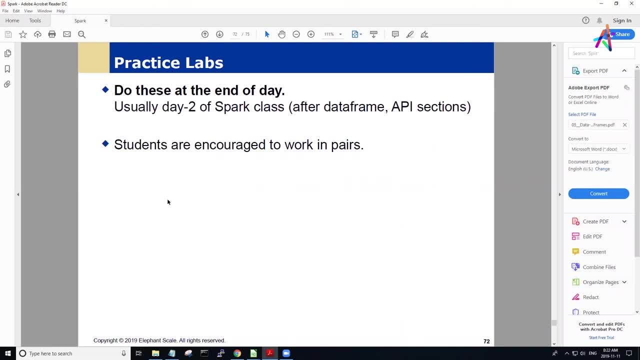 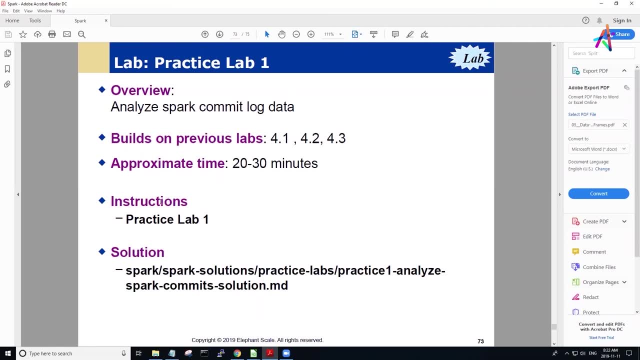 okay, thank you. uh, that's something i have to do, so i will take a look at that today. all right, okay, so now, um, if you wanted to, um, now, these are the ones that are in the workshop. so, um, who are the two participants? there's a couple in the back of a screen. 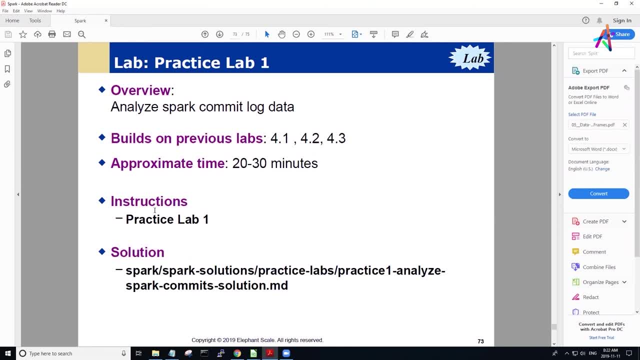 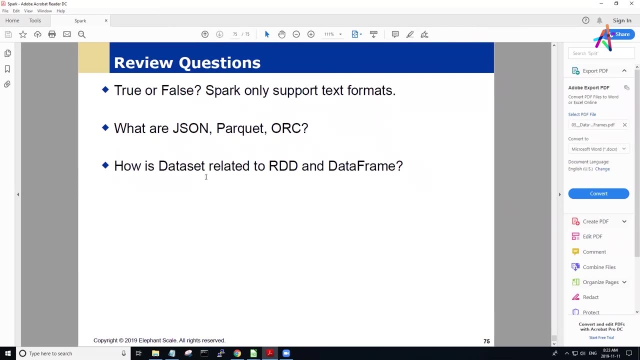 who are the two participants? uh, and i will pass the last bit of the questions to julian, so you're going to start. all right, so it looks like there's um a couple students. so, um, julian, and uh, jackie, are you going to move my slides um? 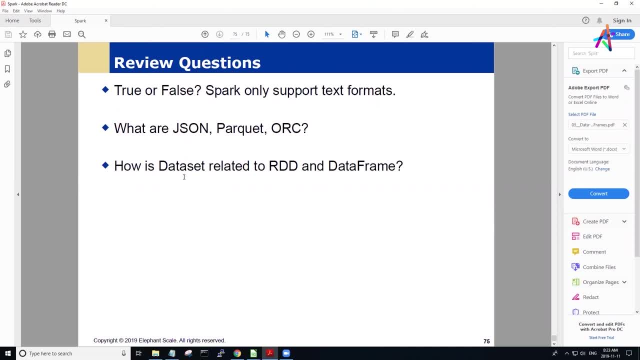 i'm seeing that. um, you don't want me to do that. okay, All right, so any questions or things that you want to mention about what we've done so far, Questions, issues that are unresolved, things that may be still confusing, or things that you need a little bit more information about? 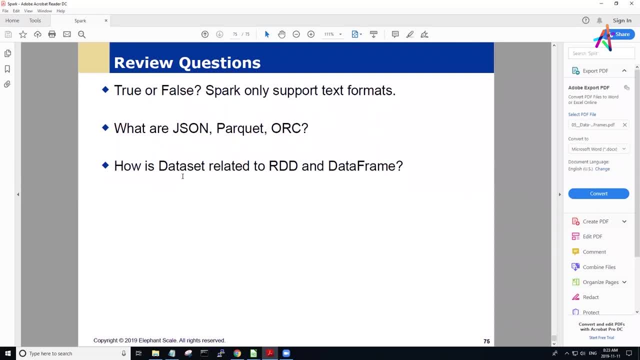 So we do have a question in terms of if Spark is running for quite a while. The previous slide you mentioned something about commit logs. It kind of accumulates quite a lot of logs. Is there a way to automatically get rid of these logs? 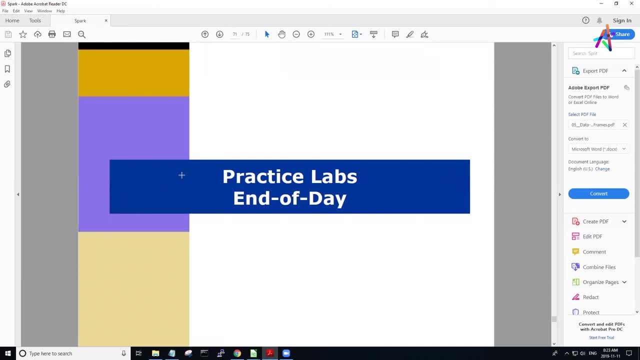 Because if you have long-running Spark applications, it feels like we always have to manually restart Spark to just get rid of these logs, if the underlying resource manager still assumes that it's a running container, so it keeps the logs. Oh, okay, that's interesting. 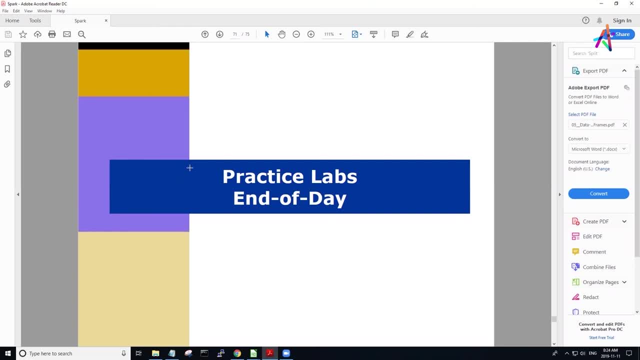 I'm just going to make a note of that and then I'm going to have to check into that, because I don't have anything, I don't have an answer off the top of my head, But let me just Okay, so the question, and I'll get back to that one tomorrow. 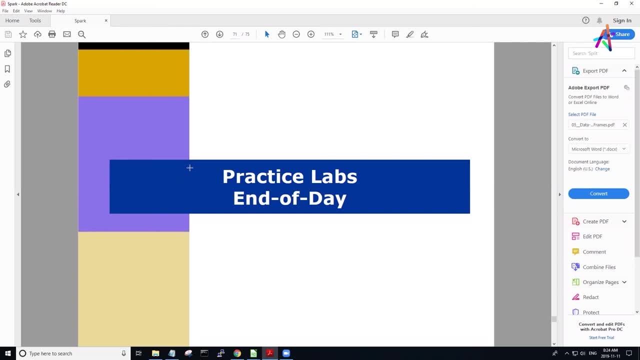 So long-running Spark commit logs- Not necessarily commit logs, but in general there are quite some logs that Spark is accumulating as an application running on top of a resource manager like Yarn. Okay, And even if the application is not doing too much at the moment, for example, 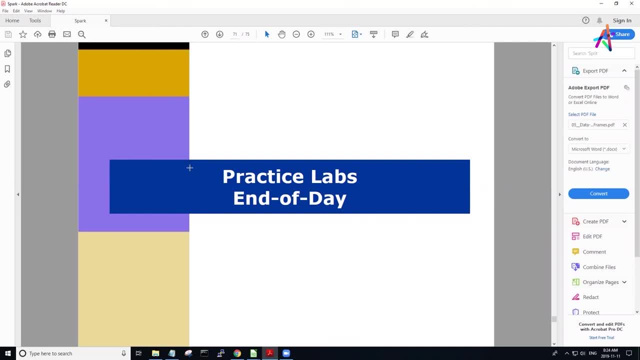 there is no incoming data, then that log is still not cleaned up because the resource manager still sees the container, the Spark container, as a running application, So it still assumes that data is still required. There's some configuration or setting that we can regularly wipe this data. 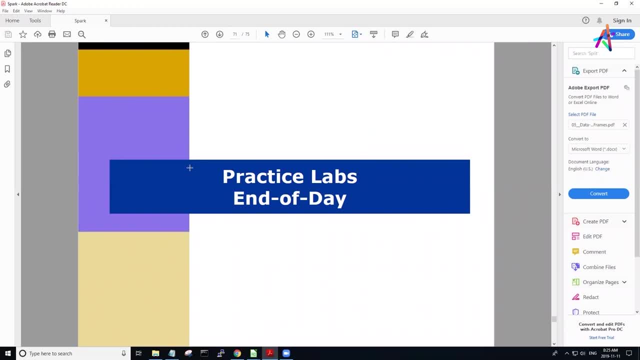 or how can this work? I will check into that for you, All right. So this is especially interesting for us as a streaming application, because we don't necessarily want to shut down the application itself, but want to get rid of old log data. 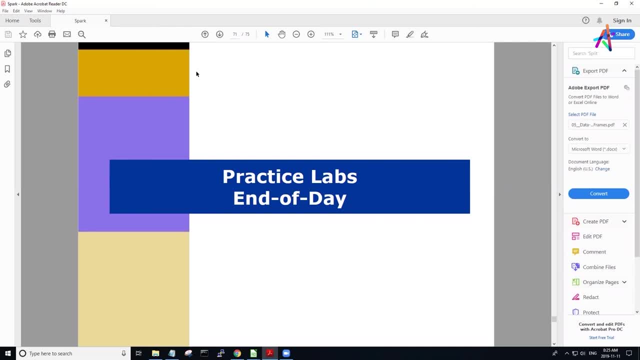 Okay, Yeah, I can see where that would be a bit of a problem. Okay, Well, that is something I will definitely take a look at, okay, Okay, thanks, I'll get right back to you. Not everything I have on the top is off the top of my head. 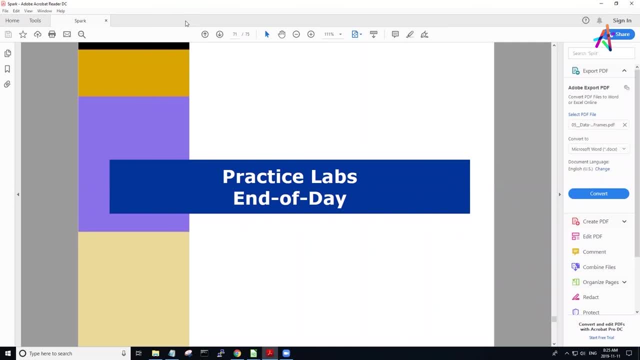 but so when it comes down to some of the details, but certainly we'll take a look at that, Okay. So, pardon me, We're going to go through A bit more theory. That's an interesting question, by the way. 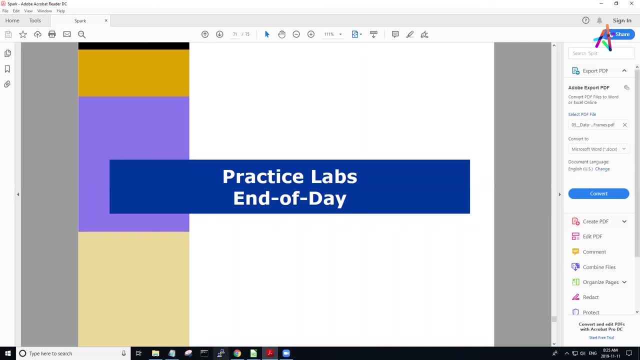 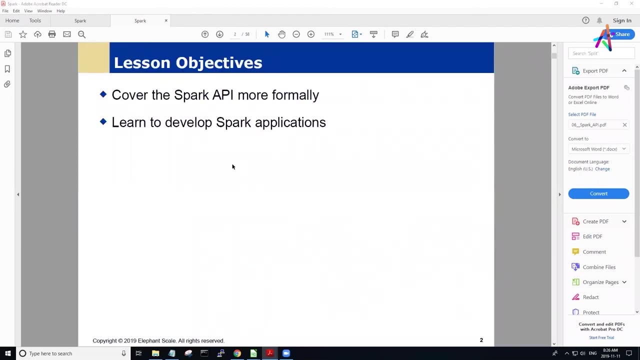 Let me see. We were just. We did that one, So we are now going to come into Dynamo Lelframe, So we're going to do a bit about this Spark API. Okay, So now we're looking at the core API. 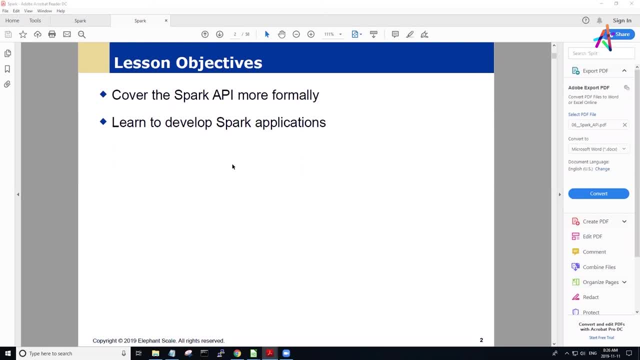 Now, when I was going through these, I noticed that some of the slides are a little bit weird in terms of the titles, but just I think somebody didn't. I'm going to put them in the right order so that they don't affect the actual flow of the presentation. 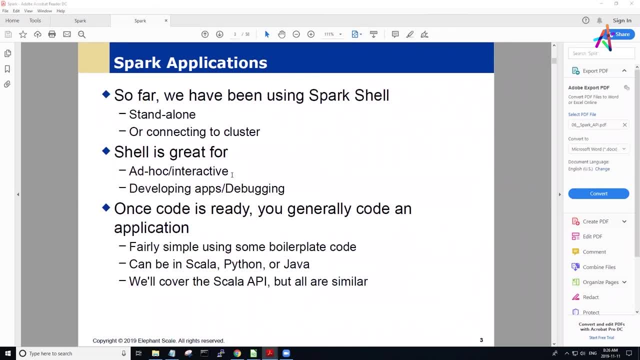 Okay. So what we're looking at here is the modes of using Spark, And what we've been doing in class is what's called the Spark Shell, where we're basically using it in an interactive mode, standalone or connected to a cluster. The idea behind the Spark Shell is this: is: 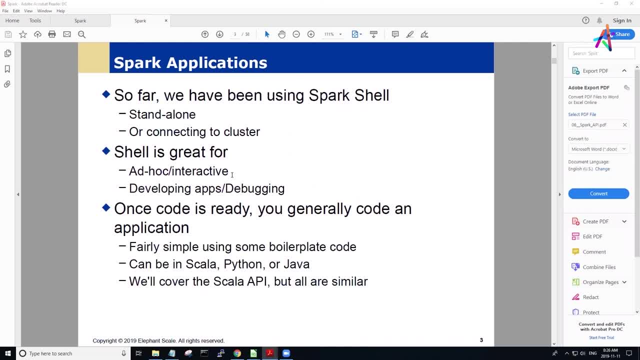 Its role is not to run production jobs, but really It's to do a lot of experimentation, to develop the particular logic, to do debugging, to run test runs to see if things are optimizing correctly And then, once that step is done, 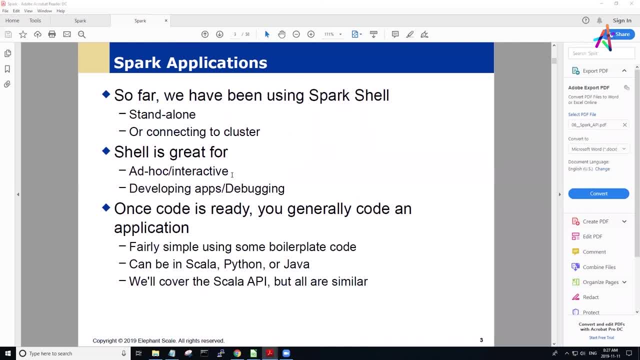 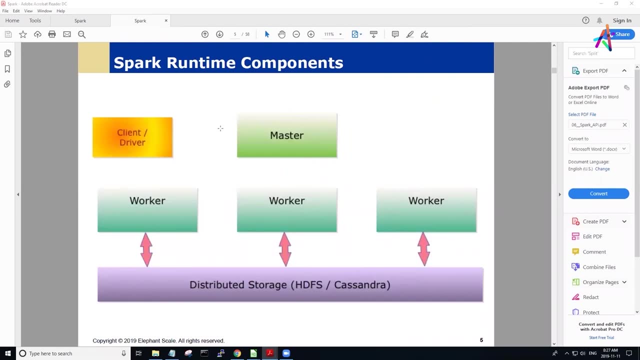 we wind up actually writing an application in one of the interface APIs and then compiling it and running it in a production mode. So the runtime components, just again to remind you, with a client driver, which is where we're interfacing with. 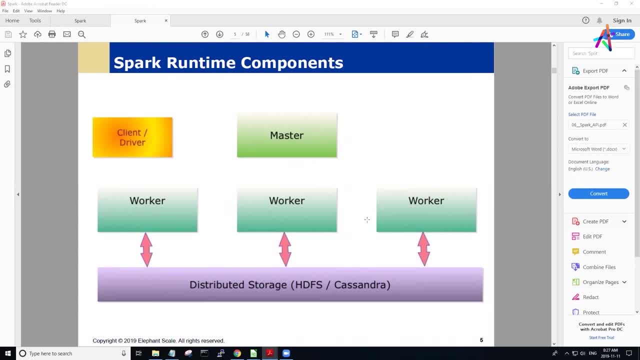 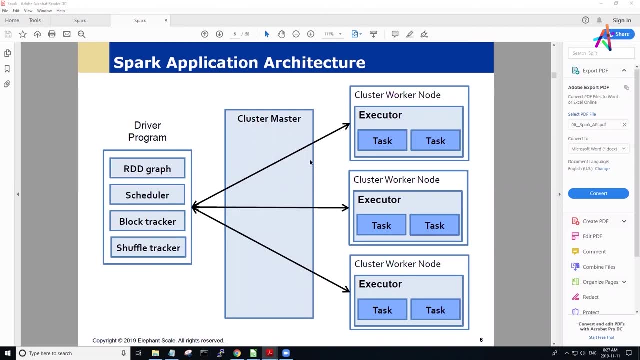 takes on to the master, which delegates off to the various workers which work on the distributed storage, whatever the underlying model is that we're using. So the cluster master is going to be Have most of the tasks delegated to it. The driver program has the various 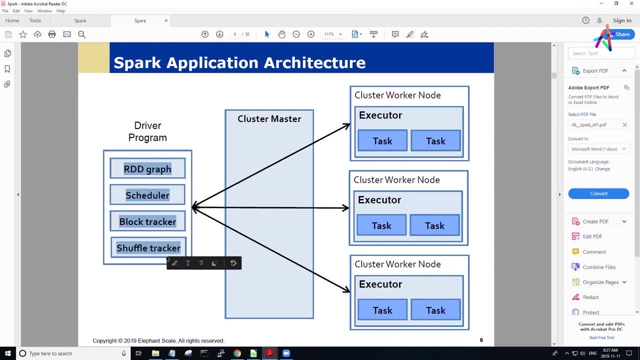 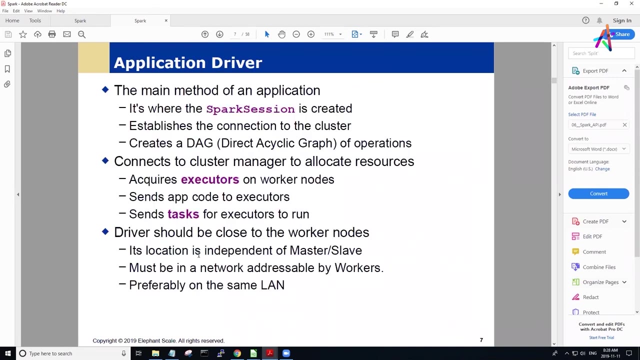 Has the various oversight components which it's using to manage the actual tasks being routed through the cluster manager, which does the appropriate parallelization and distribution out into the various nodes, And where the difference starts to come in is where some of the tasks wind up being allocated to. 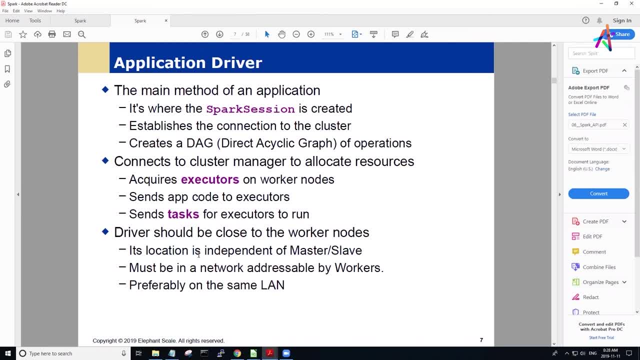 So the Spark session is the entry point into the application, Which does the initialization in the sense of setting up the initial context that we're going to be working out of, Establishes the underlying infrastructure connections to the cluster, getting into the data and is also creating this graph of operations. 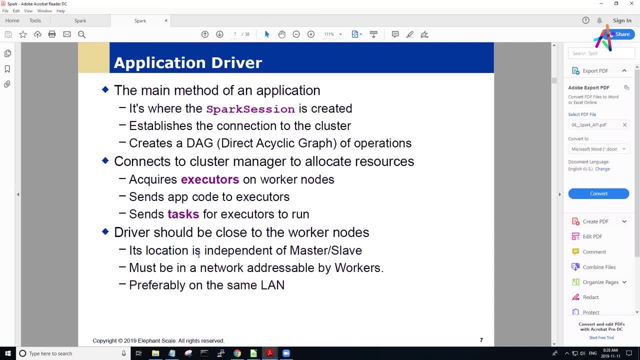 When it connects to the cluster manager, it actually Is getting the executors on the worker nodes And those things that are created are then being delegated, or getting the code delegated to them, where they're then getting the tasks to run. Now, to remember our terminology: 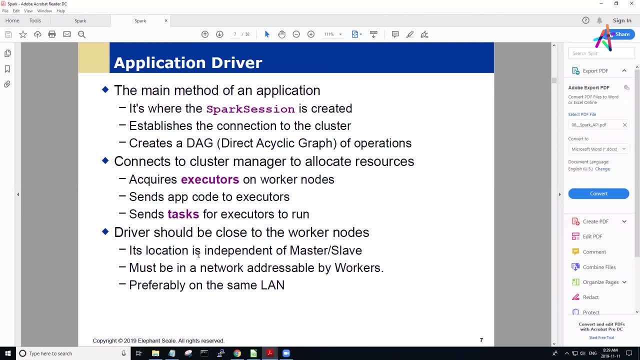 a Spark application is when we open a Spark session. When we execute something, we have a Spark job, And our Spark job may be Consist of a number of stages, And each stage is where we don't have to do any data shuffling. 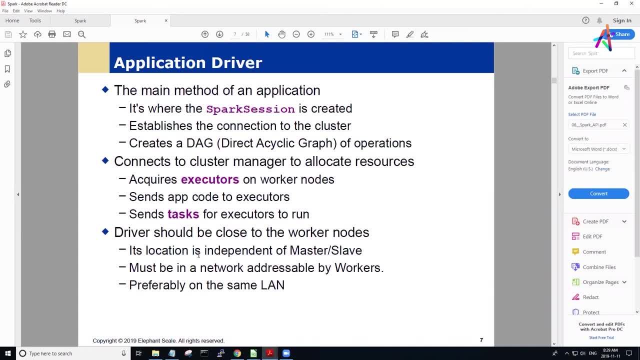 When we do a shuffling, we have to do a different stage. We start a different stage in the job. Within each of the stages, you have a chunk of work, called a task, which can be executed inside a single, Inside a single. 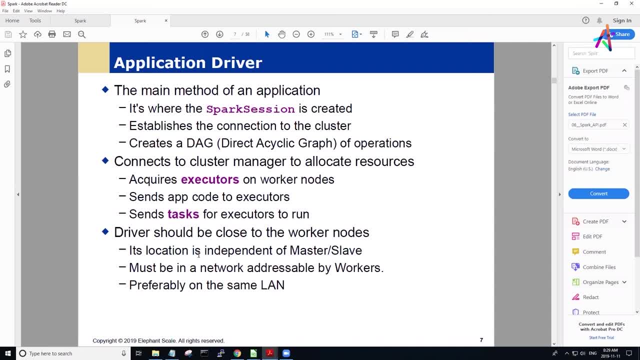 A single executor. So as long as you don't require a reshuffling of data, then each node can perform a series of tasks. So the terminology is: tasks are things that are run on the nodes within a stage, So the driver should be close to the worker nodes.